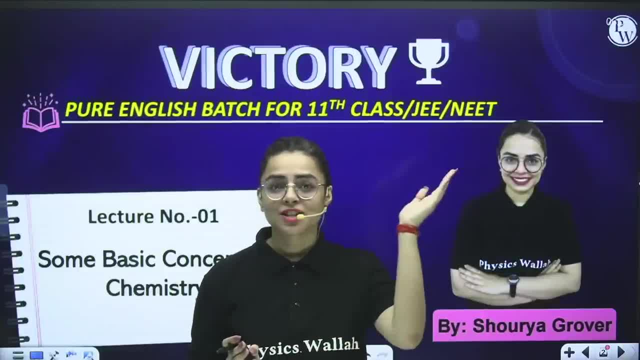 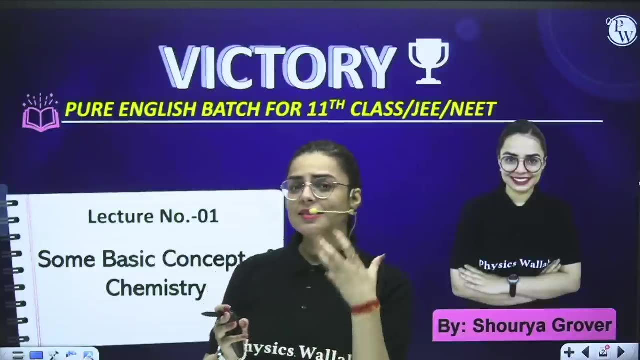 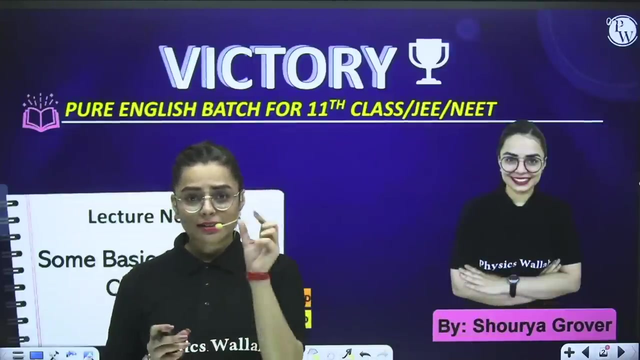 Students. as Victory Batch says, The harder the battle, the sweeter the victory. So now, with this quote, we will start our first topic: Students, as the name suggests, some basic concepts of chemistry. So I would say that there is a word basic in this. 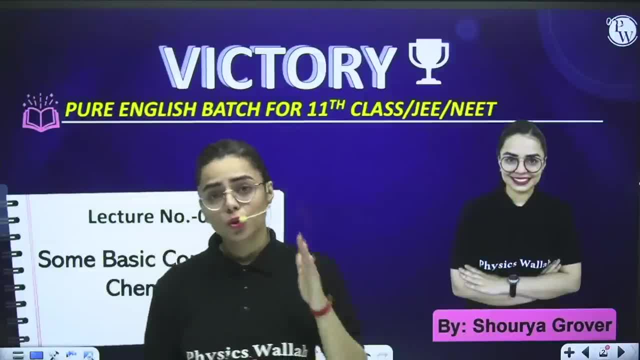 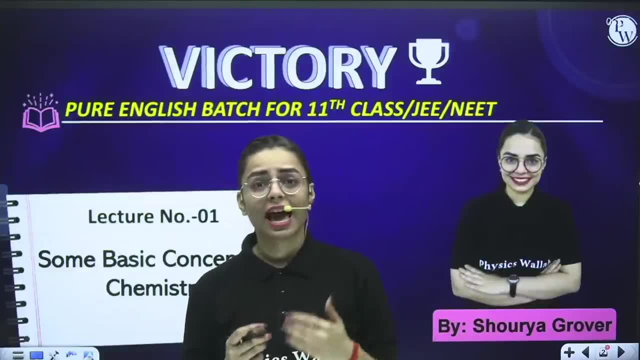 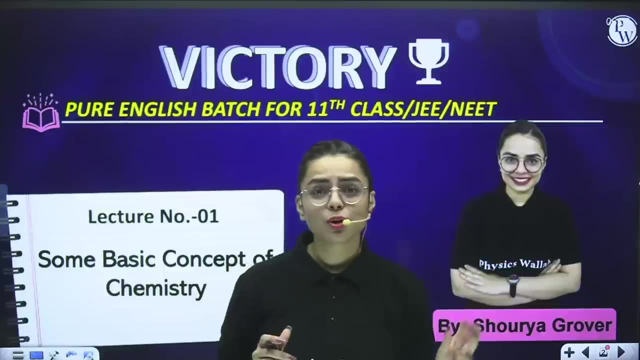 This defines us and reminds us of those classes, the previous classes, which we have studied, Like class 10th. In class 10th we have studied about matter in our surroundings. So from that portion we are going towards our 11th portion. 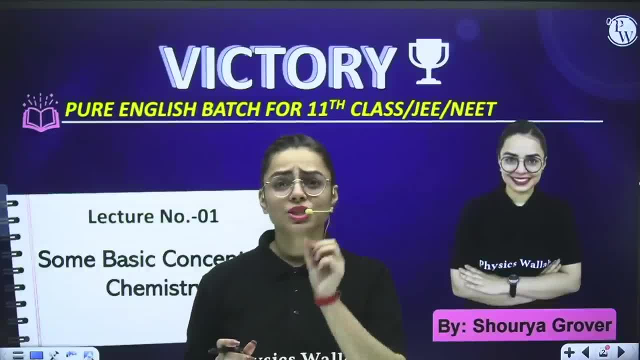 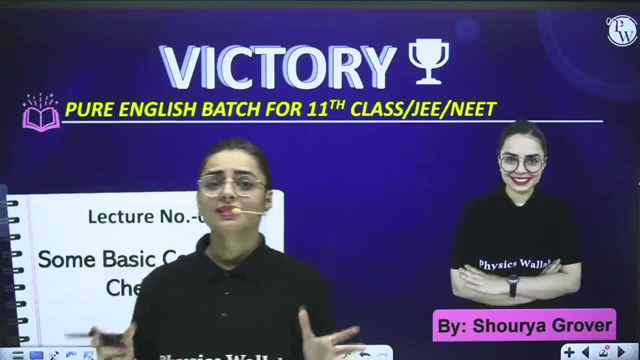 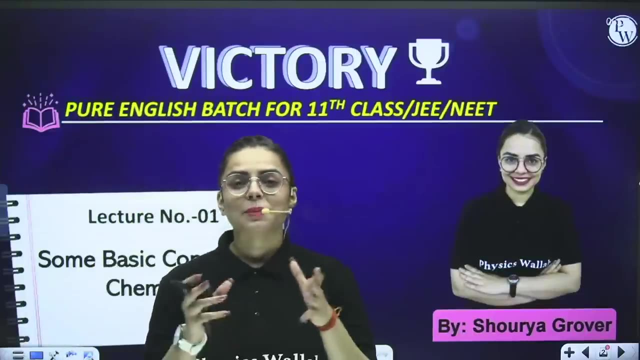 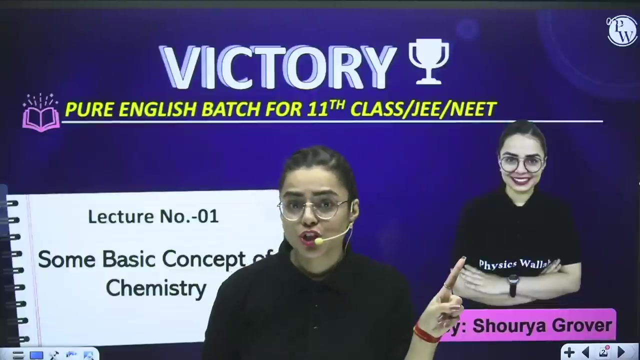 From 10th towards 11th. So I am going to tell you every detailed basic detail of the chapter. First of all, the thing that arises in everyone's mind is the subject chemistry: Students: chemistry. Chemistry is the branch of science that deals with the study of composition, structure and properties of matter. 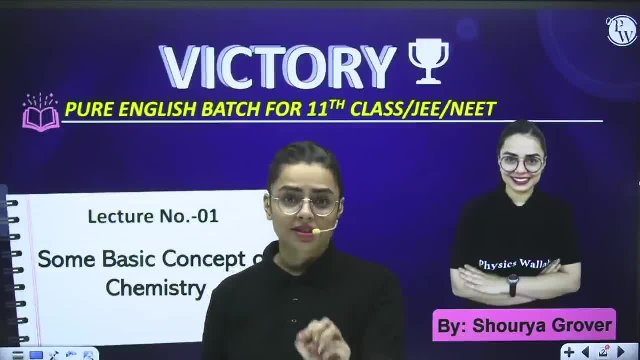 And also about the changes that matter undergoes in different conditions And the various laws that govern those changes. So, students, chemistry plays a vital role in science Students, chemistry. So students, it plays a vital role in healthcare products, applications in war, applications in industry, applications in food. 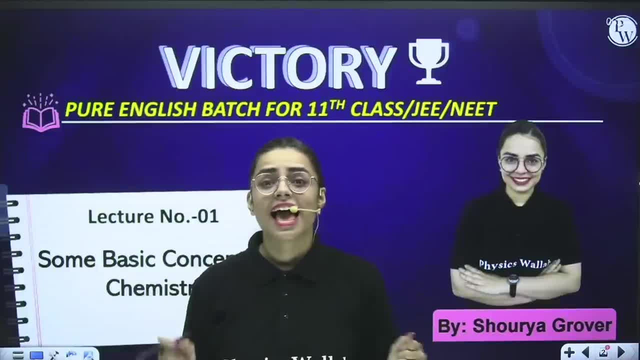 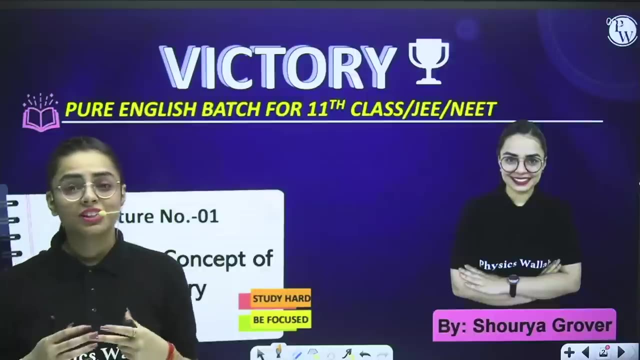 So in our day to day life, chemistry has an important role. So now, moving towards this, in our surroundings, when we look around, we look around a lot of things, a lot of objects. The most common object which a student observe in its classroom. 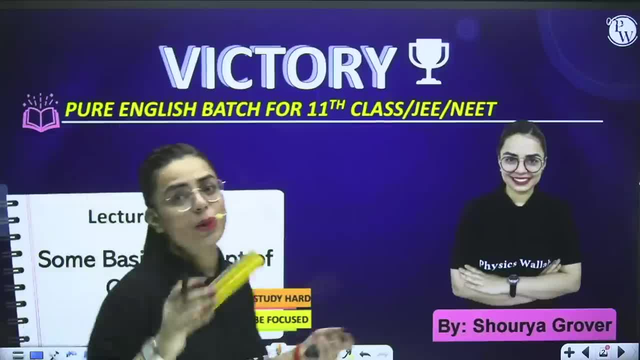 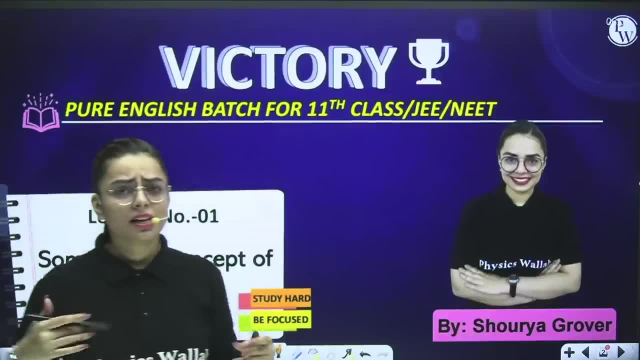 The most common object which a student observe in its classroom is the duster. Well, duster is a kind of solid object, right. Okay, Now let me tell what is a glass of water. Glass of water is a liquid right. 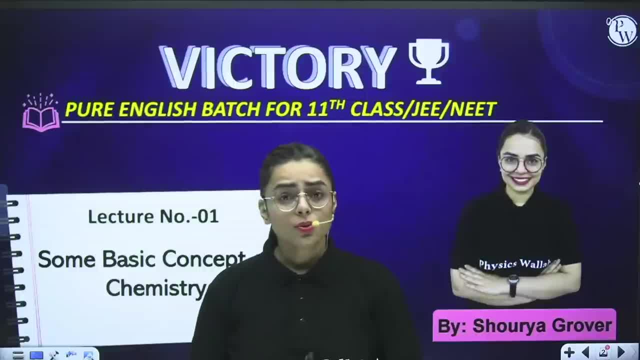 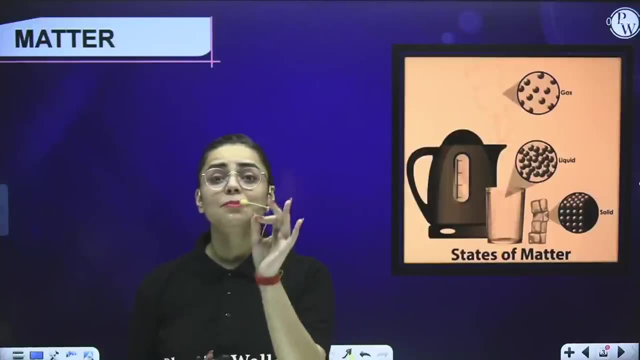 So water comes under the category of liquid phase. Now, students, these substances which we look around in our surroundings are all matter. Now, what is matter? Matter is a substance. Matter is a substance that possesses mass and occupies space. One more thing that defines this more accurately, I would say, is we can eventually feel with our senses right. 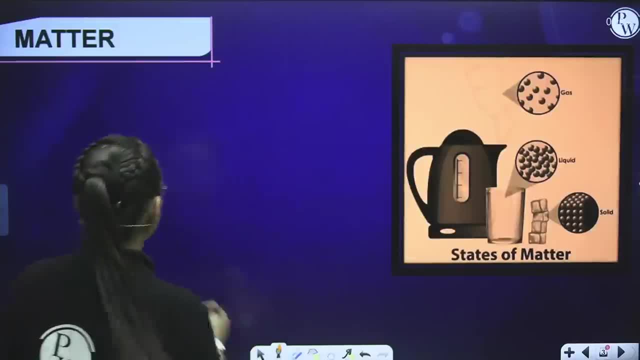 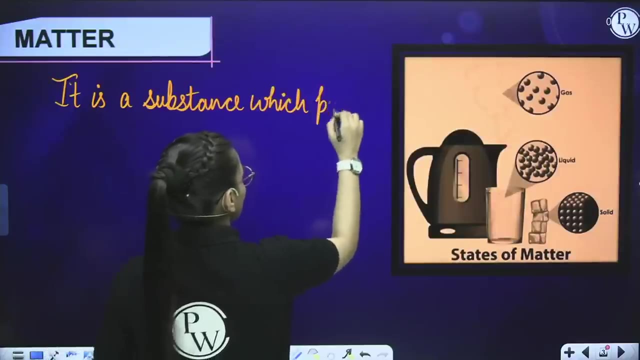 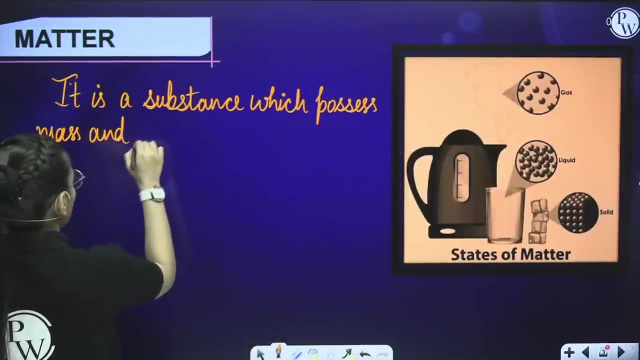 So what would be the definition of matter? I would say: matter, it is a substance. It is a substance. It is a substance Which possesses, which possesses mass and occupy space, and occupy space and can be felt, can be felt by our senses. 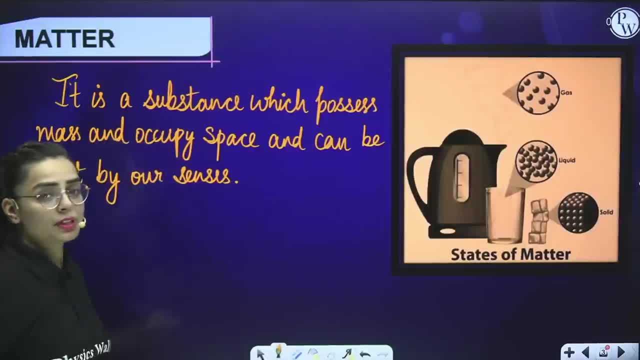 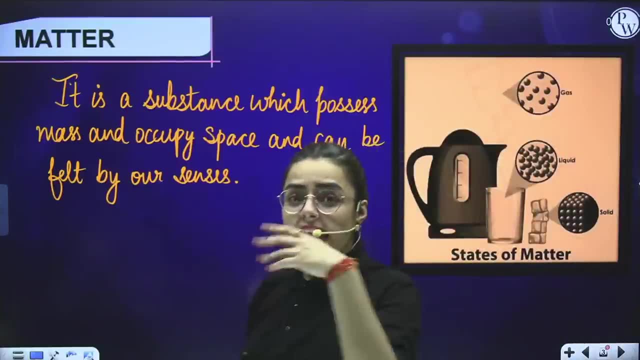 So, as I told you examples Of duster of water, we can take more examples, like chalk. We have gases around us. All these are matter. students, You know what Matter can be classified into two basic categories. The number first one is the physical classification. 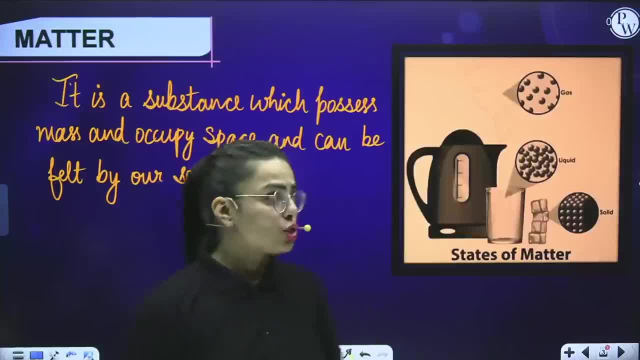 And the next one is the chemical classification. So when we classify them, when we classify matter Classification, it is the physical one and the chemical one. Students, when we study about physical classification, you know physical classification contains, it tells us about states of matter. 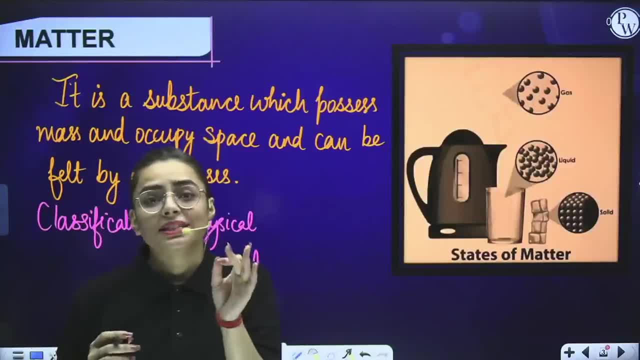 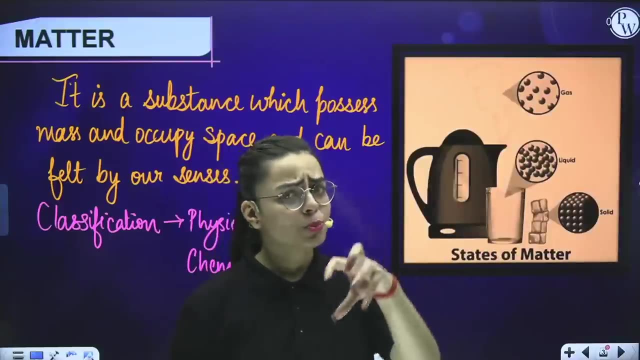 Now, what are states of matter? The most common and the famous example is in front of you. This is solid liquid and gas. Students, When we take an ice cube from our freezer in our home, in our kitchen, we take it out and we put it into a bowl, it starts melting. 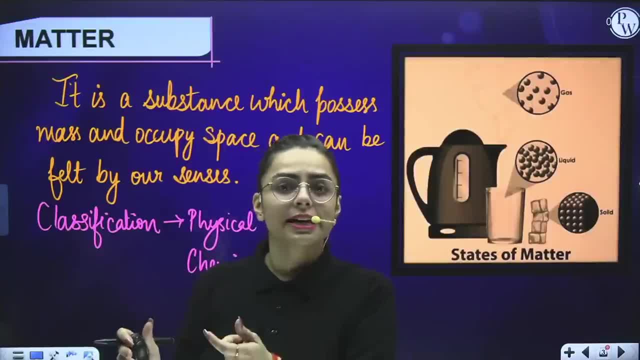 When that liquid is kept on a stove and is heated, it converts into vapors. So what is this? These are states of matter. The ice cube that we took from the freezer is a solid like the water in which it converted was liquid. 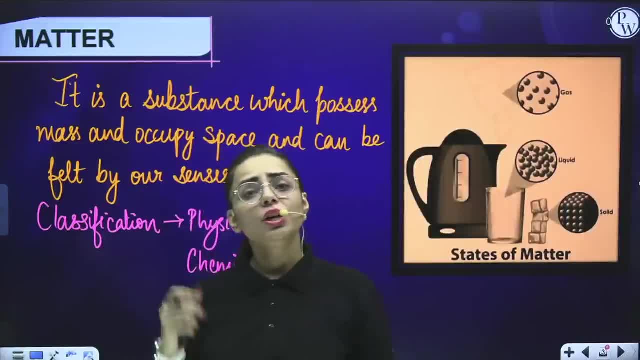 And when then it was heated? When it was heated, it converted into water vapors. that water vapors was gaseous form. So what we observe, students? we observe these states of matter in our day to day life, Right. 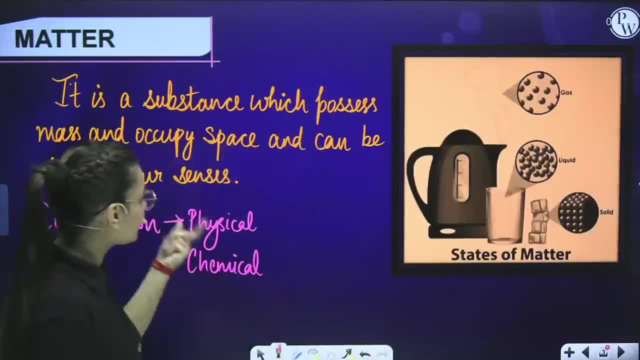 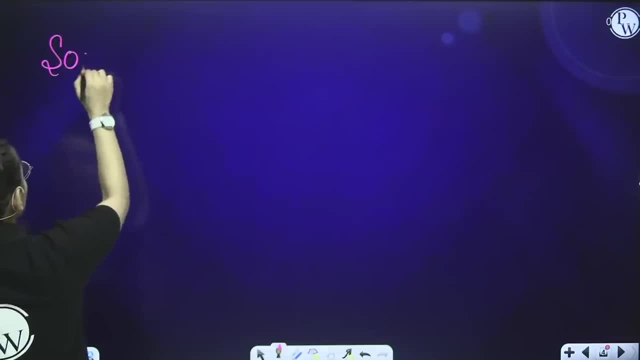 Solid liquid and gas. Now moving towards the physical classification in detail. First of all, we learn about solid. First of all, we will learn about solid. If I talk about solid, solid is an object in which What we can observe 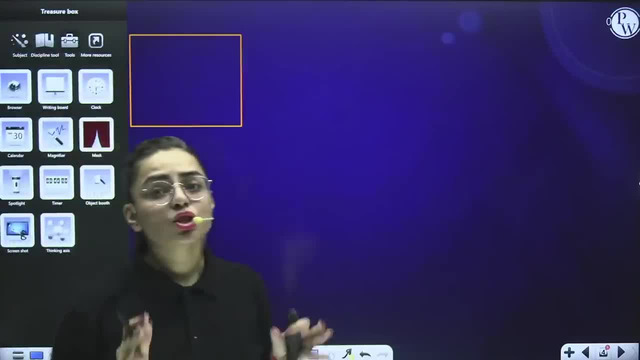 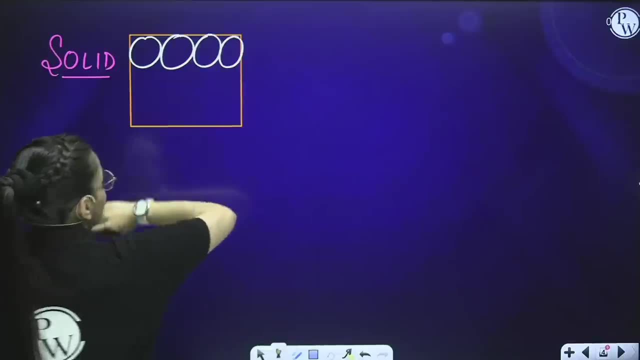 We can observe that particles in solid are so tightly packed. For example, this is my first particle, This is my second, third and fourth. This is the first layer. Now, how is the second layer formed here? The second layer is similarly, just like the first layer. 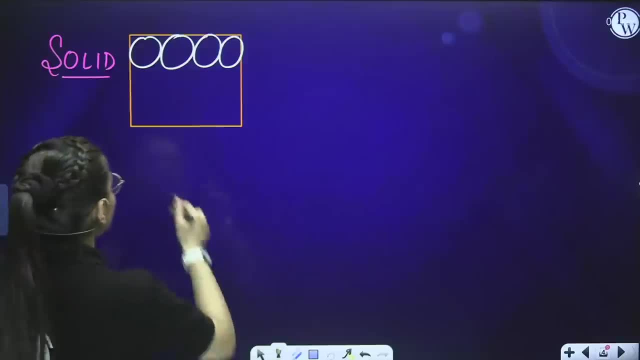 They are so tightly packed with each other like this way: One, two, three, four. Now the third layer. The third layer is in such a form Now, what you can see. by just being looking at the example, I can observe that there are some particles. 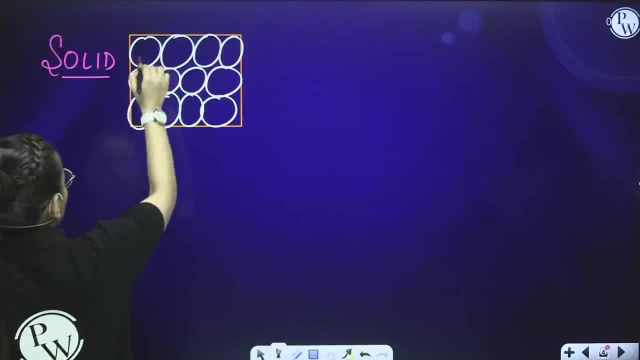 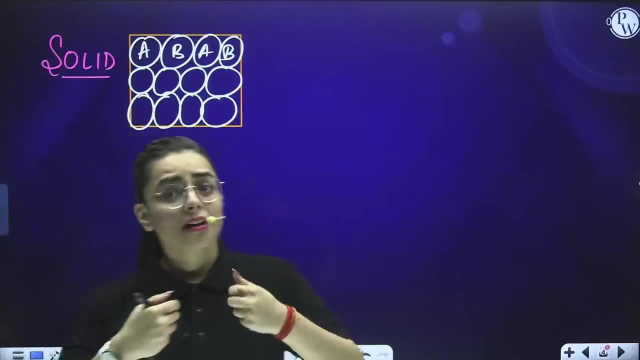 Let us say these are A particles or B particles. Okay, let us say A, B, A, B kind of particles. If I say A, B, A, B kind of particles, they are so tightly packed. This is my A particle. 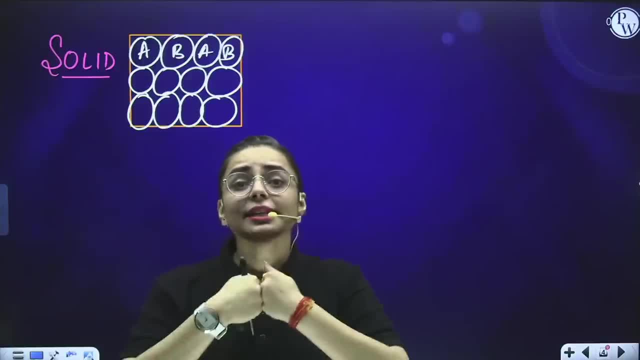 This is my B particle. They are so tightly packed that they cannot move from their mean position. They will only vibrate along its mean position like to and fro, just like this. They can't move from one position to the another position. And what is the reason behind this? that they have a strong forces of attraction. 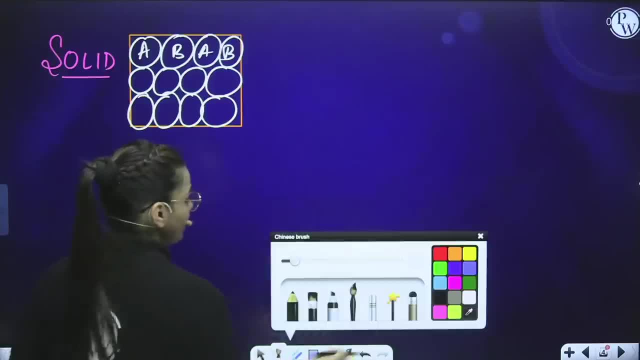 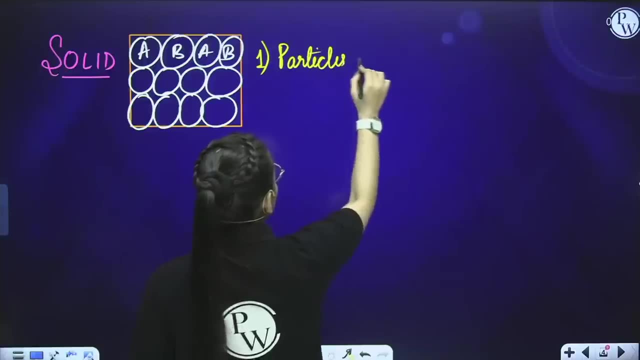 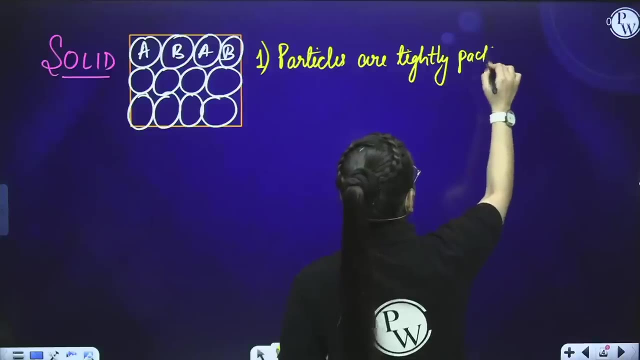 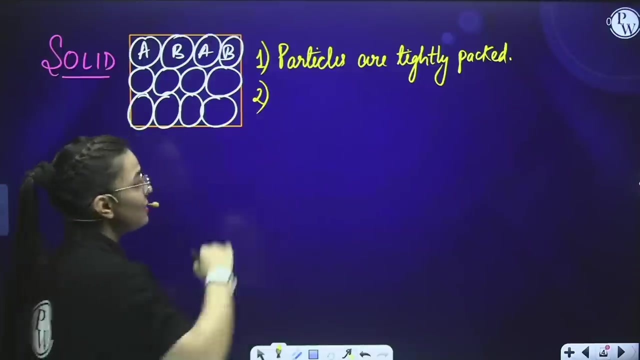 Do remember that. So the first point which we need to write here is: the particles are tightly packed. Particles are tightly packed students. The next point which we have to remember, that there is a strong forces of attraction. Moreover, we can say they have a definite shape and definite volume. 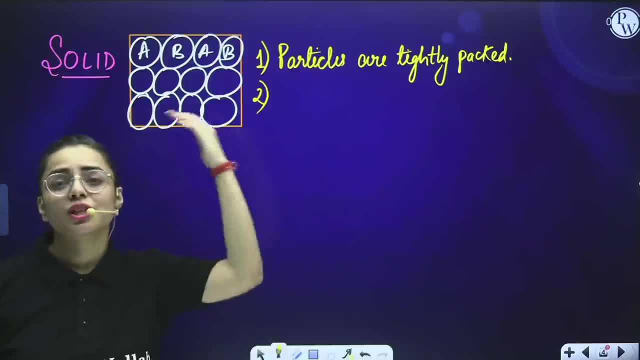 That these are the basic things: definite shape, definite volume. We have studied these in class 10th right, But in 11th, the most important thing you need to remember is the force of attraction and the force of repulsion right. 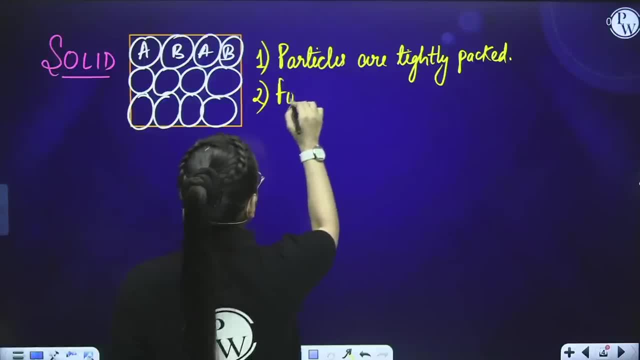 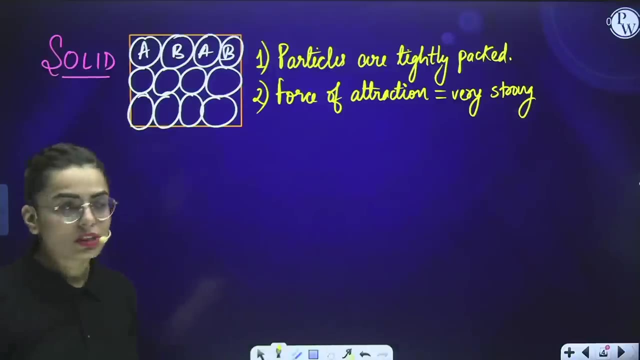 So next point is force of attraction. right, The force of attraction is very, very strong, due to which they are unable to move students. Now, coming towards the third, most point I would say, in the case of solids, there is very, very less forces of repulsion, or I would say the tendency to escape each other. 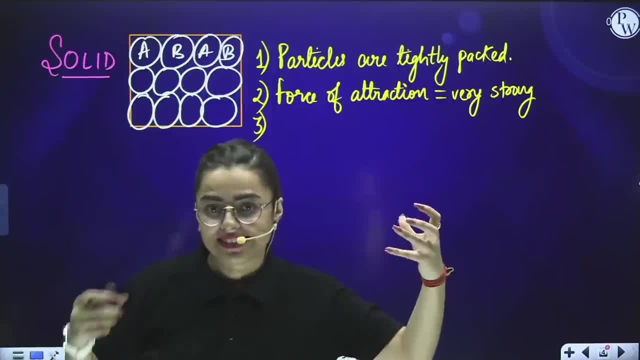 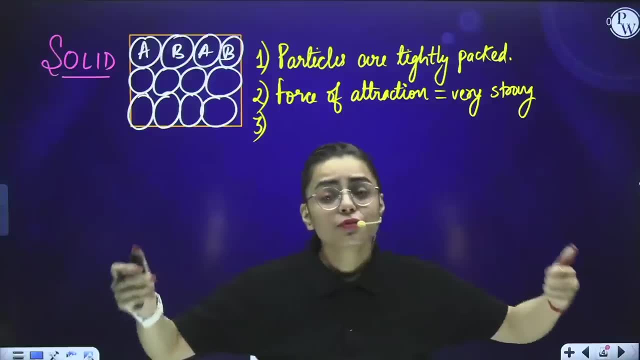 How to escape each other. If they are, If one particle is escaping from another particle, they attain a distance. They are at a farmost distance and if there is a strong force of attraction, they are attracted and they are close to each other. 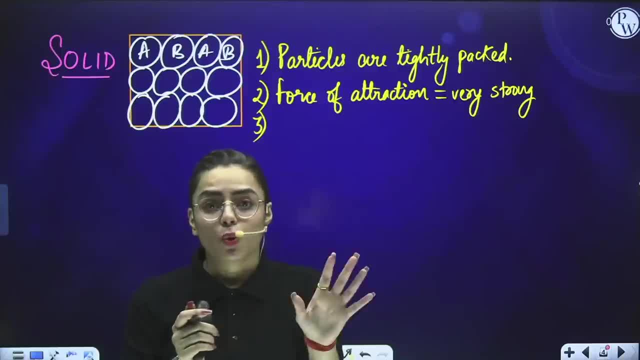 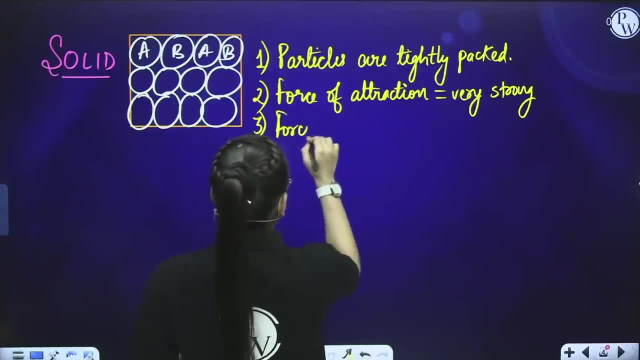 In solid they have zero, very, very less forces of repulsion. So forces of repulsion which I already told you to maintain distance between each other, right, In case of solid, it is very, very less, which is almost negligible, students. 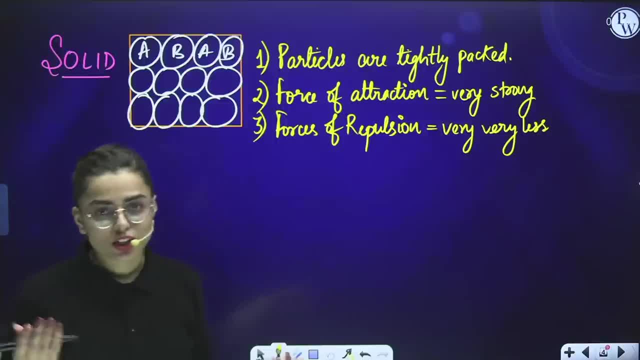 Okay, this was all about solid. You can even add more points, like definite shape and definite volume. Okay, Now moving towards the next case. the next case is our liquid. Okay, if I talk about liquid now, let us see its structure. 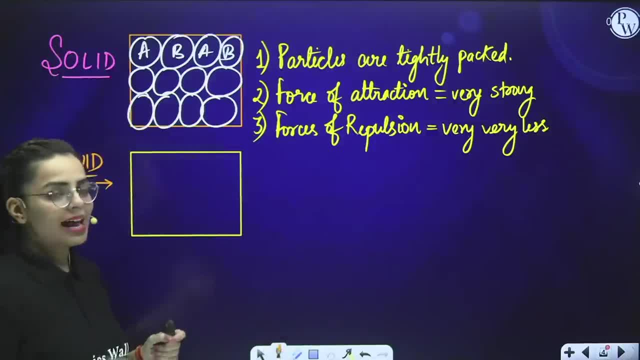 First of all, in the case of liquid, the particles are at a distance from each other, but not at a farmost distance. They are at a little bit distance from each other. For example, if I see this is my first particle, then this is the second, one, third, one, fourth one, fifth one, sixth, one, seventh, one, eighth one. 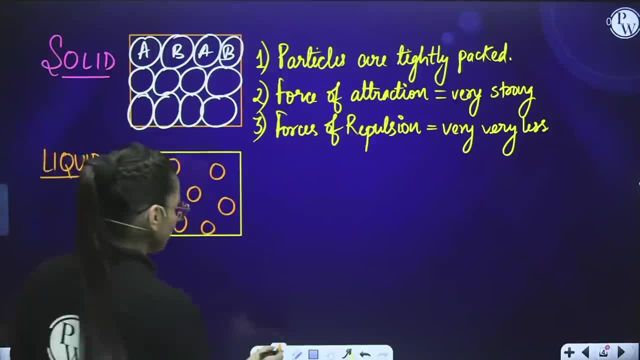 So what are the things that I am observing here, students? I am observing that number first, the particles are quite at a distance from each other, But not far. They are close, but not far, but at a distance from each other. 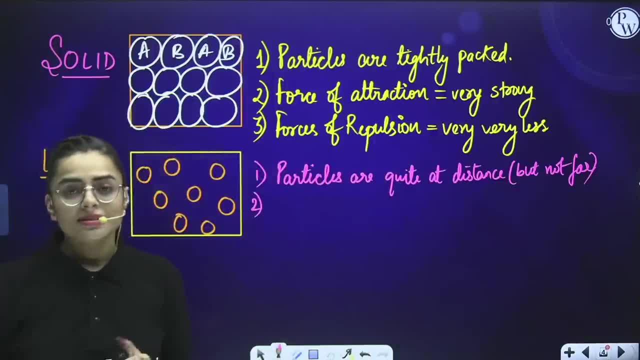 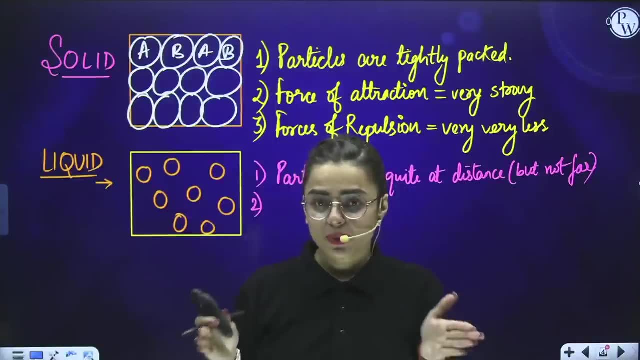 The second point which we observe here is the forces of attraction. See, in the case of liquid, both the forces act: forces of attraction and forces of repulsion. There is a forces of attraction, that is why they are attracted, And there is forces of repulsion, that is why they are not so close attached. 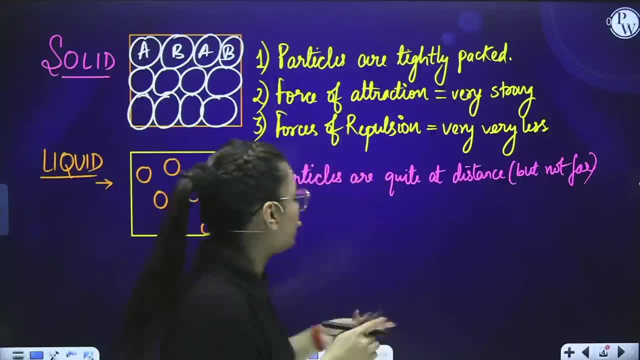 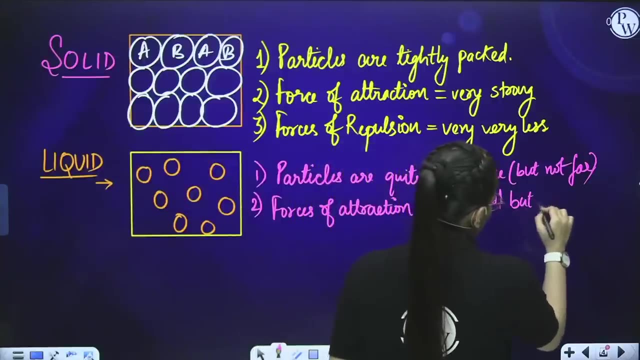 They are at a little distance because both the forces act, So I would say the forces of attraction. forces of attraction, in the case of liquids is less than solids, but more than gas, more than gas. right, Okay, now coming towards the third most point, that is, the forces of repulsion. 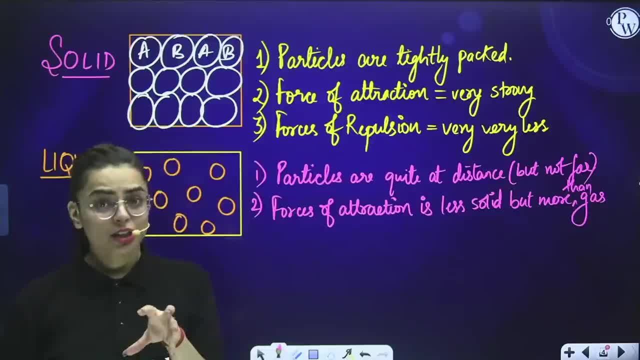 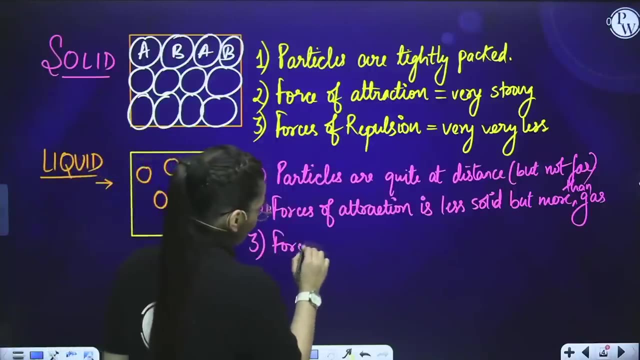 So if I talk against gases, I would say liquid, you know, has a less force of repulsion as compared to gaseous form And I would say it has more repulsion as compared to the solid form. So the third most point is: 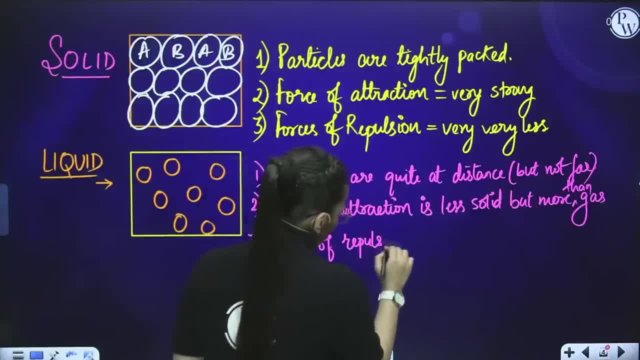 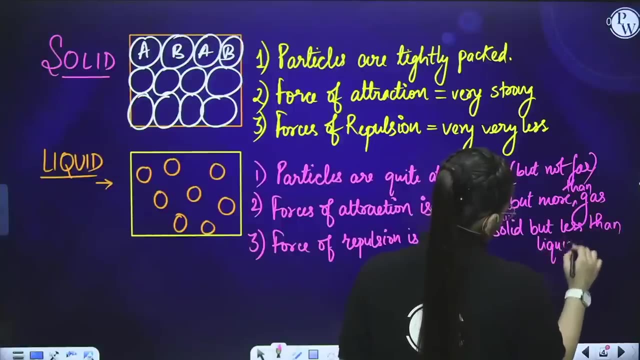 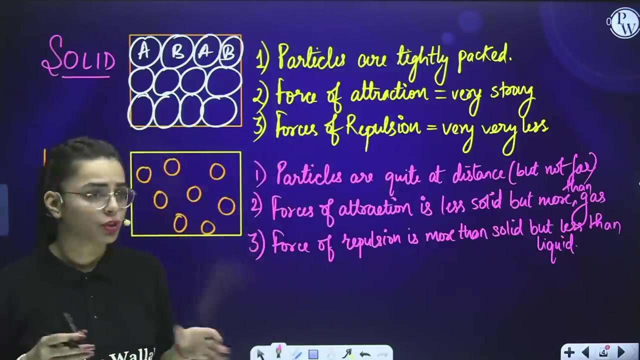 force of repulsion is more than solids, but less than liquids. Okay, so, students, this was all about liquid state. okay, I would say that they have a definite volume, you know, but they don't have a definite shape. For example, if I take a beaker, you know, and if I transform that, the you know liquid from one substance into another substance, 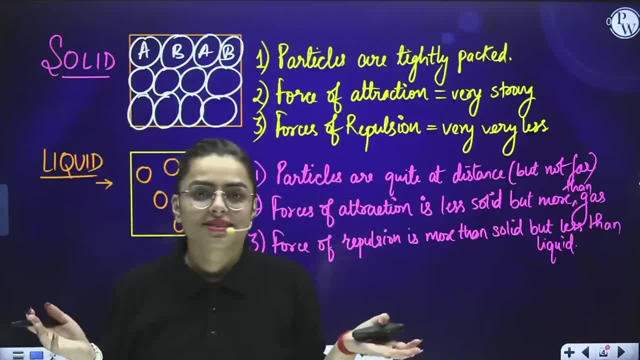 it would occupy its. you know shape. So shape is not certain for the liquid case. Hence its volume is certain. that means its volume is definite, but not the shape one, right? So the third thing that we talk about is our gaseous form. 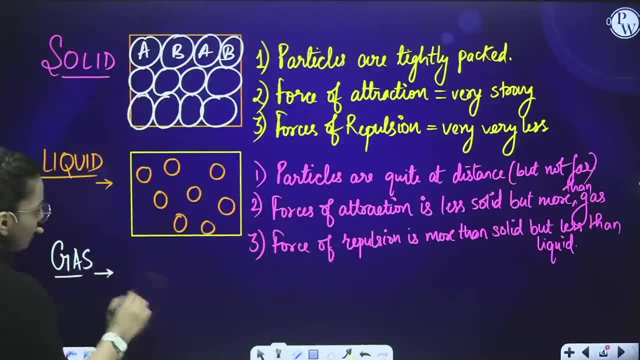 So the third thing that we talk about is our gaseous form. If I talk about gaseous form, first of all let us draw its structure. And while drawing its structure, we can easily tell the particles at a are at a far most distance. 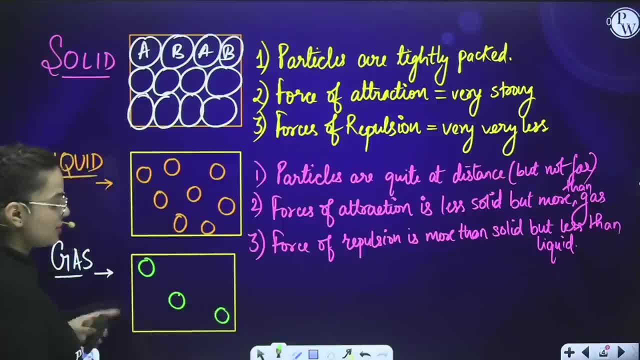 For example, this is the first particle, it's the second, it's the third. like this, They are at a distance. So you can easily observe these things like solid in they are very close. In liquid they are at a distance, but in gaseous they are at a far most distance from each other. 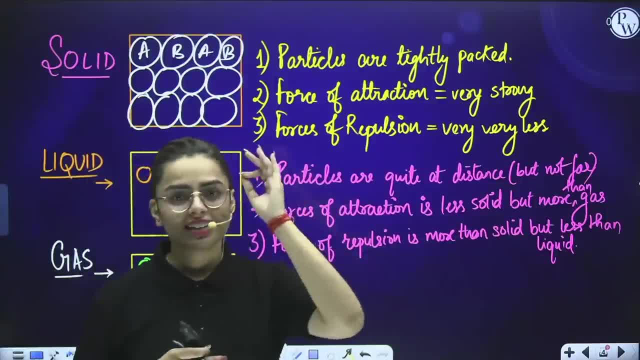 So when they are at a far most distance from each other? So when they are at a far most distance from each other, first thing, we can easily say that they have a very strong forces of repulsion. And how are the forces of attraction? 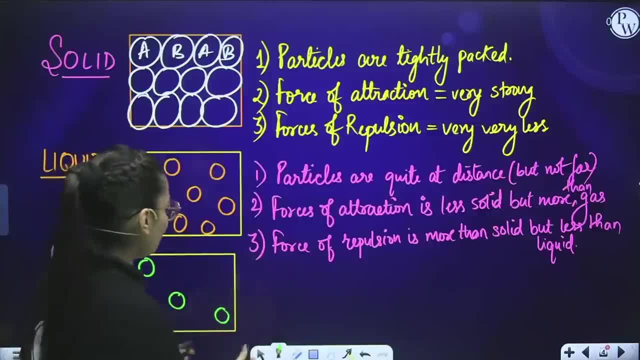 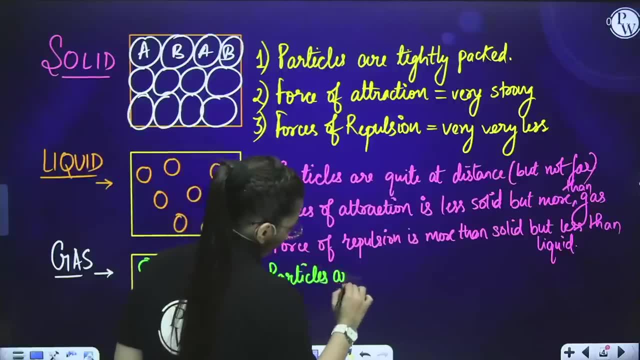 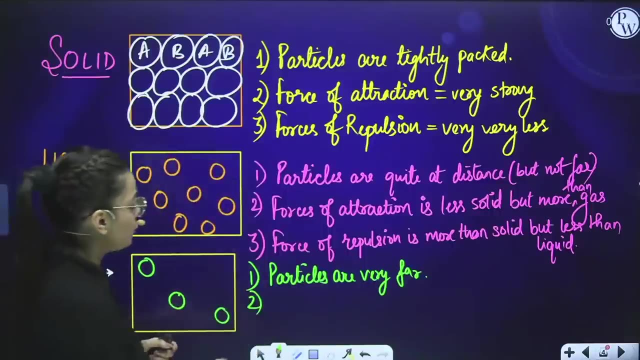 They are very less, very less. So, first of all, the very first point which we are going to write: particles are far, very far right. The second, most point, students, that I am going to write here is the forces of attraction. 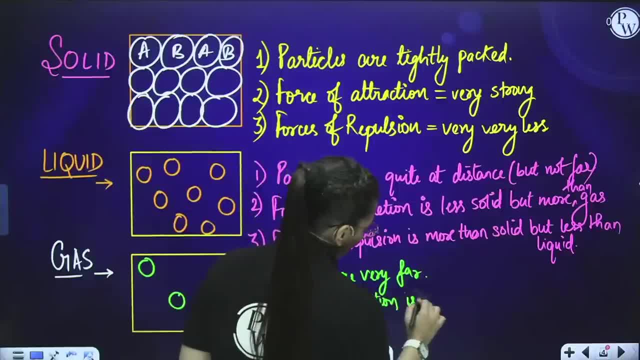 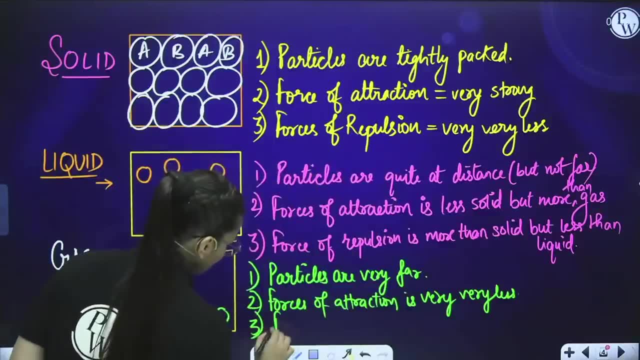 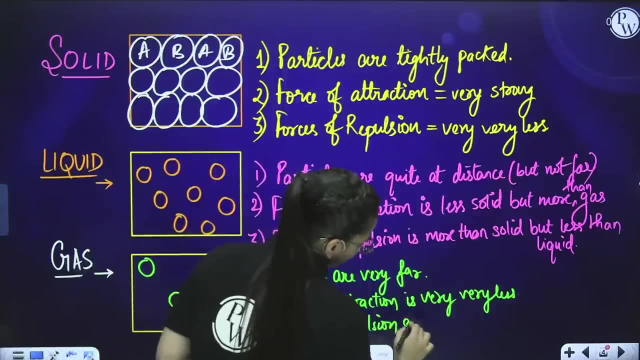 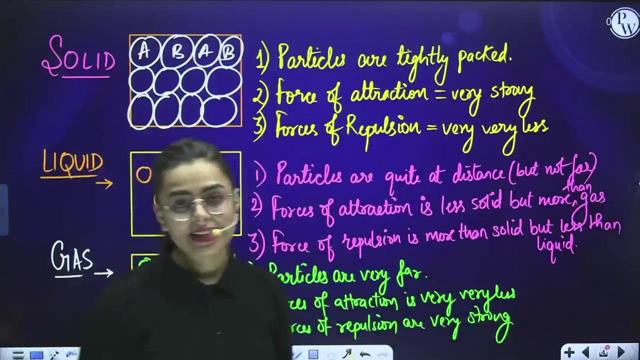 So the forces of attraction is very less, very, very less. And the very last point, students, I would say that the forces of repulsion. So the forces of repulsion are very strong, are very strong. So, students, this was all about the physical classification, right. 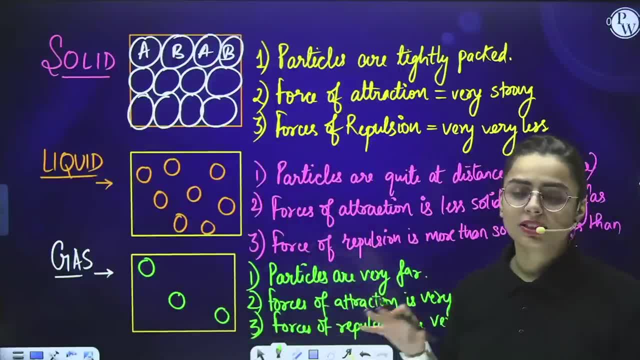 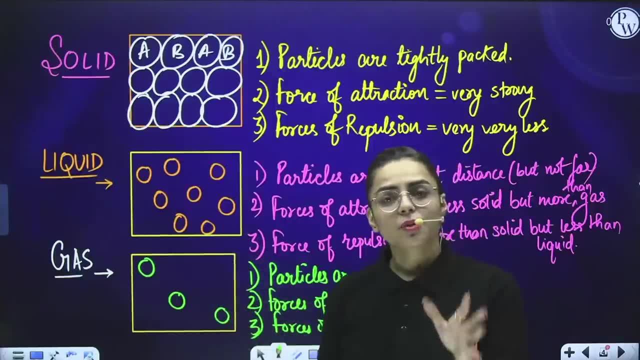 So if I say about the definite shape and definite volume cases, there is no definite shape, no definite volume in the case of caches, right? So this was all about the physical classification of matter. Now we are proceeding towards the chemical classification of matter. 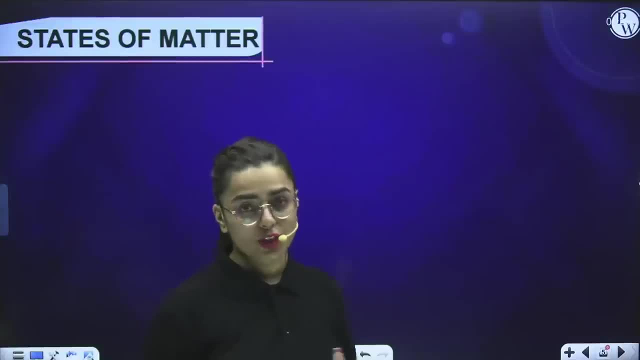 But before that, let me tell you that, in the case of physical classification, we observe that these three forms, these three states of matter are interconvertible. That means that we can say that solids can be converted into liquids, liquids can be converted into gases. 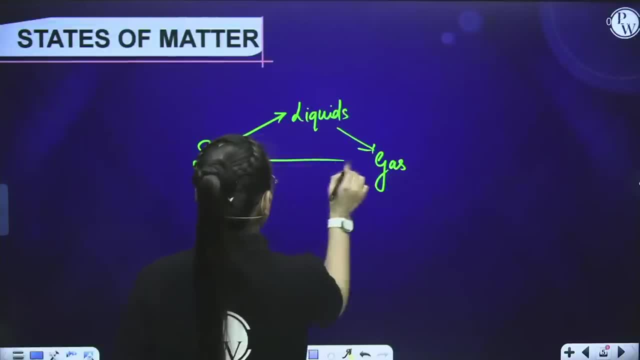 and gases can be converted into solids and vice versa. How? How? I am saying that liquids can further back be converted into solids, solids can further back be converted into gaseous and gaseous can further back be converted into liquid. How can this be possible? 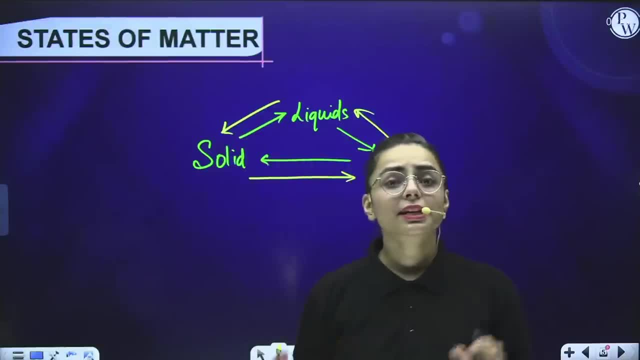 In class 10th we have already studied that while heating and cooling we observe such situations. You know, when I take ice from the freezer and keep it in a bowl, it converts right into what- Into water. When I boil that water, it converts into what. 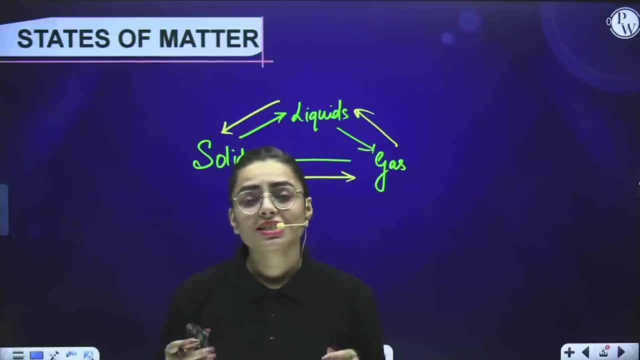 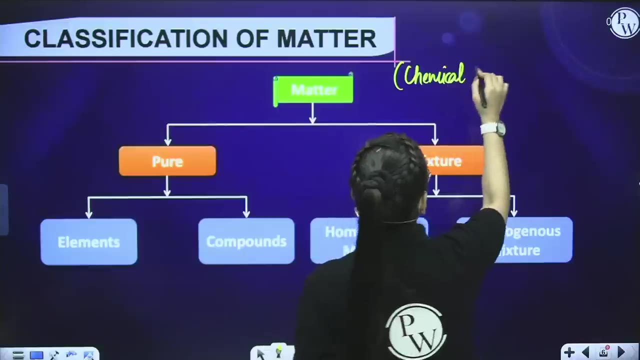 It converts into gaseous form. Okay, so these are all things. we need to understand that these three states of matters are interconvertible into each other. Now, students, coming towards the chemical classification of matter, This is our chemical classification. 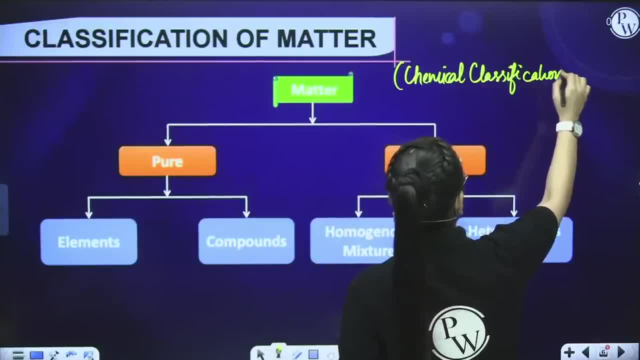 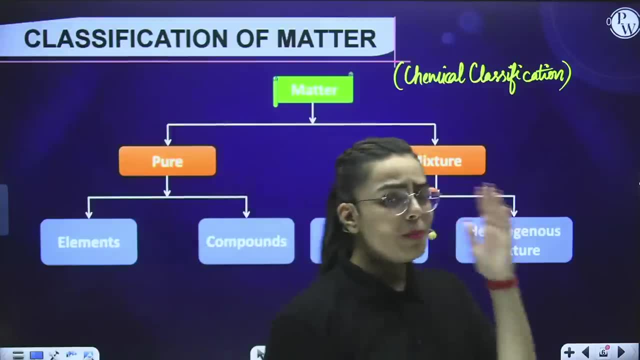 Okay, if I talk about chemical classification, the very first thing that arises is that it is classified into two basic categories. One is pure, another one is mixture. So by looking at the words, you can easily identify what do you mean by pure. 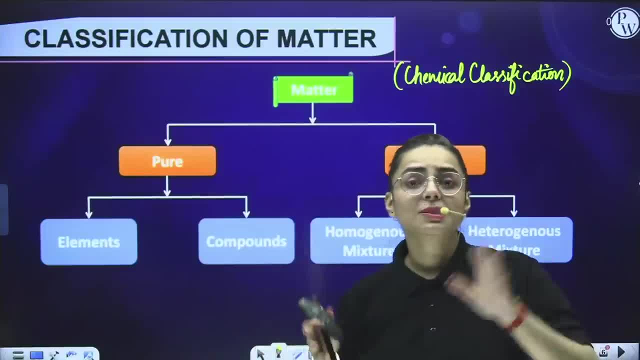 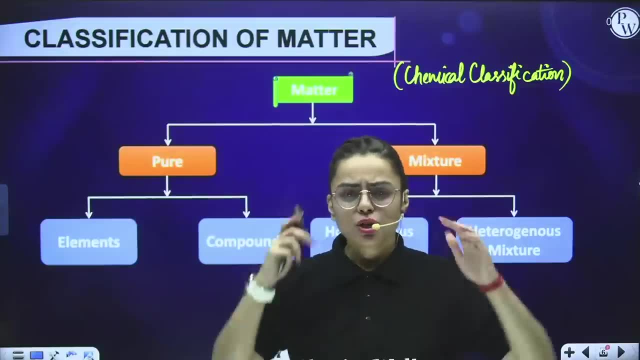 and what do you mean by mixture? Mixture is something in which something is mixed right And pure is something which is pure and something is not added into it right. So these are the basic things. when we listen to a word and we could, you know, think about it. 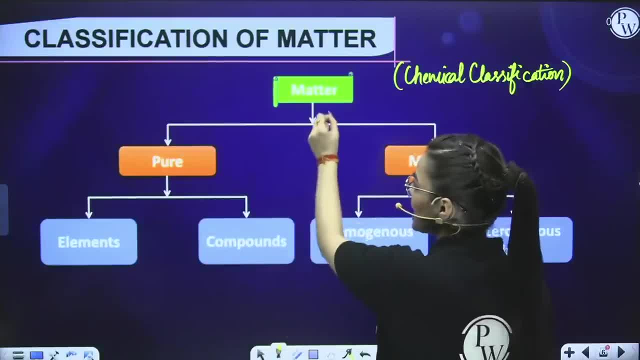 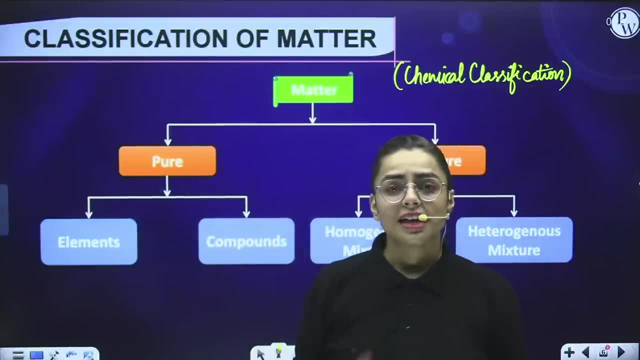 So first of all I would say that when we classify matter according to the chemical classification, we observe the pure substances. Pure substances are further classified into elements and compounds, And students elements are one of the kind. How I am saying that in elements you can see only one kind of matter. 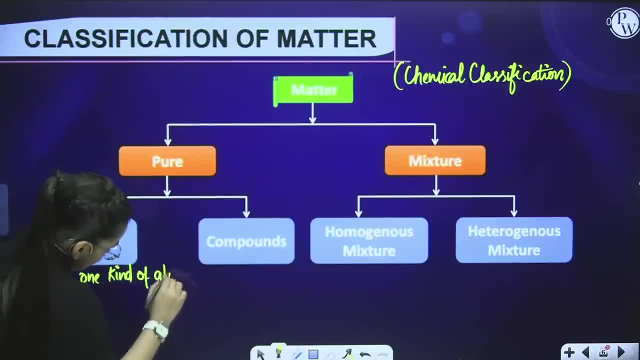 only one kind of atom. How I can say that? Example carbon, example hydrogen, Okay, example oxygen. You can even write that Only one kind, Only carbon, only hydrogen, only oxygen, only sodium, only magnesium. 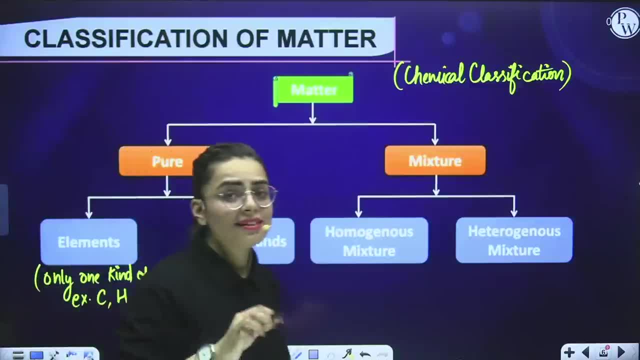 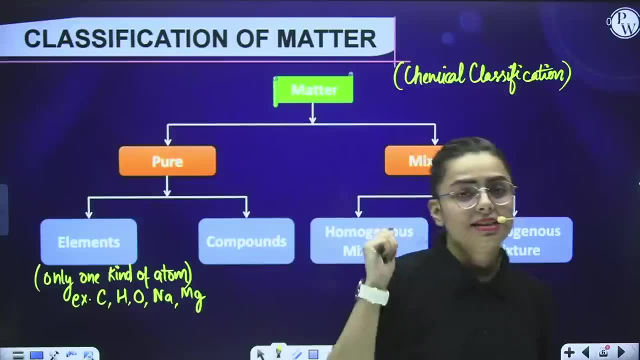 Only one kind of atom when we observe that that is referred to as an element And element students. further, is classified into three basic categories: First is metals, second is nonmetals and third one is students- metalloids. 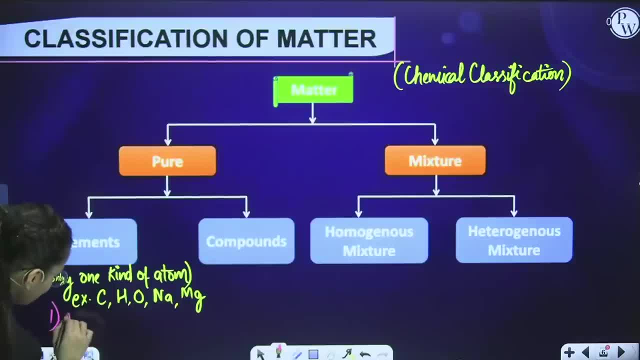 So I would say that if I classify them into elements, then it is classified into metals. The second one is nonmetals, Students, and the third one is metalloids. Now, what are metals, nonmetals and metalloids? If I speak about metals to you, metals are the ones that are good conductor of heat and electricity. 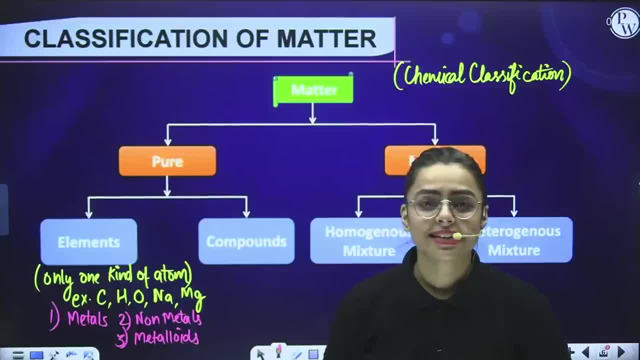 Metals are the ones that are lustrous. You have studied in class 10th chapter metals and nonmetals. Well, that is what metal is. It is lustrous, it is good conductor of heat and electricity, You know. it is malleable, it is ductile. 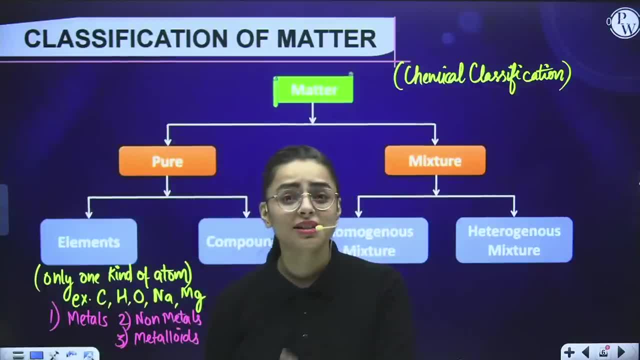 What is malleable and ductile? Malleable are the ones that can conduct heat and electricity, That can be hammered into thin sheets, and ductile are the ones that can be converted into wires, For example, copper, magnesium, iron. these are metals, right. 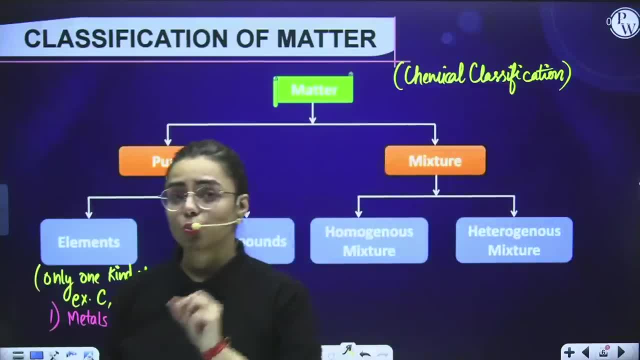 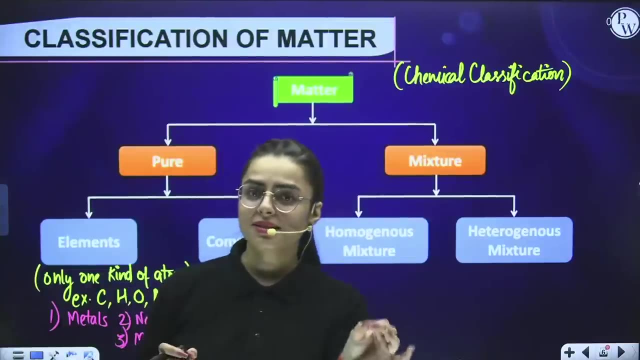 Now, coming towards nonmetals, I would say nonmetals are the ones that are poor conductor of heat and electricity, You know so. they are not malleable, not ductile. We observe these things in nonmetals. While coming across towards metalloids, metalloids are the ones that exhibit the properties of both metals as well as nonmetals. 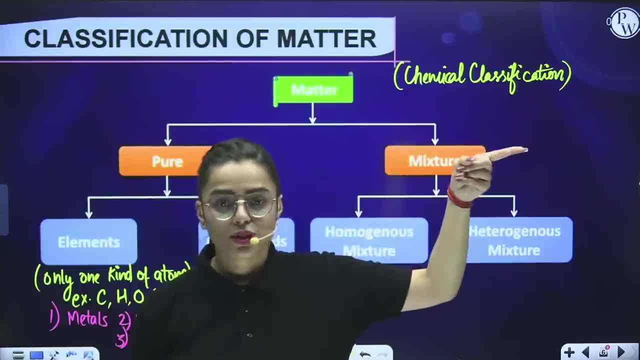 So these were the basic things that we started in the class you know 10th. If I take example of metalloids, I would say that metalloids can be antimony, bismuth, arsenic, right. 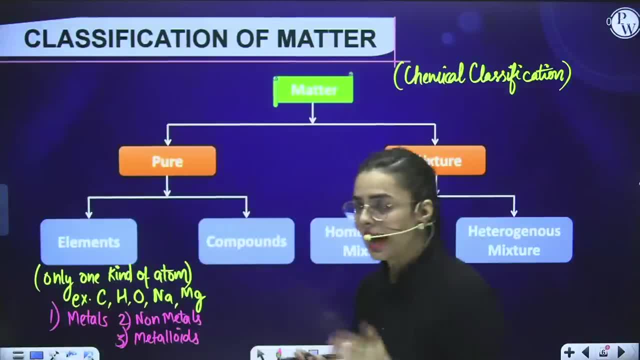 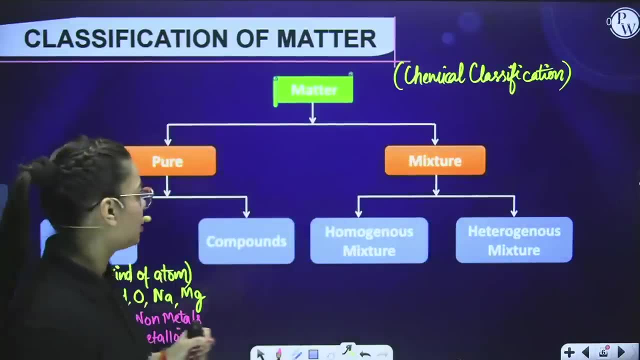 So this was all about elements. If I come towards the second category of pure substances, that is, compounds, Compounds are the one which contain two or more than two atoms. you know, Compounds, compounds, they are the one which contain two or more than two atoms. 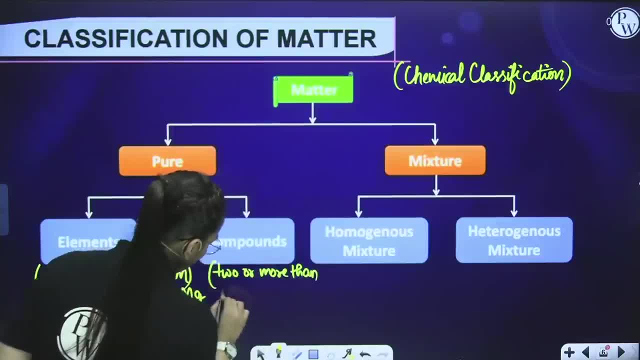 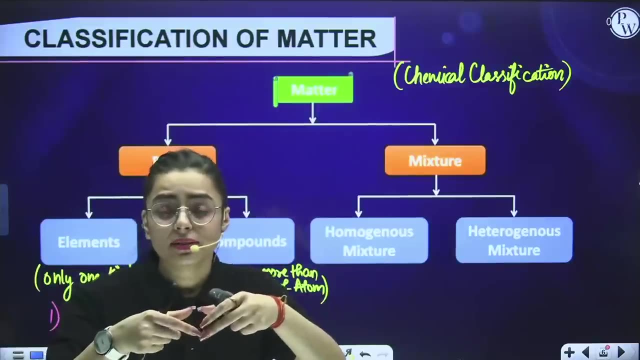 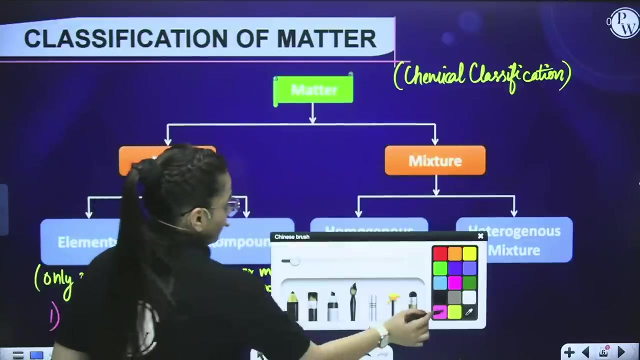 More than two kinds of atoms. See. if you find only a single atom, that is known as element. But when you find two or more than two elements which are combined together, they are known as compounds. Students, compounds can be further categorized into organic and inorganic. 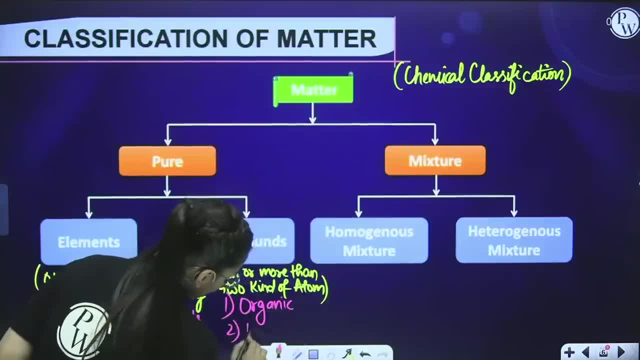 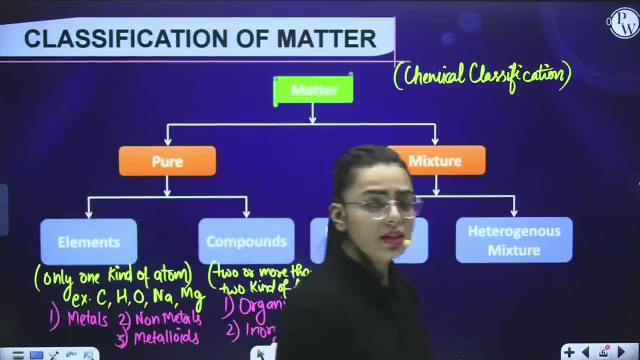 They can be further classified into organic and inorganic. They can be further classified into organic and inorganic. They can be further classified into organic and inorganic. Organic compounds are those in which we study about hydrocarbons. Now, what is hydrocarbons? 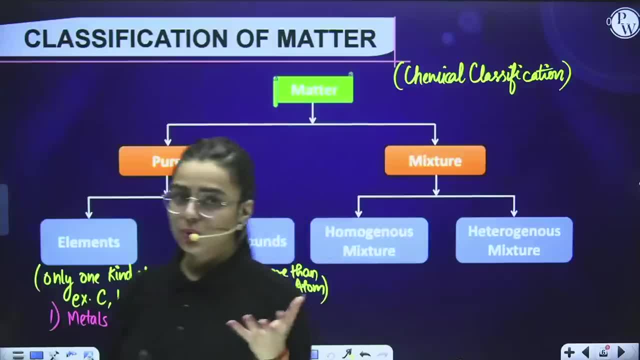 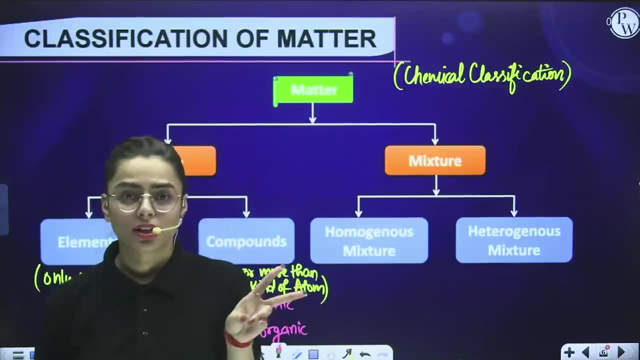 You will observe the hydrocarbons chapter in class 11th. only Hydrocarbons are the one in which we observe carbon as well as hydrogen. This is the basic necessity condition: Carbon and hydrogen should be present. Other than that, any other element can also be there, you know. 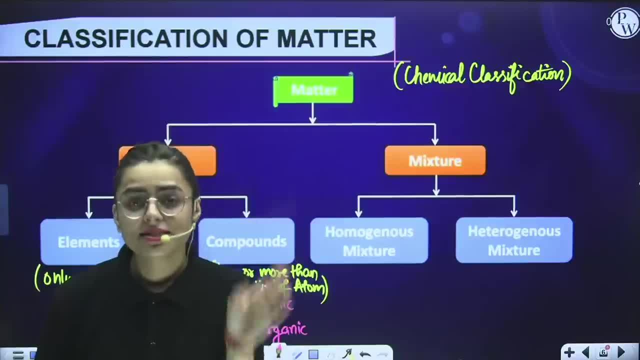 But if only carbon is present, it cannot be categorized into organic compounds. Do you remember that? So organic compounds are basically derived from animals and plants, But if I talk about inorganic compounds, inorganic compounds are the one that derived from minerals and rocks. 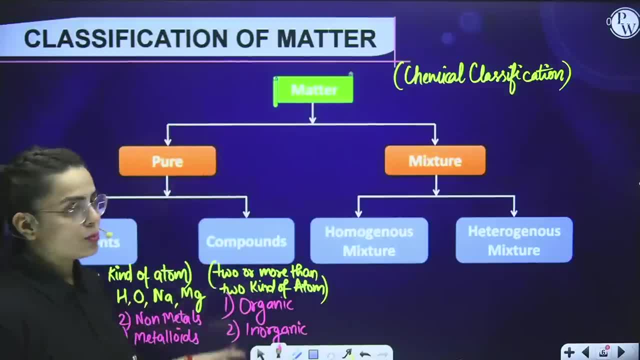 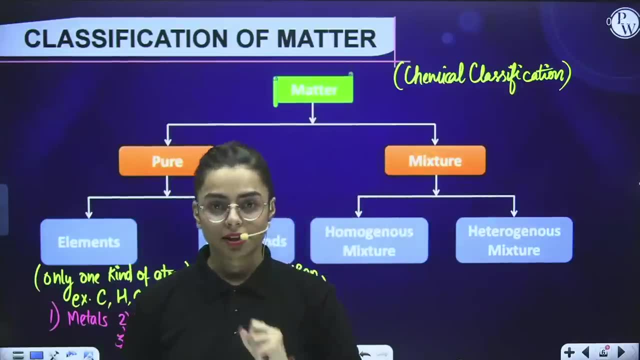 Clear. So this was all about the compounds category. Now, moving towards the mixture. As I know, mixture itself tells us that something is mixed, You know. it is further classified into homogeneous and heterogeneous, as we are assigned students, Students. 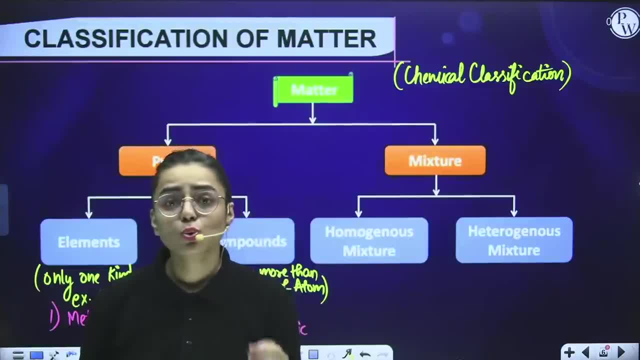 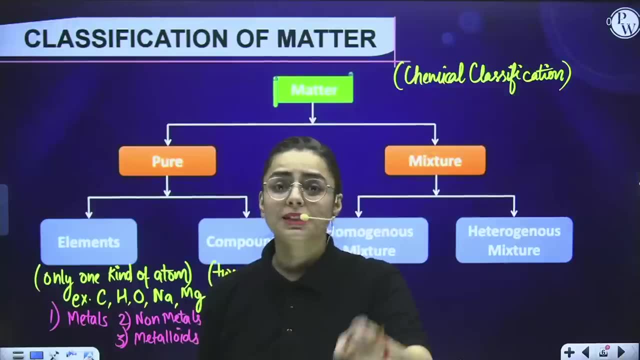 Whenever you are studying any of the topic, do remember that Kindly take the word If it is splitting into two parts. do that. It will make your concept easy and you will remember it here and you will never forget it. You know some people, what they do. 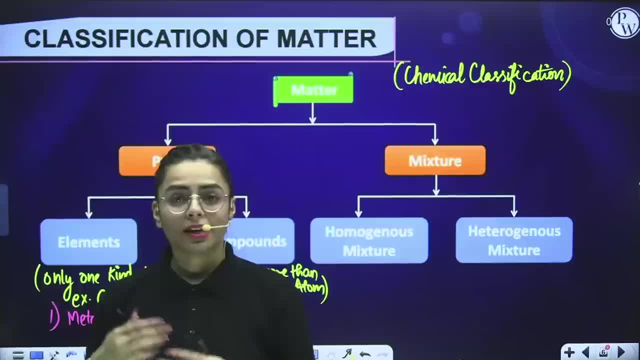 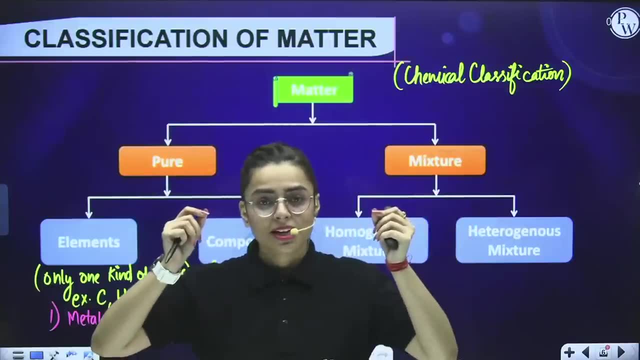 They just, you know, keep, keep again and again, again, again, writing and learning, and writing and learning, And after a few times they just forget it. When you understand any concept, you grasp it properly, You know, and then, and then you become stronger, and then you remember that. 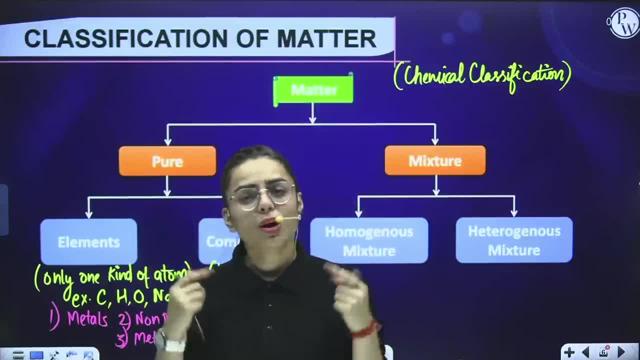 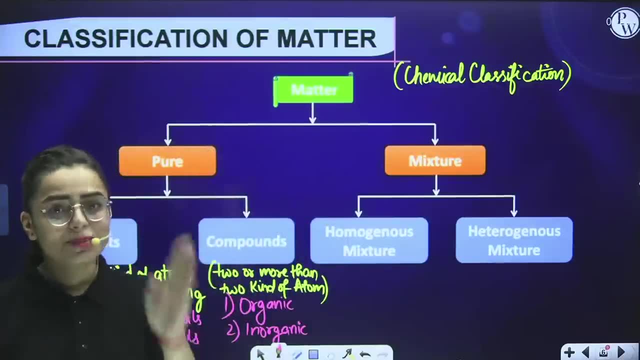 So it will help you a lot. So try to understand things instead of, you know, cramming it. So first thing is homogeneous mixture. As I told you, please split it in two parts. If I split it into two parts, I observe homo. 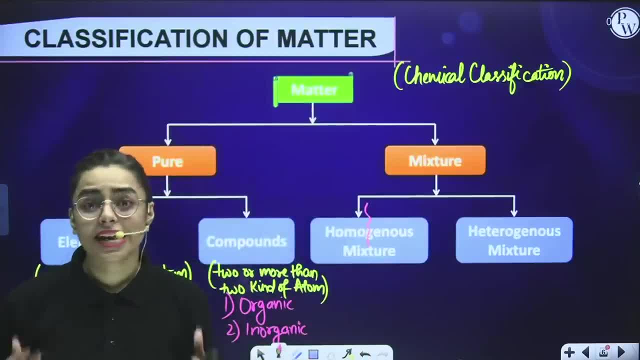 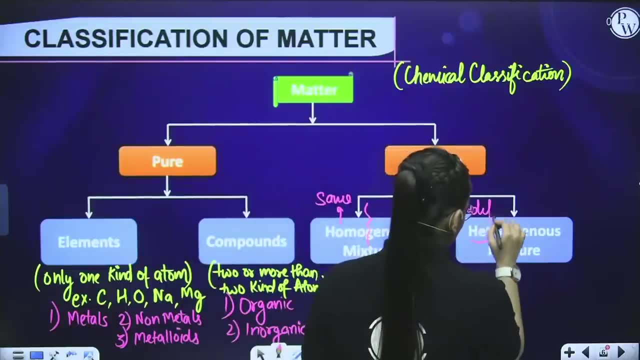 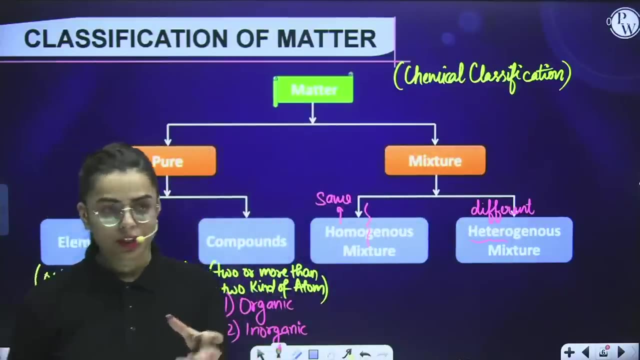 Homo refers to what Same, Homo refers to same. And if I speak about heterogeneous, hetero refers to different. Now, what is heterogeneous? What I meant by same and different? See if something is present in uniform, you know, uniform concentration or same concentration throughout. 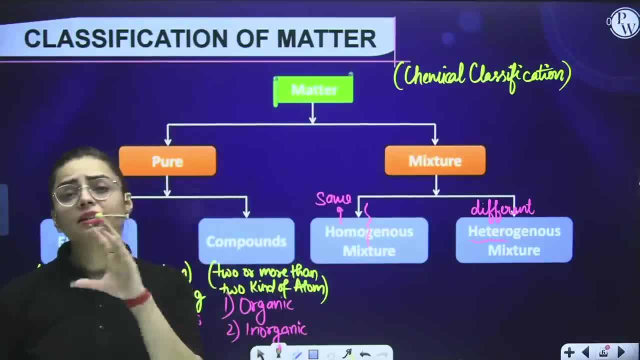 that is known as homogeneous mixtures, And if something is present in different composition throughout, that is referred to as heterogeneous Right? If I talk about homogeneous mixture, one of the examples which we observe is basically sugar in water, salt in water. 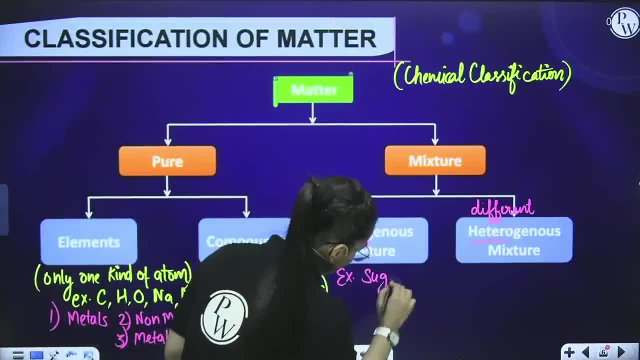 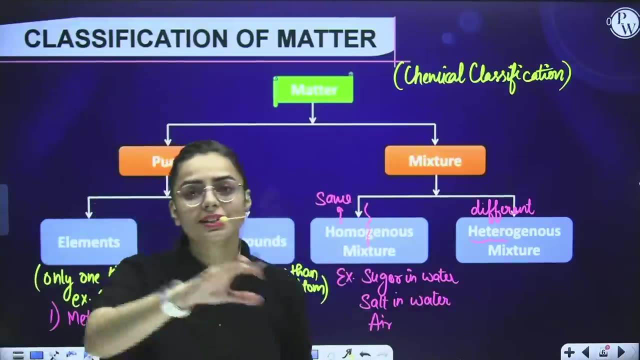 Okay. Example is sugar in water. The next one is salt in water or air. I would say Why air? I am saying because air is basically comprised of gases which are present in uniform concentration throughout. That is why it lies under the category of homogeneous mixtures. 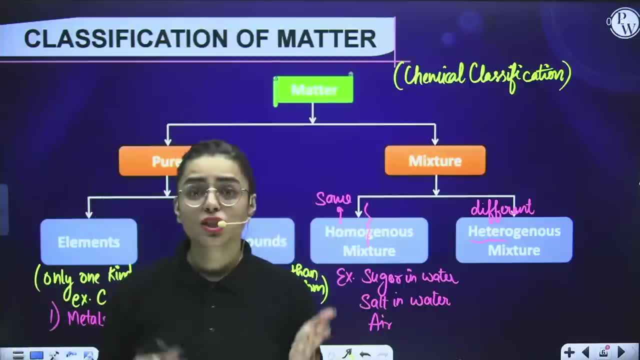 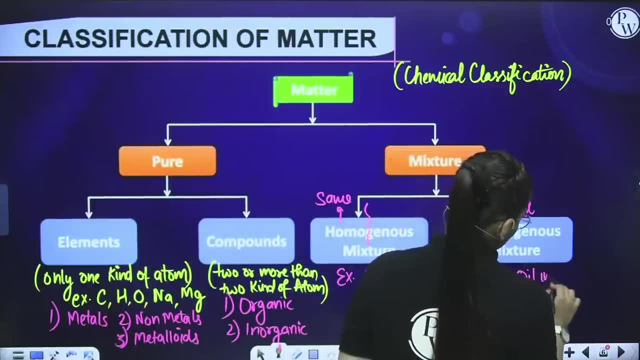 If I talk about heterogeneous mixture, one of the most common example is smoke. Other than that, is oil in water Right, So heterogeneous. we have two cases, like oil in water, Where the concentrations are not uniform. The second most example I told you is smoke. 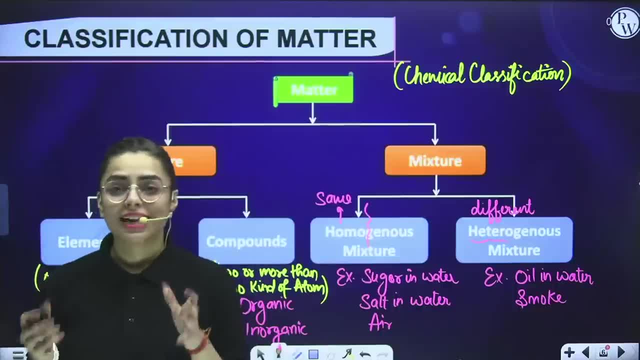 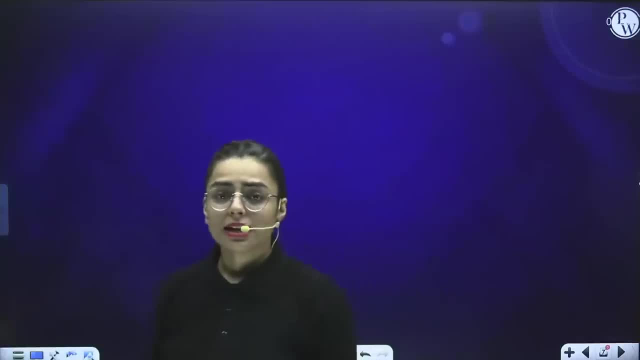 So, students, this was all about our chemical classification of matter. Okay, Now moving towards the next topic, that is, properties of matter. Now we have studied about the classification of matter, Now comes the properties, Now comes the properties of matter. 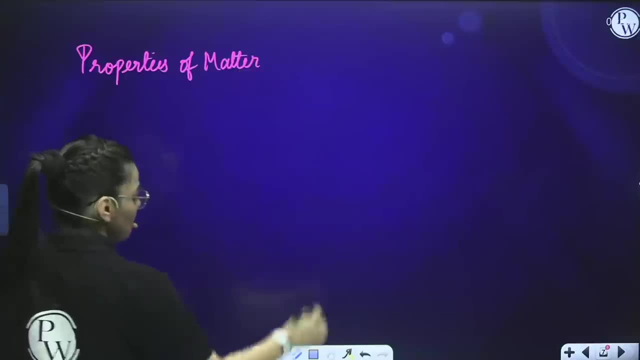 Students if I talk about properties of matter. why, Why, Why, What is the basic thing that I observe here? I see that the properties of matter can be of two types. One is the physical property, Another one is the chemical property. 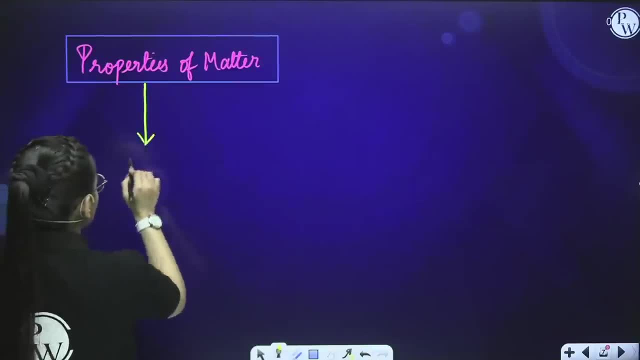 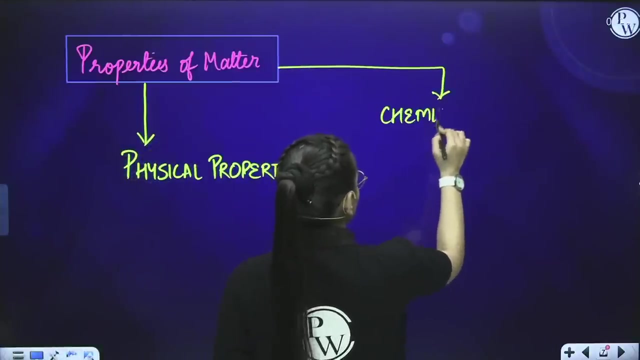 Okay, One is the physical property, Okay. The second one, students, is the chemical property. Okay, If I talk about students' physical property, What are physical properties? Physical properties are the ones which we can observe and in which the identity is not lost. 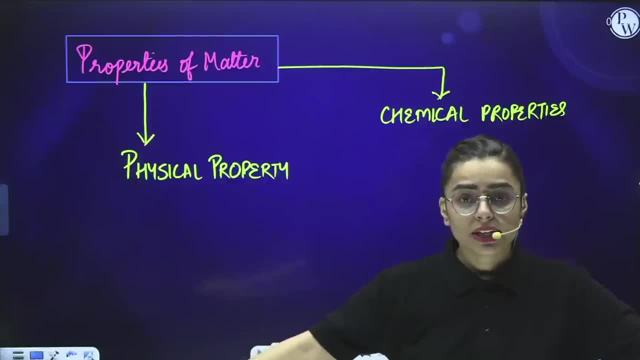 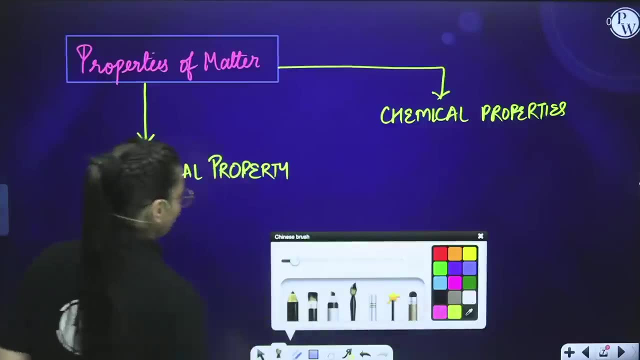 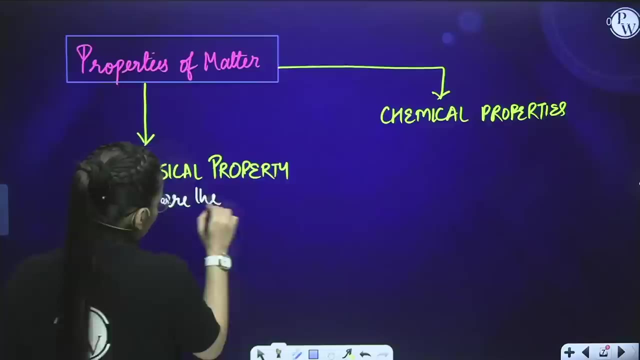 In which there is no chemical reaction. Okay, You can see that the substance remains the same throughout. So I would say that please do write it or you can underline in your NCERTs. Physical properties: these are the ones which do not. 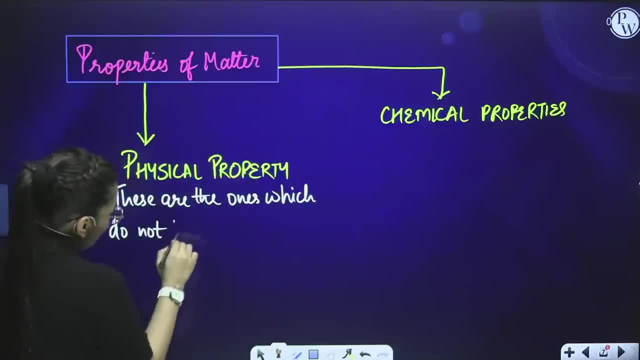 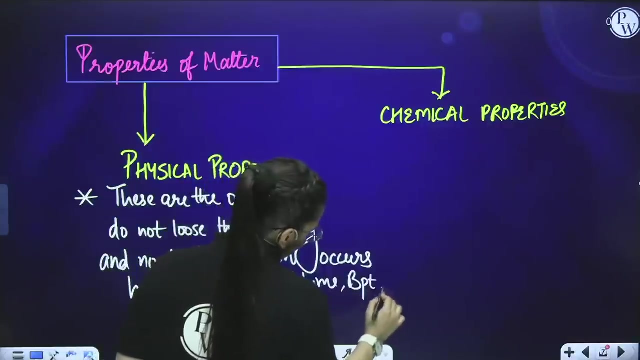 which do not lose their identity, lose their identity and no chemical reaction. no chemical reaction occurs here, Occurs here. Okay, Example I would say: density, volume, boiling point, melting point. These are the examples of the physical properties. 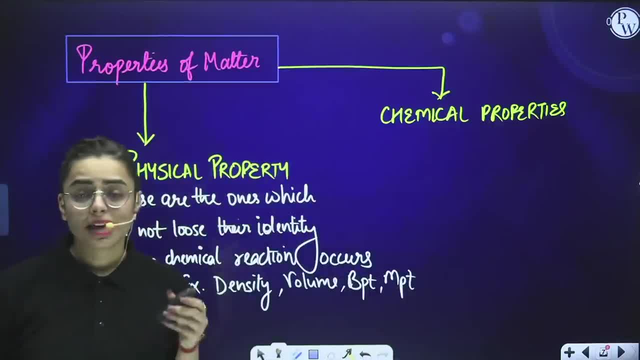 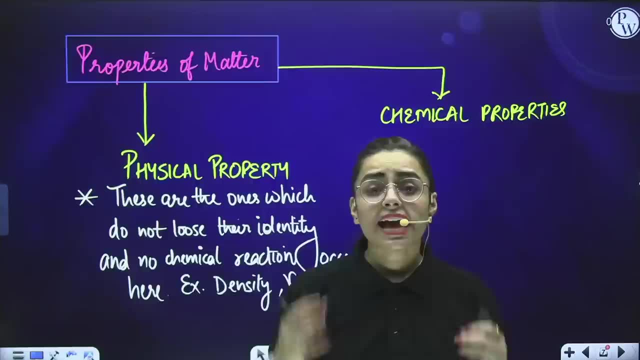 Now coming towards the next one, that is, the chemical properties. Chemical properties are the one in which reactant is being converted into the product. That means the chemical reaction is taking place. And when a chemical reaction is taking place, student's identity is lost of the reactant. 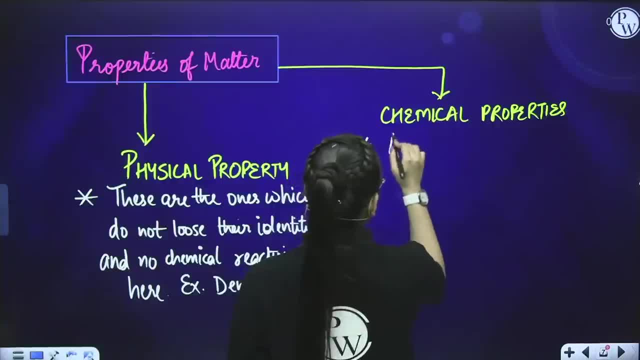 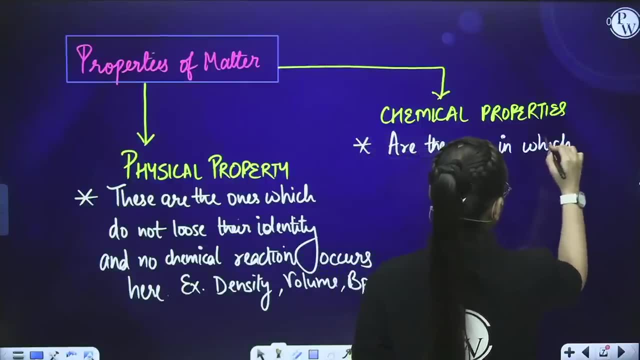 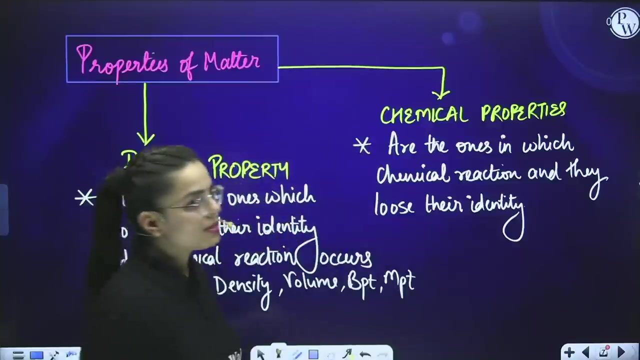 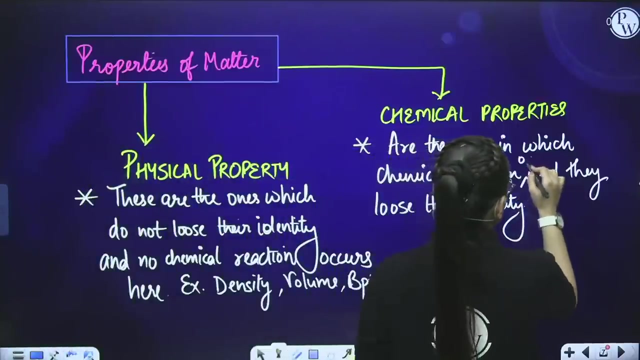 So I would say the chemical properties are the ones in which chemical reaction occurs and they lose, and they lose their identity, Okay, When they are being consumed. So, students, these are all about chemical properties in which you can add a chemical reaction occurs. 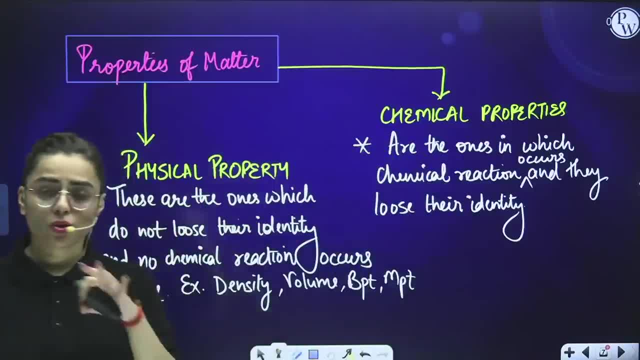 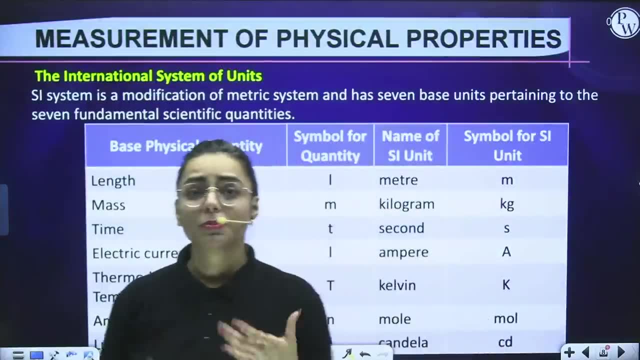 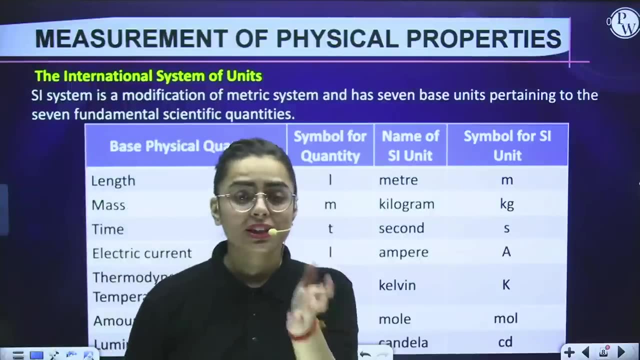 Right, Okay, So, students, this was all. this was all about the properties of matter. Now, how can we measurement, how can we do the measurement of these properties, of these physical properties, basically, which we can observe, which we can think, without any chemical change? 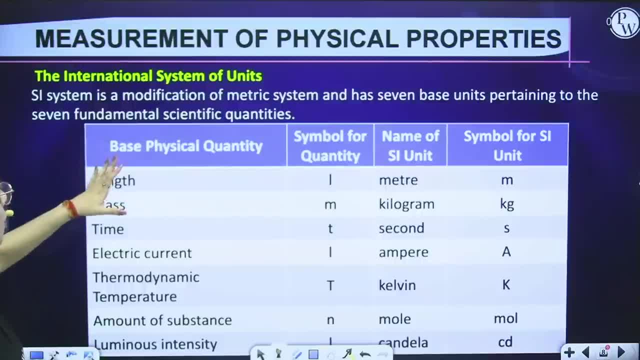 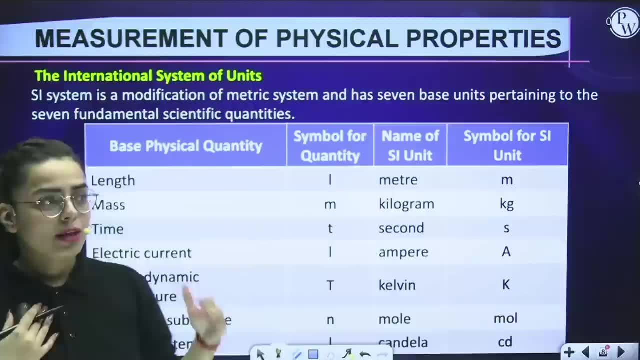 Right. So if I see here about the physical properties, we talk about the measurement. And how is measurement done? For example, if I say that I am living in my home and I want to eat some fruits or some vegetables, So what I do is 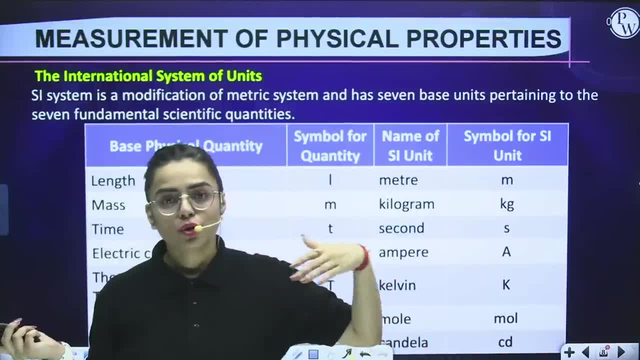 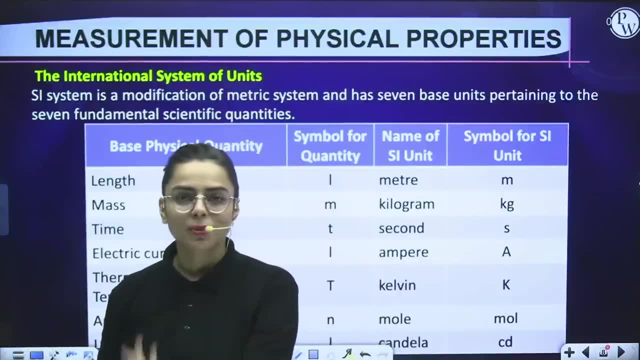 I move from a distance, I move 15, you know meters at a distance and I go to another place And what I see is there is 15 meters or 15 meters Or 15 kilometers. I am using 15 here refers to as a number. 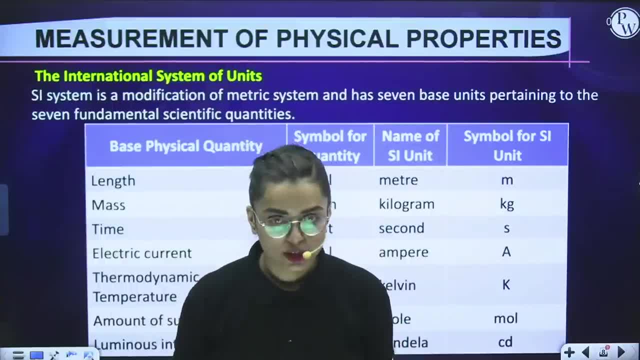 And kilometers or meters refer to as a unit, So to measurement of a physical property. to measurementize a physical property, we need to understand the basic term, that is, unit. A unit is a standard reference with the help of which we can measure any of the physical property very easily. 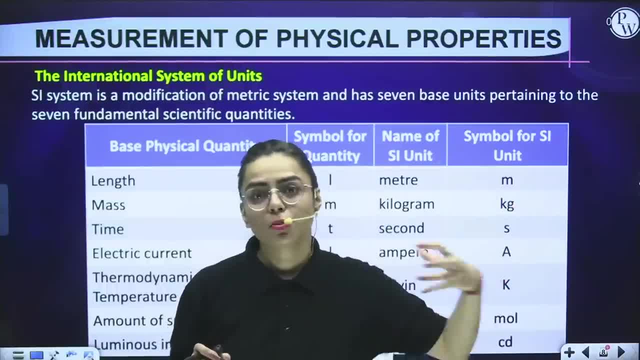 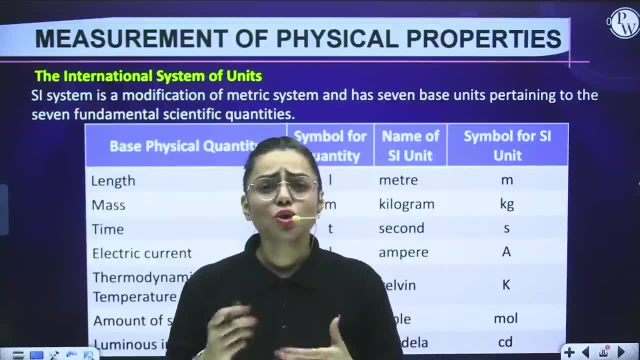 Like, we kept for distance, we kept meters, kilometers, so that we can calculate them and we can tell. For time we have kept seconds, minutes, hours. These all are units which we have kept as a standard to understand, to measure all the physical properties around us. 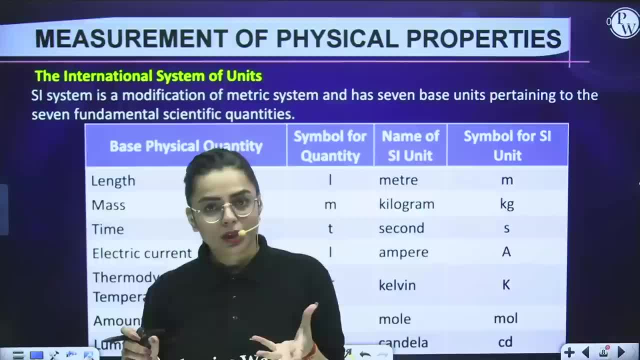 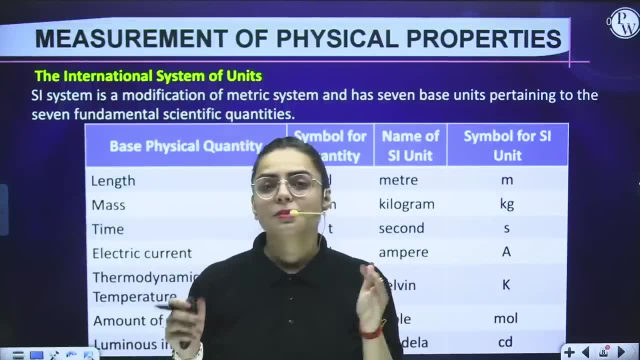 Right. So, students, now if I talk about unit, as I have explained you, unit can be further categorized into three basic categories. The number first is the basic units, Second one is the fundamental units And third one is the derived units. 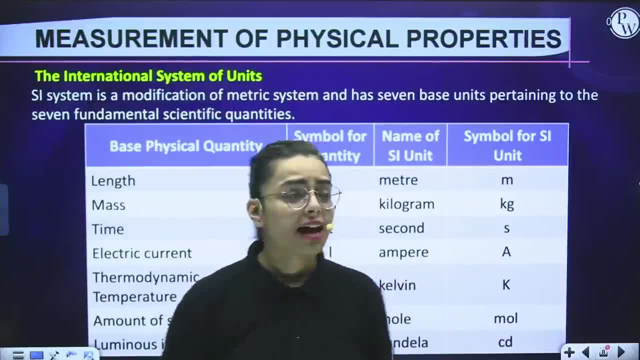 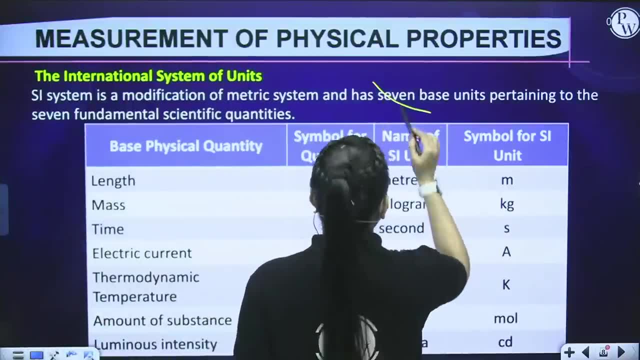 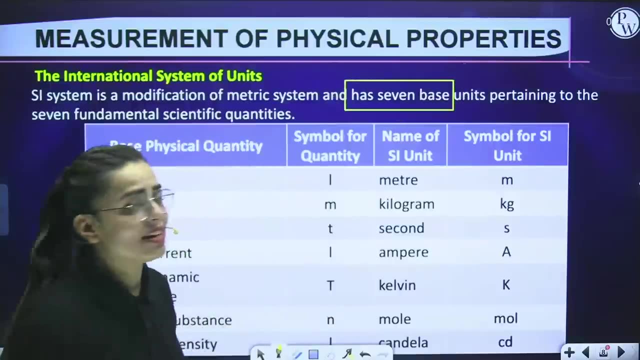 If I talk about the basic units, there are basically seven basic units. You need to please star mark the situation, I would say, Or you can put a box here In your NCRDs also. there are seven basic units. What are these seven basic units? 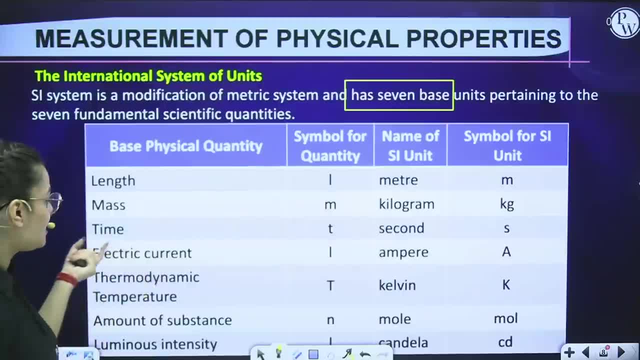 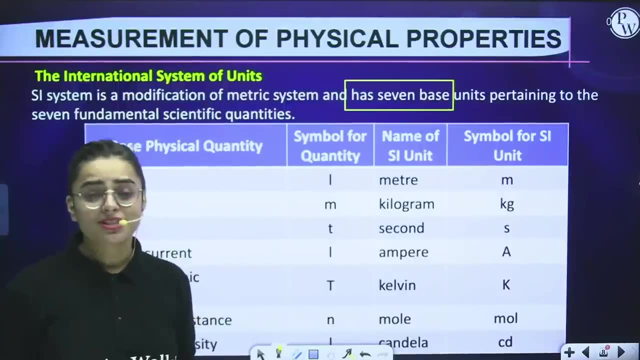 The number. first is length, The second one is mass, The third one is time, The fourth one is electric current, The fifth one is thermodynamic temperature, Next one is amount of substance And the next one is luminous intensity. So these are the basic units that we have to learn. 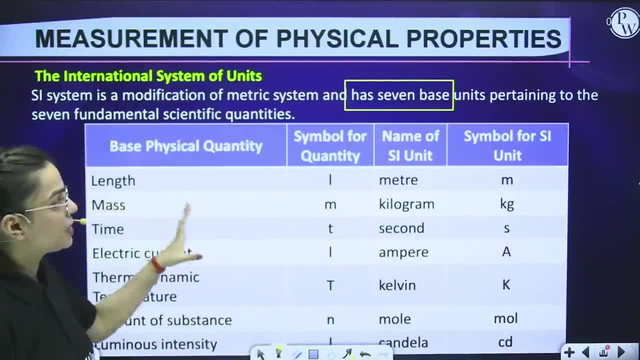 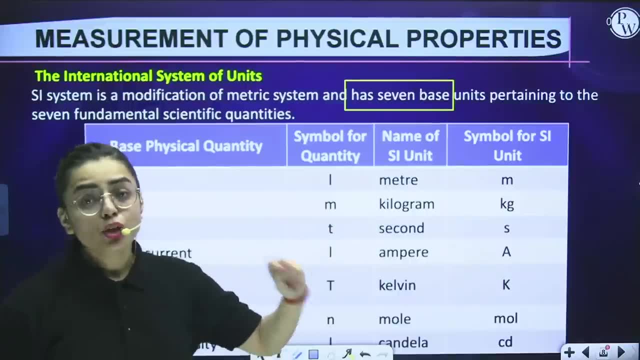 Right. These seven basic units have particular symbols for them. You know how can we represent them: To represent length, we use small letter L. To represent mass, we use small letter M. To represent time, we use small letter T. 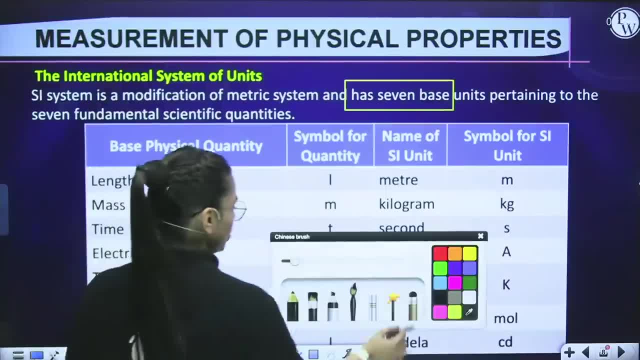 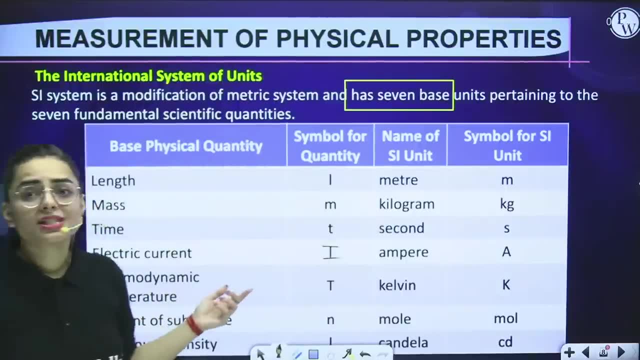 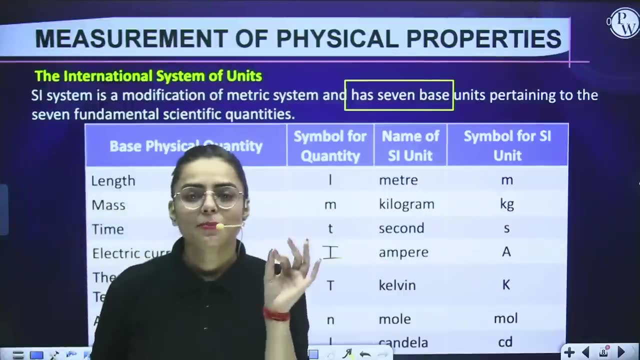 To represent electric current, students, we use I- It is capital I- To represent thermodynamic temperature. we use capital letter T Right To represent amount of substance. this is very important. It is represented by small n And you are going to study it. 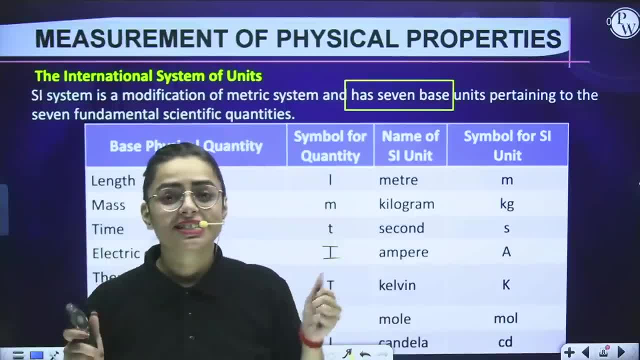 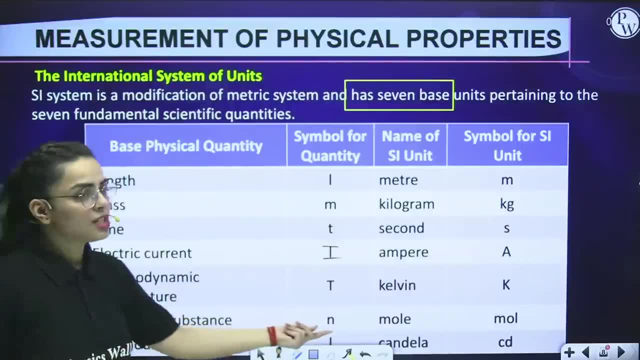 It is about mole concept. In this only chapter it is the most important and most asked topic, mole concept. So we will study this there. Okay, We represent it by small n Right. Then comes the luminous intensity That is represented by I to the base V. 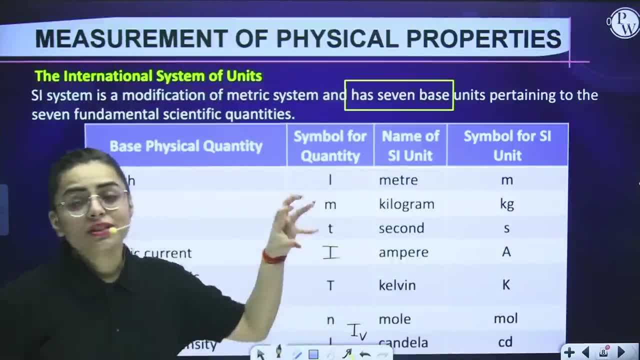 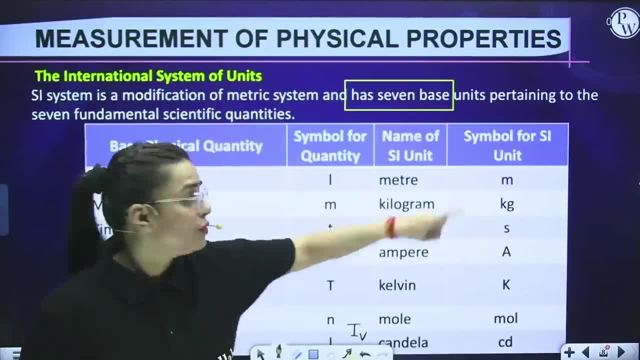 Clear Now. these all are given some units, Like length is given some unit, which is meter, Which is referred to as the standard reference With the help of which we can measure the quantity Right. So, for length, what is the SI unit? 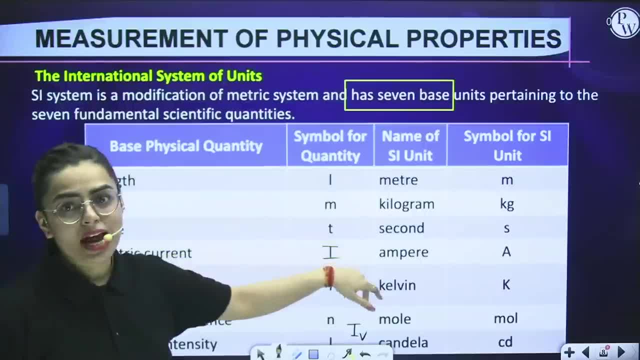 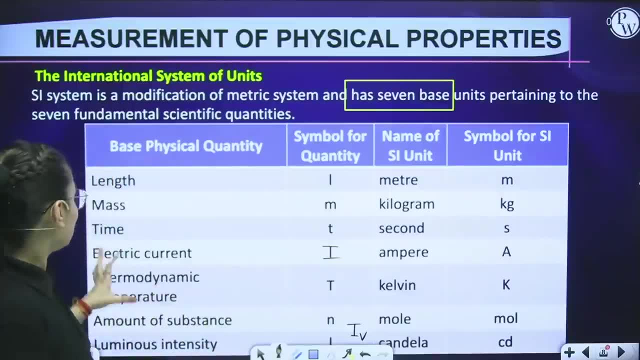 Meter For mass. what is the SI unit Kilogram For time? what is the SI unit Second For electric current? what is the SI unit Ampere For thermodynamic temperature? what is the SI unit Kelvin? 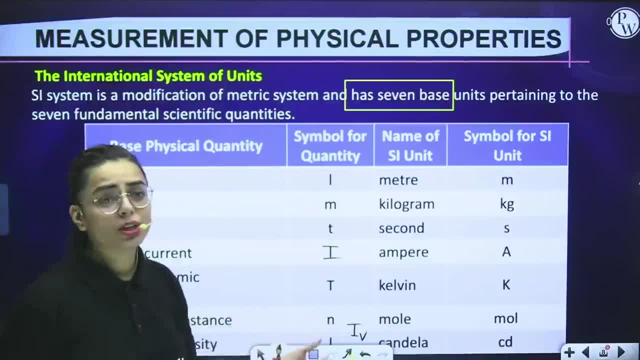 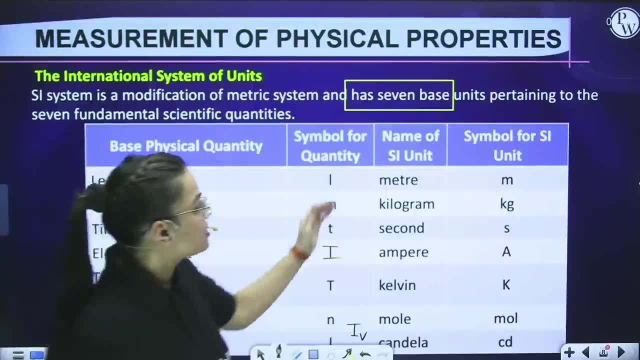 For amount of substance. what is the SI unit? Mole, For luminous intensity. what is the SI unit? Candela? Students, now these units also have a particular symbol. We don't write the big, big names, We just use the symbols to represent them. 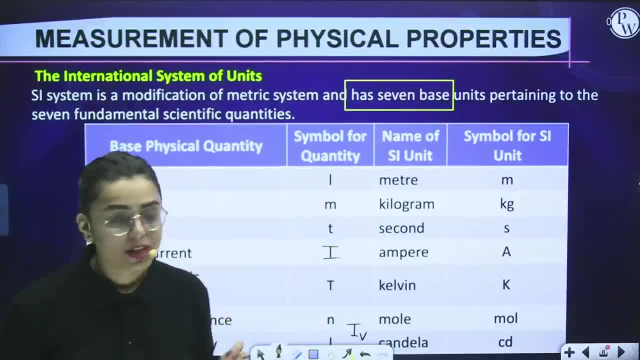 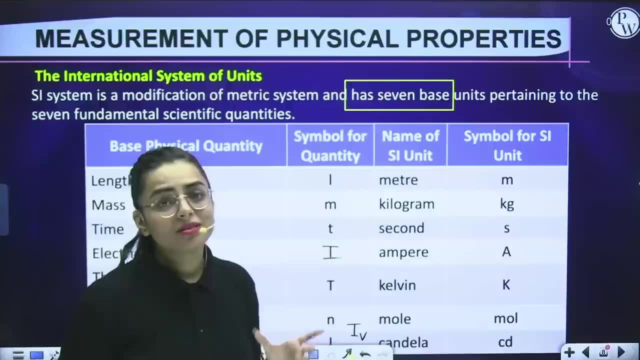 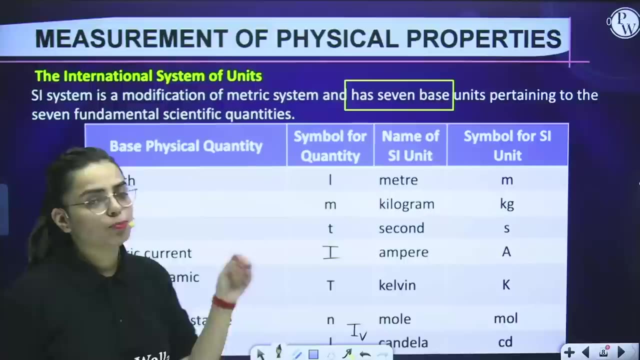 For meter, the symbol is small. m For kilogram, the symbol is kg. For second, the symbol is only small letter. s For ampere, the symbol is capital A. For Kelvin, the symbol is capital K For mole, it is mol. 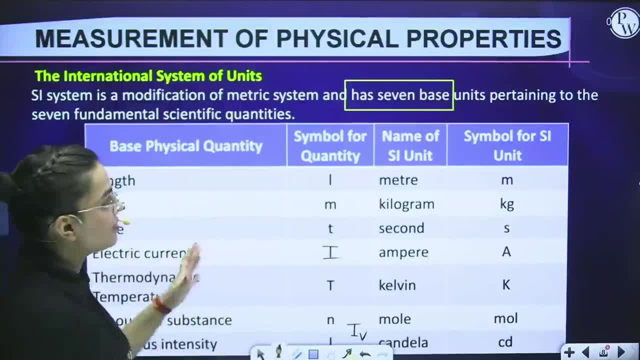 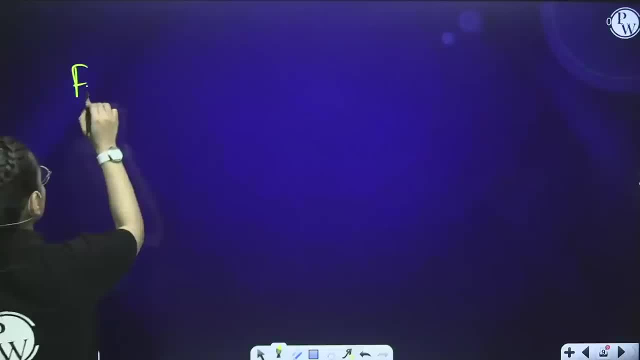 And for candela it is cd. So these were the seven basic units that you need to understand, Students. now comes the second category, That is, the fundamental units. That is, the fundamental units. Now, what are fundamental units, students? 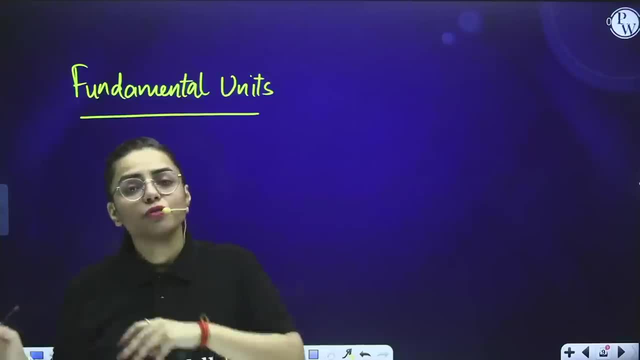 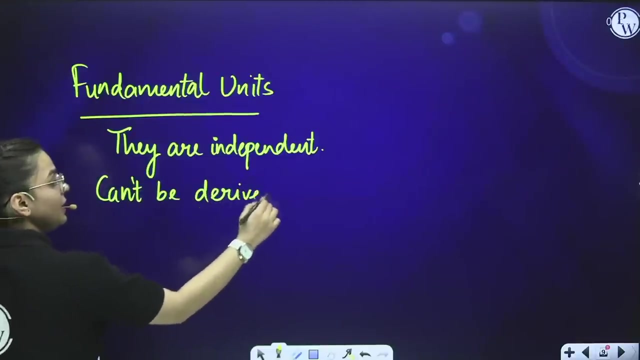 Fundamental units are the ones that cannot be derived from any another units. They do not depend on any of the unit. you know They are independent, Can't be derived, Can't be derived. We cannot derive these from any another units, From any units. 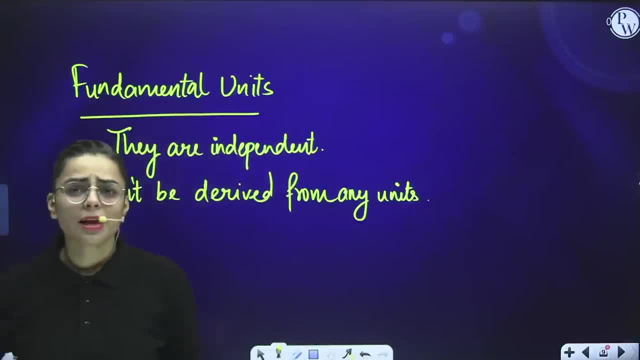 So these are the fundamental units. Fundamental units are basically the unit of mass, the unit of time, the unit of length, right. So now next comes the types of unit which are referred to as the derived units. The derived units: 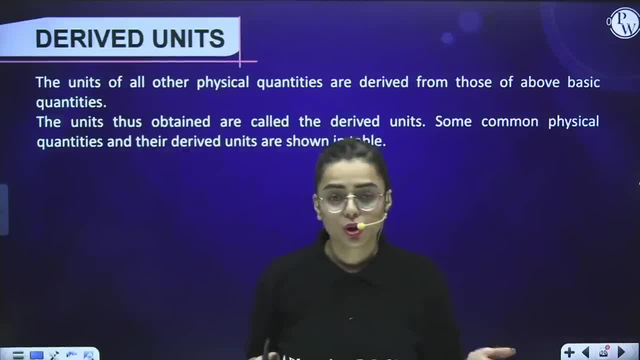 Derived units are the one that can be derived, you know, from the basic units. For example, if I take an example of area Students, if I talk about area, If I consider about square, what I see, Square has sides, equal sides, right. 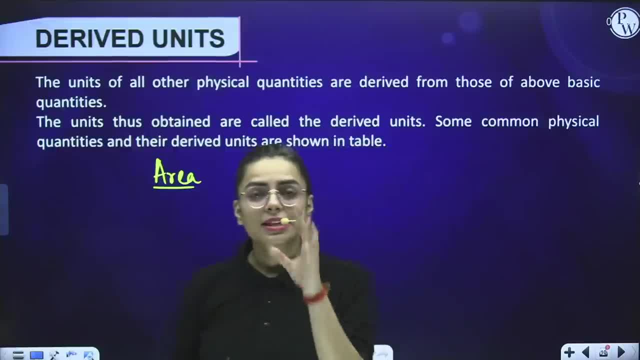 And if I say that each side has a length L, right, Or you can say A- when we consider this in mathematics, Don't worry, In mathematics there are some concepts that students feel that it's very tough. Don't worry. 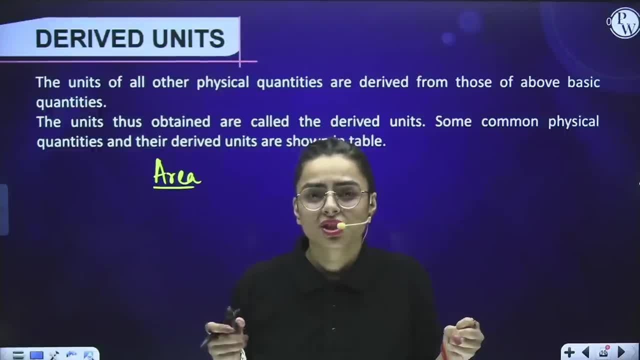 In mathematics there are some concepts that students feel that it's very tough, And in chemistry also in numerical portion. Ma'am, how we'll do that? Our maths is very weak, So don't worry, I am there for you. 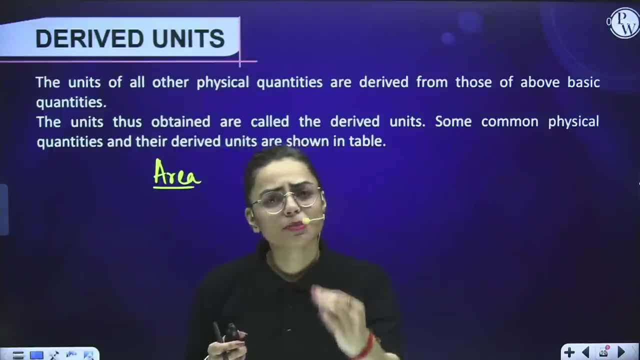 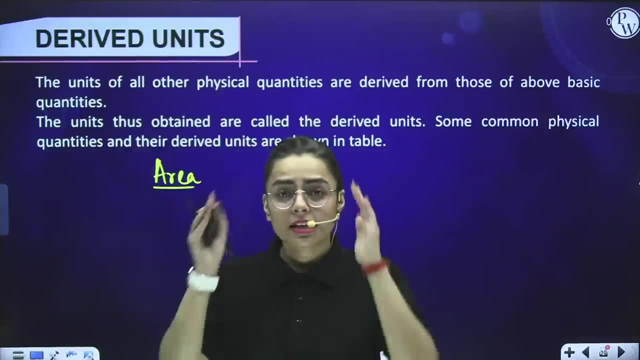 And the maths which you need in chemistry. I am going to explain you, So no need to worry. Just you need to understand it, Need to make notes by hand. First listen from me and then write accordingly, And just practice, practice, practice. 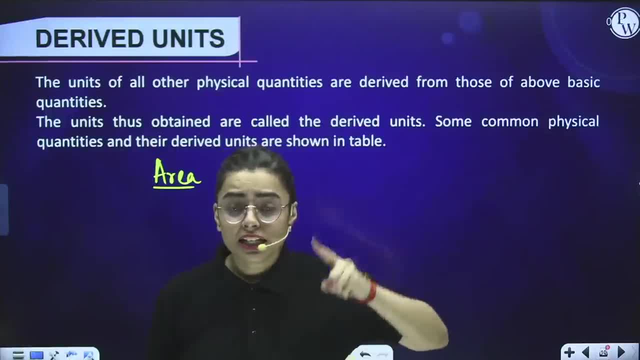 Because when you practice, that practice will lead you towards the victory, You know clear. So practice is the most important Right Now. see, I am talking about area, And if I talk about square, what is the formula of area? 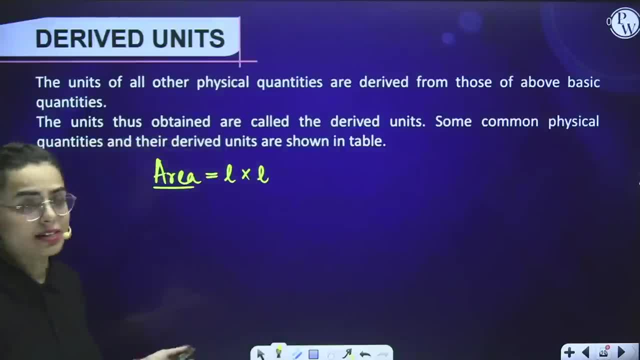 It is length into length. And now only we have started. You can see, in this case, length, Length, is one of the basic unit, And when I multiply one basic unit into another basic unit, that means I am deriving something, So hence it comes under derived units. 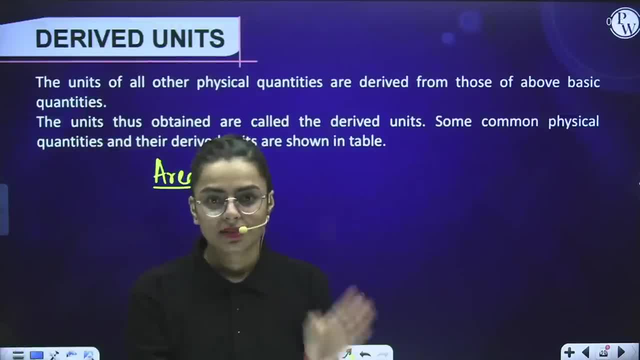 Are you understanding? If I am only talking about length, that is our basic unit. But if I am talking about length into length, that means I am deriving something. And when I am deriving something from the basic units, they are referred to as derived units. 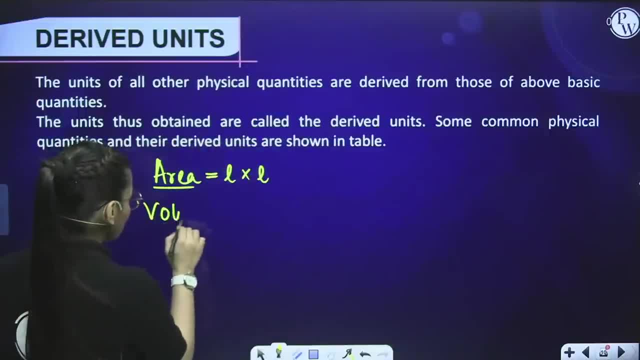 So here, one of the most- another example I would say is volume. In the case of volume, what is the formula? Length into length, into length, Right, Yeah? Otherwise, I would say: length into breadth, into height. All you can say is this: Right. 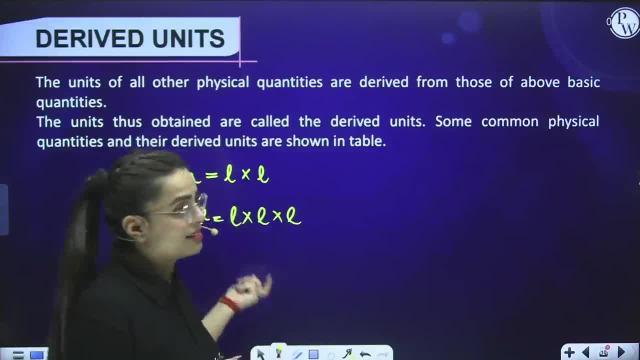 So that is volume. Here also it is derived. Why it is derived? Because length is a basic unit And when we multiply one basic unit into another, into the third one, it is the derived units. Now let us read this: 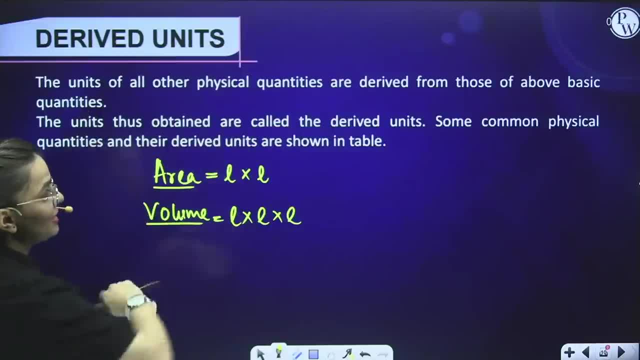 What is given here. The units of all other physical quantities are derived from those of above quantities which we have studied already. Right, These units thus obtained. these are thus obtained are derived units: Area, volume. these are now derived units. Some common physical quantities and the derived units are also given to you in this following table. 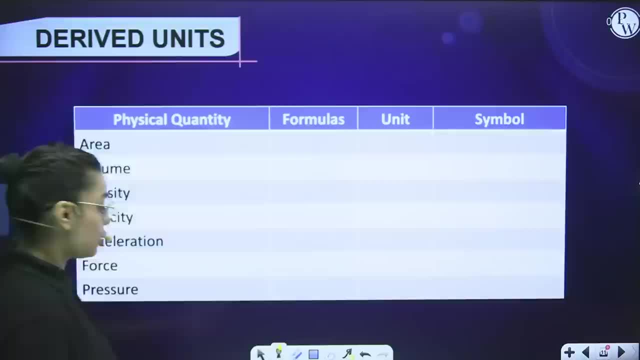 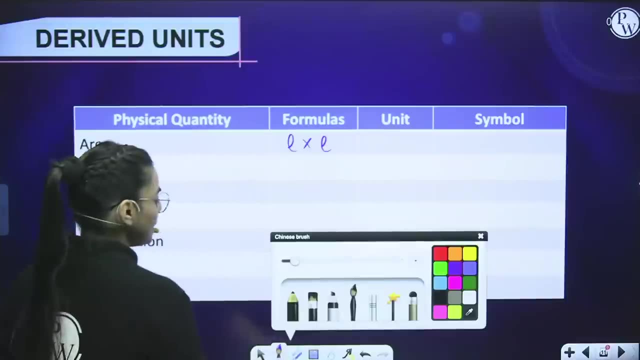 Now let us see that The number first is area, which I have already told you Students. it has a formula. What is the formula? Length into length. Now coming towards volume, I already told you, its formula is length into length, into length. 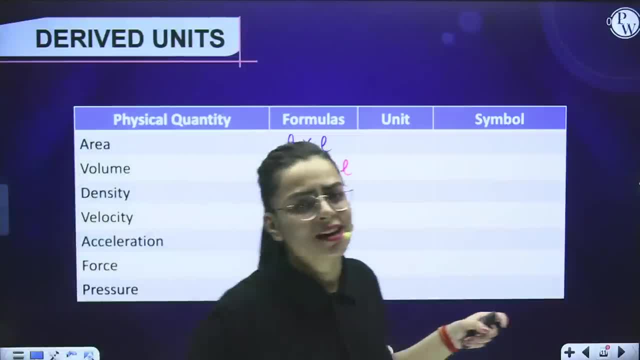 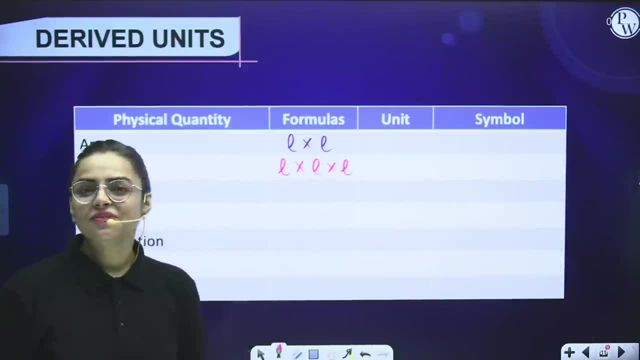 Now coming towards density, the most easy formula, which we have started in the small classes, And if you have not started, no need to worry, You are studying now, Right? So density formula is mass by volume, Right? What is its formula? 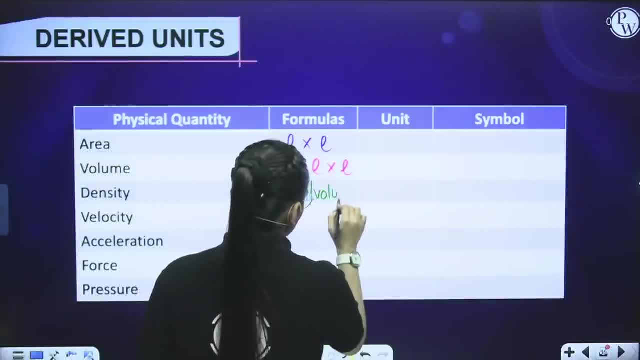 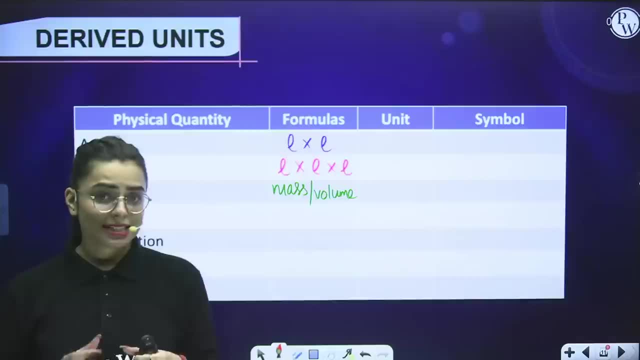 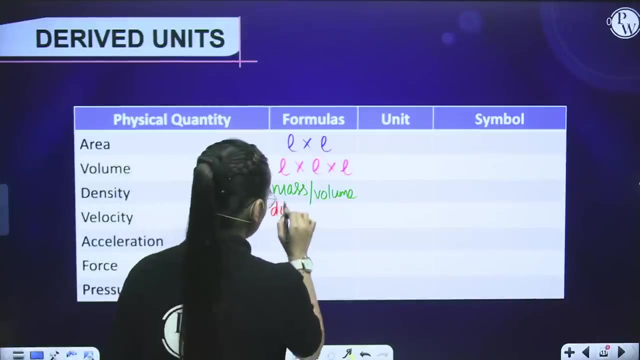 Mass divided by volume. Right Okay, students. Now let us see the next case, that is velocity. Velocity is distance upon time. You have studied it in physics, also in class 10th. So it is distance upon time, Right Okay? 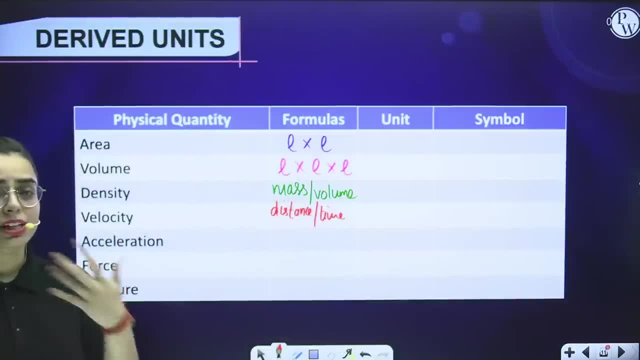 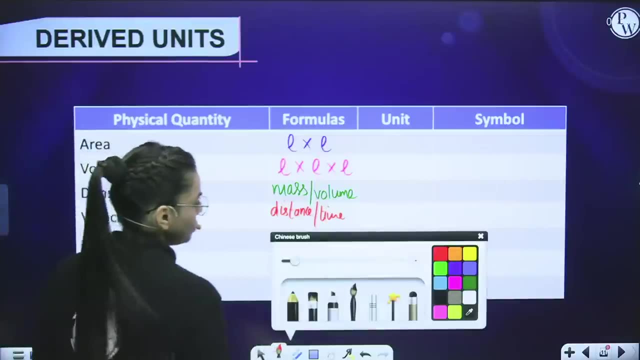 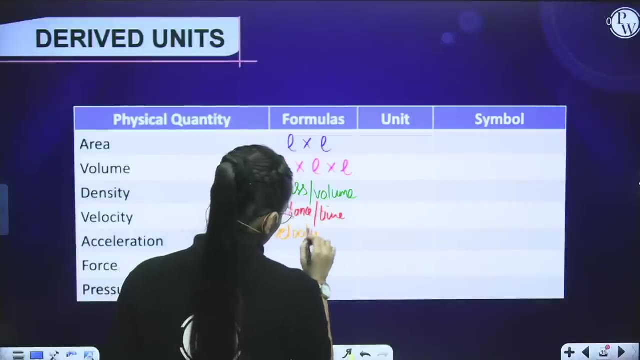 Coming towards the next acceleration. to derive acceleration first you need to calculate velocity. So when you calculate velocity just divided by time, you will get acceleration. So what is the formula of this? now? Okay, The formula is velocity divided by time. 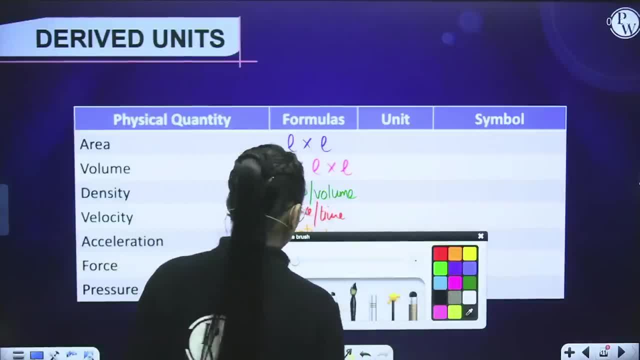 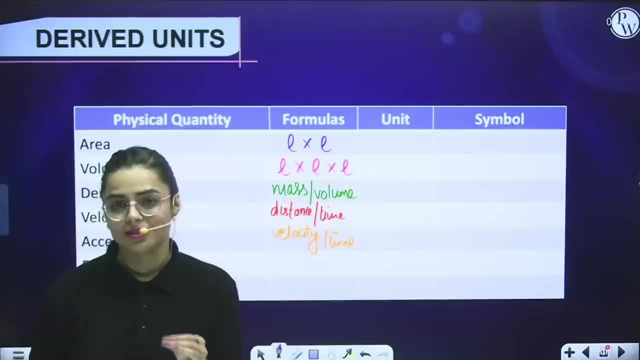 Okay, Now coming towards the next part, that is our force. What is force, students? Force is basically refers to as mass into acceleration. Right Force is our mass into acceleration And if I talk about pressure, pressure is force upon area. 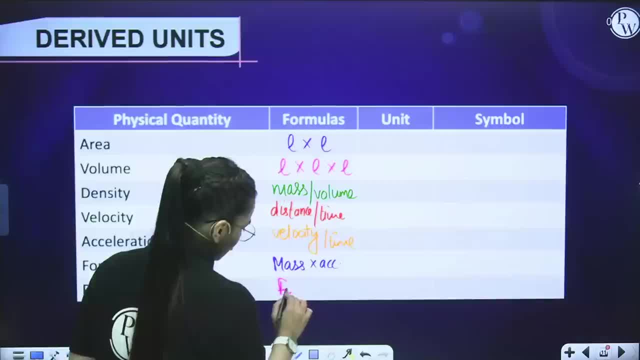 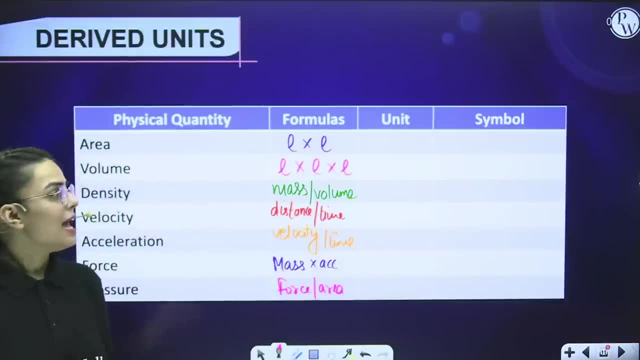 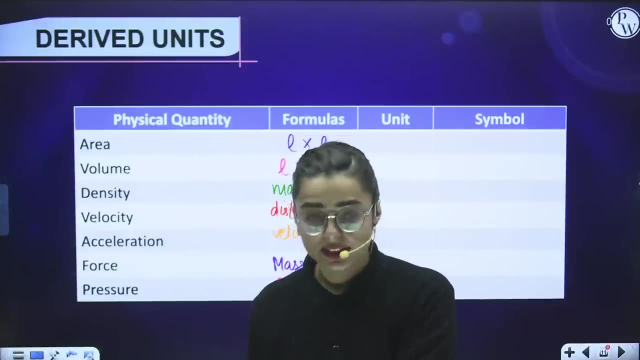 So first you need to calculate force for that, Right, Okay, Now if I talk about the units here, First of all, if I talk about area, as you know, length into length, First tell me In the basic unit now we have seen that length has a SI unit, which is basically meter. 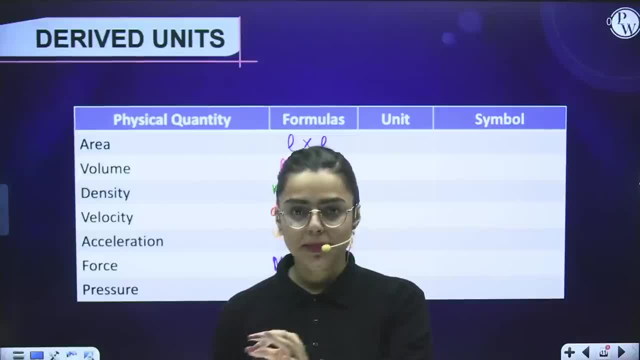 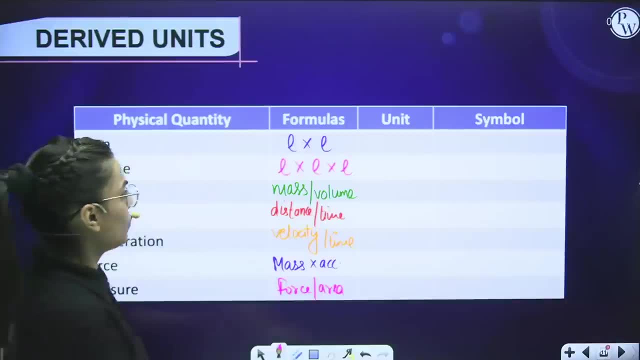 Length has an SI unit which is meter Right So SI unit. the international system of units we have studied just right now, the seven basic units are those Right So meter into meter, all I would say is meter square. 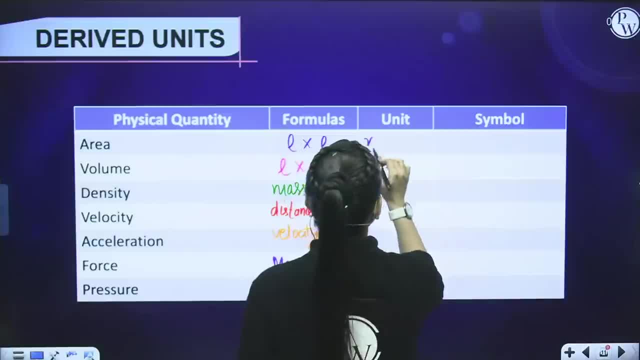 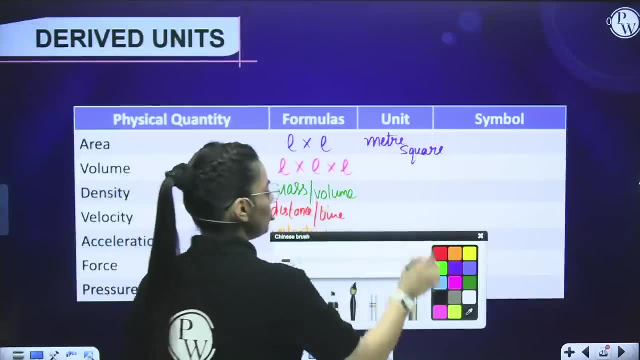 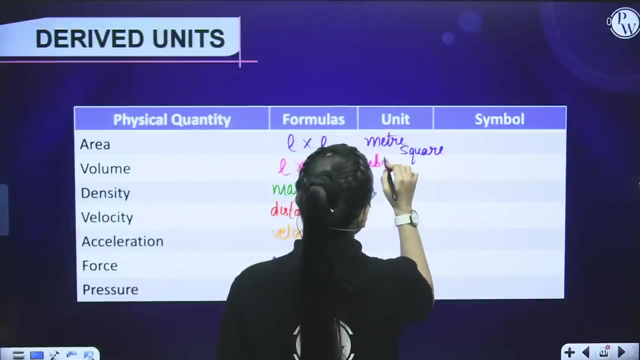 Right, The very first one is meter Square. If I talk about volume, Now see meter into meter into meter. What is this now? Meter into meter into meter is cubic meter, Right, So it has unit as cubic meter. 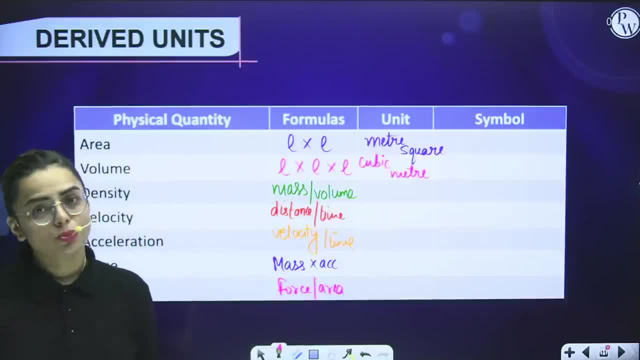 Now, students, coming towards the density, mass by volume. First you need to understand mass Mass. we have already started in the basic unit: It is kg, Its unit is SI, unit is kg And volume its unit. we have already calculated cubic meter. 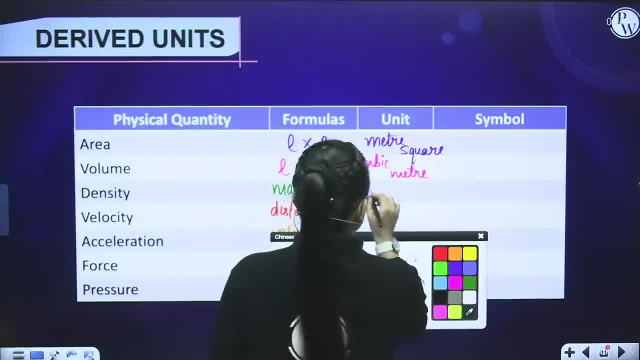 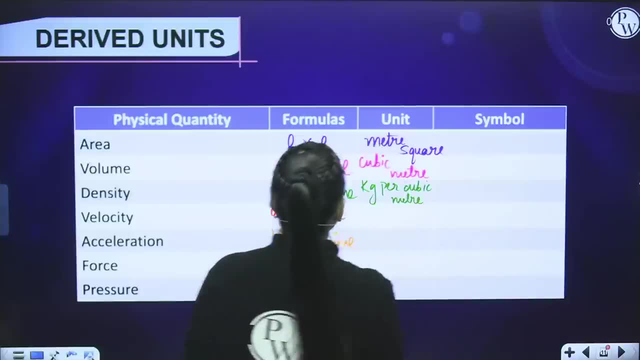 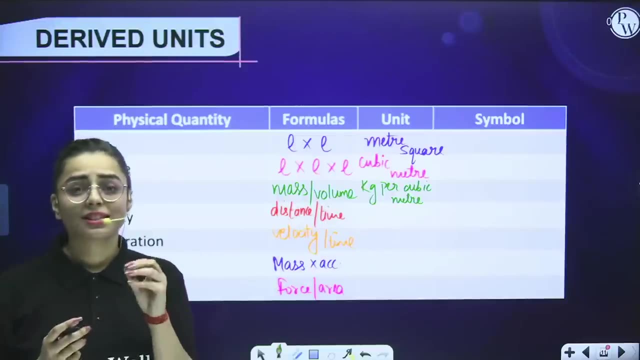 So hence we can write here Kg per cubic meter. So now coming towards velocity, it is distance. upon time That means we need to write the distance SI unit. The distance SI unit is- again we know that it is the meter. 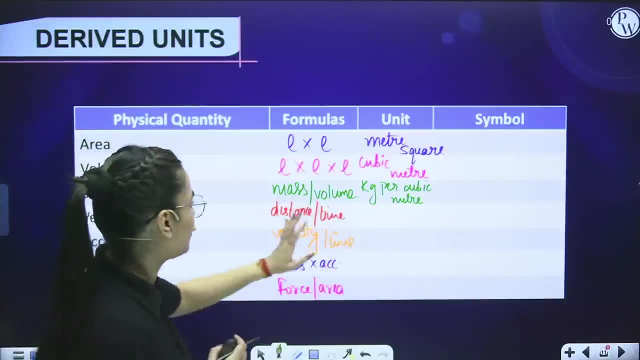 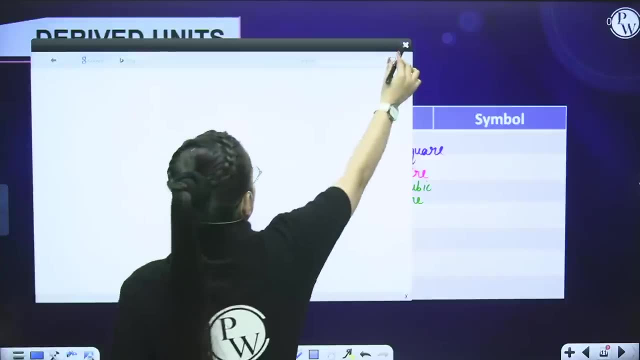 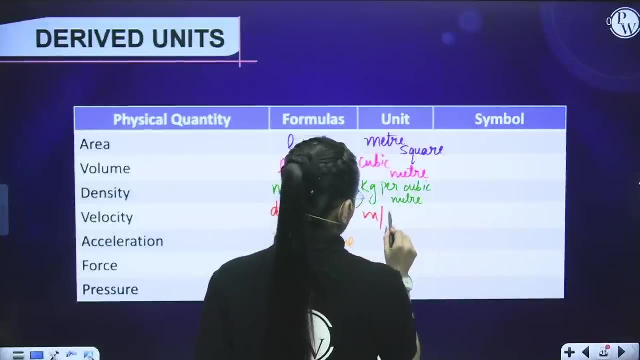 Like if I say I have travelled this much meter, So that is our meters, And then if I talk about time, it is second, Right. So if I say you hear, okay, meter per second. Now, as you all know, acceleration is velocity by time. 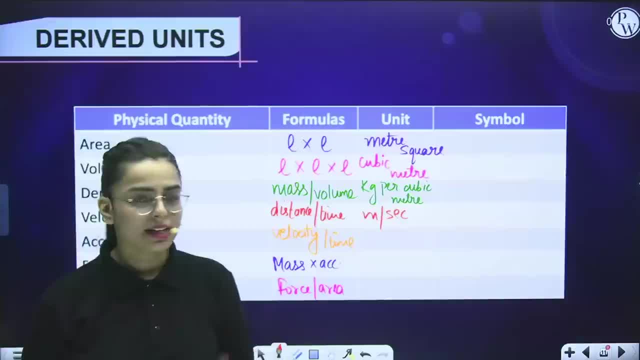 And we have already calculated the unit for velocity. It is meter per second, And time is already second. So first we will write velocity, Now it is per time. So again time, That means again seconds. 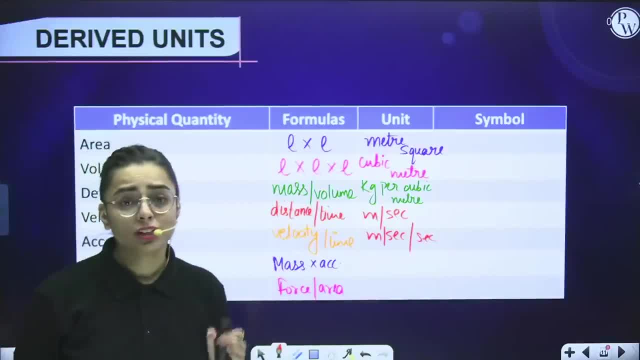 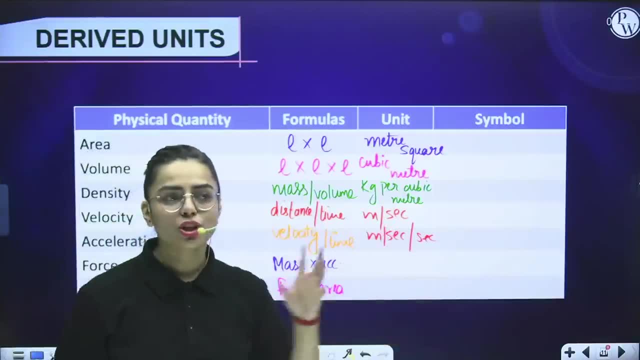 Right Now coming towards force, Force is mass into acceleration And we know that mass is what Kg, Kg And what is acceleration. Acceleration is meter per second, per second. So in short, we can write: it is Newton. 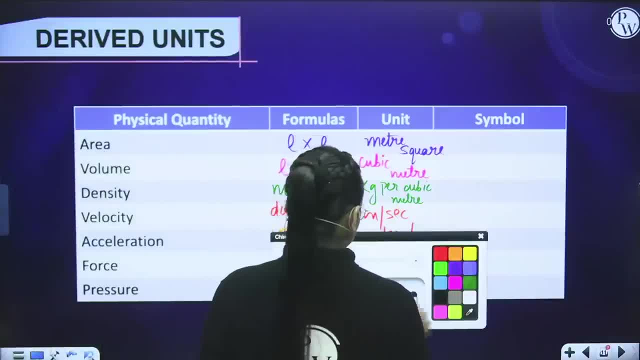 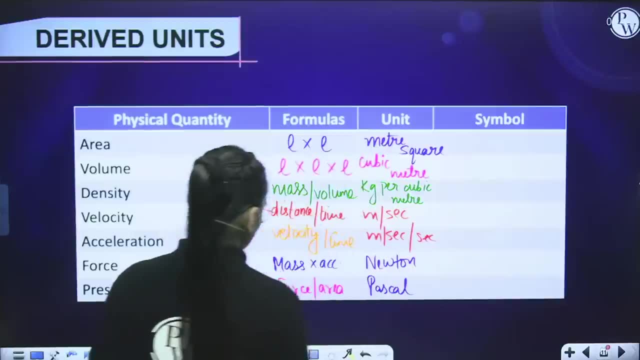 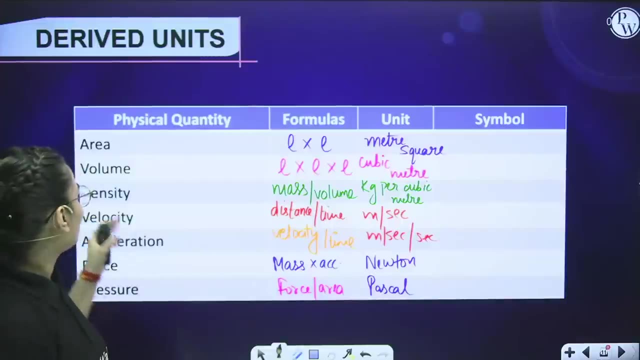 It is Newton, And if I talk about pressure, it is Pascal, Right? So these were the units. Now, for these units, we have to students write some symbols. Okay, For area we write a symbol Like for meter square. its unit is meter square. 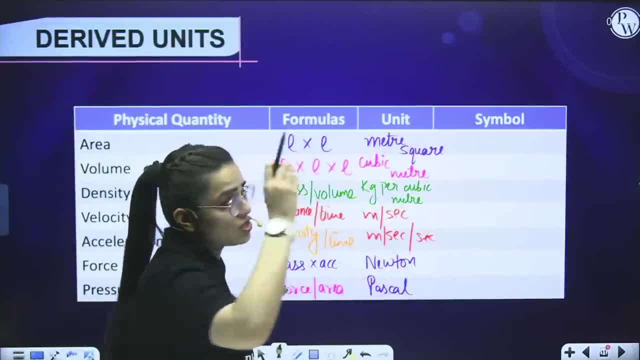 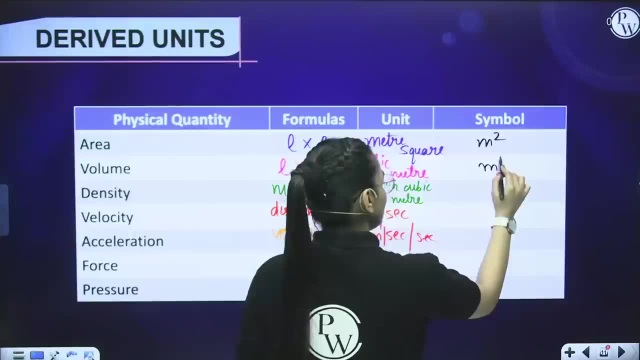 To represent it. we don't write such big names, We just use symbols to representation. Right For meter square we will write meter square For volume, its cubic meter, Then meter cube. Next is kg per cubic meter, Then we will write kg per cubic meter. 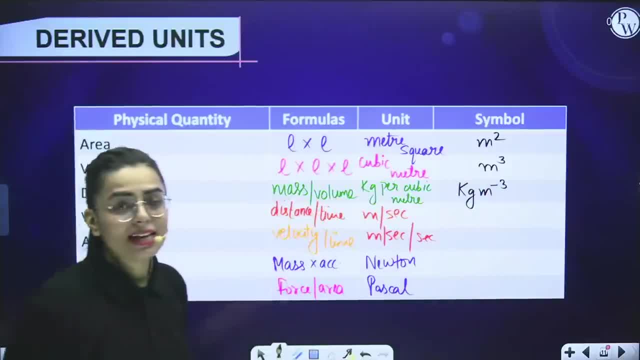 That means meter power minus 3.. Right After that, students, that is our meter per second. The next one is velocity, which is meter per second. So we are going to write meter second power minus 1.. Then comes our acceleration. 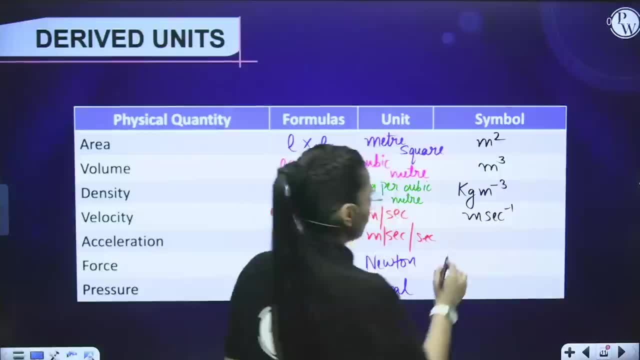 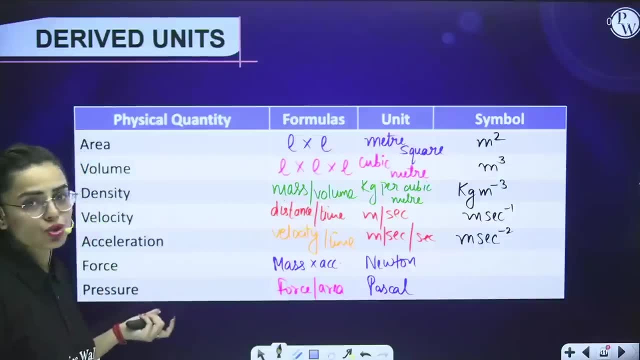 Acceleration is meter per second, per second, So we have to write it meter per second minus 2.. Right Then, next one which arises is force. Students, force is Newton, So we will write it with capital N, We will write it with Pa. 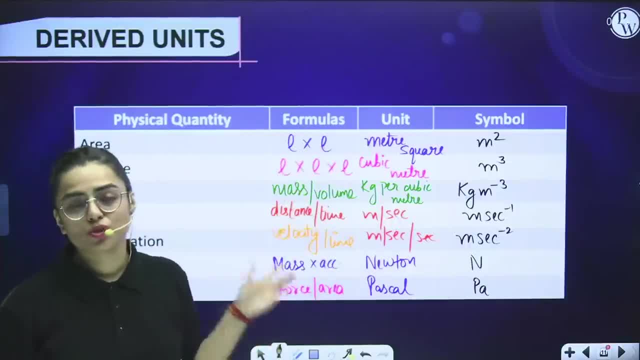 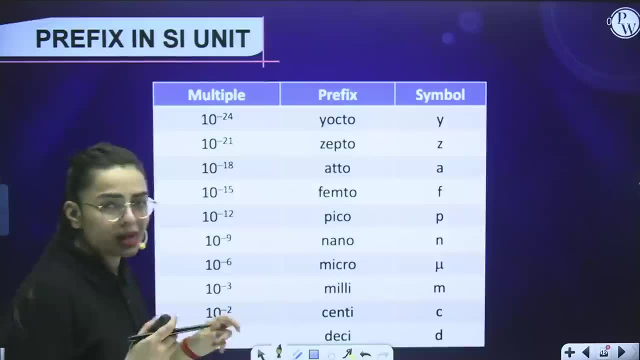 So these were the symbols of these derived units which we have calculated Right. So these were all about derived units. Now come the prefix in SI unit. What happens, students, when we, you know, do some questions? 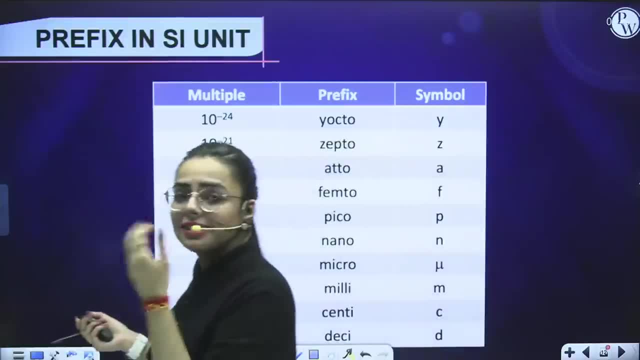 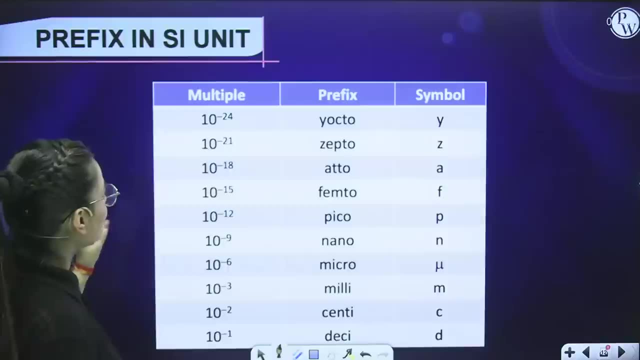 we observe that there are some numbers which are seen in decimal, in fraction. For these numbers we use some certain prefixes for the SI units. For example, in some cases you have seen that there is somewhere written: millimeter, nanometer, decameter. 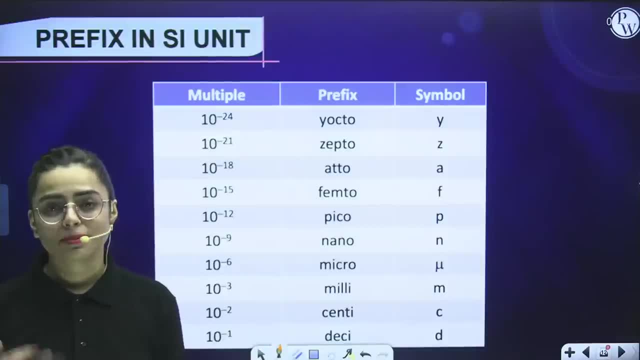 So what are these? These are the prefixes that are used for decimal fractions. all these cases, Right. So the very first which you observe, which you have seen, for 10 raised to the power minus 24, we write it as y-octo and the symbol is used as y. 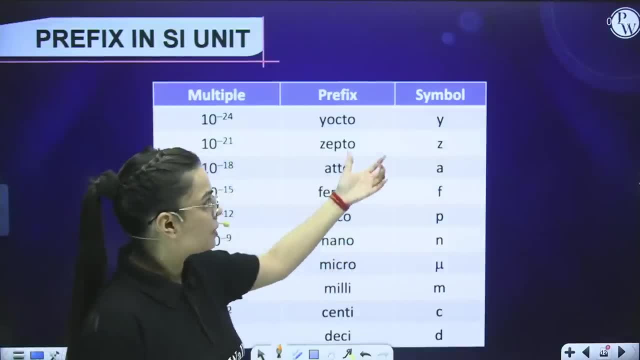 For 10, raised to the power minus 21,. we use prefix zepto and the symbol is z. See, you have to just read it once, That's it. It is not like you have to cram it. Okay, No, no, no, not at all. 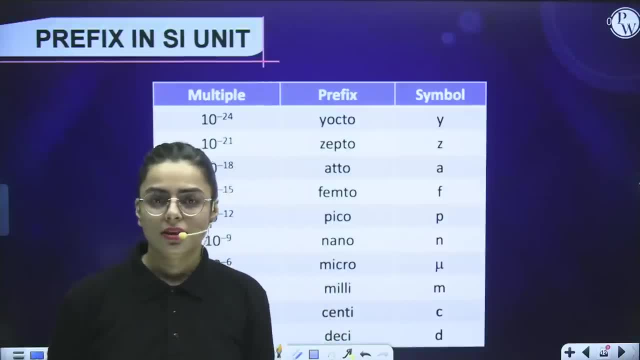 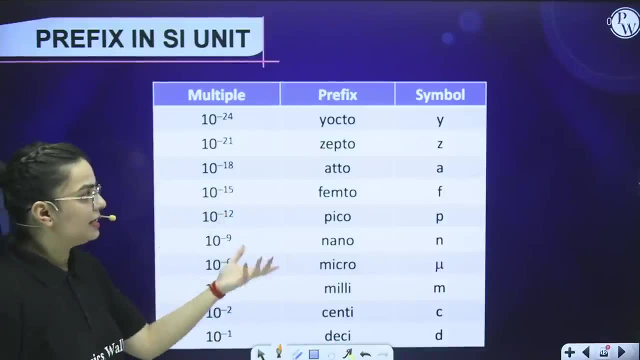 You just have to read it once, Otherwise thrice. that's it. And the ones that are most important. I will tell you to put a star mark on it, Right? The next one is 10 raised to the power minus 18,. 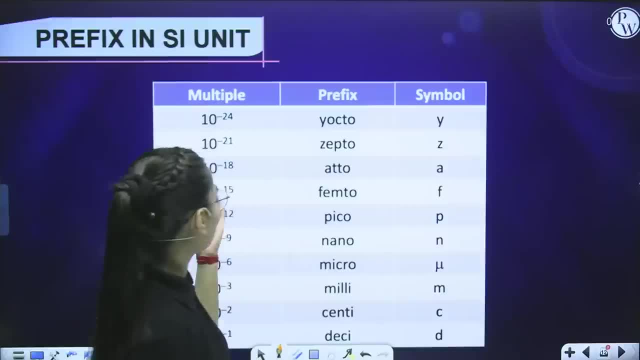 which is atto symbol is small a. Next is 10 raised to the power minus 15,, which prefix is femto and the symbol is small f. The next one is 10 raised to the power minus 12, whose prefix is pico and the symbol is small p. 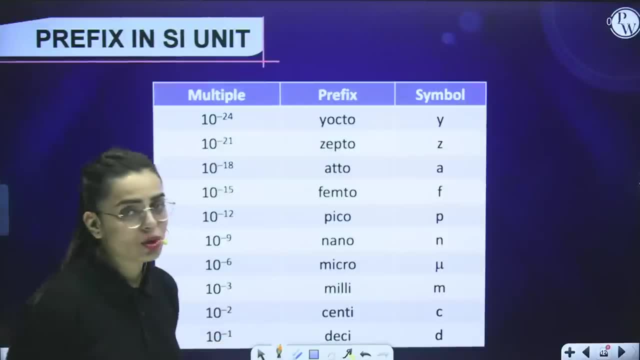 The next one is 10 raised to the power minus 9,, whose prefix is nano and the symbol is small n, which is important, As I told you. I will tell you to mark this one. The next one is 10 raised to the power minus 6,. 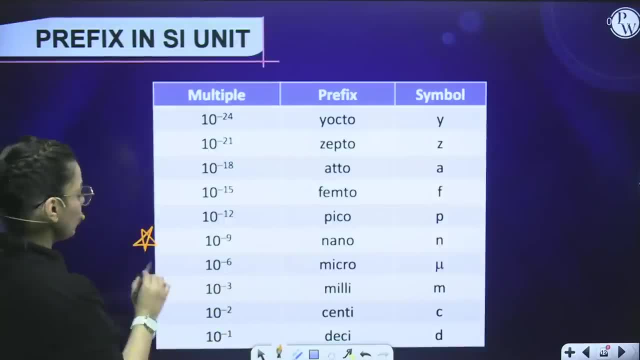 which is known as micro and the symbol is mu. Okay, This one is also important. The next one is 10 raised to the power minus 3, which is represented as milli and its symbol is small m, While the next one is 10 raised to the power minus 2. 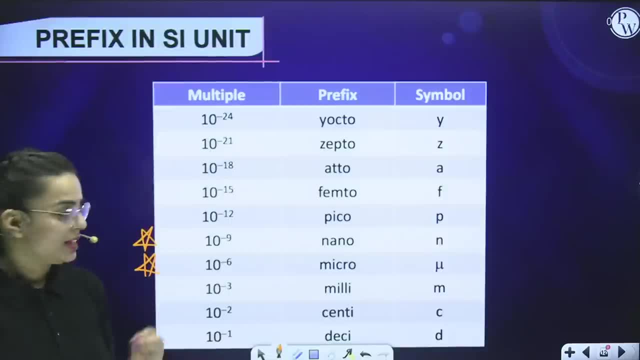 and the prefix is centi. symbol is small c. The next one is students, known as desi. Desi is 10 raised to the power minus 1.. Symbol is small d. So these are important which I have been marking star for you. 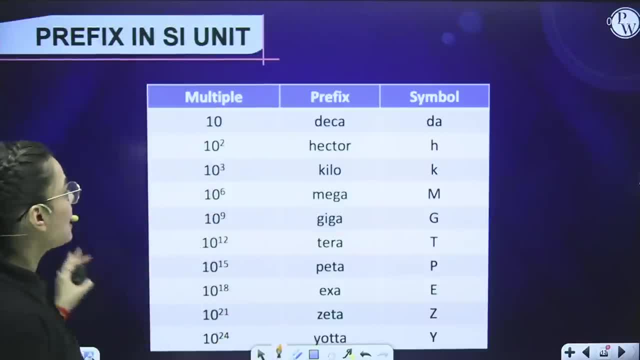 Right Now, coming towards the next of the cases, we have only 10, whose prefix is deca, which is represented by da. The next one is 10 raised to the power 2, which is hectare symbol is h. Then is 10 raised to the power 3,. 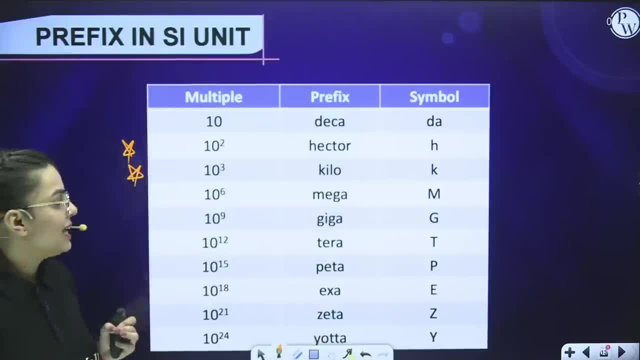 which is kilo symbol is k. Then is 10 raised to the power 6,, which is mega, which is capital M. Next is 10 raised to the power 9,, which is giga, which is capital G. Next is 10 raised to the power 12,. 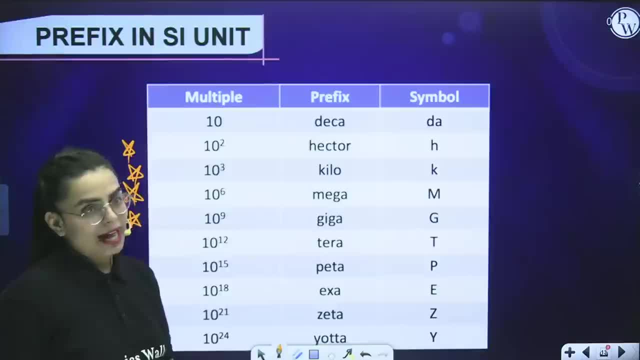 which is prefix, is tetra, represented by capital T. The next one is 10 raised to the power 15, prefix is peta, represented by p. Next is 10 raised to the power 18, exa, represented by capital E. 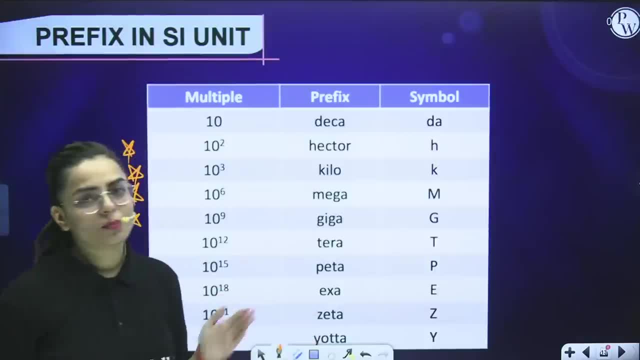 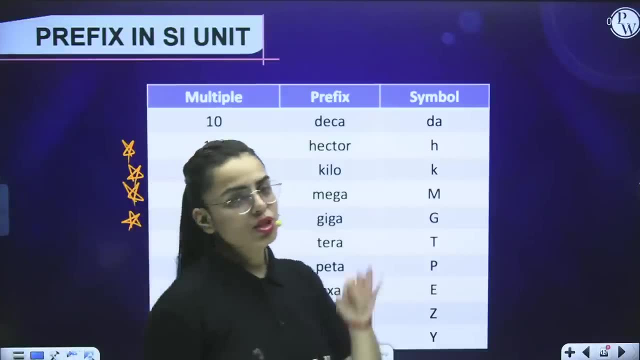 The next one is 10 raised to the power 21,, which is zeta, represented by capital Z. And the next one is 10 raised to the power 24, which is zoita, represented by y. So, students, you don't have to learn it. 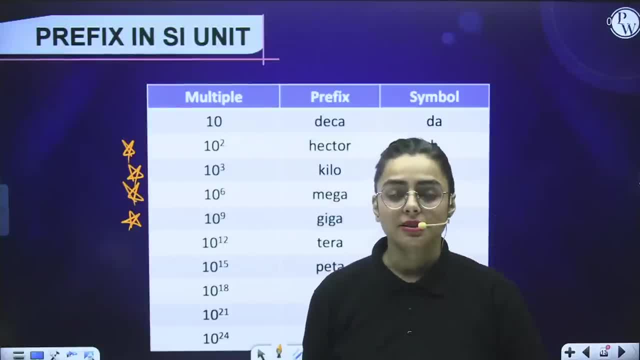 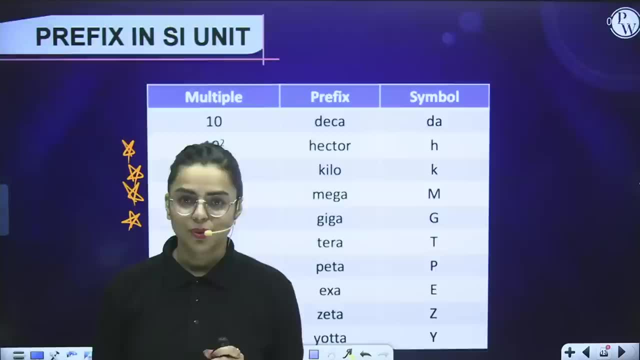 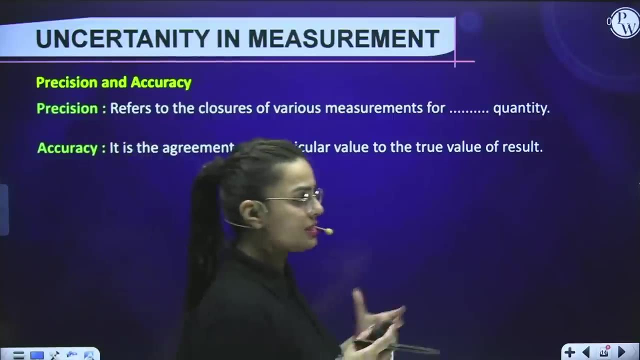 am again saying: just read it once, twice or thrice. that's it. and from ncrt you can directly mark the star ones. that's it clear. so these were all about the derived units. hence we have covered the topic units. now, students, coming towards the uncertainty in measurement, what is measurement? 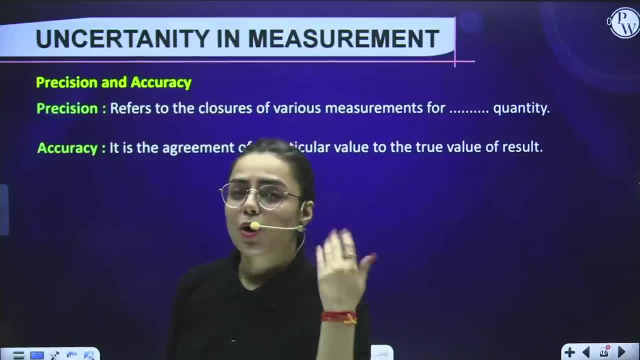 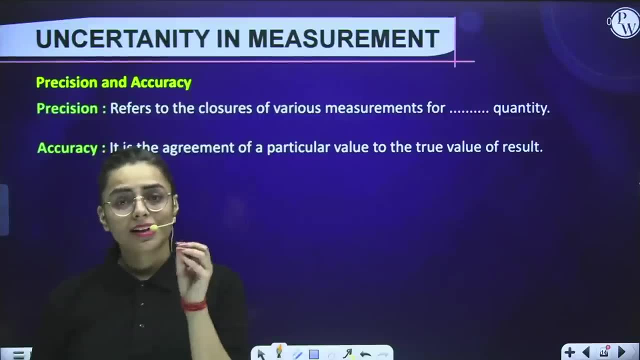 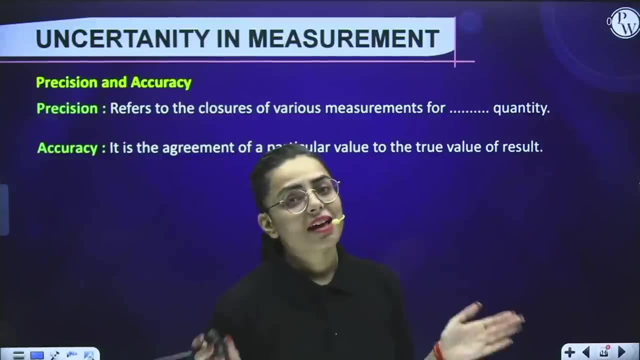 we have studied how to you know the properties of measurement and the measurement of physical properties. we have all covered this topic. now coming towards the uncertainty. uncertainty refers to as if i say some number is 1.98, 1.96 in decimals or in fractions. that is uncertain. what? 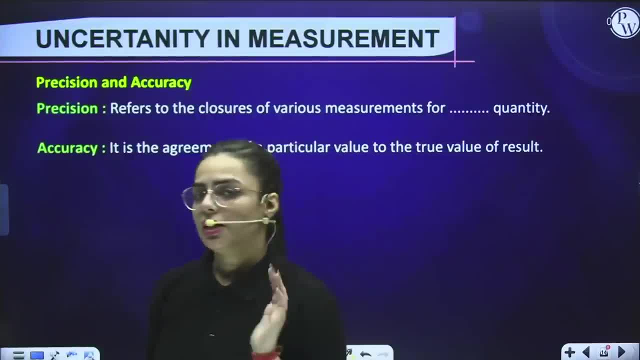 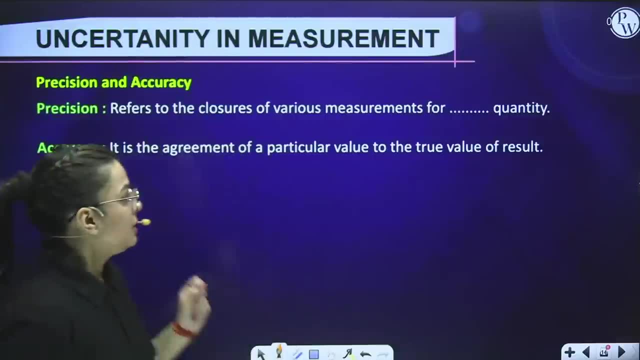 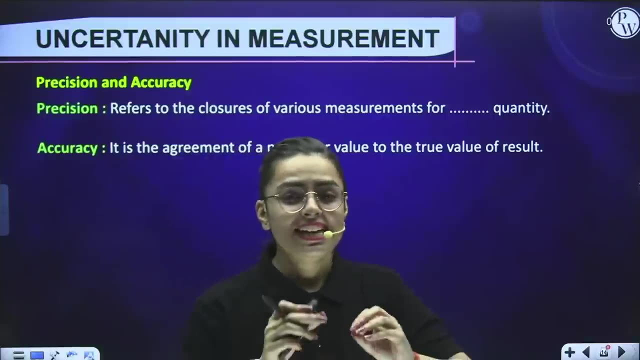 is certain, like a particular number: one, two, three, four, five, six, seven. so uncertainty is something that is, something is wrong in this. you know there is some uncertainty in that measurement. so here, two terms which we need to understand is precision and accuracy, which we are going to explain you in. 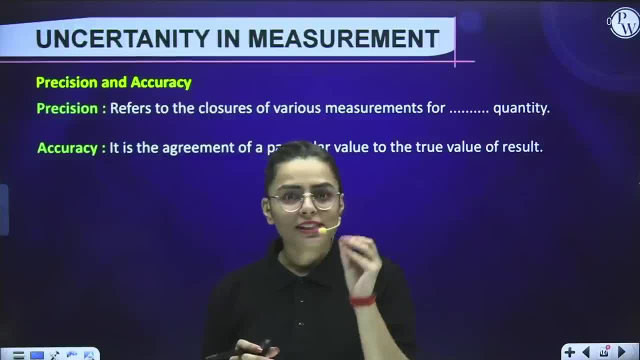 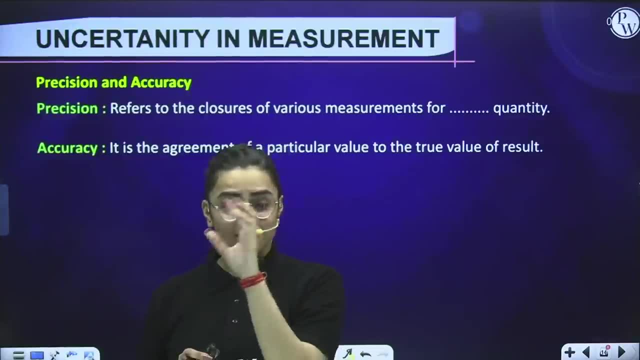 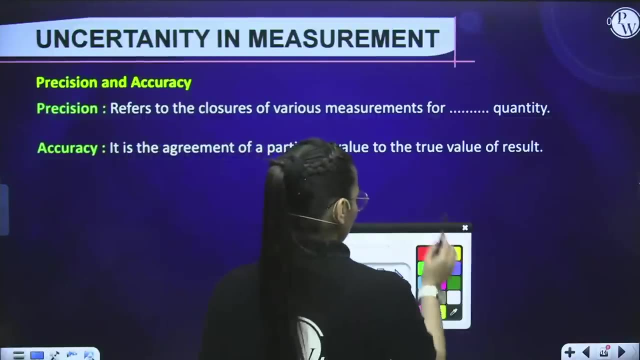 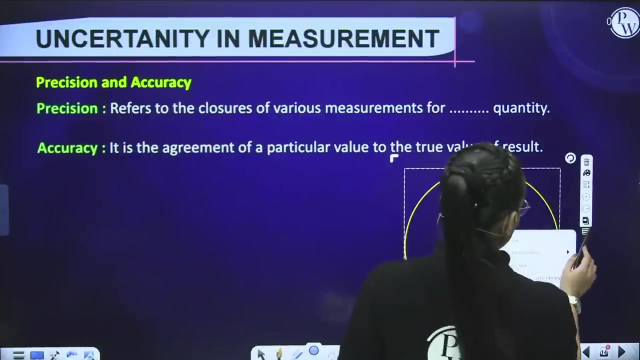 a very funny manner, you know. um, now i will take you towards your childhood. you know, okay, how many of you students have played dark- you know dark- board game. what was that? let me tell you. let us draw it first. okay, let us draw it first. it it looked like this, you know, it looked like this one. 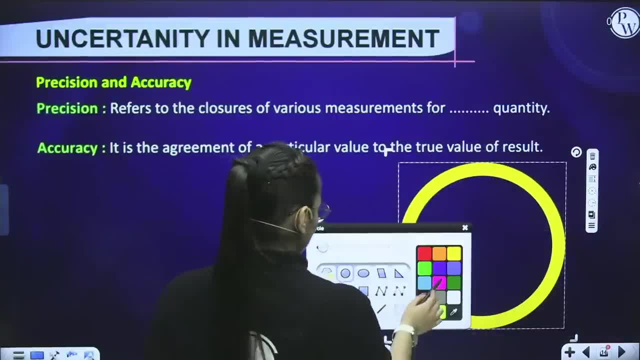 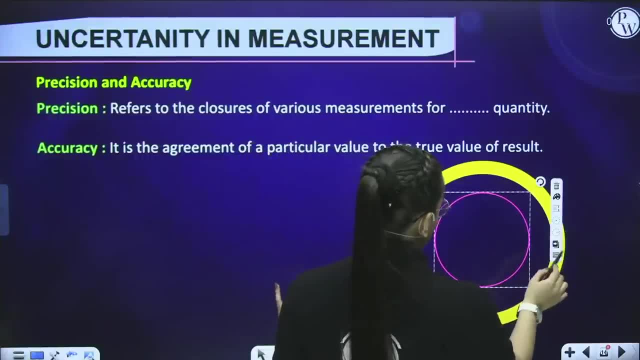 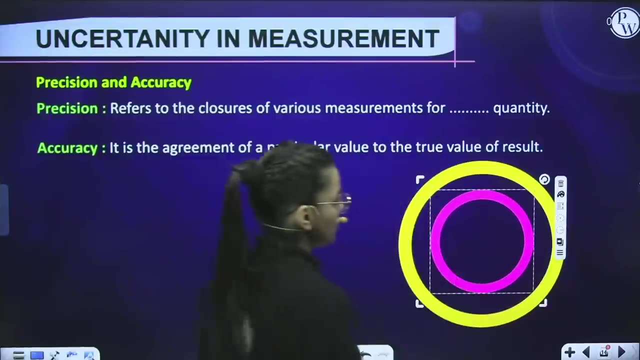 let us make it and let us understand it in a very beautiful manner. students, right, you all have played it. because i have played a lot, i will tell you the rules for this game. now we will learn chemistry with ease in a very beautiful manner, right, okay, okay, now let us make it right. 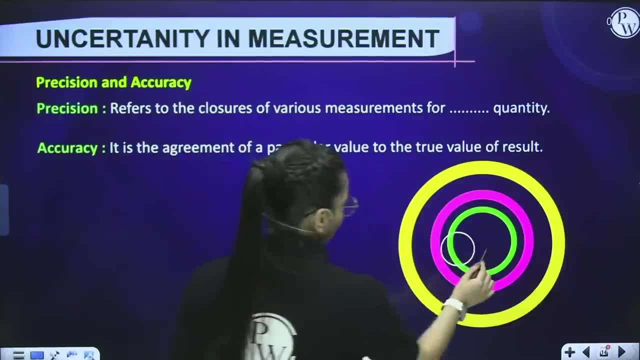 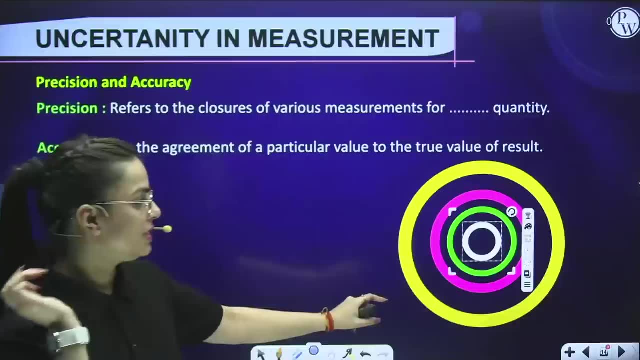 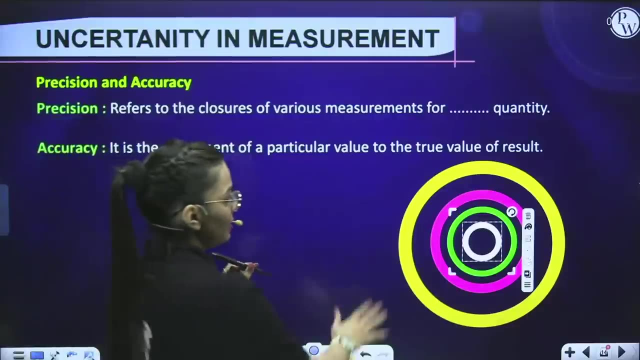 okay, okay. your goal is to put your stick, or the object which you are throwing, into the yellow, into the sorry white portion. you have to do what you have to take a stick which has a magnet in front of it, and this board also has a magnet in it. so what happens is when you throw it in such a situation, 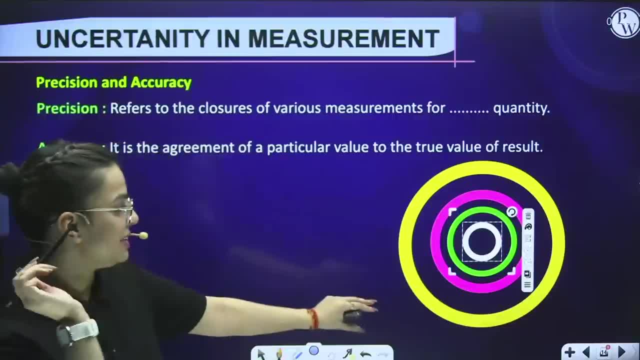 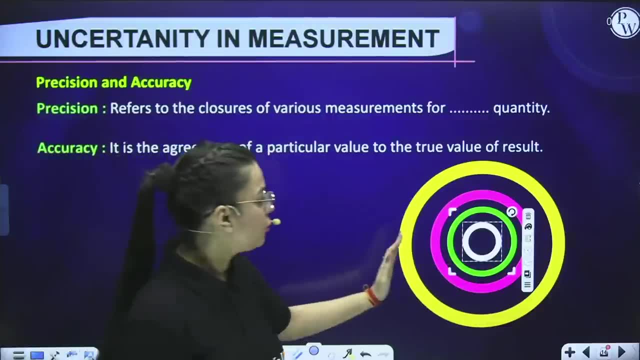 it arises just at the middle and you win the grey game. this is the basic rule of the game. and if it middle and you win the game. this is the basic rule of the game. and if it arises in you know other regions of your game board, then you are not the winner. okay, so what you need to 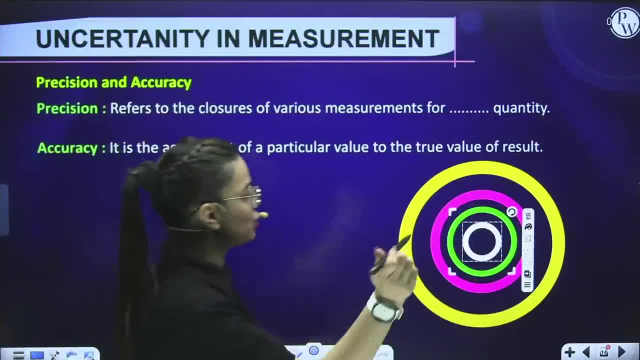 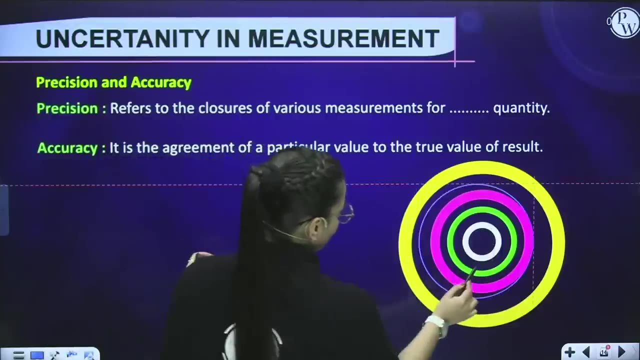 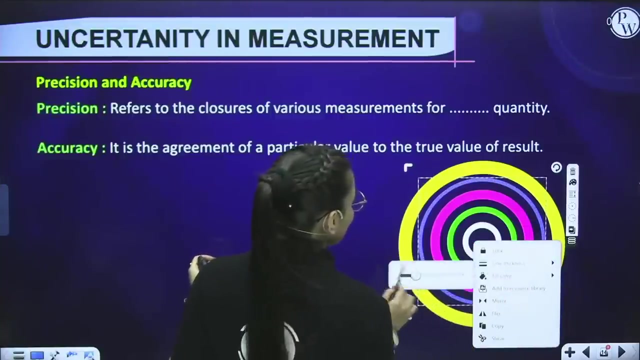 do is you just need to throw your stick from a distance and it should arise like this: tuck, okay, clear. so there, what? how do we calculate this? let me tell you. let us take one more here. okay, won the last one. one. second students: okay, yes, it is almost done. so I have made my game here for you people, so now let us learn it. 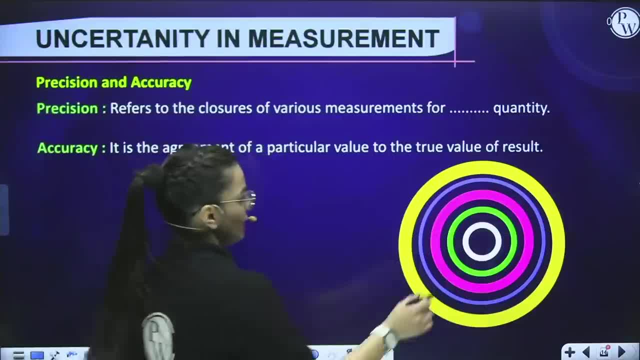 how to play some basic rules here. if you put your stick into the yellow portion, you know you will get 5 marks. okay, if you put your stick into the blue, you will: 08.41.23. totalmenteana, 08.55.04.. GelQs-a. 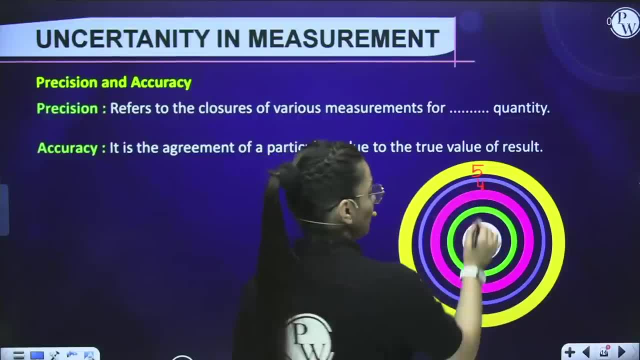 get your four marks. if you put your stick into the pink portion, you will get three marks. if you put into the green one, you will get the two marks, and if you put into the first one, you will get the one marks. so this is the basic thing that you need to know in this. 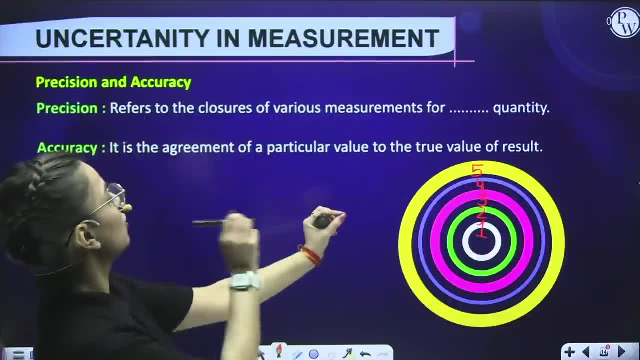 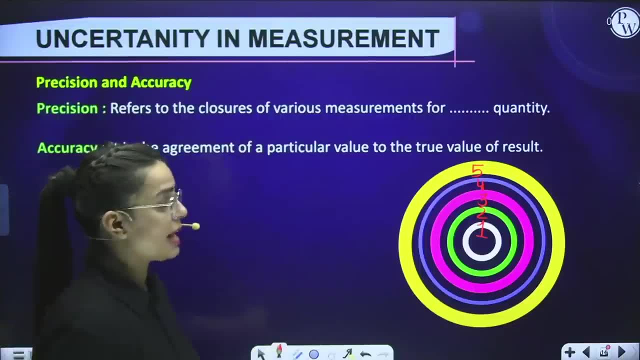 game you have to put your stick like this. you know, do like this and tuck. okay, make an angle from the eye to put into the situation. now there are two students that are playing this game. okay, so one is me and one is you, my students. i would write here: okay, one is. 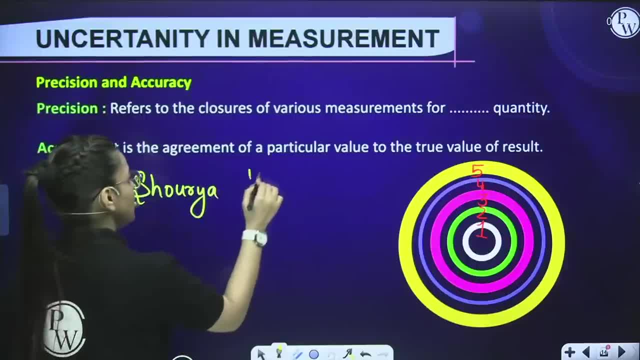 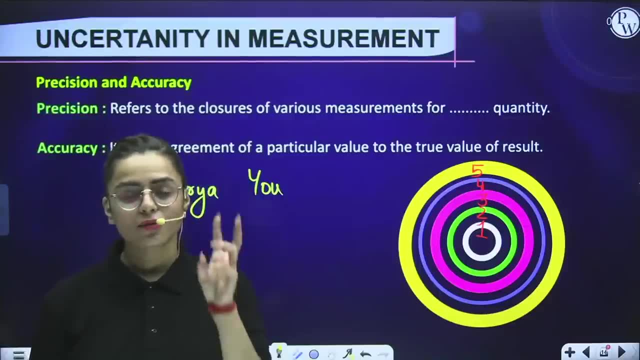 me and one is you. we both are playing this game now, okay, during the class session. so what? we are taking this stick and we will put this. put this stick four times and we will observe who is the winner. so i am writing here: case one, case two, case three, case four. 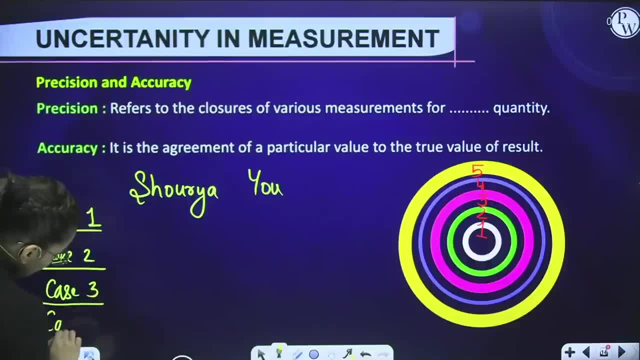 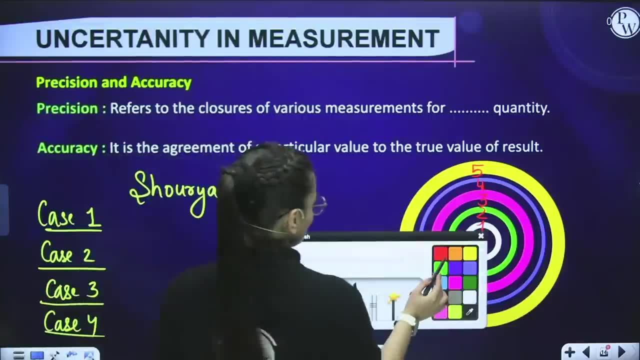 case five. case six. case seven. case eight. case nine. case ten. case eleven. case twelve. case three, case four: okay, students, let us see who wins the situation, right? okay, now in this game, students, you have taken your stick into your hand and you are going to do a blast here. let us see where you are going to put. you have put your stick into number. 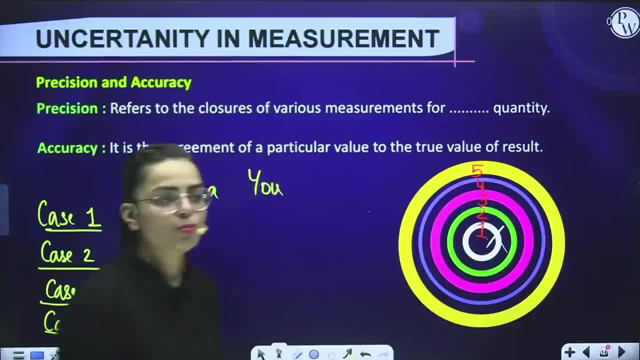 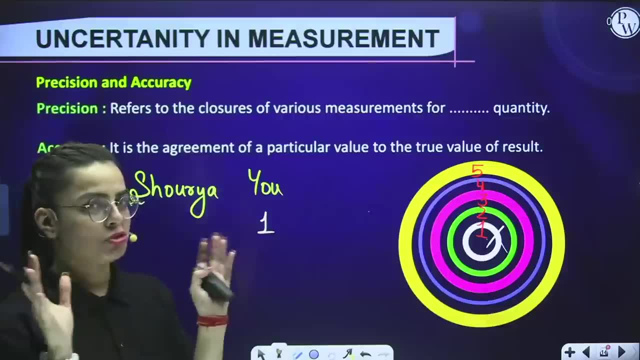 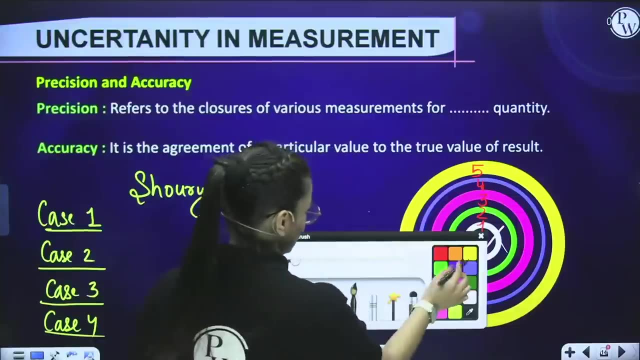 one. you have put your stick into number one. okay, now it's my turn. you know so, as i am doing, i am not so good in this game, so, but i will try my best to defeat you guys, sweet. so i have put my stick and i am putting my stick. my stick is of red color. 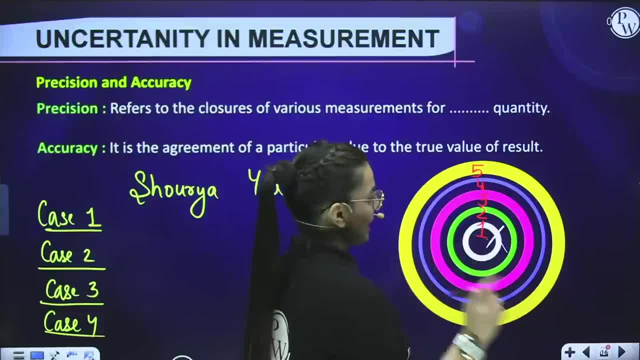 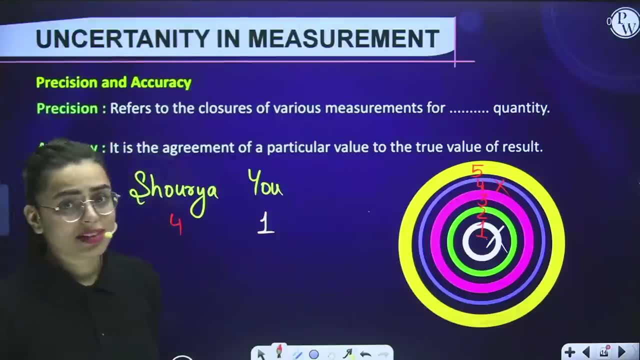 yours is, one is of white color. right, i am putting my stick into the fourth one. okay, my stick is into the fourth one. remember one thing: when your stick arises, the first one, you are the winner. but there are four chances that we are getting and we will observe these. 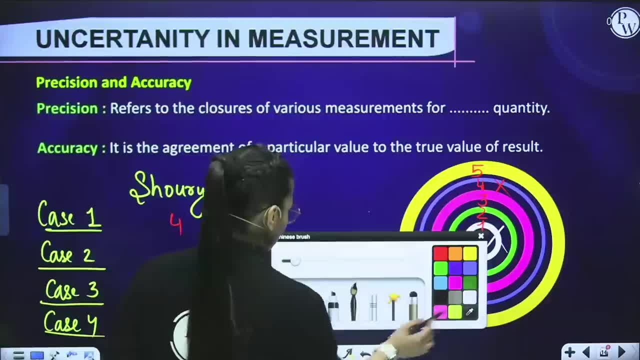 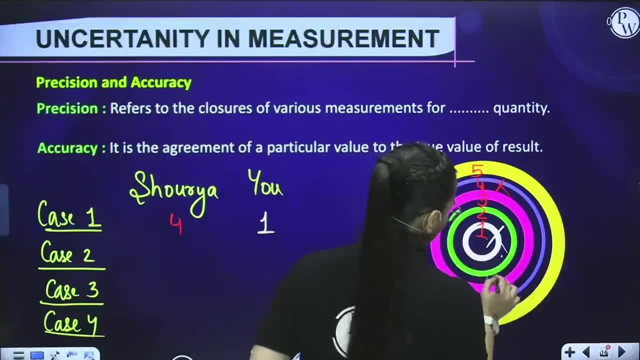 chances right now. the question is: what is the chance that we are getting? and we will observe these chances right now. the case two: again, you have taken your stick and what you are doing, you are again going to put it right. when you are again going to put it, what you have done, it arises into the second. 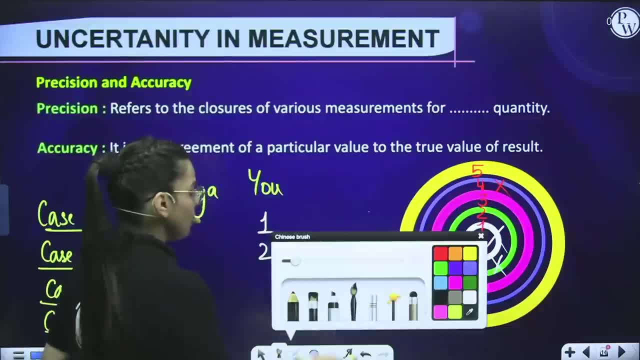 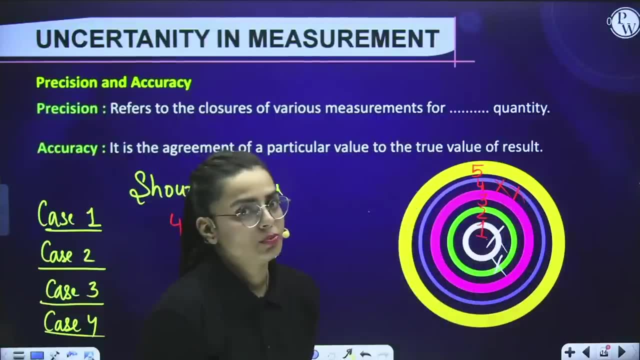 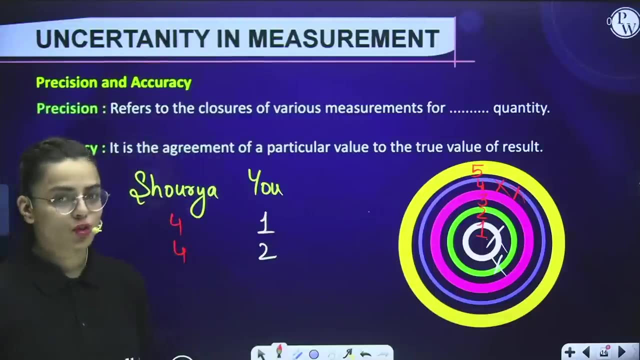 most number, okay, second most number. now, again it is my turn. i am doing this again, again. again i put into four. see, i don't know how to play it because i have not practiced it. it's long time i played in childhood, right. so again i have got fourth number because 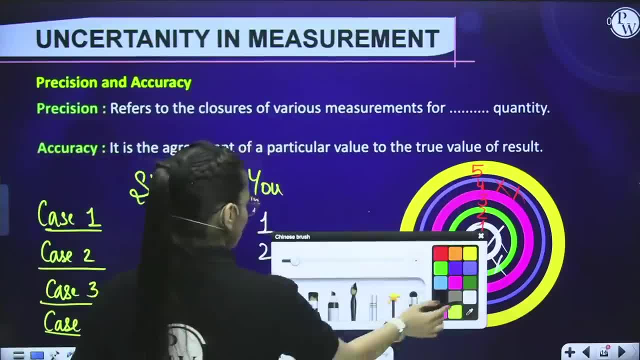 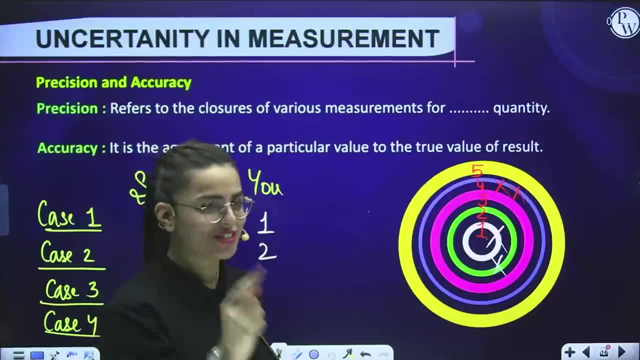 i put my slot into the fourth ring. now it's your turn, students, again, and you are full determined to. you know, win the situation. you are in the victory batch and you have to achieve it. you know that. so what you are going to do, you again put it in the first box, because this is your aim, students. 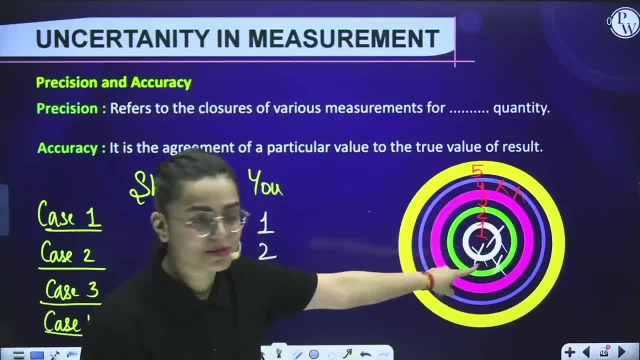 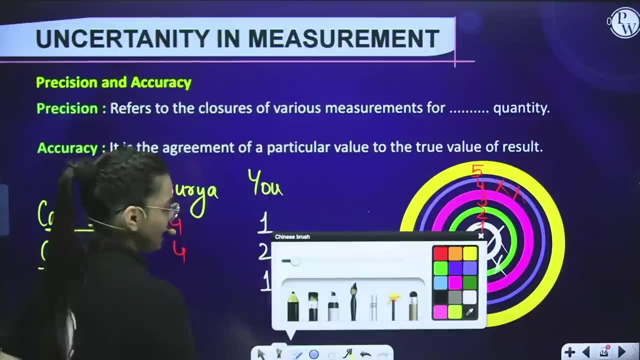 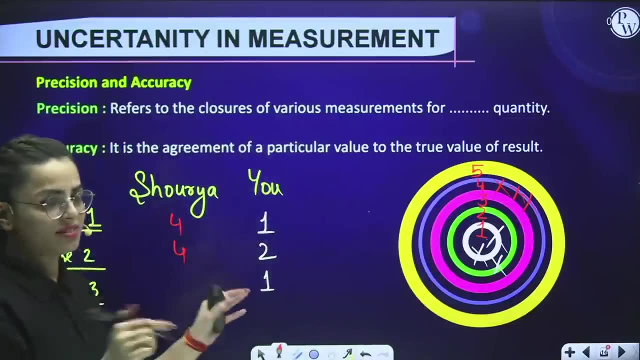 if you are for neat aspirant, je aspirant, board aspirant, you have to put your stick here. you know right. so you have put again the first one. now it's my turn. so what i'm going to do is i am going to put again here because, far at a distance, i have not practiced, i am like throwing. 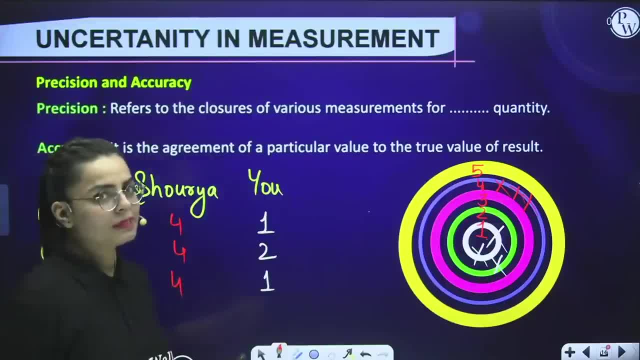 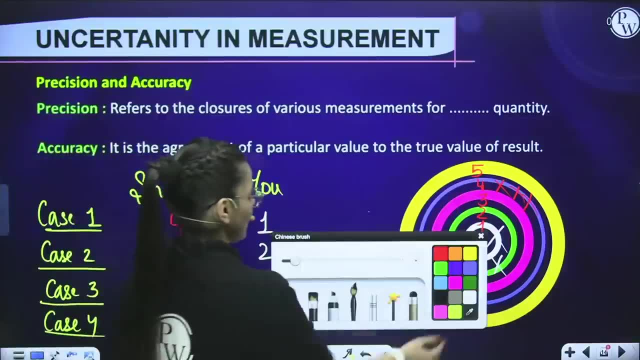 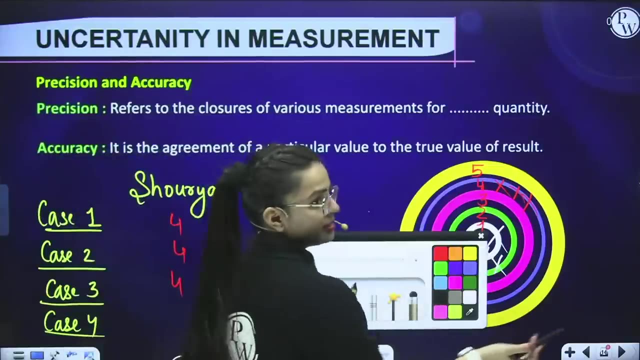 like this, you know. so again four, no problem, my students wins, then i will win automatically. i am the winner. if you are the winner, right, okay, the last case. now again, you have put your stick into the first situation. well, well done students. and again me. i have done here only in the fourth. 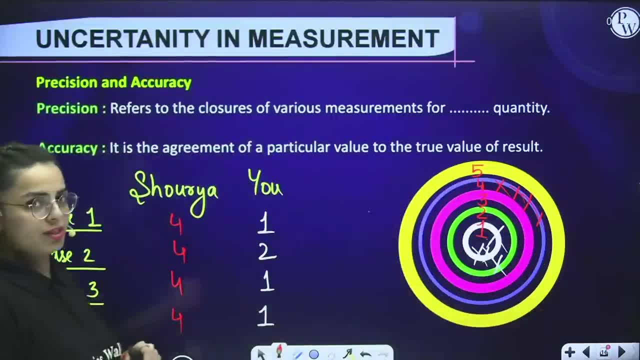 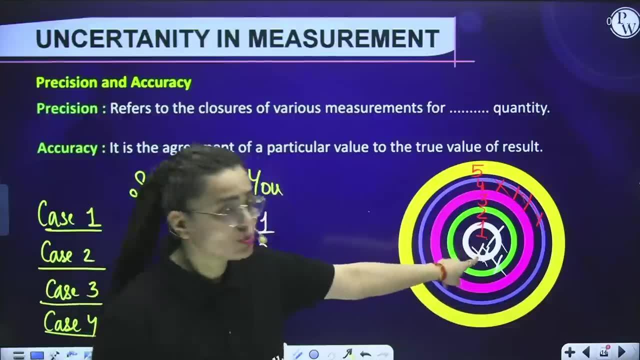 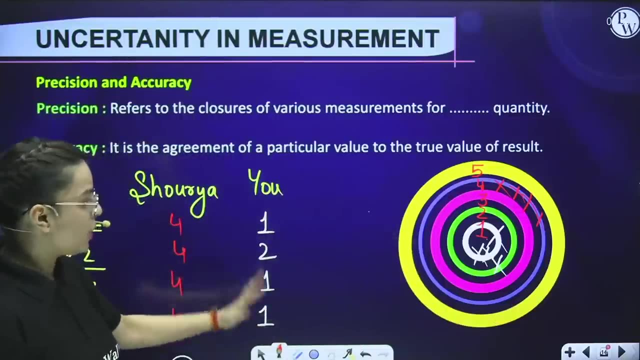 no problem, next time i will try to defeat you, right? so this was our game. now, who is the winner? most? probably, which we can see very clearly- the person who hits the center most position is the winner, and you guys are the winner. you have hit your target very easily. so one, one, one, one you have seen, but in the second case you got two. 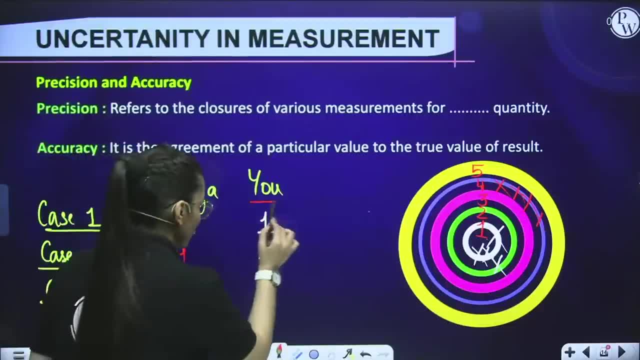 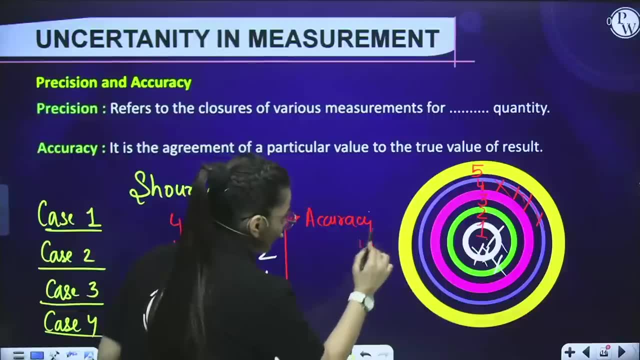 so what we have seen, this situation. this situation is known as accuracy, accuracy coming towards chemistry. students come back, come back from the game. your score is one, two, one, one. that means you have to hit one and you have hit one thrice, but once it was twice. 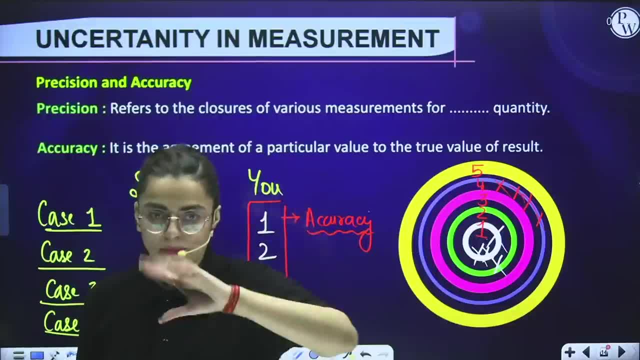 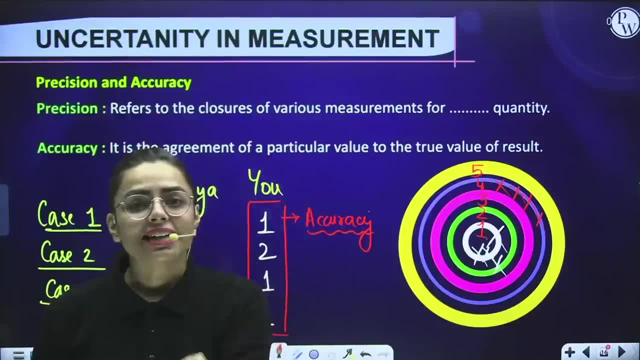 you are near to the answer. near to the answer, close to the answer, and when someone is close to the answer, it is known as accuracy. now coming towards me, who secured four, four, four, four during this hit. now i have been doing four. i was not good at the point to target it, but see what i have done. 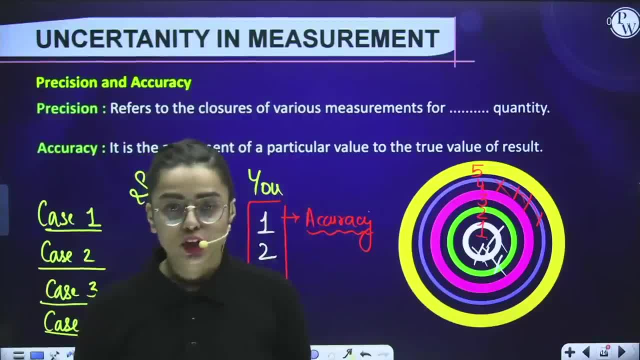 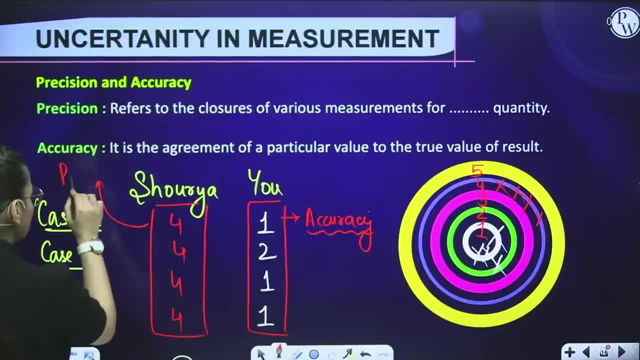 it was my consistency that i maintained it: four four, four, four four. so this situation, this situation is known as precise. this situation is precision. now, what is the situation when there is a consistency for the same quantity, like for same quantity refers to as four four, four, four four. so there, 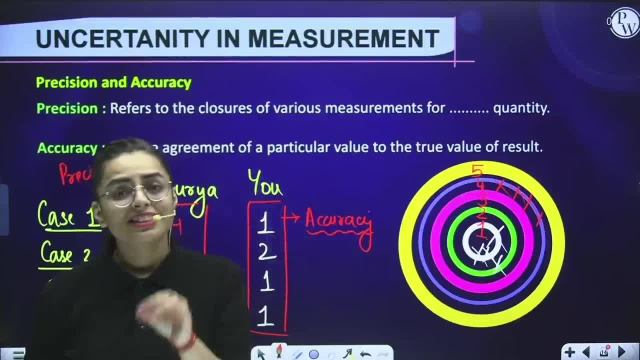 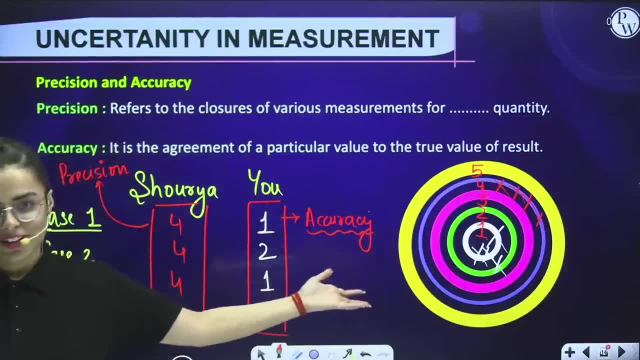 is a consistency, that is referred to as precision, and when there is a closeness towards your time target, that refers to as accuracy. hopefully, you love this game a lot, right? so let us first read these definitions to make it more clearly understandable. first of all, precision, i would 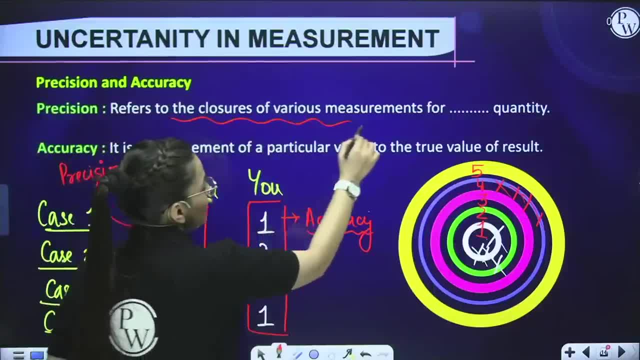 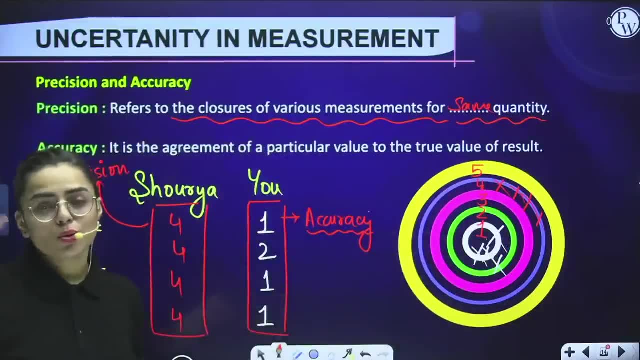 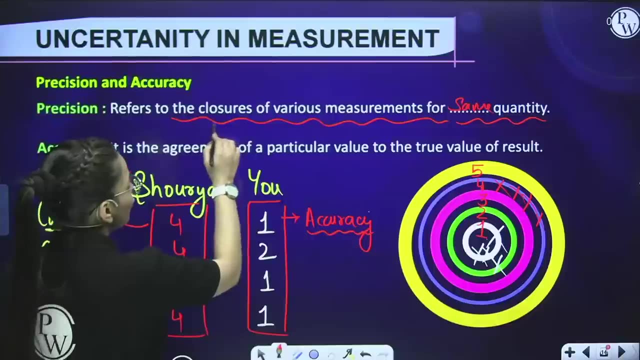 talk about refers to the closures of various measurements for same quantity. now you will say that, ma'am, for closures or for you know, close, you have told the word accuracy when it is near to the answer, but you are using the word here closure. here closure refers for the same quantity. four, four: 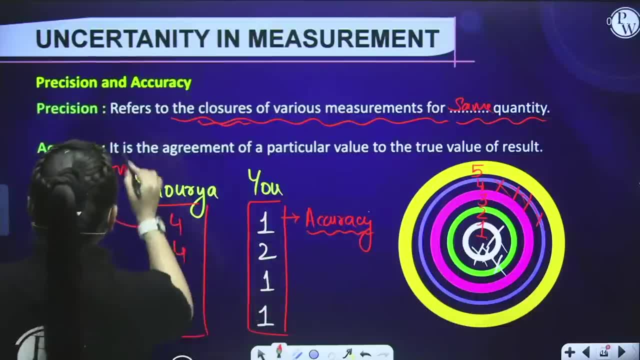 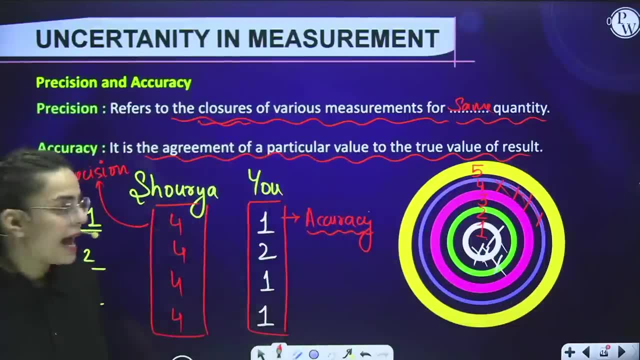 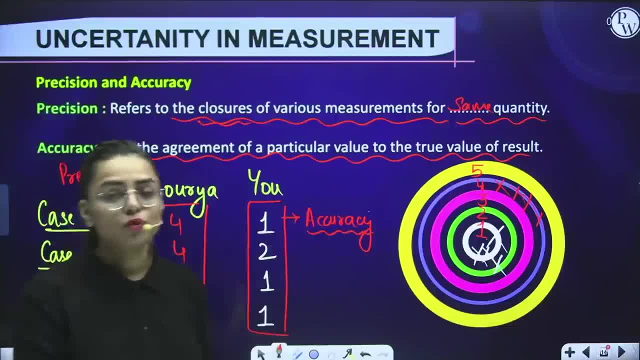 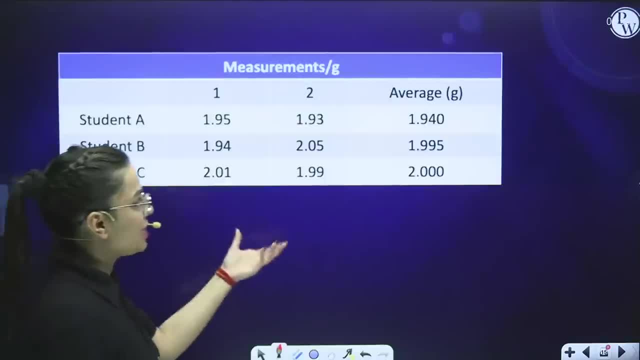 the true value. so that is accuracy clear. now let us move towards a wonderful example of ncrt. there are three students- students a, b and c- and they have been doing a match in that they got some measurements and they participated twice. so they got measurement one and measurement two. 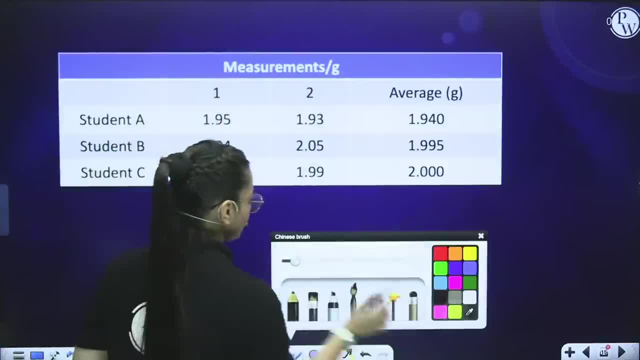 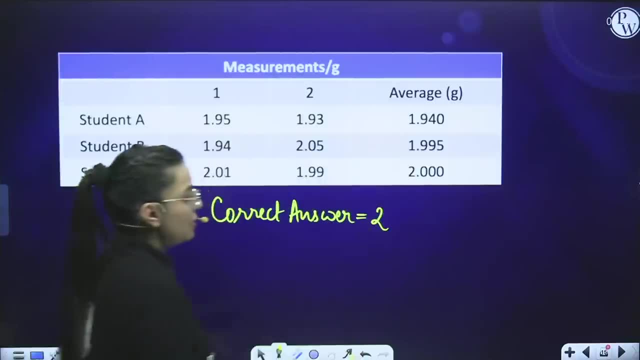 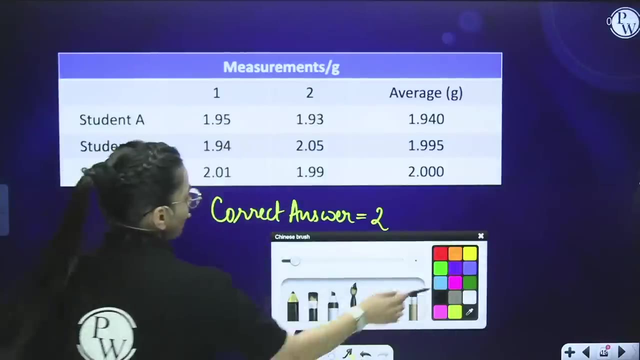 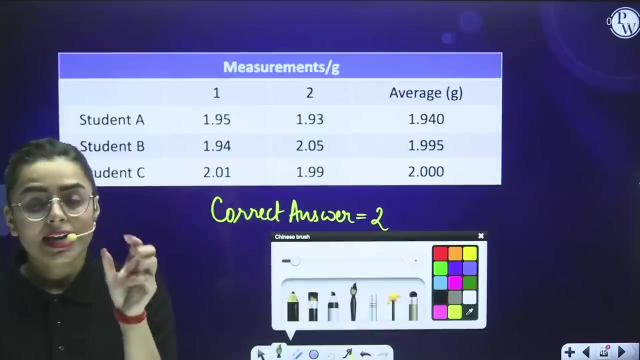 and the correct answer: students. the correct answer was two. right now, let us check here which is accurate and which is precise, right so the student first a. let us talk about student a. if i talk about student, a, students, the first time measurement was 1.95. the next time measurement was 1.93. now both the situations you know are 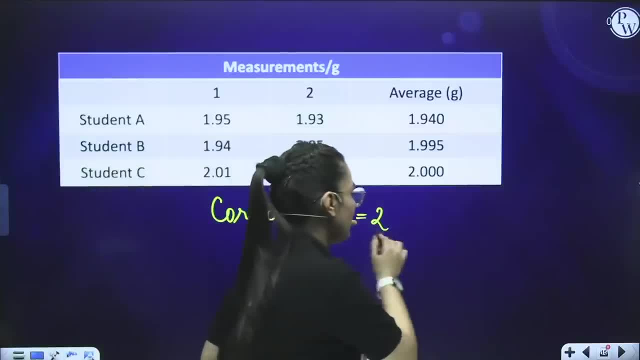 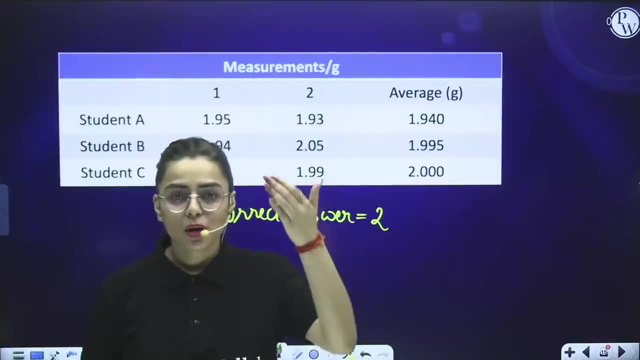 close by, but they are not close to the number. they are not close to the target too. hence they are consistent because the number is almost equal. you can say that, ma'am, you have got four four, four, four, four, but they are not 1.93. nine three, nine three, no, but at least they are close to the same quantity. closure to the same. 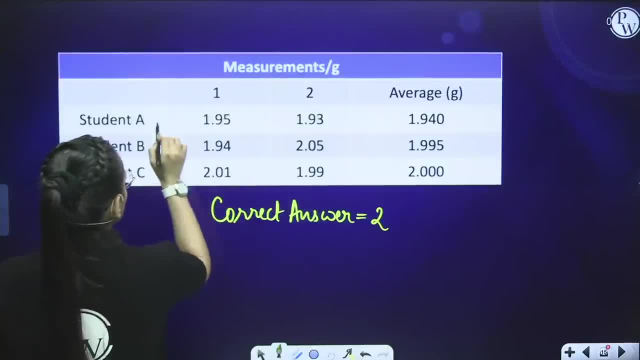 quantity. that means they are precise, they are consistent. so this situation is precise. are they accurate? when will be the accurate? they will be accurate when they are close to the target, but target is two, hence they are not accurate. so accuracy is absent in this case. right? if i talk about the second situation of the student b, there are two uh measurements again. 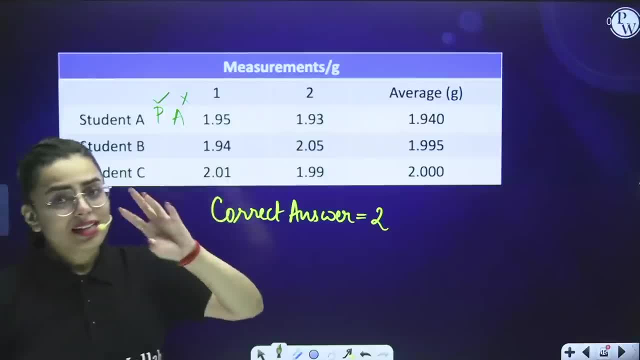 the first measurement is 1.94 and 2.05. now, students, please observe. firstly about accuracy. accuracy is the one when we are close to the target. the target is 2. is 9.1.94 and 2.05 close to 2? no, what is close to 2 close to is like uh to 2 is something like 1.99, 2.01. these are close to. 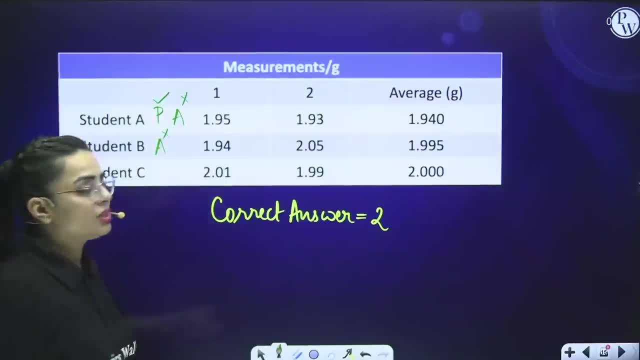 2, hence they are not accurate. so now let us talk about, uh, precision. are they precise? no, because there is no consistency. this comes under the category of one something, this comes under the category of two something, so here they are not precise at all. now, uh, if we talk about students, 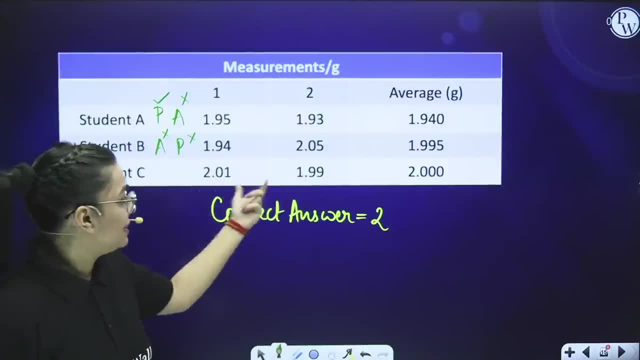 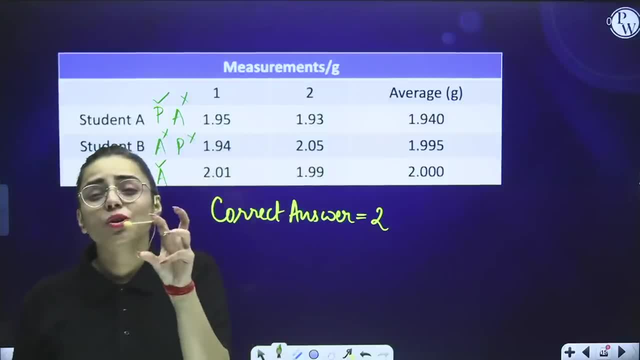 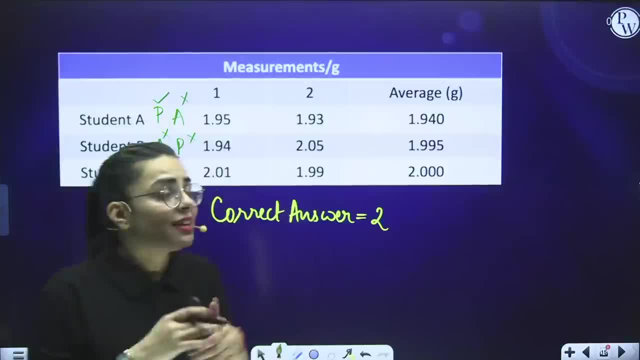 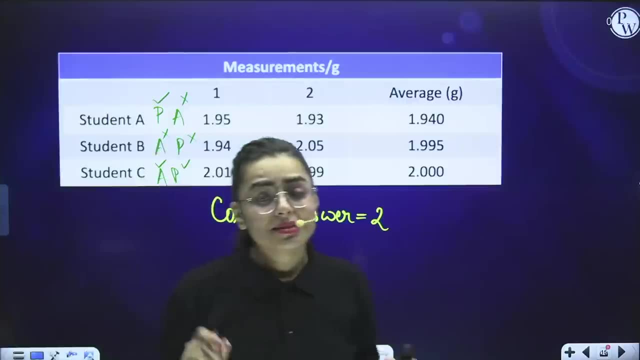 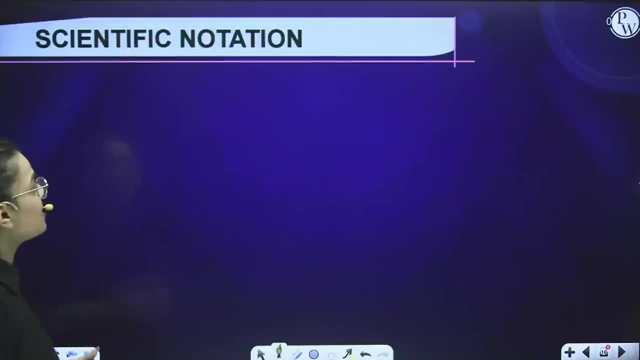 almost nearby, very nearby, and that means they have consistency, hence they are precise. so we have learnt about accuracy and precision. this is very, most important, which you need to understand and which you need to keep in your minds. okay, so now moving towards the next, that is, scientific. 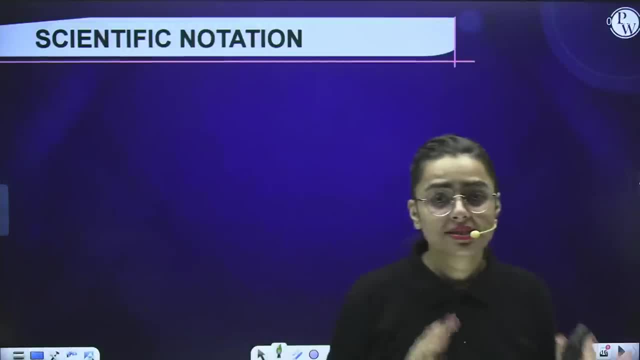 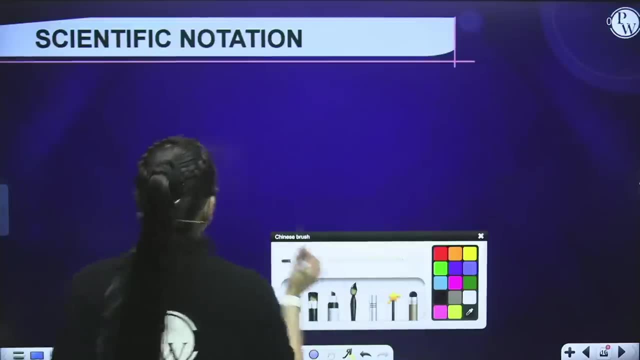 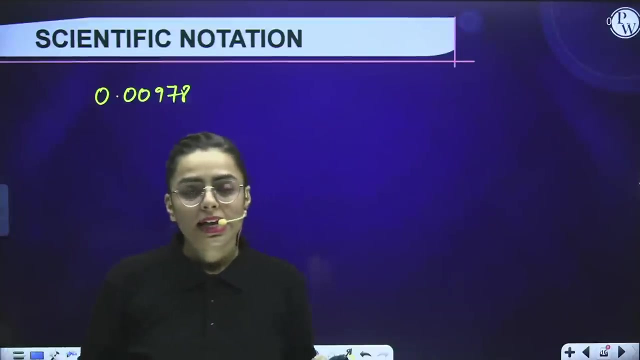 notations, students. scientific notations are the one that means when we represent a number in the form of 10, raised to the power something. for example, you have been given any number like 0.00978, you are given this number and i am saying that please represent this number in forms of 10. 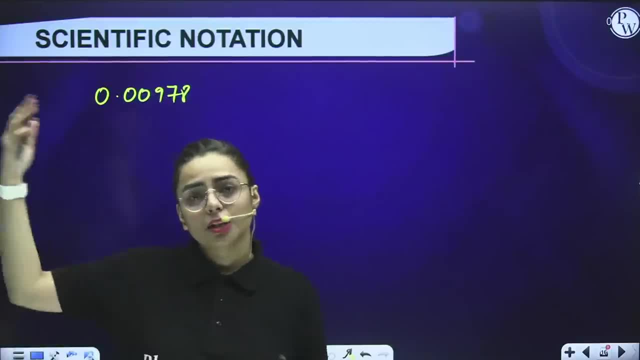 raised to the power, something. when i represent this number in terms of 10 raised to power, something, it is referred to as scientific notations, how, in 10 raise to power, n n can be 1, 2, 3, 4, 5, 6, 7. 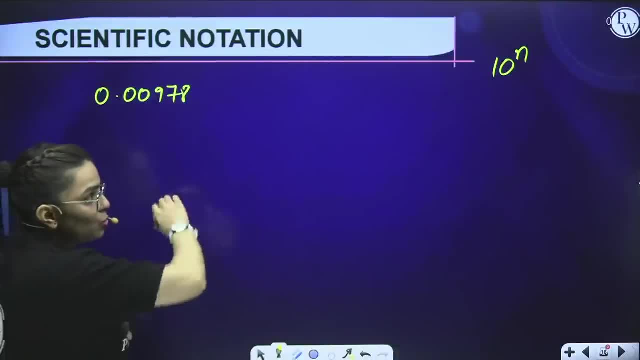 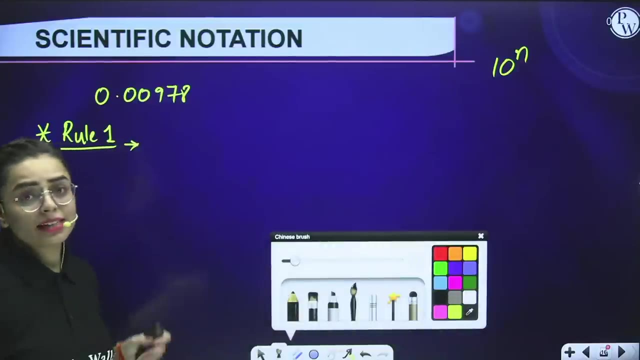 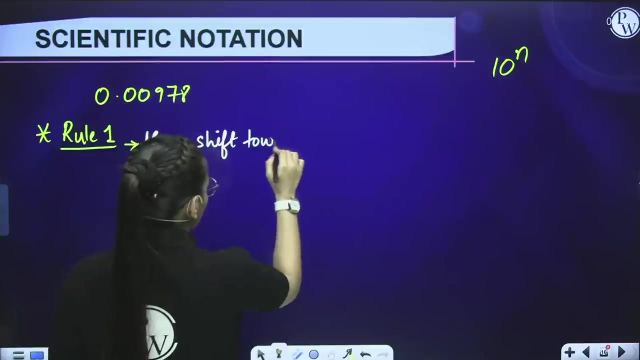 it like this right. so see how to do this, how to convert it into such situations. there are certain rules which we need to understand. the very first rule, rule number one. rule number one states that if we shift, if we shift towards the right, from the decimal towards. 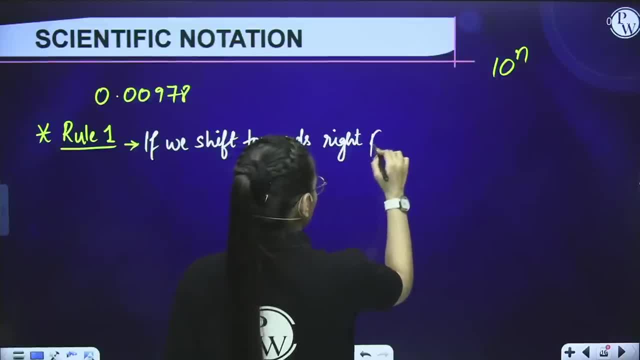 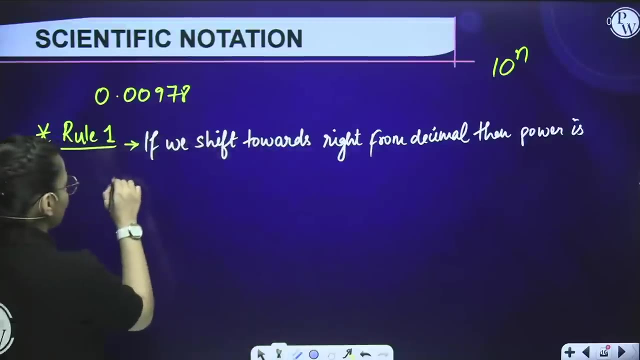 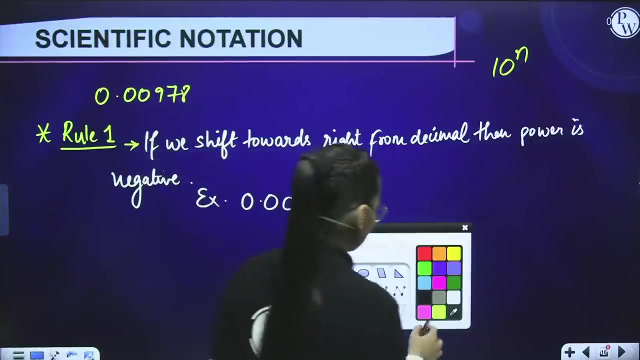 right from decimal then then, students, power is negative. power is negative example. please let us see example: is zero point zero, zero, nine, seven, eight? you need to understand the two basic terms which i already you know. i want you to know so that it becomes easy for you. 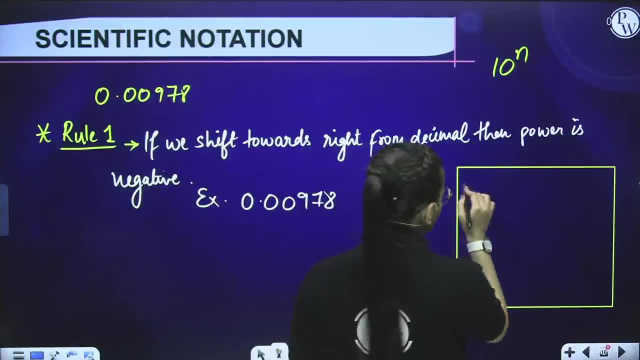 to understand the rules. if your goal is to convert it into something- okay, i am making a box here in this- you need to write non zero digits. what are non zero digits, students? non-zero digits are the one that is one: 2, 3, 4, 5, 6, 7, 8, 9. okay, which? 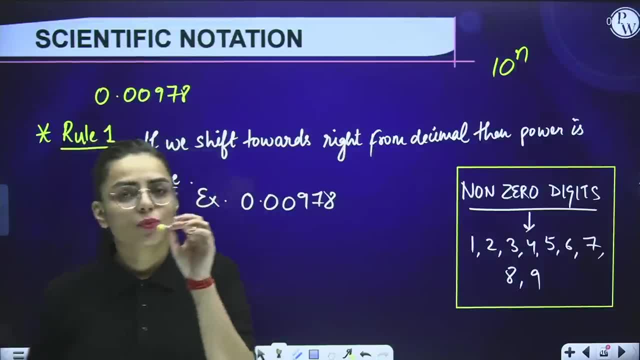 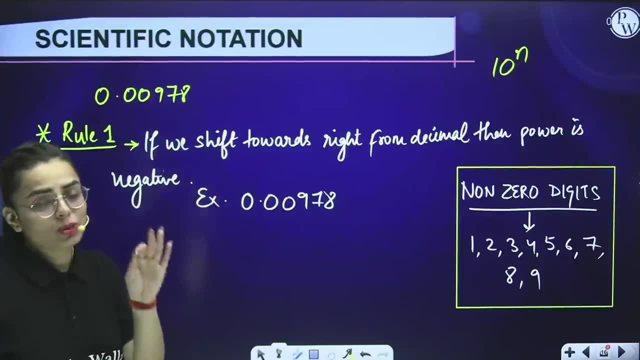 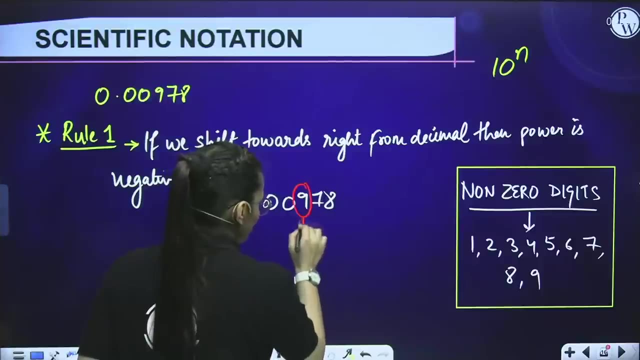 are other than zero, they are referred as non-zero digits. now you need to, for to accomplish the rule 1 told you, first find out that whenever we shift towards the right from the decimal, then we need to find the first non-zero digit. here this 9 is a non-zero digit, 0 is a zero digit. 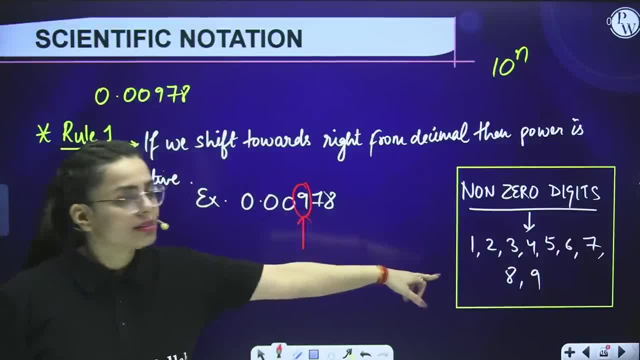 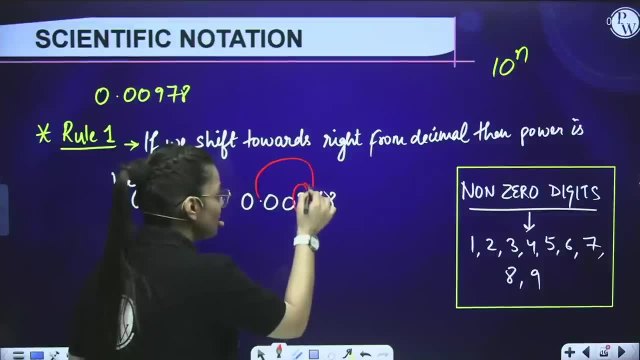 0 is a zero digit. 0 is a zero digit, but 9 lies under the category of non-zero digit. so when you find the first non-zero digit, what you need to do is you need to move this decimal after this. you have to do this to make it bring under the category of scientific. 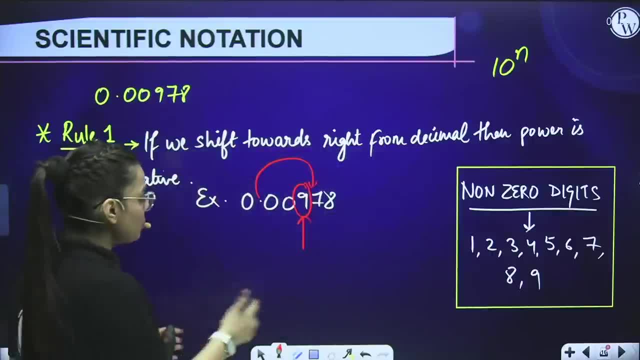 notation that is 10 raised to the power, something. so what you are going to do is you are moving in such a situation like one decimal place, two decimal place, three decimal place and after this you want to get na. so what you will do here, you will do here that after 9. 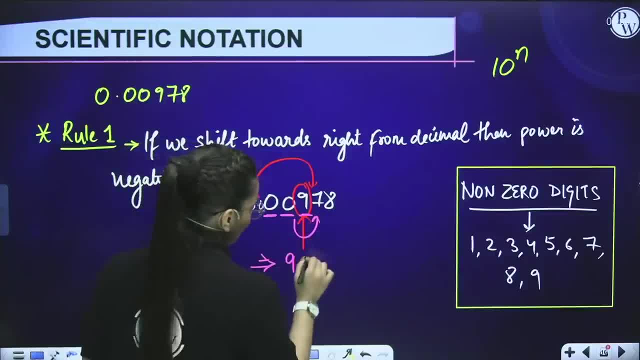 you want point decimal, you will put decimal what comes next, 7 it now. you will write into 10, raised to the power, what you are moving in which direction? towards right, in direction from the decimal, then you have to write the power in negative form and if the power is, 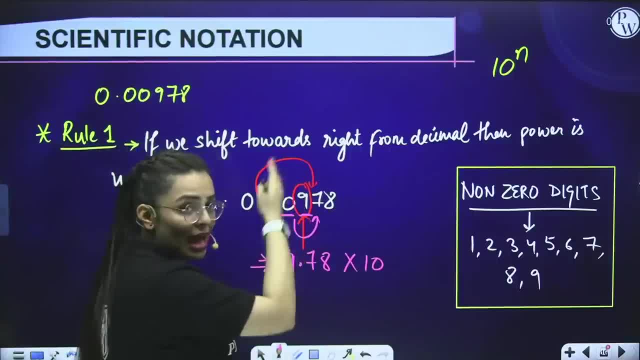 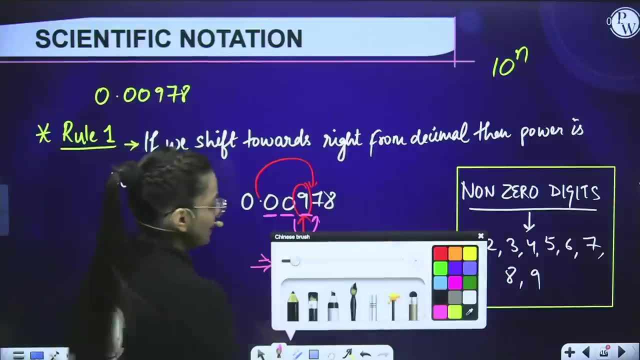 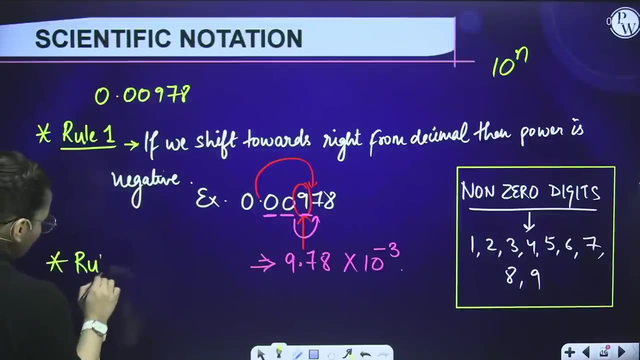 in negative form, then how can you count 1, 2, 3? after third position, decimal is coming, power is in negative form, so 10 raised to the power minus 3, clear. so now comes the next rule: students. that is our rule number 2. ok, if i talk about students, the rule number 2. 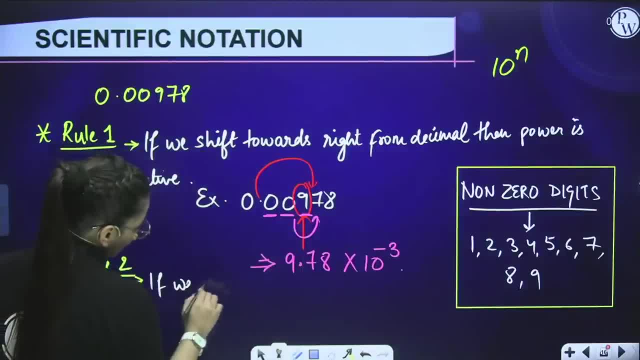 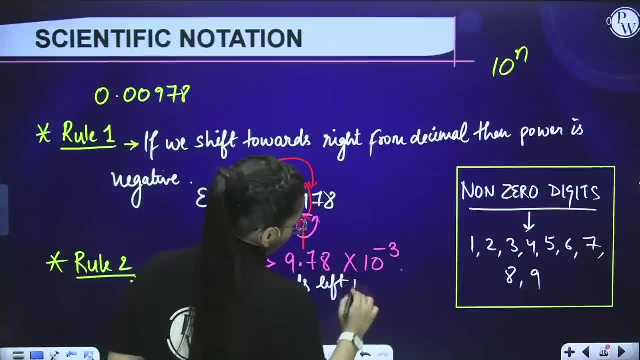 i would say that if we shift, if we shift towards left position, then we are going to have a negative form. then how can you count 1, 2, 3? after third position, decimal is coming. power is in negative form. the same way, 12 raised to the power of using front position from decimal, from decimal. 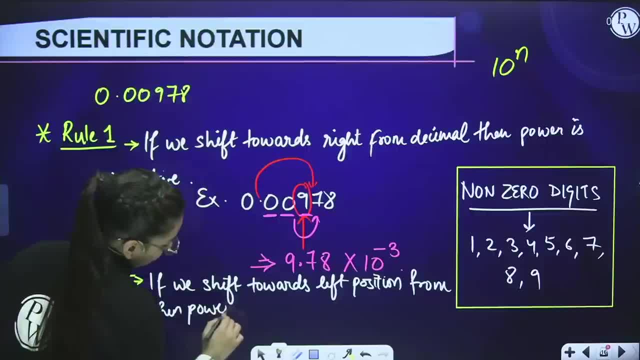 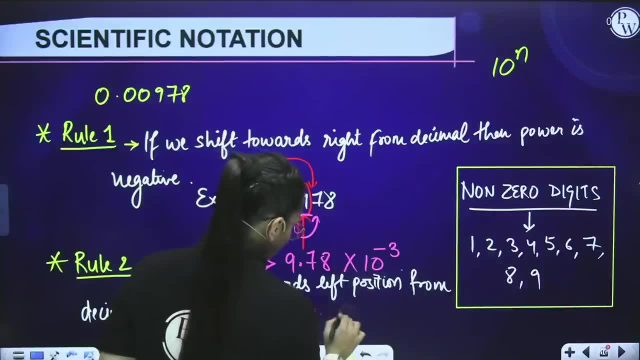 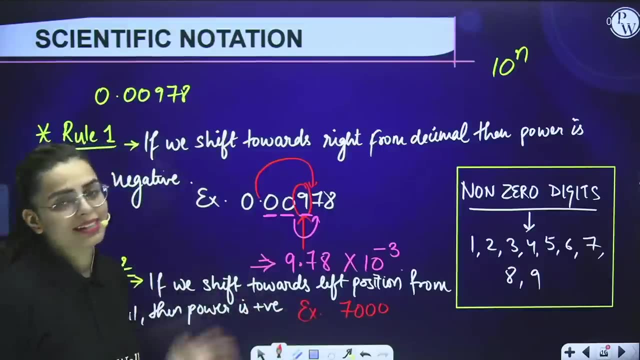 then power is positive example. ok, i am taking one more example. it is 7000. okay, now any decimal present. no decimal present, that means we have to move in from the voracious, like this one left position. we will move from the towards the left position. when there is decimal, then you have. 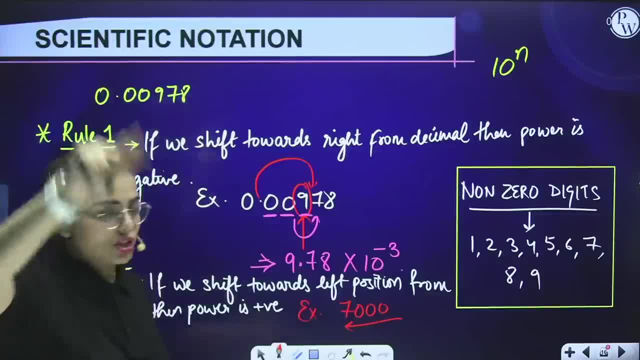 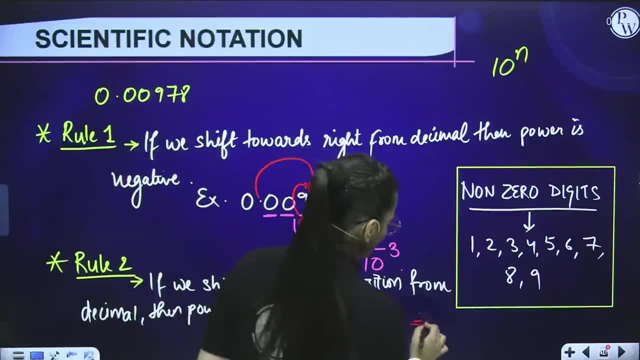 to move into the right position from the first non-zero digit. what is the first non-zero digit here? 7. so we need to put decimal after the first non-zero digit. hence, after 7 we have to put, so we have to put. we will move in this direction. to put it: after 7, how many zeros i have to cross? 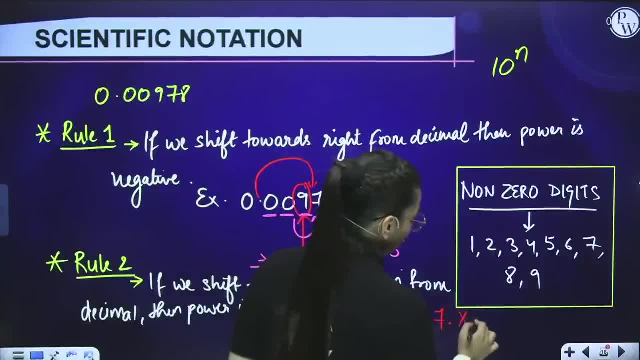 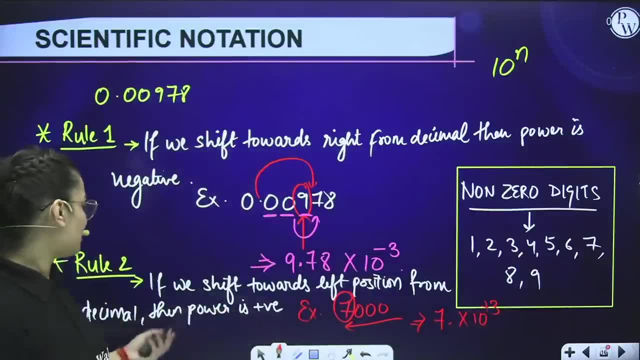 1, 2, 3, that means 7 into 10. raised to the power. what? 3? it should be positive because we are moving. in which direction? we are moving students in our left direction. so this was all about scientific notations and in ncrt also you will observe some basic things, for example, addition, subtraction. 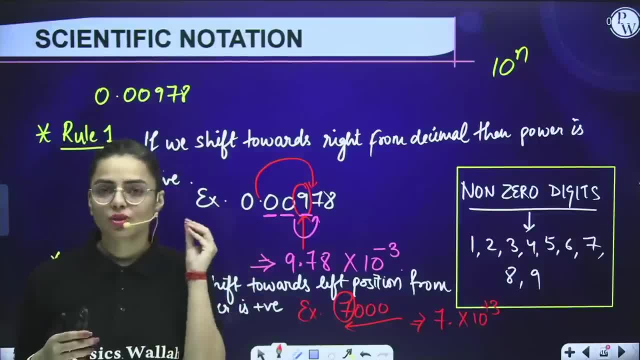 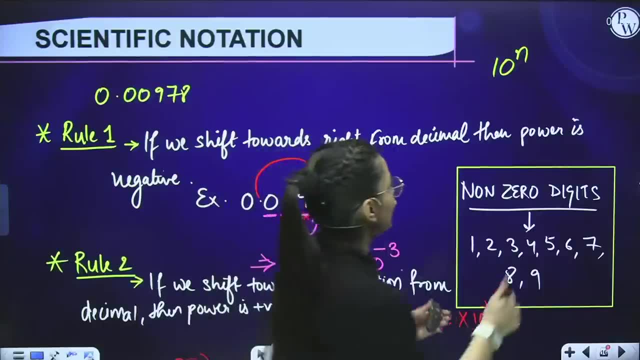 multiplication and division. the very first thing that you need to remember in all those cases is that the basic rule: when you are given some numbers to add- for example 2.1- i am taking here 2.1 plus 4.22- what you will do this: you will add both of this number when you are going to add. 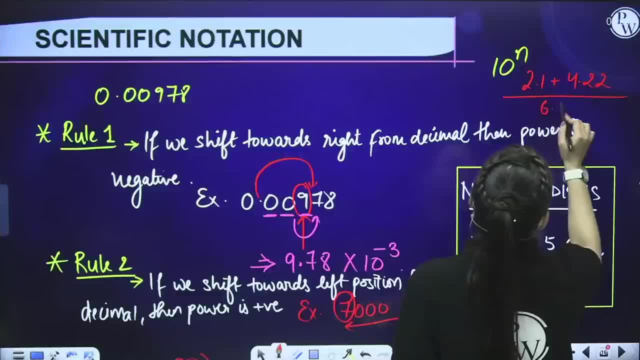 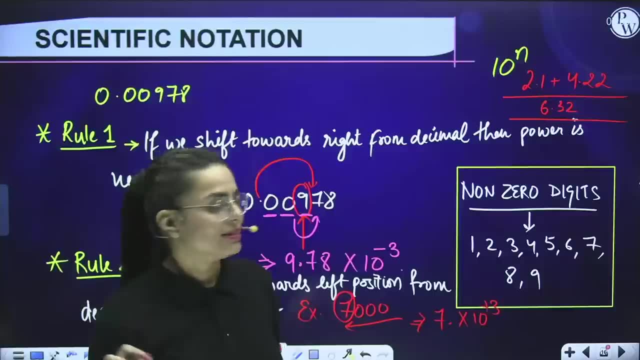 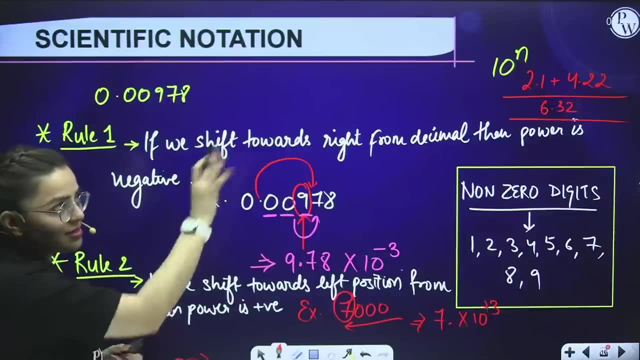 these numbers, numbers now, students, you will get. the answer is 6.32, right, you are getting this answer. this answer is incorrect. why this is incorrect? because you need to find out here what you need to find out here: that during the, you know, during this question, it is the simplest, but when you get into the terms, 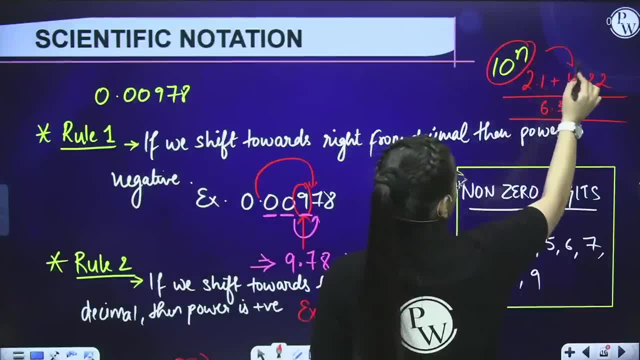 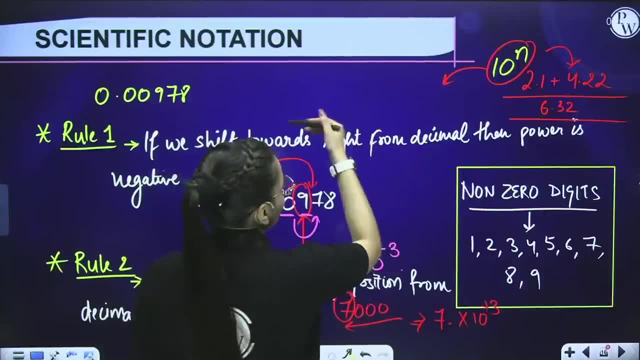 of scientific notations. this is the simplest case when you can directly add. but, for example, these decimals are not given. you are given something in 10 raised to the power, something in scientific notation. what you will do, for example, if i say 5.7 into 10 raised to the power? 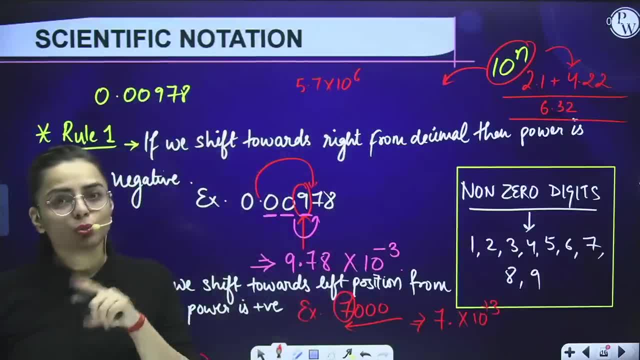 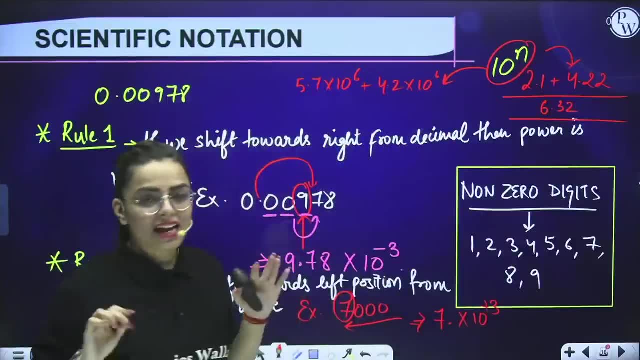 6. okay, you need to add it into 4.2, into 10 raised to the power 6. what you will do? what you will do, students, when you are going to add both of these situations, you can directly add them, but when you are given a situation to multiply, what you are going to do in multiply case it is a quite different. 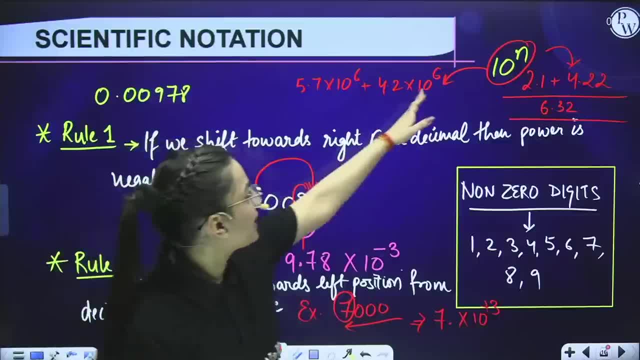 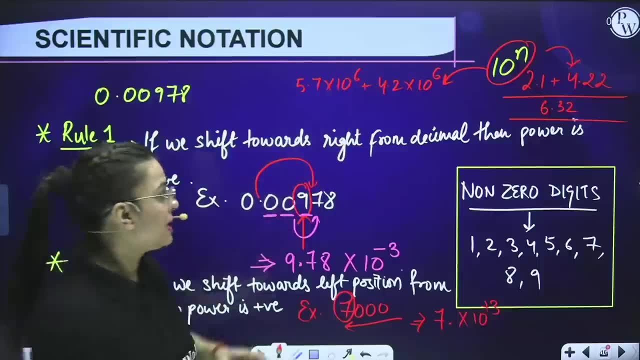 situation. In addition, subtraction it is directly. you are taking 10 raised to the power, 6 common, and then you will go to add them. this is the basic way of addition and subtraction which we do in mathematics. but if i, if i put a symbol of multiplication here, what you will do in 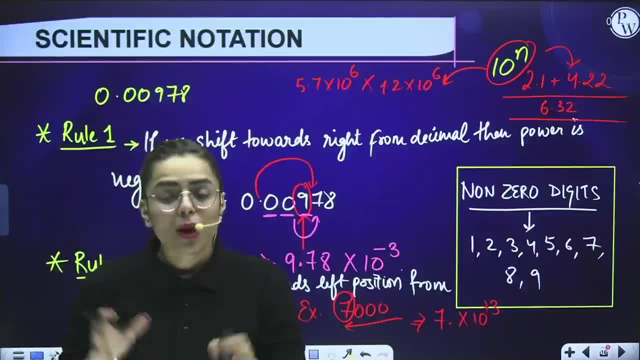 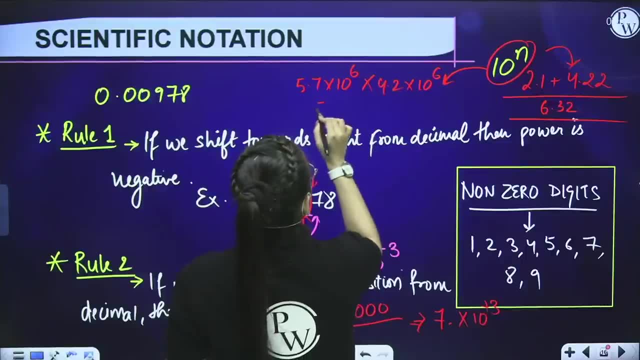 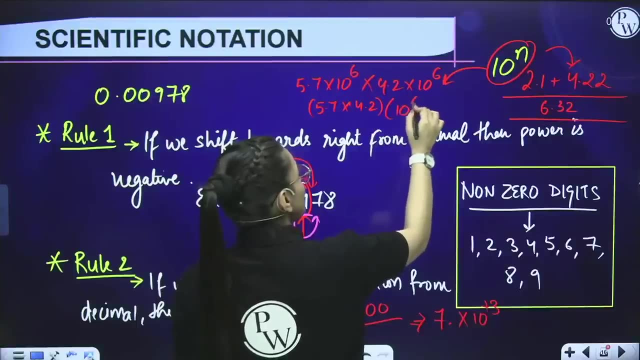 multiplication students, the powers are being added, while in division the powers are being subtracted. so when the powers are being added here, what is going to happen here? 5.7 into 4.2, as i told, powers are going to add, so 10 raised to the power 6 plus 10 raised to the power 6 can be. 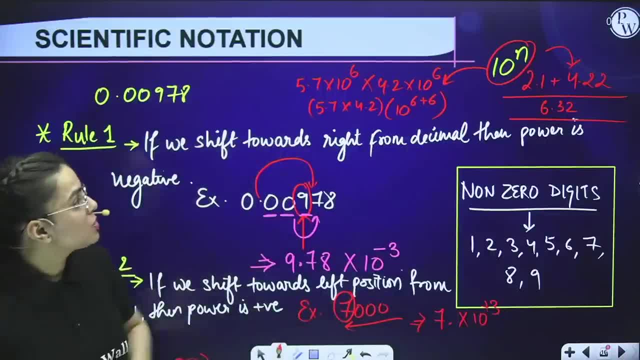 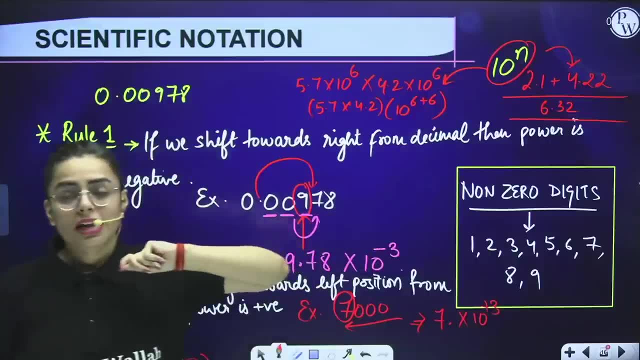 written as 10 raised to the power: 6 plus 6. clear, because powers are already being added. you can multiply this and the answer will be something into 10 raised to the power: 12. but in the case of division, for example, i give you the same situation in the division case. how can you do so? 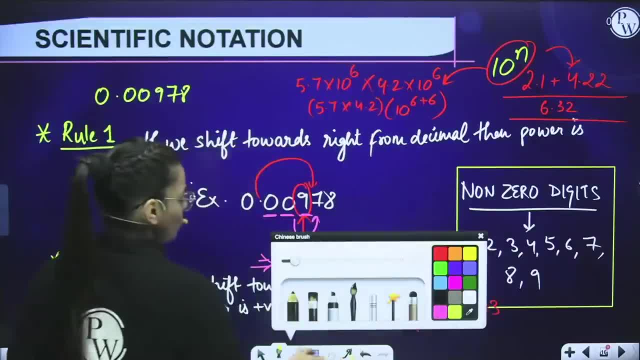 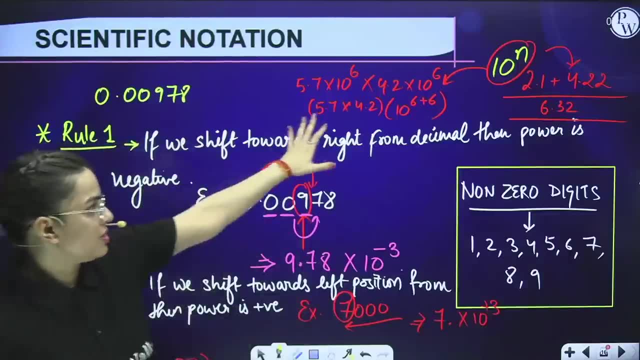 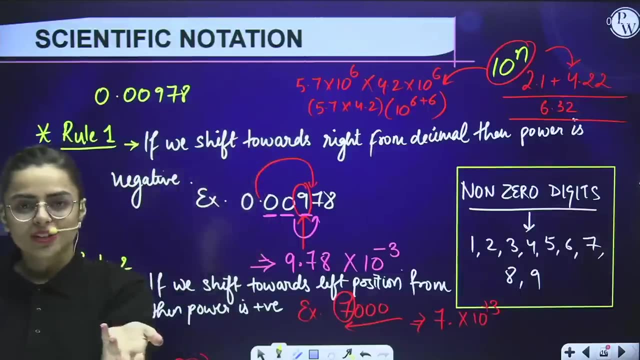 please see that also. it's very simple. you will get these all in mathematics also, but still i'm telling you so that you don't get confused. There are very less chances of the questions in these kinds of stuff. just, you need to know about these two rules, since i'm going to tell you so that it is more clear to you right? so one more. 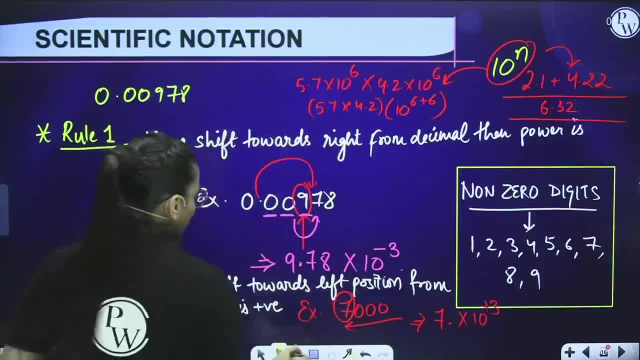 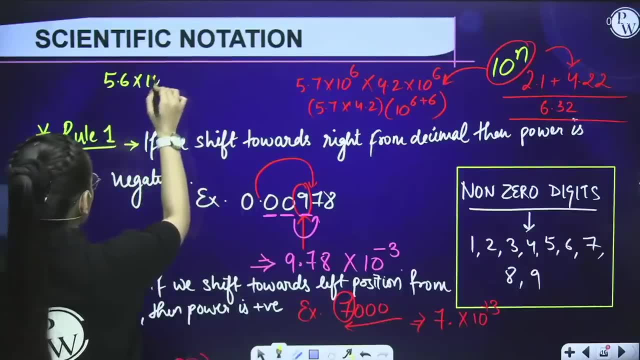 case, if i take i, if i say it is like i'm taking 5.6 into 10 raised to power 6 divided by 4.2, into 10 raised to the power 4.. So what we will do in the case of divide. 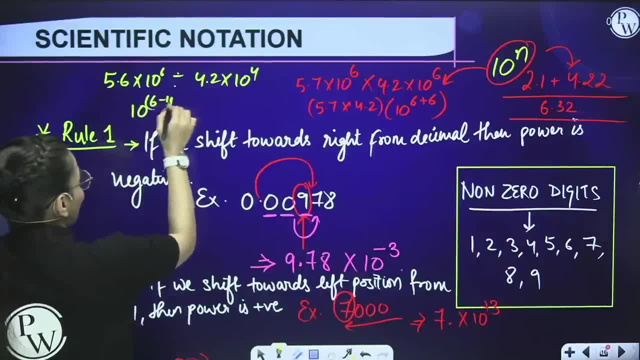 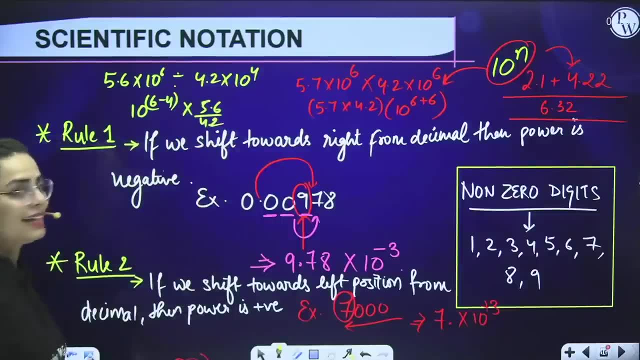 i divide. the powers are being subtracted like this: and then we are going to write 5.6 divided by 4.2, like the students. so here powers are being subtracted, here powers are being added. clear, it is very simple, students. now students, let us see the very next topic which we are. 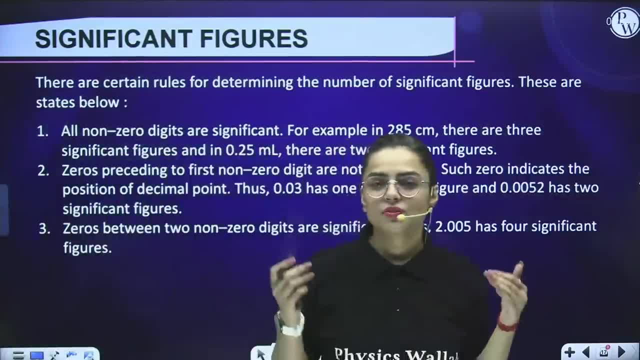 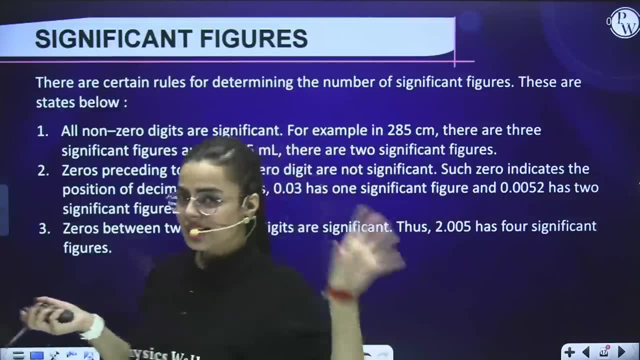 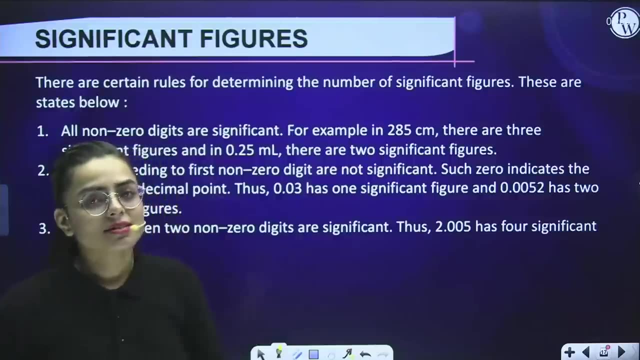 going to study is significant figures. significant figures is a very interesting topic and you will find it very easy. you know there are some students who feel math is a very easy thing. mathematics is tough, but let me tell you this mathematics topic- significant figures in chemistry- is very, very easy and interesting. there are certain rules for significant figures and 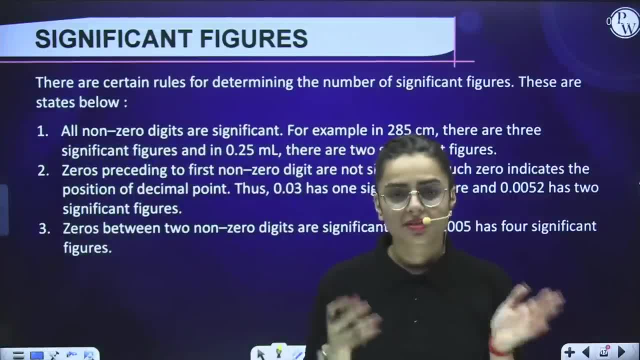 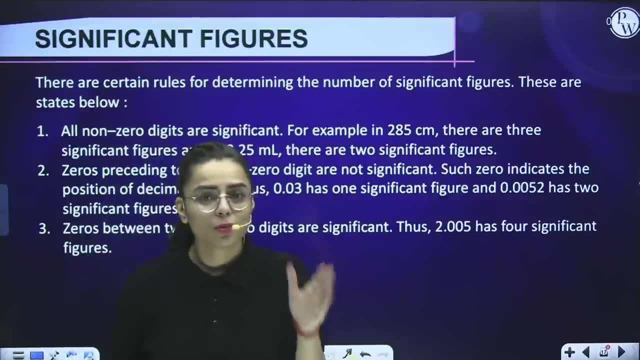 these rules will help you to find out the value of significant figures in certain questions. so there are some rules. the very first rule is that all non-zero digits. what are the non-zero digits? from first towards the ninth? one zero is not included in that right, so all non-zero. 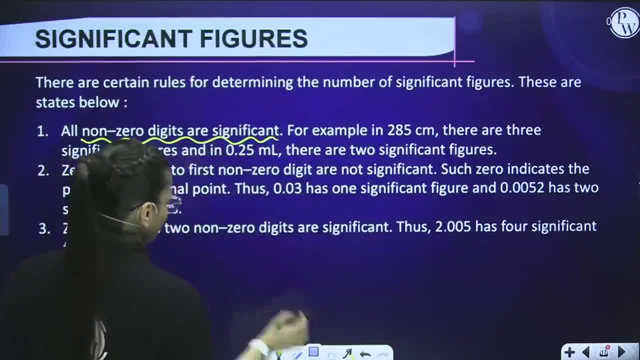 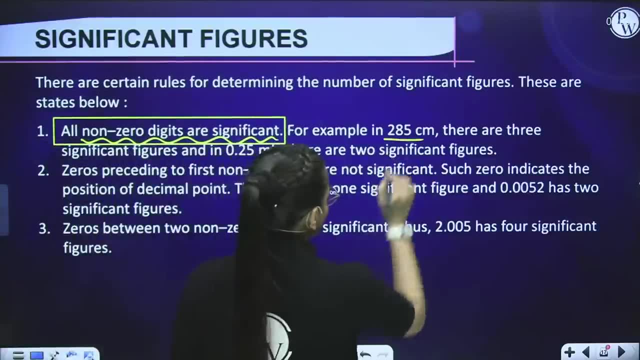 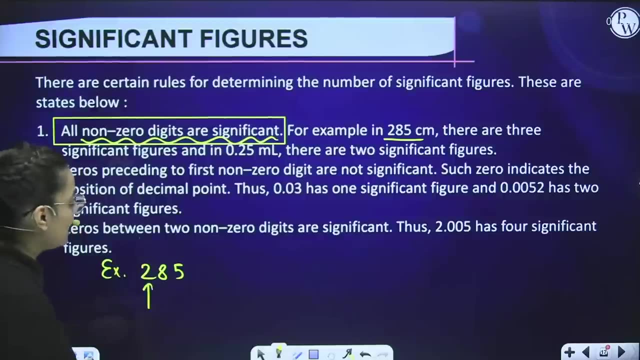 digits are significant. now let us take an example before example. please underline this. okay, it is very important rule. take an example: 285 centimeter. please let me tell you. is 2 a non-zero digit? yes, ma'am. is 8 a non-zero digit? yes, ma'am. 5 is a non-zero digit? yes, ma'am. 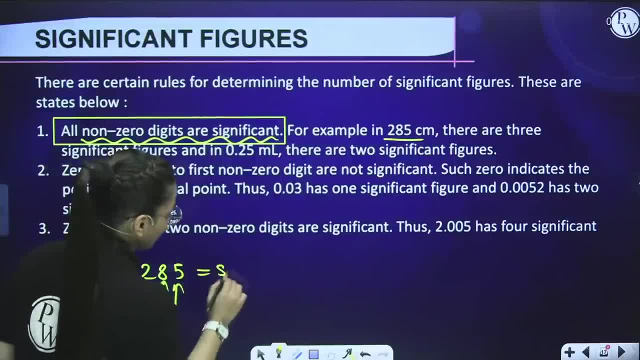 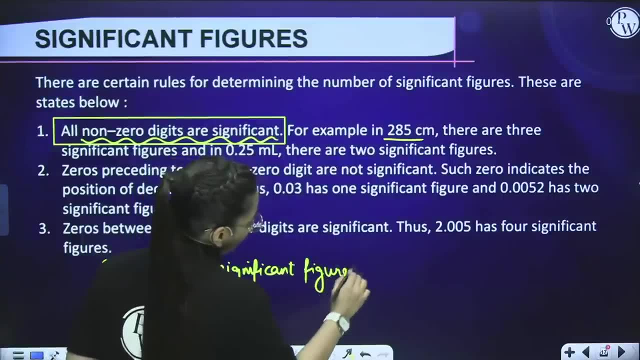 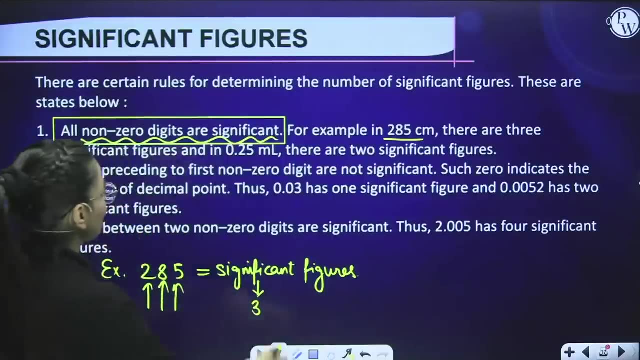 so how many significant figures are present? three significant figures are present. you just need to find out the non-zero digits, because all non-zero digits are significant. so how many significant figures here? here are three. okay, one more example is 0.25. so how many significant figures are? 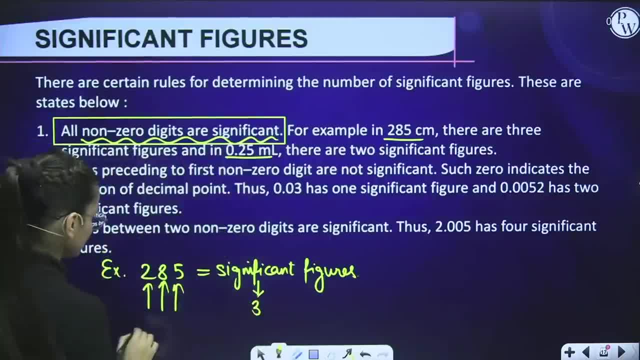 there. i have told you that only non-zero digits. 0.25 contains 0, which is zero digits, so this will not be counted. hence 2 and 5 will only be counted. so there are two significant figures. hopefully the first rule is clear to you. the second rule is zero is proceeding to four. 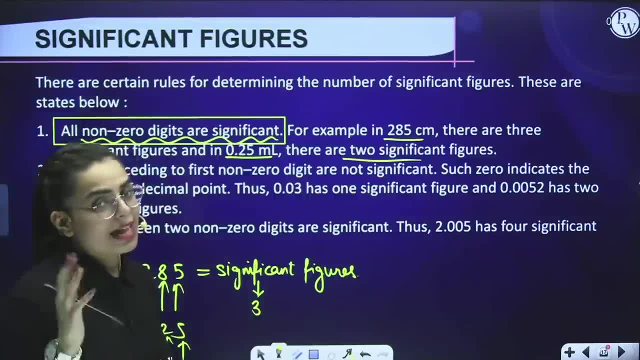 digits. so if the first non-zero digits are not significant, that means if there is any non-zero digit and the zeros are present before that, they won't be counted. okay, so let us take an example: 0.03. so this is the first non-zero digit. three is the non-zero digit. 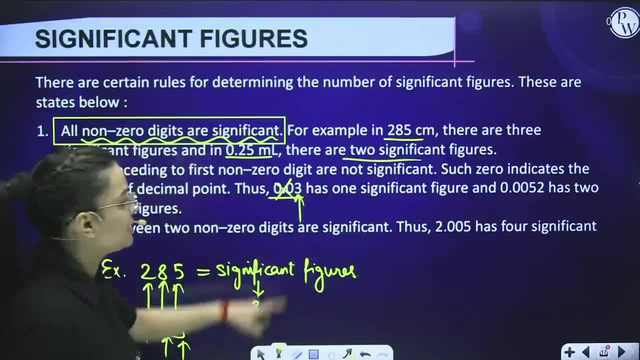 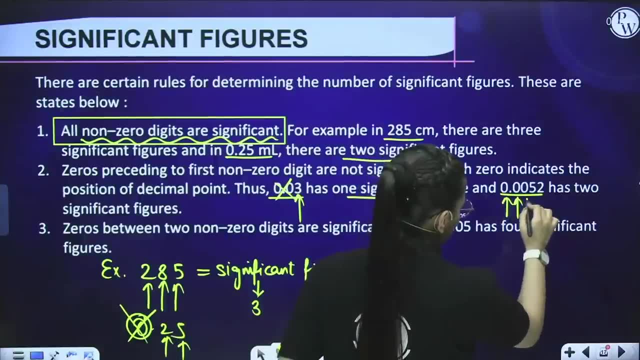 and if a zero arises before that, these zeros are not counted. hence it has only one significant figure and, coming towards the next case, 0.0052. these will not be counted because they are coming first non-zero digits. hence the answer is only 5 and 2 will be counted, so answer will be two. 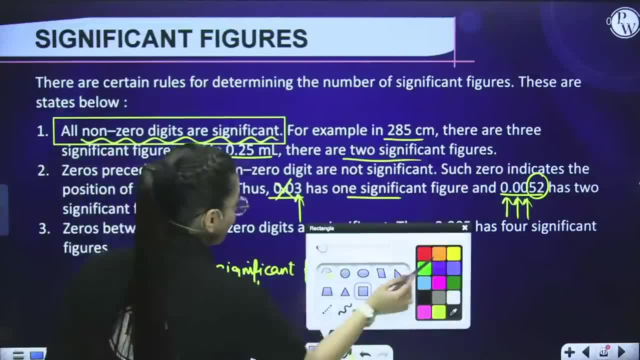 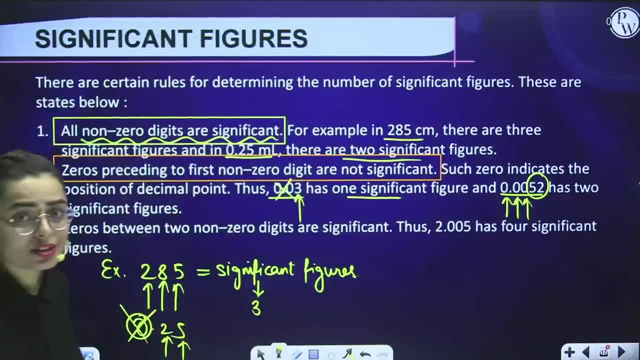 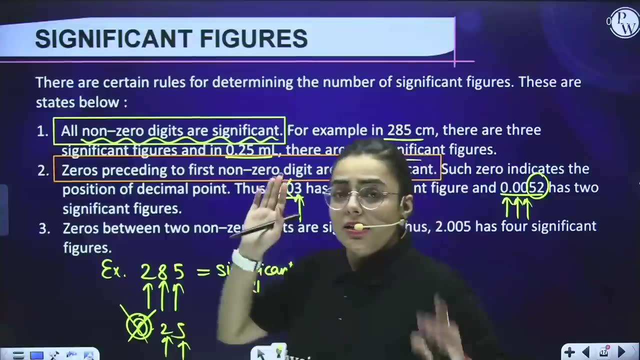 significant figures. so kindly, please put it into a box again, because this rule is also very, very important for you people. now coming towards the third rule, students: what is the third rule? i would say? the third rule is very simplest: zeros between two non-zero digits are significant, see zeros. 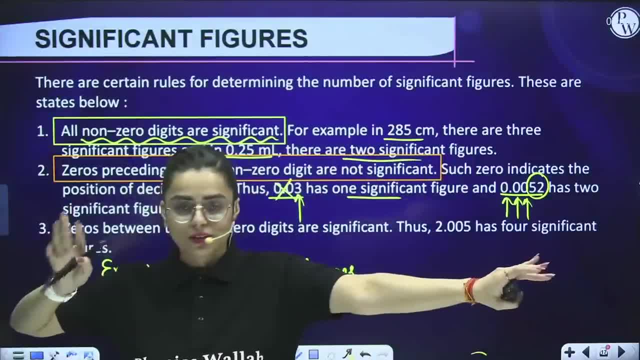 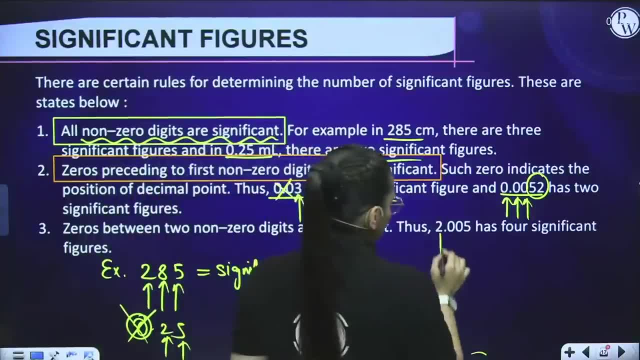 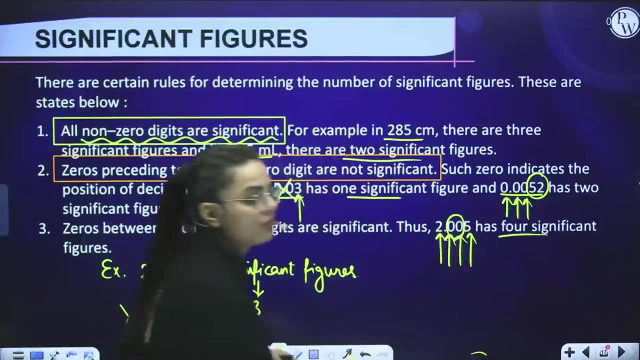 before, non-zero digit is not significant, but between between two non-zero digits is a significant. let us take an example. this is non-zero digit, this is non-zero digit and these are the zeros, so these will also be counted, and hence there are four significant figures in this. 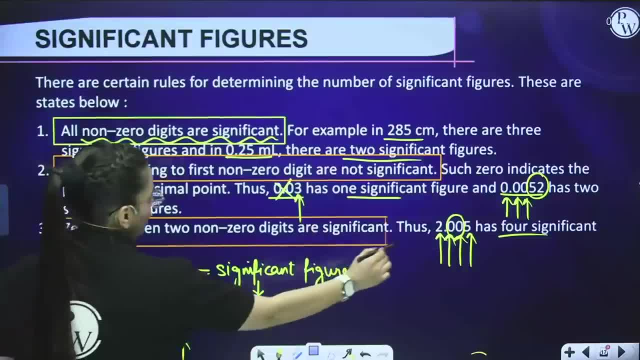 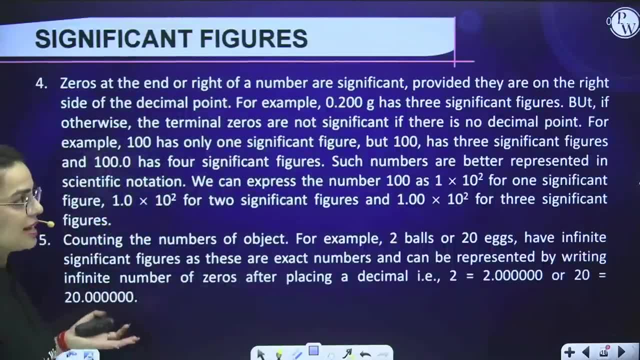 case. so this rule is also most important, so kindly underline them. and now we are moving towards the last two rules of the significant figures. the last two rules state very easy. you have told you the value of zero before the non-zero digit and in between the non-zero. 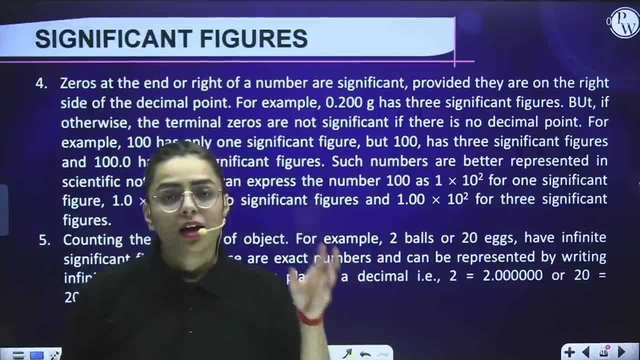 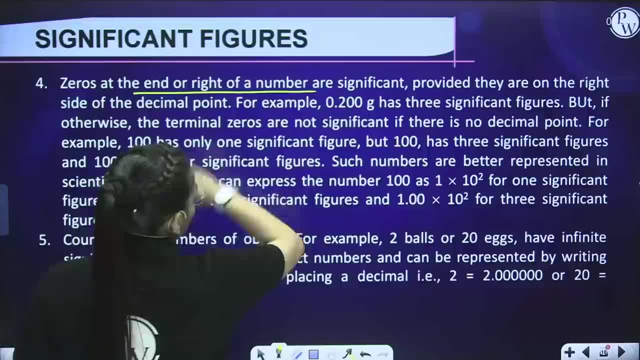 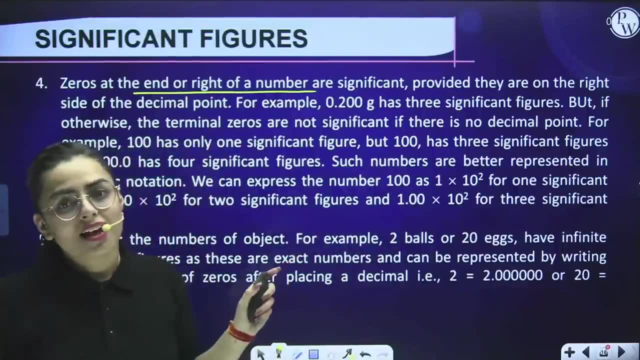 digit. now we are talking about the zero value after the non-zero digit and in the case of decimal. so let us see: zeros at the end or right of the number are significant before and center scene. now the right one case or the end, one same case. the zeros are significant, provided they are. 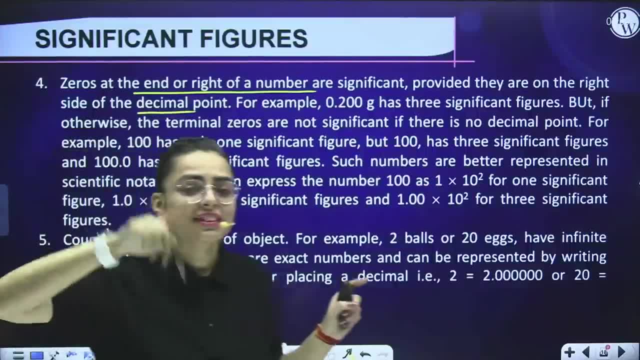 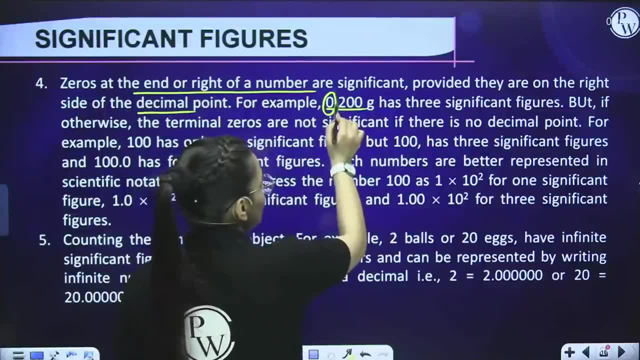 on the right side of the decimal, but they will only be counted when they are at the right side of the decimal loud. so let us take this example. will the zero be counted? no, because it is before this decimal, so it won't be counted. this two is non-zero. yes, it is counted, and these two zeros are after decimal, so 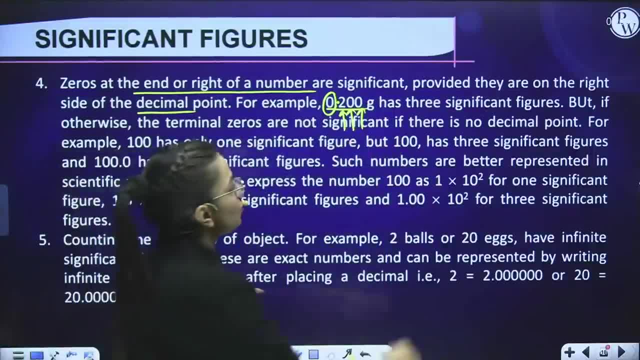 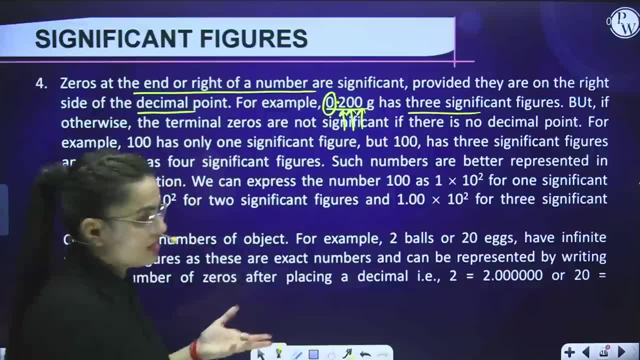 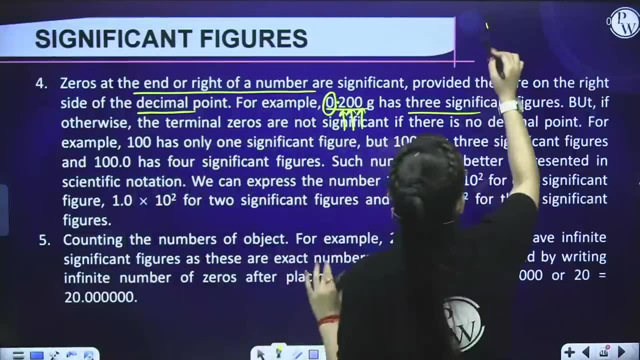 they will be counted. how many significant figures are there? there are total three significant figures here. okay, but if otherwise, the terminal zeros are not significant is there is no decimal point. so see, if there is no decimal point, for example, simply 200 is given to you. one situation is only. 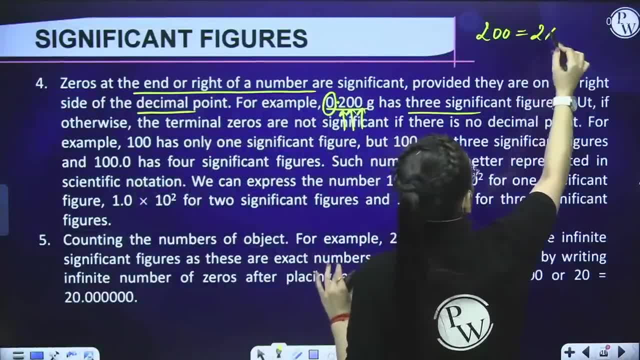 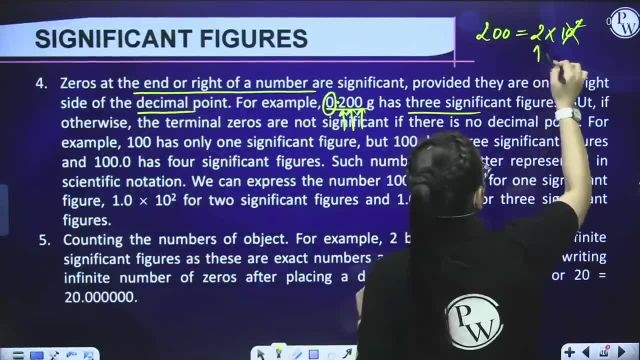 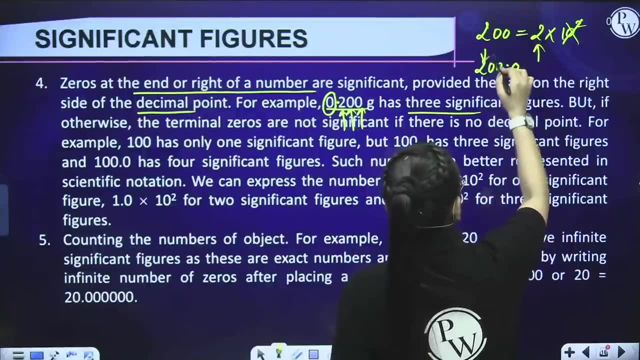 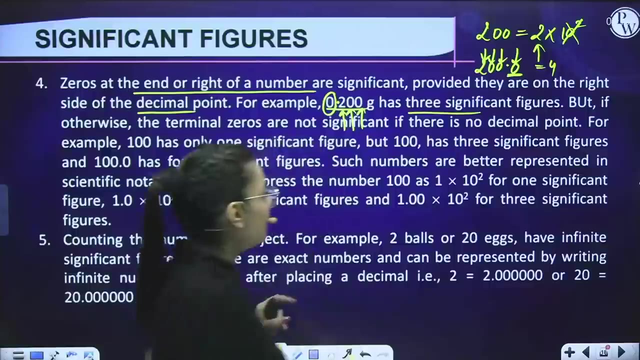 200, you will be counted if there is no decimal point. so if there is no decimal point, for example, you can write it as 10 to the power 2- we have already done in scientific notations, right. so these will not be counted and hence only one significant figure. but if it is given to you 200.0, then after non-zero digit, this is also counted. hence, how many significant figures. four, clear, okay. now let us take one more example. they have taken 100. 100 has only one significant figure. why? because we can write it as 10 to the power 2. we have already done in scientific notations, right. so these will not be counted and hence only one significant figure. but if it is given to you 200.0, then after non-zero digit, this is also counted. hence, how many significant figures. four, clear, okay. now let us take one more example. they have taken 100. 100 has only one significant figure. why? because we can write it as 10 to the power 2. we have already done in scientific notations, right. so these will not be counted and hence only one significant figure. but if it is given to you 200.0, then after non-zero digit, this is also counted. hence, how many significant figures. four, clear, okay. now let us take one more. 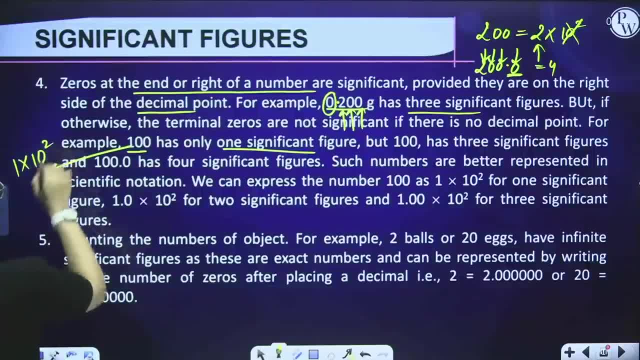 write 100 in terms of 1 into 10, raised to the power 2, and this is not counted and hence only one significant figure is there. but, students, if i talk about 100.0, then after decimal 1 will also be counted and hence they have four significant figures. the same thing which i've explained you. 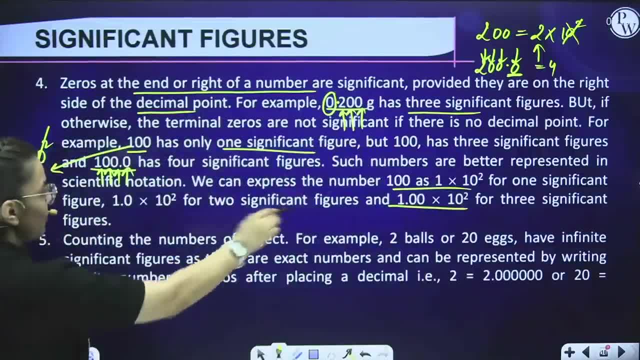 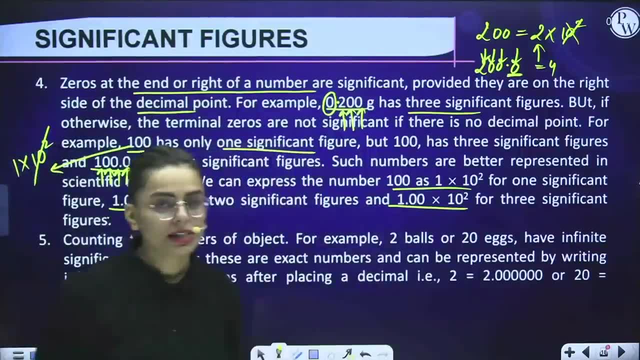 is written here: in both of the situations they have taken 100 as an example, 1.0 into 10, raised to power 2 as an example, and 1.00 into 10, raised to power 2, as an example. now coming towards the: 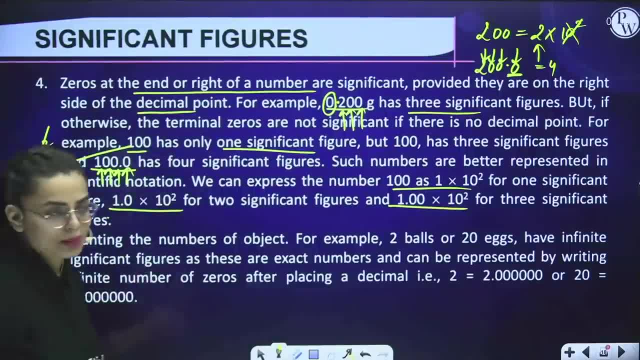 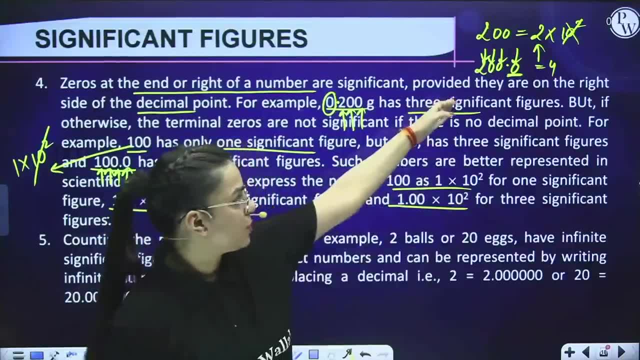 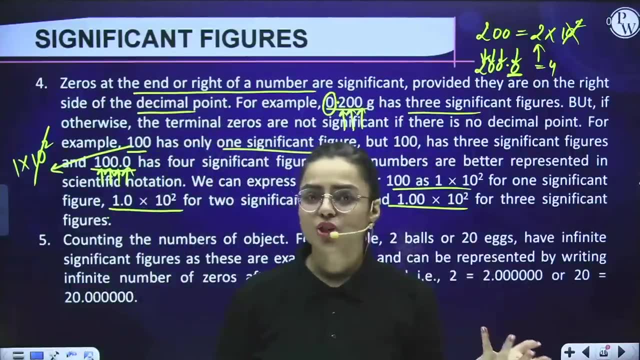 last rule, that is, counting the numbers of object. for example, if i say 200 and if i say 200 balls, so if i say 200, it is referred to as what it is referred to as this situation, which is which i've explained you. but if i talk about 200 balls, i am talking about an object and when i'm 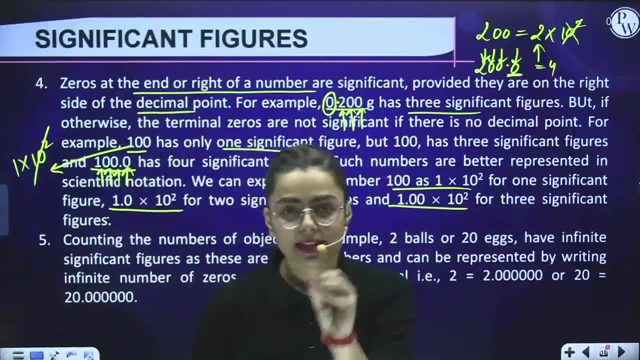 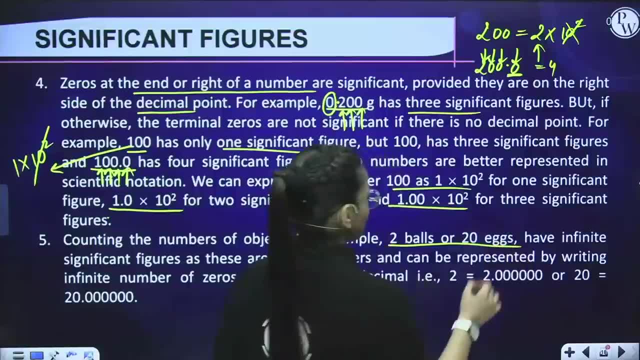 talking about an object, then it has no limit and hence its significant figures are infinity. so in this case you can see that if directly it is given to you two balls, 20 eggs, so the answer is no limit and hence its significant figures are infinity. so in this case you can see that 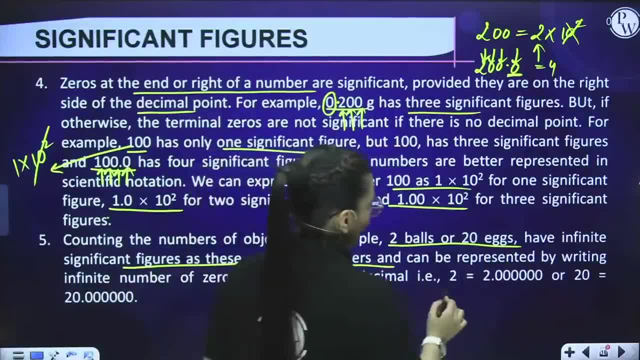 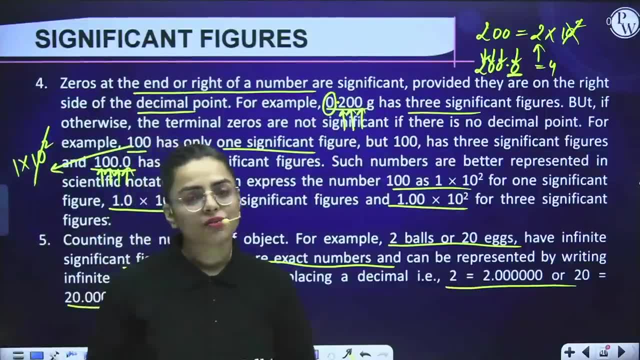 it is infinite significant figures, because they're exact numbers and we can write these numbers in such way. so when there is an object, you need to remember this thing, students, that it has infinite significant figures, but if not mentioned, then you have to do in the same case. okay, now let 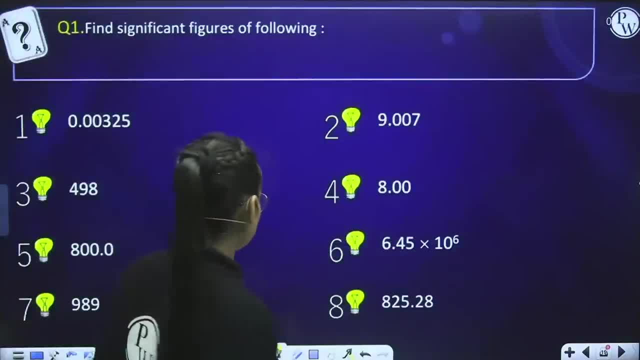 us apply these rule in the following questions. the very first question is in front of you. okay, first thing, students. as you know, questions are there. many of the students will skip this portion just for the sake of this video, so if you have any questions, please do not hesitate to. 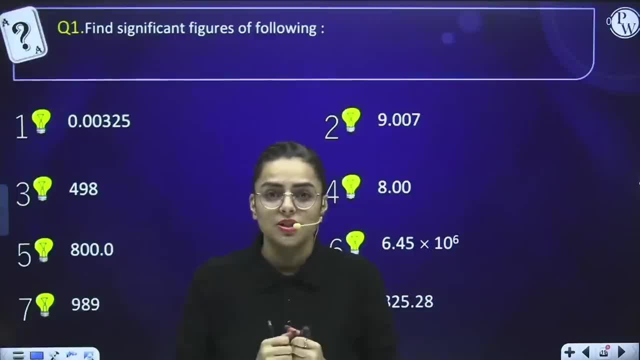 let us know in the comments below if you have any questions. please do not hesitate to let us know in the comments below. if you have any questions, please do not hesitate to, for the sake that they are very uncomfortable to do questions. let me tell you whenever you face. 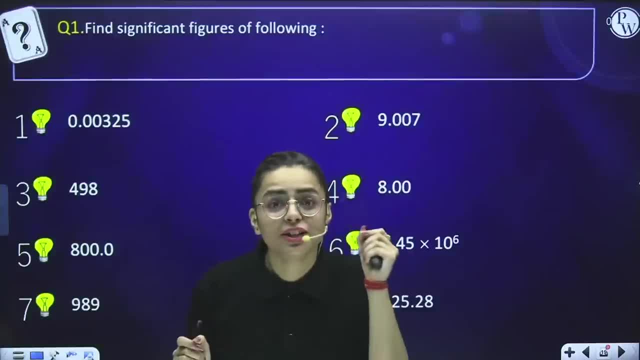 get it done. questions whenever you face, you questions whenever you face. and okay, great, don't lose hope, just try again second time again. they are not, they are not coming the exact answers. no problem, don't lose hope. try once, twice, thrice, four times, five times, six times. i am assuring you. 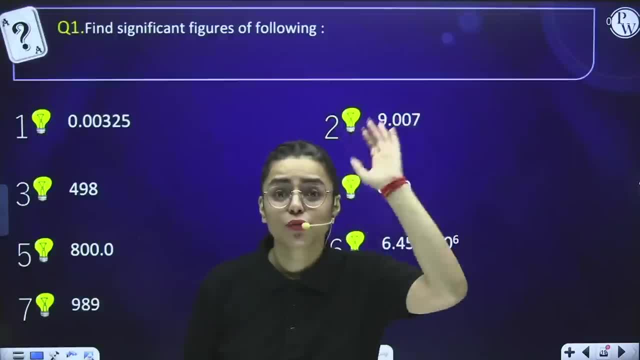 the same, that after 10th or 15th or 20th or 40th time you will be like: give me any question. i can do any question because you have understood the concept very deeply by practicing. so please, practice to achieve your success. more practice will lead you towards the success right. so first, 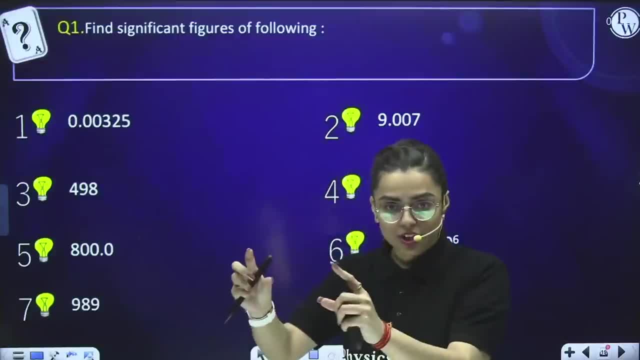 of all, i will tell you how to look into the question, which approach you should apply towards the question, and then we are going to solve. we have seen five rules. we will consider the rules and we will solve the questions. okay, with me, you are going to do and you are going to achieve it. 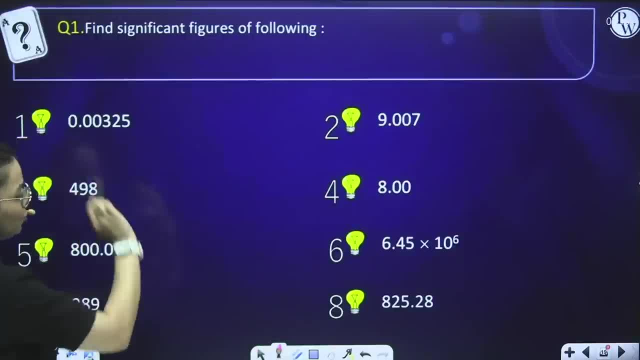 so see, the first question is 0.00325. here you need to first approach towards this concept that you need to find the non-zero digit. what is the non-zero digit? non-zero digit is the one in which zero is absent. so here, this is zero, this is zero, this is zero. 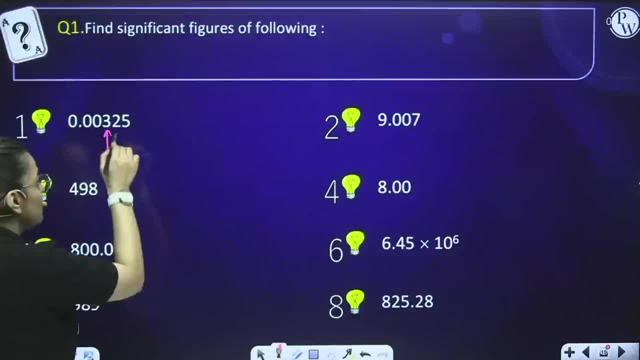 hence they won't be counted. this is the non-zero digit. this is the non-zero digit, this is the non-zero digit, so all non-zero digits are significant. and second rule was that before non-zero digit, zeros are not counted, so before the zeros are not counted. hence its answer is: 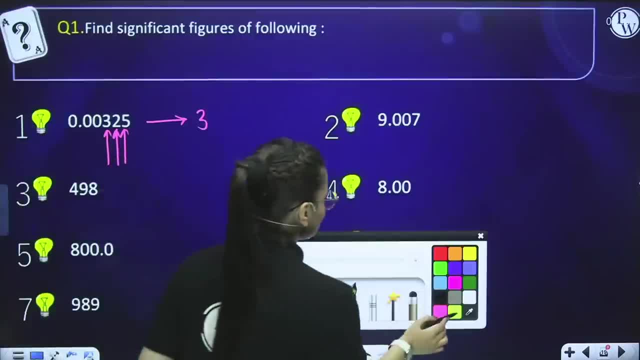 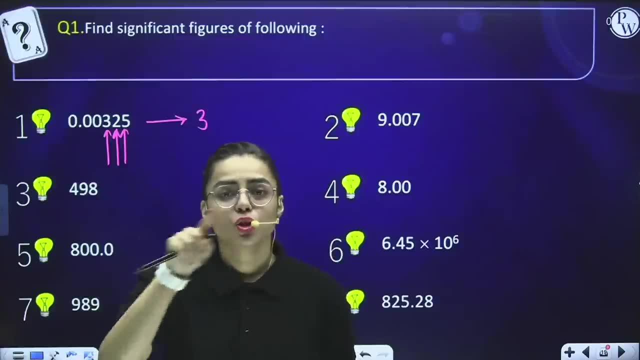 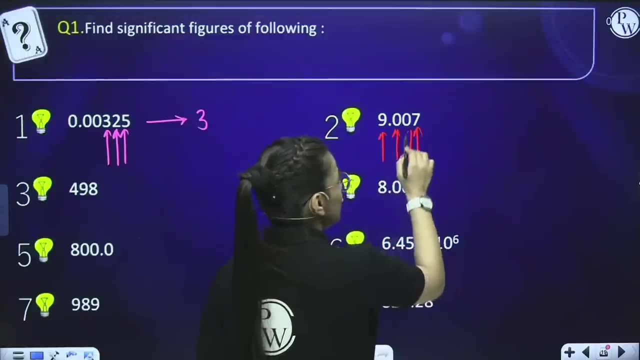 clear. now comes the next case. students see this case in this case is 9.007. we have studied this rule: if zero comes in between two non-zero digits, then they are counted. this is the first non-zero digit, this is the last non-zero digit and hence these zeros will also be counted because they 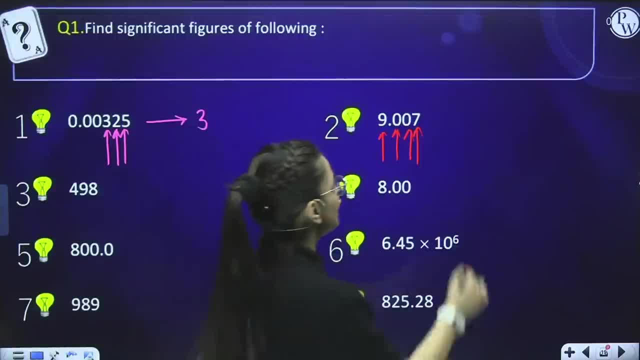 are coming in between. hence, how many significant figures are present? four, right, very good. now, coming towards the third question, as i told you, if object is mentioned to you, then you have to write infinity. if it is not mentioned, you have to directly do this. how many non-zero digits? three. 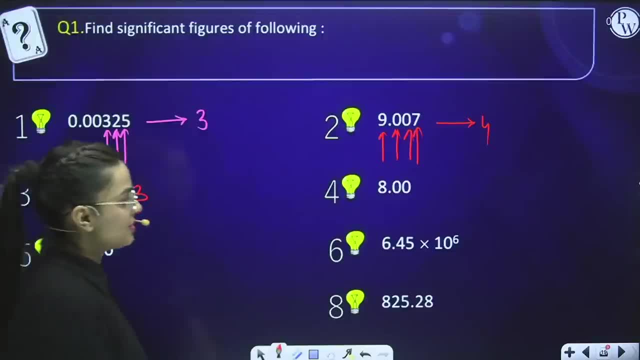 answer is three. coming towards the next case, fourth case: 8.00. i told you the after first non-zero digits. if any decimal is there and zero is approaching afterwards, then it will be counted. so these will be counted after decimal ones. answer is three. now, in this case also, answer will be: 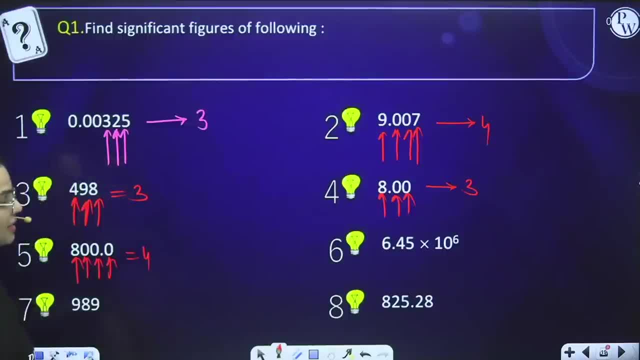 one, two, three and four students now coming towards the next case. as i told you that one into 10 raised to the power two, we have not considered 10 raised to the power two. hence again, 10 raised to the power six will not be included. answer will be one, two and three students now coming towards the next case. you can. 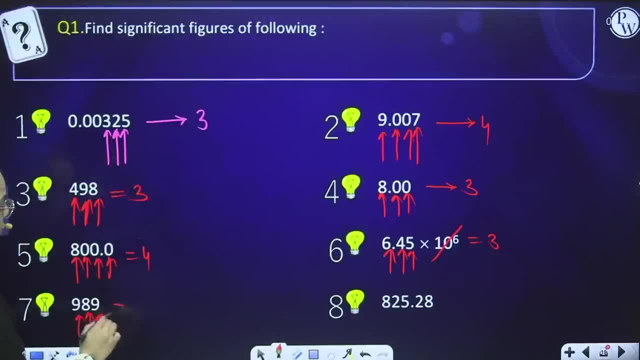 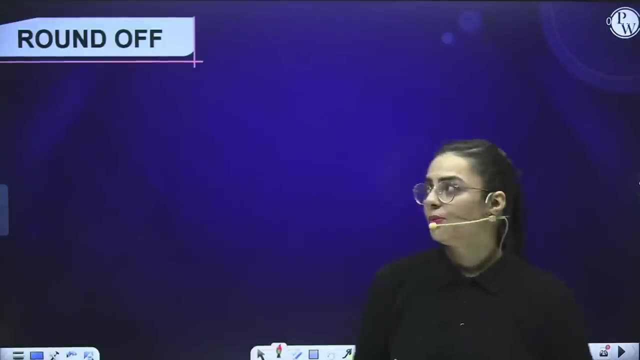 say 989, here will be three of the non-zero digits. answer will be three. the next question: all are non-zero digits- one, two, three, four, five. answer will be five. so this was all about our significant figures questions. now we are moving towards the round of portion. round of portion is very simplest portion. you have already done this in, you know. 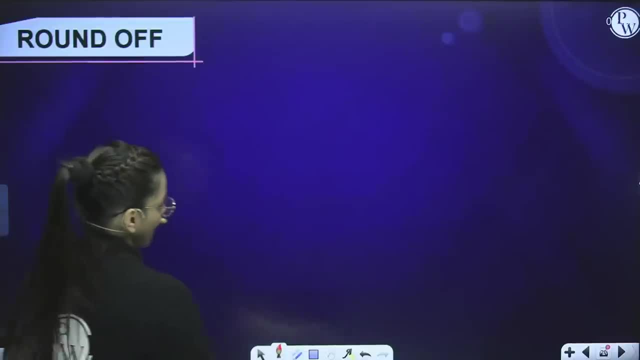 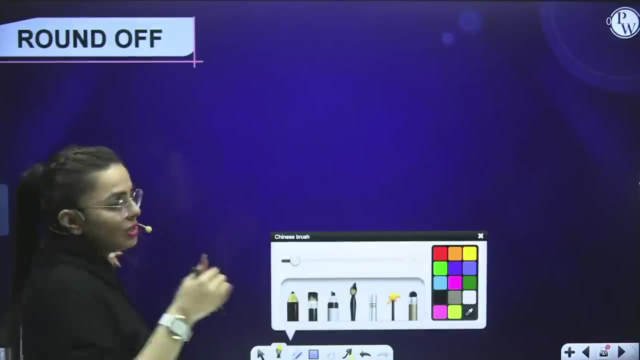 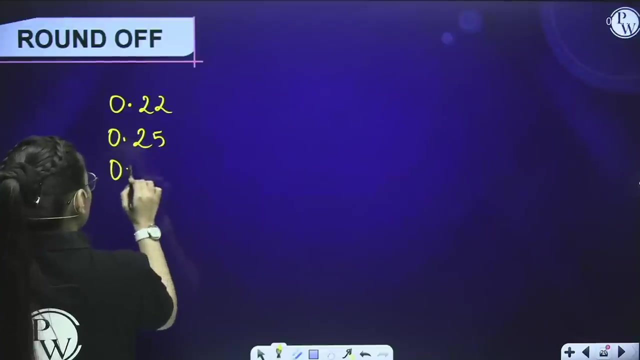 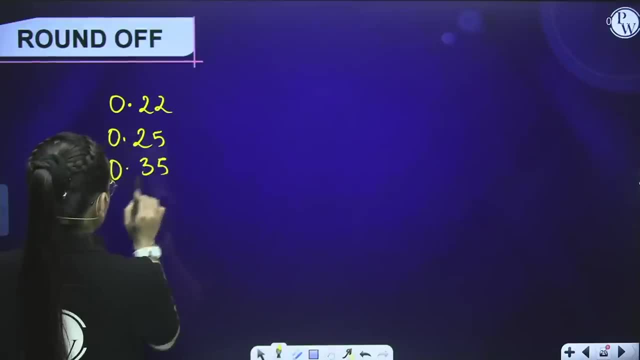 you have 0.27, you have 0.28. now what you need to learn is, whenever the last digit is more than five, then the number before them before that will get a number and the last digit will disappear. how see, in this case, eight is more than five, the last digit, so it will give its one number to. 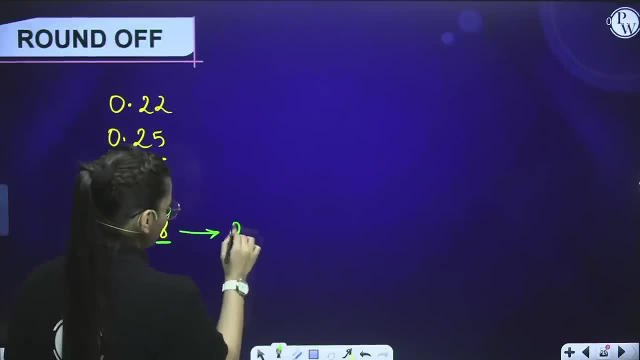 to this and will disappear and will do round off. so what is the answer? 0.3, because eight is more than five. now take this example: 0.27. seven is a big number, more than five. it will give its number to two. it will be 0.3, clear. 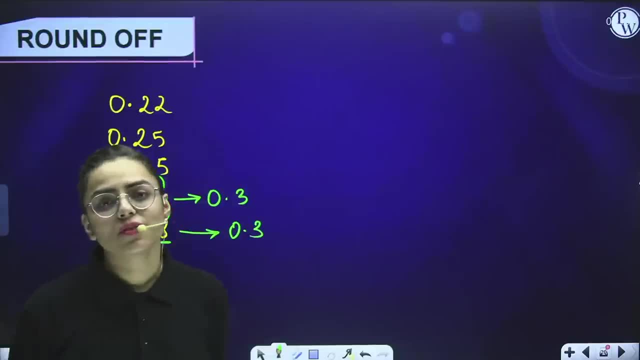 now coming towards the case when the last digit itself is five. what you will do in that case, students? when the last digit is five, but before that there is an odd number, here is three. hence it will be getting one number from it, so it will be zero point four. 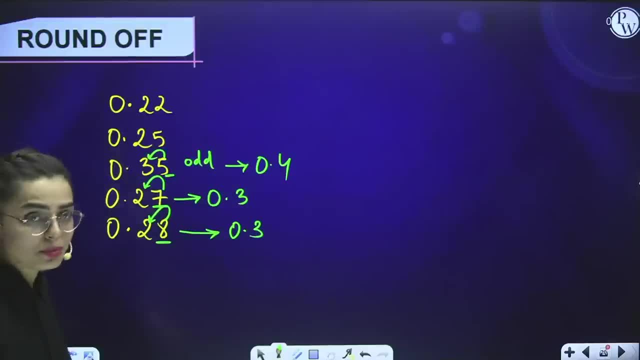 but if there is an even number before five, it will not get any point and the answer will be zero. point two, because i told you, round off only occurs when the number is more than five. that's why, okay, the last case here is zero. point two: two students, in this case the 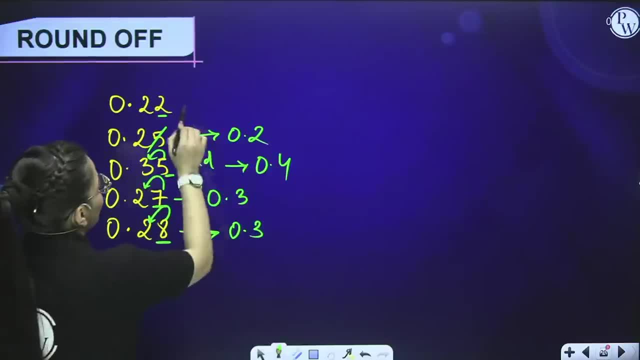 last digit is less than five. hence it will remain same and the answer will be zero point two. so this was all about round off situations. students, you- yeah, you- will be observing some of the questions in addition: subtraction, multiplication, division and distribution- you will get two. but in the round, a round of case, you just need to find out the decimal places in addition, and 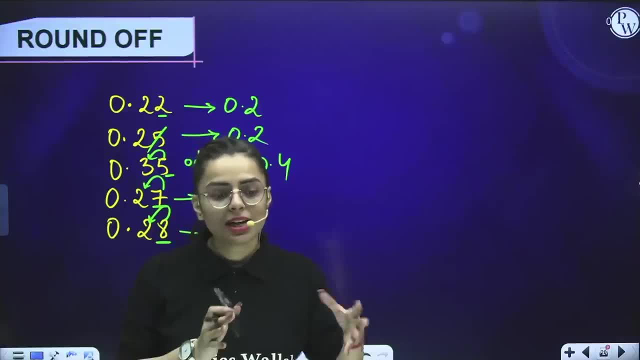 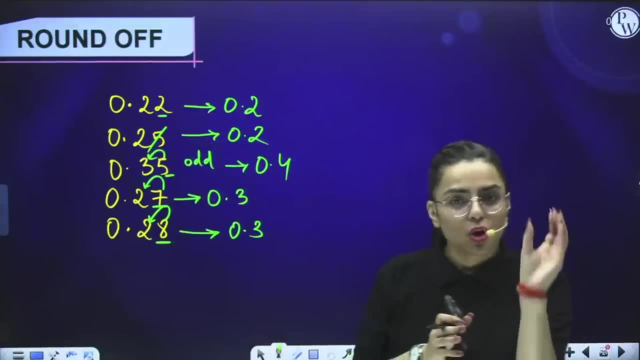 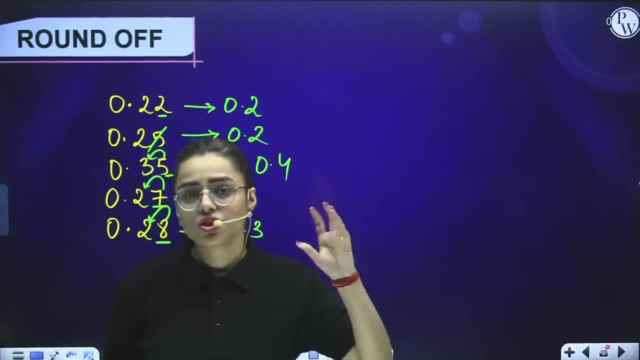 subtraction. if you are given some questions, just see how many decimal places are present and the answer will contain the same decimal places as of the shortest number. but in the case of multiplication and subtraction you have to see the significant figures rule. this is not so important, just you need to know about the round of. i just give you a brief about. 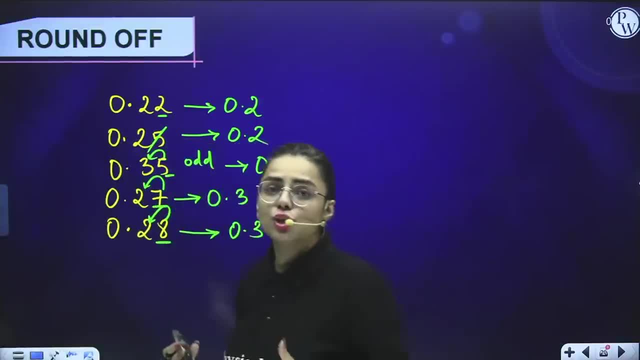 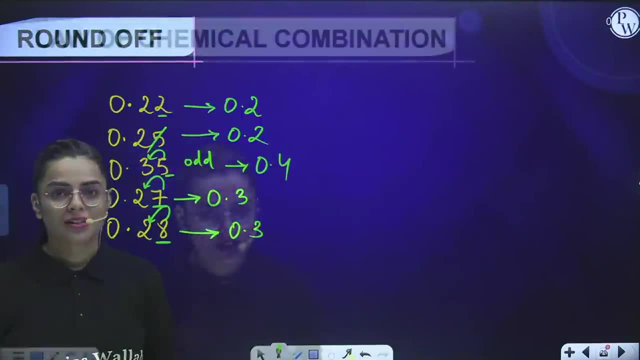 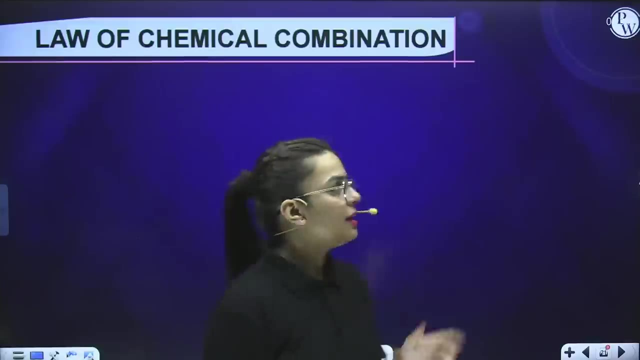 that situations. now we will move forward towards the laws. so let us start the laws position. you can note it down and you can practice more questions on this concept. law of chemical combination: students. there are various laws of chemical combination. one of them are law of conservation of mass. 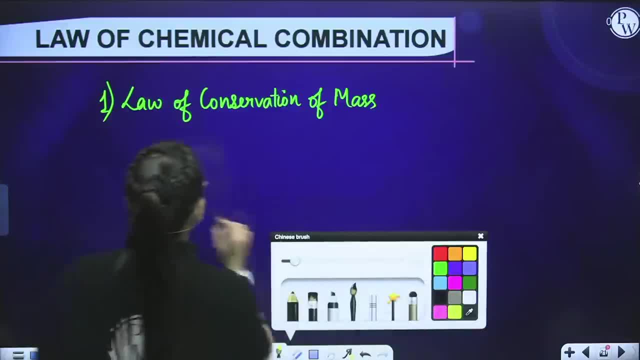 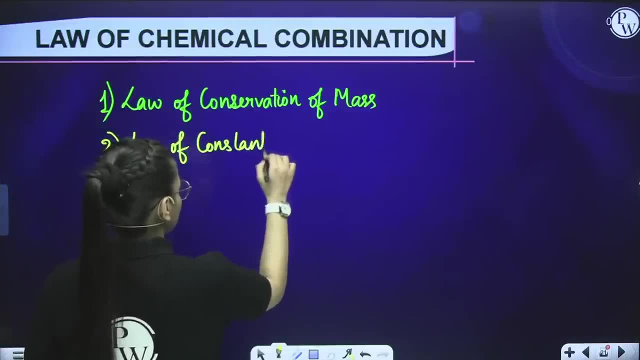 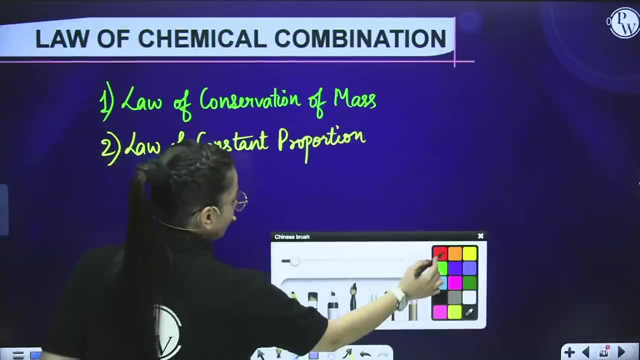 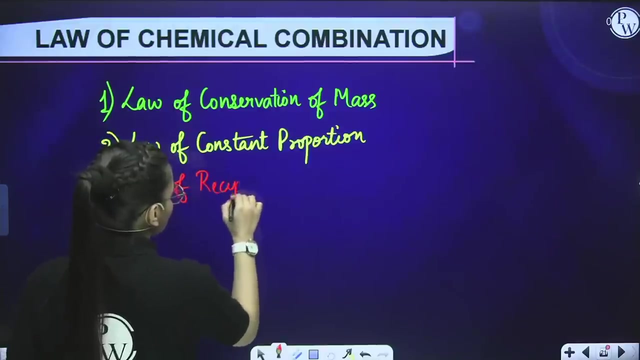 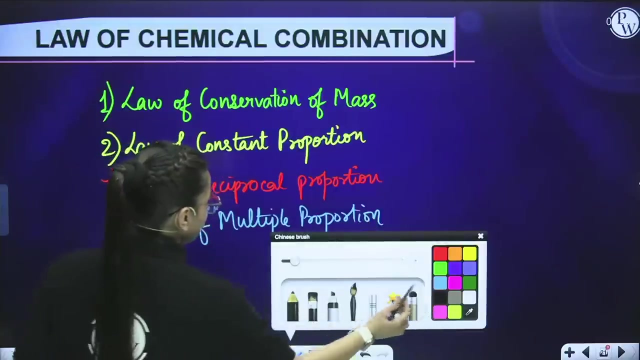 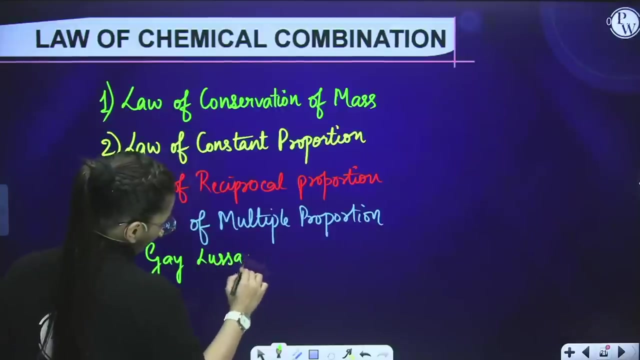 the second one is law of constant proportion, students. the next one is law of reciprocal proportion, the next one is law of multiple proportion and the last one which we will study will be gay-lussac's law of volume. okay, so now let us start from the very first law, that is, the law of conservation. 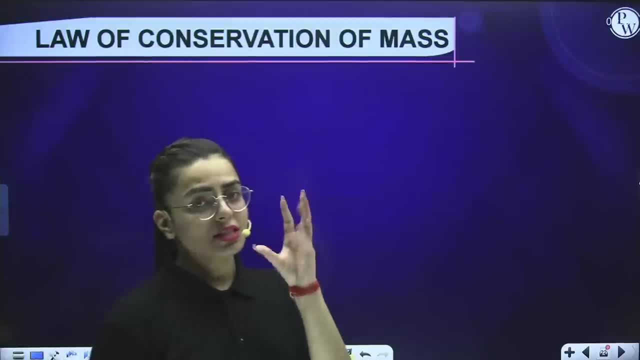 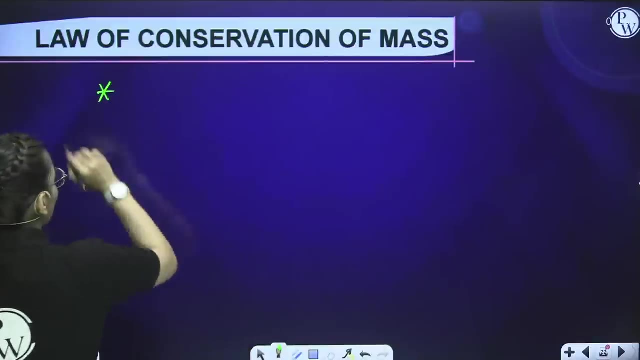 of mass students. law of conservation of mass teaches us that mass can neither be created nor be destroyed in any chemical reaction. what we observe here is that total mass of reactant is equals to the total mass of product. so this is the main important point that we 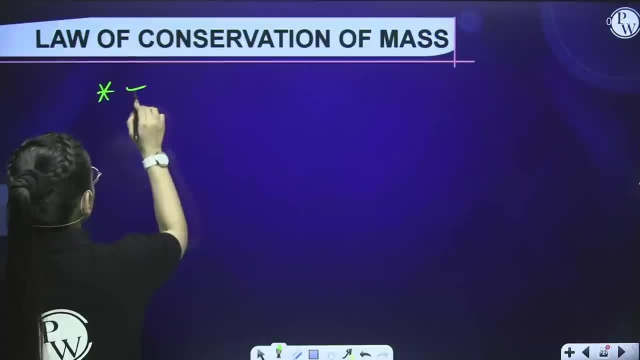 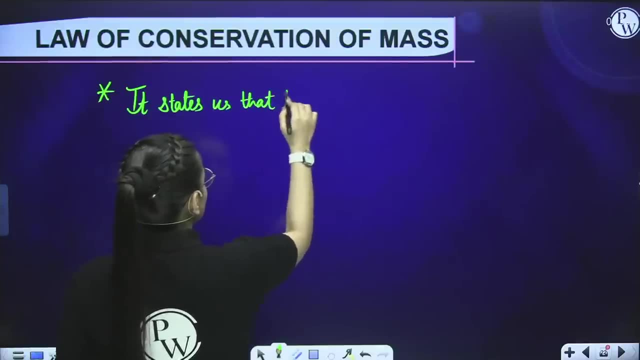 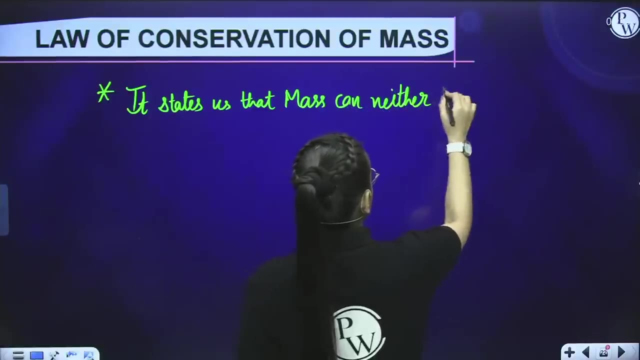 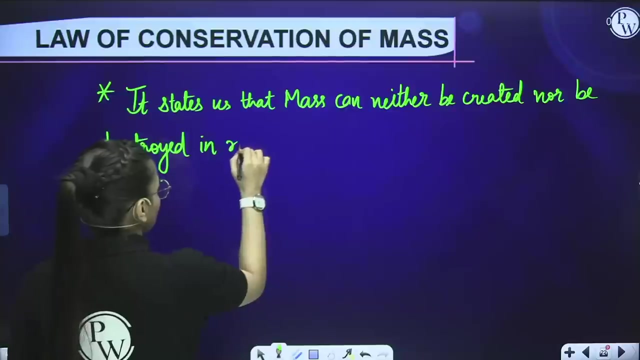 need to remember, during the law of conservation of mass, that it states us. it states us that mass can neither be created nor be destroyed, nor be destroyed in any reaction. so the most important point, that total mass of reactants is equal to the total mass of product. it is very simple, students. okay, the total mass of products. okay, so total mass. 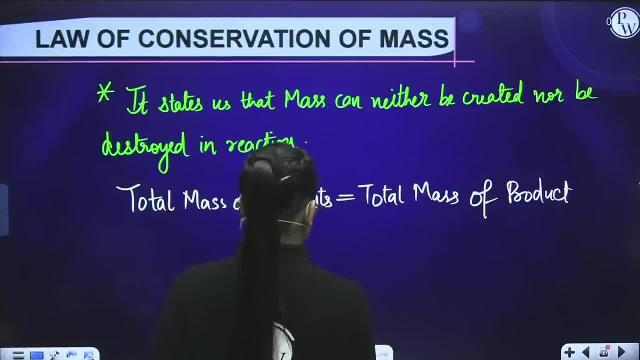 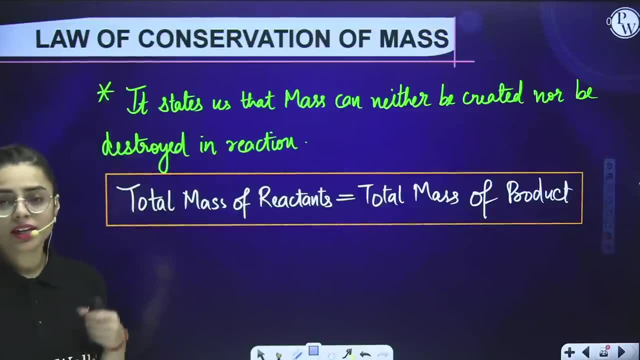 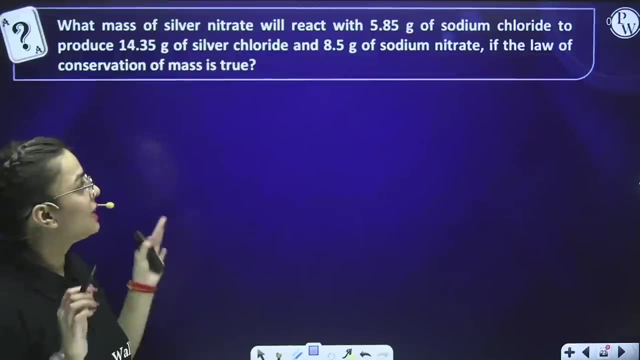 of products, guys. ok, i will pass to the question of conservation of mass. now the top. Ah, let us go ahead. right, kindly put this into a box so that you remember for your further questions. now let us apply this formula into our very first question of law of conservation of mass. 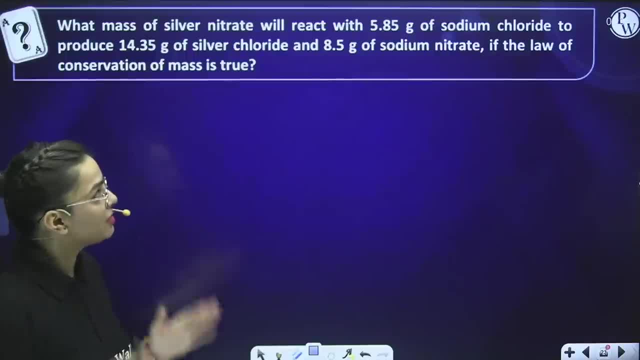 what mass of silver nitrate will react with 85.85 grams of sodium chloride to produce 14.35 grams of silver chloride and 8.5 grams of sodium material, so that 어�, you will start by saying unstoppable maw on Bai o. 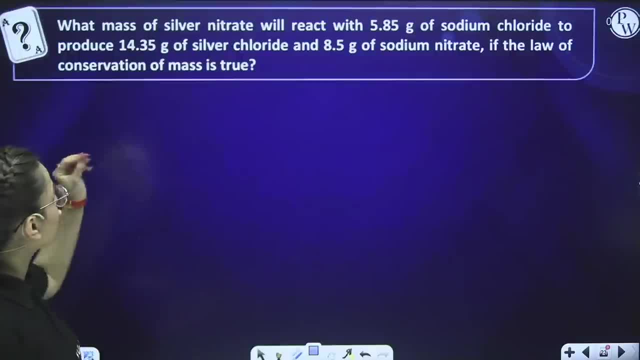 grams of sodium nitrate. if the law of conservation of mass is true, so we need to prove it. if it's true or not, okay, if it's true, then we have to follow this and we need to find what we need to find the mass of silver nitrate. right, okay, first of all, i am going to write. 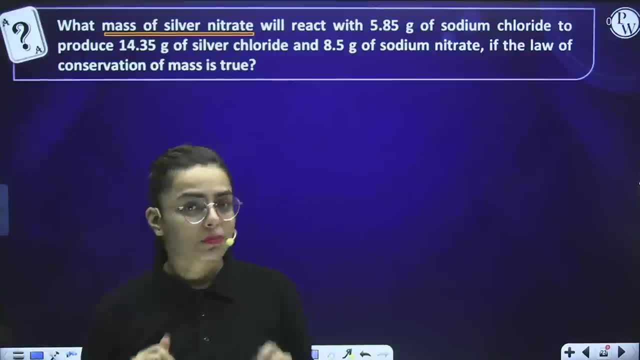 the given situations, which is given to me, the given substances and their masses, right. so it's given that silver nitrate- it means AgNO3- it will react with 5.85 grams of sodium chloride. what is sodium chloride? it is NaCl to produce. now it is producing something, that is, product is being formed. okay, then we're going to apply. 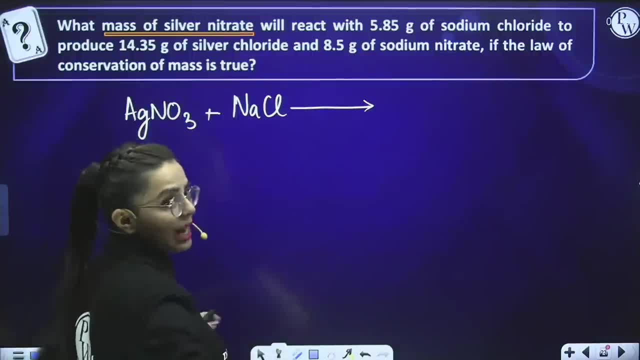 an arrow. now, what is being produced? silver chloride- that means silver chloride- is our AgCl, and 8.5 grams of sodium nitrate- sodium is NaCl. Now we need to calculate the value of sodium nitrate, as we have already done, isn't it? 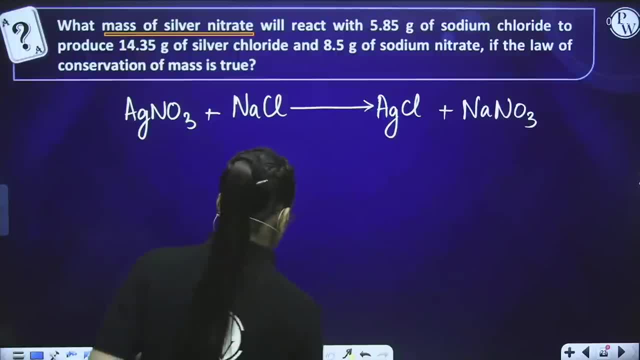 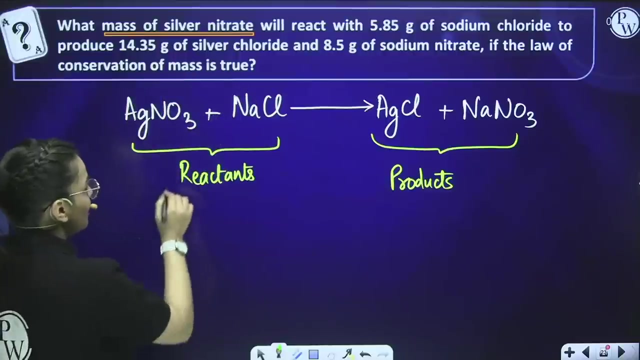 nitrate will be NaNO3.. So, students, first of all, write this as like this: These are our reactants, which react together to form products. Right, You all know these things. Good, Now, students, we have been given that we need to find the mass of silver nitrate. So let us say that. 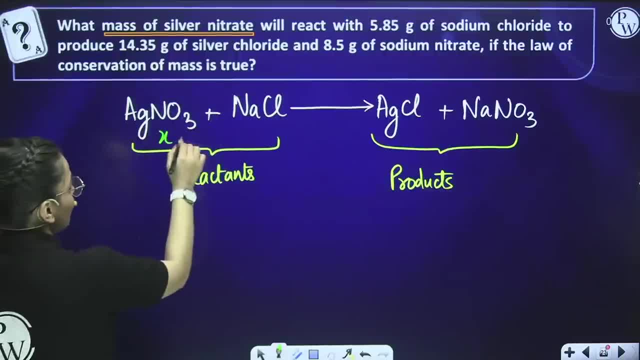 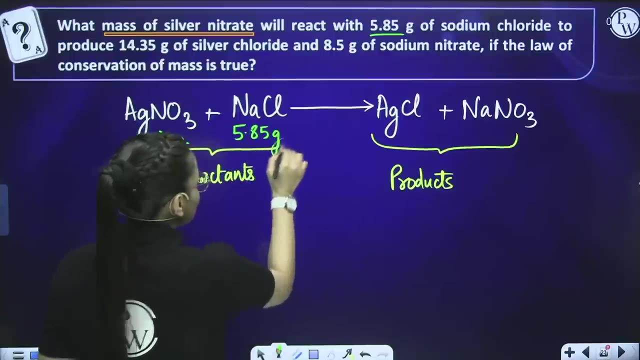 its mass is x grams, because everything is taken in grams. So we assume that the mass of silver nitrate is x grams. It is reacting with NaCl, whose mass is given to us 5.85 grams, So it is 5.85 grams, Right. Then it is producing us AgCl, which is about 14.35 grams, Right? 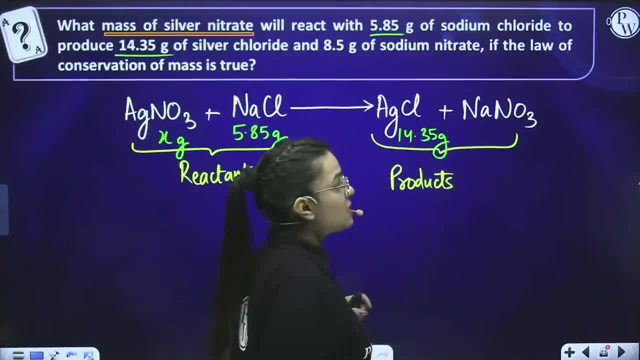 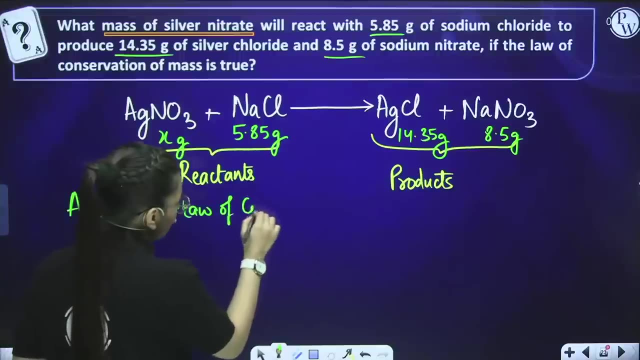 14.35 grams. Moreover, it is producing NaNO3, which is 8.5 grams. So now, as you all know, according to law of conservation of mass, mass can neither be created nor be destroyed. Hence, what do we say? that We say total mass of reactant is. 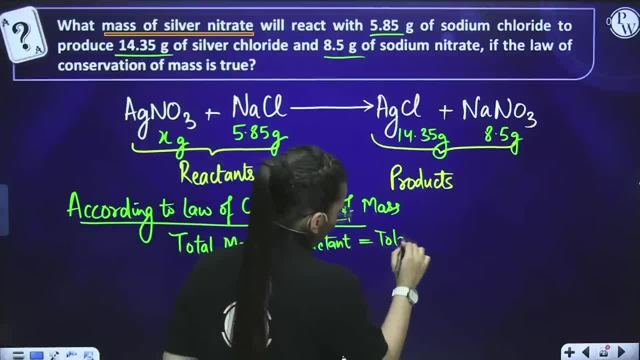 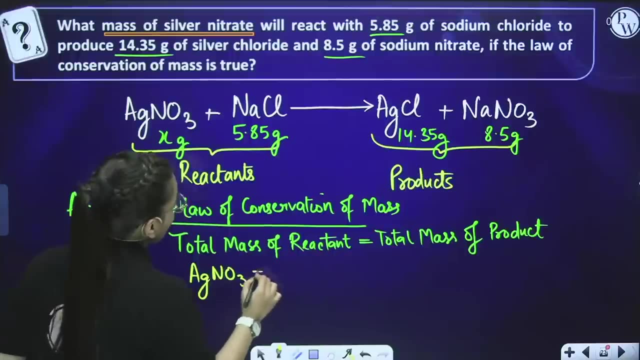 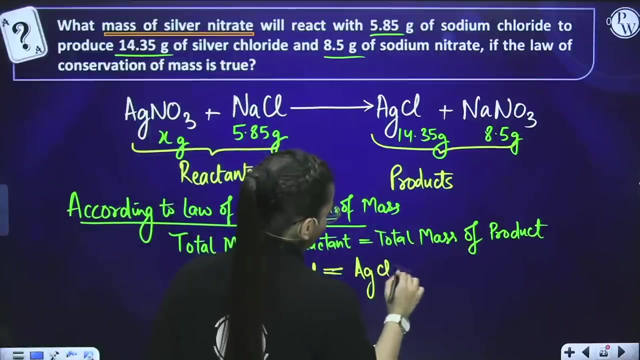 equal to total mass of product. Clear students. So what will be the general formula? General formula will be AgNO3 mass plus NaCl. mass will be equal to the products mass, AgCl plus NaNO3.. Hence we can write that x. 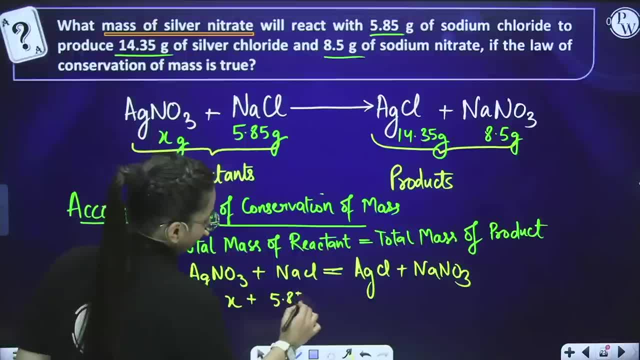 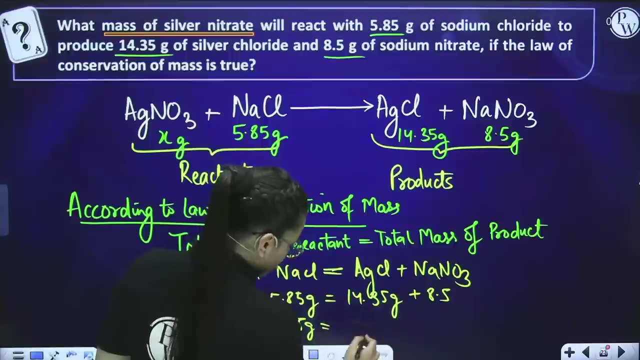 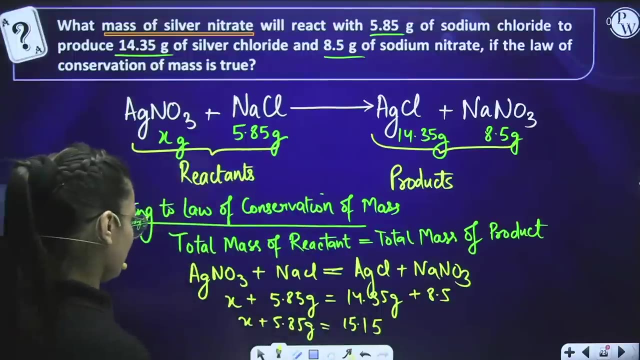 grams plus 5.85 grams is equal to 14.35 grams plus 8.5 grams. Okay, Now, this is x plus 5.85 grams is equals to: we are going to add these: It is going to be students. Okay, Right, It is going. 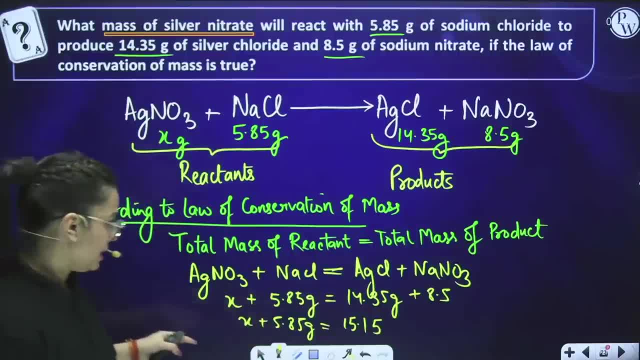 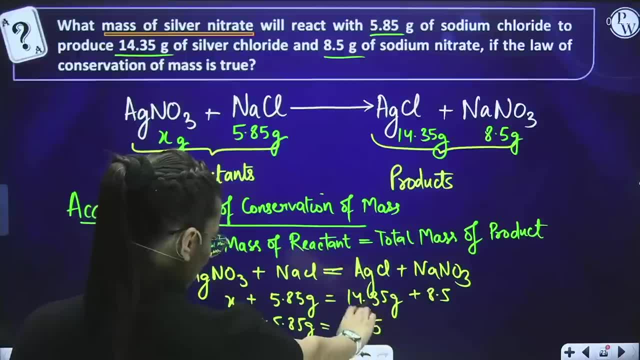 to be 15.15 grams. Let me check this: 14.35 grams plus 8.5 grams, Right, Okay. Okay, Now we are going to take this on the another side, Right, One second. Kindly correct this. Yes, Just to solve this. 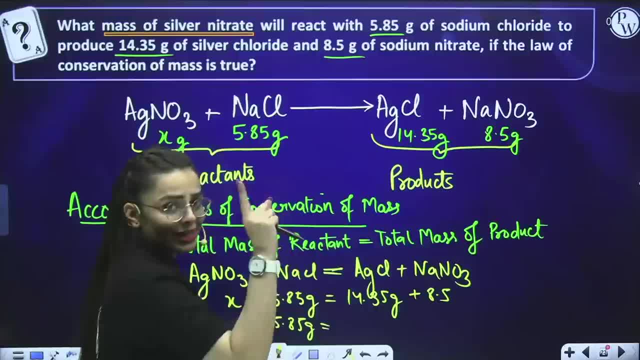 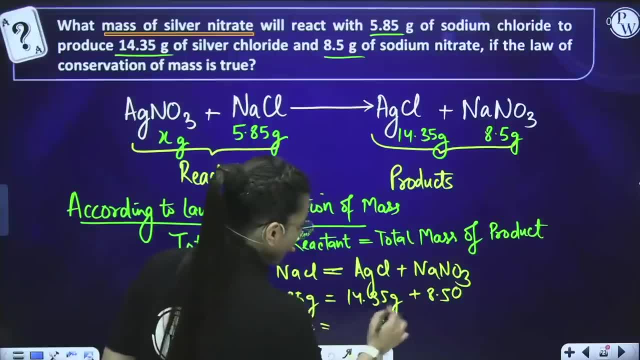 in a better situation. what you can do is, if you are getting this at a one decimal place, put a zero aside here So that it will be easy for you to calculate. Now, 5.35 grams will come here, and this is 8, and 8 and 4 is 12 and 1 is carried forward, so it is 22.85,. 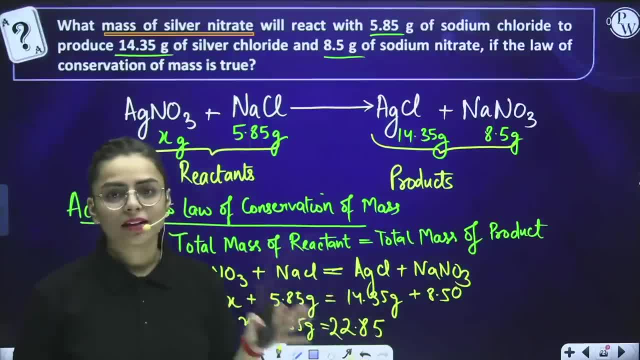 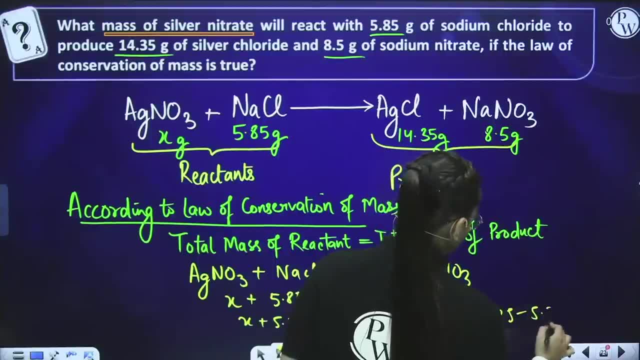 clear. okay, now we are going to this on this side and our x value will come out. so x will come out to be 22.85 minus 5.85, which is about 17 grams students. so our answer is 17 grams. 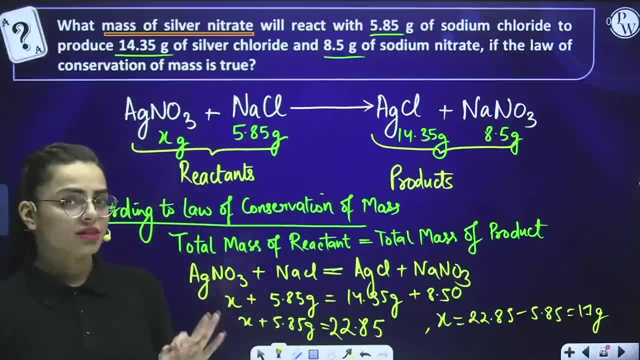 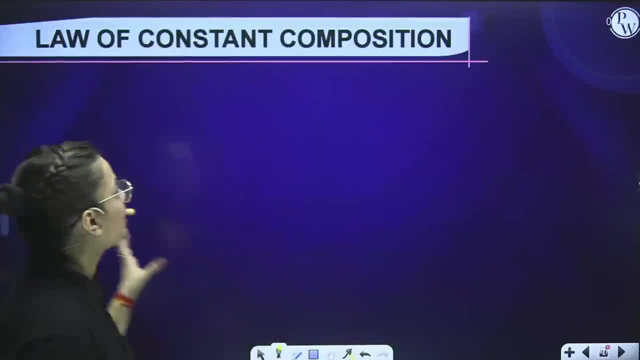 okay, clear, simplest thing that we need to remember in the law of conservation of mass is: total mass of reactant should be equal to total mass of product. clear, very good. now proceeding towards our next law, that is, the law of constant composition. 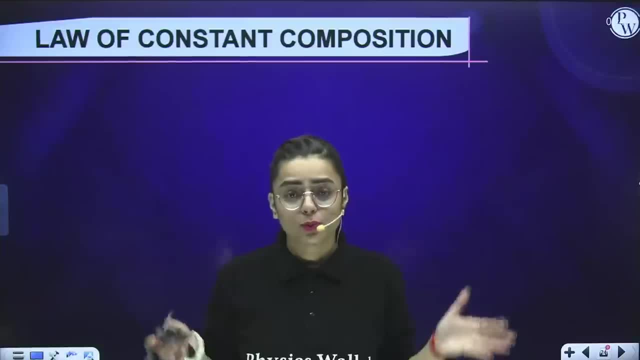 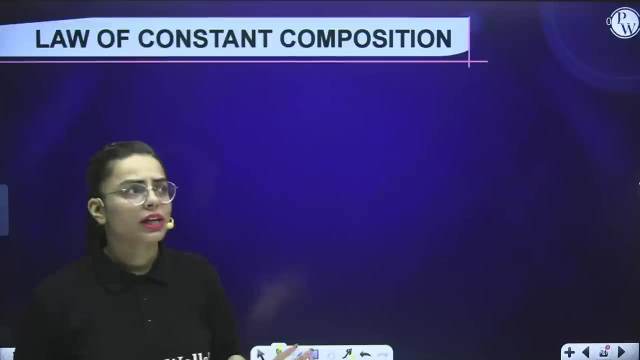 basically, law of constant composition defines us that when two elements combine with each other, they combine in a simple, fixed whole number ratio. okay, now just take an example. if I want water, okay, I am taking a water from you know, at a mountain hills I am taking. 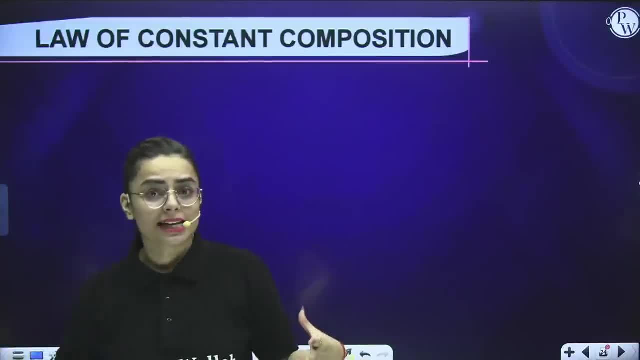 water from river, I am taking water from lakes, I am taking water from pond. the water I am taking from different region is still composed of fixed ratio. water is made up of, like you know, 2 ratio of the like oxygen. there are 2 parts of hydrogen combining with 1 parts. 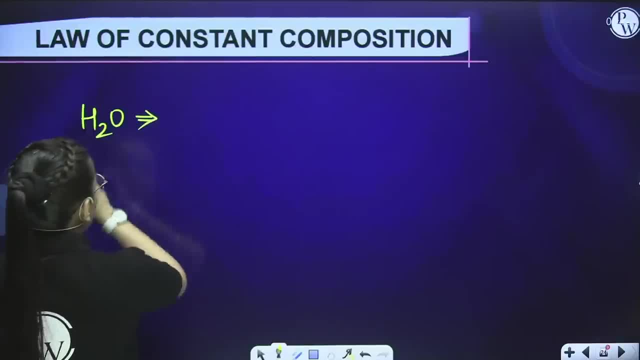 of oxygen. that means if I say what is the ratio of water, water ratio will be 2 ratio 16. that means 1 ratio 8, so if I go on a mountain or if I go on a river, or if I go in a lakeside, 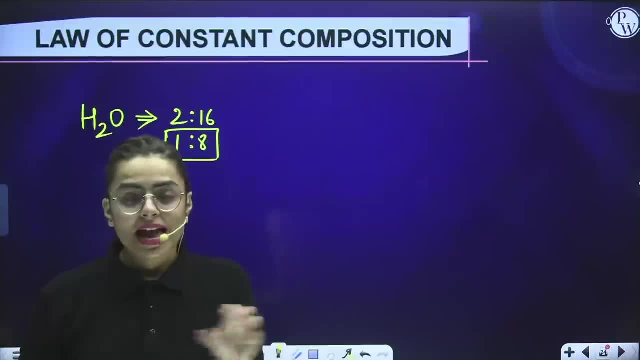 to get water. the ratio will be still the same at any places. so this is what this is: the law of constant proportion: that when 2 elements- the 2 elements are what hydrogen and oxygen, when they combine with each other, then the fixed mass or the fixed weight is observed. 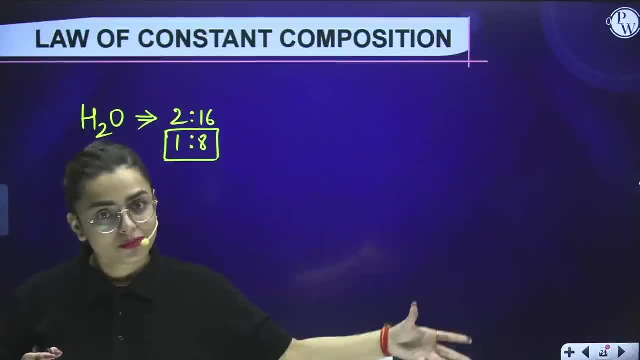 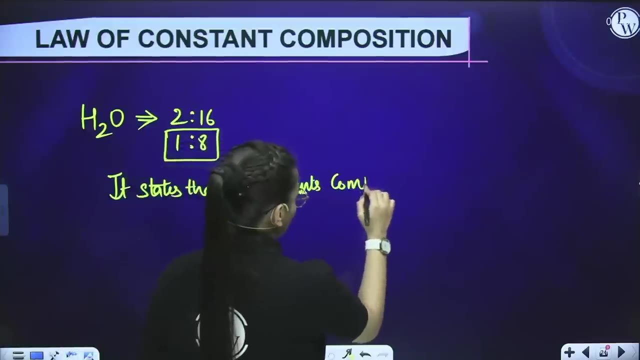 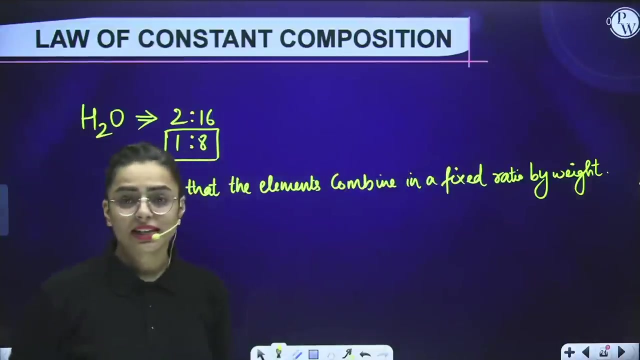 they combine in a fixed ratio of weight or fixed ratio. Right, so we can write that it states that it states us that the elements combine in a fixed ratio by weight. clear, okay, students. now coming towards our next law, that is the. 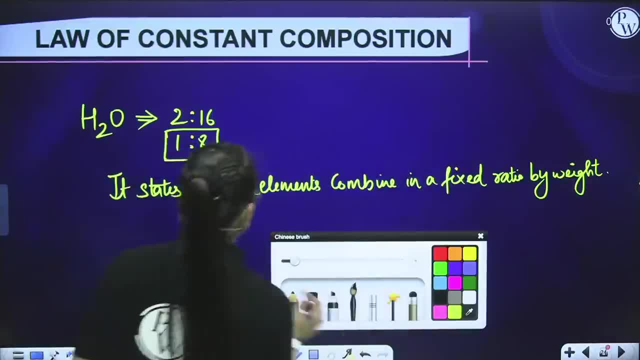 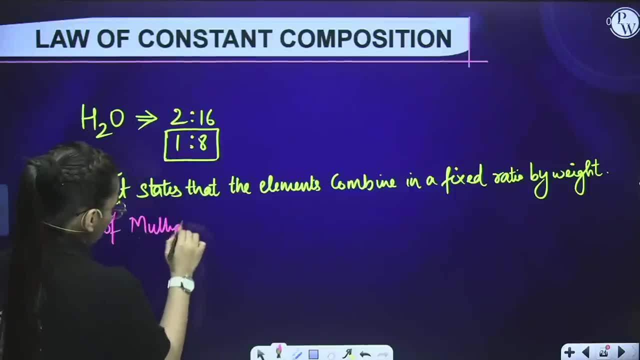 law of constant proportion. Okay, we are going to do the next law that is, law of multiple proportions. the best way to deal with laws is students kindly understand the concept, like in this law, what we are observing. we are observing about the 2 elements concept: that 2 elements are combining with each other. 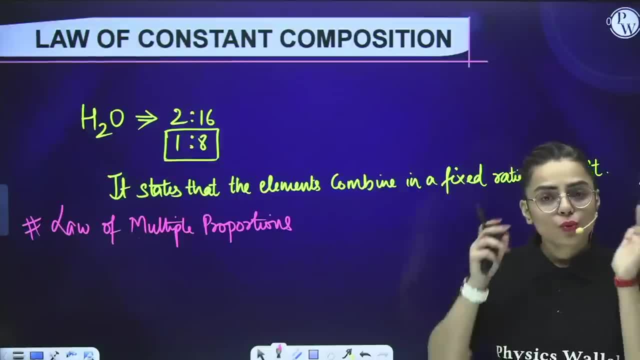 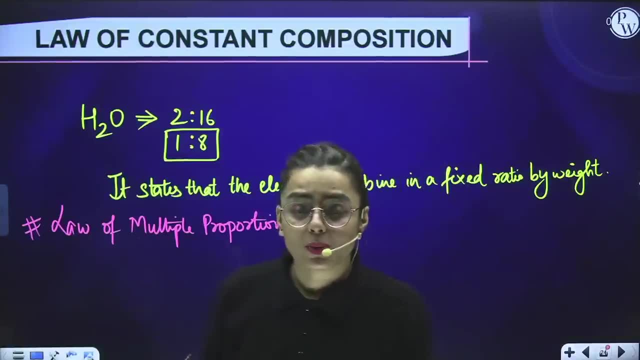 and they are present in the fixed, you know, ratio. so whenever you see the questions and there are the 3 compounds given to you, Kindly consider that those 3 compounds contain the same kind of elements so that you can identify that this is the kind of law of constant composition, because there will be the same. 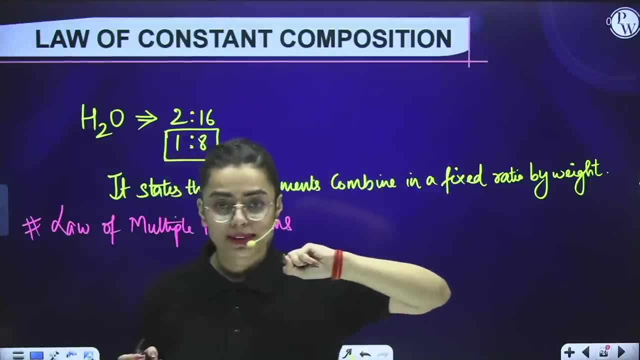 elements, then only there will be the fixed ratio of these elements, right? so when you come across the law of multiple proportion, kindly consider this: that there will be at least 3 elements in this situation, 3 different elements in this situation. so in the case, 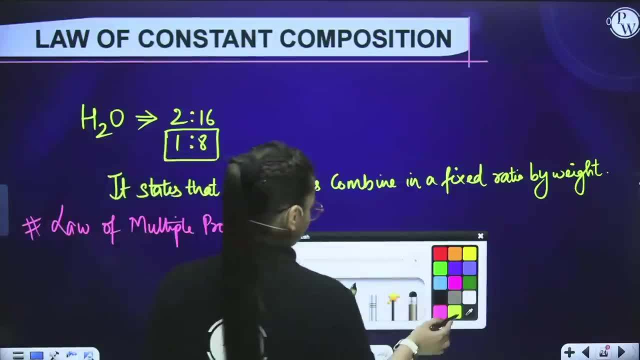 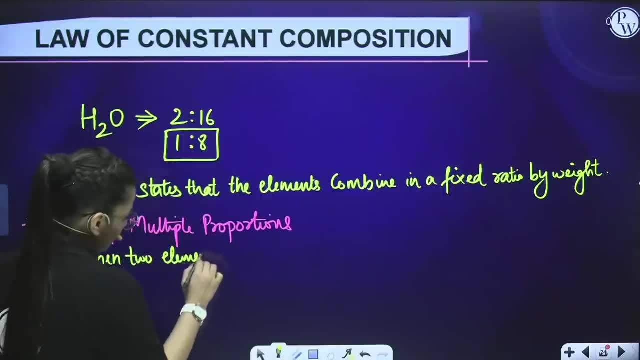 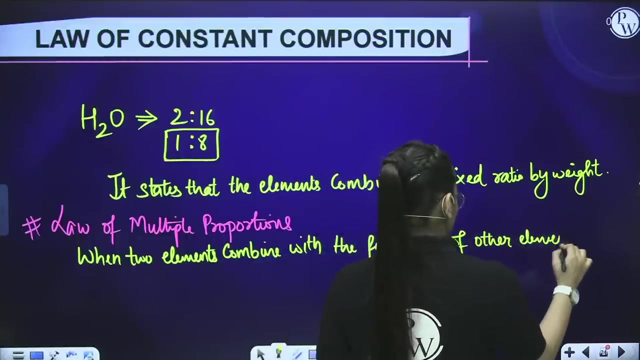 of law of multiple proportion. what we say? that when 2 elements, the 3 elements, are combined with, when 2 elements combined with the fixed- you know the fixed mass of the other element, they are present in the fixed ratio of the other elements. 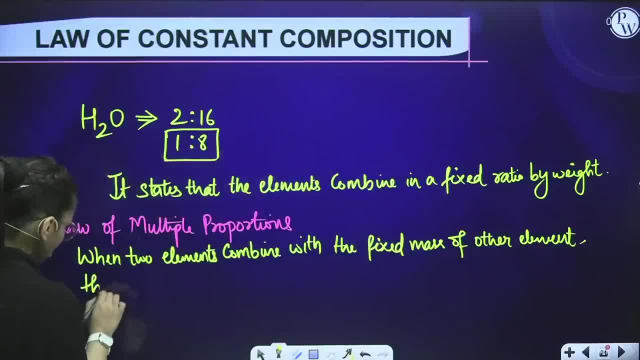 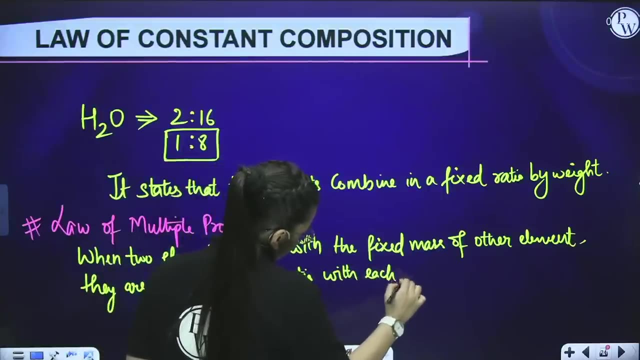 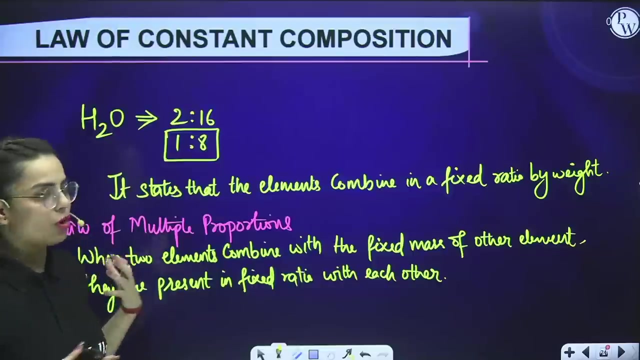 Okay, Okay, Okay. If the 3 elements are combined with each other, the 3 elements of the other element will remain fixed, fixed ratio with each other. Okay, To understand this in a very better form, I would take an example of law of multiple proportion. 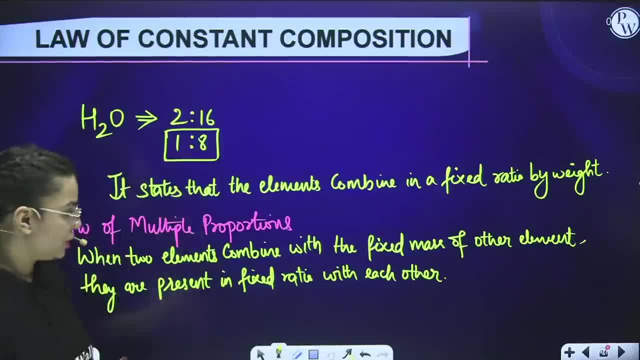 if I say that of carbon dioxide and carbon monoxide, I am taking 2 examples. it is like carbon dioxide and carbon monoxide and the two ones which I am talking about. I am having a different approach to it, right, and this is okay. 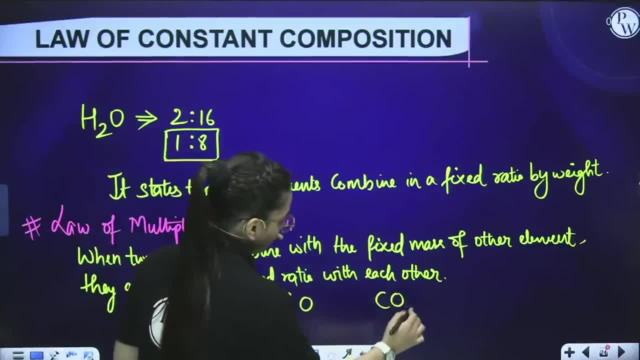 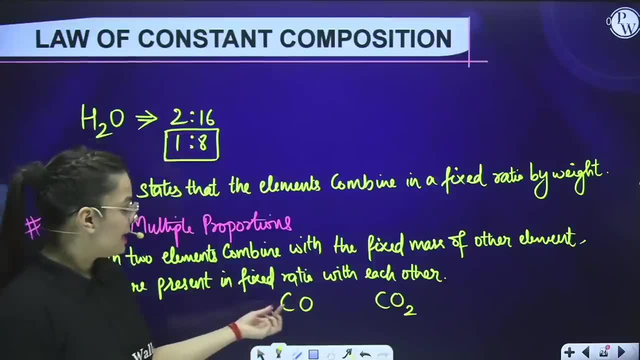 carbon dioxide and carbon monoxide. so what i am observing is this: when two elements combine with the fixed mass of other elements, like in carbon oxygen, here one element, like if i am taking off carbon carbon is in one part, oxygen is in one part, while if i take in this, carbon is in. 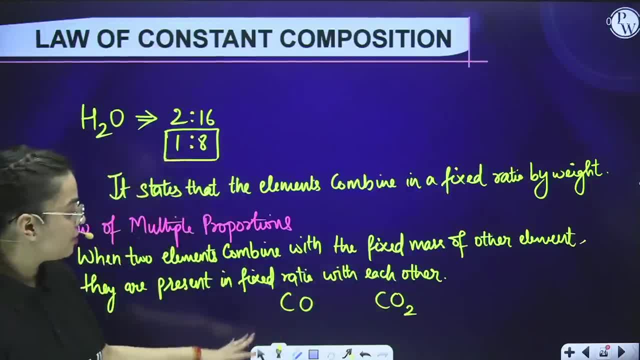 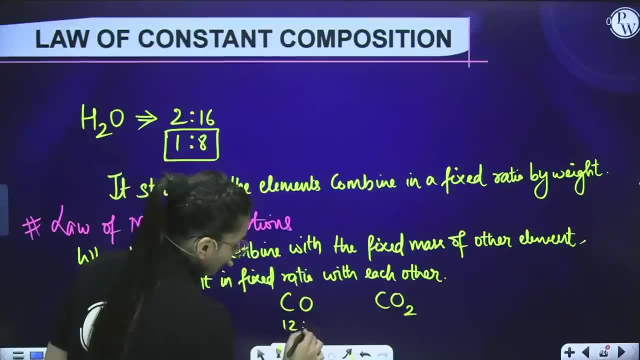 one part, while oxygen has two parts. so in this case, carbon monoxide, co, we observe that the ratio of carbon to oxygen is going to be 12 ratio 16, while if i take off co2, what i observe is the ratio is going to be 12 ratio 32. why 32? because one oxygen has a mass of 16 and two oxygen will. 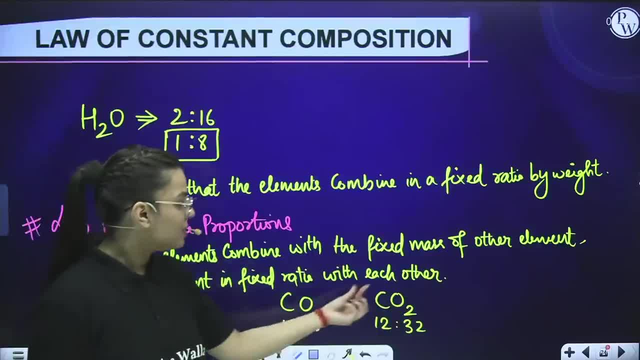 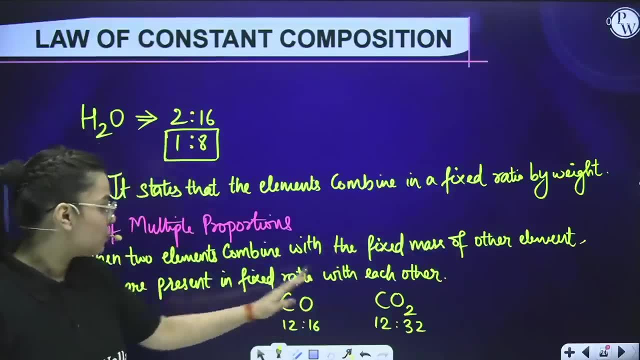 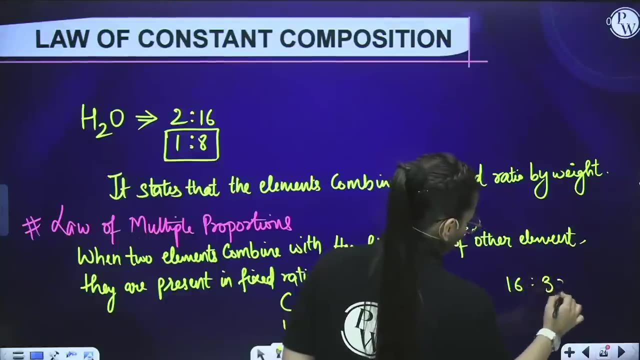 have a mass of 32. so what i observe is one element has a fixed mass, the fixed mass. one element has the fixed mass, while the other elements will be present in fixed ratio with each other. hence, the oxygen's ratio will be 16 ratio 32. o ratio o2 will be 16 ratio 32, which is one ratio 2. so it is a fixed ratio. what we, i am 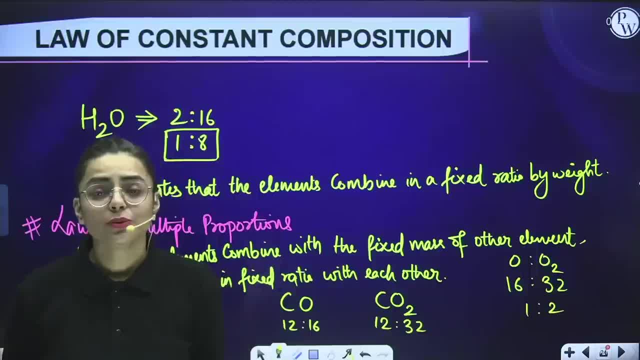 what i am trying to convey to you, that whenever you are looking to the law of multiple proportion, you will see that there will be elements like in both of these elements: one element will have a fixed mass and that will be combining with the other element and that other element will have 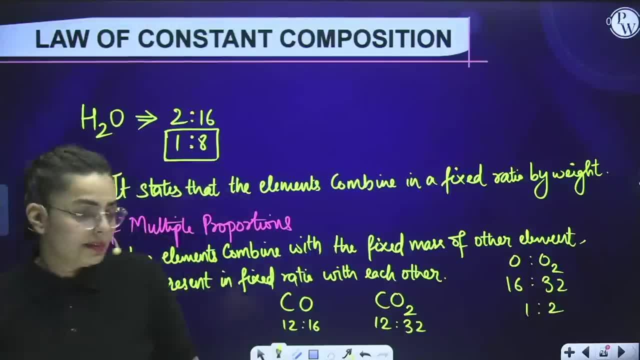 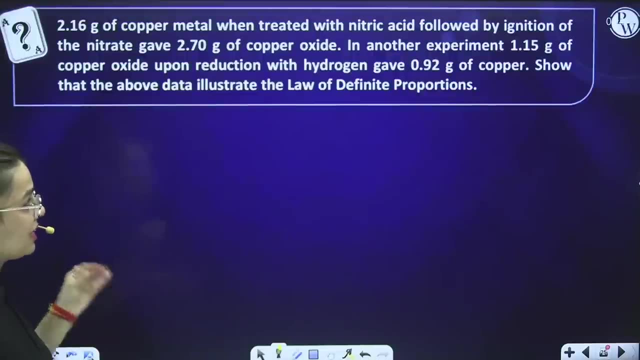 the fixed ratio with the compound of the other element, like in this. this oxygen will have fixed ratio with this o2, which is going to be one ratio 2. so this is the example of law of multiple proportion. now let us take an example over this: 2.16 grams of copper metal when treated with nitric acid, followed by 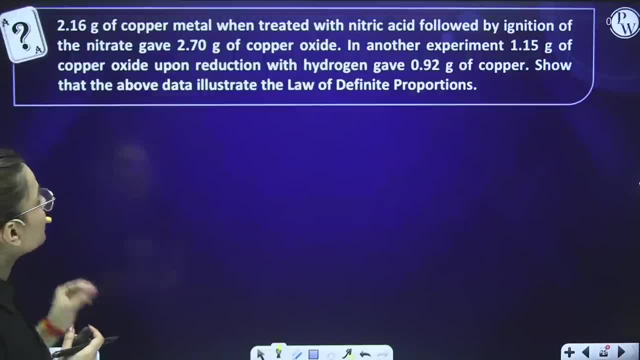 ignition of the nitrate gave 2.70 gram of copper oxide. in another experiment, 1.15 gram of copper oxide upon reduction with hydrogen gave 0.90 grams of copper. so that the above data illustrate the law of definite proportions. so, students now 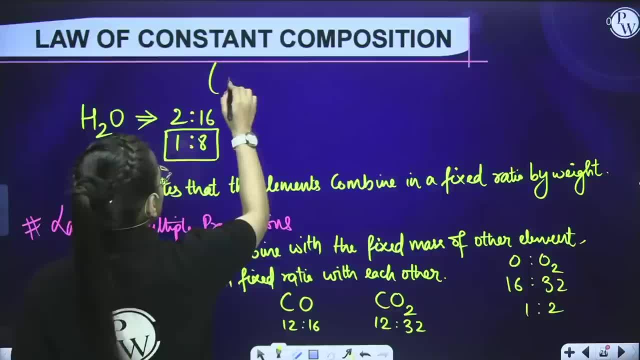 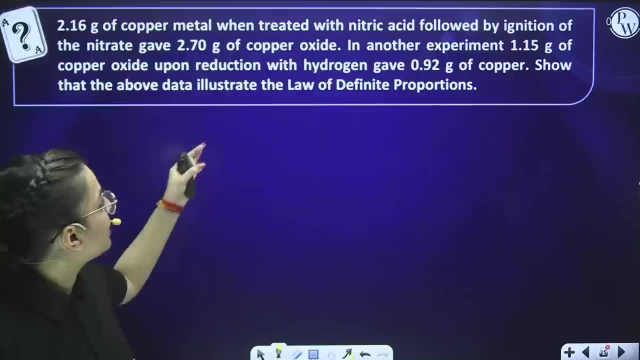 only, we have studied the law of constant proportion, which are also known as law of definite proportions or definite composition. so don't get confused. what is law of definite proportions? it is still the same. now, what we are going to do is, as i have already told you in this case, what it tells us: that there will be always a fixed ratio. 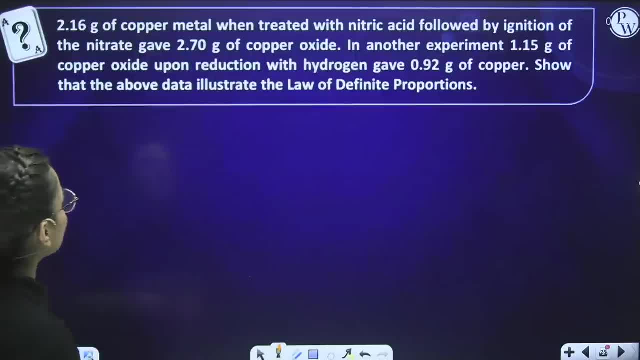 by weight. so we are going to find that only now. taking the example 2.16 gram of copper metal: 2.16 gram of copper metal, you know it is treated with nitric acid, followed by ignition of the nitrate, which is producing 2.70 gram of copper oxide, like 2.16 gram of co is producing 2.70 gram. 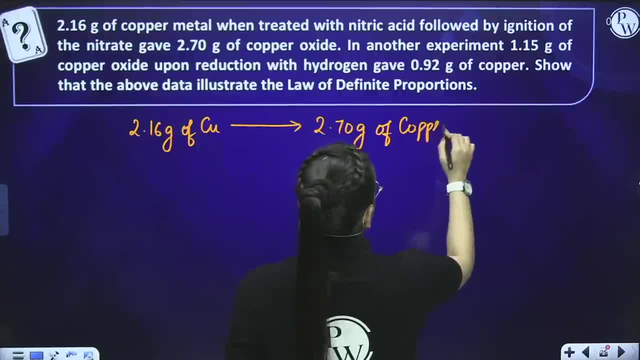 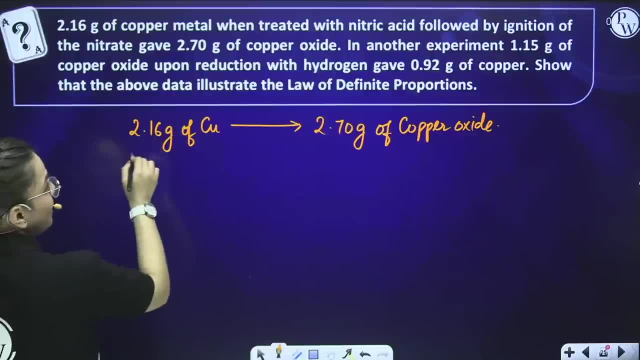 of copper oxide clear in another experiment. what is going to happen, students? in another experiment, zero pointer. do it. in other experiment: 1.15 grams of copper oxide upon reduction with hydrogen gave 0.92 grams of copper. kindly consider this in the next one, in the next situation experiment. 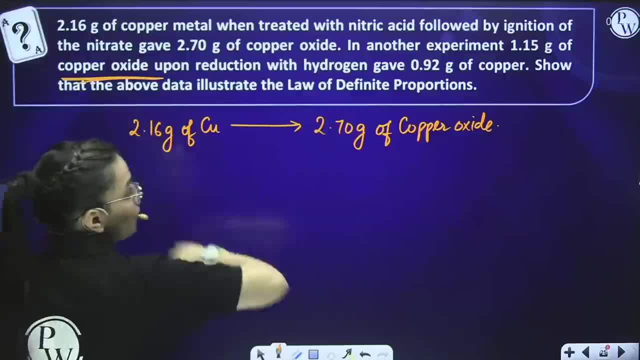 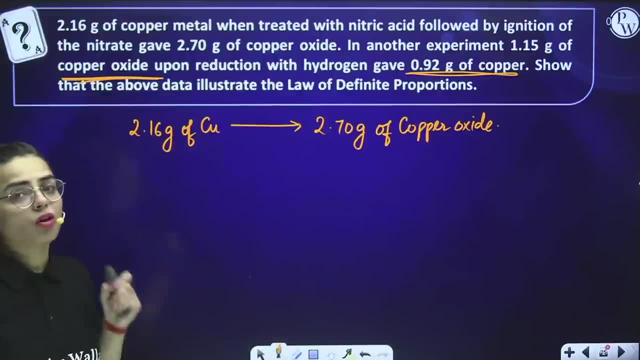 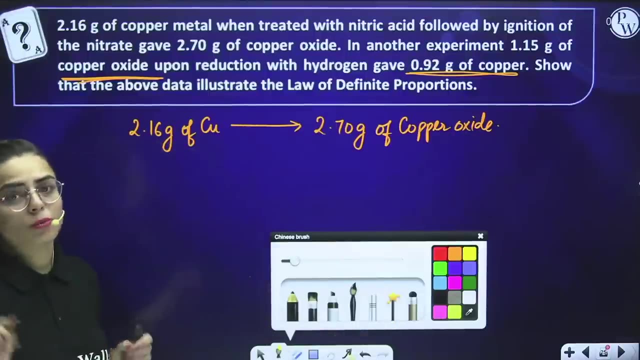 what we are seeing, that this much copper oxide on reduction with hydrogen is giving us this much copper. so we need to show that this data is following the law of definite proportion. how can we explain them? we will find the percentage of copper and oxygen in copper oxide. so, first of 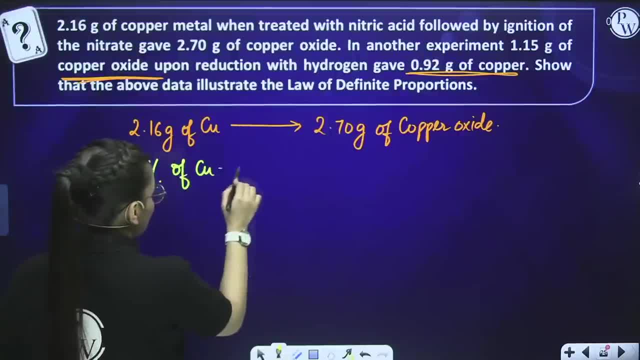 all, i will find the percentage of cu in copper oxide. so what i am going to do: the mass of cu which is given to me, divided by the total mass of the substance, that is, the copper oxide, into 100- so it is 2.16- divided by 2.70 into it is going to be 100. in this way, students, we are going to calculate. 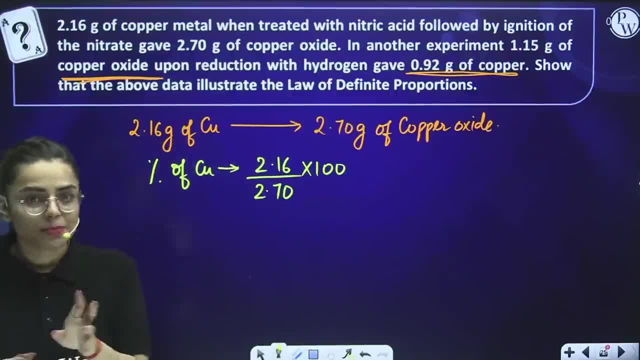 such situation and we are going to get 80 percent here right when you are going to solve this. it is about 80 percent. so what we have found, that cu percentage in copper oxide in the experiment one- i am talking about experiment one- in experiment one it is 80 percent. so the left over percentages: 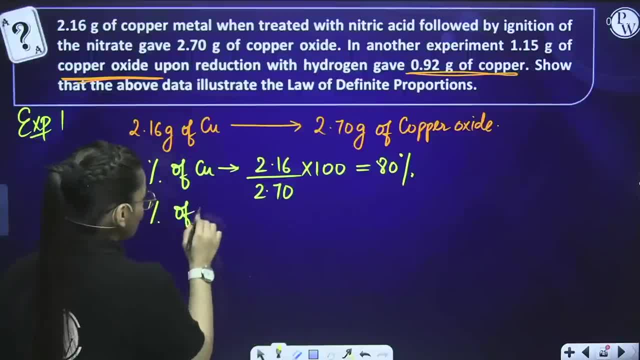 of oxygen, right? so percentage of oxygen is 80 percent. so the left over percentages of oxygen. so percentage of oxygen in copper oxide in experiment one it is going to be 20 percent right now. let us see the next case, the experiment two case. if i talk about experiment, 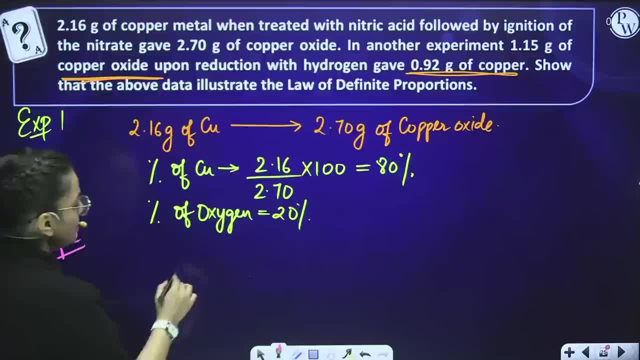 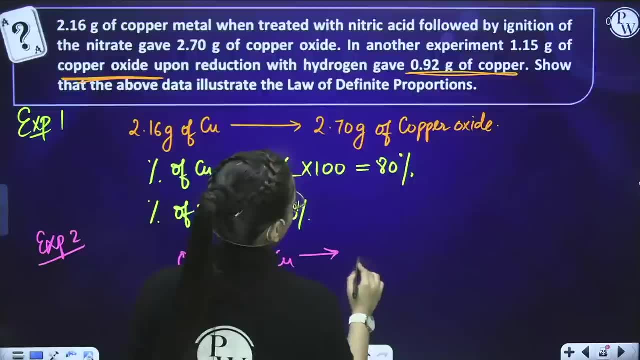 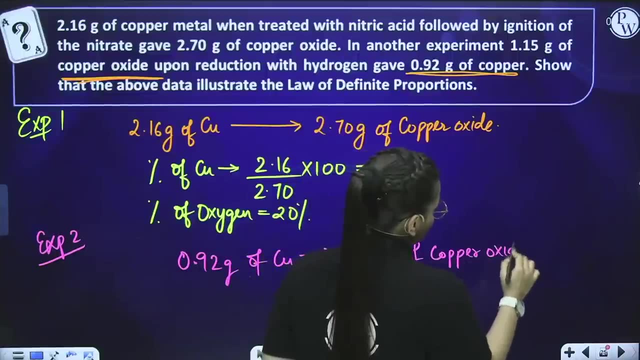 two students in experiment two: what it is given is 0.92 grams of copper is produced. from how much copper oxide? from 1.15 grams of copper oxide. so again, i'm going to find here the percentage of copper as well as of oxygen. so if i found the percentage of copper, what i need to do? 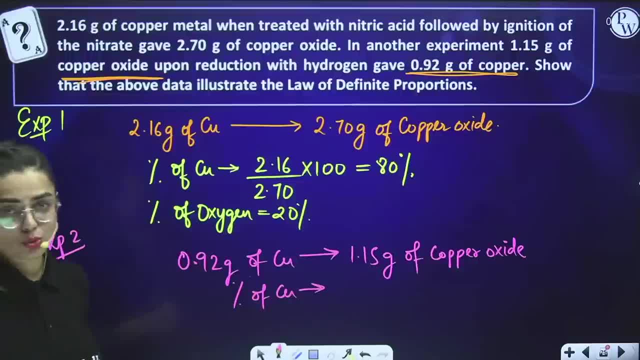 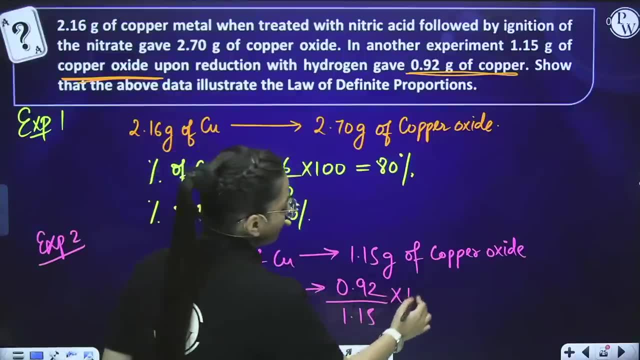 is. i need to write the mass of copper upon the mass, total mass into 100. same 0.92 divided by 1.15 into we'll do 100, because we need to find the percentage students. so when we calculate it, students, it is about 80 percent. okay, it is about 80 percent. so the leftover is oxygen. hence we can. 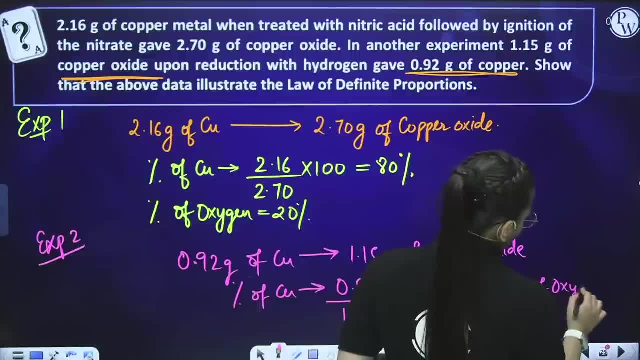 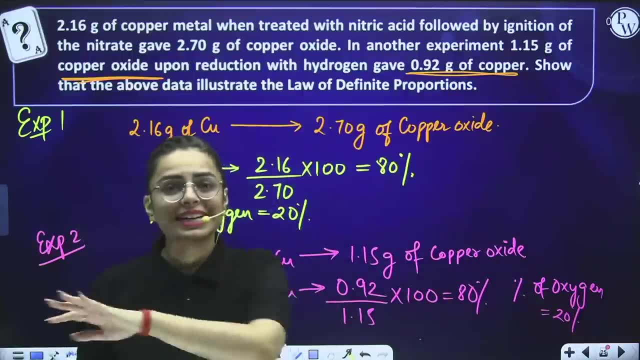 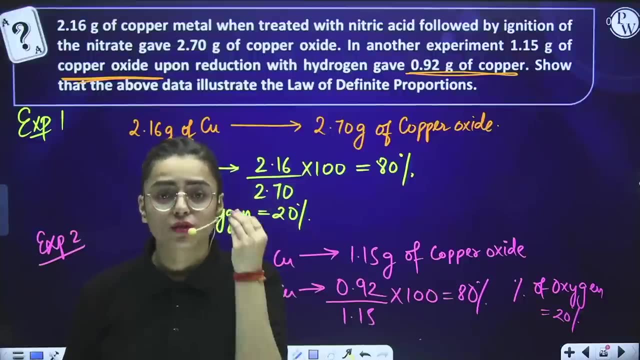 say that percentage of oxygen is 20 percent in experiment 2. so now tell me, as i already told you in the previous case, that water, in any area, in any aspect, will have the same, you know, the same fixed ratio of their masses, of their weight, wherever you go, wherever. 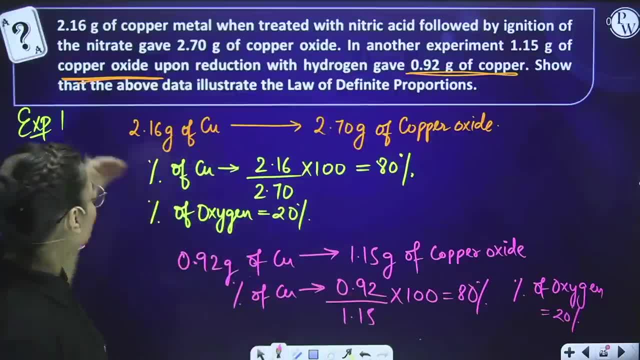 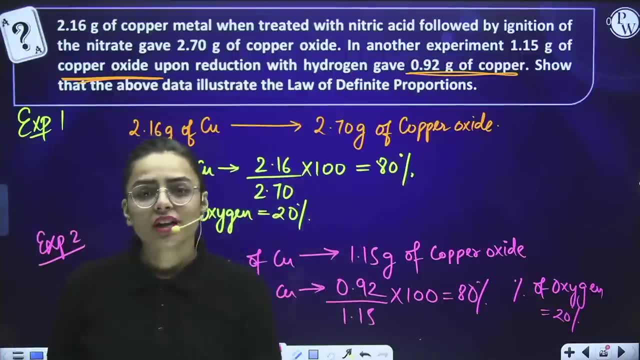 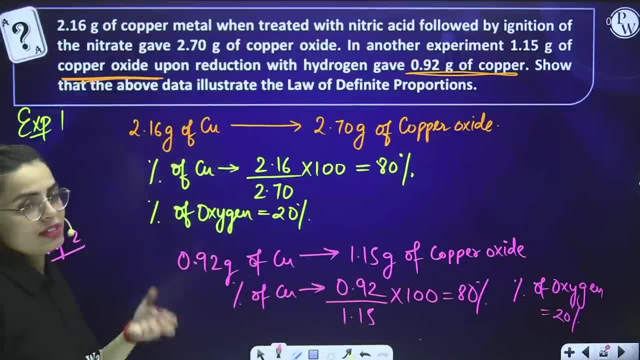 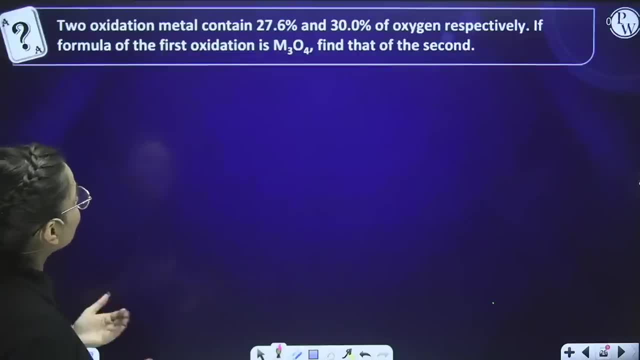 yes, it illustrates the law of definite proportions. clear. good, now, students, coming towards our next question. two oxidation metals contains 27.6 percent and 30 percent of oxygen respectively. if formula of the first oxidation is m3 o4, find the formula for the second one. so it is very. 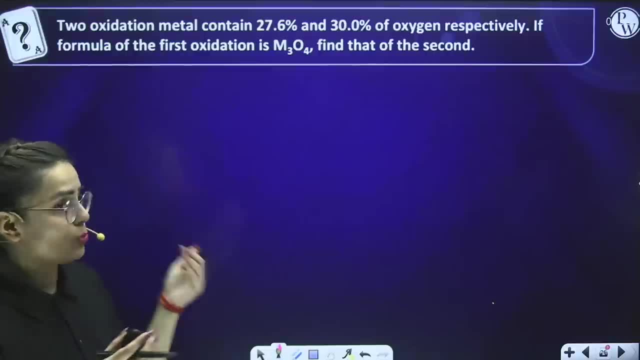 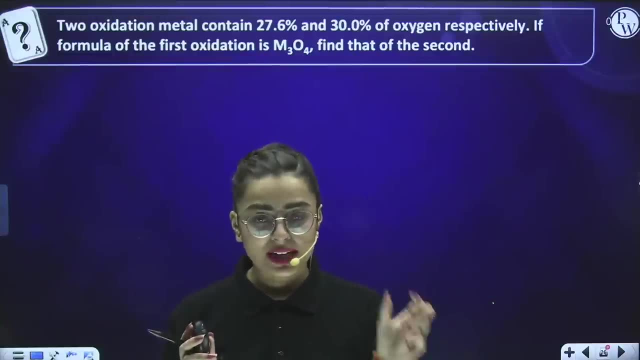 simply, it is given us that there are two situations in which metal is being reacted with the oxygen and it is forming metal oxides. there are two experiments, but for the first one we have been given the formula, but for the second one the formula is different, so we have to find the 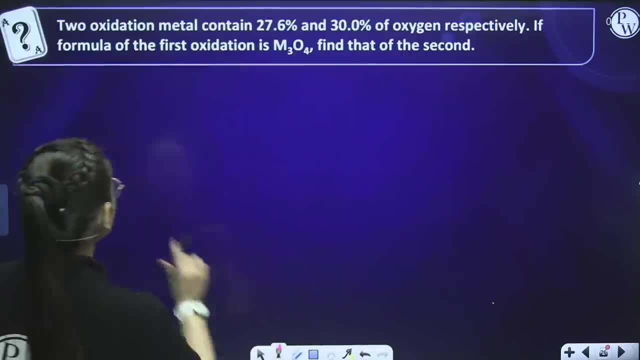 formula for the second one. so we have to find the formula for the second one, so we have to find the. so how can we calculate this? first of all, write the experiment one or the situation one in the experiment one. what we observe is the formula has given us, which is m3 o4, right m3 o4, and we have 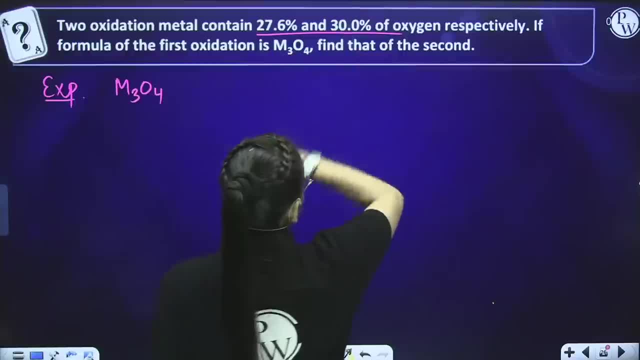 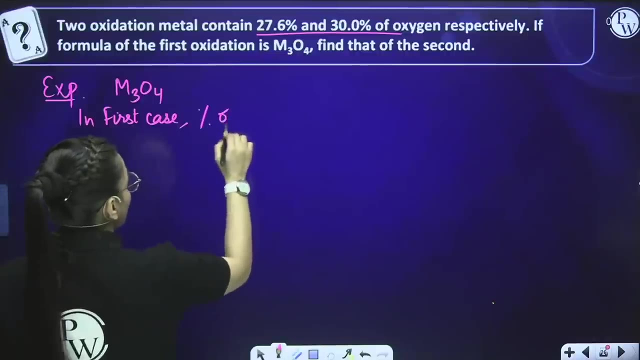 already been given the percentages of oxygen. in both the cases, like in the first case, they case they are saying 27.6 percent of oxygen is present in the first one. in first case, percentage of oxygen is 27.6 percent. now, students, please just just tell me that m3, o4 and the 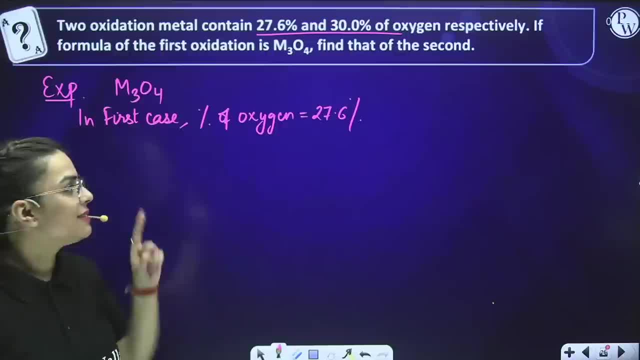 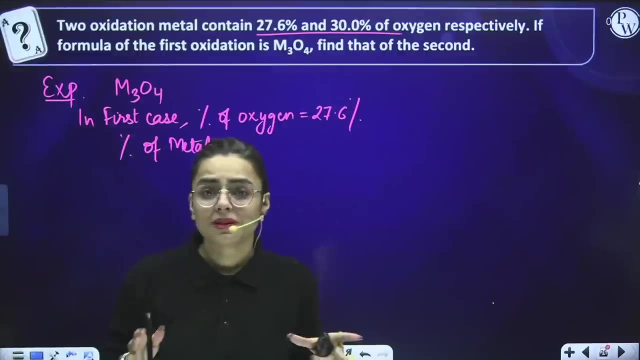 percentage of oxygen is 27.4, we can say that. how many oxygen atoms are present here? four oxygen atoms are present there, but before that, tell me the percentage of metal here. how can you calculate? look, whenever such questions arises, always consider that the total percentage is 100. hence, if oxygen is present 27.6 percent, what will be the? 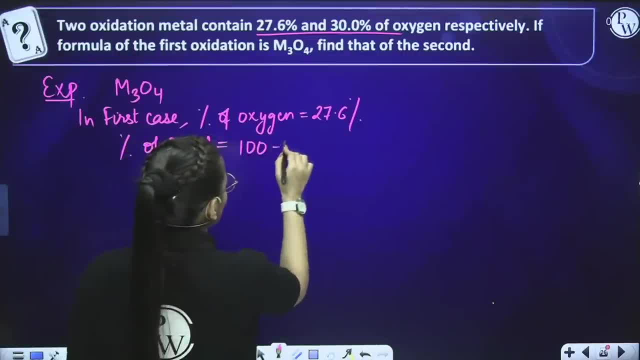 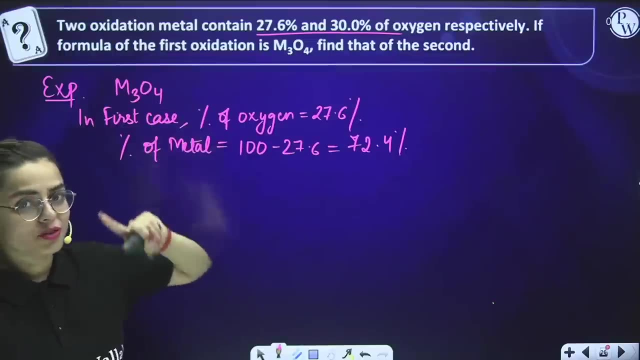 metal: 100 minus 100 minus 27.6 percent, it is going to be 72.4 percent. my dear students, it is going to be 72.4 percent. now we have calculated the percentage in the first case, where we have been given the formula right now, what we are going to do. 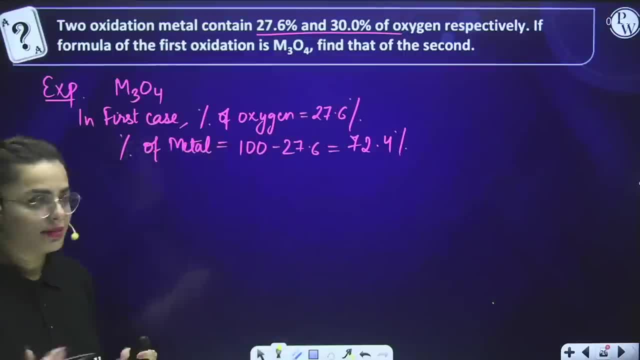 we are going to do? we are going to write the second case right in the second case, in the second experiment. what information i've got? i don't have the formula, but i know that percentage of oxygen is 30 percent, right? so the percentage of oxygen in the second case is 30 percent. so the other portion. 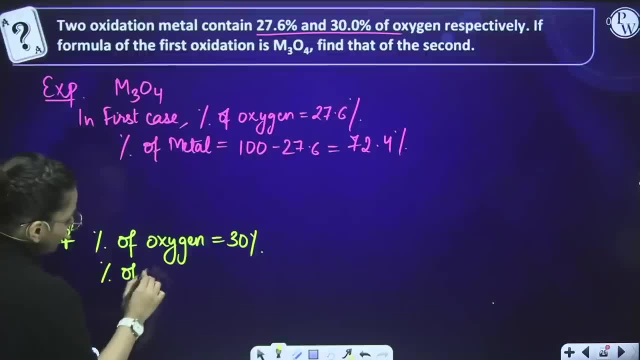 obviously will be the metal right. so i would say that percentage of metal would be 100 minus 30, hence it will be 70 percent. now, in both these cases, we have already calculated the percentage of metal. now what will be the other next step? in the next step, we will observe that here four parts of oxygen. 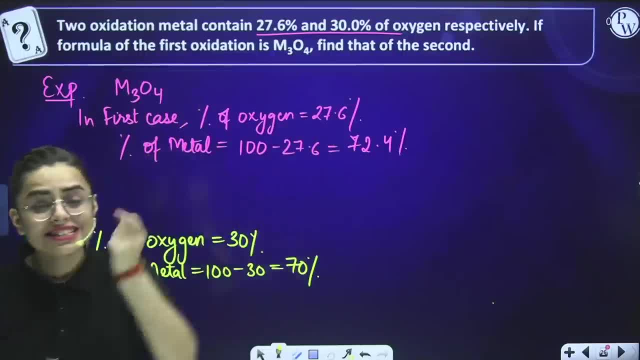 you know, have percentage 27.6 right. so how much, i would say, oxygen will be present? for the next case, we need to calculate it. it is little bit of mathematics you can consider, but don't get confused by step i am going to explain you. first of all, i am going to explain you about the metal m. 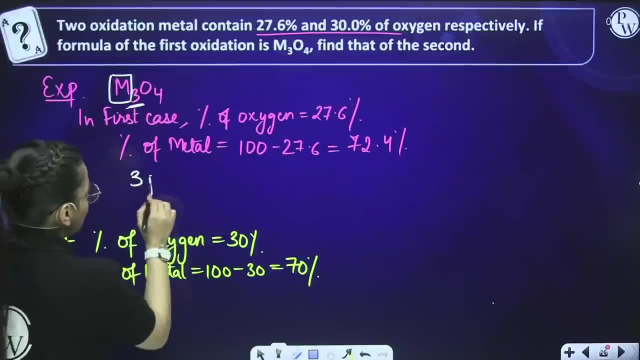 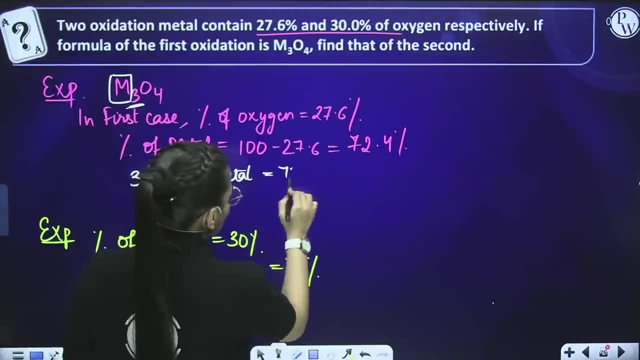 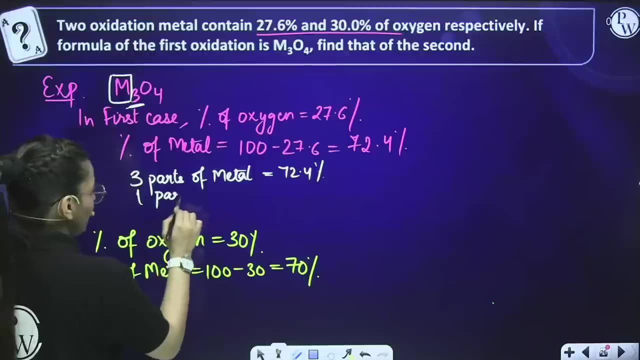 see three parts. these are three. three parts of metal gives 72.4 percent of metal. right, you know this thing. now, if i say one part of metal will give how much, one part of metal will give you how much. this you need to carry, this you need to calculate. 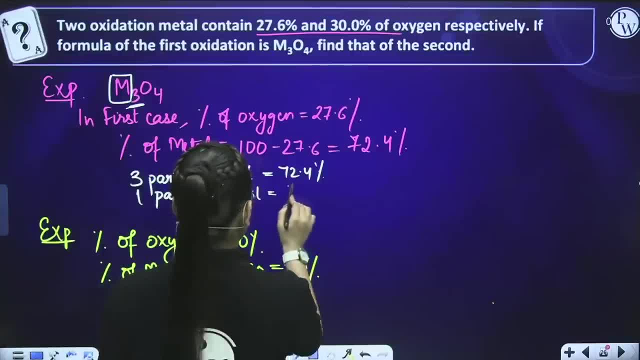 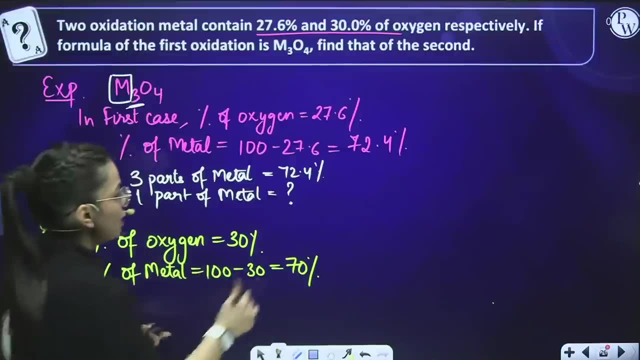 so, in other words, we need to calculate the percentage of oxygen in the second case, but it has already told us that the percentage of metal is 70 percent in the another case. so we have been given 70 percent is already present. we don't know how many parts of this metal will be formed. 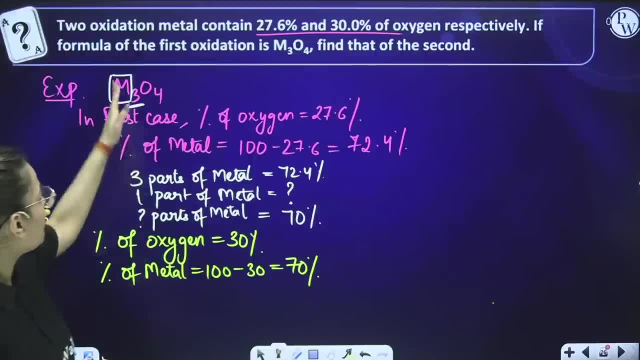 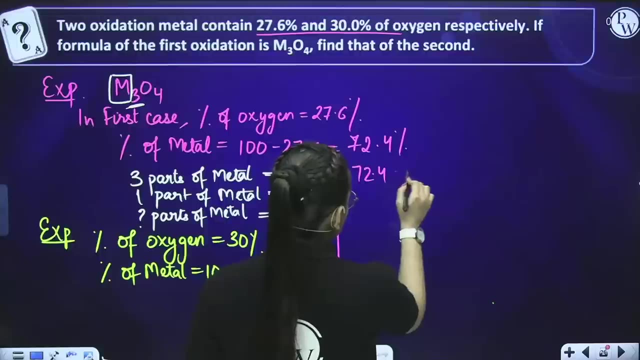 we don't know this situation. we just only know that three parts are giving us seventy two point four percent. so how many parts will be formed when seventy percent is there? in short, reverse the situation. to do this question, it will be easy for you. i would say: 72 percent is present in three. 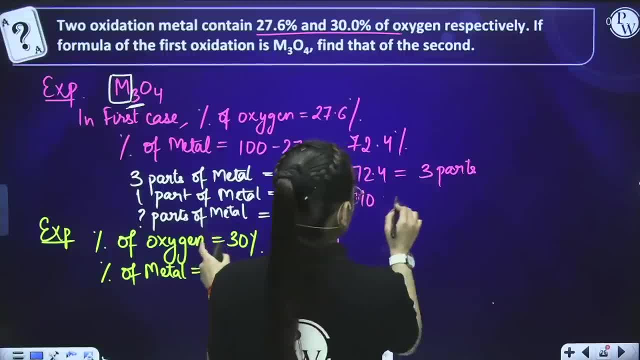 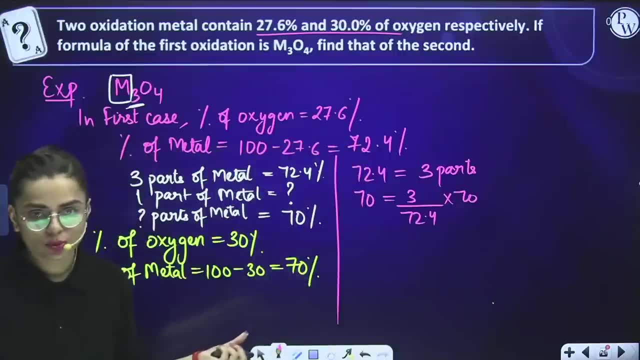 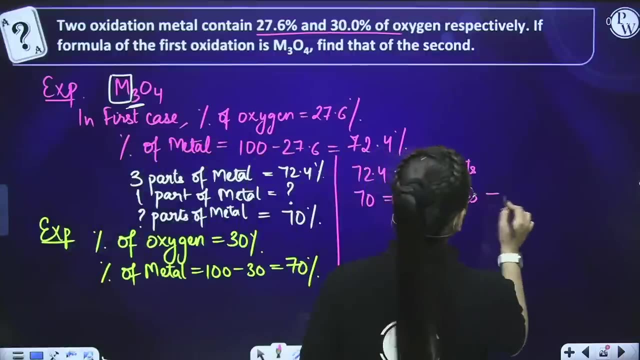 parts. so in 70 percent, how many parts will be present? it will be 3 by 72.4 into 70. like this you can do the question first of all: write the situation, understand the situation, what they are going to tell you. so whenever you will solve the students, it will be um approximately 2.90 something. 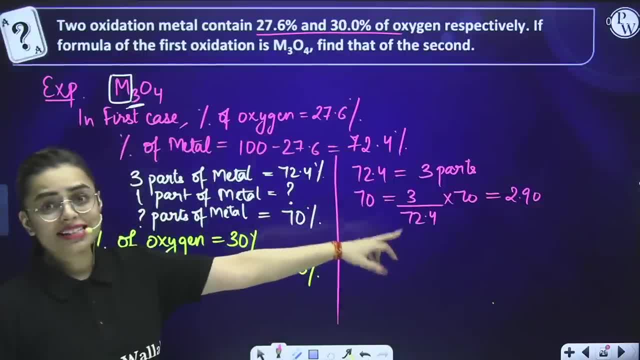 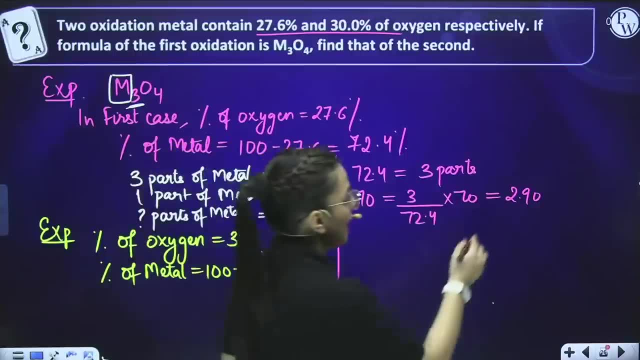 it will be approximately this much. now. what is this? these are the parts of metal that rises. here are three parts. now you have already found how many parts are there. how many parts are there of metal? 2.90 parts of metal in case two. similarly, we are going to calculate for the oxygen part. 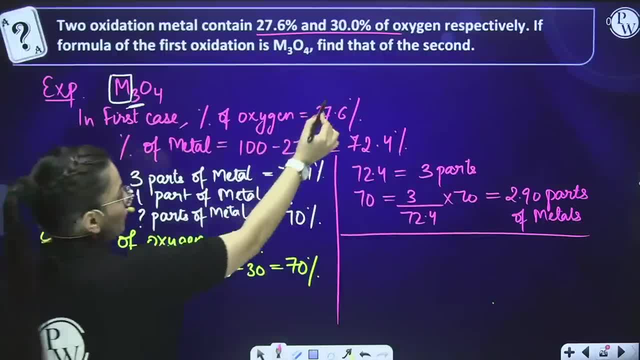 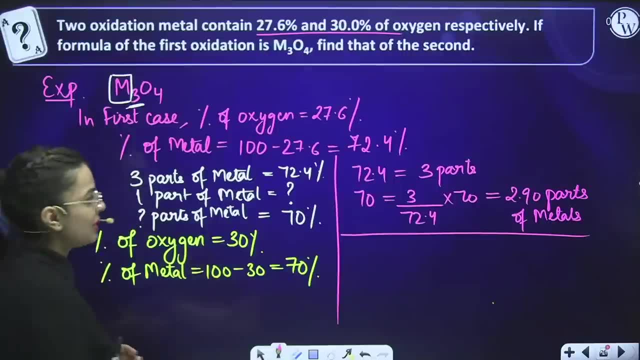 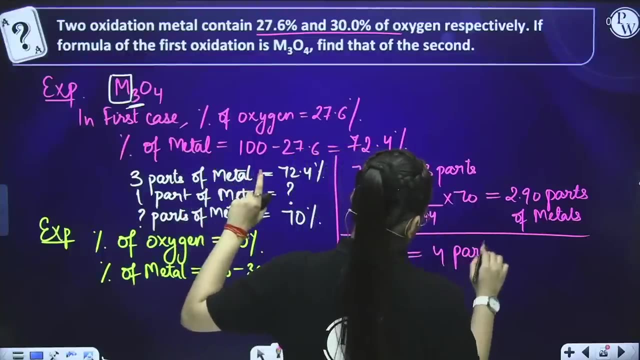 now see again. i am telling you here the percentage is given 27.6 percent. 27.6 percent gives four parts. so how many will 30 percent give? same thing arises. i am saying: 27.6 percent gives us four parts. right now i am telling you: 70 will give 4 by 27.6. 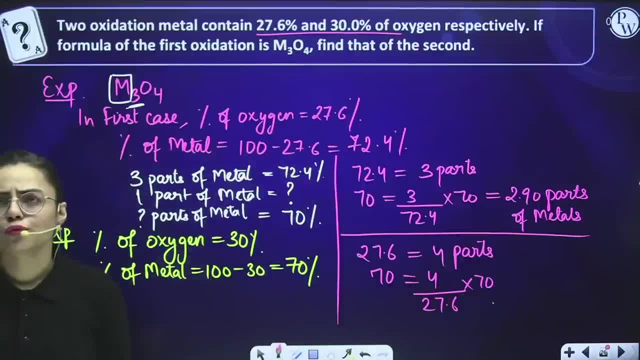 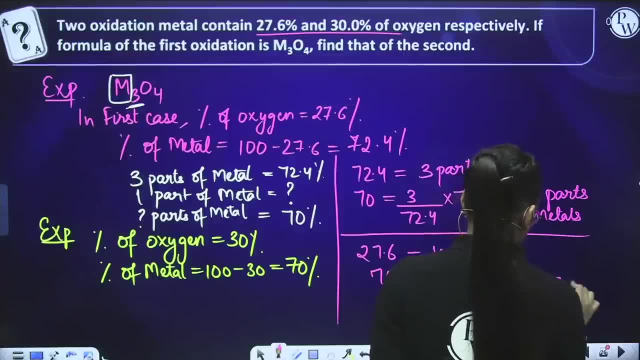 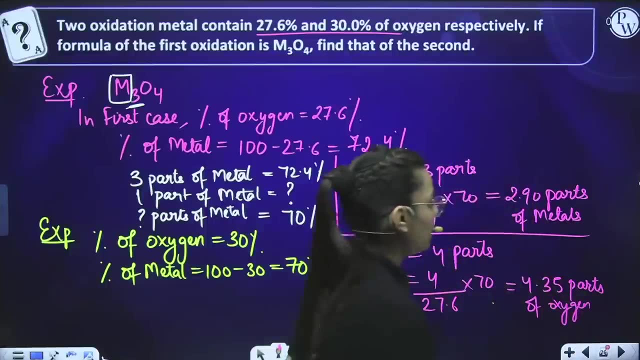 into 70, my dear students, it will be about 4.3, three, five, four point three. five. parts of oxygen. okay, now, we have already calculated the parts of oxygen as well as the parts of metal. now, as you know, we do the ratio forms. so we are going. 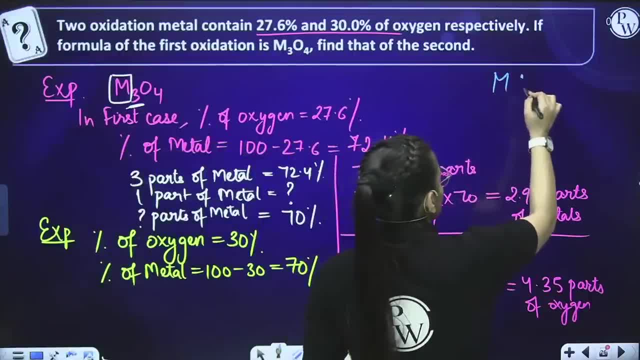 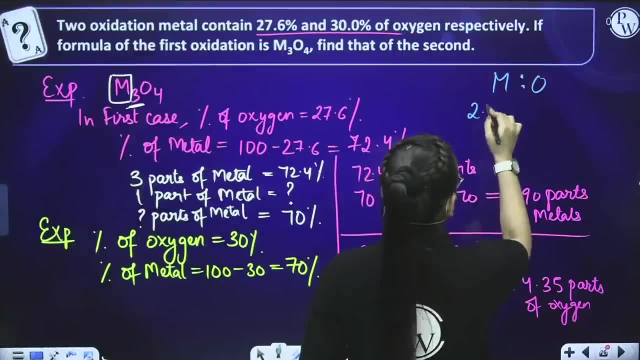 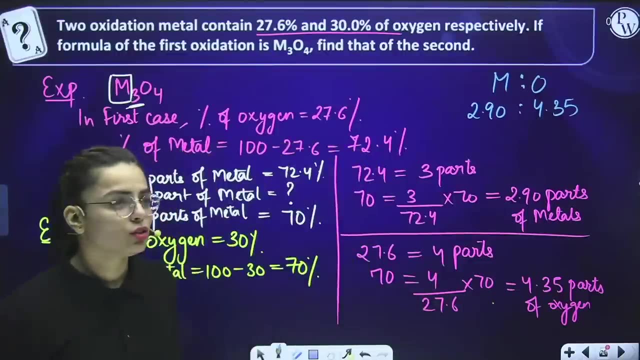 to write it here: metal ratio- oxygen. for the second case now, firstly, you need to write for the metal. for the metal, we have calculated 2.90. for oxygen, we have calculated 4.35. my dear students, it is going to be near about one ratio, i would say 1.5 approximately. 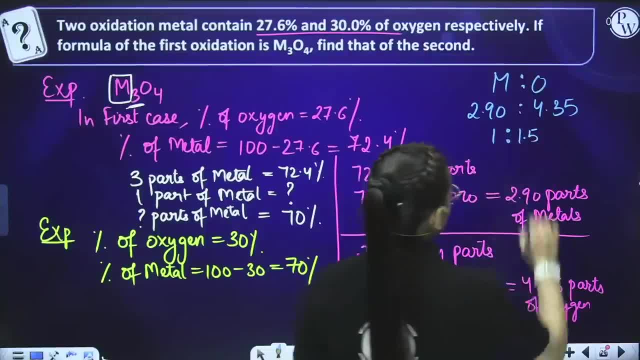 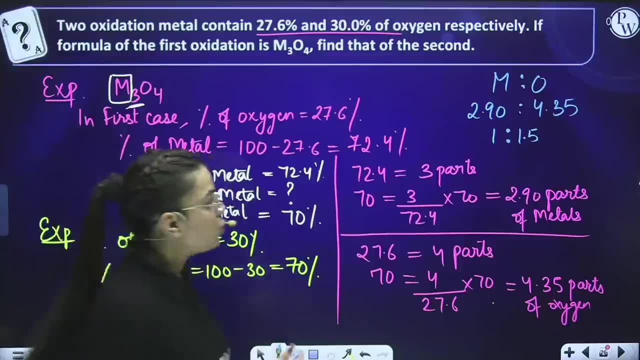 2.. yes, one ratio, one point. so, in short, whenever we get it in decimals, we try to convert it into a fixed number so that it is easy for us. so to convert 1.5 into a number, i would say: just multiply with 2 that. 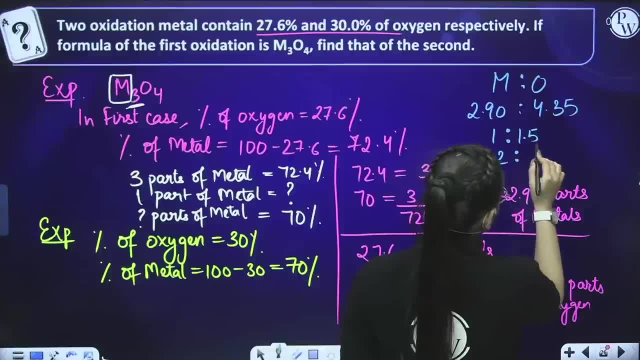 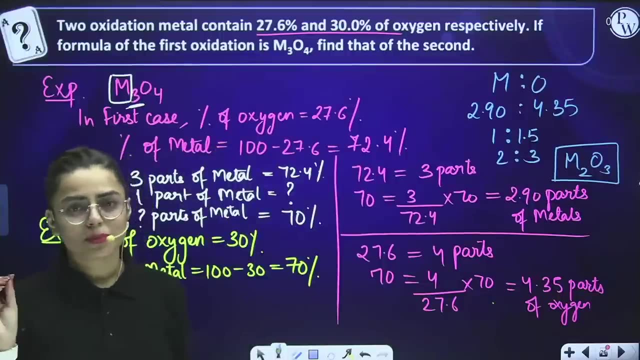 would be easy for you. so if you multiply with 2, it will be 2 ratio, three students. hence what will be the formula: m base 2, oxygen base 3. so the formula that is obtained for the second part is is M203. it is clear to you. it is very simplest question, but it the students get confused. 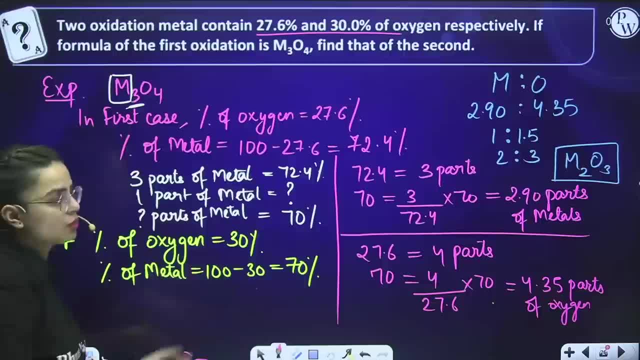 in this confused in this question, like in this part of the question. so you need to understand first right situation in such a way and find out what you need to calculate. you need to calculate the parts. so kindly convert this in this form. it is a simple basic mathematics. 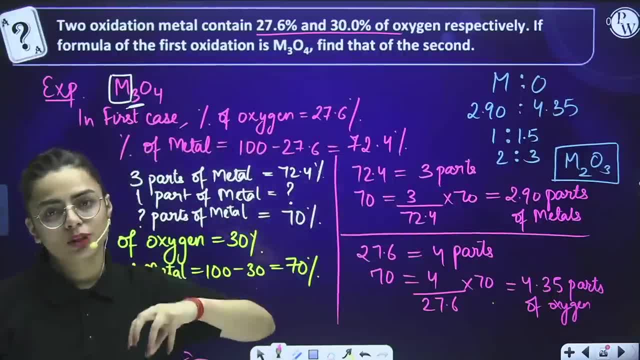 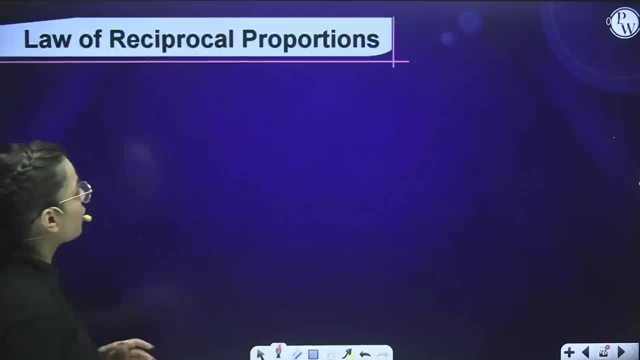 so that it will be easy for you to calculate the formula and formulate it right. so through this question we can elaborate and calculate different questions. now moving forward towards the next law, that is, the law of reciprocal proportions. students, law of reciprocal proportions states between the three elements, like if I say there is carbon, there is Hydrogen there. 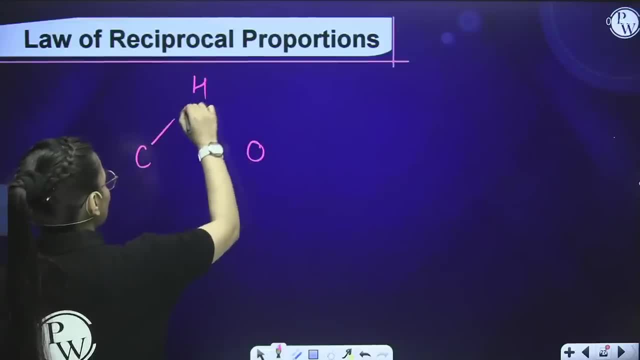 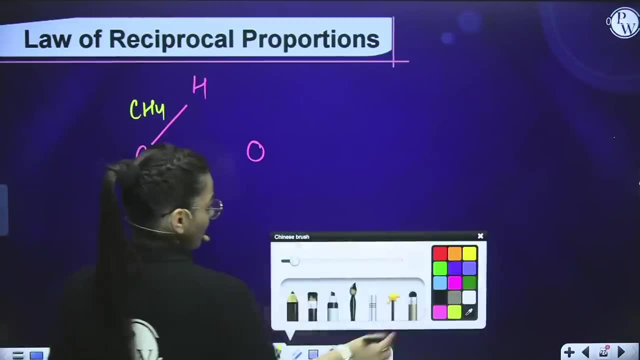 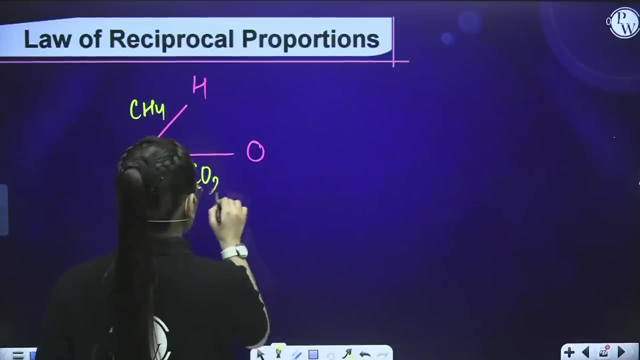 is oxygen. what happens is carbon forms bond with Hydrogen and forms a compound which is CH4. then I see a case where carbon forms a compound and forms a compound which is CH4. carbon forms bond with oxygen and the compound that is formed formed is co2. in the next case, 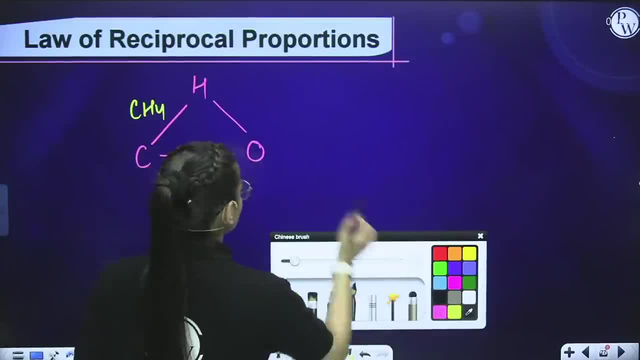 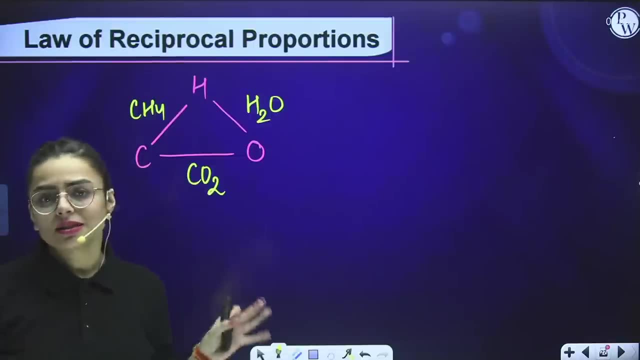 students. hydrogen oxygen also combines with each other, forming water. so what is the law of reciprocal proportion? it stays- states us that when two elements consider any two elements- for example, i am considering carbon and oxygen- when these two elements combine with the fixed mass of the third element of the third element means hydrogen. so first see what i am speaking. i am saying when 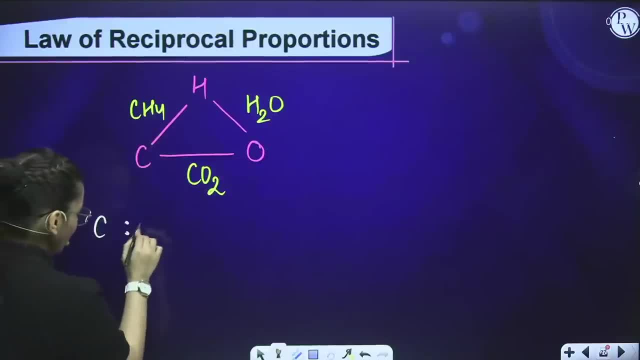 carbon combines with hydrogen, it forms a ch4. what will be their ratio? students: in ch4 it will be 12 ratio 4 right now. when oxygen combines with hydrogen. students: oxygen combines with hydrogens forming water: what will be their ratio? 16 right. ratio 2 right. we need to make one of the elements ratio constant. so i am making constant the ratio. 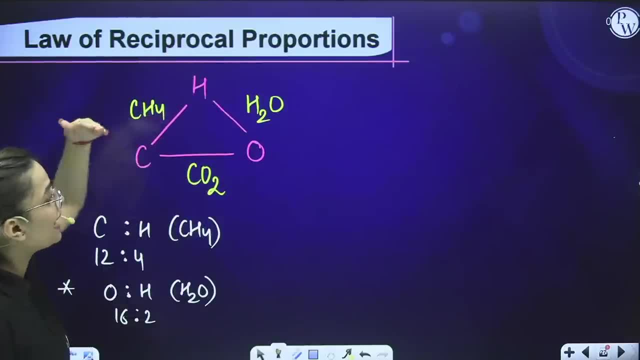 of hydrogen, because i am considering these two formulas. you can consider any of the formulas by taking one as a constant fixed ratio. i am taking hydrogens fixed ratio. so in this case, hydrogen is four parts. in this case, hydrogen is two parts. so what i am going to do is i am going 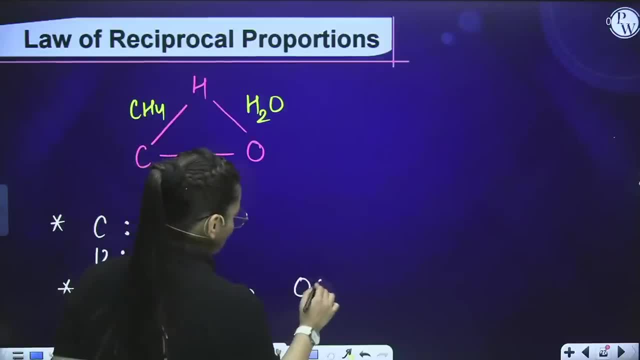 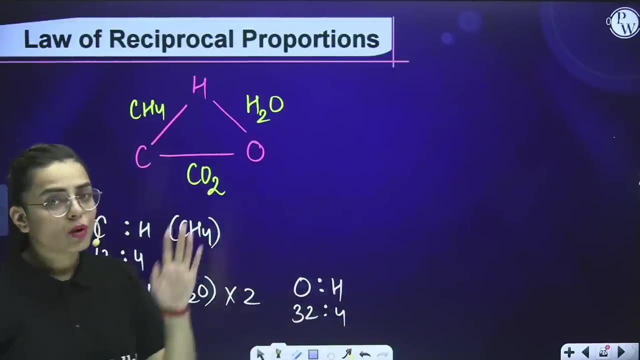 to multiply this with two. now what i am getting is oxygen ratio hydrogen. that means when it is multiplied with two, it is 32 ratio. for students clear now: the new ratio is 12 ratio 4 for ch4 and for water. after multiplying it with two, we are getting 32 ratio 4. what happens is the ratio of hydrogen is now fixed. so what we are 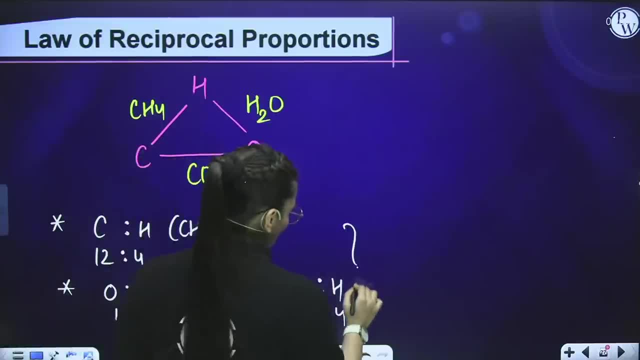 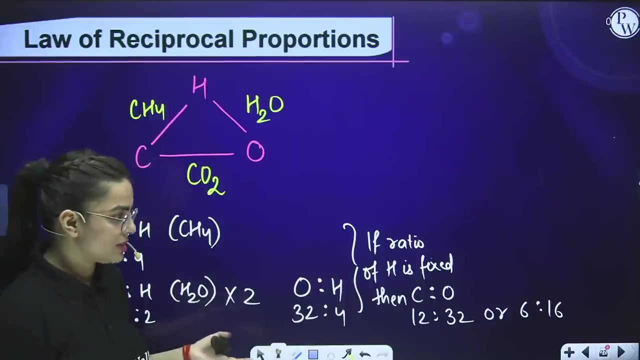 observing. we are observing that if the ratio of, if ratio of hydrogen is fixed, then then carbon oxygen ratio will be twelve, will be 12 ratio 32. clear, students, it is simplest, or i could say. or i could say, if i divide it on the table of 2, i would say: 6 ratio, it's 16. right, it is 6 ratio, 16 if i divide on the table of 2. 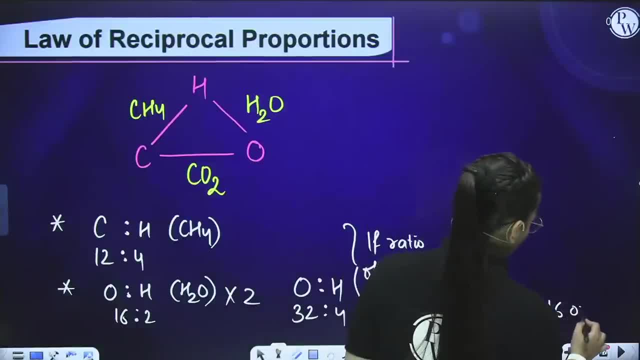 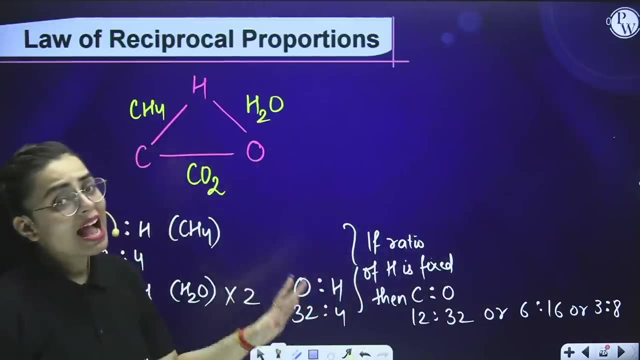 or if i further divide it on 2, it will come out to be 3 ratio 8. clear, simplest. okay now, students, i have found that after fixing the ratio of hydrogen, the ratio of carbon and oxygen is 3 ratio 8. now, uh, individually, what will be the ratio? let us calculate that individually. if i 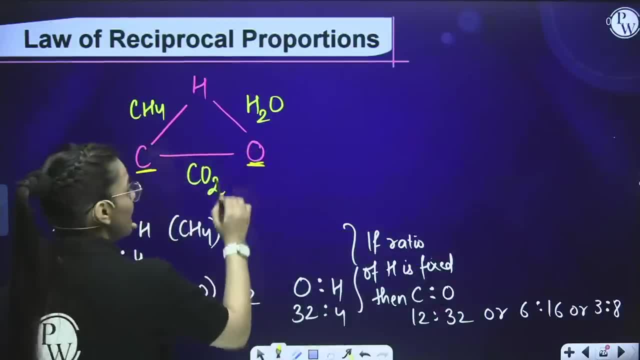 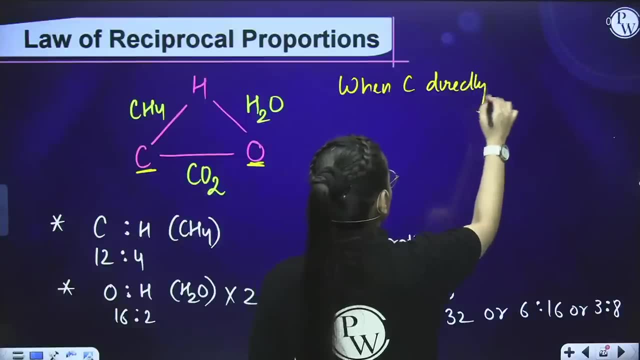 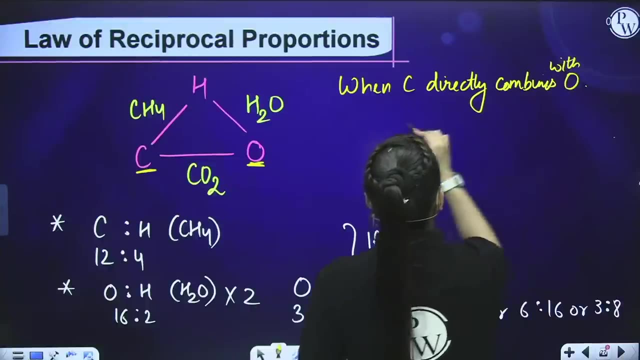 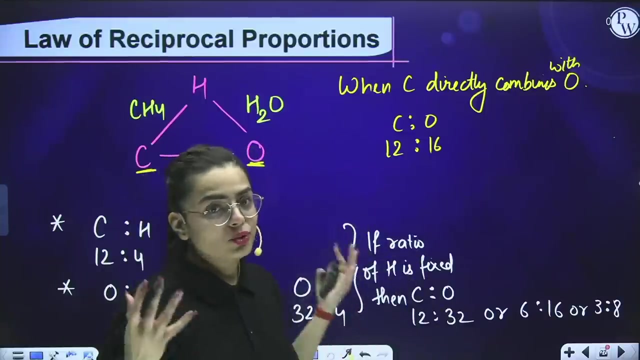 consider both of these cases: when carbon directly combines with oxygen, when carbon does not combine with oxygen, when carbon does not combine with oxygen, when carbon does not combine directly, combines directly, combines with oxygen. students, what we get? what the? what is the ratio? we get 12, ratio: 16. now i will again divide it on the. 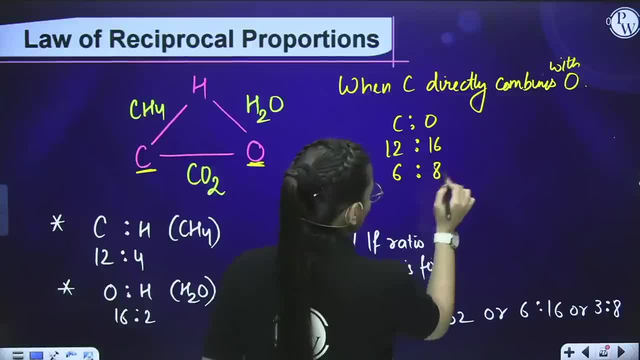 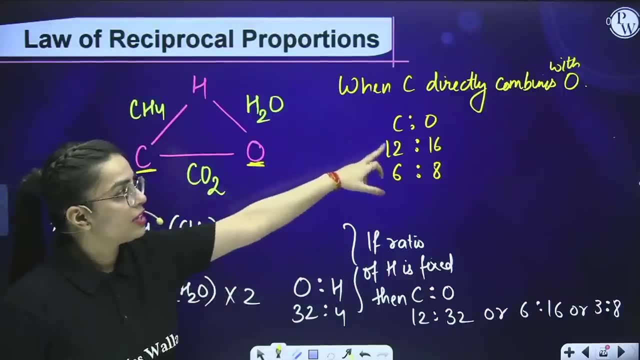 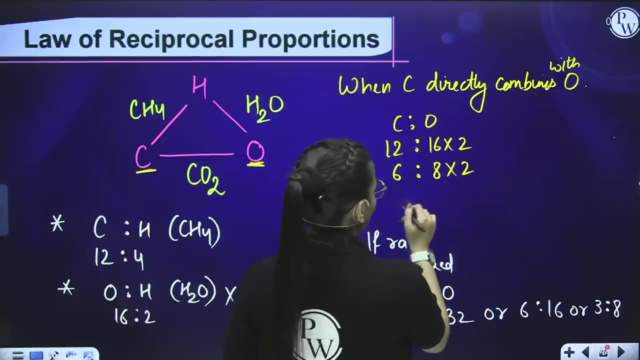 table of 2. what i am getting 6 ratio, i am getting 8. what i am getting here is 6 ratio 8. but please do remember the compound here formed is carbon dioxide, not carbon monoxide. so here it will be 16 into two, hence 2 into 8. or i would say again, if i cut it on the table of 3: 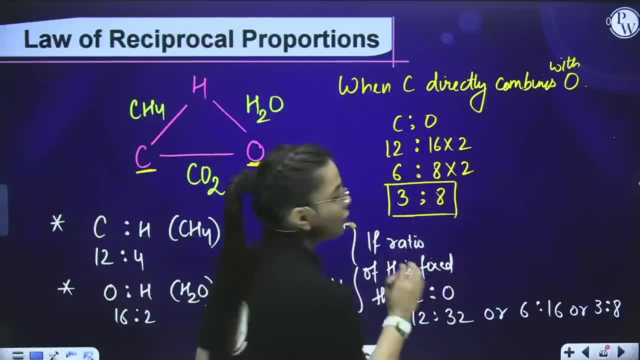 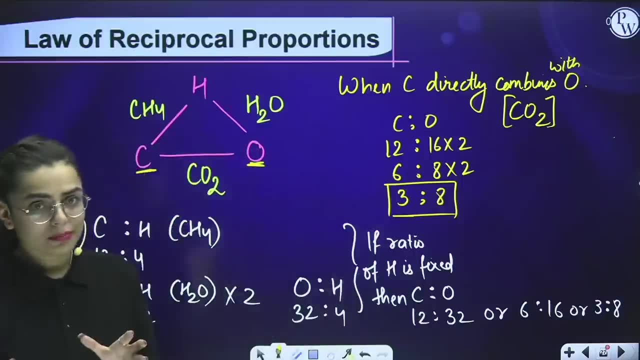 it is three ratio 8 on the table of two. sorry, it will be 3 ratio 8. here the formula is a co2, not co. here the formula is a co2, not co. so you have to remember in your minds the formulas. first formula is ch4. accordingly you will write the ratio. second formula is water. accordingly you. 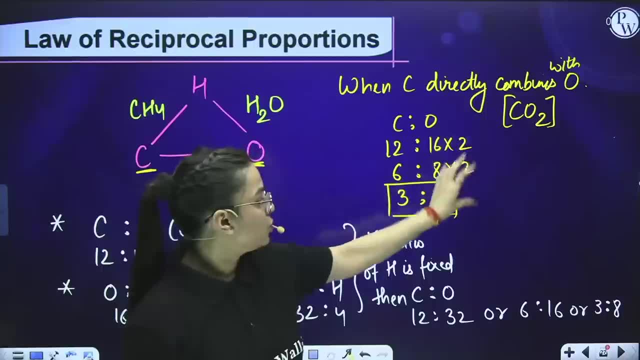 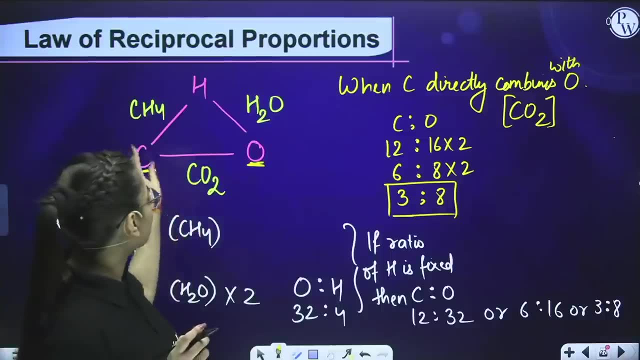 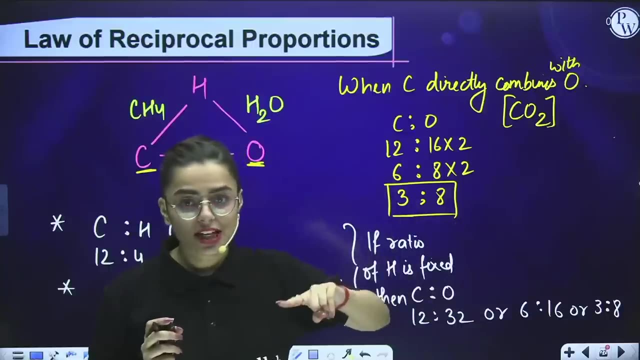 will write the ratio. third formula is co2. accordingly, we'll write the ratio. so this meansச. So what is the thing that is we are observing here? We are observing that when we are considering the two elements and keeping the ratio of the third element fixed, we are getting both of these. ratio is 3, ratio 8, which is equal. 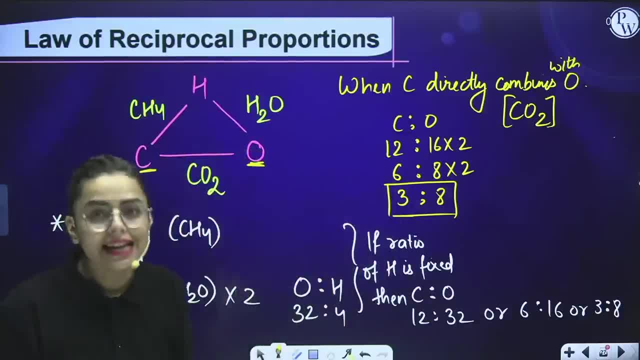 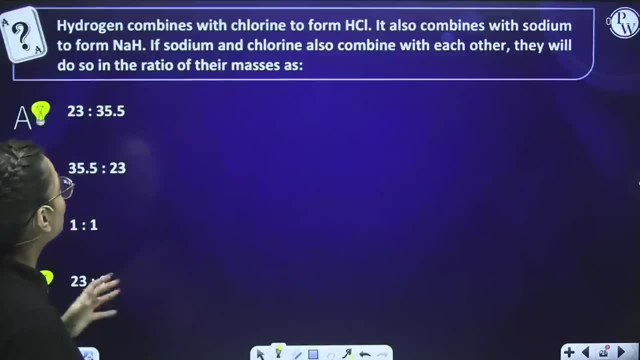 to the situation when they both combine directly. Hence this is law of reciprocal proportions. Hopefully it is clear to you. Now, moving forward towards our question, Hydrogen combines with chlorine to form HCl. Clear, I am going to write the situation. 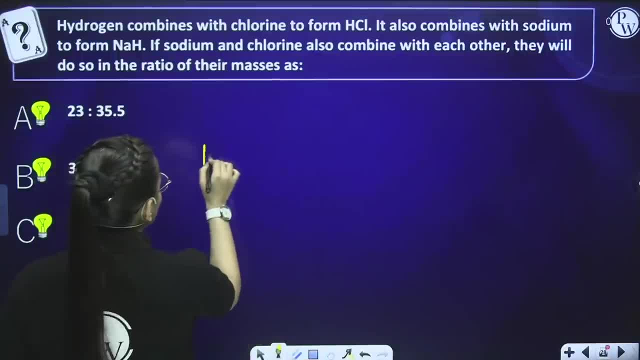 It will be easy for you, Right, Hydrogen, what it does? It combines with chlorine, right, To form HCl- Okay. The next one is sodium combines with hydrogen, again to form NH, Okay. Now it says if sodium and chlorine also combine with each other. 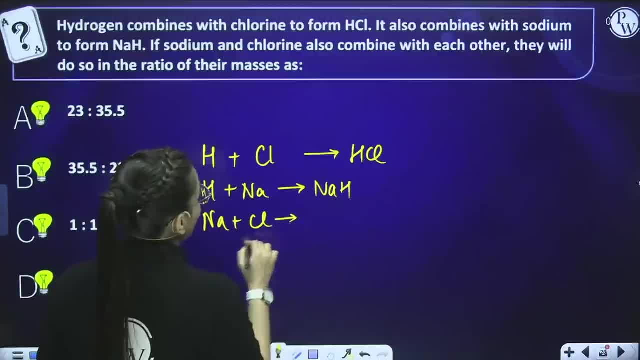 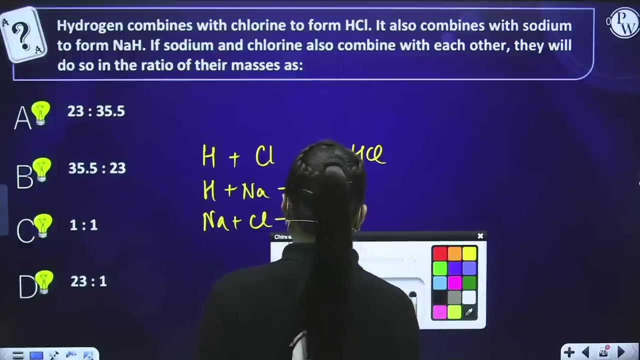 Sodium and chlorine also combine. When they combine with each other, students, they will do so in the ratio of their masses. we need to calculate the ratio of their masses Now. we have already done this situation. See, we have already calculated the situation. 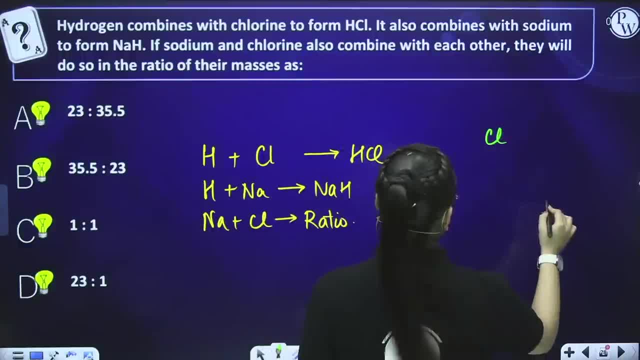 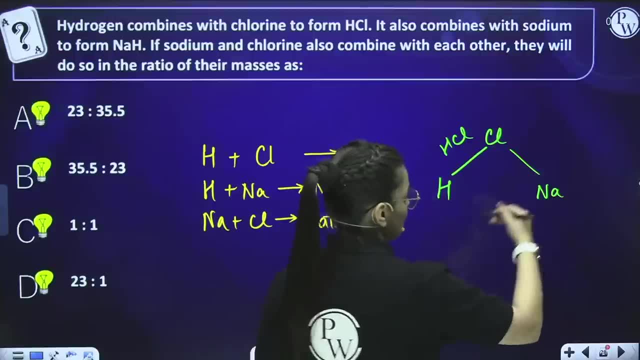 See hydrogen, chlorine and I would say sodium. When hydrogen combines with chlorine, it is forming HCl. When chlorine combines with the sodium, it is forming NaCl. When hydrogen combines with Na, It would have formed HCl, is forming NaH. So look into the situation like we did previously. First of all, in the case of HCl, 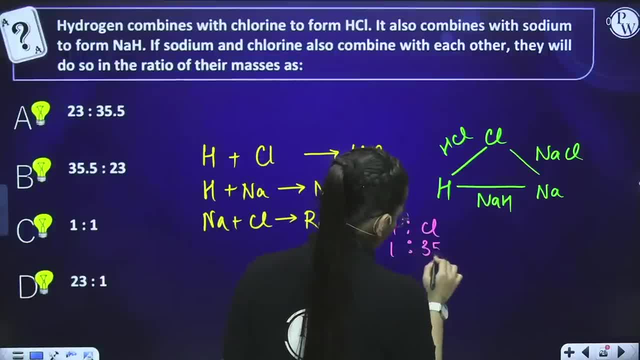 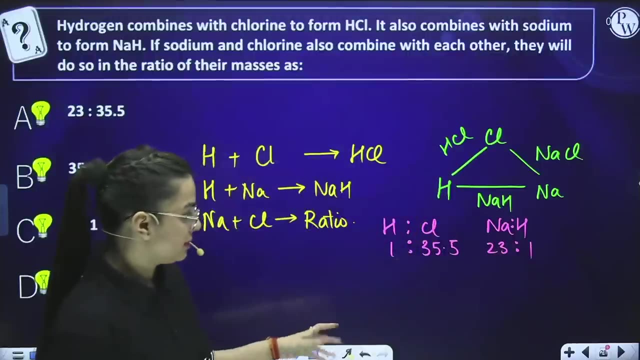 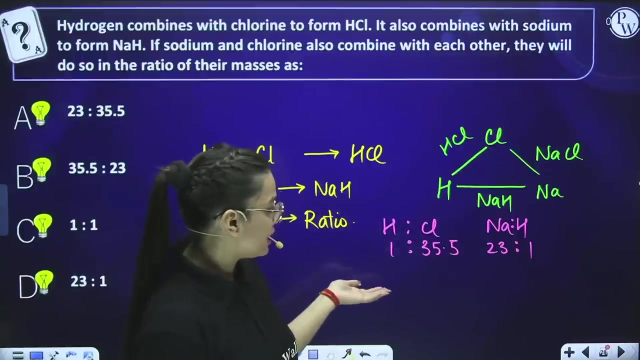 the ratio will be 1 ratio 35.5.. We are always taking the masses their weight right. In the case of NaH, again, sodium ratio, hydrogen Na is 23 while hydrogen is 1.. So what we are observing here, the hydrogen mass, is already what. It is already fixed. right, If it is already fixed, my dear 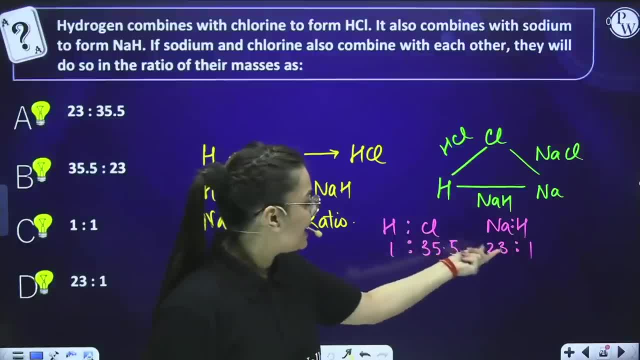 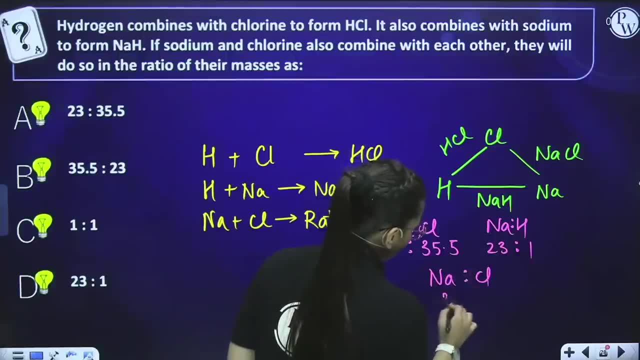 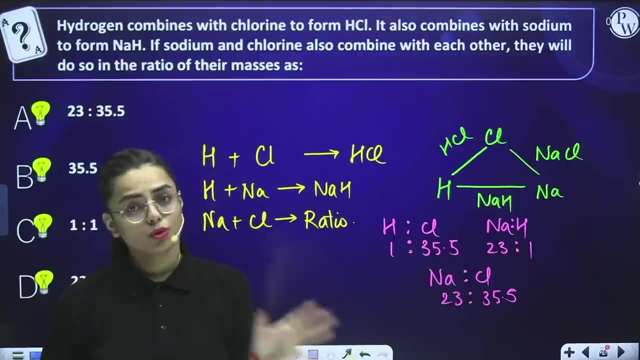 students. so what we observe in this situation: that Na and Cl will have. what Na and Cl will have: 23 ratio 35.5.. Clear, Because hydrogen masses are now constant in both of the cases. So the leftover is these both, and these are 23 ratio 35.5.. 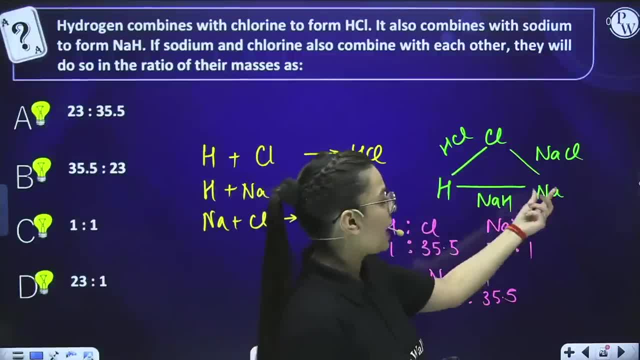 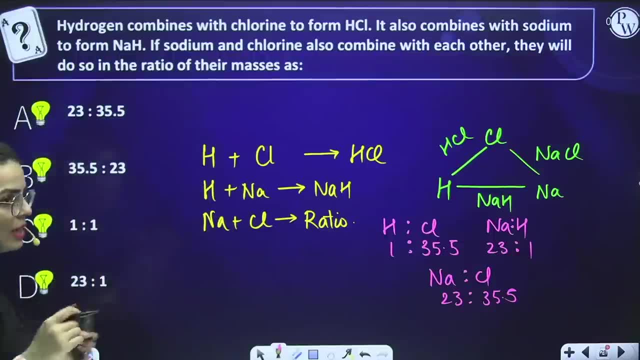 If we did individually also, then also it will be coming out 23, ratio 35.5.. Now you will say that I mean these options A and B are almost similar. How to identify? Please look at the formula. The formula is NaH, So first of all you have to write the ratio, the mass of Na. then hydrogen Na is 23, then 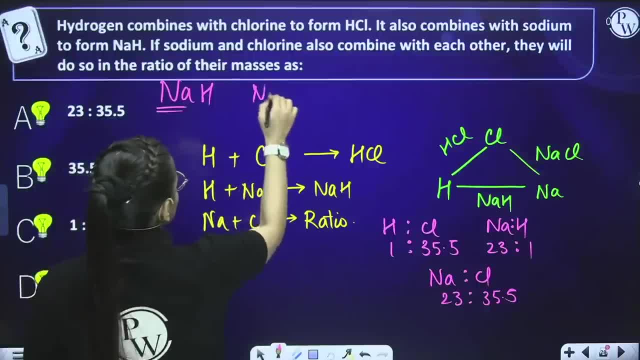 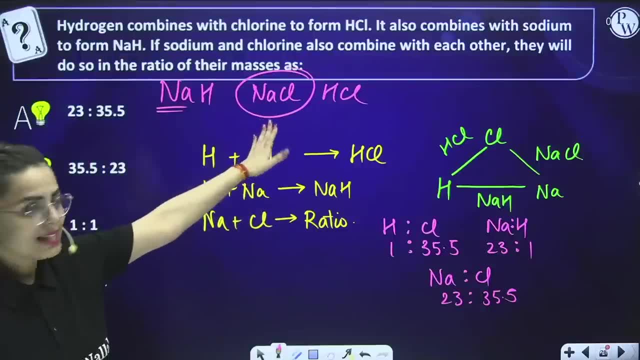 sorry: NaH and NaCl and HCl. It is like this now and it is being asking about NaCl. So first of all will not say: is Cl, my dear students? but then I will be writing about Na, then we will write about Cl. so Na is 23, then it 35.5. so which option will be correct? A option, will the correct answer, will the? 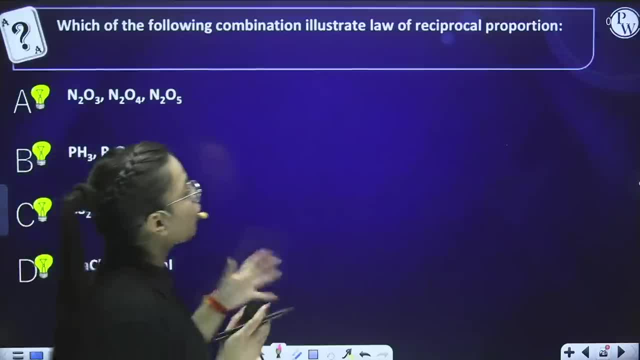 b, option number A, Clear. Okay, now proceeding towards the next questions, my dear students, which of the following combination illustrate the law of reciprocal proportion We have already understood? in the law of reciprocal proportion, we at least need three elements, that is being contact with each other, right. 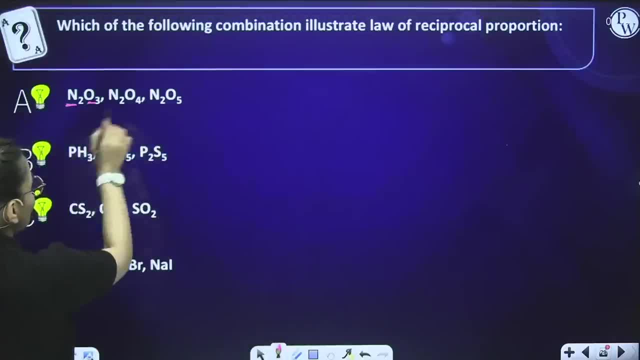 right. so in the first case only nitrogen and oxygen, in the second also compound nitrogen oxygen, in third also. so this is not possible at all because we need at least three elements different. in second b option again: phosphorus, hydrogen, phosphorus oxygen, phosphorus, sulphur- see likewise. i gave you the previous case. what we did was hydrogen chlorine and na the. 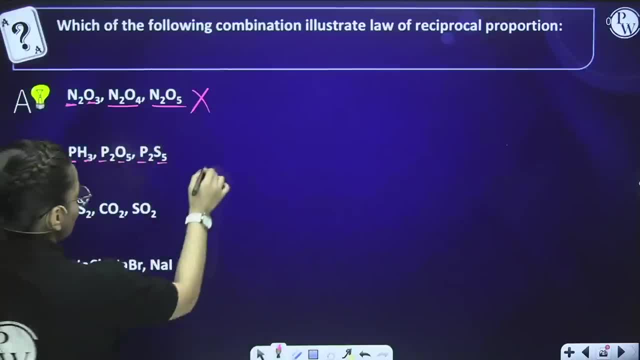 three had connection with each other. but here what you see? phosphorus, hydrogen oxygen, sulphur- it is not possible. it is not possible. four elements: no. so it is not considered. now the c option: carbon is present, sulphur is present, oxygen is present. carbon is forming bond with. 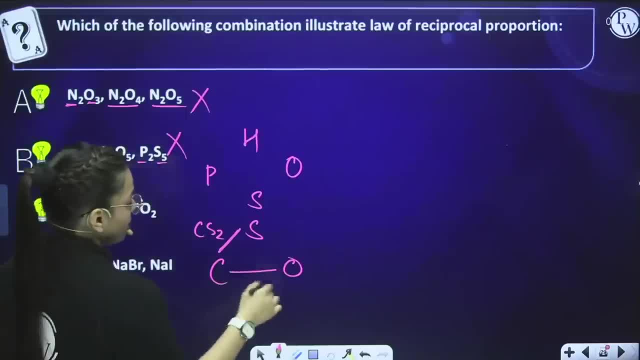 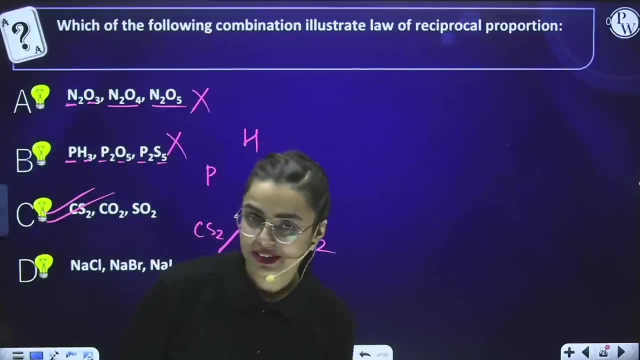 sulphur, which is cs2, carbon is bonding with oxygen, forming co2, and sulphur is forming bond with oxygen as so2. so you can directly see that it follows the law of reciprocal proportion. hence the answer c will be our correct one. clear, very good students. 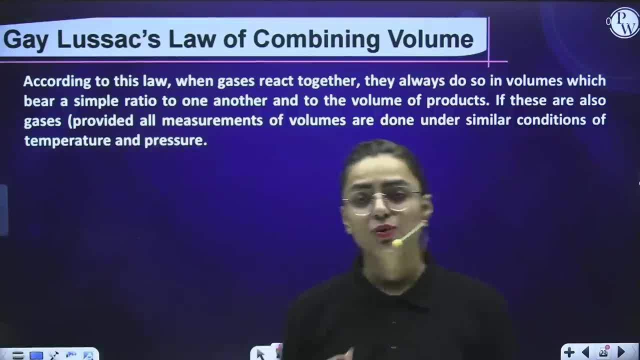 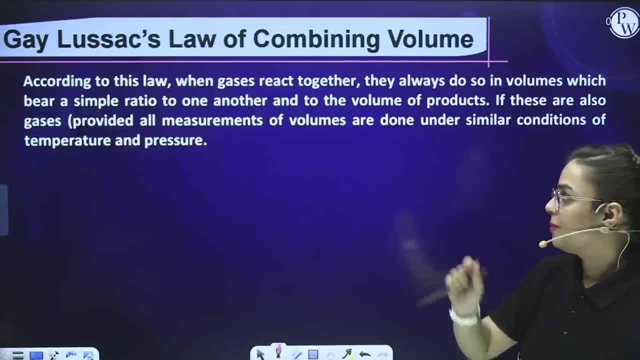 now we are proceeding towards the last law, that is, the gay-lusacz's law of combining volumes. what does it states us? it states us that, according to this law, when the gases- please consider this- when gases reacted together, they always do so in the volume which bear. 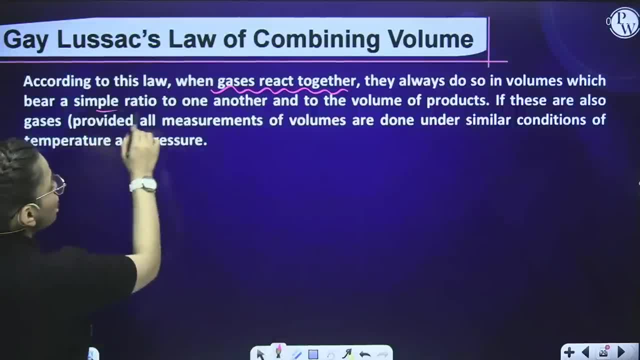 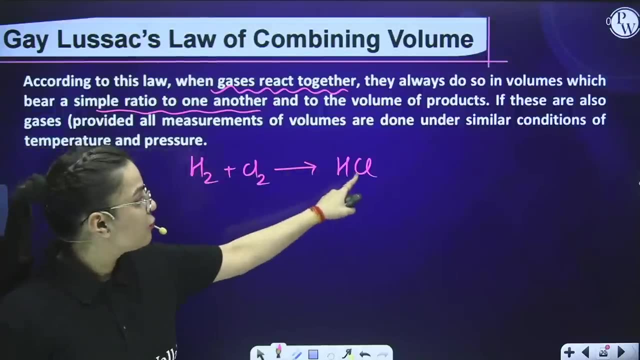 a simple ratio. a simple ratio to one another and to the volume of products. for example, if i say h2 reacts with cl2 to form hcl students, first of all balance it out. we are not going. here are two elements of hydrogen, here are two elements of chlorine, here are only one and one. 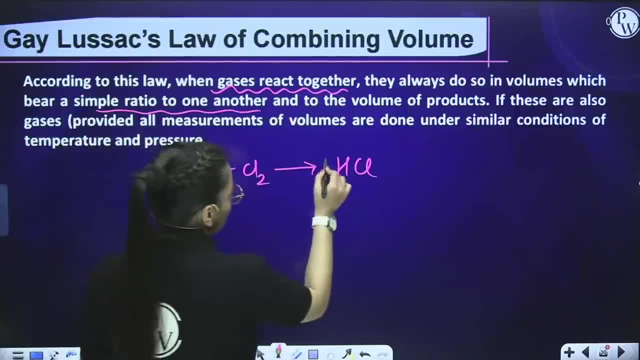 elements of hydrogen and chlorine. so what you'll do is you'll put a twice number here so that it is balanced out, right? so what? we say that here it is one one, right? so if i say that, if here it is one part, i would say if it is gaseous. so here one volume of h2 reacts with one volume of h2. 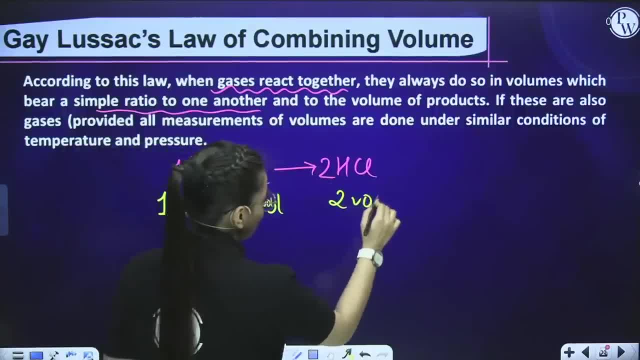 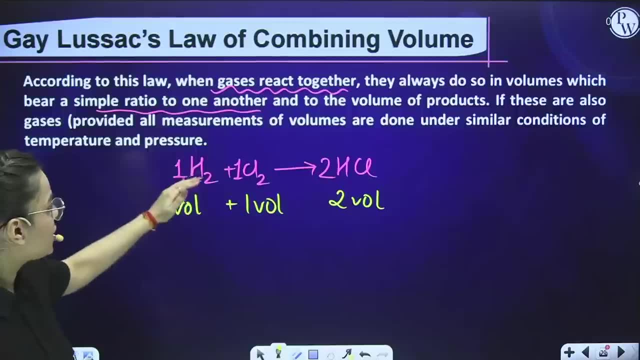 to cl2 to give two volume of hcl. how i can say that, on the basis of the stoichiometry, on the basis of these numbers which are present in front of them, like one h2 is combining with one cl2 to give two hcl, that means one volume of h2 is combining with one volume of cl2 to give two. 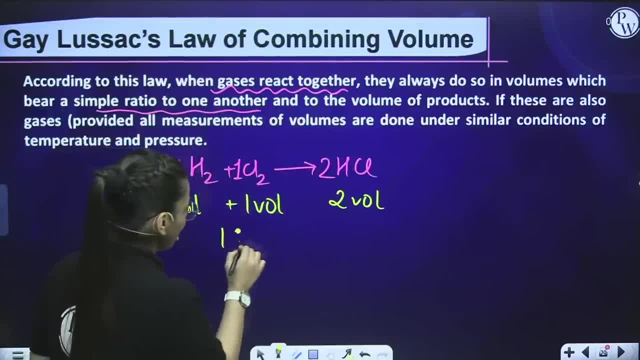 volume of hcl. so in which ratio are they? they are in one ratio one ratio two. they bear a simple, fixed ratio. so this is the law. according to this law, when gases react with each other, they do so in volumes, in volumes right, which bear a simple ratio to one another. 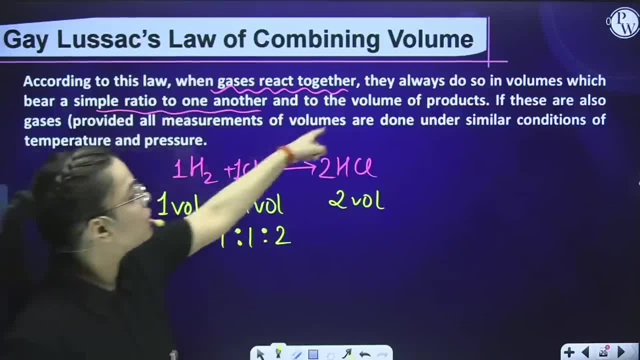 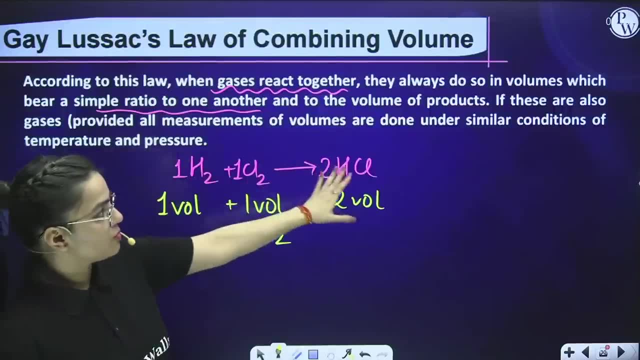 to one another- they bear a simple ratio- but also to the volume of product, also to the volume of product if these are also gases, provided all the measurement of the volumes are done under similar conditions of temperature and pressure. they are done under the similar conditions of temperature. 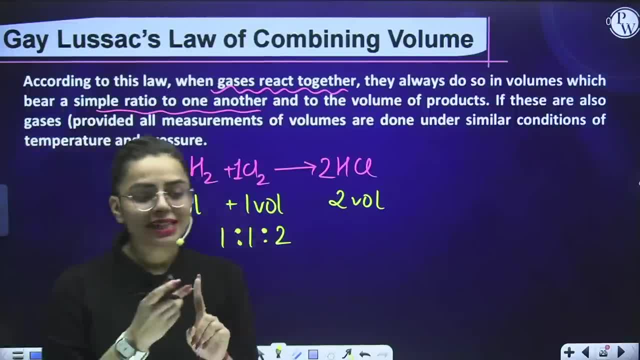 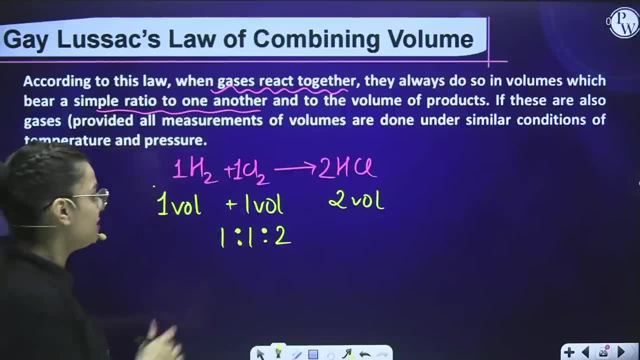 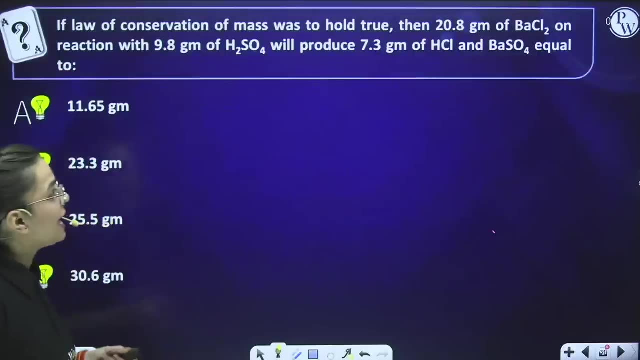 and pressure. so this was all about the galeusax law. you need to just put the stoichiometry correct, that's it. if you will able to do this balancing out, then you can find this ratio very simply. first balance out, then you can find the ratio. it is as simple as it is right, students. and now comes the question part. just look. 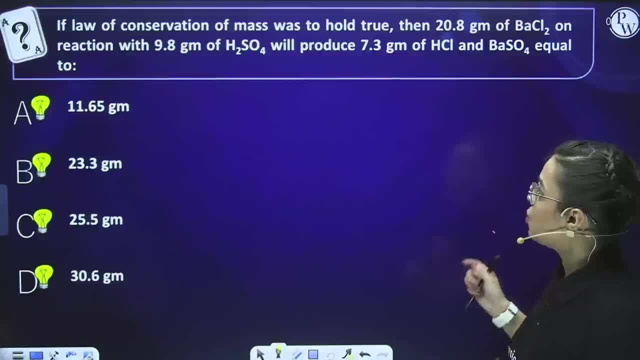 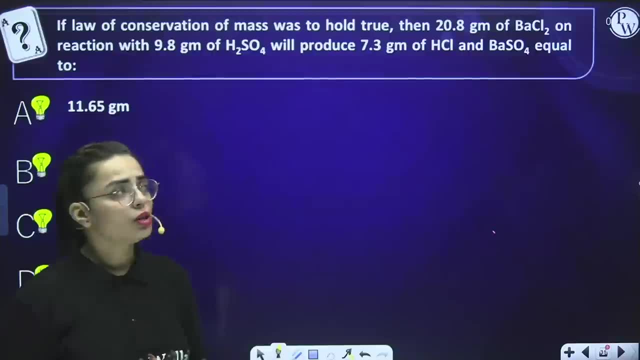 at the question: if law of conservation of mass was to hold it true, now what was law of conservation of mass? when total mass of reactant is equals to the total mass of product? this was the law of conservation of mass. then, 20.8 grams of bascl2. 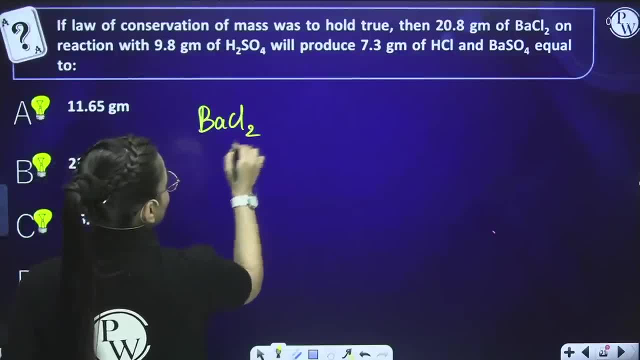 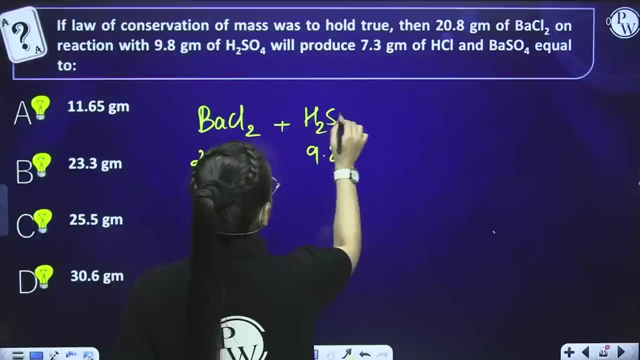 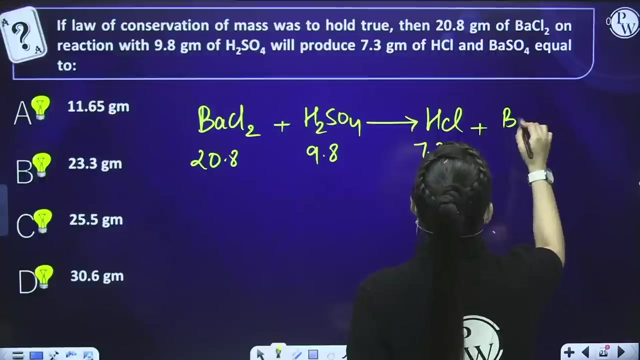 bascl2. bascl2: how many 20.8 grams reaction with 9.8 grams of h2so4 will produce 7.3 grams of hcl. let us write it down: okay, it is given a 7.3 grams of hcl and baso4 equals to. we need to find out the mass of. 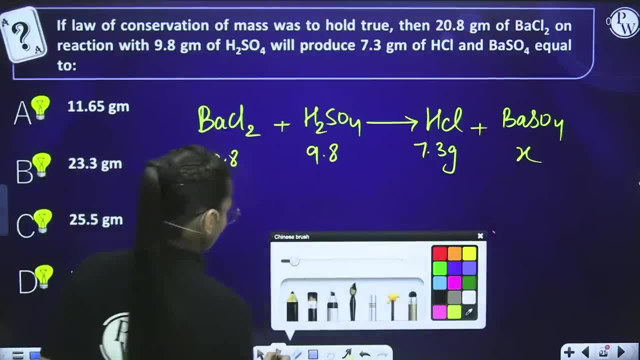 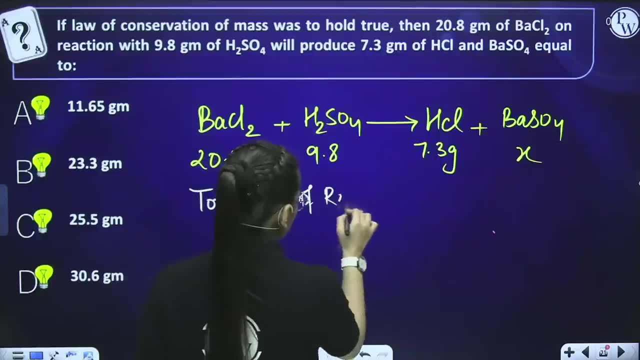 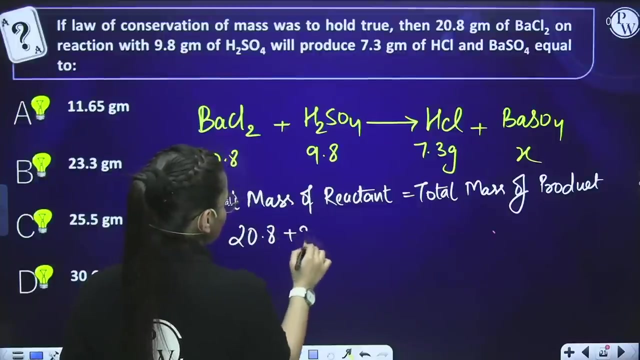 baso4. so it is as simple. what was the formula of law of conservation of mass? when total mass of basc2 has equal mass, equal to, we need to find out the mass of reactant. so which is sort of your- instead of bascd- valued mass of reactant. roll it by. bascd object much further to 0.. structure. retion b: total mass of reactant is equal toweight ion x. total mass of reactant would be: total mass of reactant will be bright, you can out to be. the mass of reactant will be massive, but the mass of fault would be positive because earth mass of the product, students. now, the total mass of reactant will be twenty point eight, nine point eight is equal to seven point three plus x right, plus x right, first of all, the add it is thirty point eight right. so multiplied it is、. 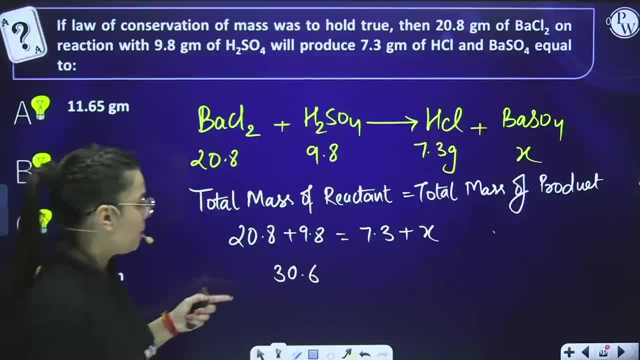 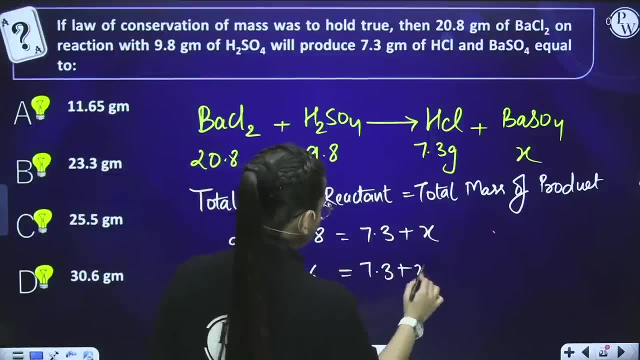 30.6 students, it is going to be 30.6. let me just do this again: yeah, so is equals to 7.3 plus x. now this will come here and subtract: 30.6 minus 7.3 is equals to x, which is going to be 3. 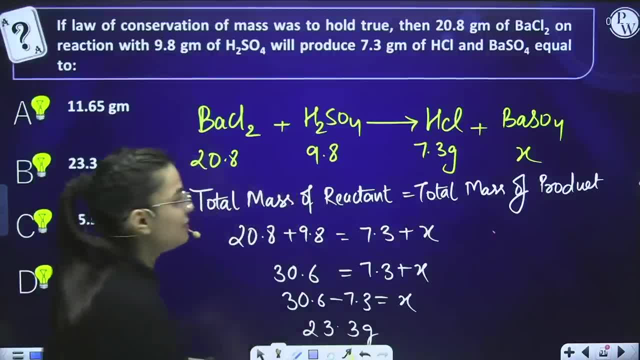 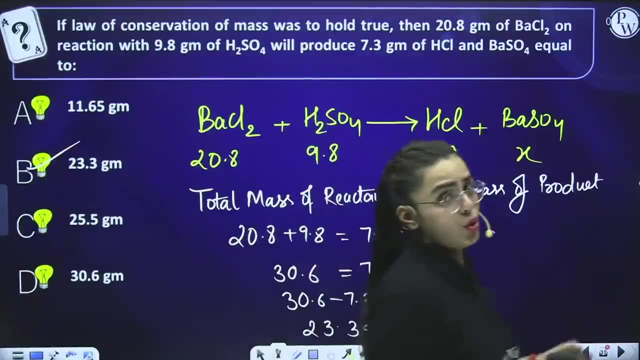 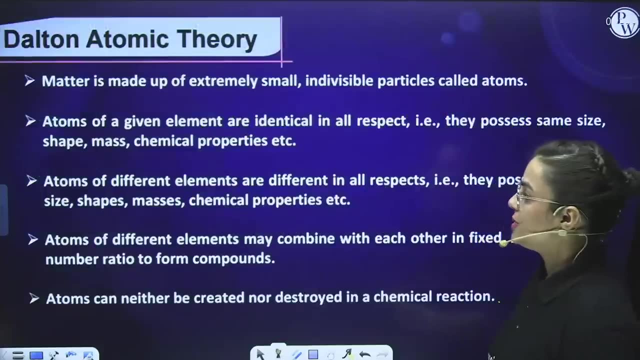 so it is going to be 23.3 grams, my dear students, now let us see the options. hence b option is our correct one, clear. so the law of conservation of mass states us that total mass of reactant is equals to total mass of product. so here, students, comes the dalton atomic. 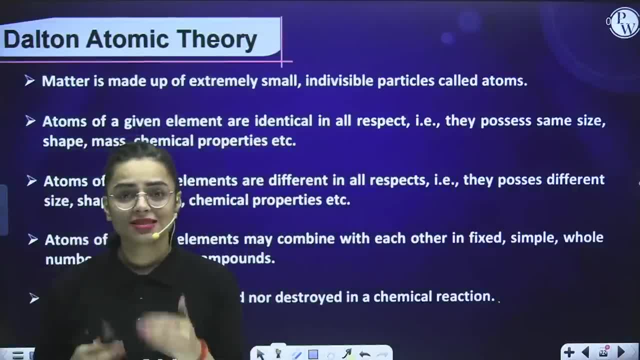 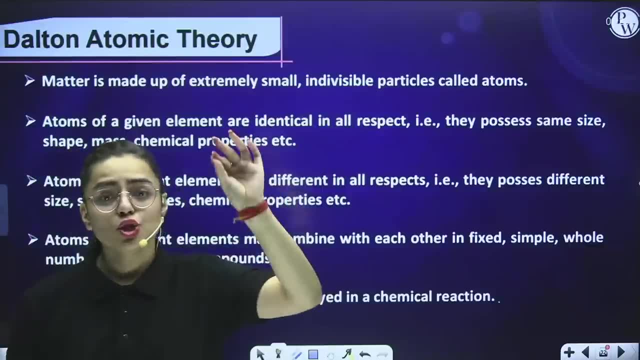 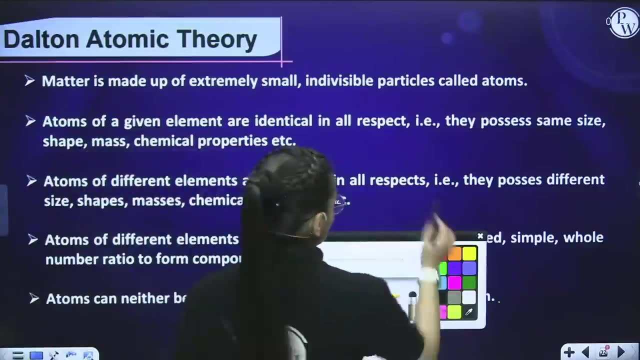 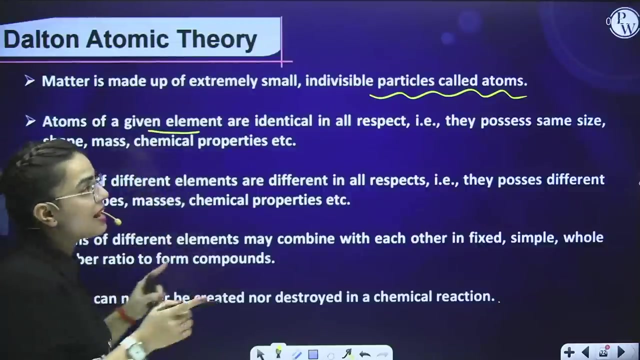 theory after the laws dalton atomic theory states us about atom. basically, dalton atomic theory tells us that matter comprises of very small, extremely small, indivisible particles that cannot be divided. students which are known as atoms, which are known as atoms, and these atoms, these atom students of a given element, are identical in 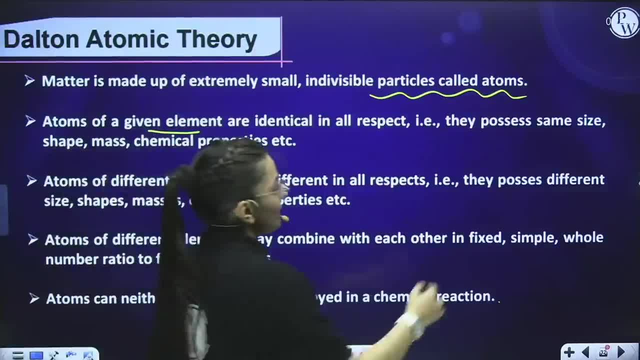 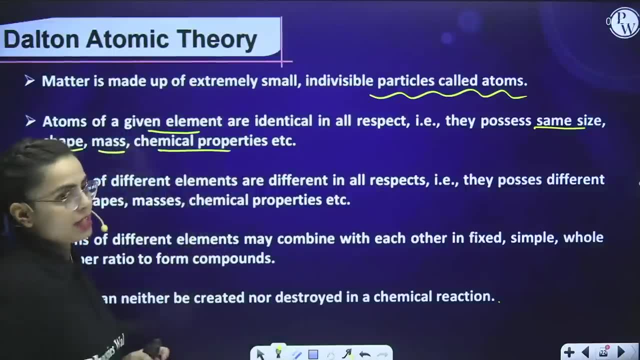 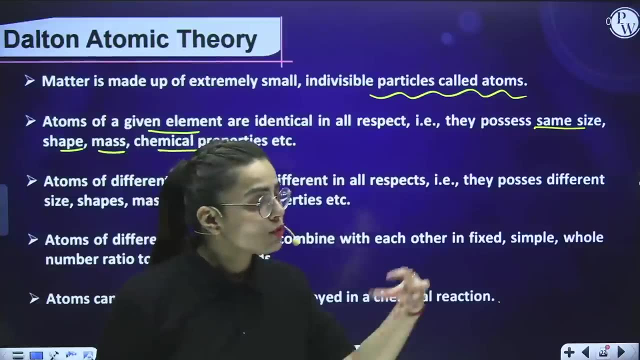 all aspects, in which which aspects they are identical? that they have same size, they have same shape, they have same mass, they have same chemical properties. the next thing is that atoms of different elements are different in all respects. see, atoms of same element will have all the same properties, but atoms of different elements will exhibit different properties. 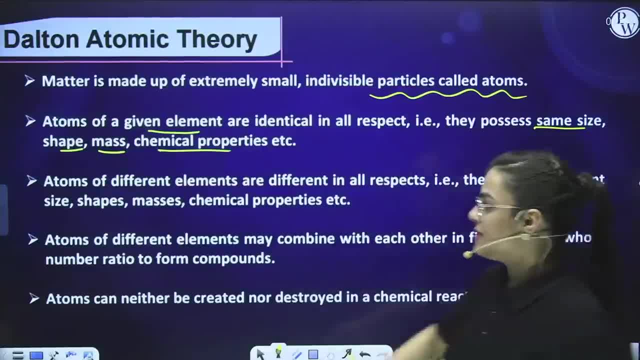 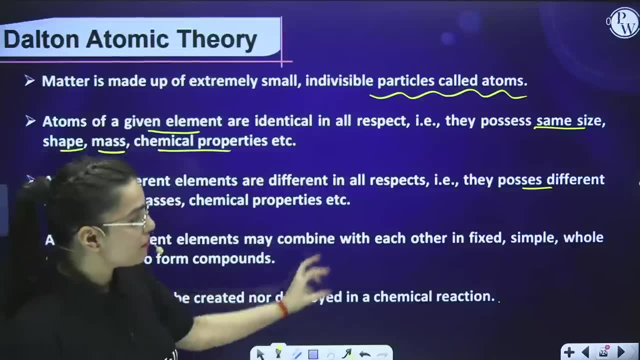 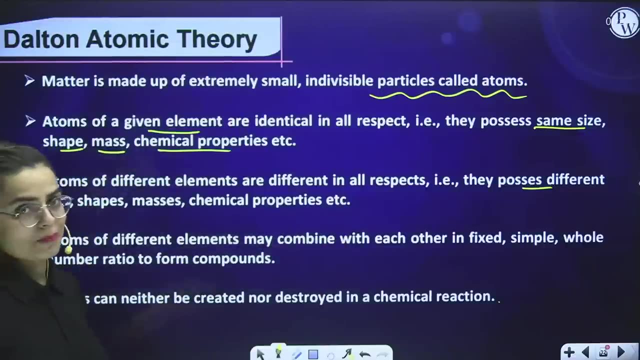 for example, they possesses different, say, shapes, sizes, mass. in all of this, right then it comes that atoms of different elements may combine with each other. they can combine with each other in fixed, simple or whole number ratio to form compounds. clear, they can form compounds. next thing is, atoms can neither be created nor be destroyed in a chemical. 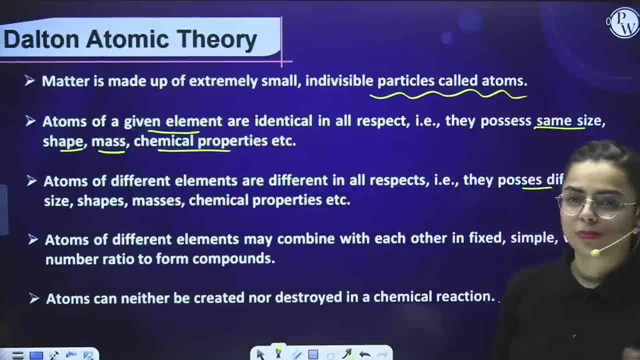 reaction students. but there were the limitations of dalton atomic theory, which couldn't explain us about isotopes, you know, because atoms cannot be created in a chemical reaction. so now let's you know. the second thing was that they were are they weren't able to explain about how they were. 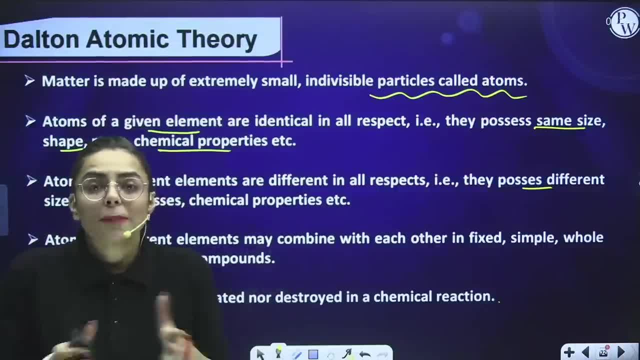 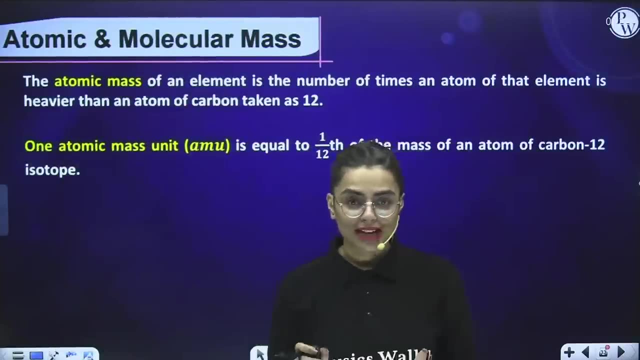 able to form compounds, how different elements could combine and form compounds. so these were the limitations of dalton atomic theory, right? so now we are proceeding towards our next topic that is going to be atomic and molecular mass. but before atomic and molecular mass, we need to understand about atom, which we have already done in dalton atomic theory- that atom is the smallest. 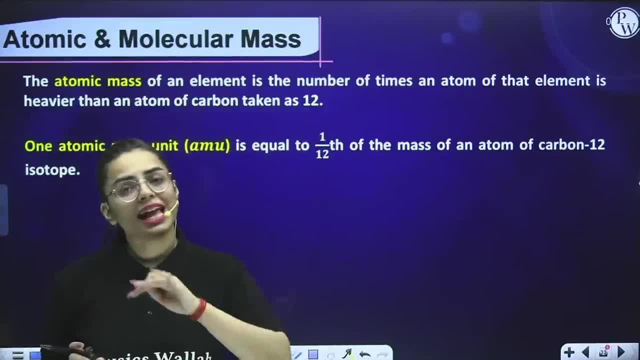 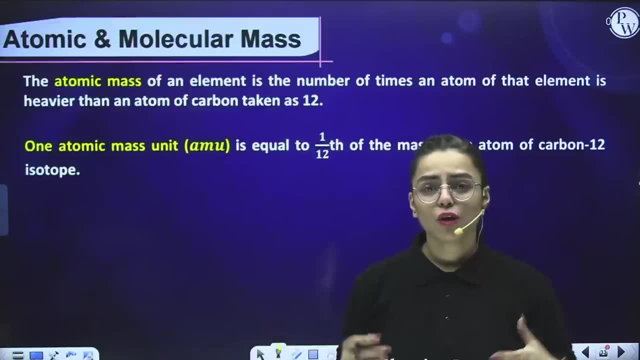 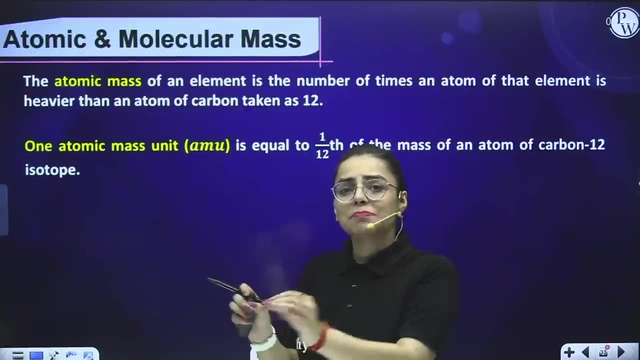 indivisible particle and it is responsible for any chemical reaction. right, but what we see is that when we go into market, what is the need, you know, of mole concept, of bringing this chapter to you? the main reason is that there are many quantities which we can measure, but there are. 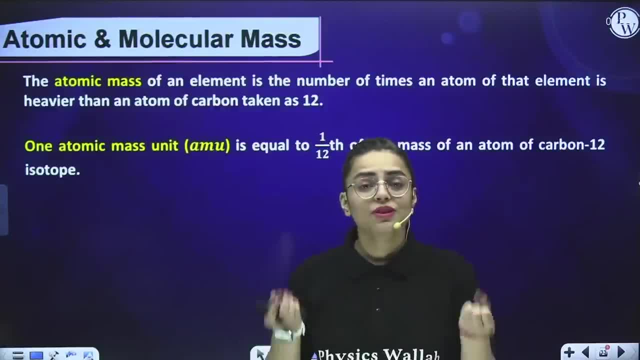 some quantities which we cannot measure. to measure them we have introduced mole concept. how i am saying that if i go to market to buy some fruits or bananas, i say that i need one dozen bananas. one doesn't stand for 12 bananas. bananas, right. and then the next day i go in i ask: 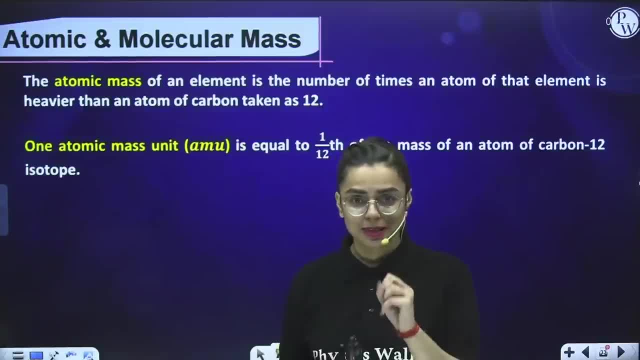 for five dozens. so how many bananas i'm going to get? 60 bananas i'm going to get. so what i've done for bananas, i have set an equation, i've set a set a standard like dozens, right, so i can calculate that in terms of fruits and vegetables. but when i come across chemistry there 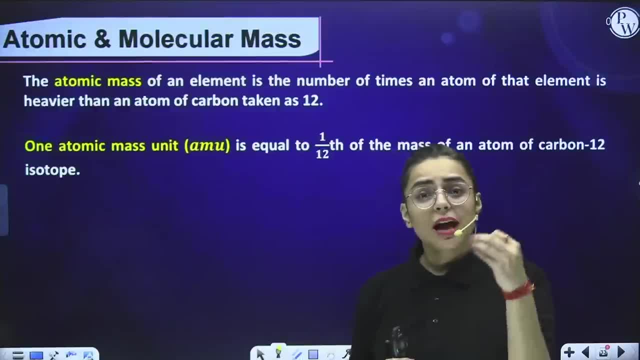 are some quantities, there are some atoms whose amount of substance is not being calculated in terms of dozens or kgs or like this, no, so we need to introduce a term, and hence we introduced atom. so these atom, these atomic mass, helped us to calculate the amount of substance in chemistry. 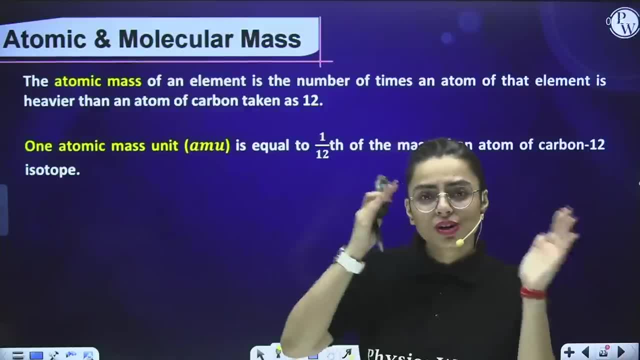 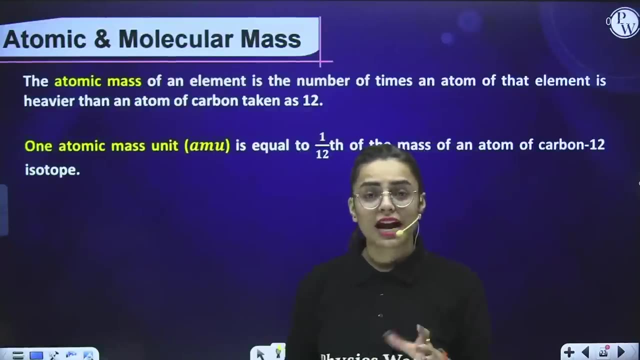 field in chemical reactions. so whenever we could correlate this with the daily life situation, for daily life we have referred a standard. similarly, for chemical reactions, we have kept a standard that is c12 carbon as our standard rate reference. with the help of that we are going to calculate. 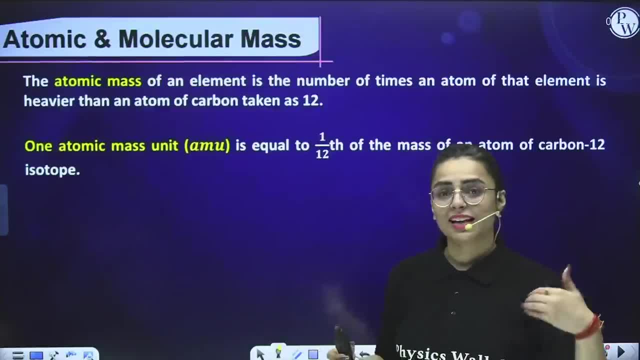 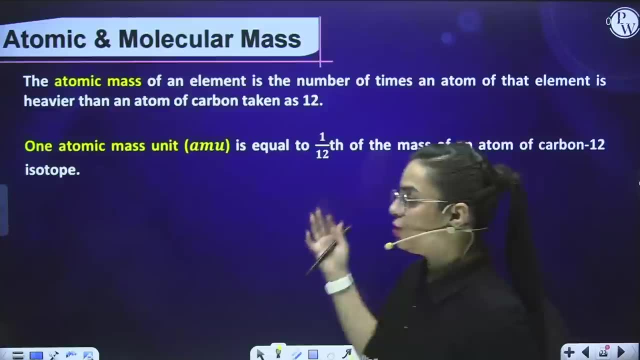 all the masses. like with the help of carbon atom, we can calculate other atoms, element masses, and through them we can calculate atomic mass and molecular mass. so what is going to be the atomic mass, students? atomic mass of an element is number of times an atom of that element. 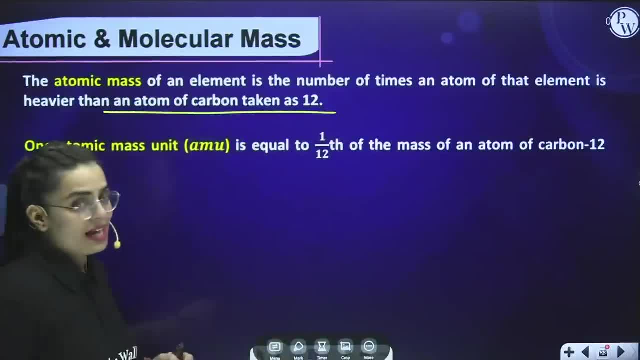 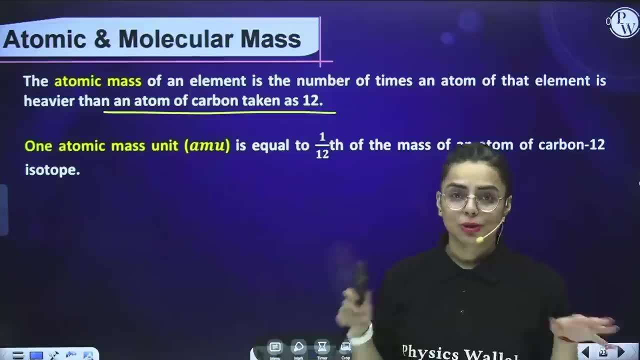 is heavier than an atom of carbon taken as 12.. why we are considering here carbon here? because, as in the case of vegetables, we took dozens as in reference in the case of chemistry, we took carbon as our reference. that's why, Then, the definition which is reported to you is this one, that one atomic mass unit which 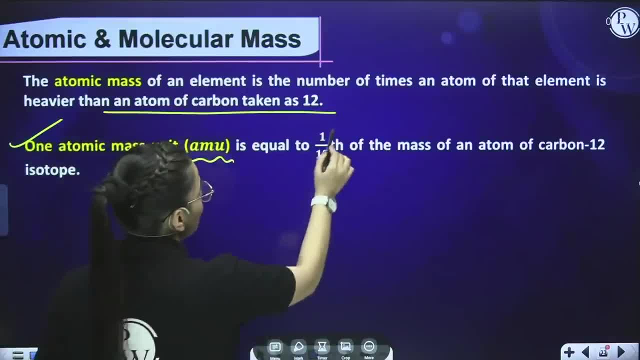 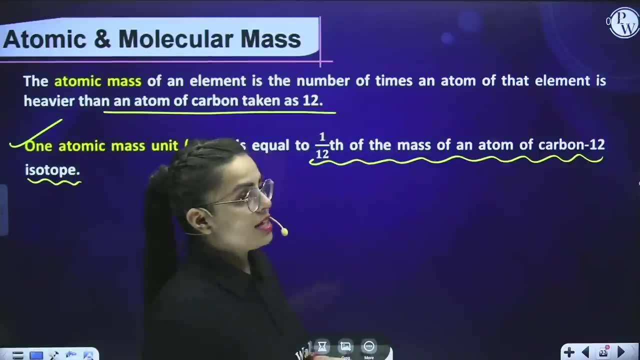 is known as AMU. it is equal to 1 by 12th of the mass of an atom of carbon-12 isotope. Clear, students. So now we are going to start mole concept in detail, considering each and every situation when volume is given to us, when molecular mass is given to us. 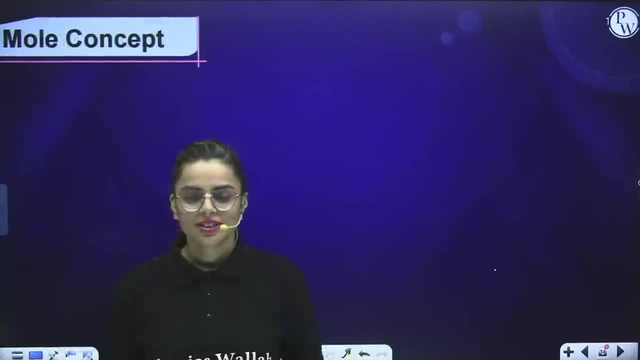 So now let us start towards the mole concept. So yes, students, as you all know, we are doing mole concept and mole concept. first we need to understand what is a mole. Basically, a mole of a substance is 6.022 into 10, raised to the power, 23 particles, which is referred to as Avogadro's number. So I would define first of all mole for you. What is mole? Mole is defined as. mole is basically defined as: one mole of a substance is equal to 6.022 into 10, raised to the power, 23 particles. 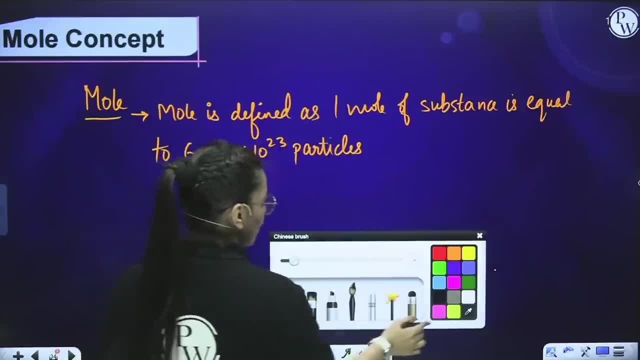 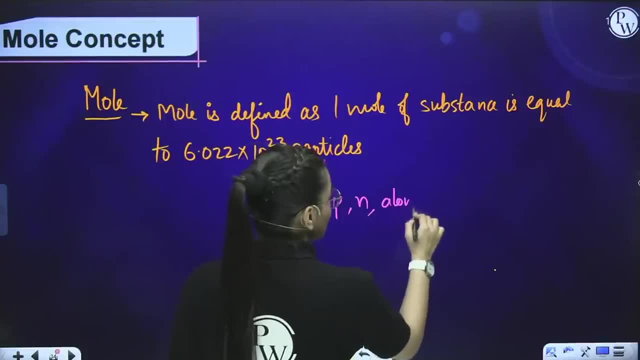 Now, students, I am talking about particles. Clear particles are of various kinds. it can be electrons, it can be protons, it can be neutrons, it can be atoms, it can be ions, it can be elements. everything lies in these. you know, particles can be any of them. 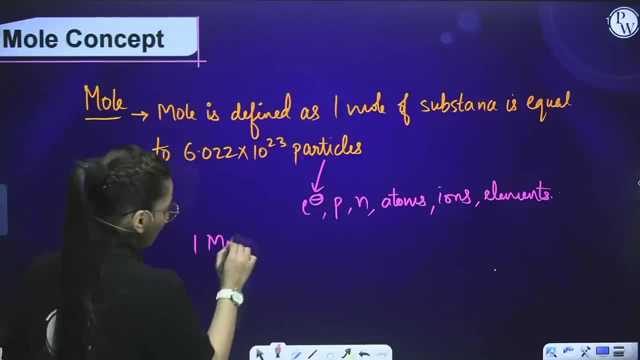 So in short I can say that one mole is equals to 6.022 into 10 raised to the power 23 particles. Here you can add molecules also instead. So one mole is equals to 6.022 into 10 raised to the power 23 particles. 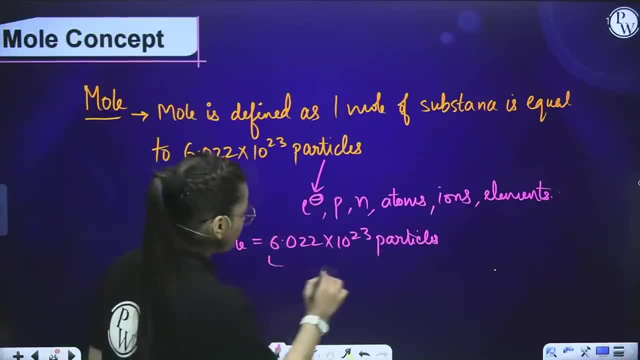 Particles. I have already told you these can be this thing and this value, students is known as Avogadro's number. Okay, now, what is the use of this Avogadro number? we will use this in formulas and it is going to be very interesting and very easy topic. 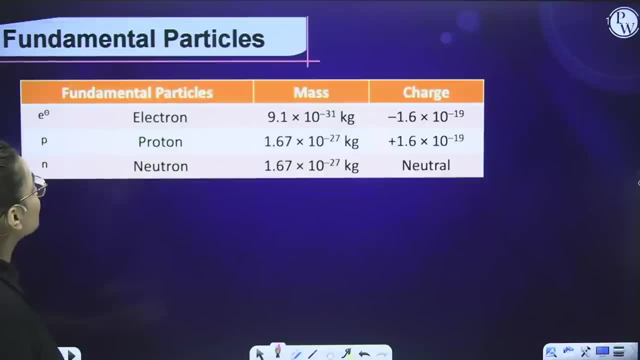 Okay, so now let us proceed towards our next fundamental particles, which I have already told you About: electron, protons and neutrons. Now, the particle electron has mass 9.1 into 10 raised to the power minus 31 kg, and its charge is minus 1.6 into 10 raised to the power minus 19, as it is electron, so negative. 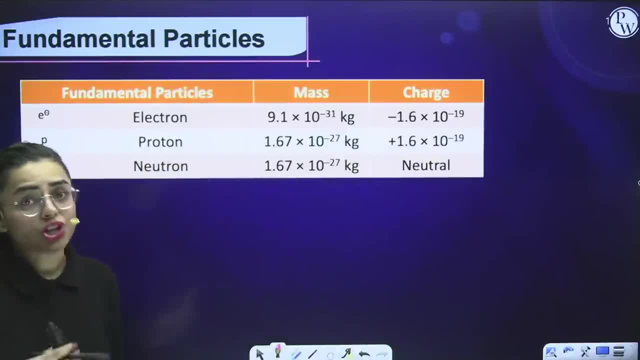 charge comes in front of this. Then protons come, which are positively charged particles. Proton, basically, is represented by small p and its mass is 1.67 into 10 raised to the power minus 27 kg, and its charge is 1.6 into 10 raised to the power minus 19.. 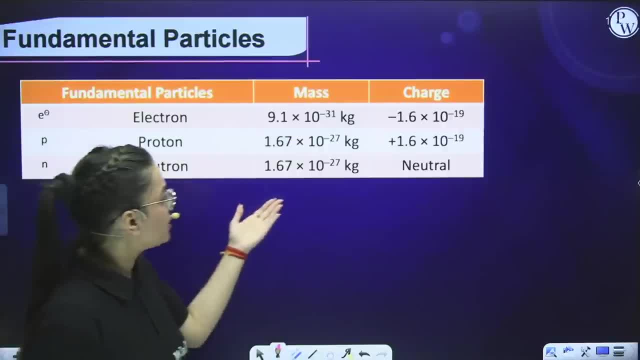 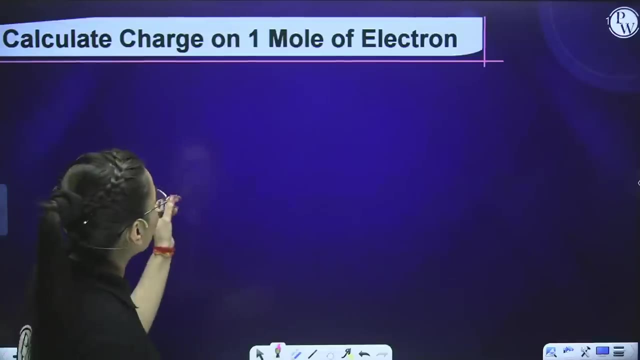 While if I talk about neutron, then the mass is 1.67 into 10, raised to the power, minus 27 kg, and its charge is neutral. So these are the fundamental particles which we should know right. Okay, now one of the question that they can ask you is: calculate charge on one mole of? 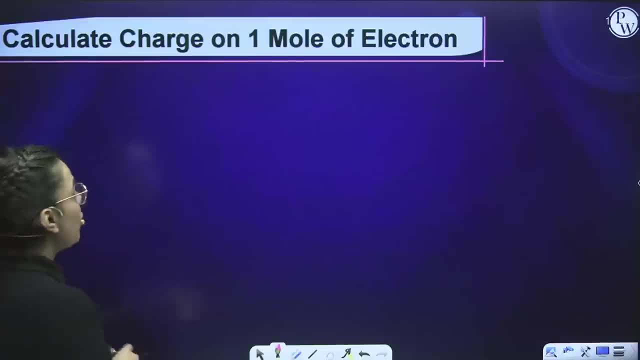 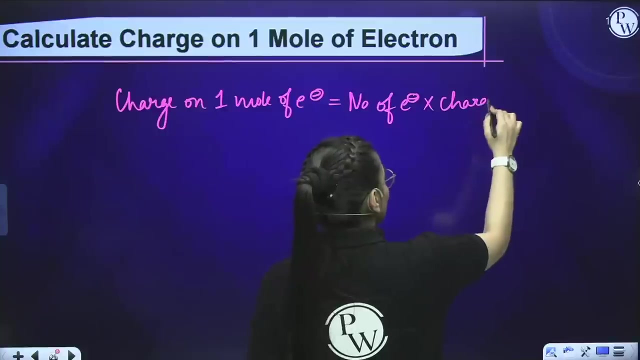 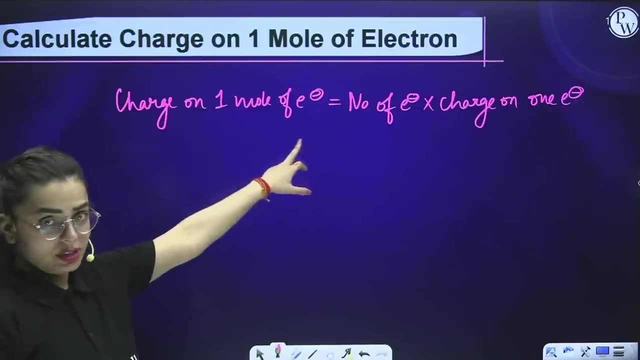 electron. Basically, students, to calculate charge on one mole of electron, Charge on one mole of electron, We need to calculate it by number of electrons into charge on one electron. See, we have to calculate charge of one mole of electron right and for that the formula: 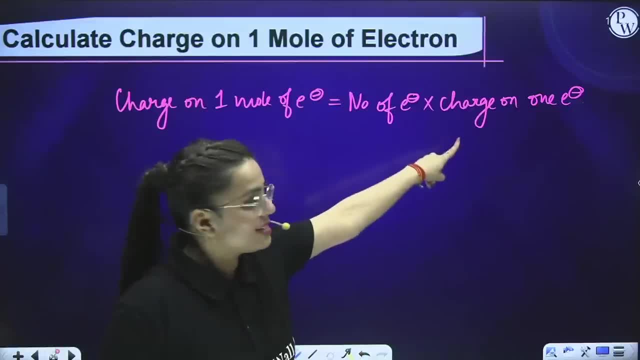 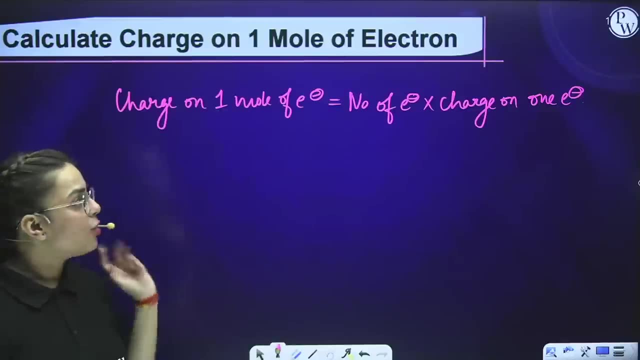 is number of electron. total number of electron into charge of only single electron will help you to calculate the charge on one mole. As you all know, one mole is basically one mole contains how many electrons we have just done right now. One mole contains this kinds of particles: 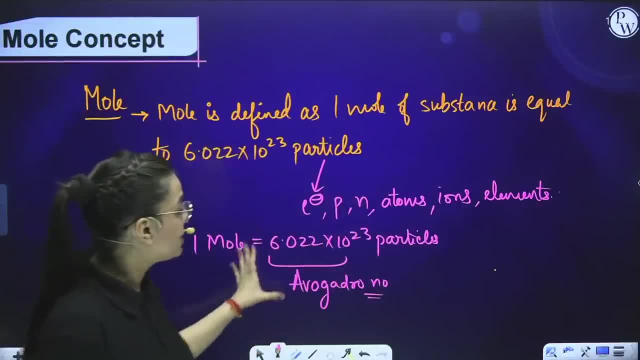 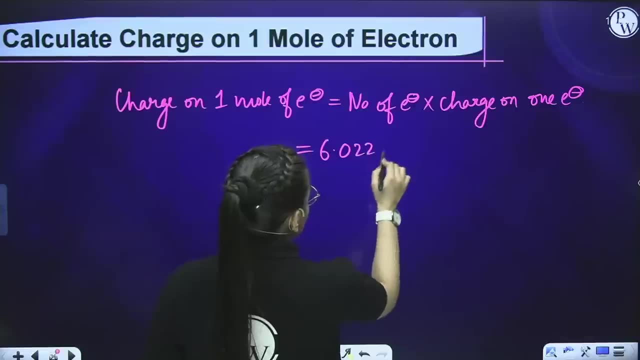 Particles can be electron. that means one mole have this much of electrons right. So now here, how many electrons are present: 6.022 into 10, raised to the power 23, which is Avogadro number, and it is represented by Na clear into. now comes the charge on one. 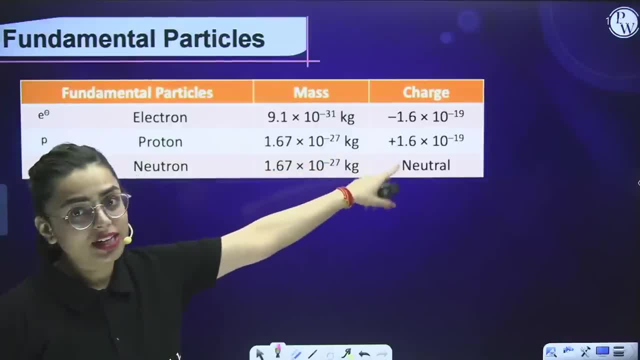 electron We have just done right now, charge is 1.6 into 10, raised to the power minus 19.. You don't have to put this negative sign when you are calculating something. it is just to represent that electrons are negatively charged. Okay. 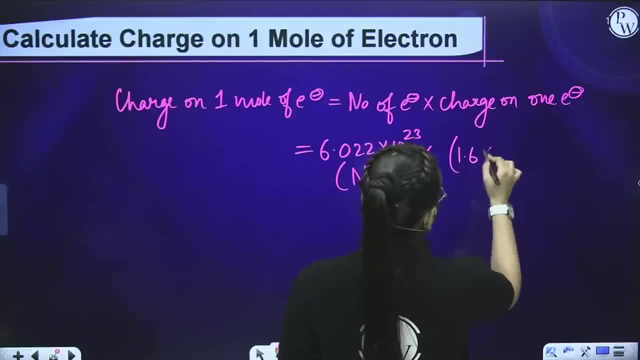 So now we will put the same value 1.6 into 10, raised to the power minus 19, right? So when we will solve it, it will come 965 00 coulomb. It comes in coulomb. you can convert it into faraday also, which is equals to 1 faraday. 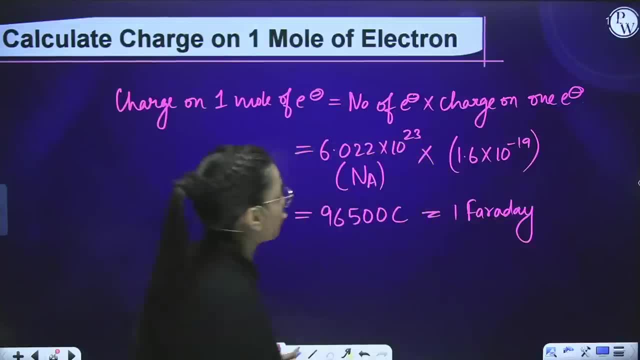 So by this way we can calculate the charge on one mole of electron. for example, they ask you on two mole of electron, then you can multiply it further. So these kinds of question can be asked on fundamental particles. it is the basic thing that you can do. 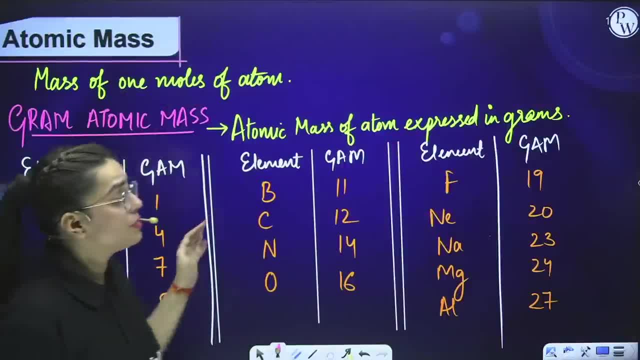 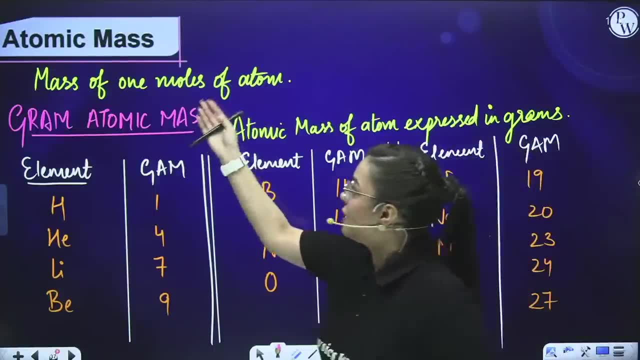 You can get to know. right now, students, I am coming across the most important and interesting part of the chapter, which is atomic mass. basically, what is atomic mass? atomic mass is the mass of one moles of atom, and there are certain atomic mass that you need to learn, for example, 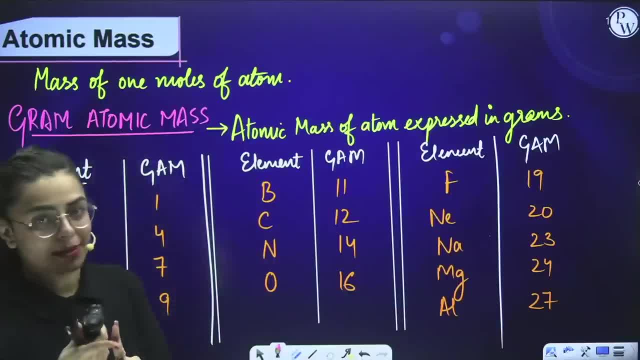 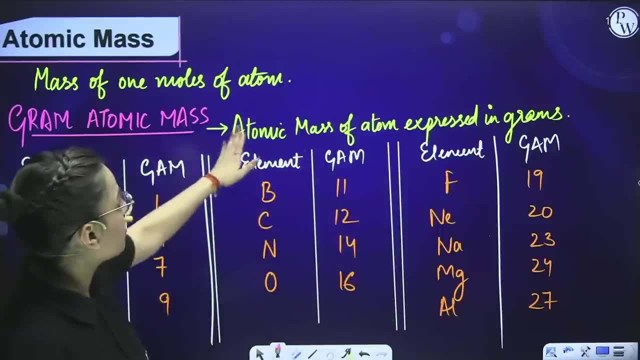 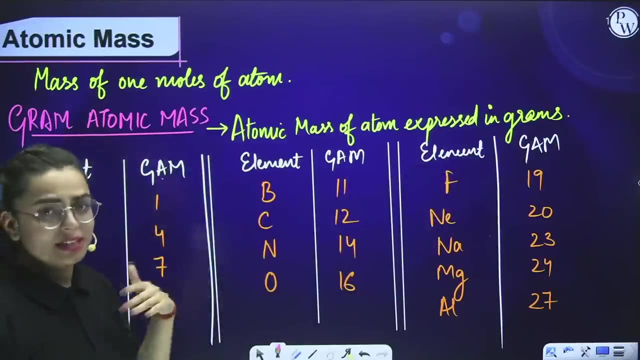 the atomic mass. that you need to be learned. you have to learn it in grams, basically, gram atomic mass is referred to as when we represent mass in terms of grams. when atomic mass of atom is represented in grams, It is known as gram atomic mass. For example, hydrogen has gram atomic mass one this you need to learn the table which. 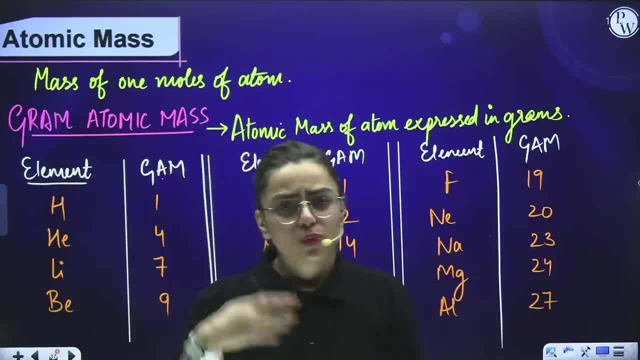 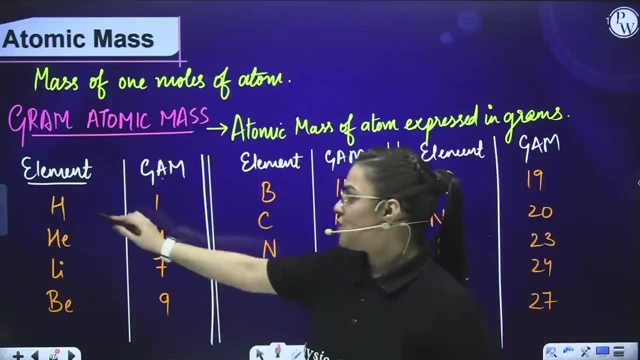 I have drawn here other than this, only one. two, three, four would be there that you could recall and learn right, but these are important for you to learn to calculate molecular mass. Okay, hydrogen has gram atomic mass. one. helium has gram atomic mass. four, lithium has gram. 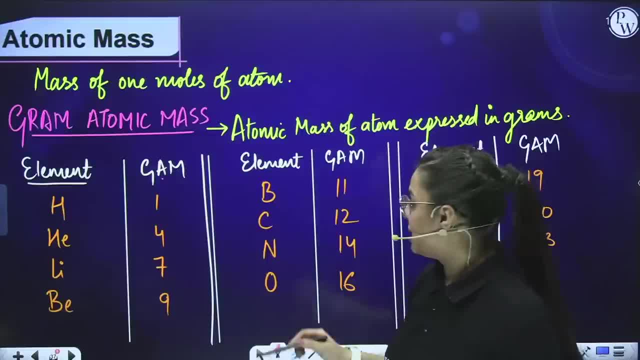 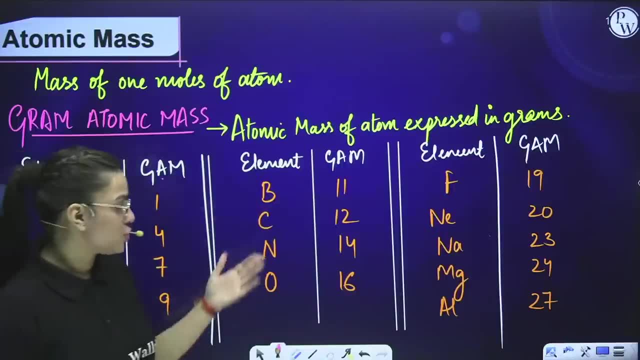 atomic mass seven. beryllium has gram atomic mass nine. then we have further boron, which is gram atomic mass 11.. Then we have carbon as 12, nitrogen as 14, oxygen as 16, fluorine as 19, neon as 20, sodium as 23. 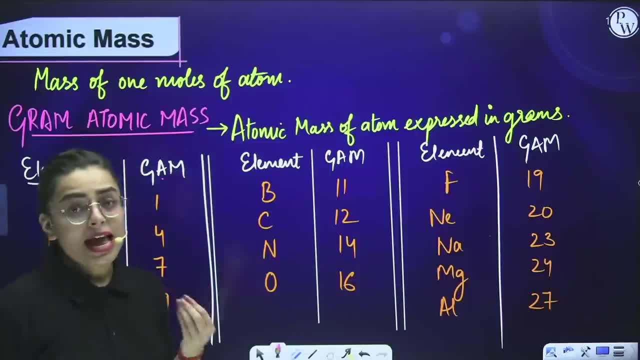 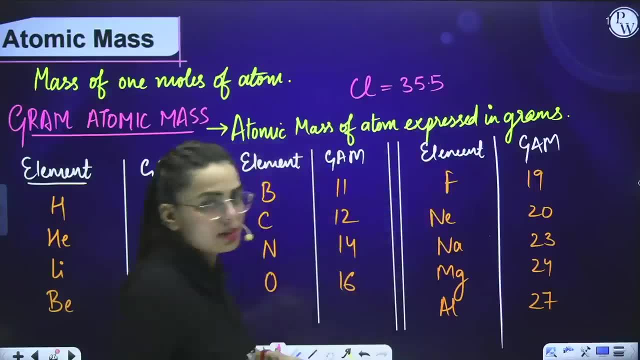 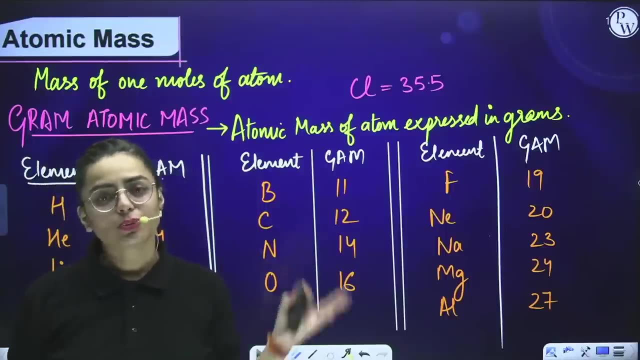 magnesium as 24, aluminium as 27, and you can all. they can also ask you about chlorine, which is about 35.5. okay, this is a little bit different, so they can ask you the same also. so you need to learn these elements and the gram atomic mass practice will make you perfect when you 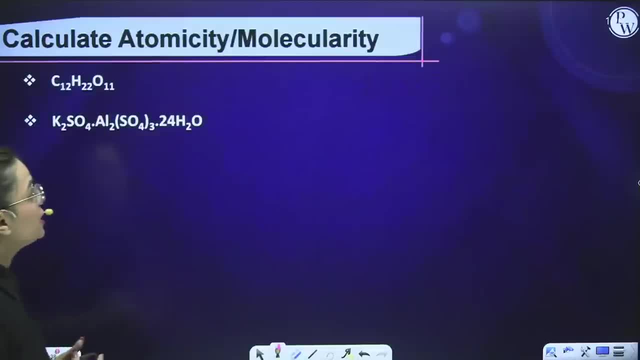 will apply them on questions. Right, Great Students. now you need to calculate the atomicity or molecularity. what do you mean by atomicity or molecularity? it tells us how many atoms are present in a molecule. So for the first case, it is given that C12H22O11. how many atoms are present in this case? see 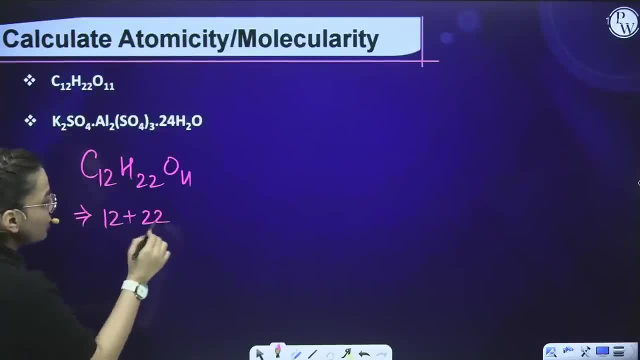 how many carbon are there 12? how many hydrogen are there 22? how many oxygen are there 11? so we will add them. it is it is 45. That means 45 atoms are present in this case. now, taking this case, how many potassium are? 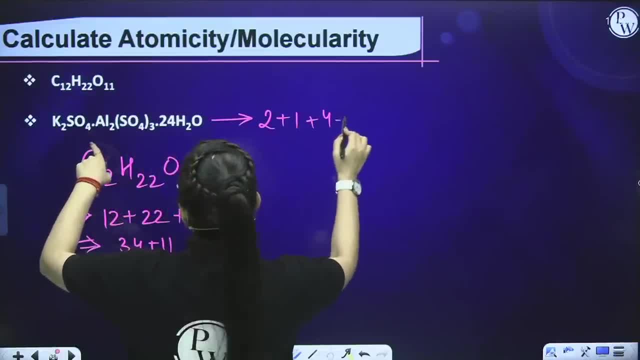 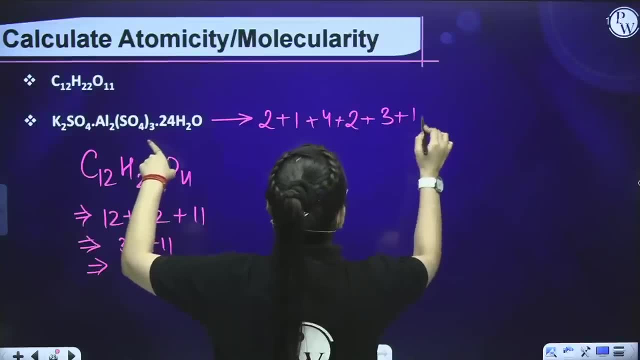 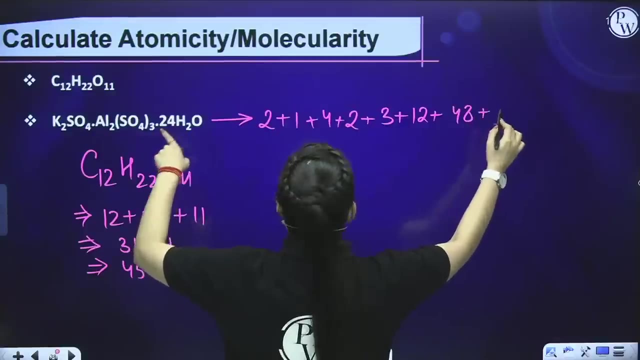 there: 2 how many sulfur, 1 how many oxygen? 4? how many aluminium? 2 how many sulfur it is into 3 plus how many oxygen it is, 4 into 3, that is 12. how many hydrogen? again 24 into 2, it is going to be 48, plus how many oxygen, it is 24. so, students, by this way, when you 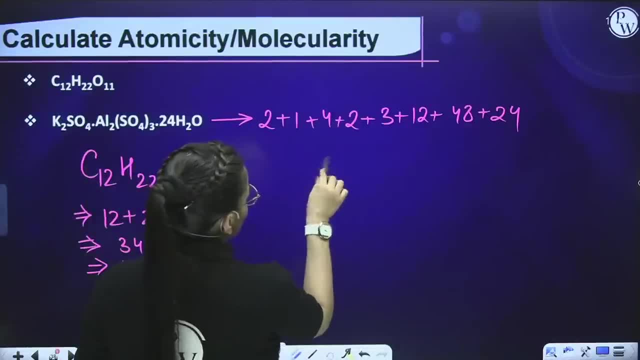 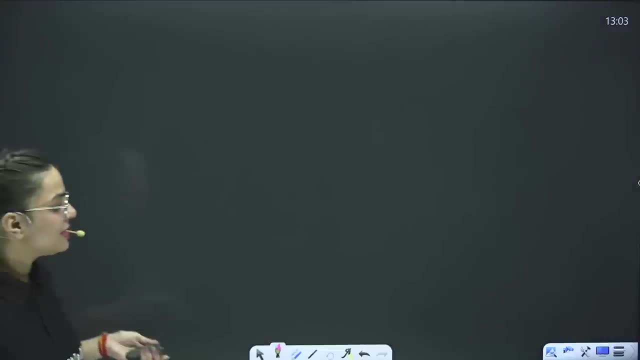 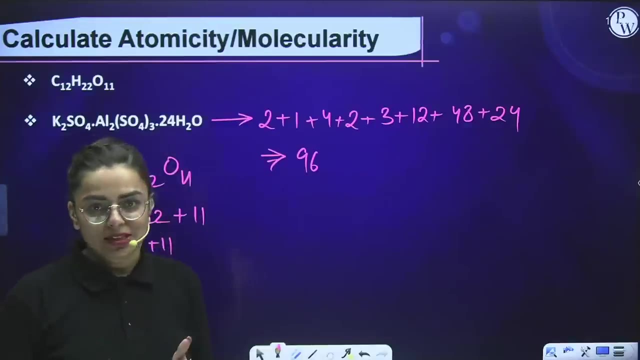 will calculate. it is about 3 plus 4, 7, 6, 7, 8.. It is going to be about 96, right clear. so basically it tells us about the number of atoms present in a molecule, right? so we need to calculate all those elements, the number. 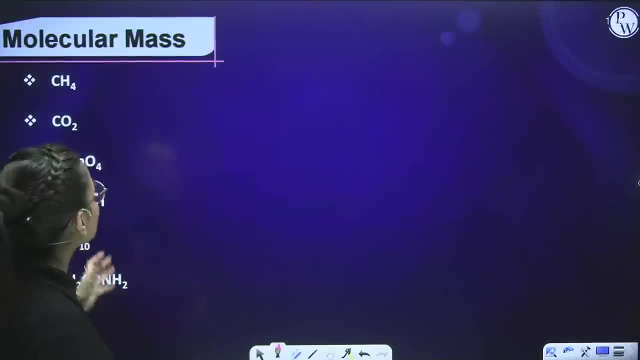 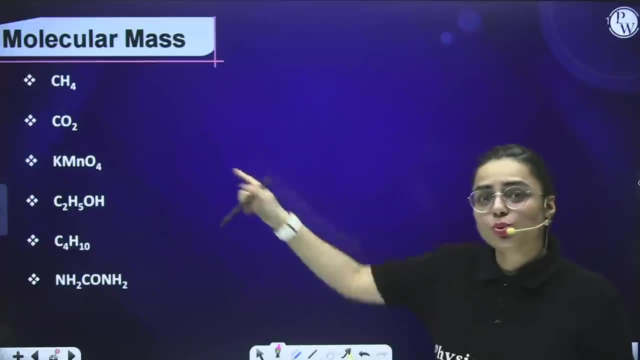 of elements. right now, students, the next thing that comes is the molecular mass. molecular mass is the mass of one molecule. how do we need to calculate it? for this, you need to learn the table which I already told you. You need to individually calculate the number of atoms present in a molecule. 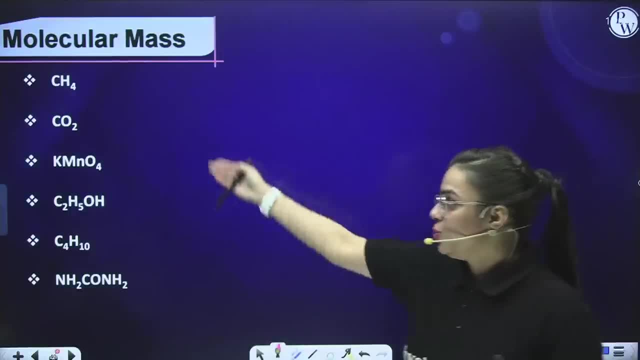 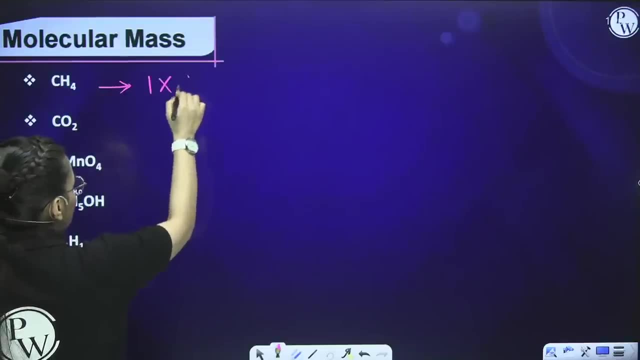 You need to individually learn the elements, gram atomic mass, so that they can. you can apply here and you can solve it now. let us see for the case of CH4: how many carbons are there- 1, so 1 into carbons mass plus how many hydrogen is there- 4, 4 into hydrogen mass by 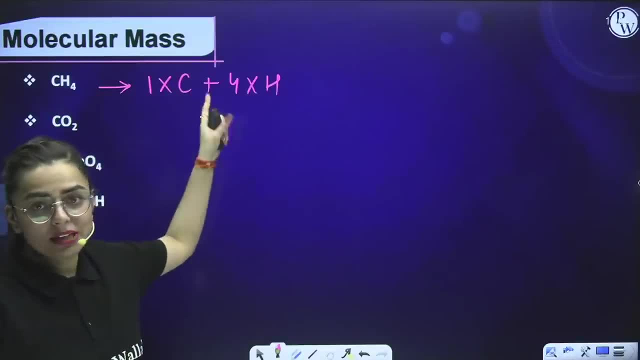 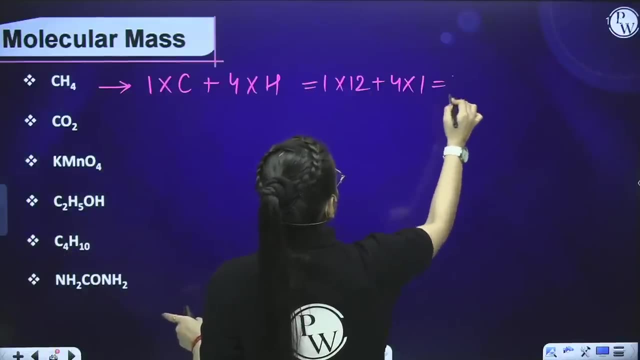 this way you can calculate what was the mass of carbon in the table. it was 12. you can go back and check. so 1 into 12, plus what was for hydrogen, 4 into 1, so it comes out to be 16. so 16 is the molecular mass. 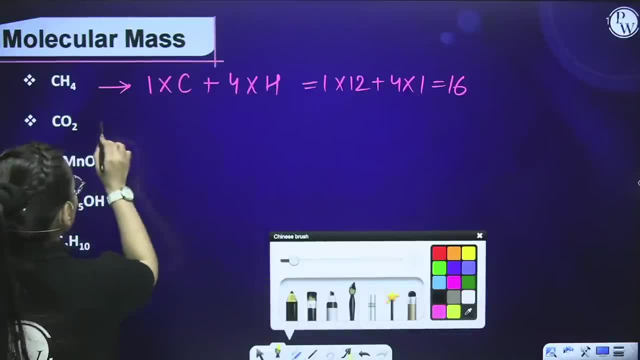 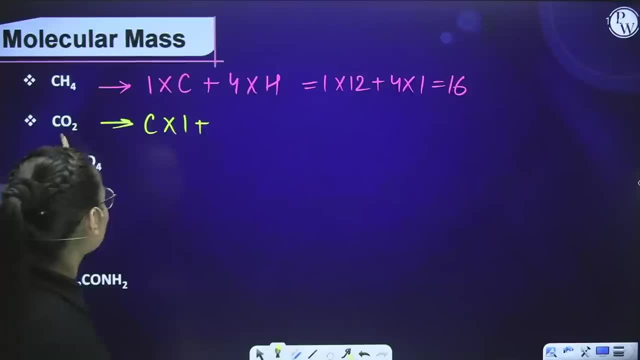 Now coming towards CO2 again, how many carbon are there one? so carbon into 1, that means mass of carbon into 1, because 1 carbon atom is there 2 oxygen atoms are there 2 into oxygen atoms mass. so carbon atoms mass is 12, 12 into 1, plus oxygen mass is 16, 16 into 2.. 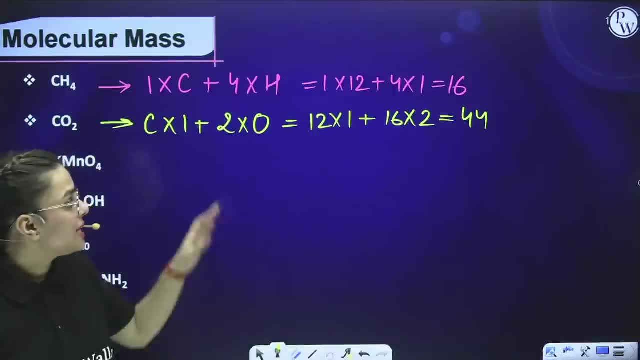 So it comes out to be students. 44 these table. if you have learned, then only you can calculate the molecular masses. Otherwise it will be quite difficult for you. Now. the next table is about carbon and CO2.. Now coming towards KMNO 4.. 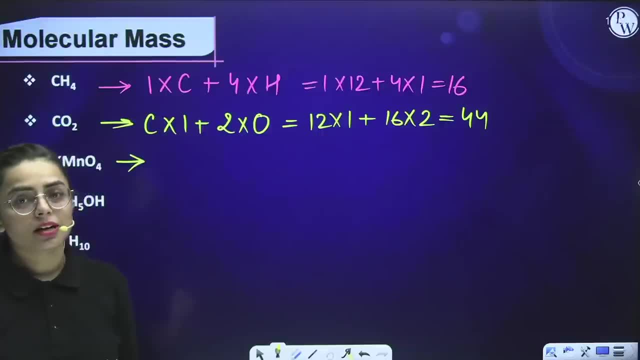 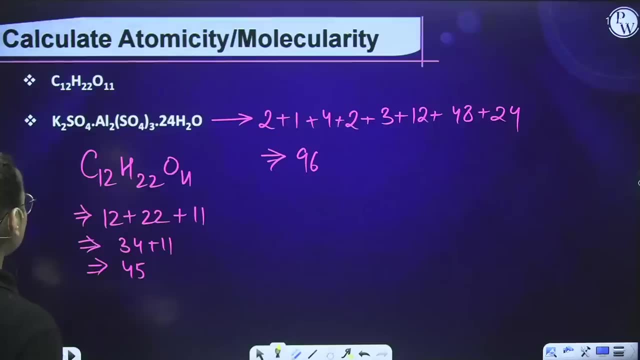 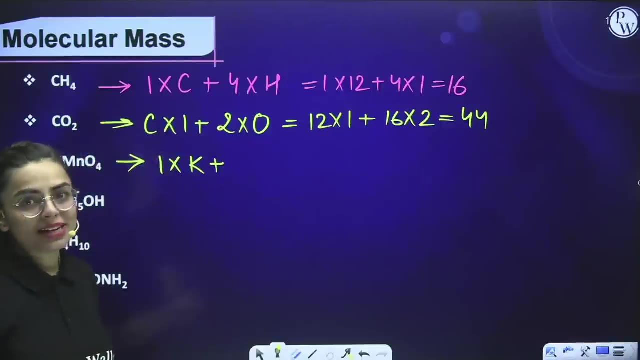 Now, if I talk about KMNO 4 students, then we need to write the masses for potassium as well as Mn right. So the mass for one second, the mass for potassium, is 1 into potassium's mass, plus 1 into Mn's mass, then plus 4 into oxygen's mass, right. 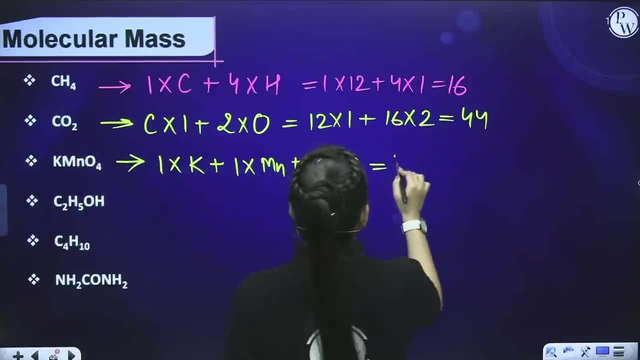 Potassium mass is 39 right. So 39 plus. now comes for Mn mass. it is about 55. then comes for oxygen. that is 4 into 16.. So it is 39 plus 55 plus 64, which comes out to be 94 plus 54. it is near about 158 students. 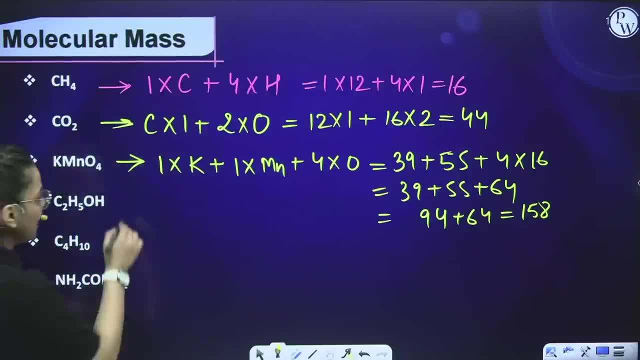 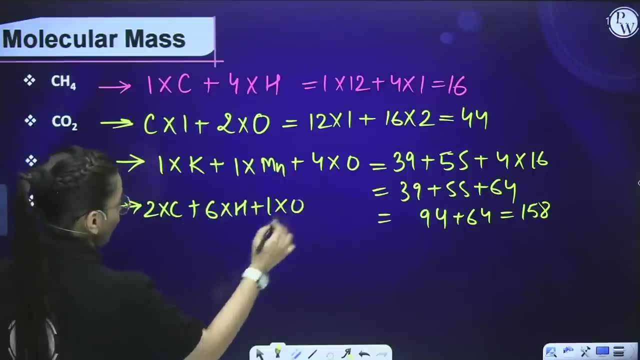 Clear Now: if I talk about C2H5OH, how many carbons are there? 2.. 2 into carbons mass Plus how many hydrogens- 6 into hydrogens mass plus 1 into oxygen mass? Carbon mass is 12.. 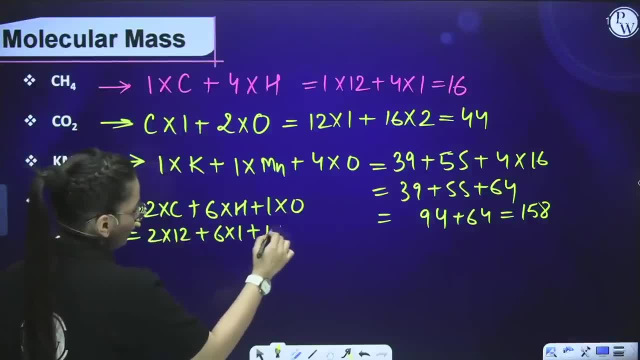 So 2 into 12 plus 6 into 1 plus 1 into 16.. If we solve it out, 24 plus 6 plus 16.. How much students? It is 46.. Clear Now, okay, coming towards a C4H10.. 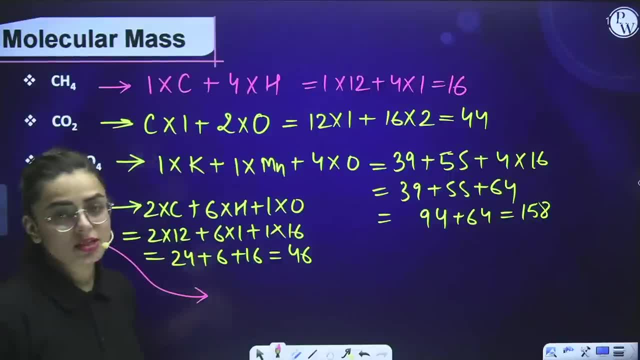 So more, more practice will make you more clear. So first of all, learn the gram atomic mass Individually for the atoms, then apply it here. it will be coming in seconds. Clear C4H10.. How many carbon are there? 4.. 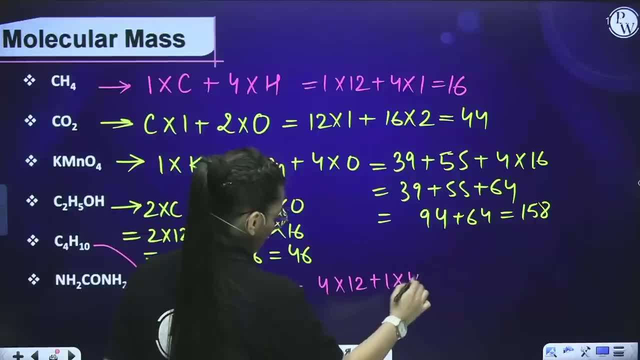 4 into carbons mass plus 1 into hydrogens. number right 1 is the mass of hydrogen. So if we solve it, it is 48 plus 10, that is 58.. Now comes the last part, that is urea here. 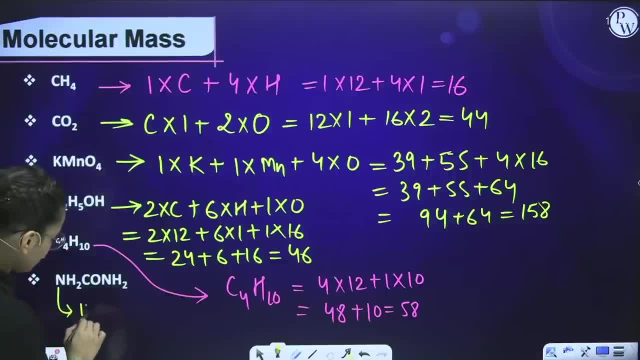 Okay, Nitrogen mass is 14 and here are 2 nitrogens, So 14 into 2, plus There are total 4 hydrogens and its mass is 1.. So directly, I am writing 4.. Carbon is 1, so I am writing 12, and oxygen is 1, so I am writing 16.. 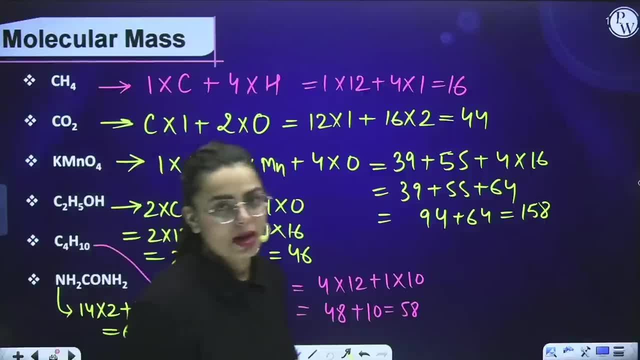 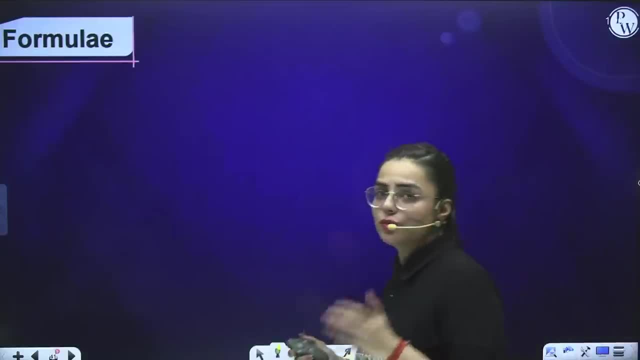 So it comes out to be 60.. So it is the molecular mass for urea Clear. So by this way you can calculate the molecular masses. Now, students, coming towards the formula for the mole concept, that is very, very important. There are 3 basic formulas that you need to apply. 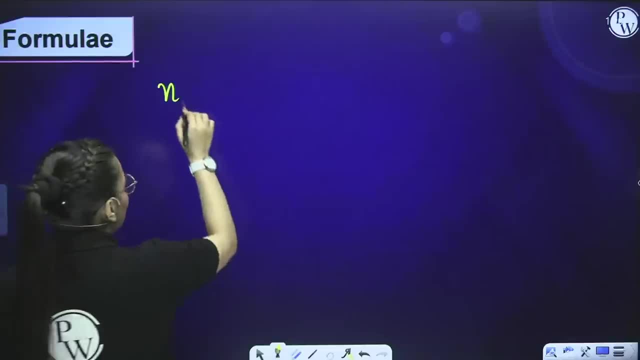 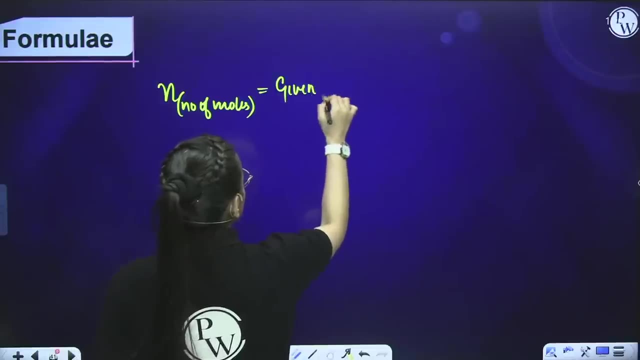 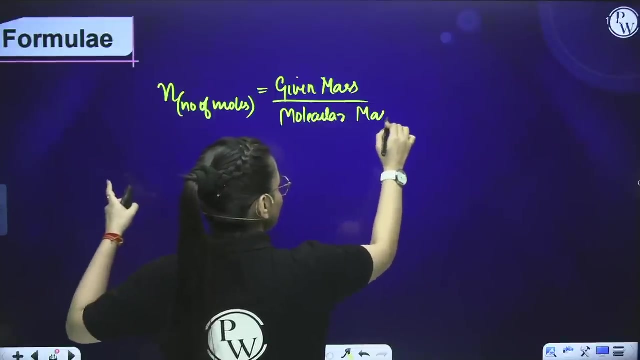 Number 1 is number of moles are represented by small n. It is number of moles which is equal to given mass upon molecular mass. The very first formula, Molecular mass, you have calculated just right now. Given mass, will be given to you in question, right. 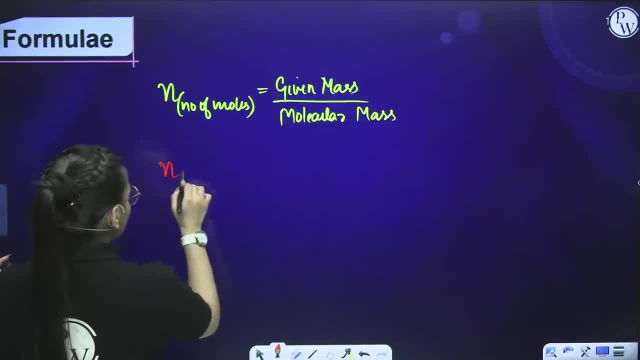 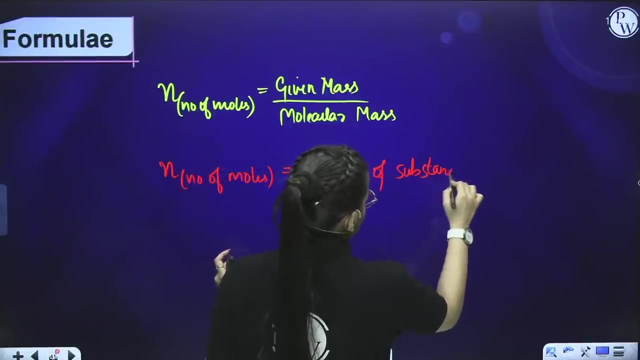 This is the first formula. The very next formula which is important for you is number of moles, in terms of volumes, will be 20.. It will be volume of substance, Substance. it will be volume of substance divided by 22.4.. So this is in the case of when you have given the volume. 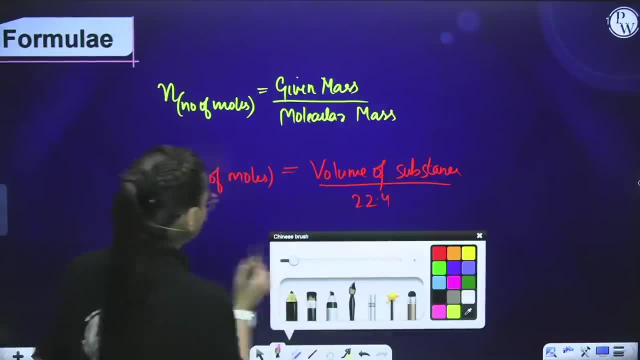 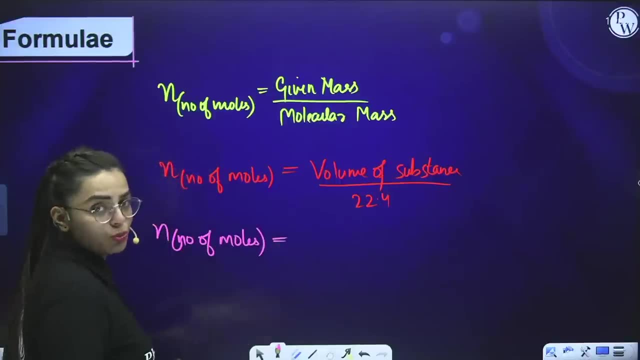 You can apply directly this formula And the very last formula that you use for number of moles, for the case of molecules or atoms. So number of molecules or atoms divided by 22.4.. Evogadro's number, which is 6.022 into 10, raised to the power 23.. 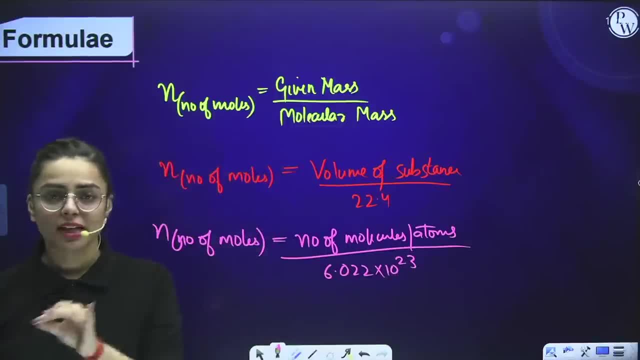 So these are the 3 basic formulas that you are going to apply for the questions. in the case of mole concept, If you have to find the number of moles, you can directly use these formulas according to the given situation. If you are given given mass, then you can calculate this. 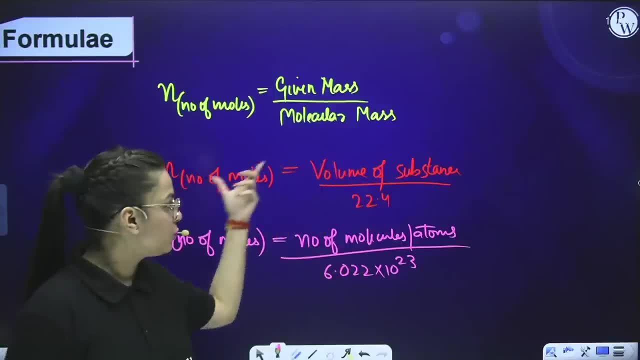 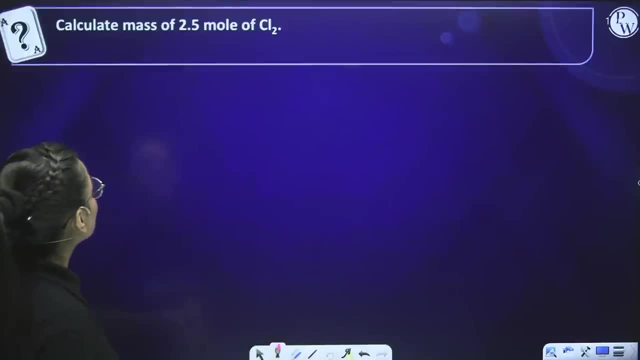 If you want to calculate the volume you are given number of moles, you can use this formula. If you want to calculate number of moles and you are given number of molecules, you can use this formula. Now, students, one question: is there Calculate mass of 2.5 mole of Cl2.. 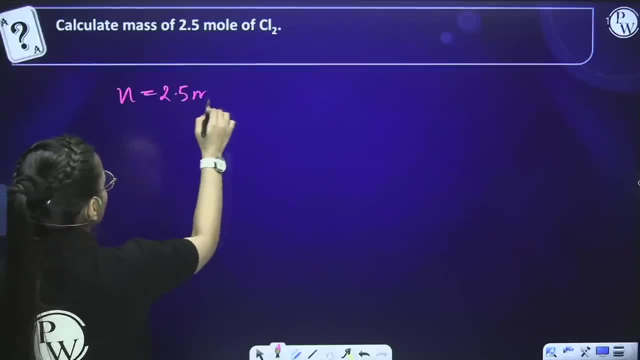 Now number of moles. here it is given 2.5 moles right And we have to calculate the mass of Cl2.. That means, given mass of Cl2 is missing, So we can calculate molecular mass. we have just learnt that Cl2.. 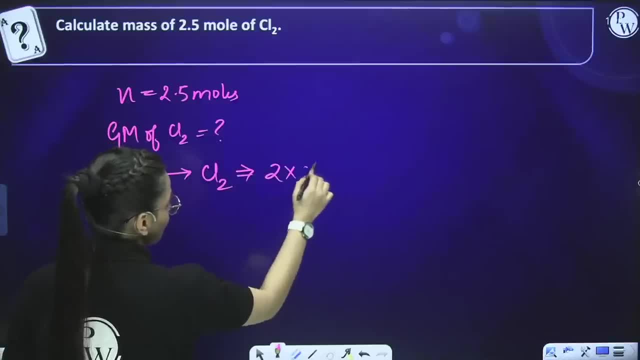 I have told you how many Cl2 into Cl's mass. Cl mass is 35.5, right? So if I solve it, it is 71 students Now after this Number of moles, formula is: number of moles is equals to given mass upon molecular mass. 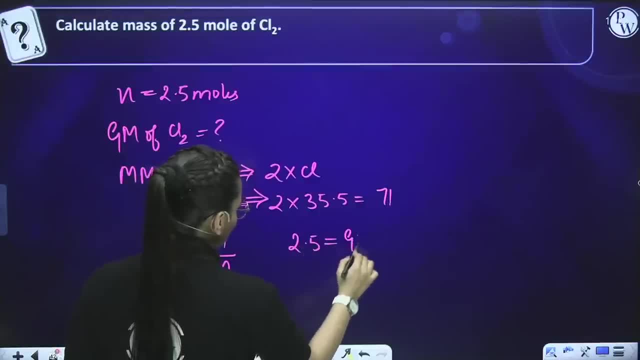 Now, number of moles is 2.5, given mass we need to calculate, and molecular mass is, students- is 71.. Now when we cross, multiply it, it comes out to be 177.5, clear. So let me calculate it in detail so that it is easy. let us check first, I guess. 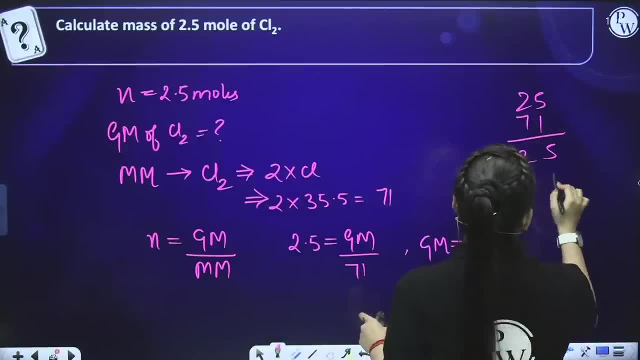 Ok, 177.5, 2. yes, it is the same, 177.5, clear. ok, now it will come grams, because we are taking it in grams, right? Ok, students, now let us see the flow chart. flow chart here is to represent the 3 basic. 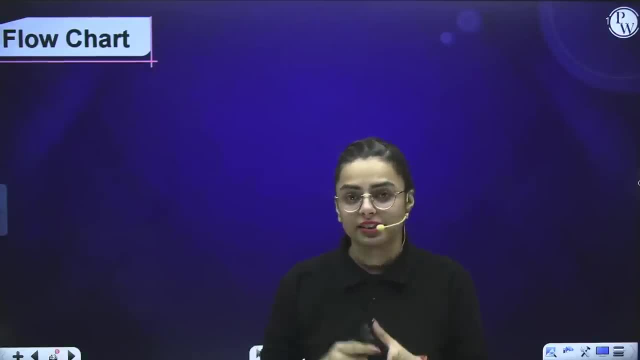 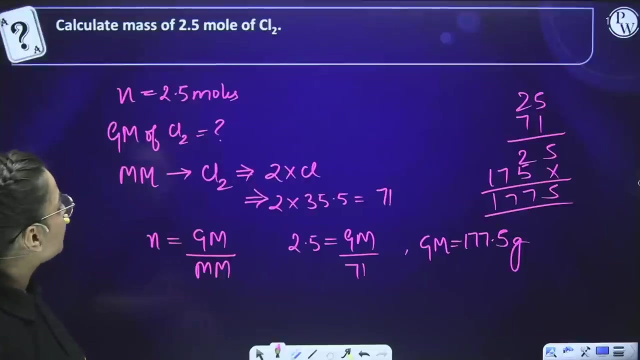 formulas how 3 basic formulas can be correlated with each other. see: if you are given given mass And you are asked to calculate number of molecules, you can directly use this formula to calculate how I have used this formula. ok, I will tell you about this slide. see number. 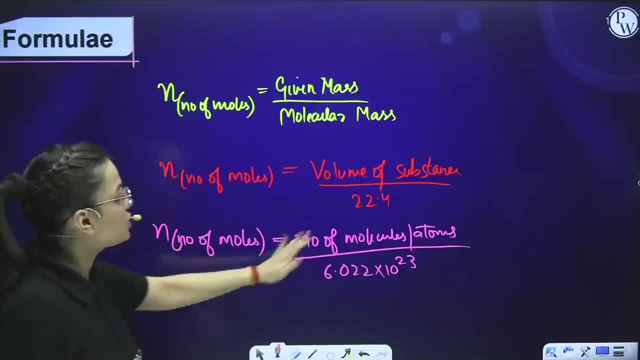 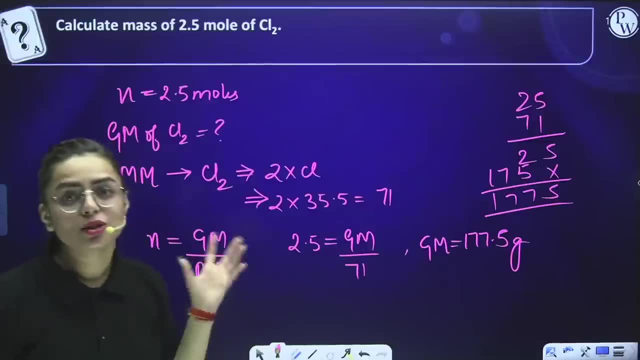 of moles is equal to given mass upon molecular mass. also, number of moles is equal to number of molecules divided by Avogadro number. So if left hand side is equal, we can put the right hand side equal. so this is the core relationship of these formulas which we can apply. 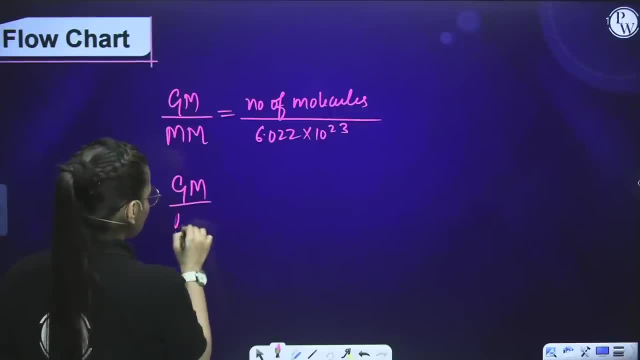 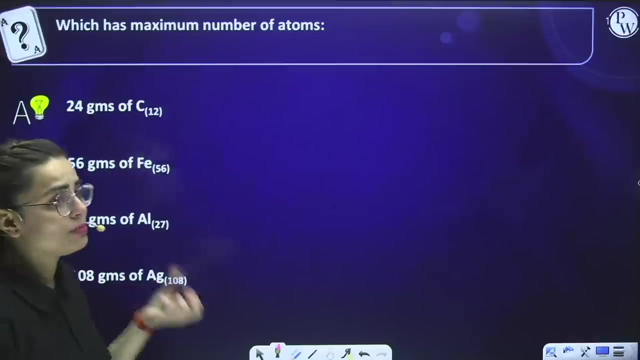 Another with the volume. also, you can do the same, given mass upon molecular mass is equals to volume of substance by 22.4, right, students? so this you can use as a correlation of the 3 basic formulas of mole concept. Now, students, next comes our question: which has the maximum number of atoms? now let us 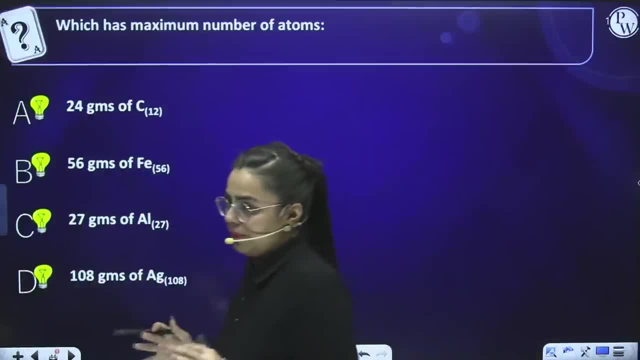 see that The first case is 24 grams of carbon. In the case of 24 grams of carbon, we have 24 grams of carbon. In the case of 24 grams of carbon, we have 24 grams of carbon. In the case of 24 grams of carbon, how many number of atoms are present? now see what is. 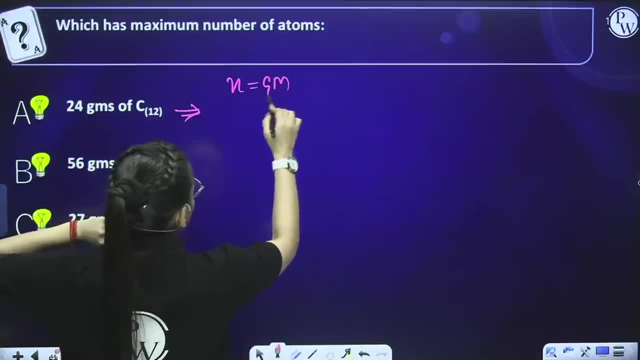 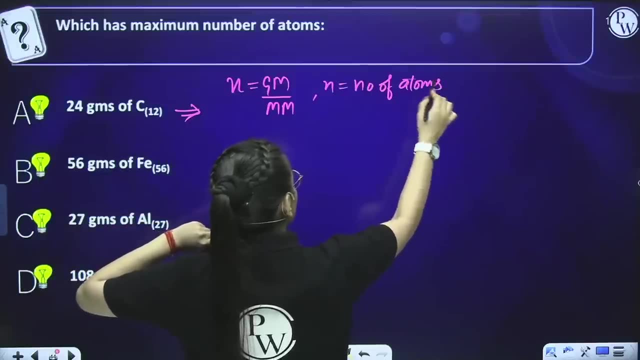 the formula of number of moles. number of moles is given mass upon molecular mass, and also number of moles is equals to number of molecules or number of atoms divided by Avogadro number, that is, 6.022 into 10 raise to the power 23.. 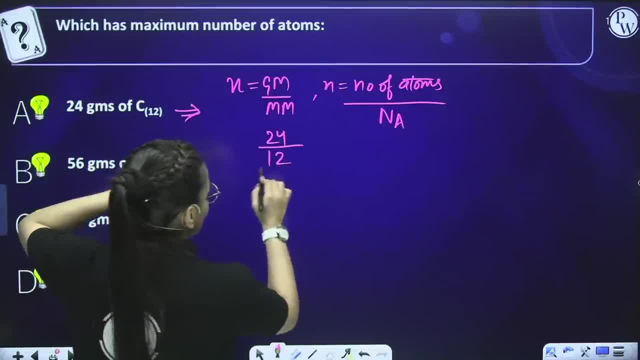 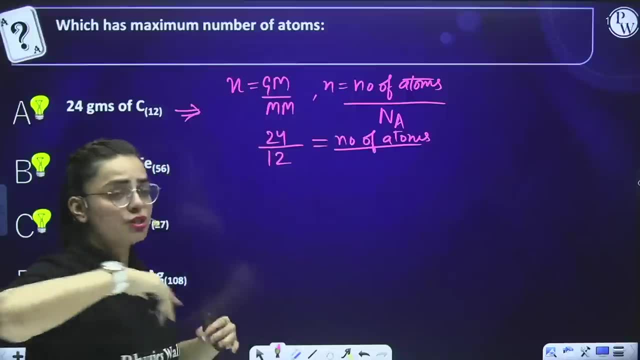 So here, given mass is 24, molecular mass of carbon is 12 is equals to. we need to calculate number of atoms. Do not write the number of atoms. Do not write students Avogadro number in the full form, like 6.022, into it will be very 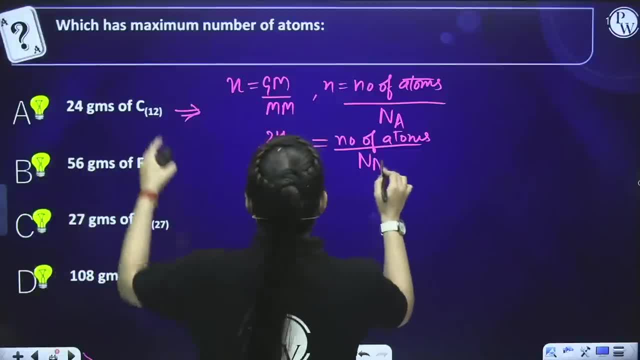 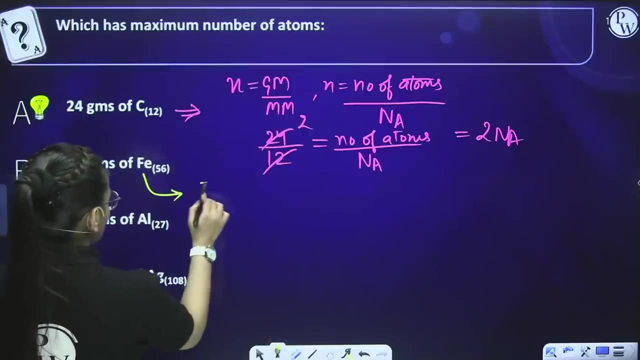 complex. so just write it as n a, because we need to compare it right. so when we divide it it is 2, it is 2 n a. so for the first case, number of atoms that came out is 2 n a. Now for the next case. now, for this case it is given: mass is 56, molecular mass is also. 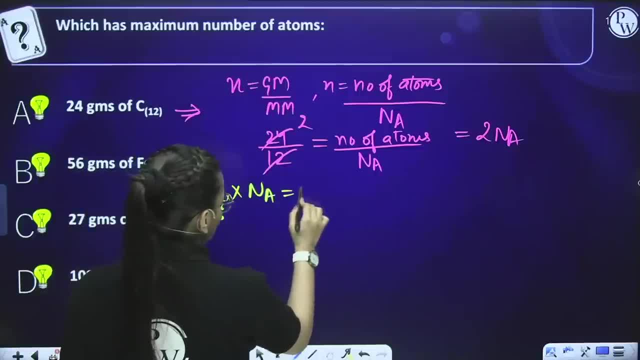 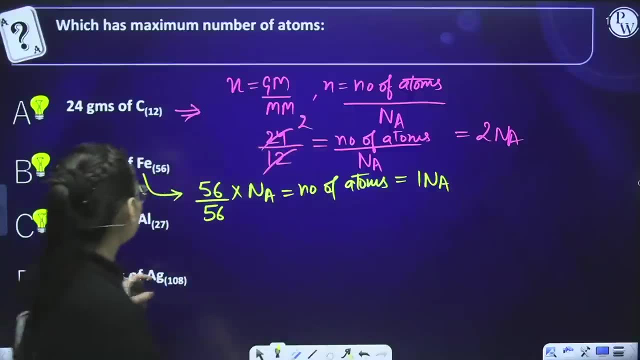 56 into n? a will be equal to number of atoms. Now for the next case. now, for this case, it is given mass is 56, molecular mass is also 56 into n? a will be equal to number of atoms. Hence it comes out to be 1 n a, right, ok. now the third is aluminium: 27 grams of aluminium. 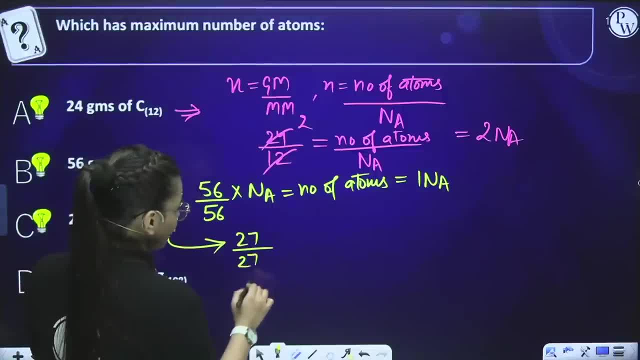 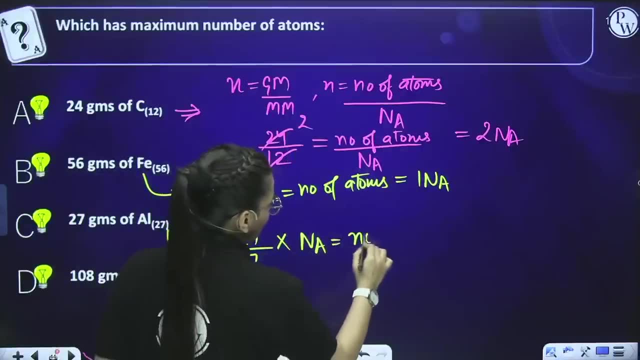 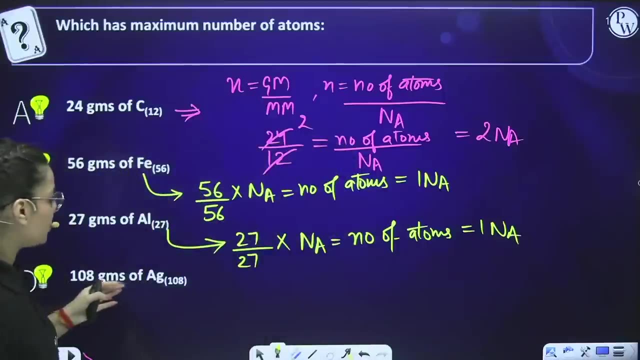 given mass is 27 and aluminium mass is also 27 right, and when we will cross, multiply according to this formula into n? a, it will give us number of atoms. hence, students, it's come out to be 1 n? a, and the very last one we have 108 grams of Ag. again, given mass is 108 molecular mass. 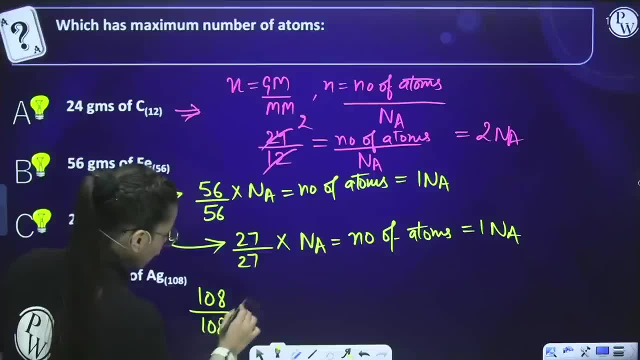 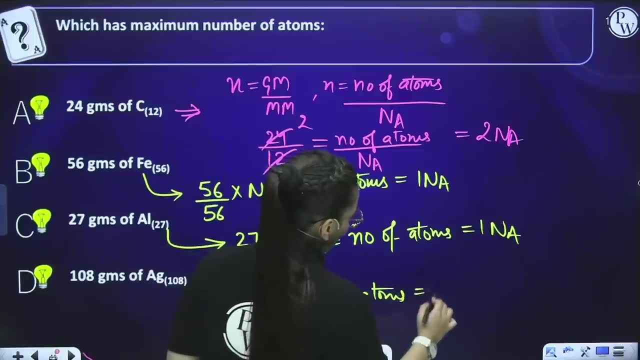 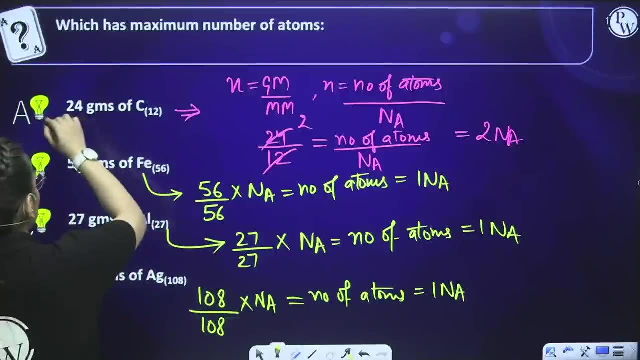 is also 108 grams. Molecular mass is 108 into. we will do n a right to get number of atoms. so it again comes out to be 1 n a. so, students, what we have done here is we need to find the maximum number of atoms, and we have found the maximum number of atoms in the case a, which is 2 n a clear. 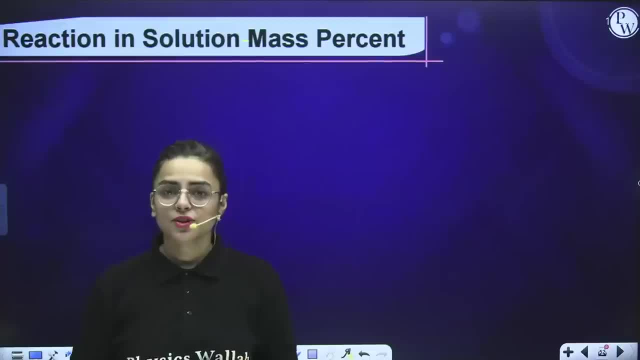 now we will proceed towards our next topic. So yes, my dear students, now we are going to start reactions in solution. we are going to see the concentration terms. So the very first thing we are going to do is we are going to see the concentration terms. 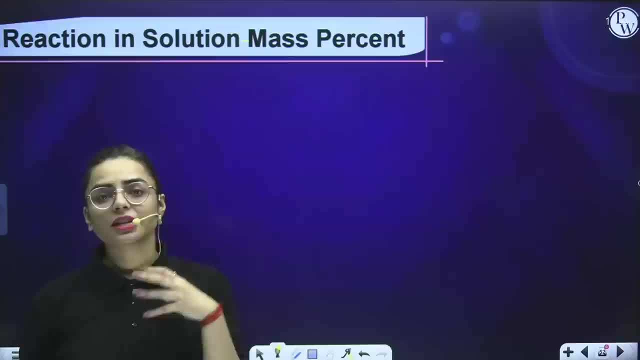 So the very first term is mass %, mass % or mass %, or in other terms, we defined it as weight by weight %. how do we calculate it? according to the name mass %, that means there is a relationship between mass right. so the definition for mass %, or I would say weight by weight %, is that. 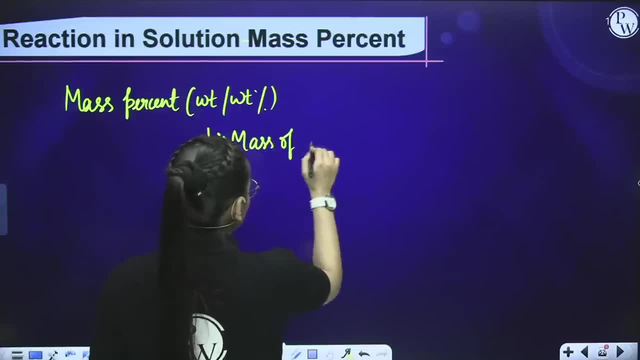 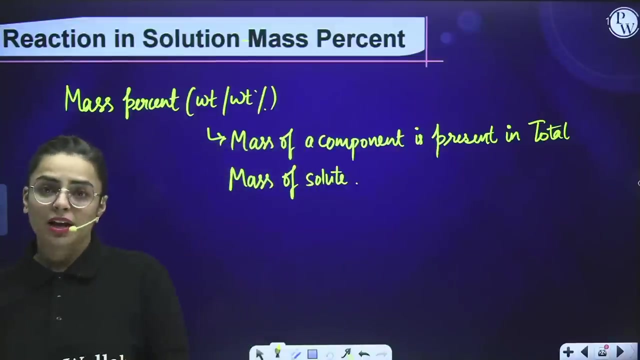 mass of Accumulated Weight, component that we need to calculate is present in total mass of the solution. It defines us that how much mass of the component is actually present in the total mass of the solution. If I define its formula, what would be the formula of weight by weight percent? 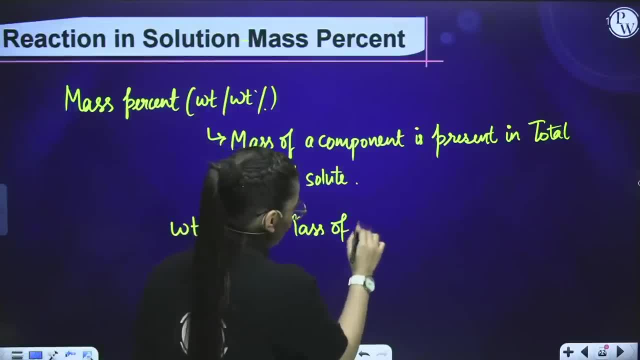 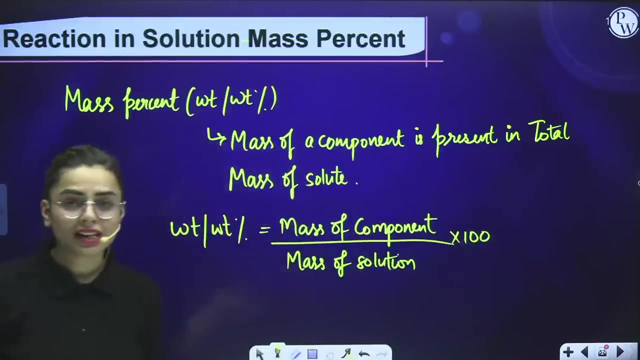 It is refers to add mass of component divided by mass of solution into 100.. If I speak in terms of solute and solvent, what do you mean by solute and solvent, Students? solute refers to the substance which is present in the total mass of the solution. 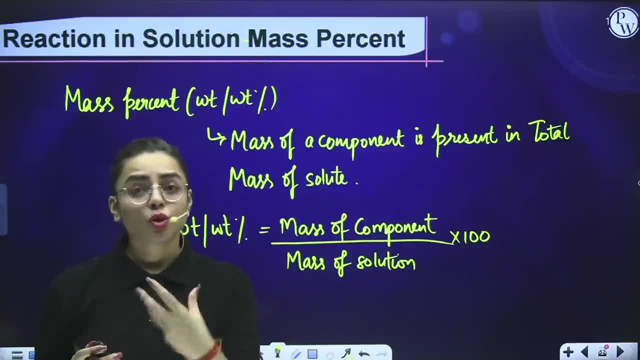 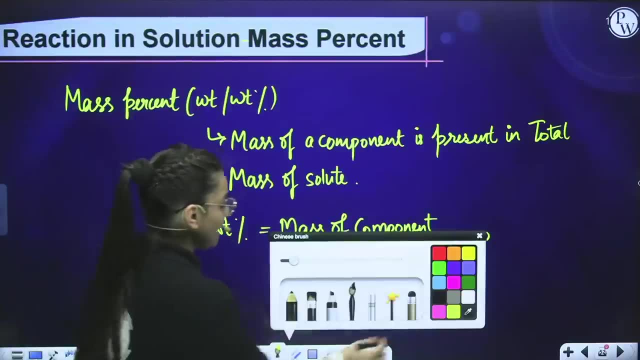 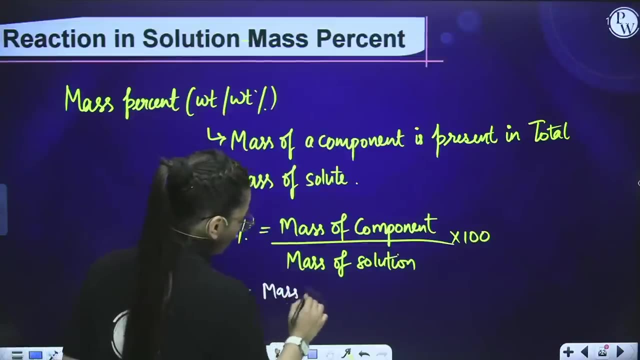 It is present in less amount and the solvent is the one which is present in the more amount Solute and solvent comprises to form solution. So if I speak in that terms, I would define mass percent or weight percent as mass of solute divided by mass of solution into 100. 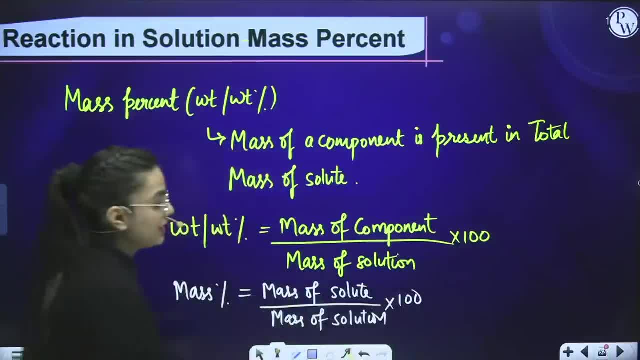 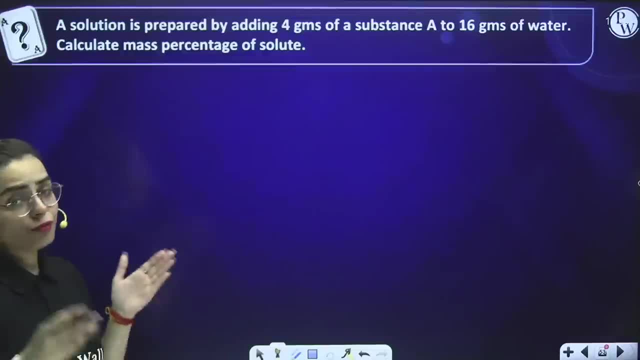 Why do we multiply this into 100?? Because we are calculating this In the terms of percentage. That's why. So now let us see one question. A solution is prepared by adding 4 grams of a substance A to 16 grams of water. 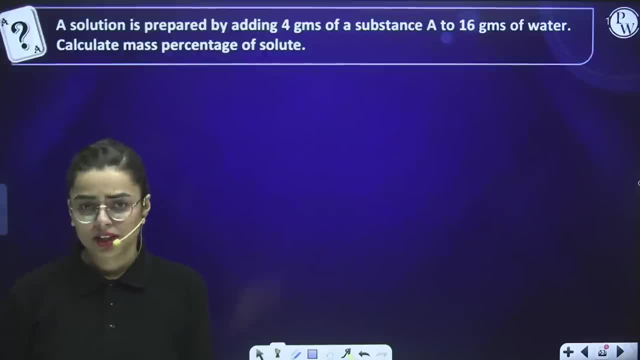 Calculate the mass percentage of solute. It is very simplest question, students. Here we need to calculate the mass percentage of solute. As I told you, the mass of solute is always present in less and the solvent is more Like the one that is being dissolved is solute. 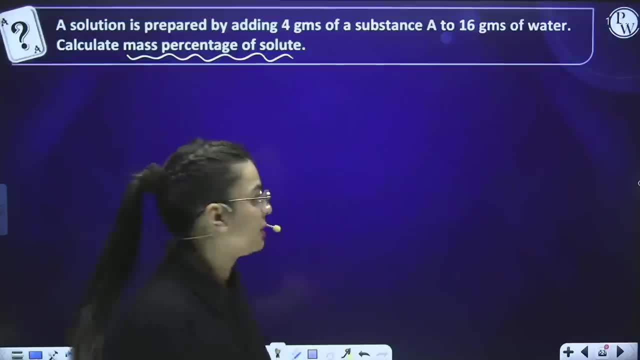 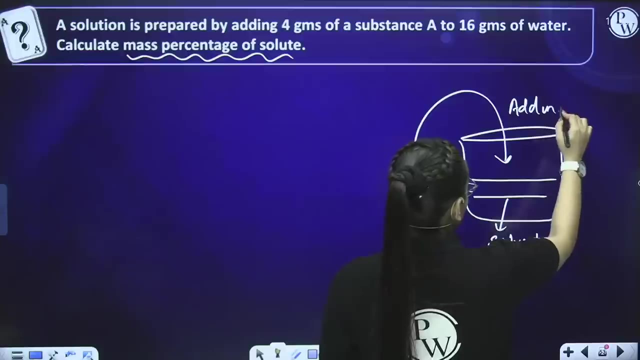 And into which It is being dissolved is solvent, For example. let me explain you in detail. This is my beaker: It contains solvent. Now, the thing that I am adding from above is known as solute. So when solute is being added into solvent, it refers to as solution. 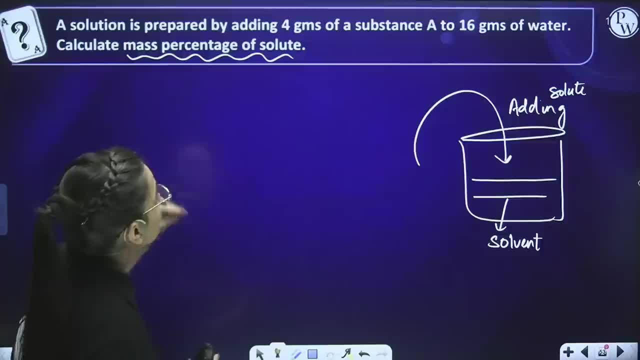 It consists of solution. They are asking us to calculate the mass percentage of the solute that is being dissolved. That means they are asking about the mass percentage of the substance A that is being added into the solution. So what is the formula? Its formula is mass percent or weight by weight. percent is equals to mass of component, which is the component A: 4 grams mass. 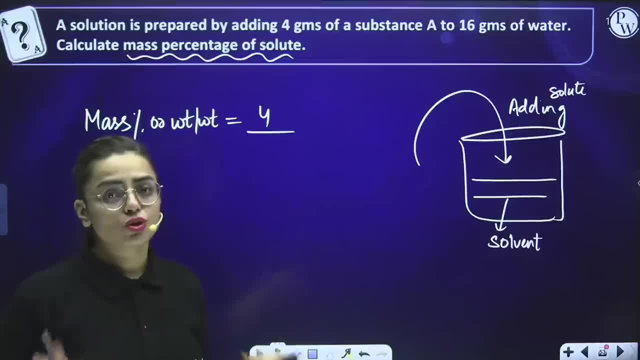 Divided by mass of solution. Now solution comprises of both solute and solvent. That means 4 grams of substance A plus 6 grams of solute Plus 16 grams of water will make a solution Into 100.. So it is 4 by 20 into 100. 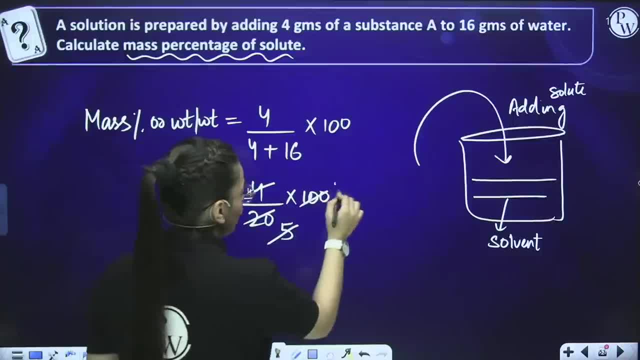 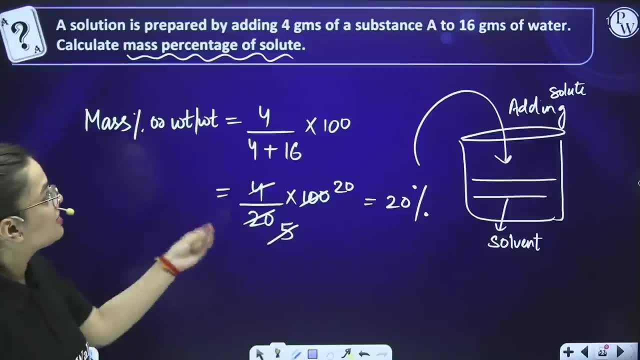 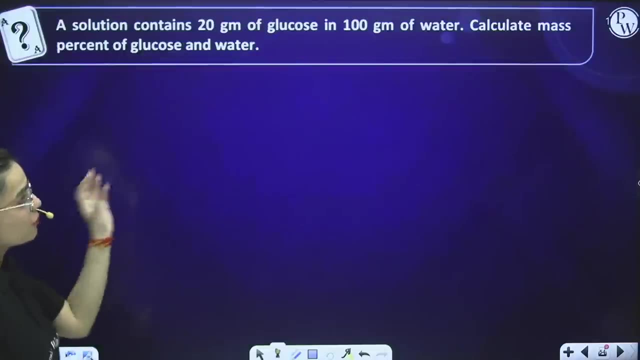 Now, 4 x 5 is 20.. 5 x 20 is 100. Hence, answer is 20%. That means the mass of the solute is 20%. It was an easy question. It was an easy formula. So now, students, we are considering one more example here. 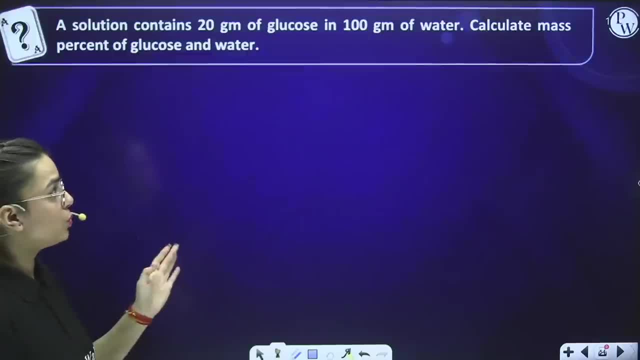 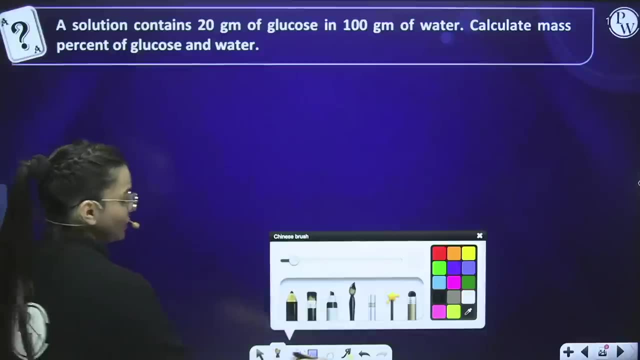 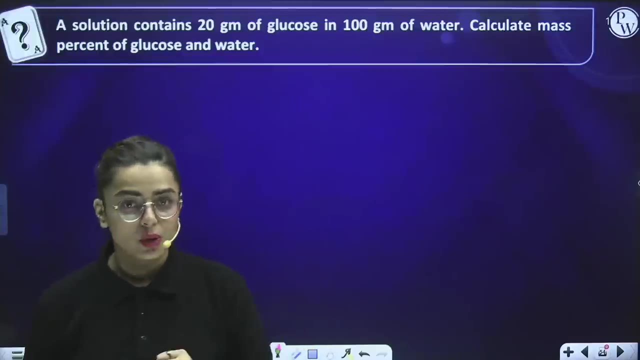 See. A solution contains 20 grams of glucose in 100 grams of water. Calculate mass percentage of glucose as well as water. Now, see, we need to calculate the mass percentages of both the components of glucose as well as of water. So the first formula will work here. 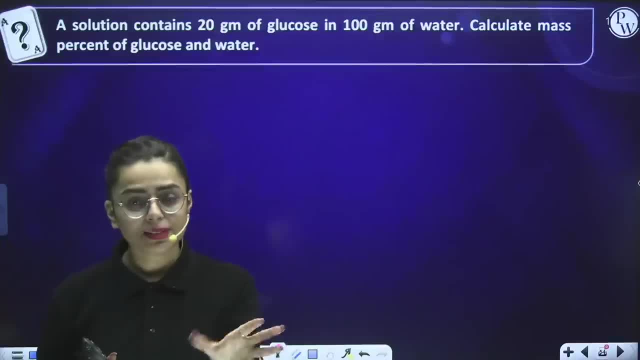 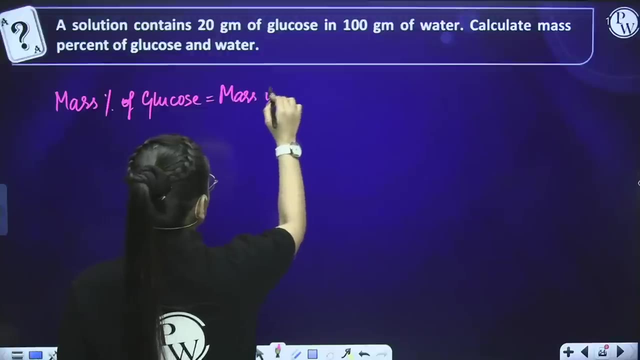 Like the component whose mass you have to calculate, divided by total mass into 100. So it is as simple as that. First of all, you need to write the mass percentage of glucose. To calculate the mass percentage of glucose, you need to calculate the mass of glucose upon total mass of the solution. 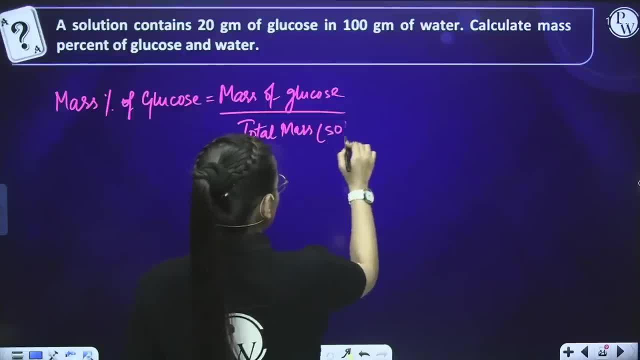 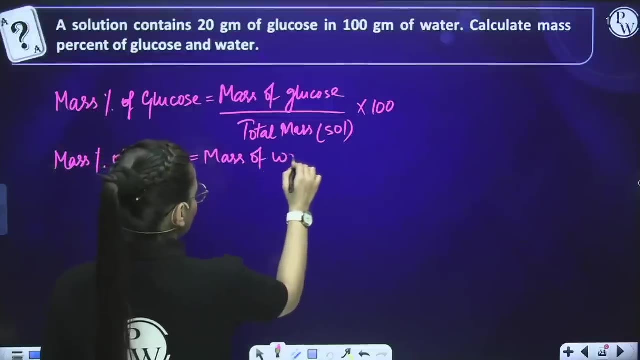 Total mass of the solution and into 100.. This will calculate for glucose. Now, if I ask about mass percentage of water, what will be the formula? It will be mass of water divided by total mass, Divided by total mass of solution, students into 100. 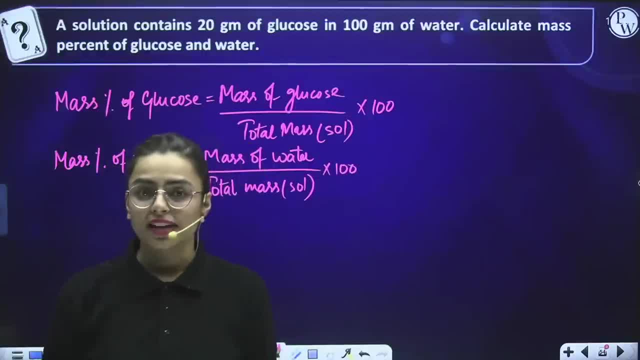 Now the component, whosoever you want to calculate, should be kept on the above, on the numerator and on the denominator. always you have to put the total mass of solution. Please remember that you have to put of solution, not of the particular solvent. Sometimes students only write what is given in the question. 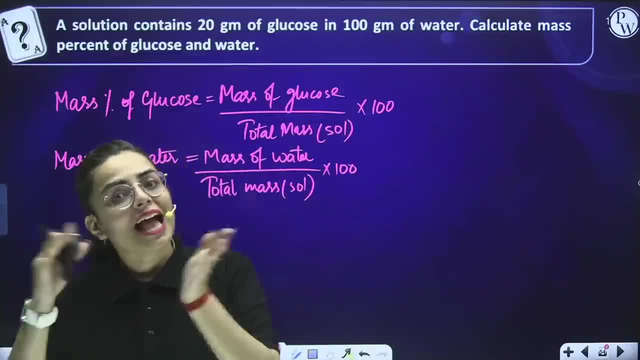 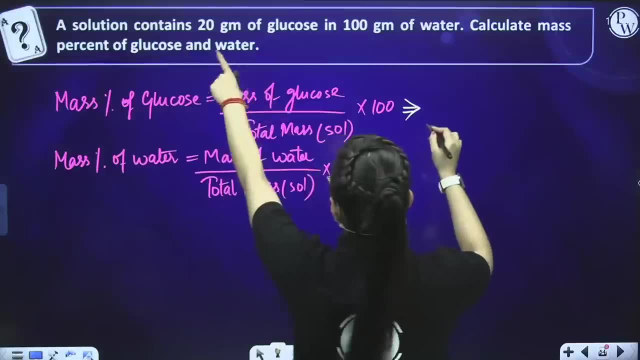 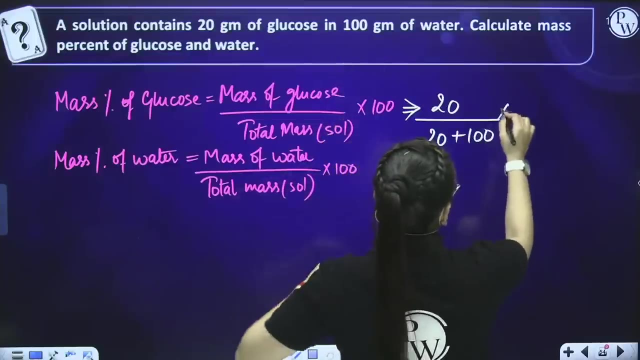 Don't forget that solution is consisting of solute as well as solvent, Right? So now, if I put into these situations here: mass of glucose is given 20 grams and solution mass is going to be the addition of both of them, That is, 20 plus 100 into 100. 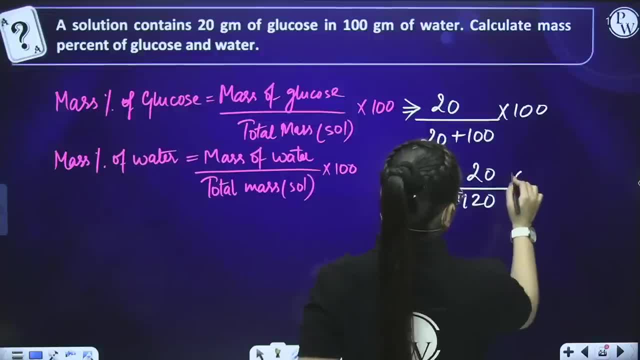 So when we solve it, it is 20 by 120 into 100.. Right, I am cutting the zeros. Then two, six are 12.. Here I am getting 100 by 6, which is going to be 16.67 percent something. 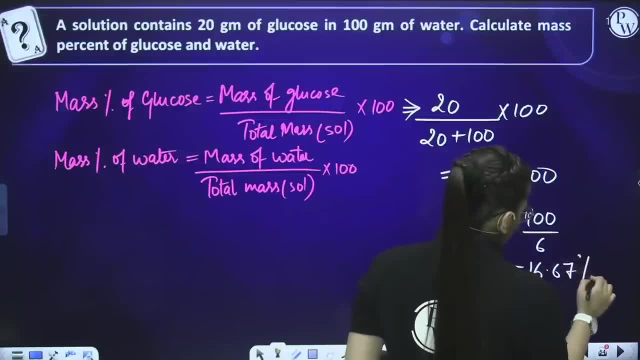 It is 16.67 percent. So the percentage mass of glucose is 16.67 percent. Now I am going to calculate the mass of water. So the mass percentage of water is mass of water divided by total mass into 100 students. 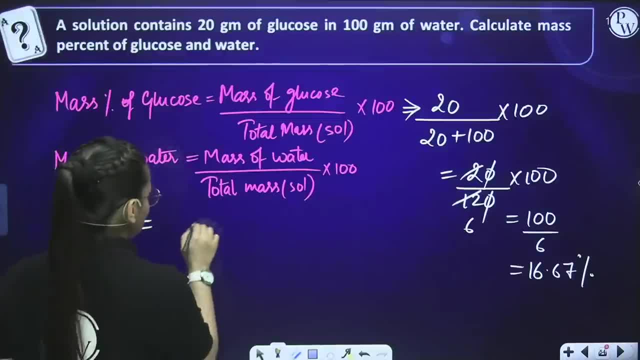 So the mass of water, what it is- 100 grams given in the question- Right students, It is already given to us in question- Divided by total mass of the solution. Solution consists of solute as well as solvent, So we need to add both of them. 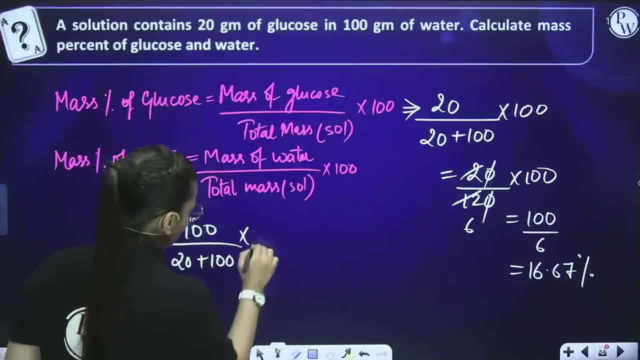 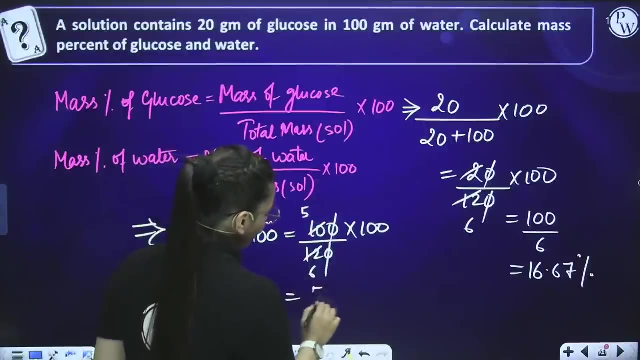 That is 20 plus 100 into 100. So here what I get: 100 upon 120 into 100.. Again, one zero is cancelled with other zero. Now, if I cut it on the table of two, It is 500 by 6 students. 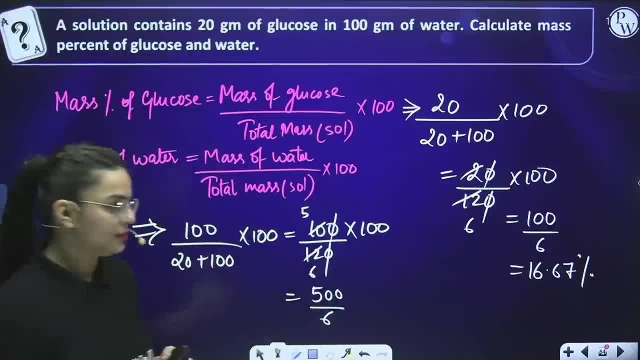 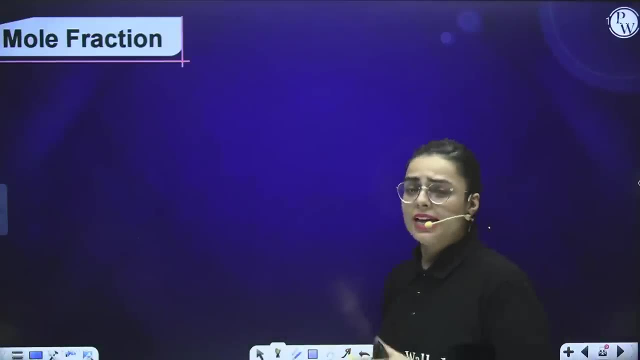 So I am getting it 83.33 percent, something Right. So this was all about the mass percentage question. Now, students, we are moving towards the next concentration term, That is referred to as mole fraction. It is the most simplest concentration term, I would say. 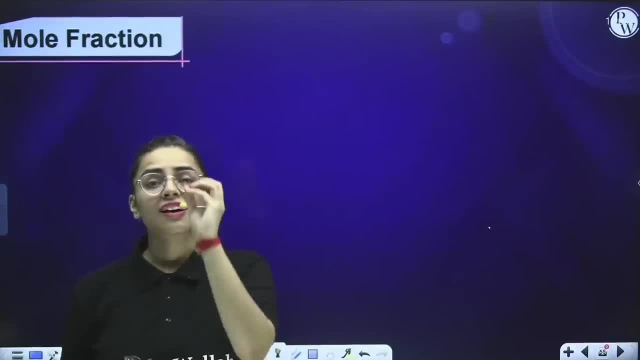 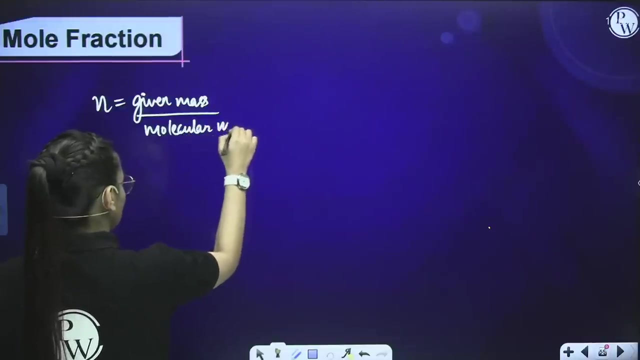 Mole fraction. What do you mean by mole fraction? First of all, understand this. What is moles Moles refers to as given mass, Given mass upon molecular mass, Right. Okay, Now to define mole fraction in detail and to discuss about moles in detail. 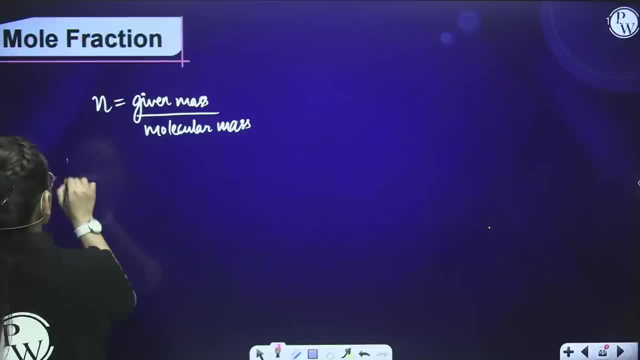 Students, first of all, you need to understand about mole fraction. Mole fraction is represented by zeta. It is equals to number of moles of substance A Divided by Number of moles of substance A plus number of moles of substance B. 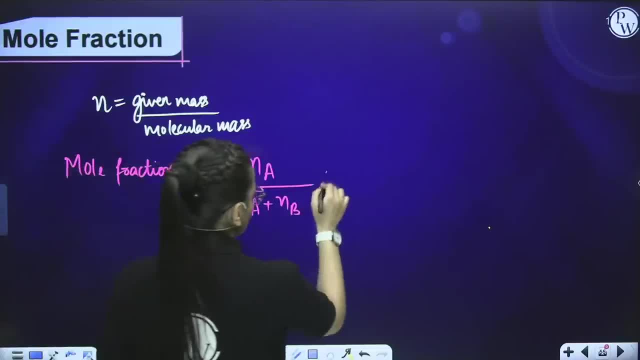 That means total substance moles into 100. Right? So, students, I am considering that there are two beakers, or it is divided into like half of the category. So one contains A particles, another contains B particles. Now if I have to calculate how much is A particles present in that beaker? 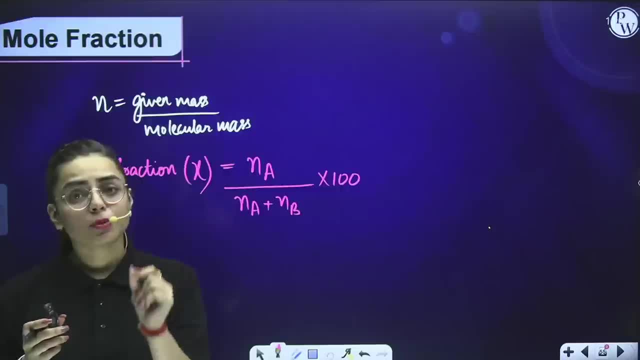 I need to calculate number of moles. To calculate number of moles for the particular component, you have to keep the number of moles of that component on the above position, and it should be divided by total number of moles. So hence, if I have to calculate the mole fraction of A, I will keep number of moles of A above. 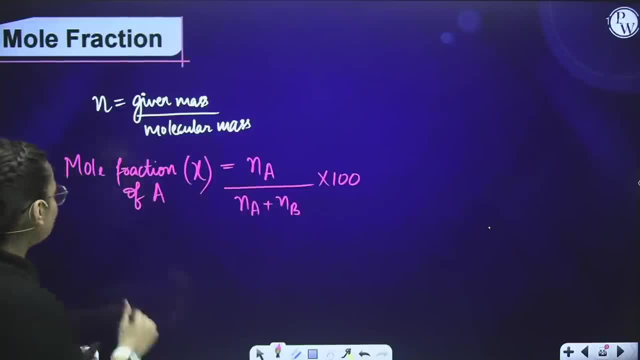 divided by total number of moles, into 100.. Right Now, moving towards the mole fraction of B, What will be the formula? Number of moles of B divided by total number of moles, Divided by total number of moles into 100.. 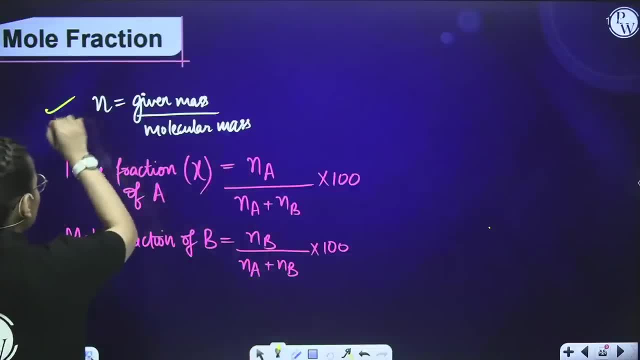 Now I have already written this formula also in case in some of the questions what happens is there are: they don't give you directly moles, they give you given mass as well as molecular mass. So first of all you need to calculate number of moles with the given formula: given mass. 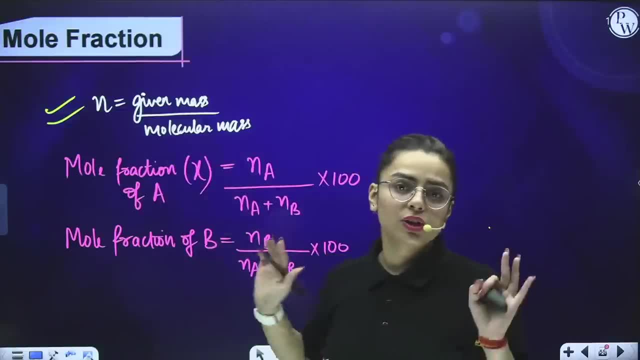 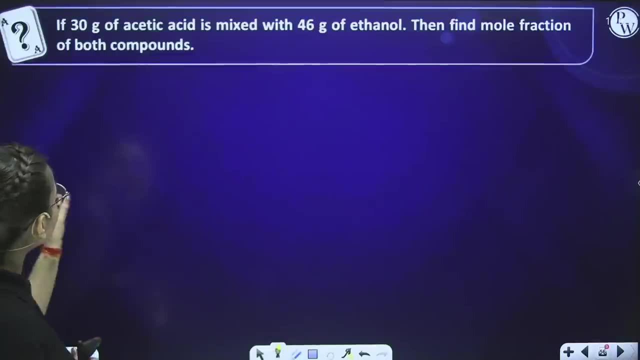 upon molecular mass, and then you need to apply into the following formulas: That's it, students. So students, now let us see an example for this. If 30 grams per kilogram Right Of acetic acid is mixed with 46 grams of ethanol, then find mole fraction of both the 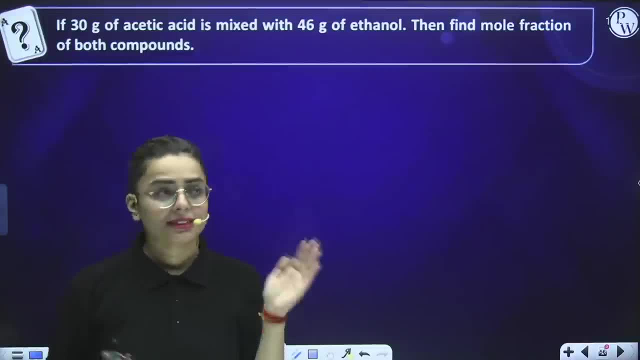 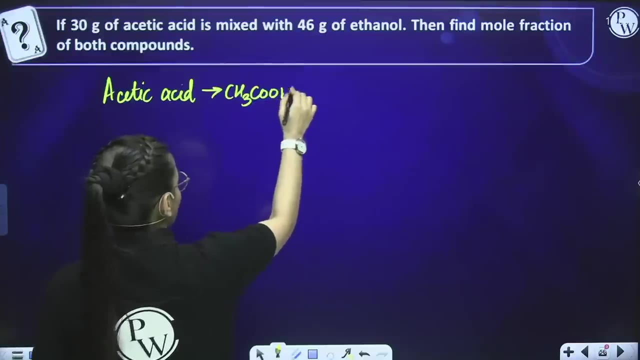 compounds. Now for A as well as for B, That means for acetic acid as well as for ethanol, we need to calculate the mole fraction. So first of all, acetic acid is CH3COOH Right And ethanol formula is C2H3COOH. 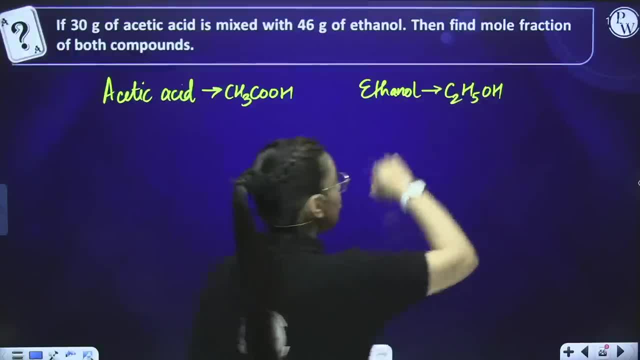 No need to worry that, ma'am, we don't know the formula. no need to worry. In organic chemistry, when you will come across the chapters, you will learn these concepts also. what is the formula? how is the composition? you will get to know in that terms. 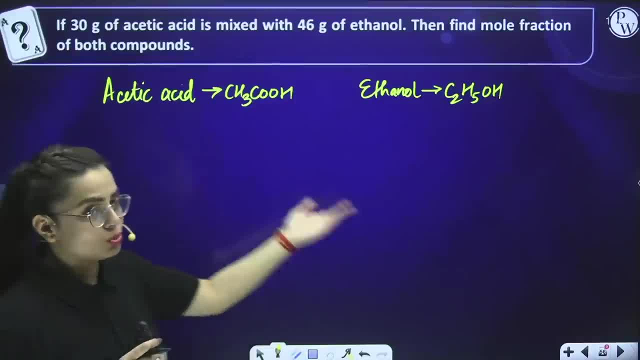 First of all, I am already telling you, because you are new to these terms, Right? So acetic acid is CH3COOH, while ethanol is C2H5COOH. now we need to calculate the mole fractions. So first of all, we need to calculate the molecular mass. 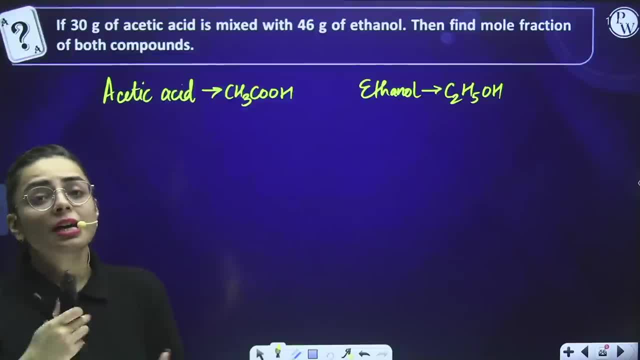 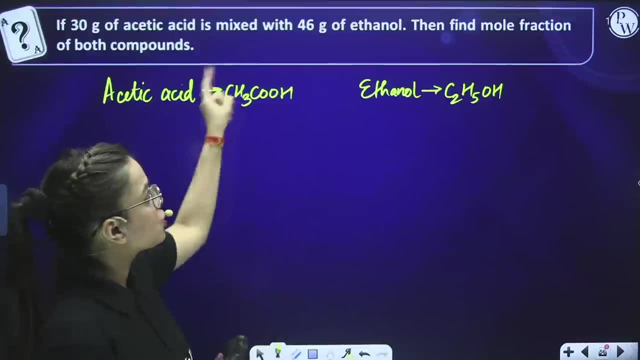 Why I am saying we need to calculate molecular mass? because students here, number of moles are not given to us directly. So first we need to calculate number of moles for the particular components and for that given mass is already given in the question. Now we will calculate the molecular mass, students. 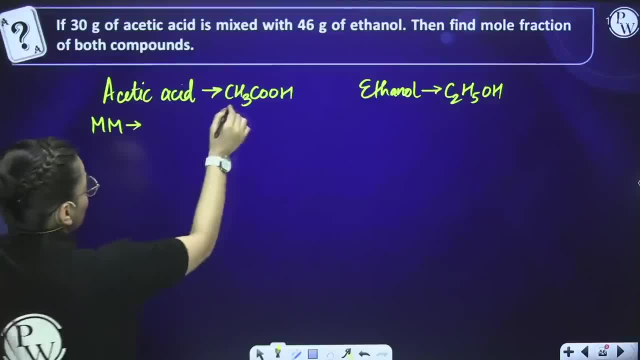 Right To calculate the molecular mass. what we are going to do see how many carbons are there: 2 carbons, 2 into carbons. mass, that is, carbon mass, is 12.. Plus how many hydrogen? 4. 2 into hydrogen mass. 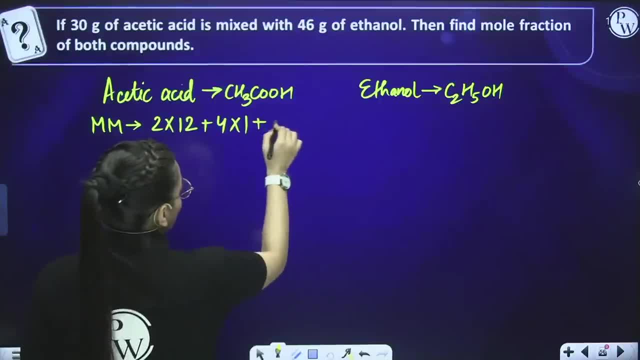 Hydrogen has 1.. Right Plus 2 oxygen atoms into 1 mass of oxygen atom is 16.. So what will be the molecular mass? 24 plus 4 plus 32, that is going to be 28 plus 32. that means it is 60 grams. 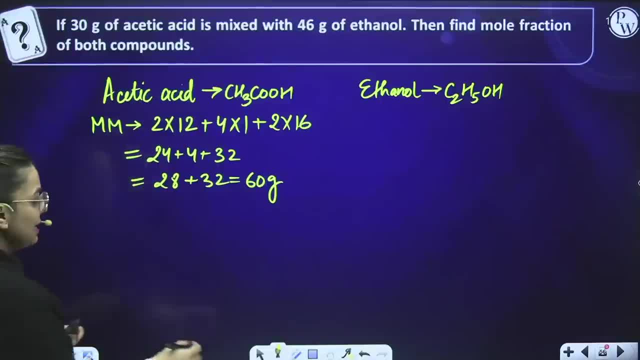 This is the molecular mass for acetic acid. Now let us calculate its number of moles. Number of moles for acetic acid is given mass, Given mass upon molecular mass. What is the given mass in the following question? 30 grams divided by molecular mass is 60.. 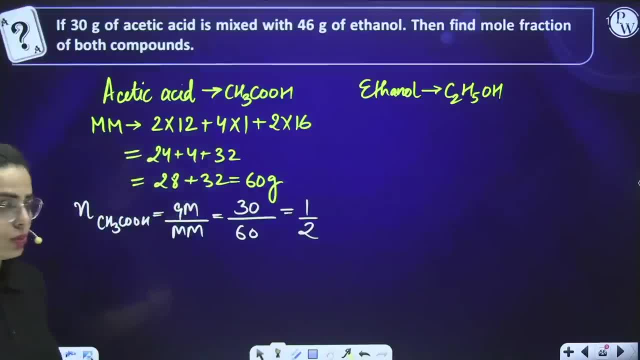 So I am getting number of moles as 1 by 2.. Right Now, moving towards the ethanol portion. first of all we need to calculate the molecular mass. What will be the molecular mass for this? How many carbons 2.. 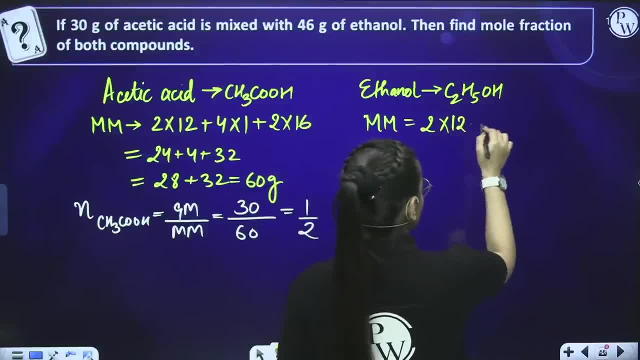 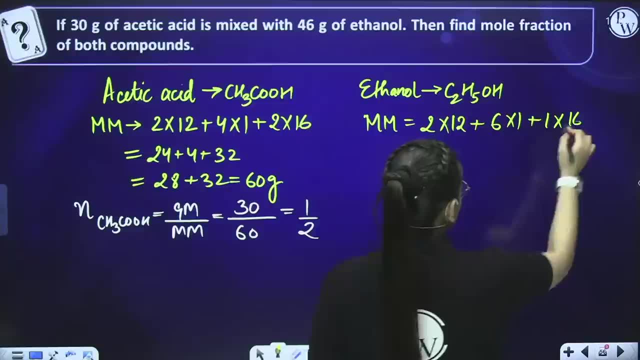 The mass for 1 carbon atom is 12.. So we will multiply it with 12.. Plus how many hydrogen, 6.. The mass of hydrogen plus 1 into oxygen's mass, that is 16.. So it is going to be 24 plus 6 plus 16, that is going to be 46 students. 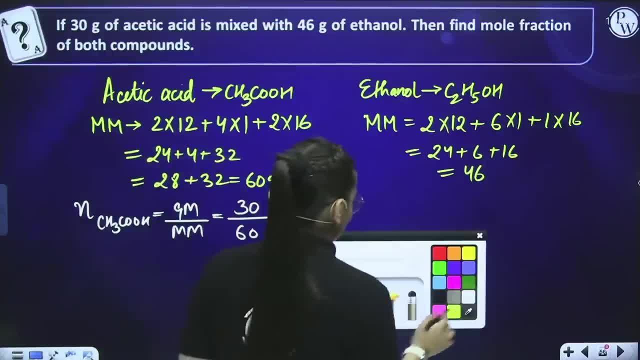 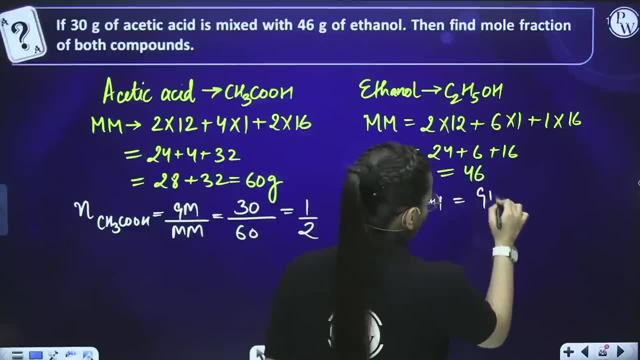 So this is the molecular mass for ethanol. Now we will calculate number of moles for ethanol. Ethanol has molecular formula C2H5OH. So I am writing is like this: Given mass upon molecular mass gives us number of moles. 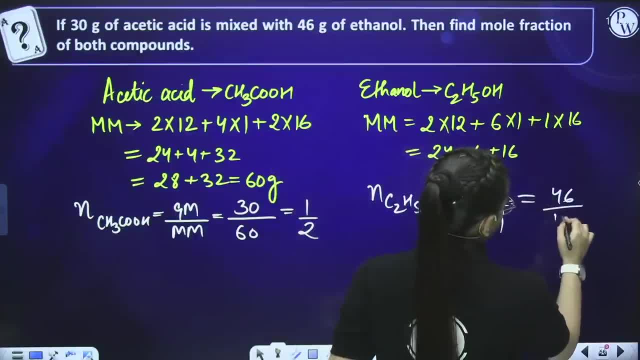 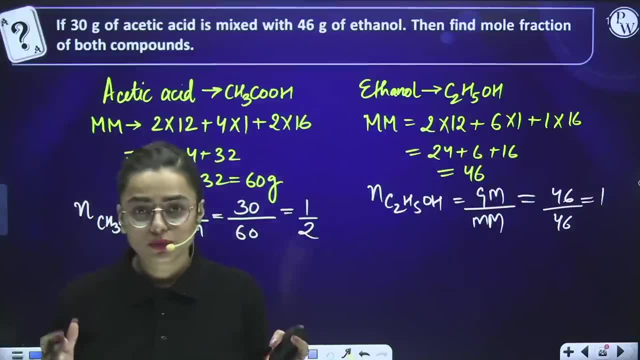 What is the given mass given in the question 46.. What is the molecular mass? we have calculated 46.. How many moles? 1 moles. Now to calculate mole fraction. we have already calculated number of moles. We will apply our basic formula. 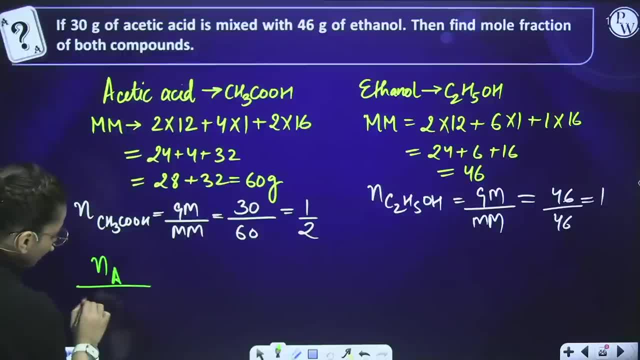 What is the basic formula? Number of moles of A component divided by total number of moles is equal to number of moles for the A component. Let us say this is the A component and this one is the B component, Right, So okay? 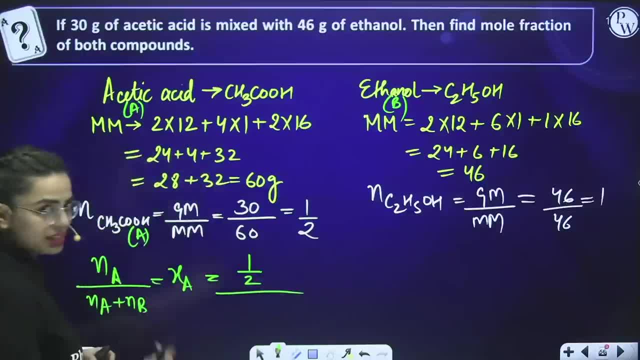 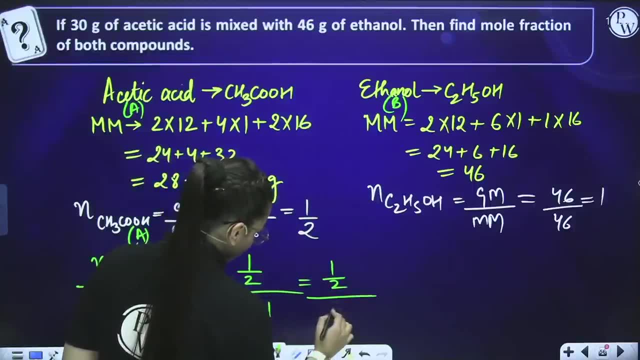 First of all, number of moles of A component is half divided by total moles. that is going to be half plus 1. So it is going to 1 by 2 divided by 3 by 2.. Hence it is coming out to be 1 by 3.. 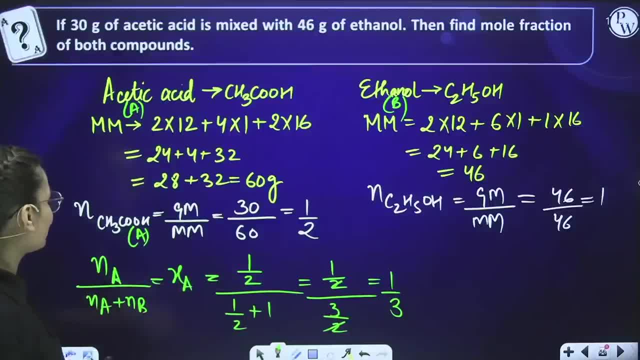 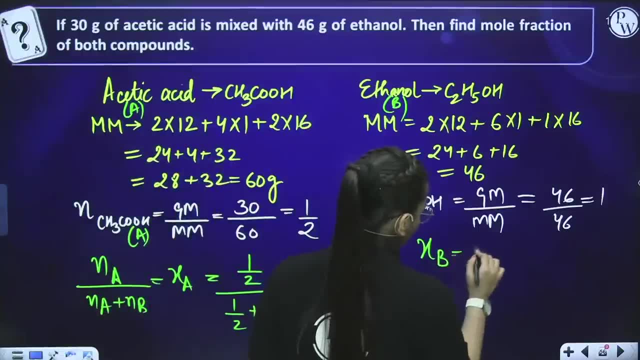 So the mole fraction I would say for CH3COH is going to be 1 by 3.. Now to calculate for ethanol we have to do same. Mole fraction is going to be number of moles of B divided by total number of moles. 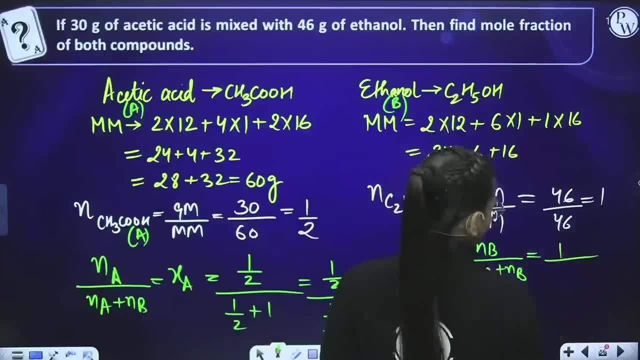 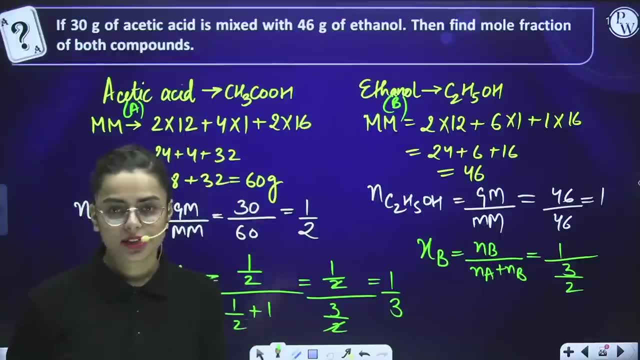 What are the number of moles of B? They are 1.. So mole fraction is going to be 1 by 2 divided by what are the total? It is 3 by 2, as 1 by 2 plus 1 is 3 by 2.. 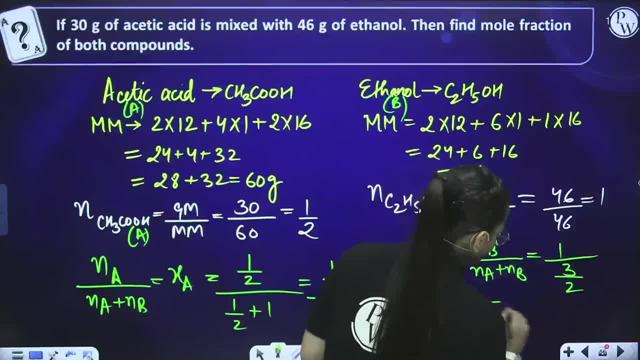 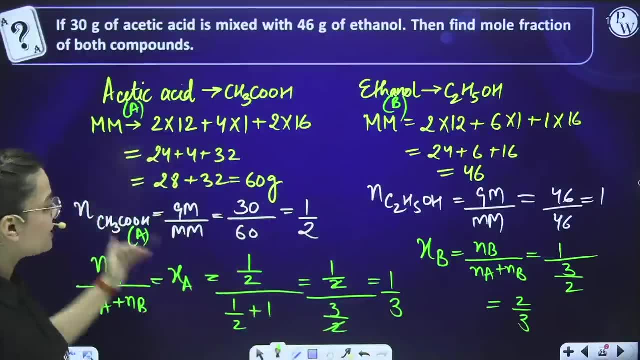 So I have directly written that: 3 by 2.. So 2 will go upwards, it will be 2 by 3.. Hence mole fraction for ethanol is 2 by 3 and for acetic acid is 1 by 3.. So this is the formula, how we can calculate mole fraction. 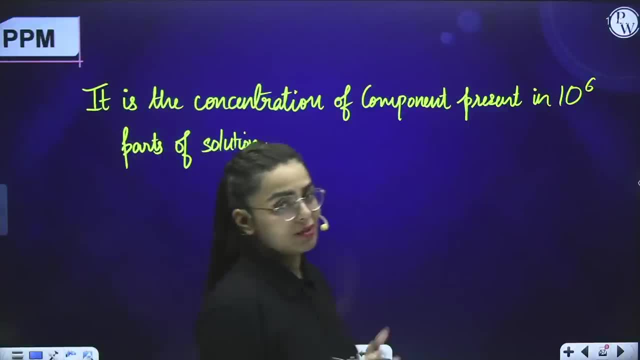 Right students, Now we are moving towards our next concentration term. that is known as ppm. It is very simple, It is the most simplest. What is ppm? It is the concentration of component. Basically, the component whose concentration we need to calculate, present in 10, raise to: 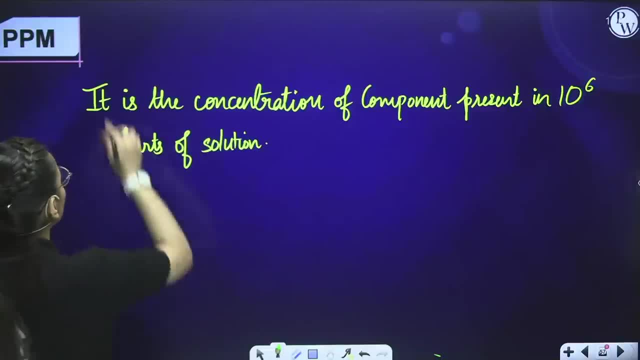 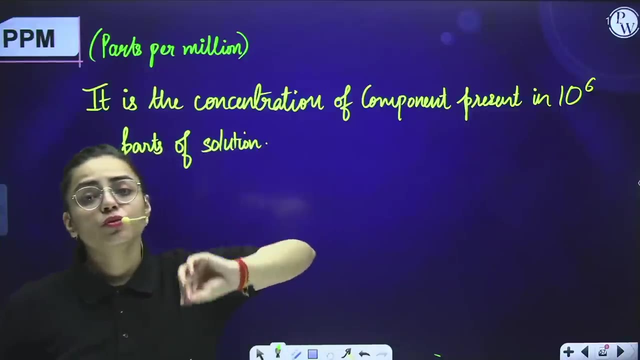 the power 6 parts of solution. First of all, write the full form of this: parts per million. As you can know, here it is written parts per million. that's why we have taken 10 raise to the power 6 here. So what is going to be the formula for ppm to calculate? 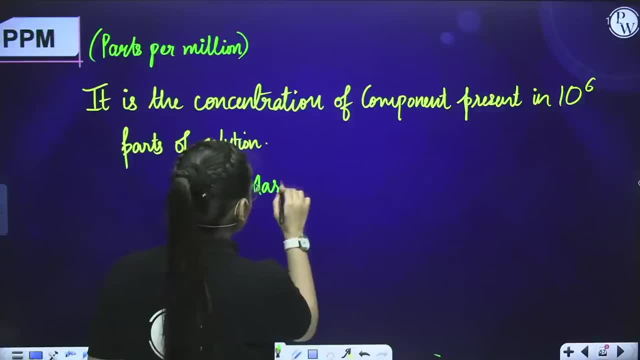 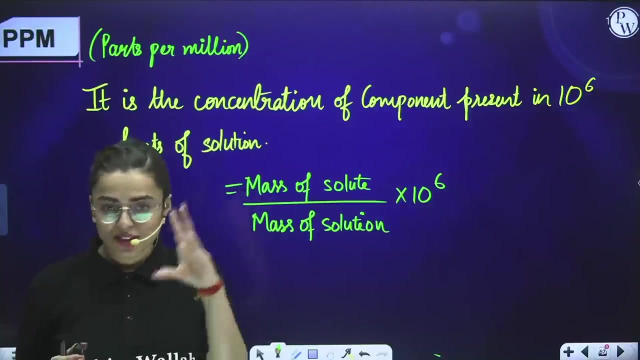 ppm. the formula is: mass of solute divided by mass of solution. students into 10 raise to the power 6.. Now let us once again. solution will come here. kindly correct that. Just think that when we were doing mass percentage, what we were doing mass of solute divided. 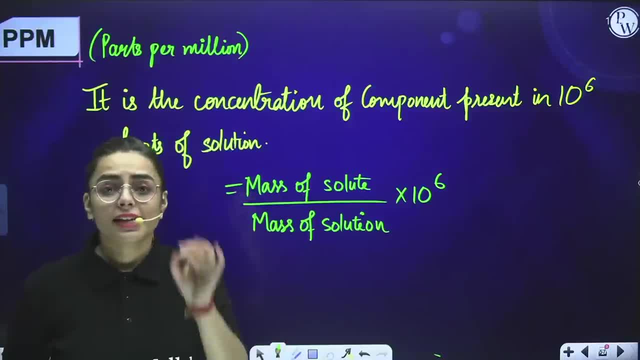 by mass of solution into 100.. But now we are taking mass of solute divided by mass of solution. So what we are doing, We are taking mass of solute divided by mass of solution into 10 raise to the power 6.. 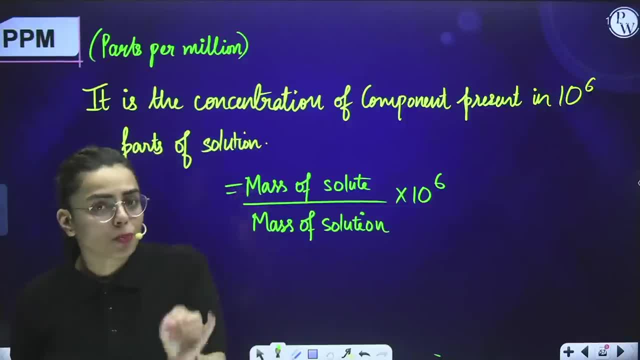 What is the basic difference between both of these? Here we are talking about parts per million. That's why we are multing it with 10, raise to the power 6.. This is the basic difference. That's all students. So this formula is being applied to calculate the percentage ppm, that is, parts per million. 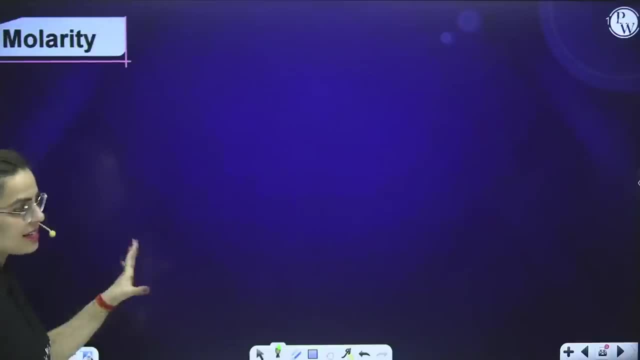 percent. So now we will move forward towards our next concentration term, that is, molarity. And students, you all will be thinking that, ma'am, So many formulas, how will we will learn these formulas? So, trust me, these formulas can only be learnt by your own practice. 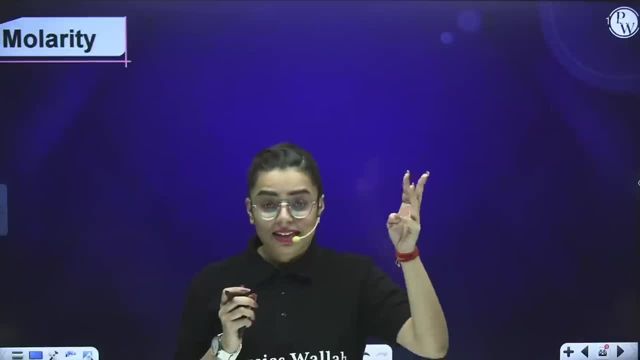 Practice, determination and consistency- These three things will lead you towards success, And if you will follow these three things, then you can achieve anything. See for the very first day, when you start doing these questions and when you listen to our lectures, Some of the students will grasp it quickly. 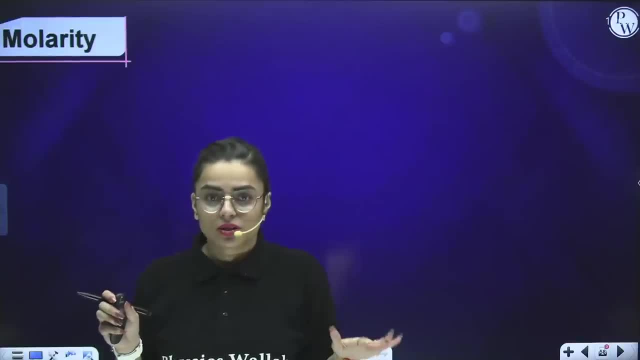 While some of the students will feel like it is taking time for us, No need to worry at all. Just three things you need to do is you need to increase your day to day time schedule. If you are working for one hour, you are studying for one hour. increase it to one and a half. 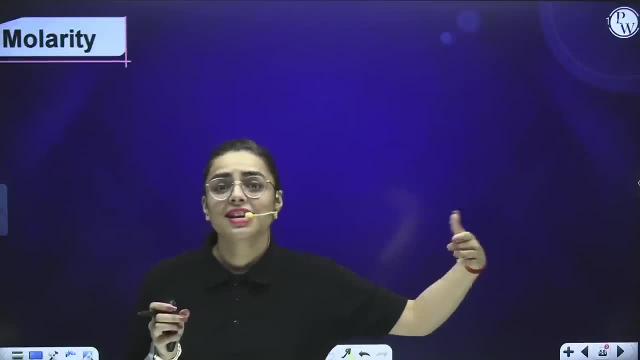 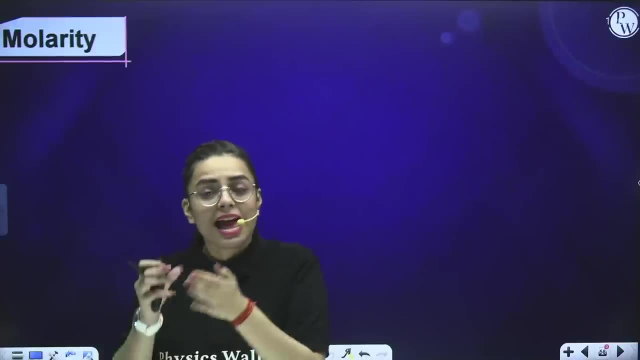 hour, then increase it to two hours, then, on the next day, increase it to two and a half hour. Like this, you will be able to sit and do your work and do practice, and the consistency will increase and maintain. So So these are the basic things. 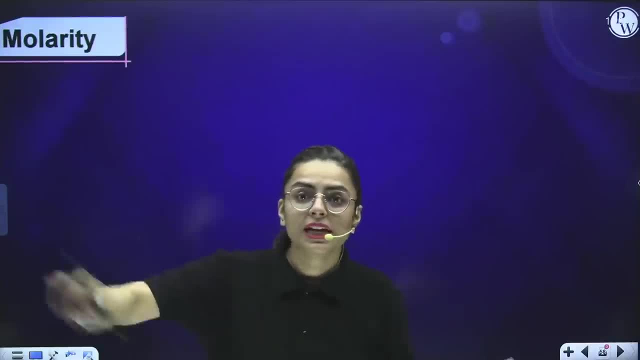 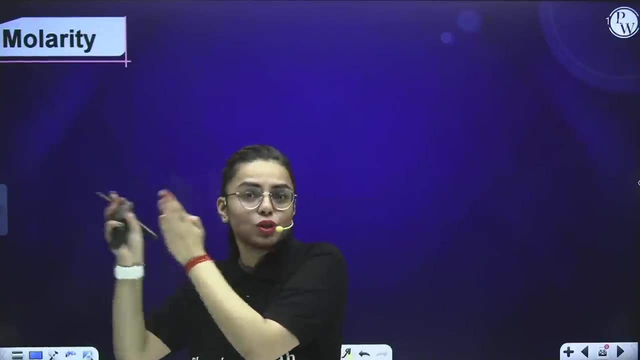 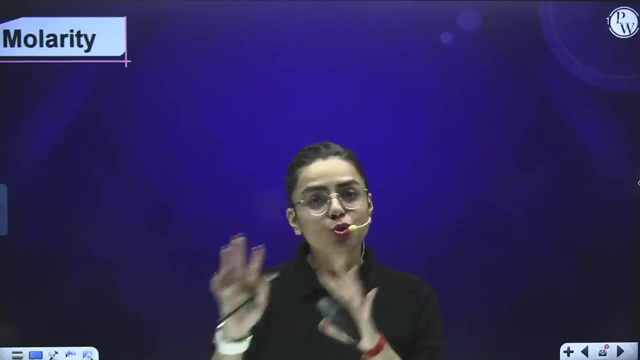 Don't start in a rush that I have to do complete in a day. I have to do complete syllabus in a day. No, no, no. Take small, small steps and then you will achieve to your success. Right, As you know, like if there are two students, you know there is two way to achieve to success. 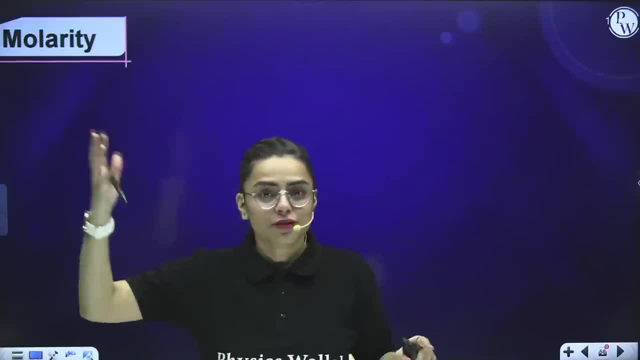 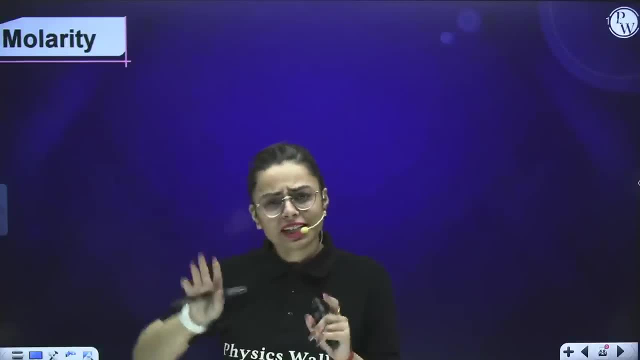 They won't stop you to achieve to success. You can go through stairs, but it will take time. it will take time, small, small, small, small, little steps. But what if lift falls or lift stops in between, towards moving from ground towards the height? What happens? what you will do? you can't do anything. 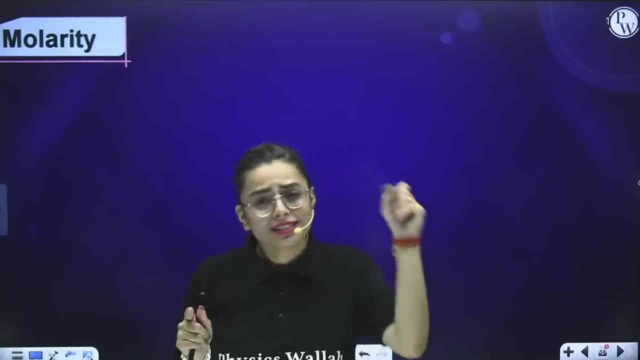 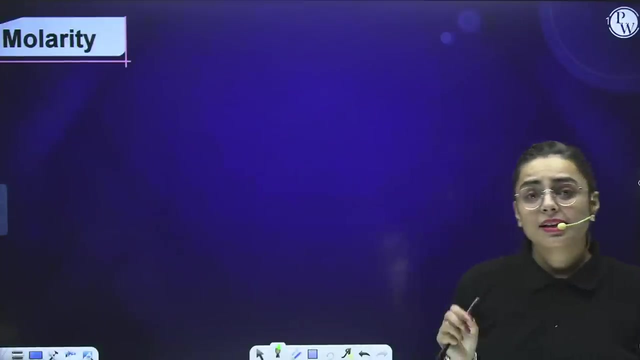 So always the method which is hard, try to do that, No problem. that it is taking time, there is no problem. you have time and you can do so. do and you will achieve success. Right, small, small efforts leading towards molarity. what is molarity? molarity is the simplest term. 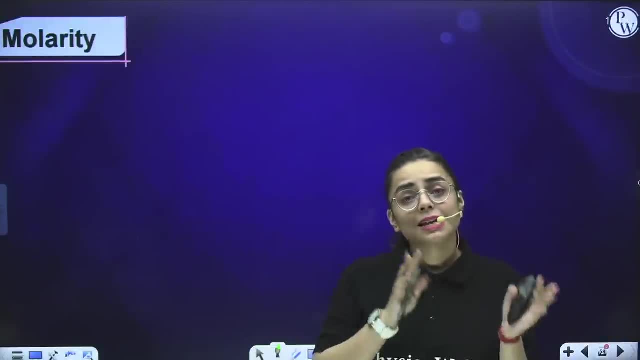 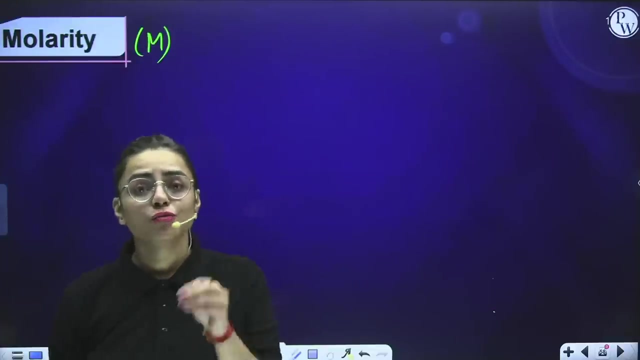 simplest concentration terms, which defines as that number of moles of solute present in hundred volume of solution, hundred liters of solution. clear students? so, students, molarity is symbolized by capital m. right, we symbolize molarity by capital m. what is molarity? basically, molarity is number of moles of solute present in one liter of solution. so what will be the formula? 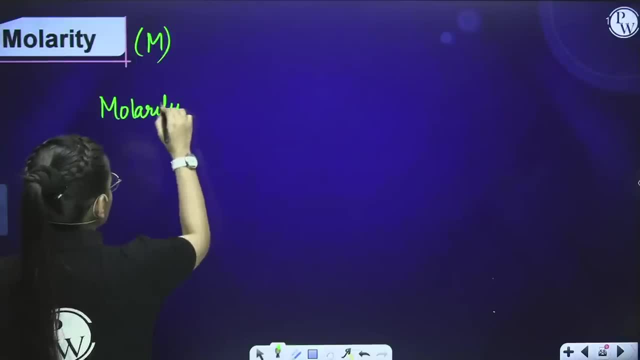 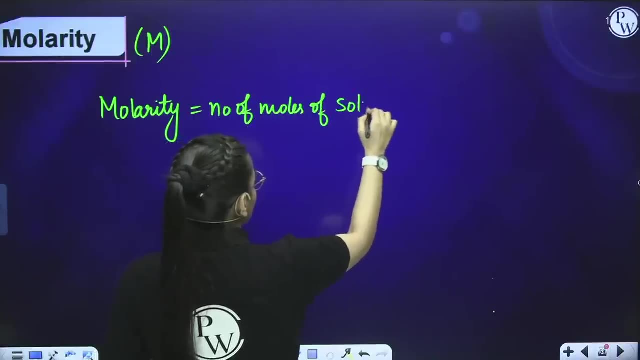 of molarity. molarity is number of moles of solute present in present in one liter of solution. that means we have to take volume of solution below, and it should be in liters, right? if you are taking volume of solution in milliliters, the formula will be: 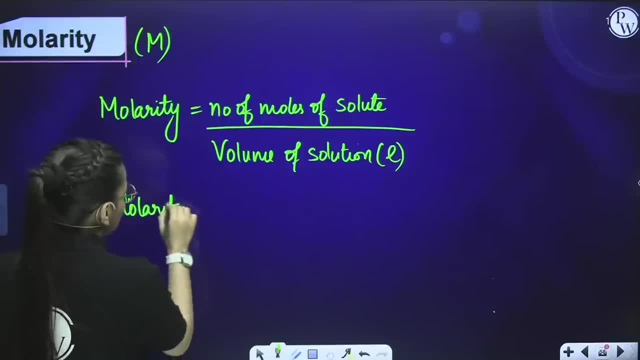 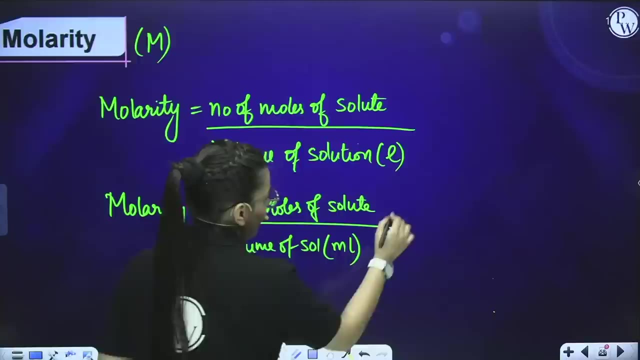 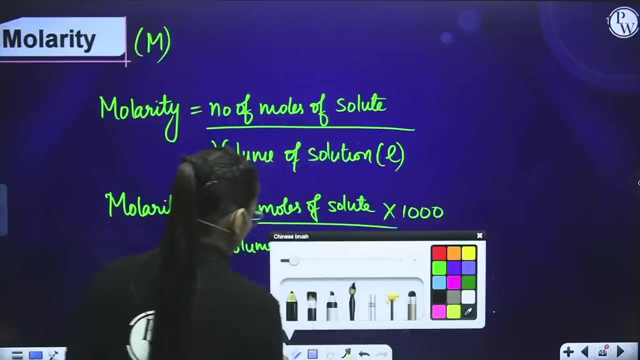 modified as molarity is equals to number of moles of solute divided by volume of solution in milliliter. hence it will be divided by thousand if you are taking in milliliter terms. one thing more, students. the twist that comes in the questions is that they don't give you directly number of moles. 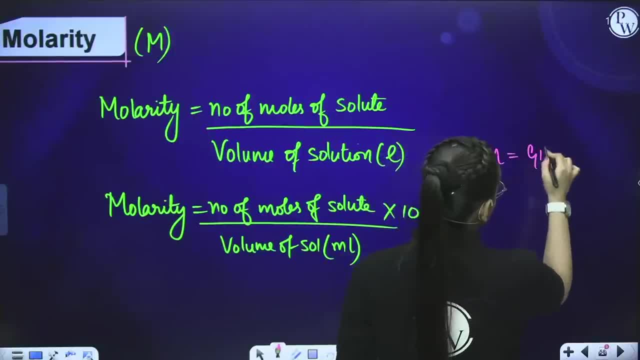 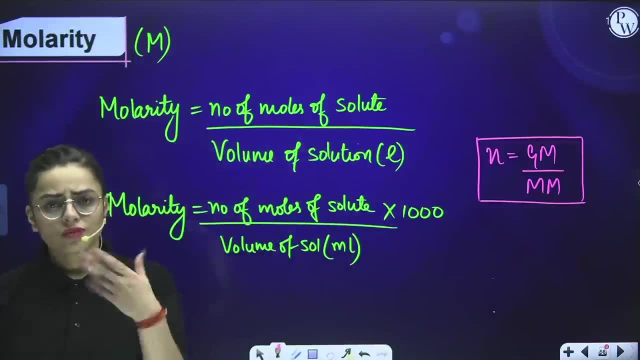 they will give you given mass. so you have to replace number of moles by given mass upon molecular mass. they can give you direct, but in some cases they don't give you number of mols, they give you given mass, molecular mass. you need to calculate and put it into the 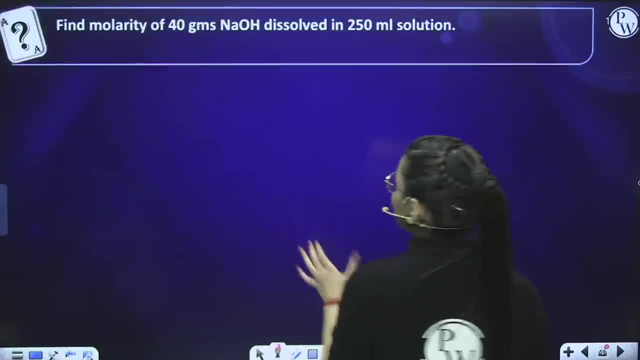 formula. so this was all about molarity. students in molarity. one of the questions is: in front of you find molarity of forty grams naoh dissolved in two fifty emils per wattовать難 of forty grams of naoh dissolved in two fifty emils per watt. 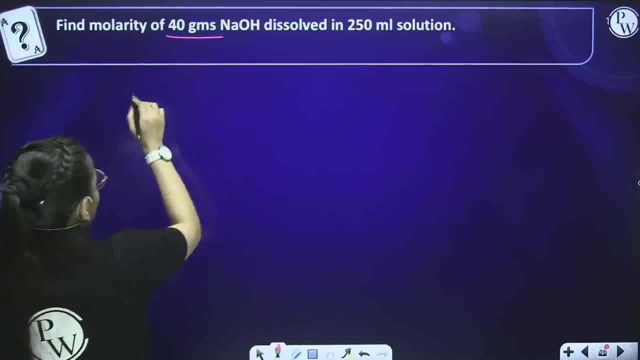 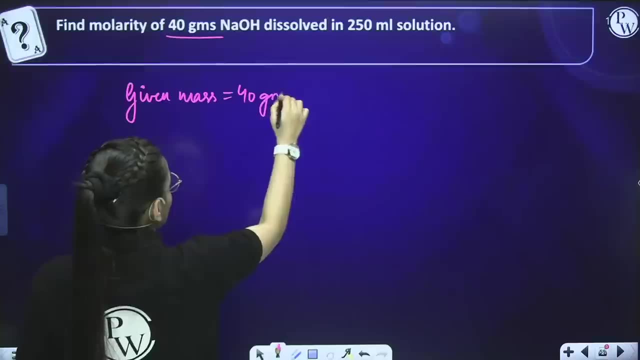 solution. so listen, what is given mass here? 40 grams, as i told you, they will not give you number of moles directly, so given mass is 40 grams. okay, now NaOH: what will be molecular mass, molecular mass for NaOH? how many sodium? 1 sodium mass is 23. oxygen mass is 16. hydrogen: 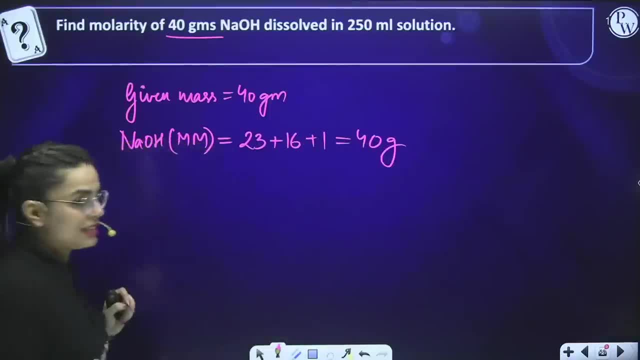 mass is 1, hence the molecular mass is 40 grams. so now we need to calculate molarity. what is the formula of molarity? molarity is number of moles. what is number of moles given mass upon molecular mass? given mass is 40. molecular mass is 40 divided by volume of solution in 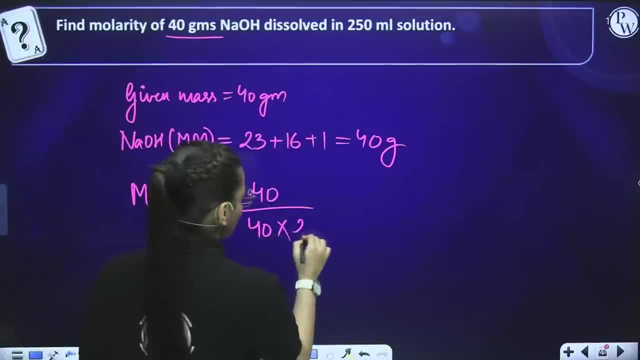 milliliters. now, when we take in milliliters, we divide it by thousand. so 250 divided by 1000, 40 is cut by 40 and then it is again cut. hence we get 4 molar students, we are getting 4 molar, right, okay? 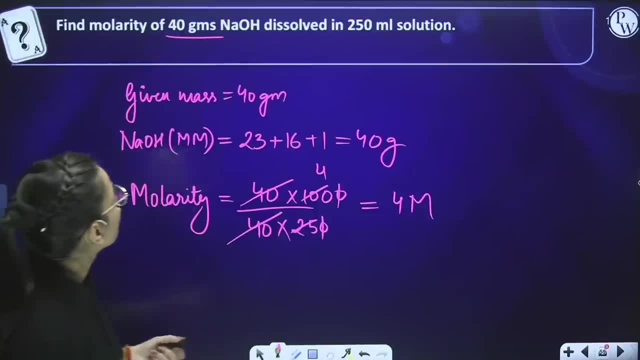 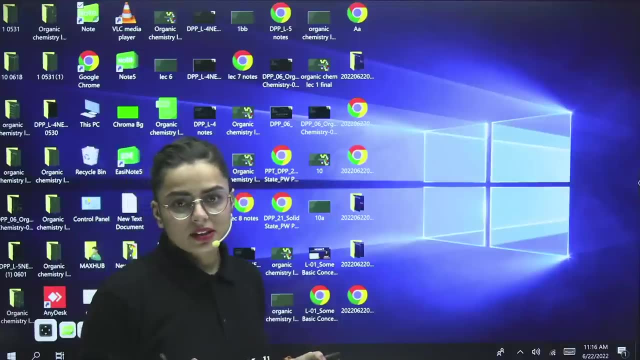 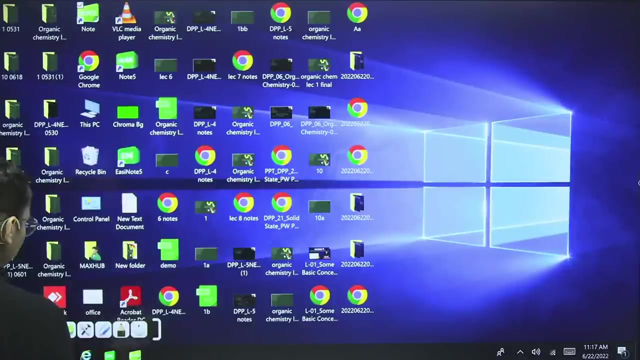 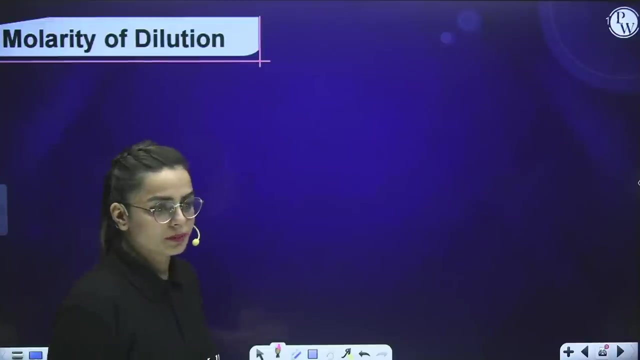 Now, students, what we need to do is we have to do molarity of dilution. what do you, sir, cut here? you note the time. i will tell them once the time is 3, 5. okay, from where it happened? okay, continue, let us continue. now we are going to do molarity of dilution, students, dilution. 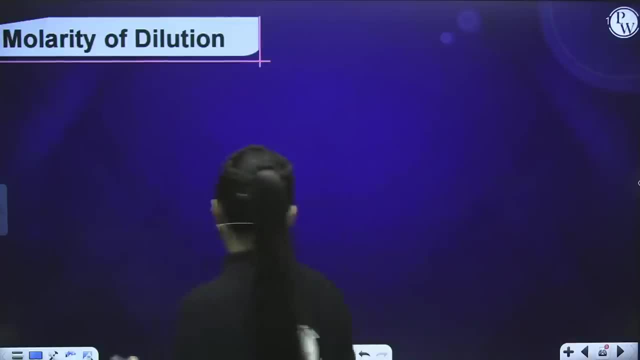 means to add something right. if i am having one beaker, what i am doing, i am having two beakers, right, i have two beakers now in this beaker students, this is my volume V1. it has volume V2.. Okay, Okay, And this has number of moles as n, and this has number of moles as n. what happens is initially: 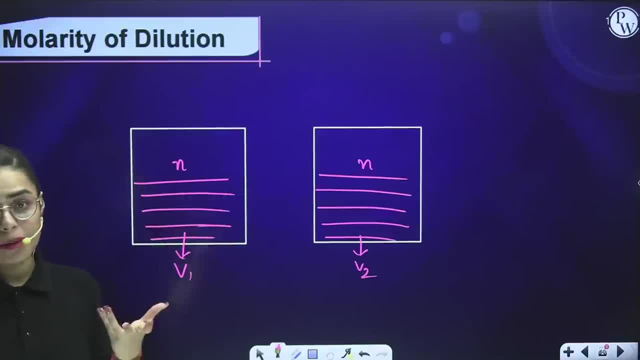 i had this beaker. i just added some amount into this, and so it converted into volume V2, but number of moles remained same. why number of moles remained same? because number of moles is depended upon given mass and molecular mass. that's why- and we are adding something- 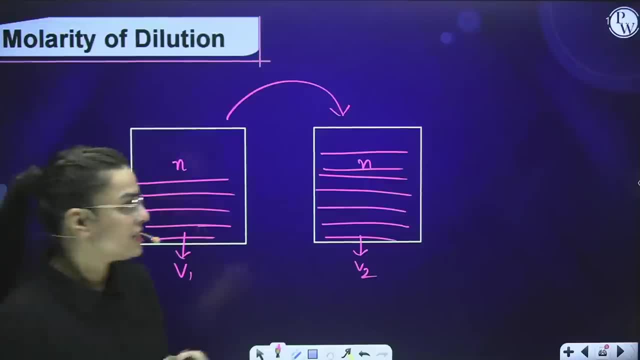 and number of moles. you know what is molarity is 40. Okay, So what is the molarity formula? molarity formula is number of moles of solute divided by volume of solution, and when we are adding liquid, then volume is being increased, not. 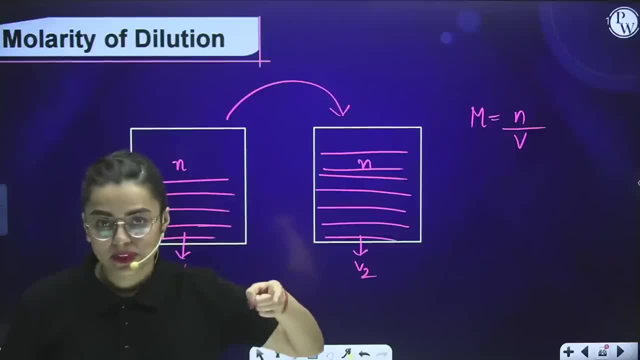 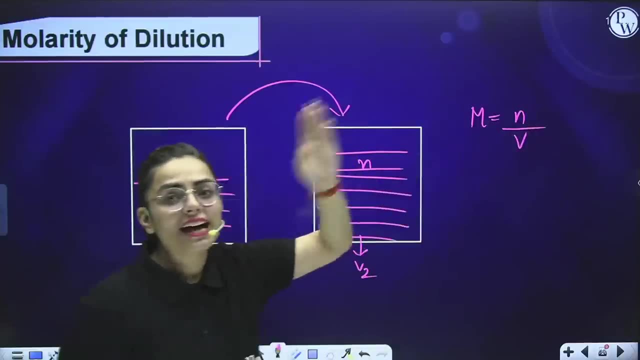 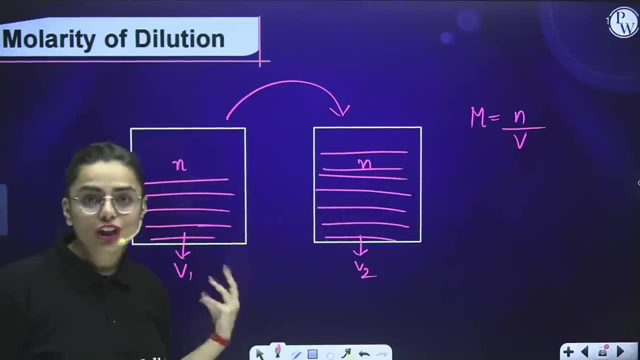 number of moles, number of moles of solute, remains the same because we are taking here solute moles, not solution moles. if we used to take solution moles then it would had increase. but we are taking of solute, so n stays remain in both of the cases, while volume changes. 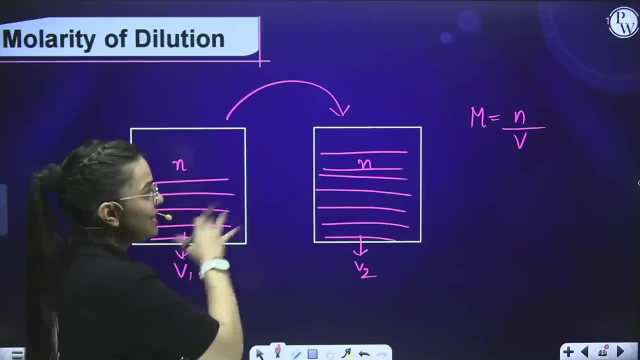 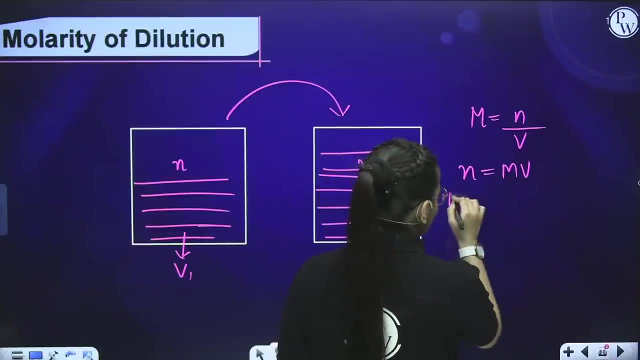 from V1 towards the V2.. Now what happens is students, Okay, It is same for both of the cases. what we say: n is equals to mv. now what we can say: if n is equals to mv, then we can write: n is equals to m1- V1, and n is equals to m2- V2. now both. 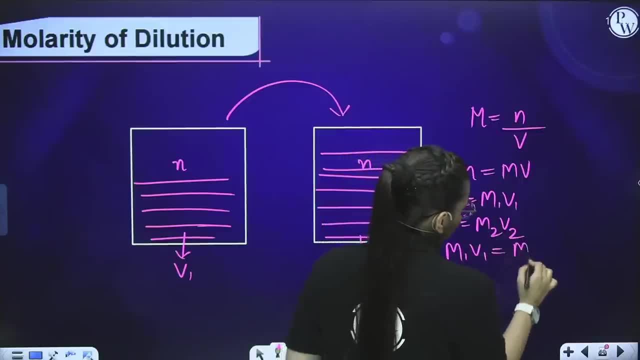 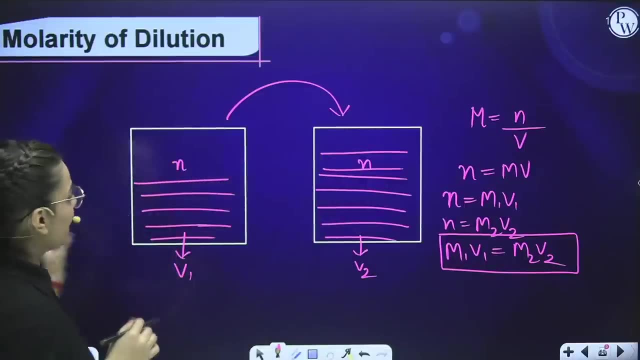 of the terms will be equal. hence, the formula obtained is m1. V1 is equals to m2- V2. this is the formula for molarity in dilution, molarity of dilution. that means, for example, you are given a question, Okay, Okay. 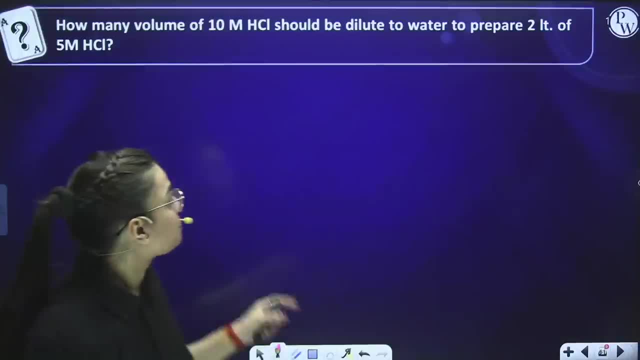 How many volume of 10 molar HCl solution should be dilute to water to prepare 2 liter of 5 molar HCl. now let us see with an help of diagrams to make it more understandable. I have these two beakers. in the very first beaker they are saying how many volume of 10 molar HCl. 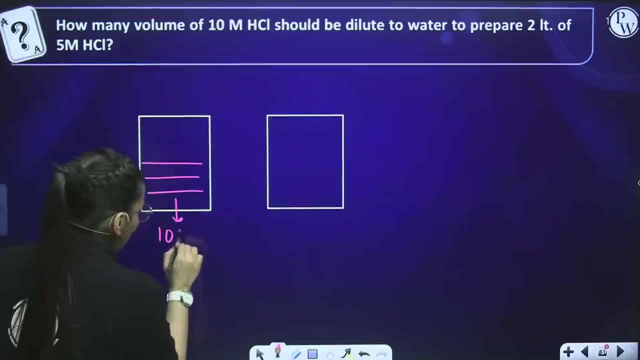 I have molarity here. 10 molar right should be dilute to water should be dilute. Okay, What should we add into it? to prepare what we need to prepare, what we are preparing students. you need to check this, what we are preparing. one second: yes, I am adding something into. 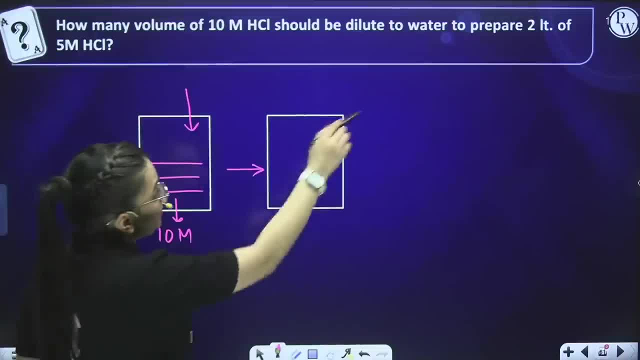 this and it converts into this and to prepare 2 liter of now it is becoming 2 liter and 5 molar HCl. now what I have got? I have got this volume V2, I have got this molarity m2 and in the start I have molarity m2.. 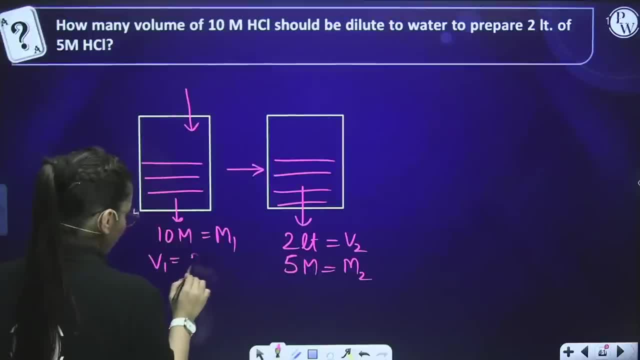 Okay. So what I am going to do is I am going to calculate the molarity m1, while I don't have V1 right. So first of all I will calculate V1 right, see. so m1, V1 is equals to m2, V2, m1. I know. 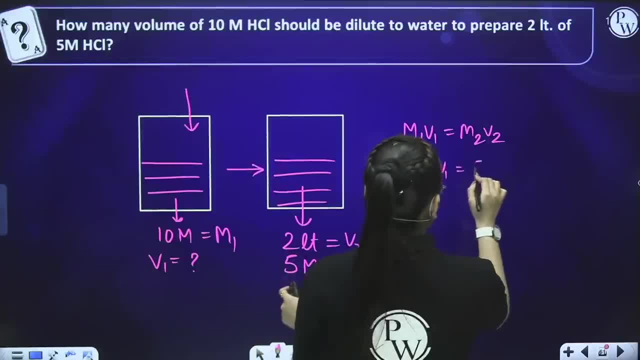 is 10, V1- I don't know- is equals to m2, is 5 and V2 is 2. V1 is equals to 5 into 2 by 10, hence V1 is 1 liters. that means that means the first beaker had 1 liter volume, but the 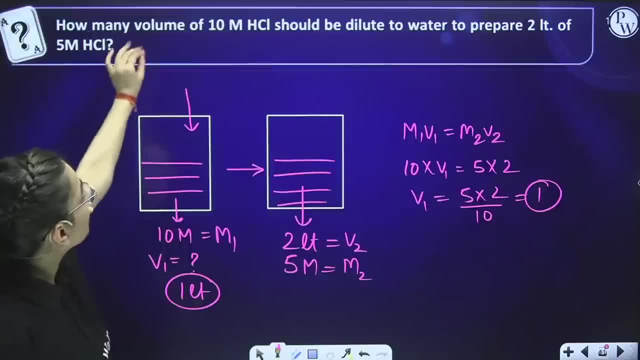 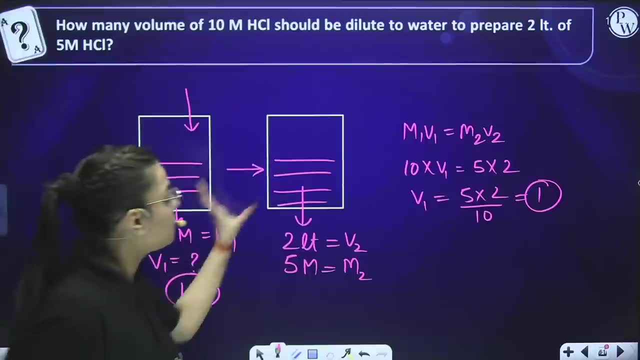 question is incomplete. Now they are asking us how many volume of 10 molar HCl should be dilute. it should be dilute. how much should be added so that it becomes 2 liter? what should be added in 1 liter so that it becomes 2 liter? obviously, 1 liter will be added into 1, so how many volume? 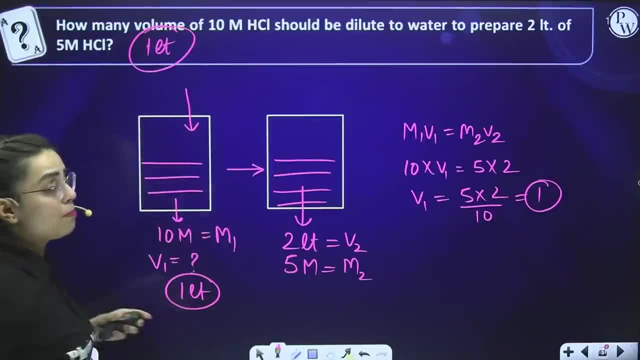 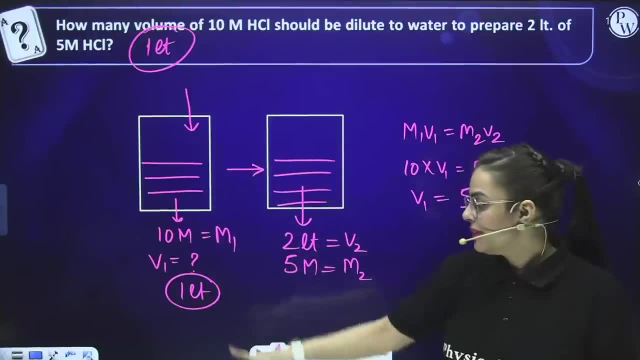 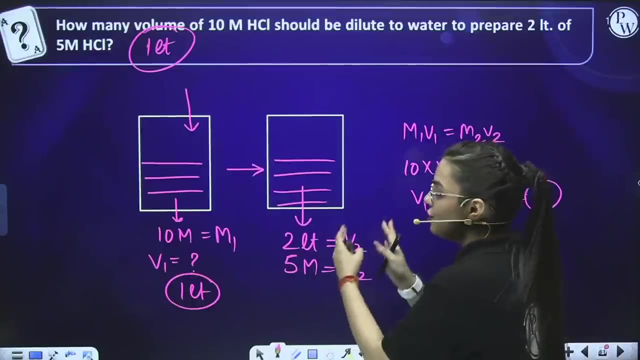 will be added. 1 liter volume will be added. but if it asks you in question what is the volume of beaker first or before dilution, then you would say 1 liter, And when it asks you how much dilution is required, then you will subtract your V2, right. 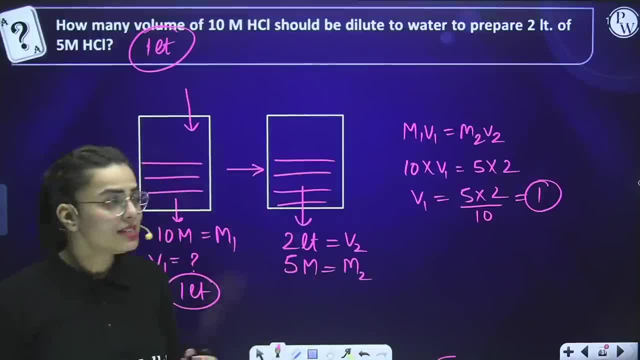 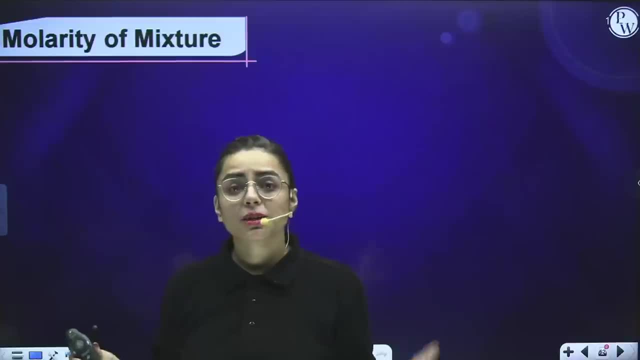 V1 from V2 and you will get your answer right, students. ok, Now comes molarity of mixture. molarity of mixture refers to as when one beaker is mixed into another beaker and we are getting a mixture. for example, I have this beaker, I have this. 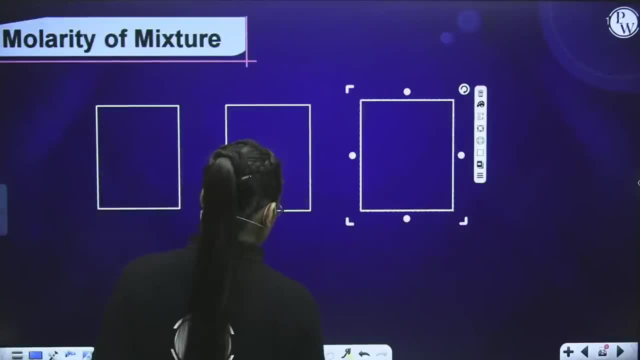 beaker. then, students, I have this beaker right. See, Here I am adding these two and I am getting this product right. this is my beaker A, this is my beaker B and this is my solution, which I am getting after the addition of both of. 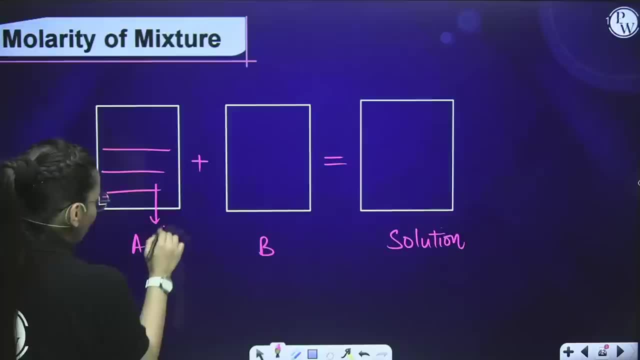 them here. in A, molarity was M1, volume was V1. here, molarity was M2 and volume was V2. here molarity will be M- M refers to as the total molarity of the solution- while volume will be V1 plus V2. right, so what will be the formula to calculate the solutions: molarity, the complete. 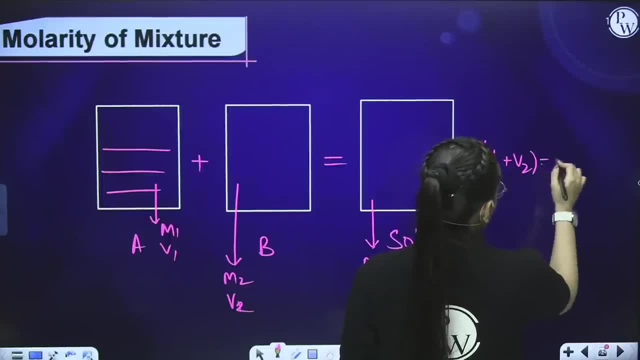 formula will be M1, V1 plus M2, V2. now to calculate molarity of the solution. molarity of the solution, that is capital M, is equals to M1, V1 plus M2, V2 divided by total volume, that is, V1 plus V2.. 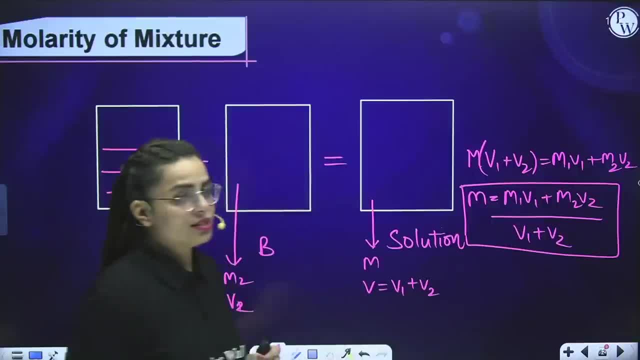 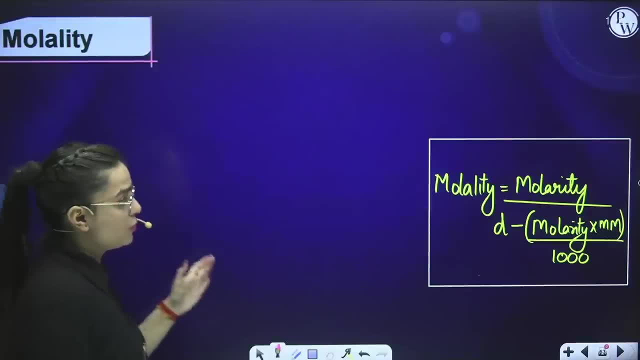 Ok, Hence, this is the formula that is used to calculate the molarity of mixtures. clear students, very good. now, students, we are moving towards the relationship between molarity and molality. what is the relationship between molarity and molarity? before that, let us understand. 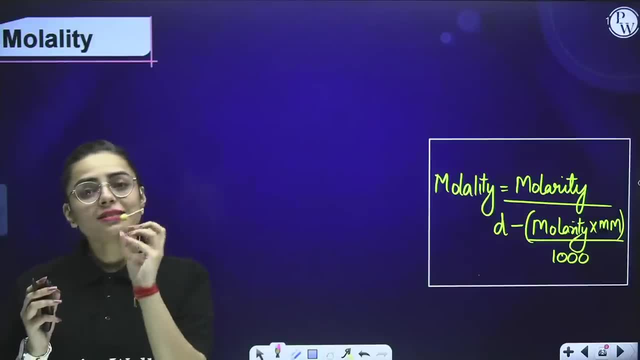 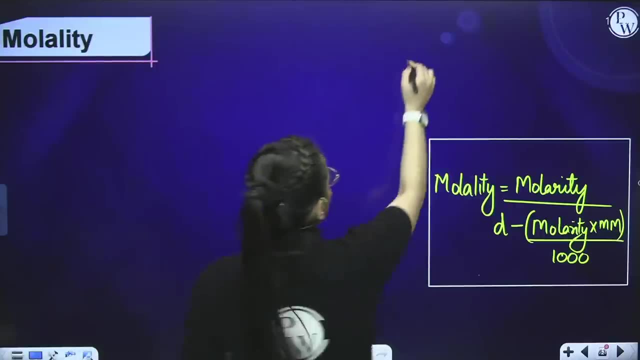 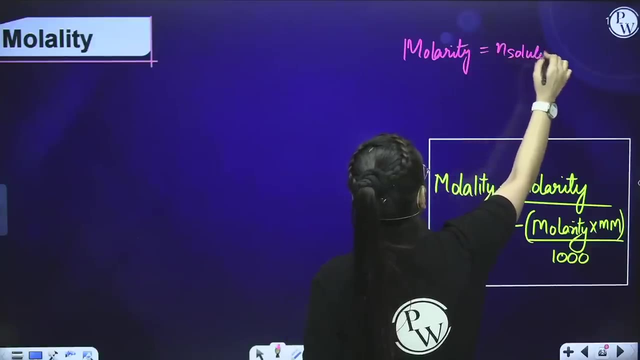 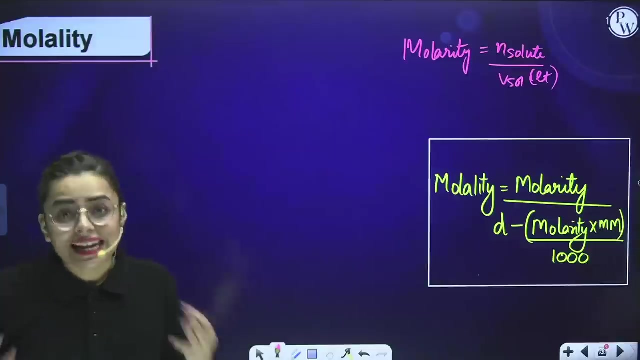 the basic difference between molality. Molality is that concentration term in which we don't use volume students in molarity. what we used to do, We used to define molarity as number of moles of solute divided by volume of solution. in liters, this was molarity. but when I talk about molality, what do you mean by molality? 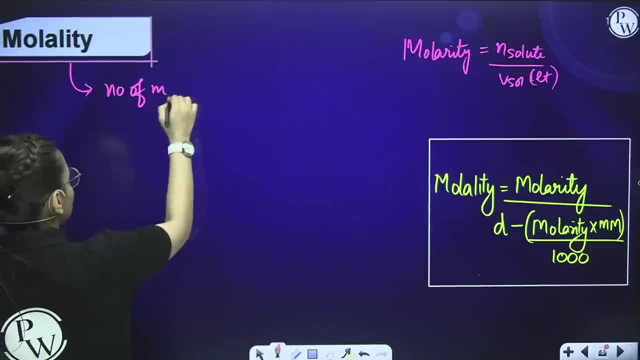 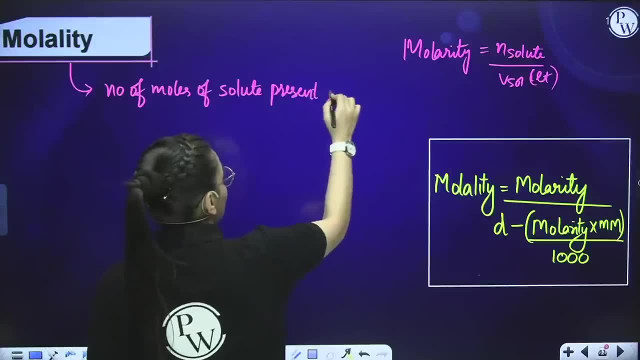 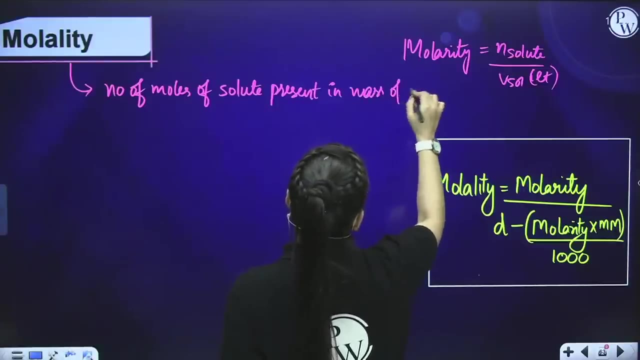 molality is number of moles of solute present in number of moles of solute present in molarity. Ok, Ok, Ok, Ok. So we can say that molarity present in mass of solute in kg. Now one more difference which you will observe is in molarity. we were taking volume of solution. 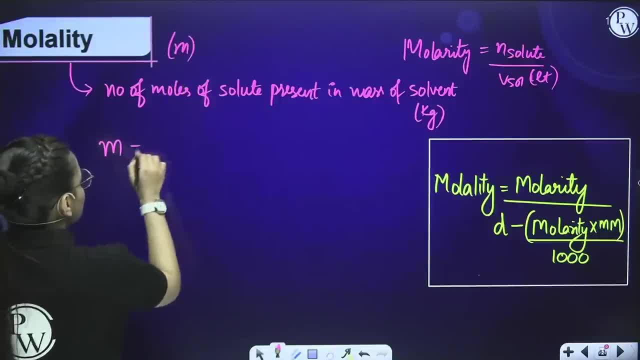 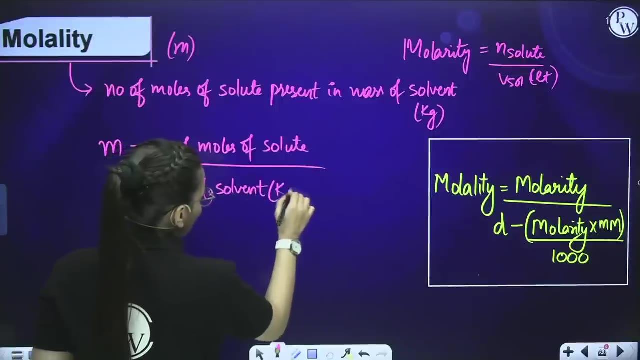 but in molality we are taking mass of solvent and in kg. So formula will be: molality is represented by small M. It is number of moles of solute solvent in kilograms. so this is the basic formula that you need to remember. now the relationship: between molality and molarity. what is that? this is the relationship that you need to know. molality is equals to molarity divided by d, refers to as density minus molarity into molecular mass divided by 1000. this is the direct formula that you can apply in the questions when there is a 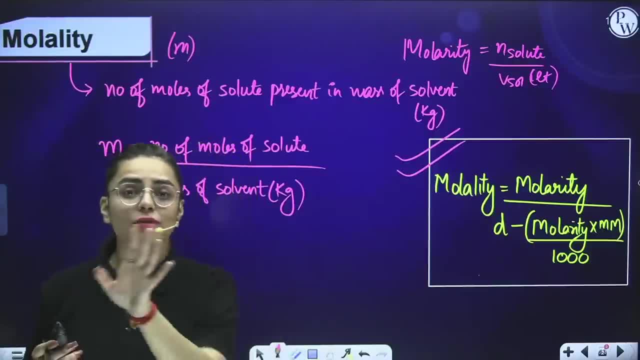 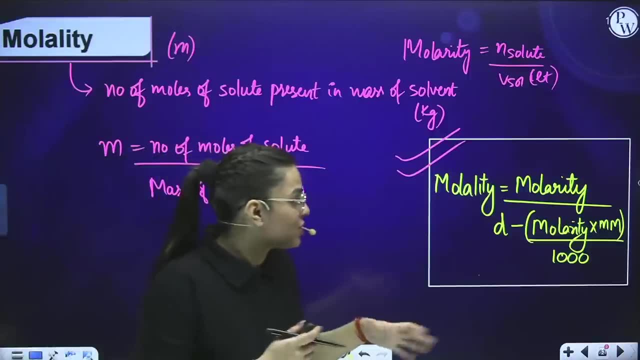 relationship when you are being asked about molality and you have been given molarity so you can directly equate and get your answers clear. students, so this was the most interesting concentration terms, as there is the relationship. try to solve as many questions as you can so that 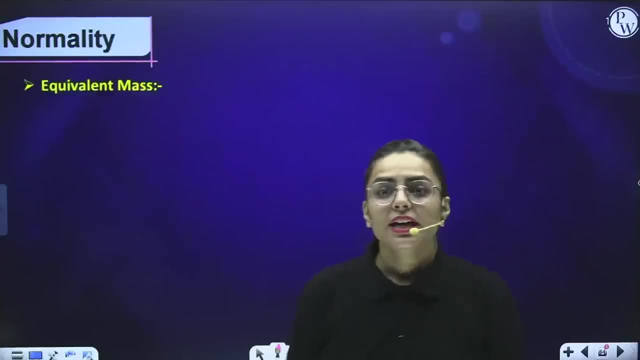 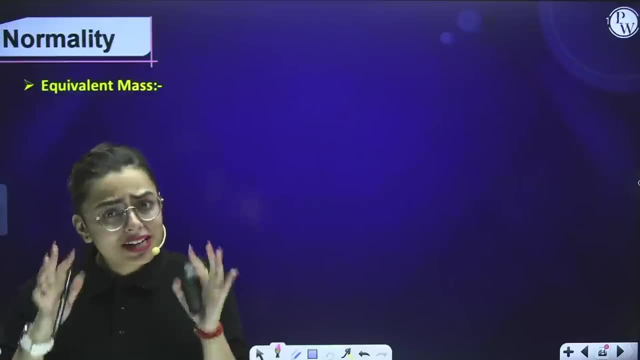 the relationship formula stays in your mind right. okay, now, students, comes the next concentration term that is referred to as normality. to understand normality, first we need to understand what is equivalent mass. what is equivalent mass, students? equivalent mass, basically, is molecular weight by valency factor. 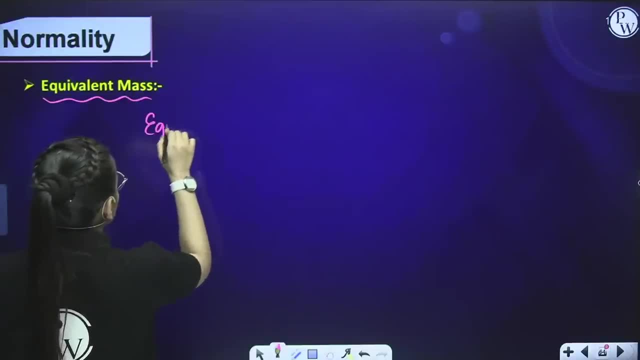 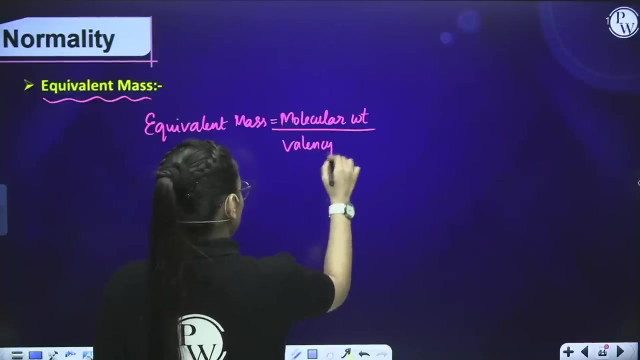 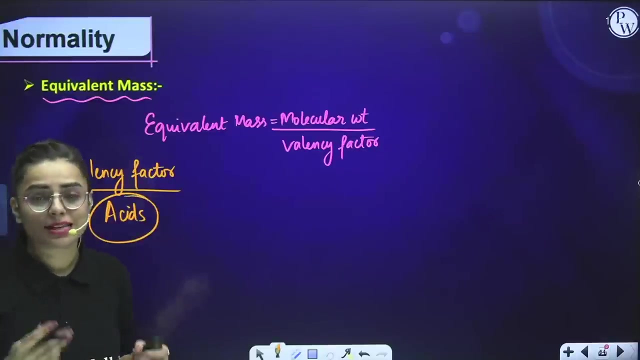 equivalent, equivalent mass is equals to molecular mass or molecular weight, basically divided by valency factor. valency factor or X, you can represent it. so, students, now what is valency factor? see for acids. if I talk about acids, bases and salt, first we need to calculate valency factor. 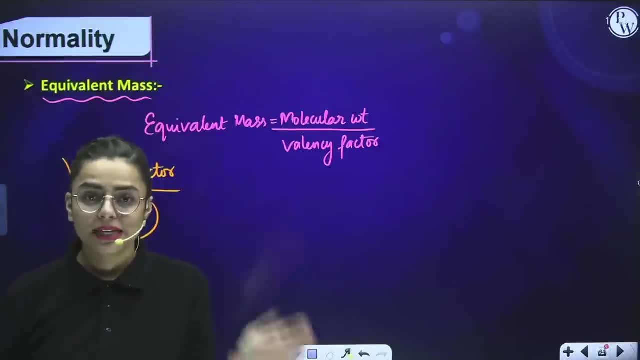 for acids, we always go for basicity. for base, we always go for acidity. ma'am, what are you saying? what is acidity? what is basicity? how do we identify it? so, students, first of all you need to understand the basic formula that is going to help you to calculate normality. first, you will 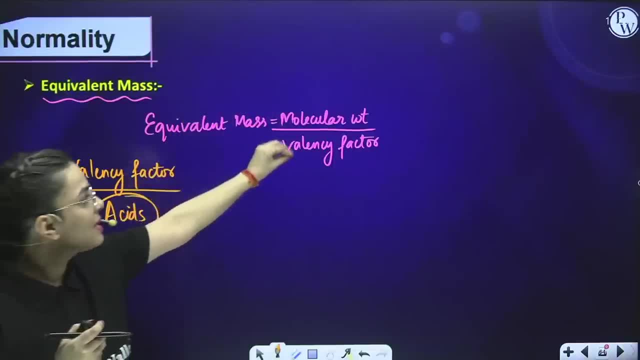 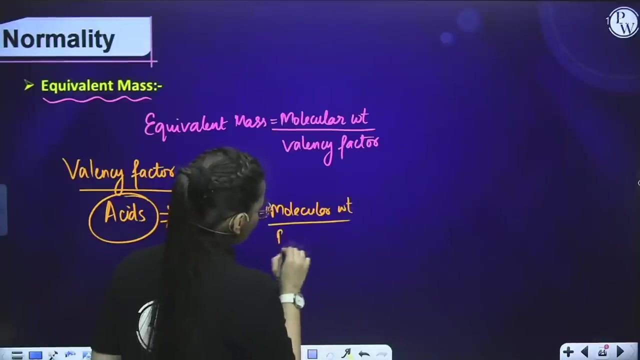 calculate equivalent mass. how to calculate equivalent mass molecular weight by valency factor. then, students, valency factor for acids. the formula will be changed. formula for acids will be: equivalent mass is equals to molecular weight by basicity. what is basicity? basicity is the number of H positive ions that are liberated. 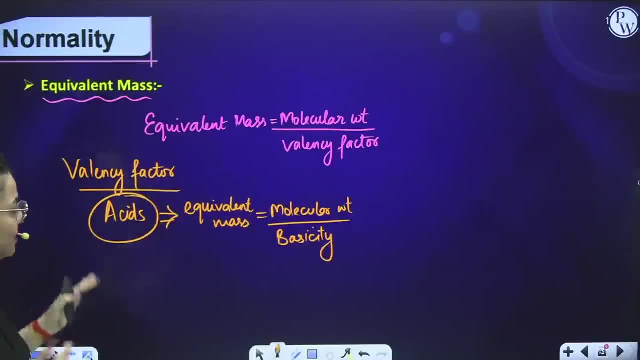 for example, students. now let us take an example to understand the situation. you can take H2SO4, I guess, and other than this, you can take any of the acids. right, and for base students, first let us write all the formulas, then I'm going to take some of the examples, right. 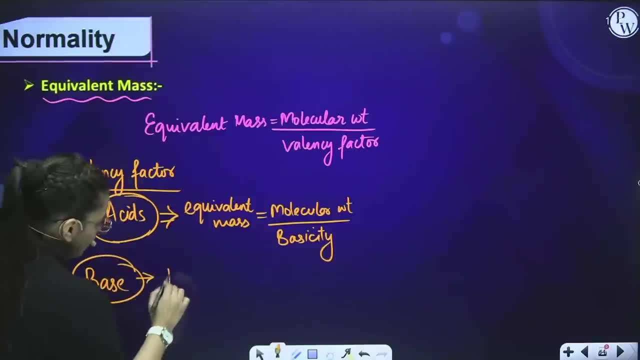 for acids for base. for base, the formula is going to be: equivalent mass is equals to molecular weight by acidity is equals to molecular weight by acidity. students, acidity refers to as how much OH negative ions are being relay liberated. for example, in any OH, how many OH ions are liberated? 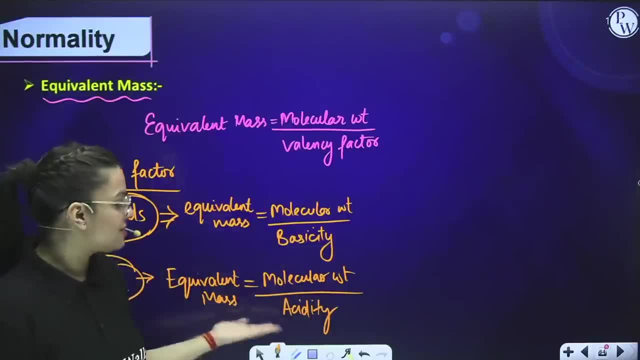 liberated one right. so basis its acidity will be one. you will write one here and for the following question you will write the molecular weight and you will calculate the equivalent mass. but if i talk about salt, if i talk about salt students, in the case of salt what happens is: 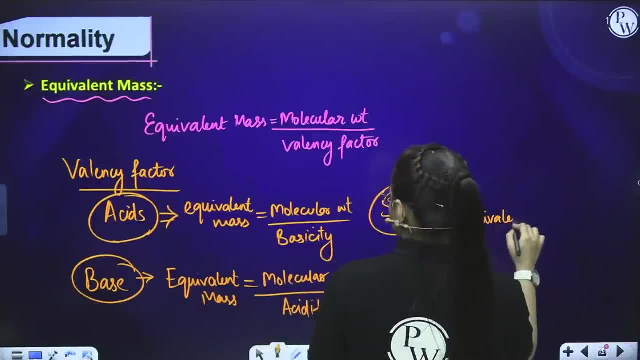 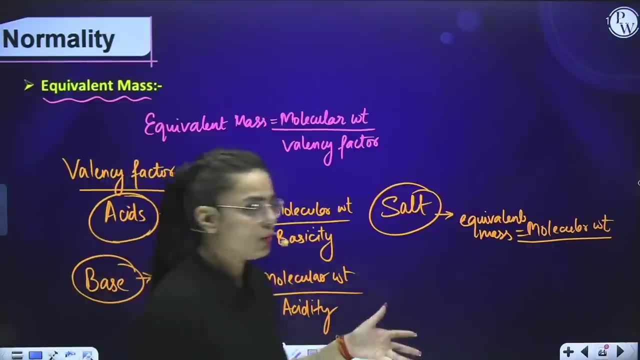 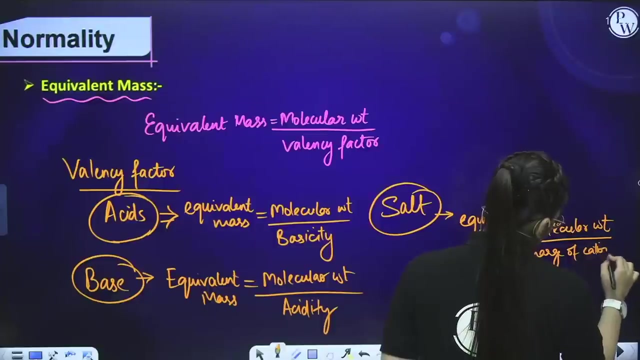 equivalent mass is equal to molecular weight divided by what. now you have to see the charge. you have to see either the charge of cation or the charge of anion. any one of these right cation or anion, for example MgSO4 in MgSO4, divide it. it will split into Mg plus 2 and 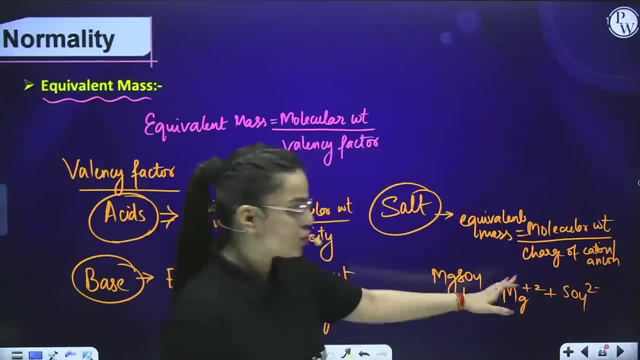 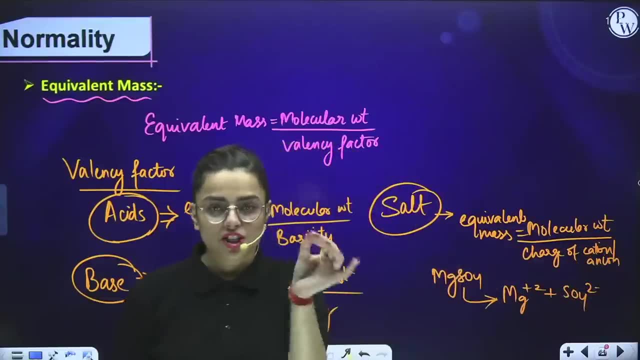 SO4 2 negative. so you either take it or you divide it into Mg plus 2 and SO4 2 negative. so you either take the charge of the positive or the negative. it's two, so it's valency factor, that is, the charge of cationine will be two. don't put the charges positive, negative, that won't be put it, only you. 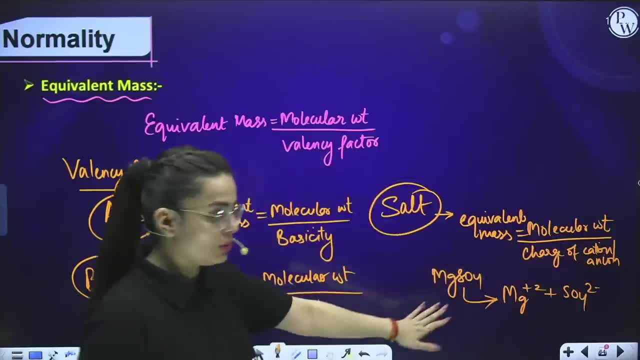 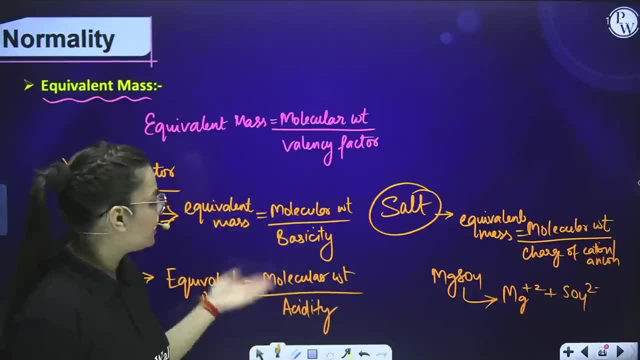 have to put the number, that is two. so valency factor in this case will be two. now for basicity. as i've given you example of noh, how many ohms are liberated? only one, then its acidity will be one. similarly, for acids you can go for like basicity. basicity refers to as how many h positive. 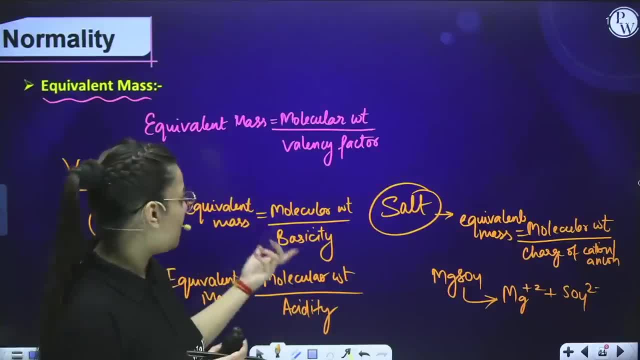 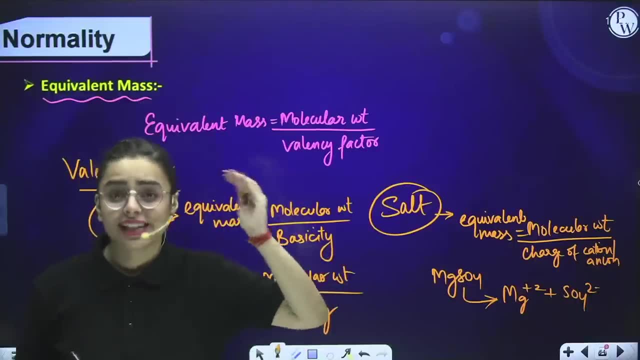 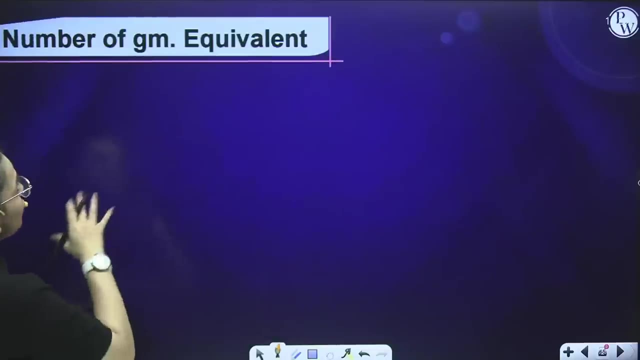 ions are liberated. that will tell you it's about basicity. so this was all about valency factor, which will lead you towards the equivalent ways, and when you have already calculated equivalent way, we will move towards the formula of normality. students- now students. number of gram equivalent. 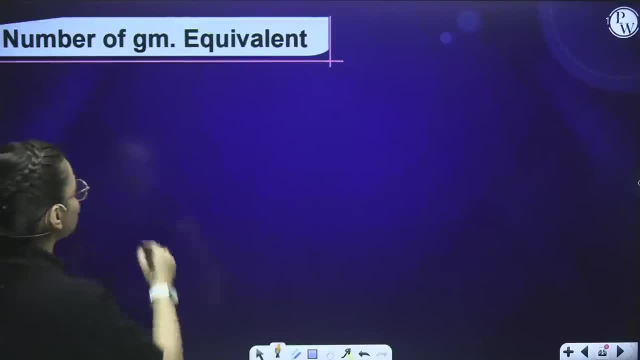 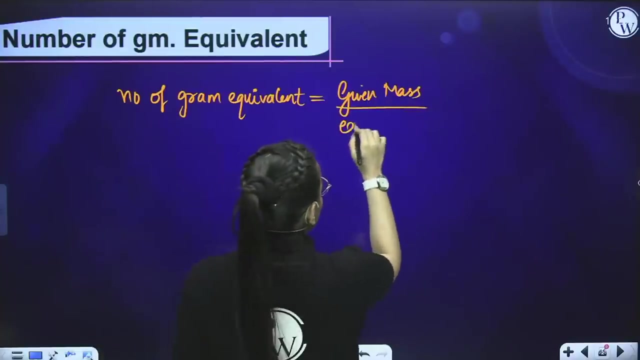 we have to calculate number of gram equivalent. what is this number of base? We have calculated equivalent mass, equivalent weight. so first of all we will write: given mass divided by the one that we calculated before, that is equivalent weight. and you know what is the formula of equivalent weight: molecular weight divided by valency factor. so first, 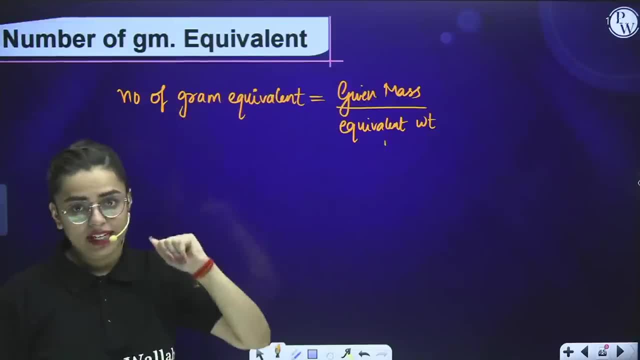 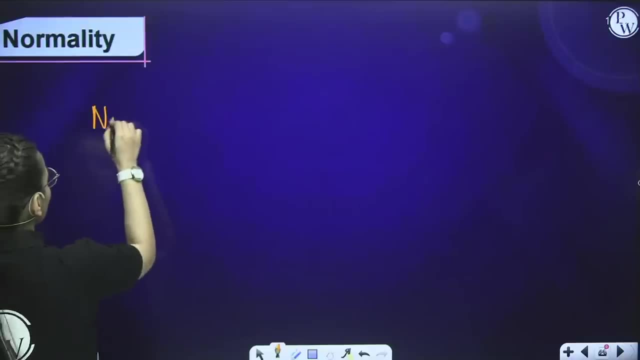 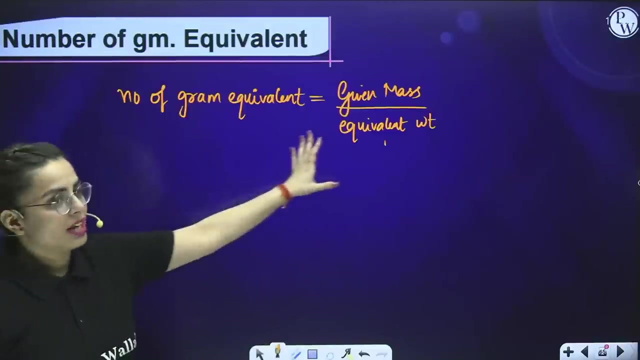 you will calculate this, then you will calculate number of gram equivalent and now we will calculate our normality students. how do i calculate number of gram equivalent weight? number of gram equivalent weight divided by solution x. Number of gram equivalent weight divided by volume of solution x in liters. 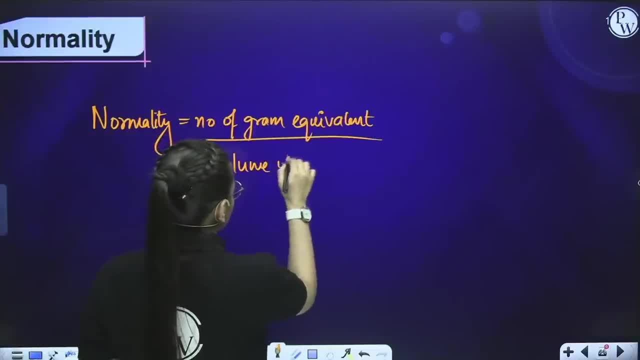 in liters? mortar pipe, jujube slurry, vanillin water. they ask in milliliters, then you need to divide it by thousand. So, students, it was about normality. and when so ever they ask you, relationship between normality and molarity, what is the? 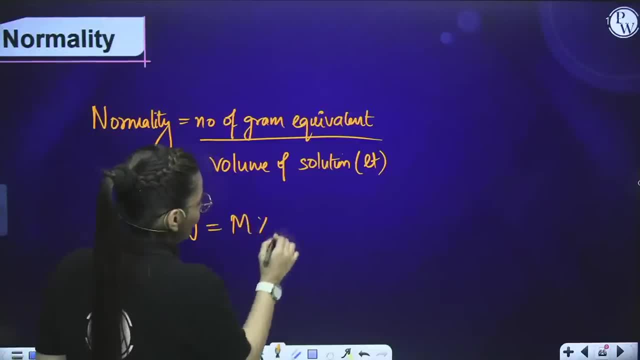 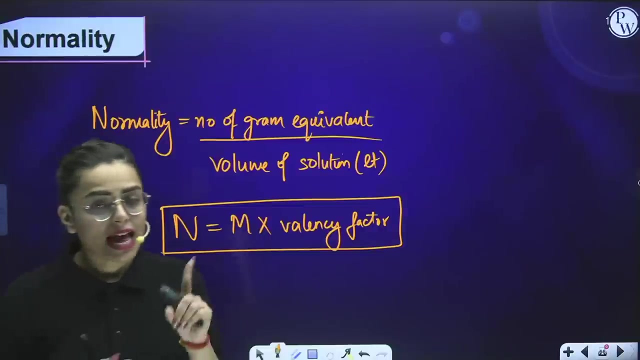 basic formula, Normality is equals to molarity into its atomicity. that means valency factor, which we calculate for acid bases and salt. So this is the relationship between normality and molarity Clear. We have done two relationships between molality and molarity. Now we have 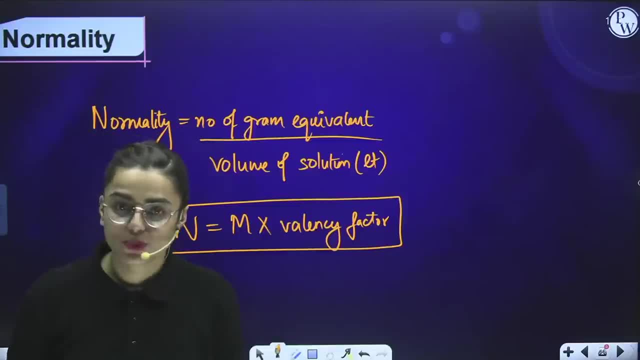 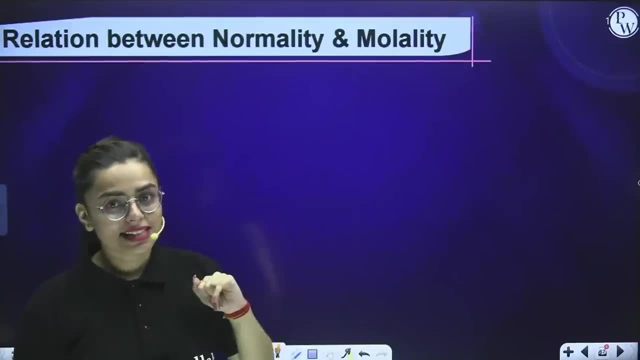 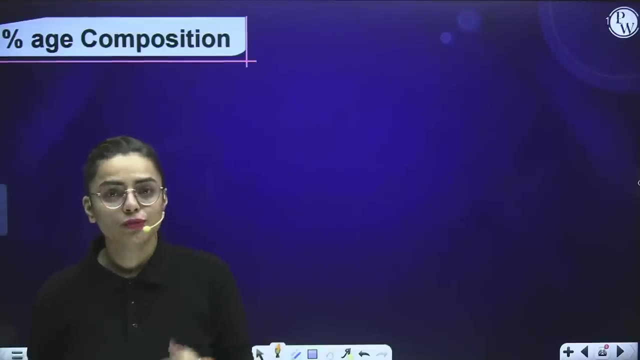 done between normality and molarity, Clear students, Very good. Now students, the next thing that comes is the relationship between molarity and normality. I have already explained you in the previous slide. I will proceed towards the next topic, that is, percentage composition. Now, percentage composition is required for empirical and molecular formula. 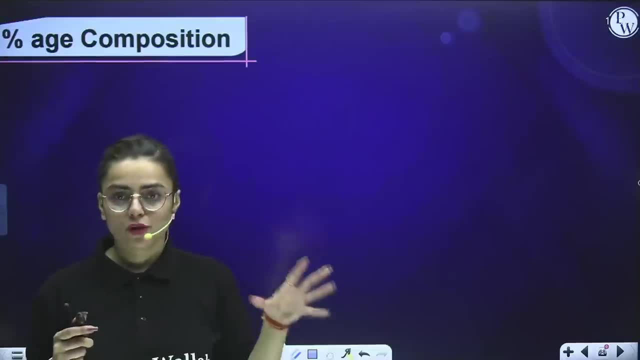 First of all we need to calculate. we have been given empirical formula- Then we need to calculate the percentage composition. So we need to calculate the percentage composition, Then we will calculate its molecular formula. So, before understanding into these terms the basic terms that will help us to calculate, that is, the percentage composition. Now let 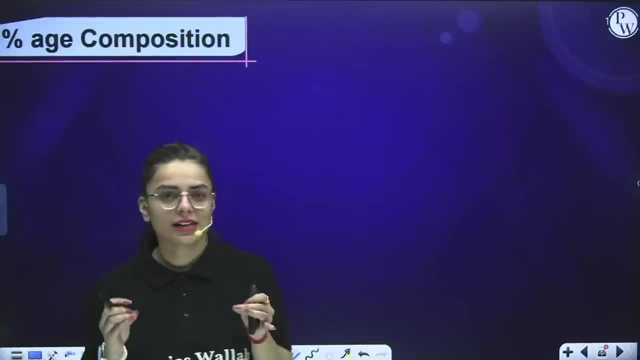 us start this. So yes, my dear students, now we are doing percentage composition. Basically, percentage composition is going to help us in empirical and molecular formula. What is percentage composition? For any component, we defined it as mass of that component divided by total mass of the solution into hundred. 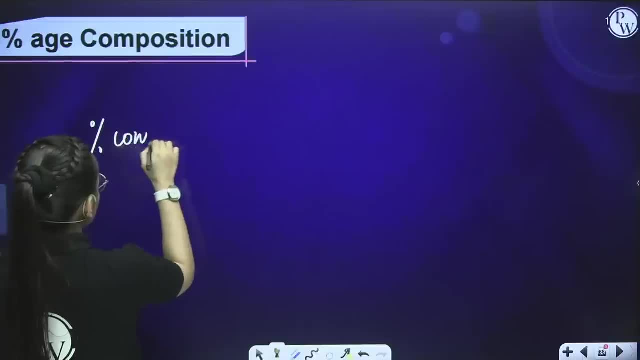 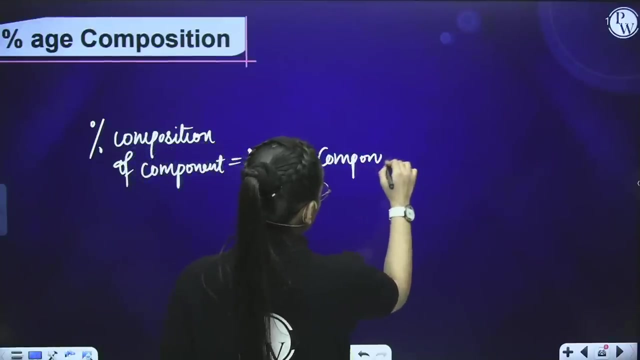 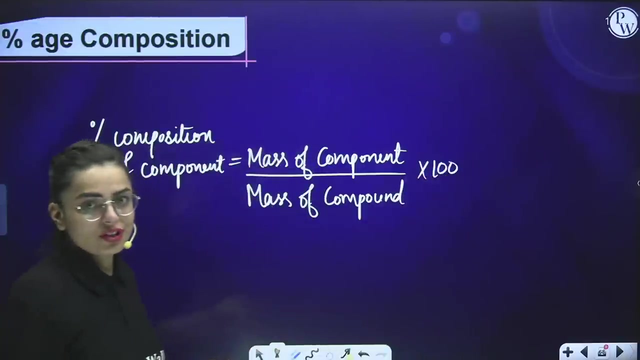 So the percentage composition of any component is equal to the mass of component. whosoever we needs to find out the percentage that will be written on the above, divided by mass of the compound, full compound into hundred. Now let us take an example for the students. We have the example: calculate percentage composition of carbon in CH4.. 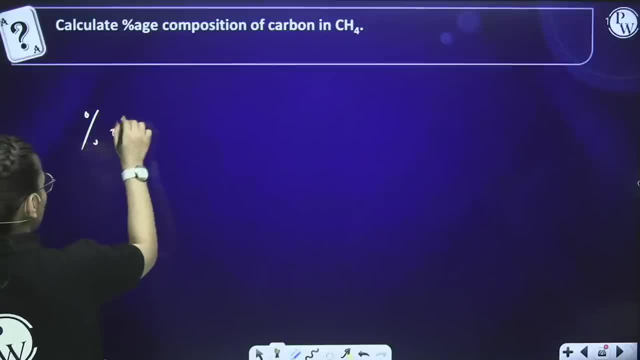 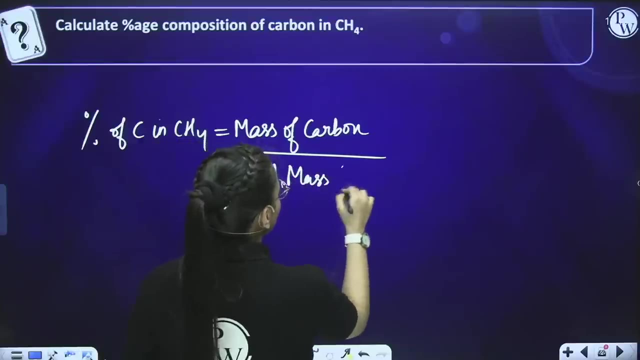 So it is very simple. First of all, percentage of carbon in CH4 will be mass of carbon divided by total mass, total mass of compound. What is the compound here? CH4 into hundred. So now students, what is the mass of carbon? It is 12.. 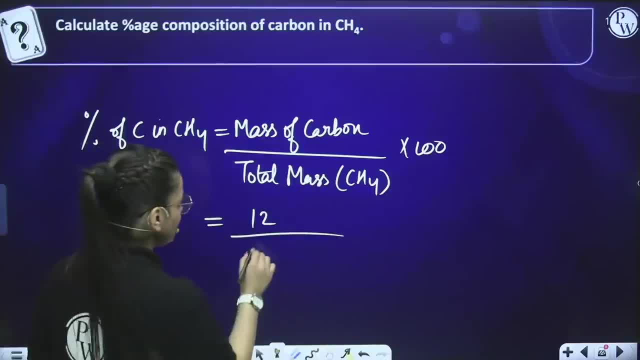 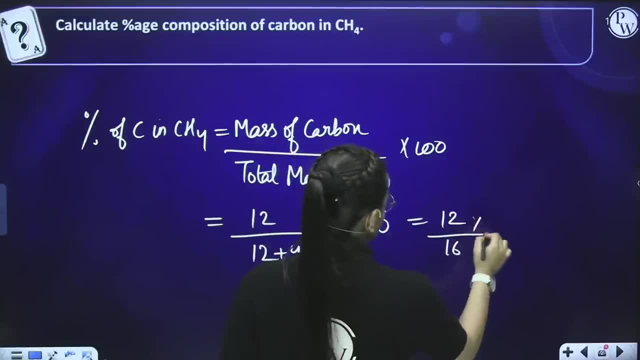 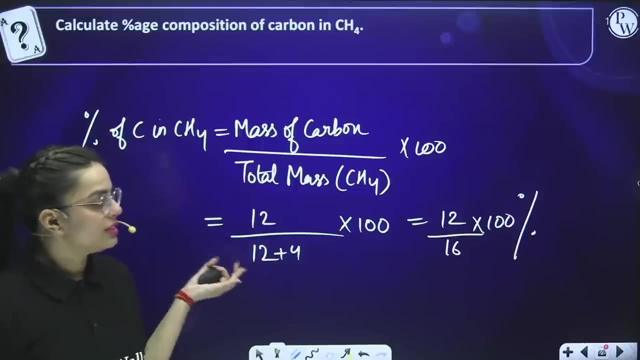 What is the total mass CH4 molecular mass? It is 12 plus 4 right into hundred. Hence it will come out to be 12 divided by 16 into hundred. This is the percentage composition for carbon in CH4.. Students, we can further divide it like: if we go on 2 table, then it: 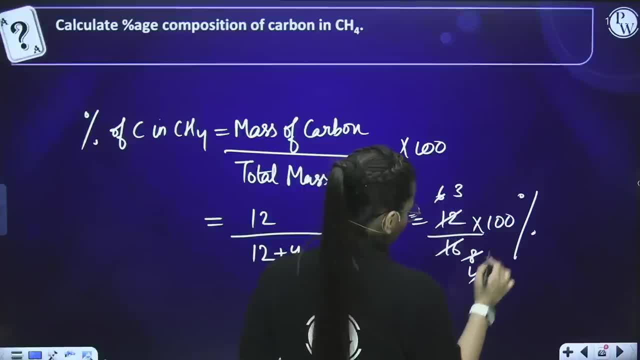 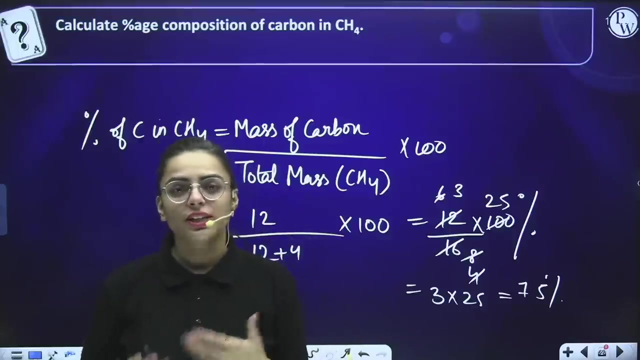 is divided further, It is 75%. that means carbon is present 75% in CH4. and once they ask you about one component, they can even ask you about another one, for example hydrogen. So hydrogen you can calculate in the similar way like you did in the carbon way. First you will keep the mass of component. 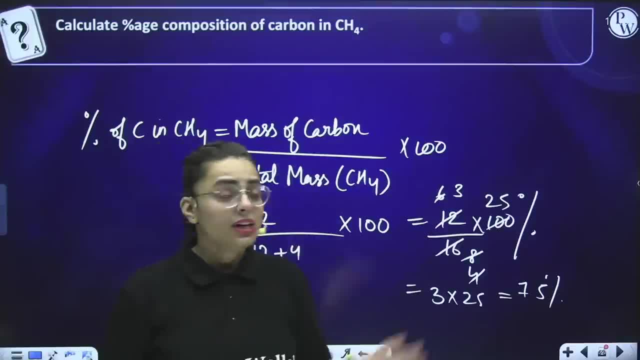 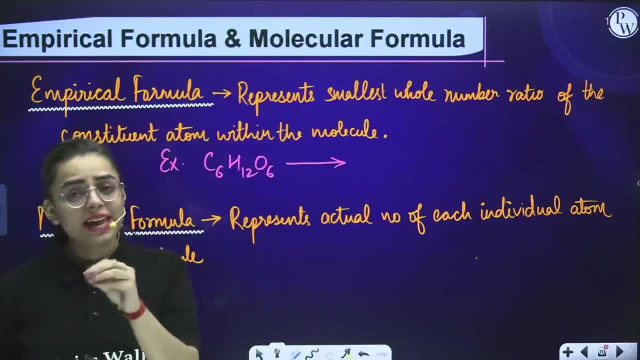 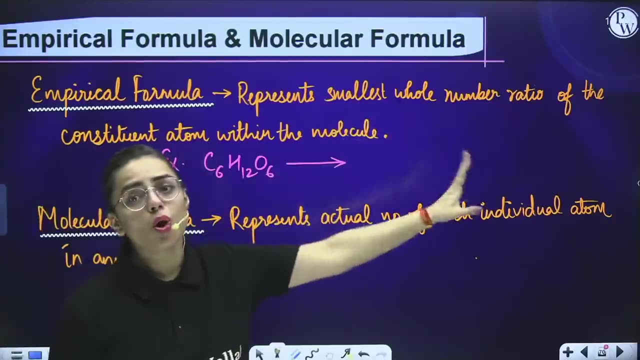 of hydrogen divided by total mass into hundred. Now this is going to help us in empirical and molecular formula. What do you mean by empirical and molecular formula? See, whenever a compound We observe has two formulas, The empirical formula represents the smallest whole number. 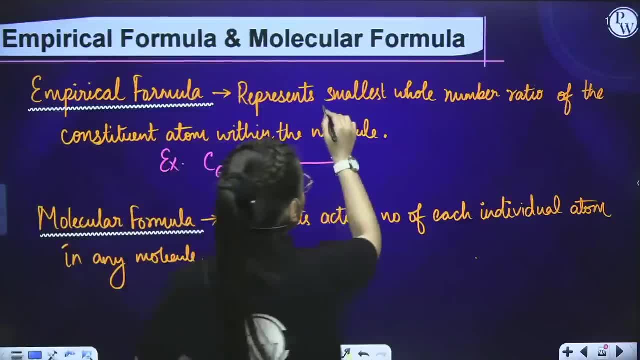 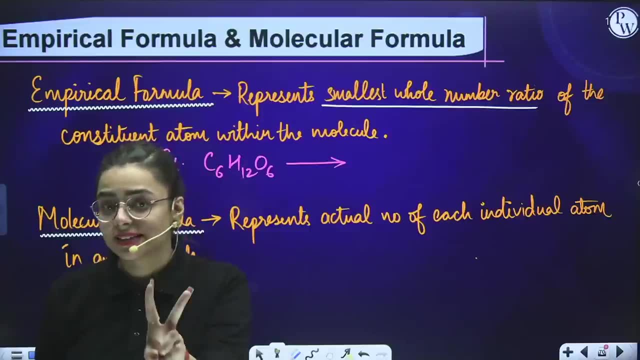 ratio Smallest whole number ratio. this is the most important line that you need to remember Whenever you see a compound. a compound can be represented in two categories: empirical as well as molecular formula. So in empirical, we need to see the smallest whole number ratio. 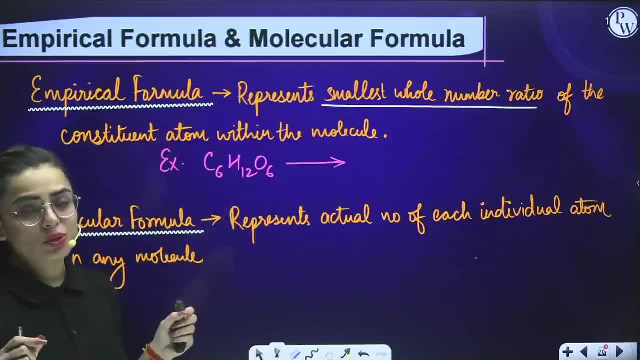 for example, this is our compound: What will be the smallest whole number ratio, That the number through which they can be divisible, Like 6, 12, 6, they can be divisible on 6 table. So if I divide this then it will be C1H2O1 that. 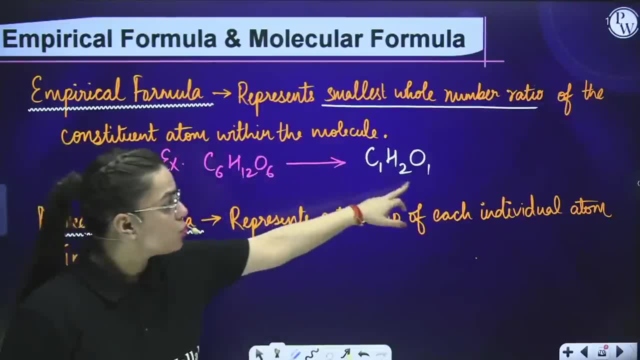 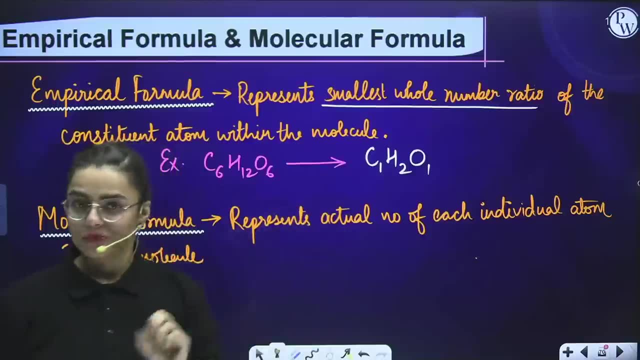 means CH2O. CH2O is the simplest whole number ratio that means for this compound. this is its empirical formula. Clear Now, What do you mean by molecular formula? Molecular formula represents the actual number of individual atom in any molecule, For example in C6H12O6. What is the actual number of atoms? It's not a number, It's a number. Let me explain. So it's the number of atoms it represents, say, in a molecule. We know that a molecule is a number. Remember, we know that the number of atoms is mean in a molecule. So if we put 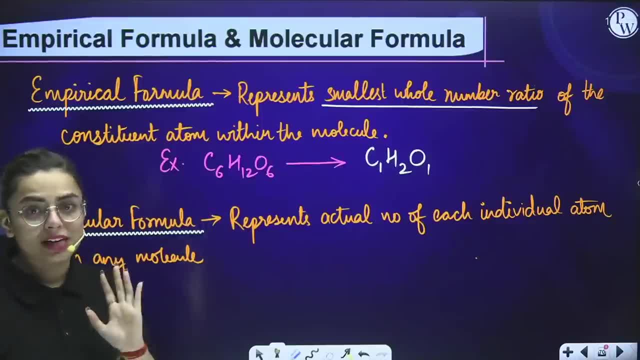 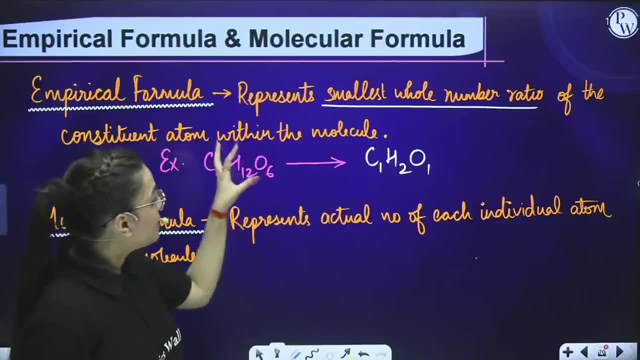 number of carbon: 6. what is the actual number of hydrogen: 12. what is the actual number of oxygen: 6. so molecular formula represents actual number of the each individual atom, while its simplest whole number, ratio, represents its empirical formula. now, students, what is the relationship between? 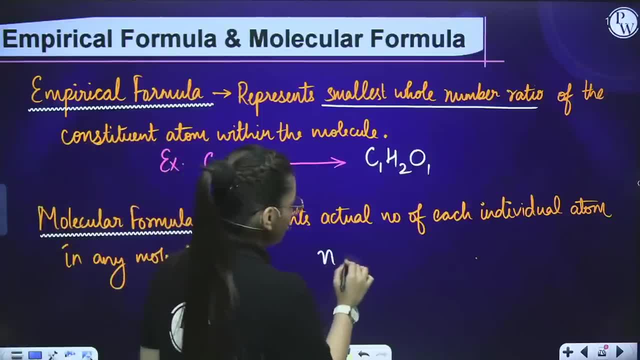 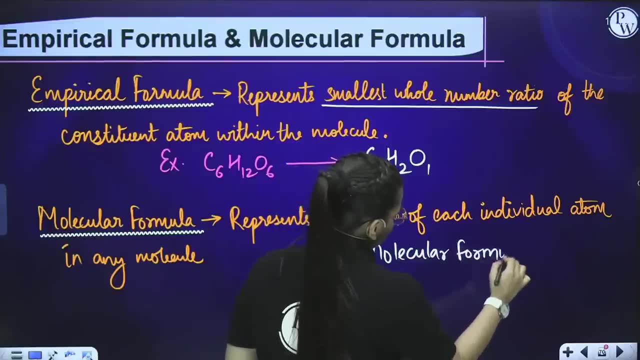 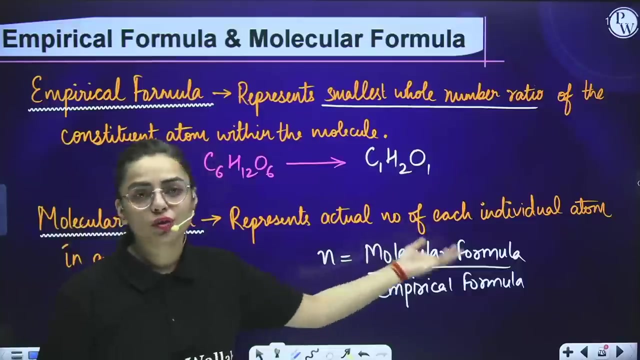 empirical formula and molecular formula. so i would say n is equals to molecular formula divided by empirical formula. so this is one of the relationship. what we can say it molecular formula- we can take molecular weight instead of this- and an empirical formula- we can take empirical weight instead of this. 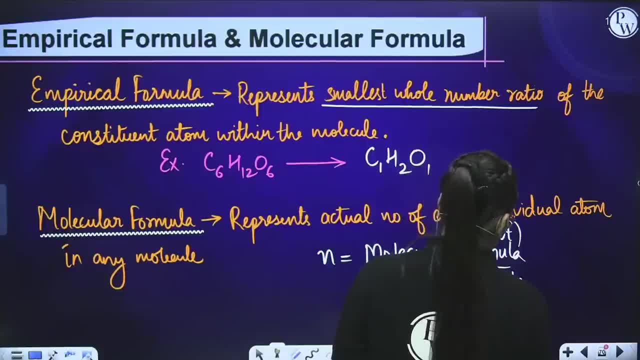 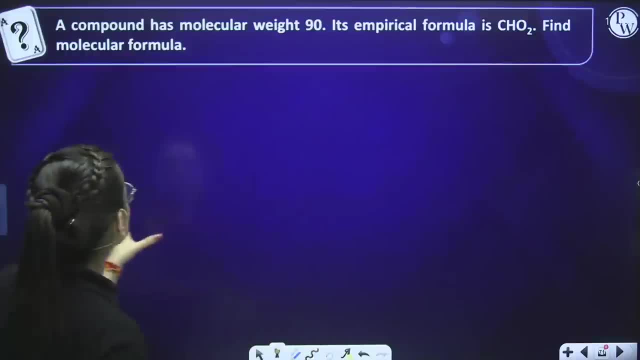 because we need to calculate weight here for both of these, right? okay, now i'm taking an example for you people where we are going to use this formula. The question is: a compound. is molecular weight 90, right? Its empirical formula is CHO2.. Find the molecular formula Now, students. 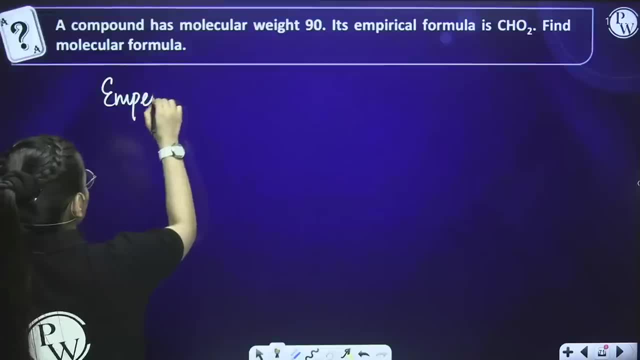 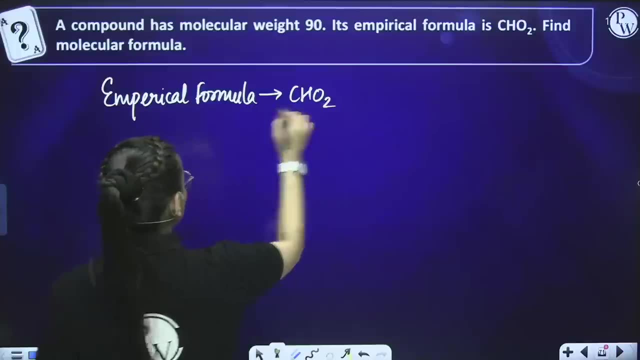 we have been given empirical formula. We have been given empirical formula. Empirical formula is CHO2.. What will its empirical weight? Empirical weight: How many carbon? 1.. So 1 into carbon's mass, plus 1 into hydrogen mass, plus 2 into oxygen mass. Carbon mass is 12.. Hydrogen mass is 1 and 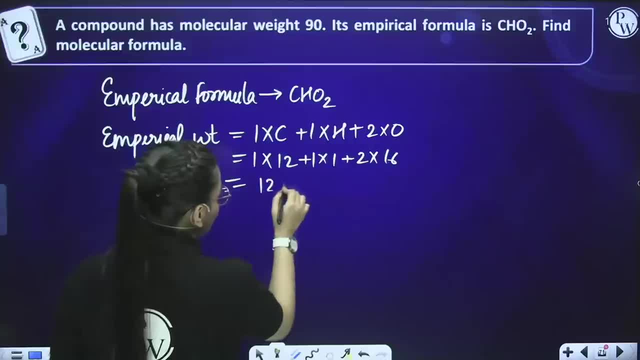 oxygen mass is 16.. So when I calculate it it's 12 plus 1 plus 32.. That means 13 plus 32.. It means 45.. 45 is the empirical weight right. We have calculated empirical weight from empirical formula. 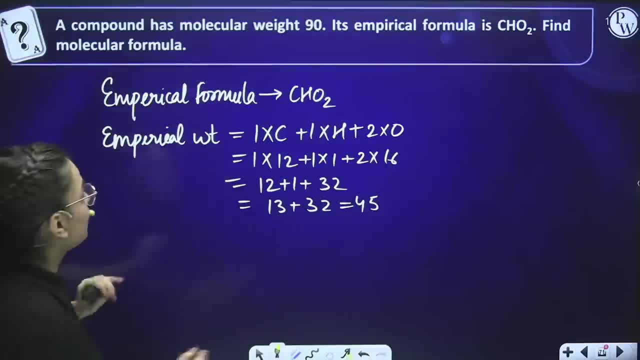 but we need to calculate molecular formula. We have molecular weight with us. We have molecular weight which is 90 with us. Now I have given you a formula which is: N is equals to molecular weight 90 divided by empirical formula or empirical weight. that is 45. What comes out to? 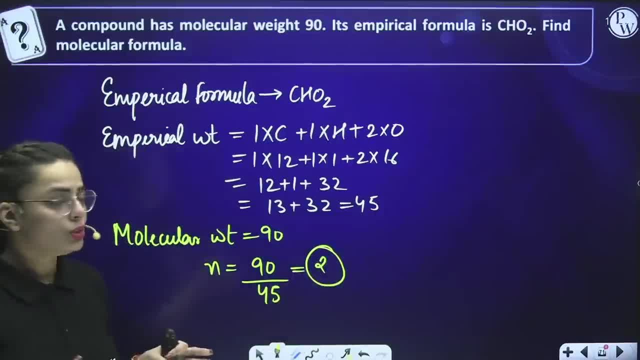 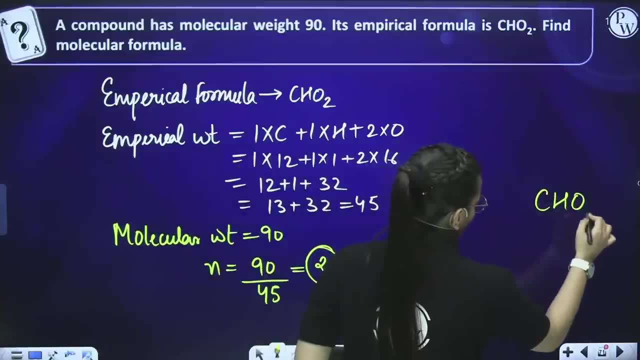 be? N? N comes out to be 2.. So what is N? N comes out to be 2.. So what is N? N comes out to be 2.. So what is N? N comes out to be What we will do now. we have our empirical formula, which is CHO2, which is CHO2, so I will 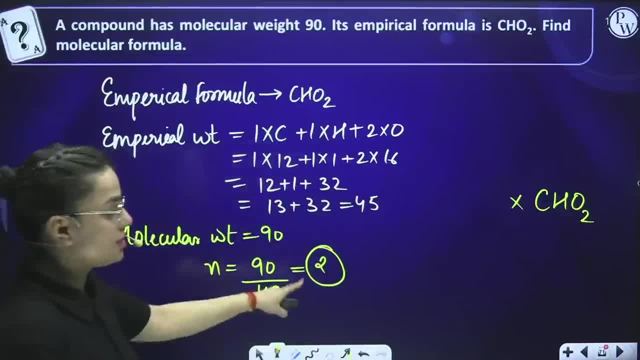 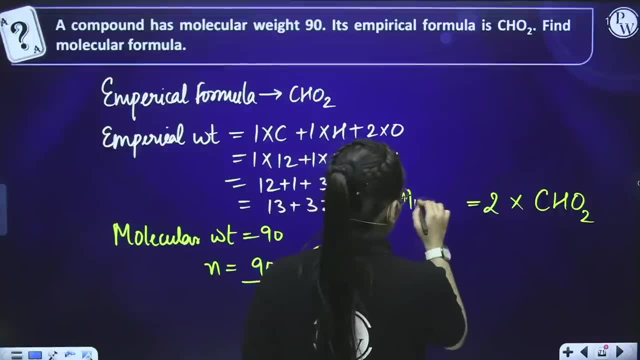 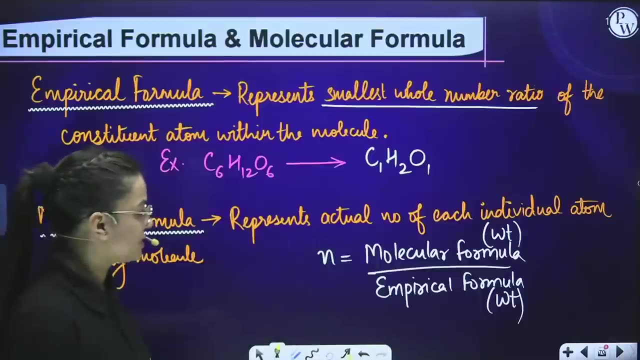 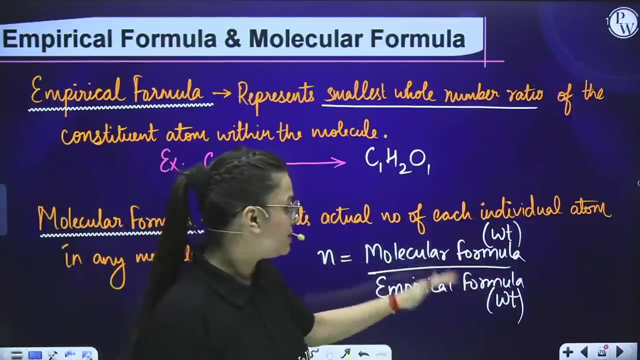 multiply. I am going to multiply this with 2 so that I can get my empirical. sorry, so that I can get my molecular formula, because I told you in the previous case same this question, there are two kinds of formulas. one is molecular formula divided by empirical formula. the other one is molecular weight divided by empirical weight. we have used both. 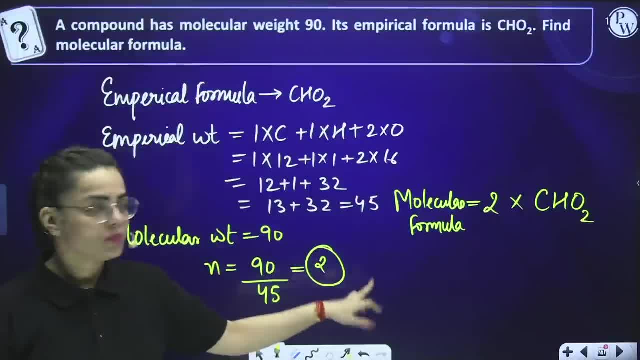 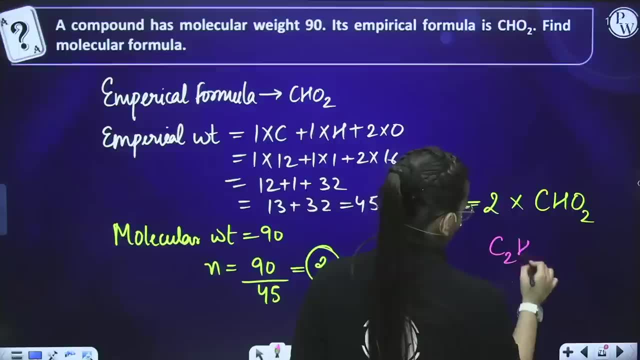 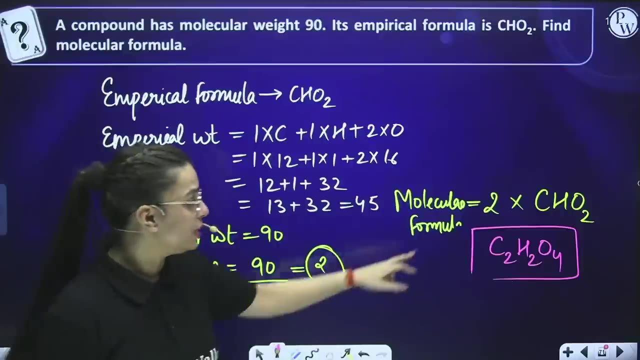 of the formulas. first we use the weight one, then we use the molecular formula one. so what will it comes out to be? it comes out to be C2H2O4. so this is going to be the molecular formula. like this, you need to put it into the down, at the base, not on the top. you have 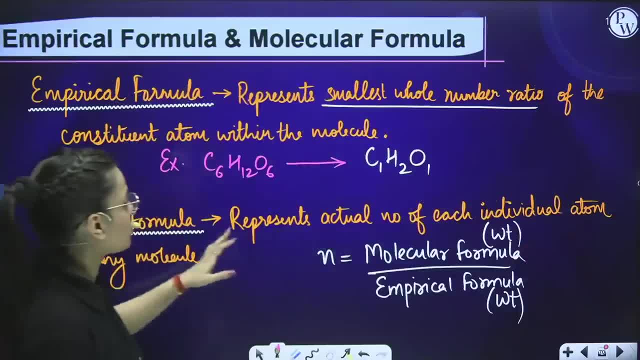 to write it C2H2O4.. Because here, also in the previous case, I told you what is the number that divide it into the simplest whole number ratio, right? so we are dividing it. that is n, right? so here the complete number of atoms it represents. 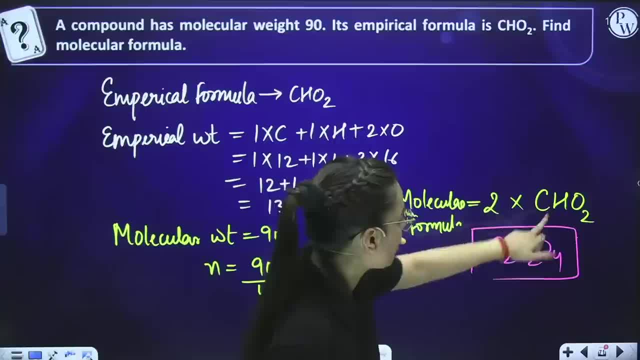 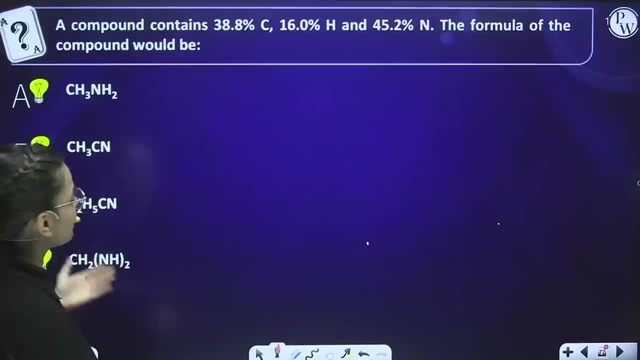 the 1000, while it represents the simplest whole number ratio. and this is empirical formula, this is we molecular formula, so you can calculate these kinds of questions in such a way. Now, students, proceeding towards the next kind of question, what you need to do is most of 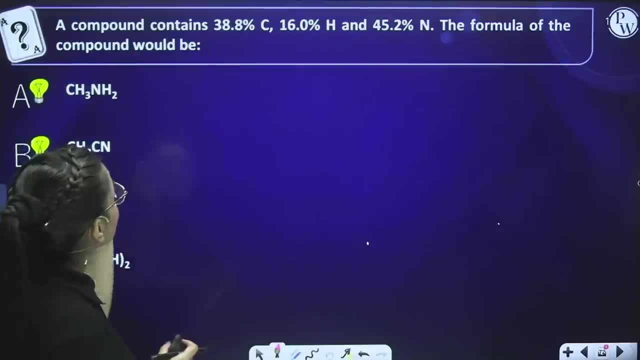 these questions are observed. a compound contains 38.8 percent carbon, 16 percent hydrogen and 42.2- 45.2 percent nitrogen. the formula of the compound would be: first of all, you need to write element. first of all, you will write about element. how many elements are present? this carbon? 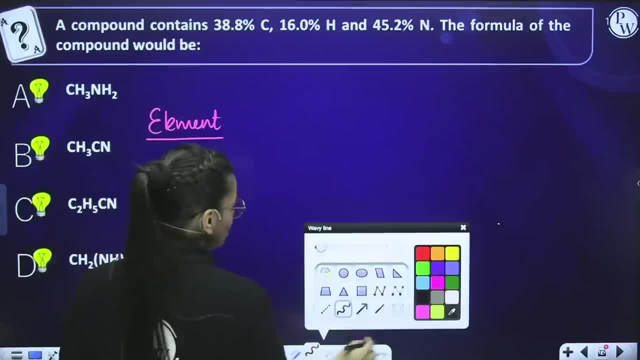 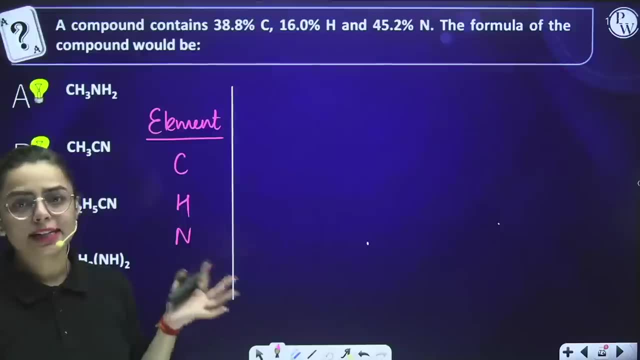 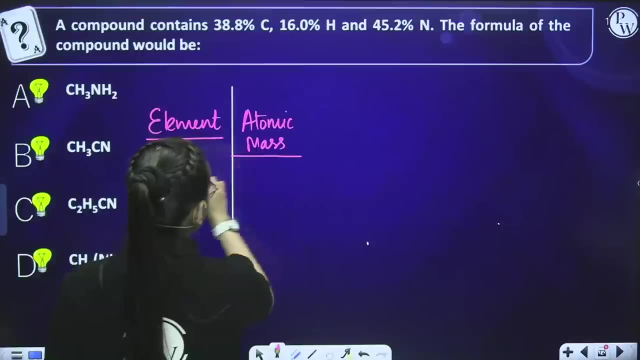 hydrogen nitrogen. the next thing. students, what you need to write down is the next thing. you will write the percentage, composition, or you can write atomic mass first. so i'm going to write atomic mass first of these compounds: what is the atomic mass of carbon? 12. what is the atomic mass of hydrogen? 1. what is the atomic mass of nitrogen? it's 14 right now. the next: 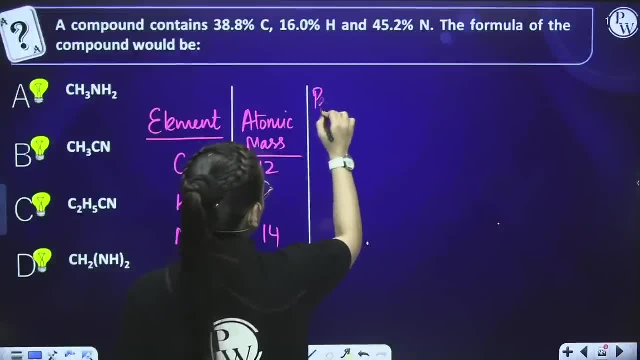 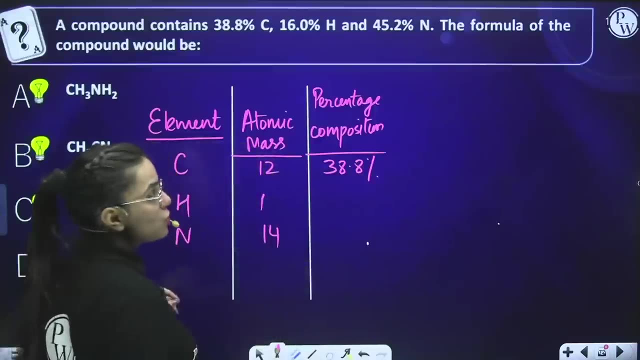 thing that we are going to write is the percentage composition that is given to you in the question. percentage composition now. what is the percentage composition for the case of carbon? it is given as 38.8 percent. what is the percentage composition for hydrogen? it is given to us 16 percent. what is the percentage composition of nitrogen? it is. 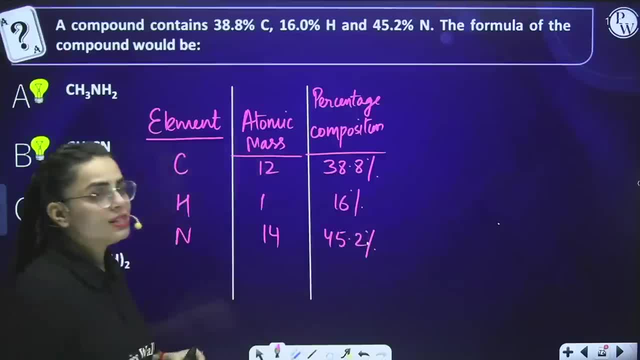 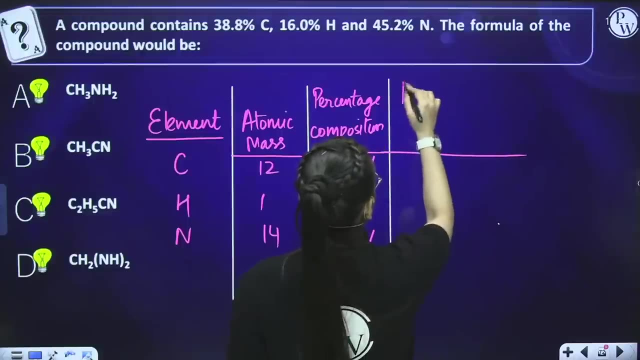 given to us 45.2 percent students. now the next step is going to the going to be that we need to find the stoichiometry, that is, we need to divide percentage composition by atomic mass. so what will come? let us see. we will divide percentage. 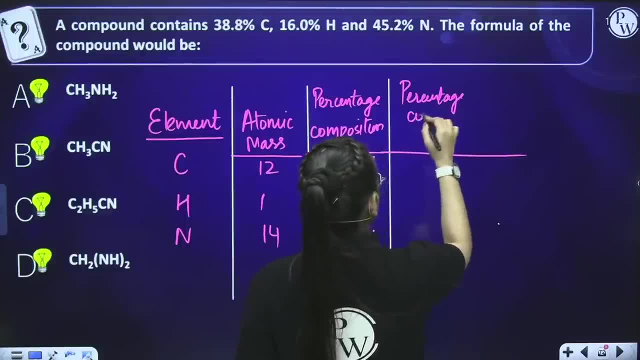 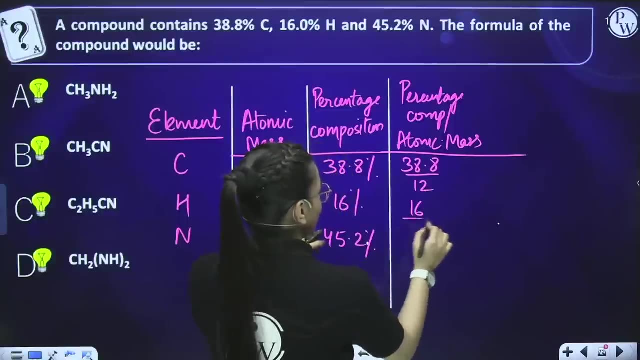 composition by atomic mass. so in the case of carbon, it will be 38.8 divided by 12. for the case of hydrogen, it will be 16 by 1. now for next case, it will be 45.2 divided by 40. now, students, when we are going to solve it out, it comes out to be 3.23, something it comes out to. 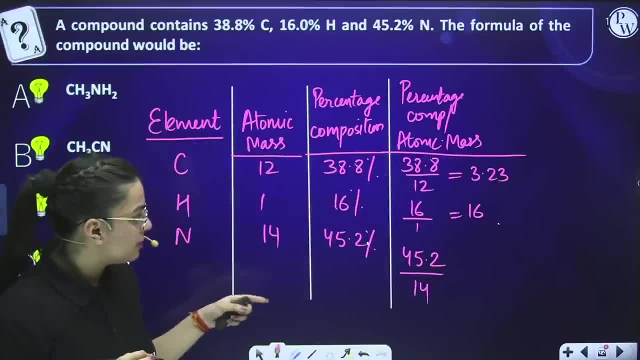 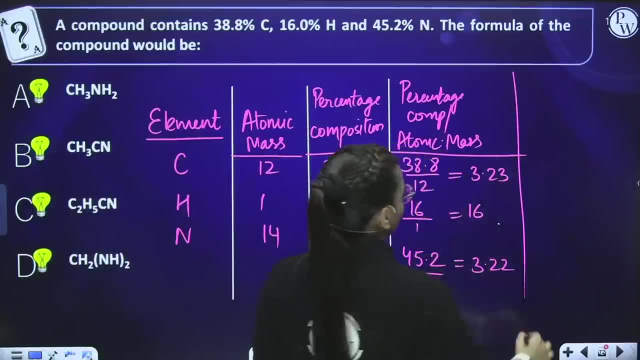 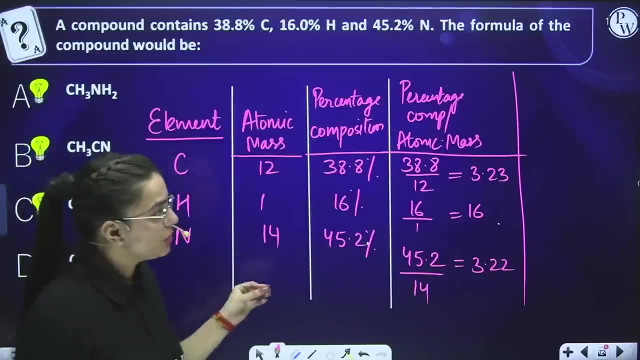 be 16 students, then here it comes out to be almost 3.2322, something only right. so we have just calculated these. now we have to put into the simplest form students. how to put them into simplest form? let us divide it in such a way that we get the answers like the: 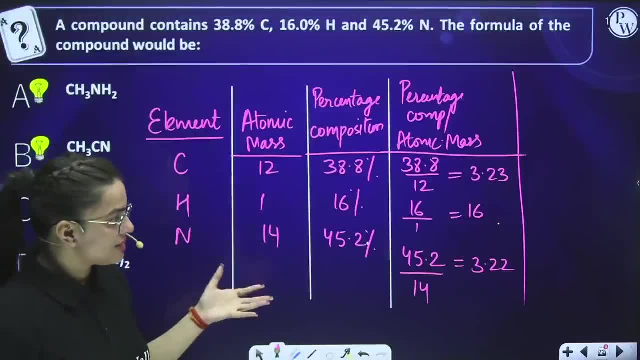 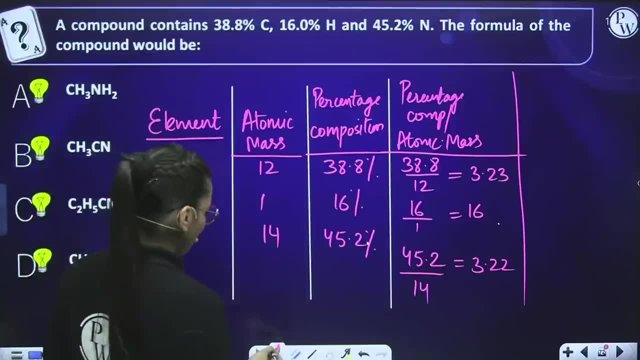 first one, we have done 3.23, then we have done 16, then is 3.23. what is the number that divides all of these? the number that divides all of these here, it would come out to be: it would come out to be: 1, 5 and 1. 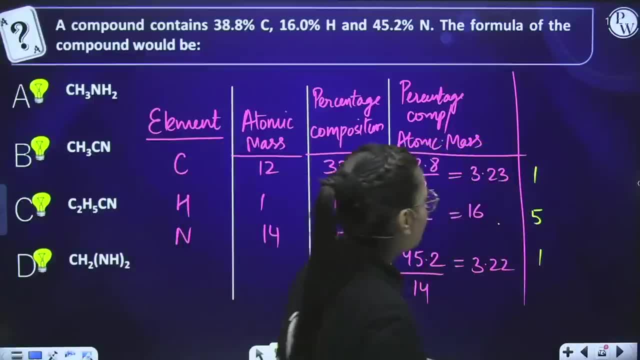 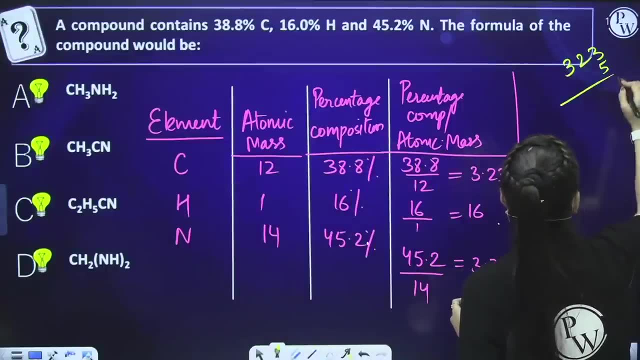 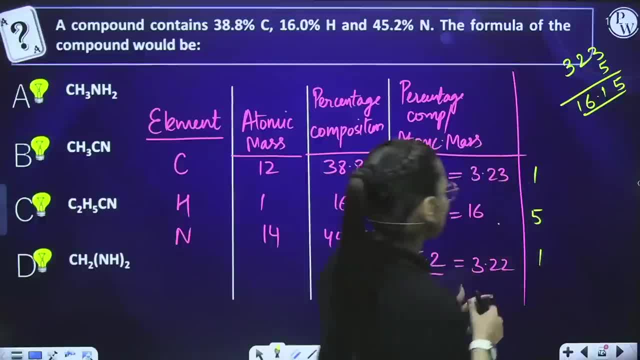 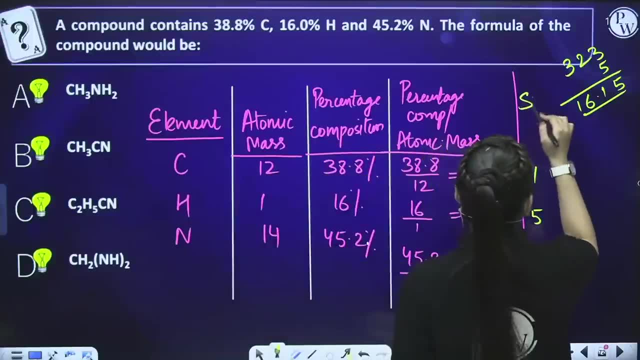 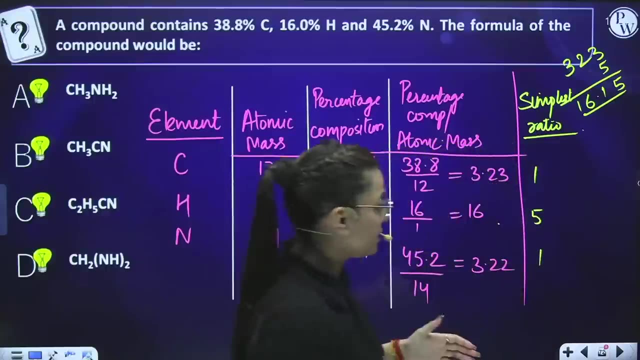 See, it is 16.15.. So it is approximately 16.. That's why we always take at the approximate situation, because it's the percentage composition. So this is our simplest ratio. This refers to as the simplest ratio. So what does we do? 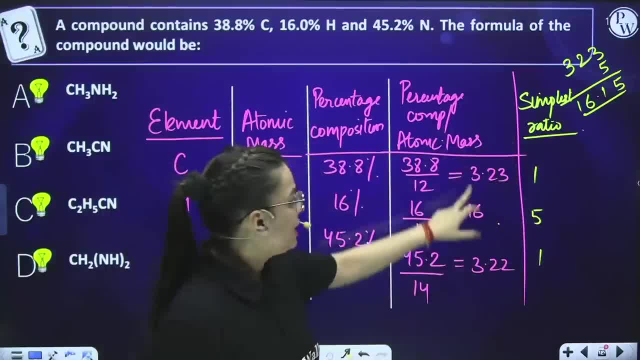 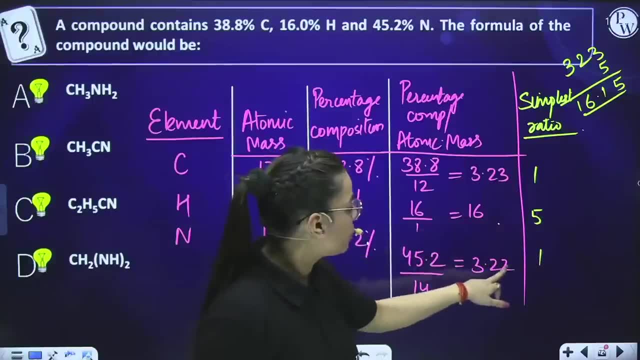 When we get this situation, we divide the smallest number with everyone. We are dividing 3.2 with 3.23.. We get 1.. We divided 16 by 3.23.. We get 5.. We are dividing 3.23 divided by again 3.23. 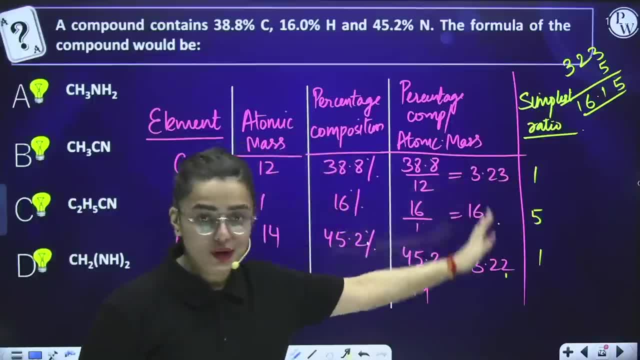 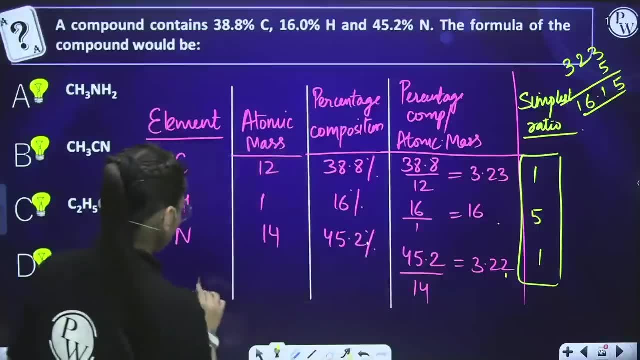 So we are getting 1.. The smallest number is being divided by all of them. So this is the simplest thing that we observe here Now what we have to do: Carbon base 1, hydrogen base 5, nitrogen base 1.. 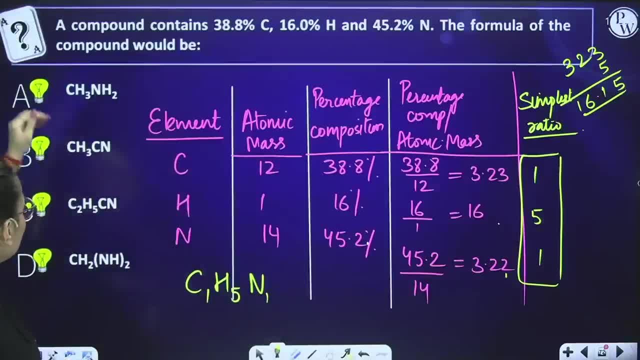 Now let us see the examples. you know the options here. In all of these options they have opened it up, So we also need to open it up: How many carbon- One carbon- In this case one carbon- is there? 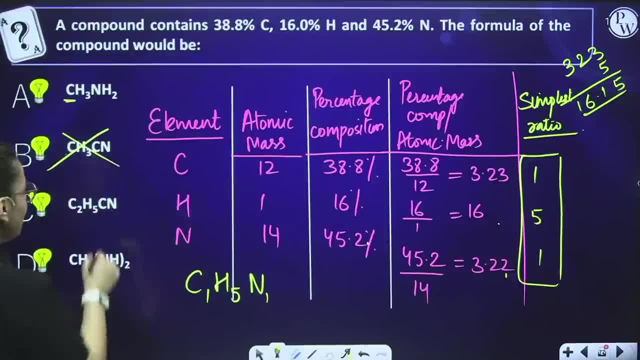 In this case two carbons are present, So B option is incorrect In this also. it is incorrect. In this case one carbon is there, Next 1 nitrogen and 5 hydrogen. Now 1 nitrogen and 5 hydrogen. 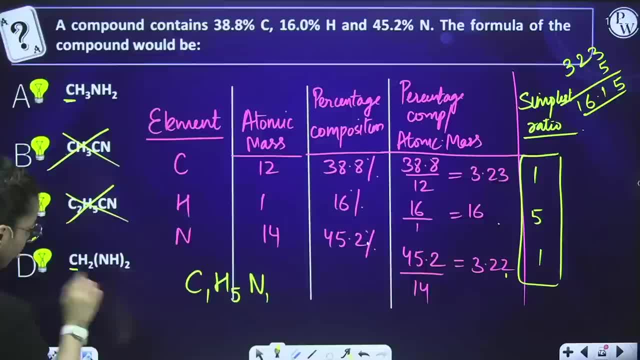 It is possible. Okay, here it is 2 to 4 hydrogen and 2 nitrogen. It is not possible. Hence our A option, that is, CH3.. NH2 is totally correct, students. So these kinds of questions can arise. 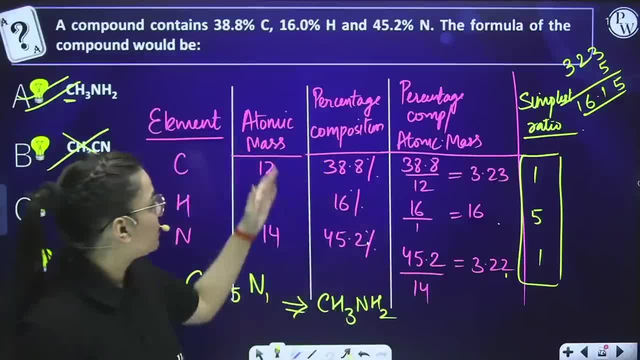 First of all you need to write the atomic mass, Then you need to write the percentage composition which is given in the question, Then you need to divide them And after that you need to select the smallest one and divide them. 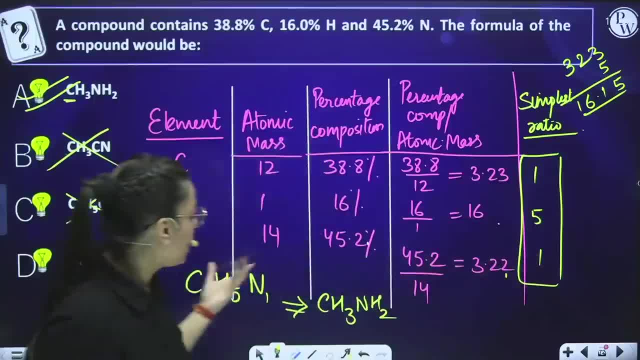 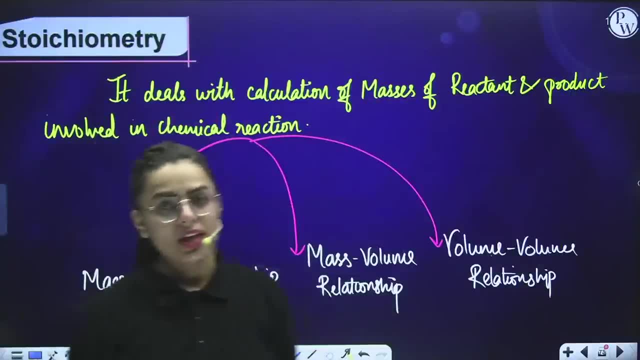 so that you can get the simplest number. Now the simplest number is put into the base and the formula is obtained. So, students, now we are moving towards the stoichiometry. What do you mean by the stoichiometry? Basically, stoichiometry deals with this. 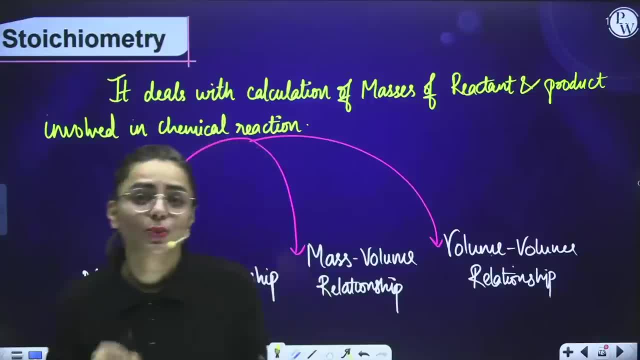 It deals with the calculation of masses of reactants as well as products in the chemical reaction. Whosoever mass we want to calculate, whosoever volume we want to calculate, with the help of stoichiometry we can do this. They establishes basically three kinds of relationships. 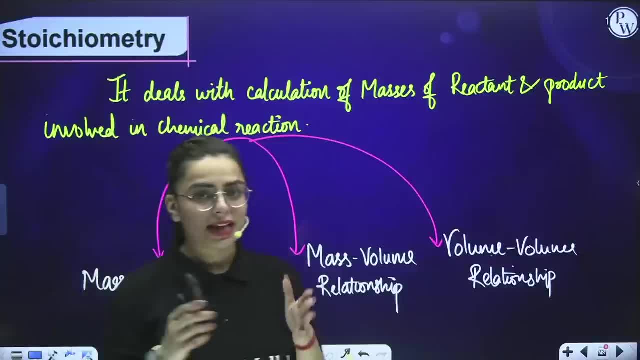 The first one is mass-mass relationship, For example, when two reactants react together and they form product. So in the question what they will do, They give you the mass of reactants and they will ask you the mass of product. 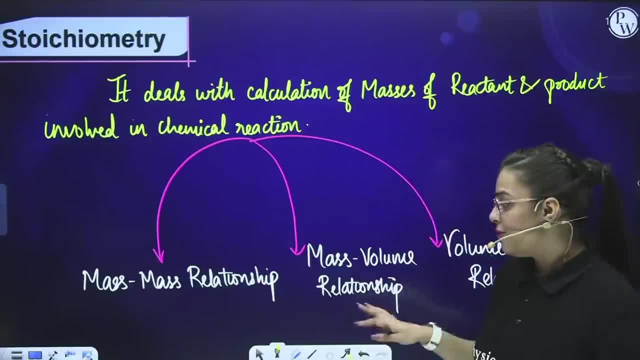 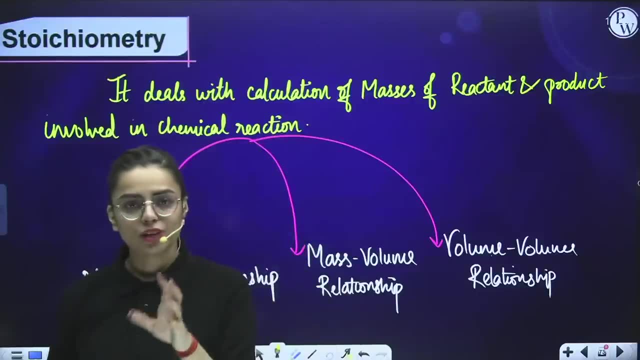 So that comes under the category of mass-mass relationship. When they give you mass-volume relationship, what do you mean by that? One of the question: one of the reactant will be given mass. one of the reactant will be given as volume. 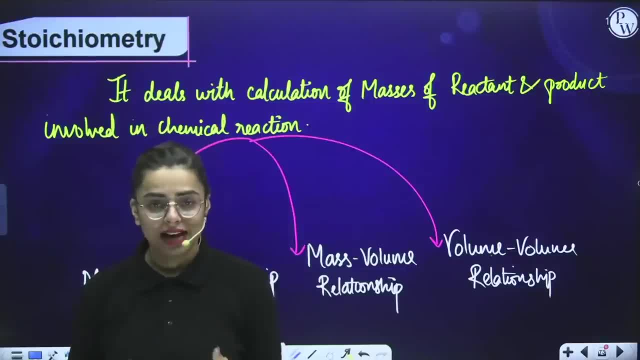 and they will ask you about the mass of the product. So these kinds of relationships are mass and volume relationship. The last kind is volume-volume relationship, when the reactants volumes are given and the product volume is being asked. So, students, one of the stoichiometric question is in front of you. 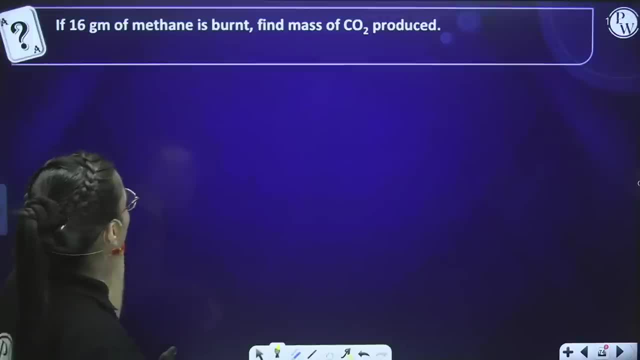 How to do. I will tell you. If 16 grams of methane is burnt, find the mass of CO2 produced. So see, methane is burnt When it is burnt, right? So when methane is burnt, what happens? 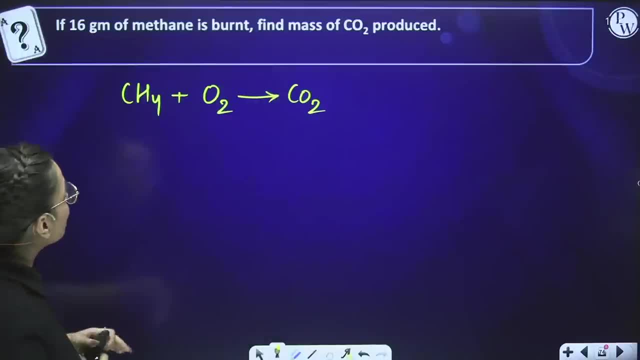 What happens is CO2 here is produced right. So what we observe here is what we need to find out: the mass of CO2 produced here. We need to find out the situation, and also water will be produced here right Now. the very first thing, the very first step that you need to do is balance the equation. 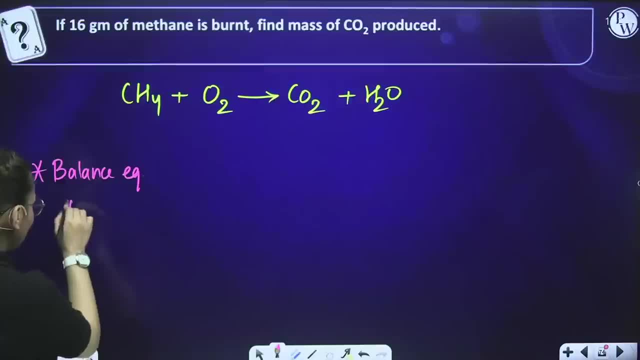 How to balance the equation. Write reactant- this side. write product- this side. How many atoms are present at the reactant? First of all, we take off carbon atom. Carbon in the reactant side is 1.. In the product side it is also 1.. 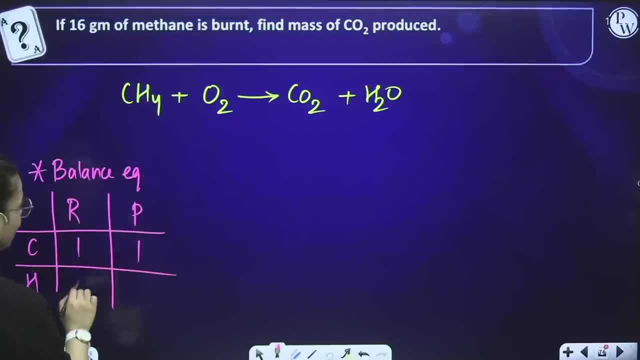 Okay, the next one is hydrogen. In the reactant side, it is 4.. In the product side it is 2.. Next is oxygen. In the reactant side, it is 2., While in the product side it is 3.. 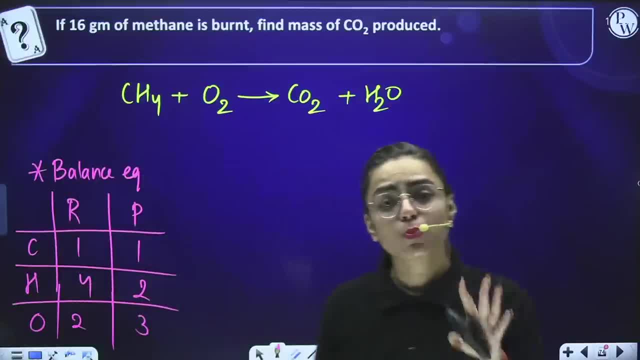 So we need to balance it out. That means we need to equalize it in both the ways. Now, students, first of all, we can multiply this product, side hydrogen, into 2, so that it is equal to 4.. So what I am going to do? I am writing 2 here so that it is multiplied. 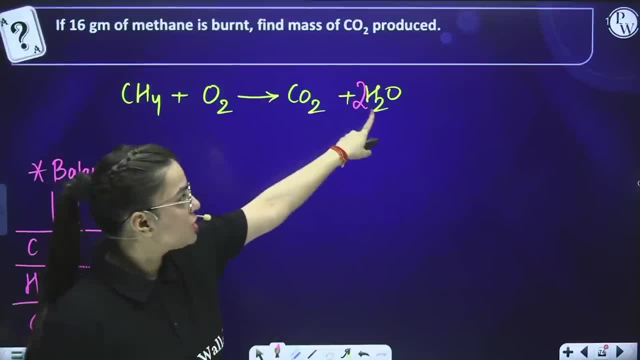 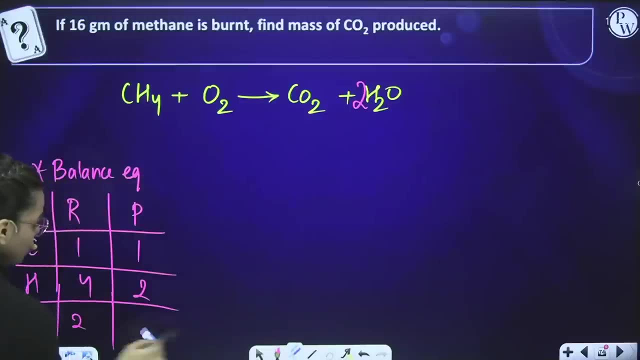 Now, after putting 2 here, hydrogen is 4, but oxygen is also 2.. That means on the product side we have 2 plus 2, 4 oxygen. We have now 4 oxygen with us right Now. students. 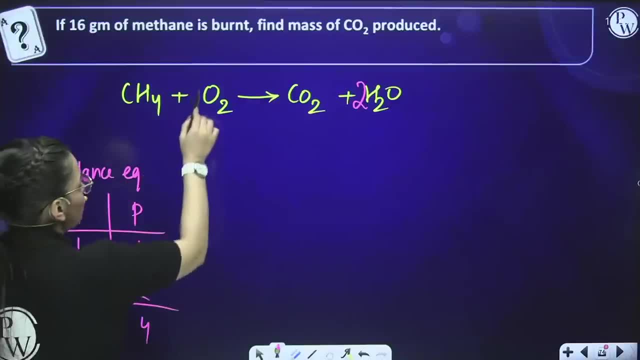 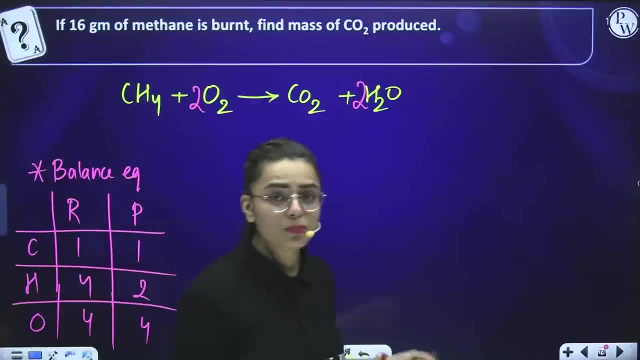 but on the reactant side 2 oxygen are present. That means we need to multiply here with 2.. So here it is, 4. Now check all the elements that they are equal in both the sides, in reactant and product. 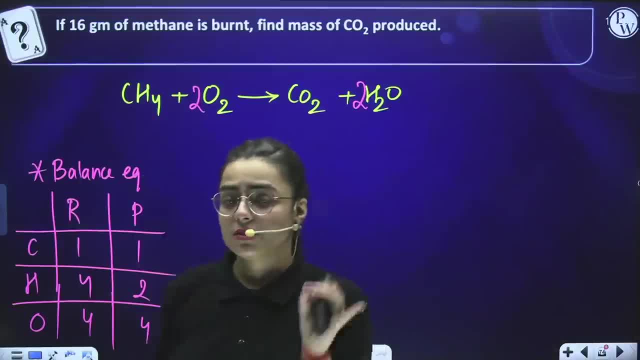 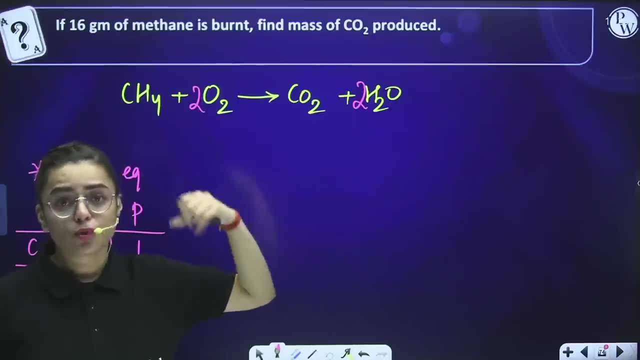 Then yes, it is equalized. Why did I this? this Because stoichiometry is the most important role we need to understand to calculate mass-mass relationship, mass-volume relationship, volume-volume relationship. right Now, students look here. 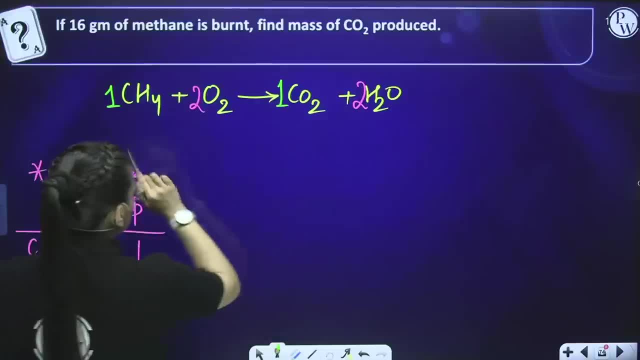 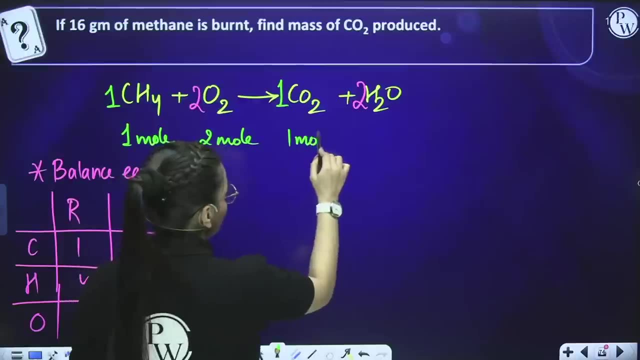 Here it is 1.. When nothing is given, we consider it as 1.. Here it is 1.. It means 1 mole. It means 2 mole. It means 1 mole, It means 2 mole. Now, what do you mean by this? 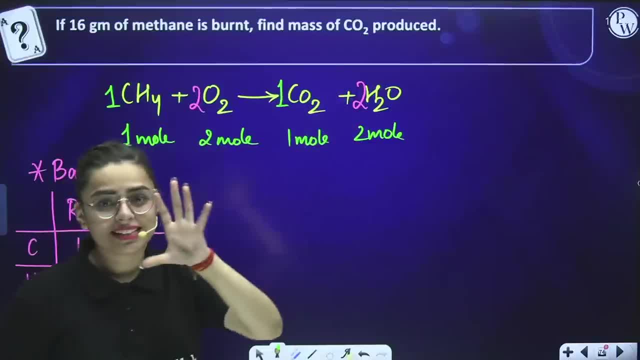 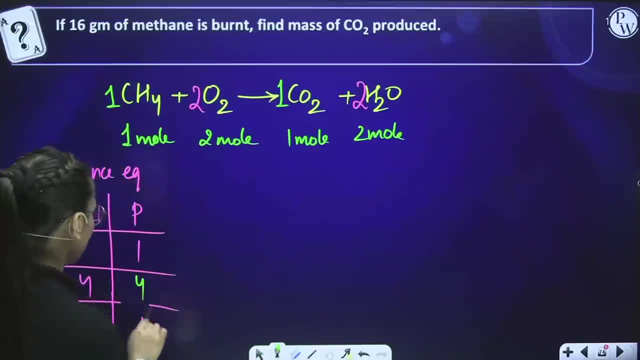 These stoichiometry are the relationships that are being established students. These stoichiometric basically are the relationships Currently. correct this here. Now, hydrogen is also 4, right, These are equalized here. These are also 4.. 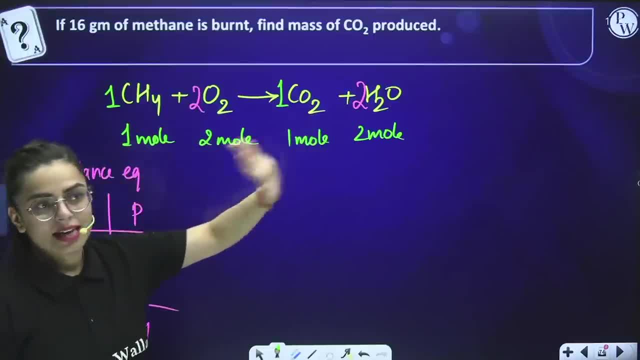 Even oxygens are also 4 on the both the sides. Hence we have done this right: 2 plus 2, 4, 2 plus 2, 4.. Now how to calculate the mass of CO2 produced. 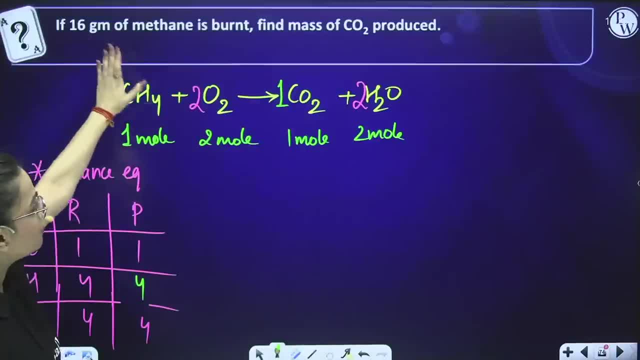 See students. what happens is they have given us the mass of methane, CH4. And we need to calculate the mass of this. So I would say 1 mole gives 1 mole of CO2.. I can say that 1 CH4, 1 mole of CH4. 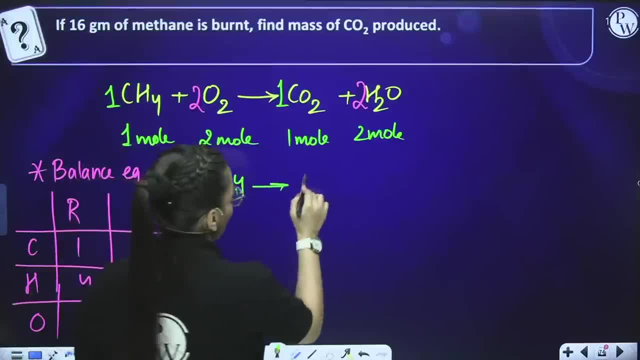 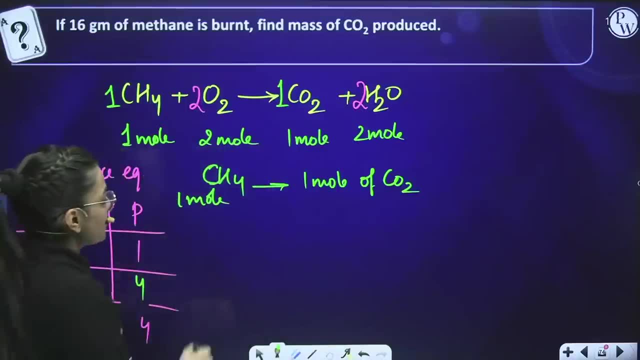 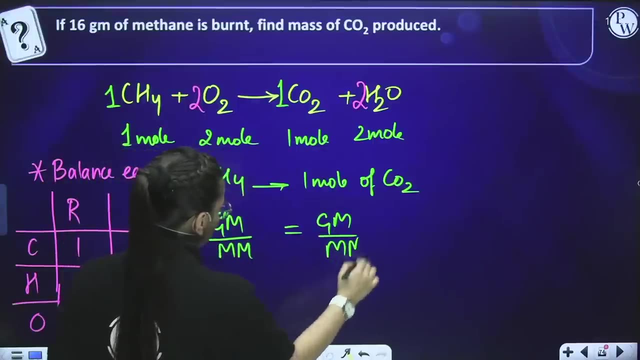 1 mole of CH4 gives 1 mole of CO2, right, So their moles are equal. And what are moles? Given mass by molecular mass? Here it is equal to given mass by molecular mass of CO2.. 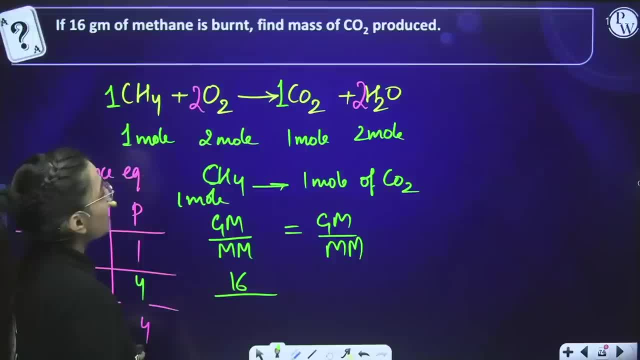 What is the given mass here of methane-16?? What is the molecular mass of methane-CH4?? It is 16. again, It is equals to given mass that we need to calculate, divided by molecular mass of what CO2.. Its molecular mass is 44, right. 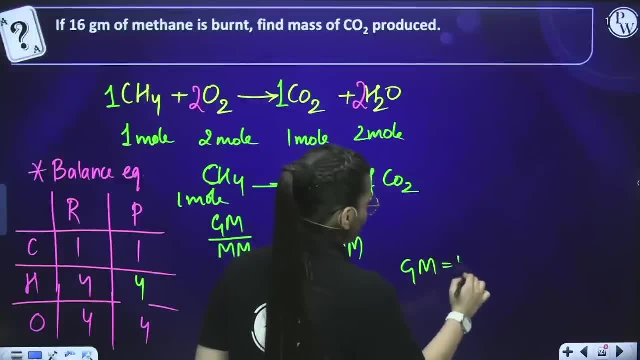 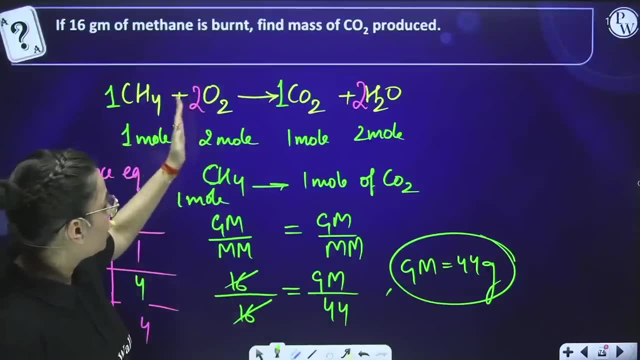 So if we will solve it and cross multiply, we get the given mass as 44 grams. Hence we can calculate. But most of the students can ask: why not we are considering this O2?? 2 mole gives 1 mole. 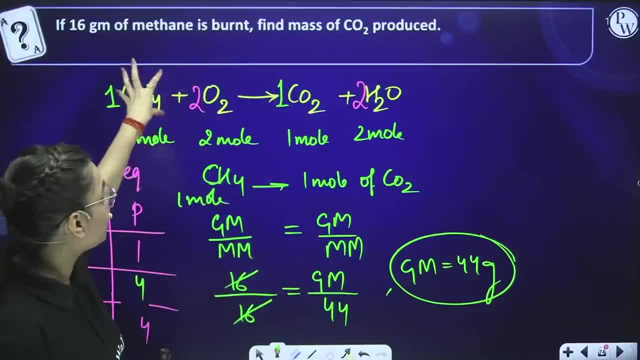 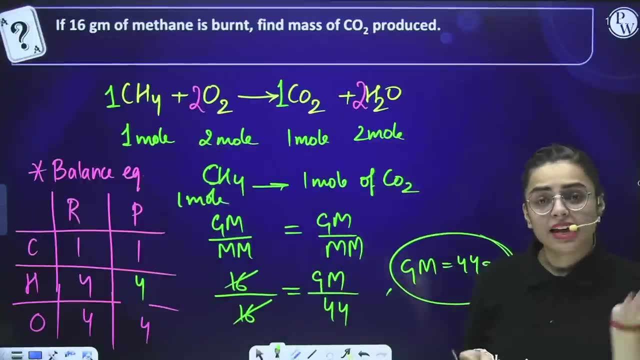 Because they have only given us 1 situation. When 2 situations are given, then we consider about limiting reagent. When 2 of the reactants information is being provided, then we first find out what is the limiting reagent And then we do. 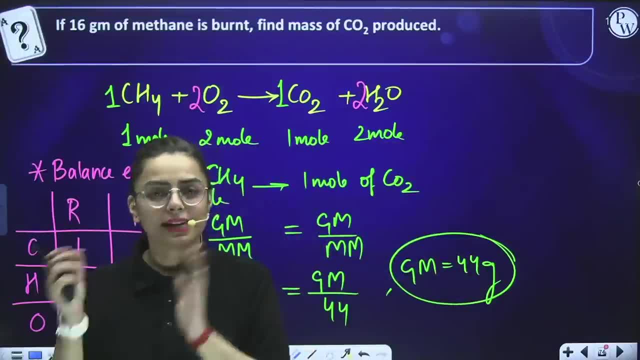 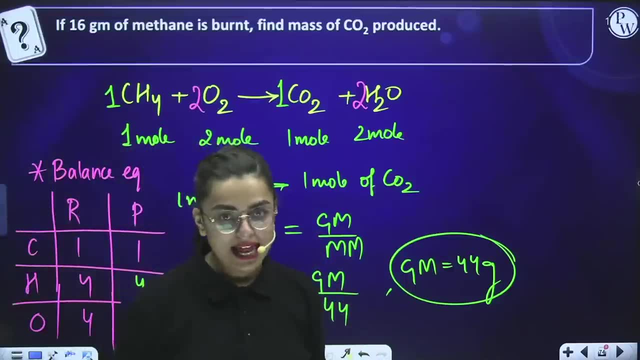 Then if only 1 equation is given to us, then we directly do according to the stoichiometry And we apply that if moles are equal, then their formulas will be equal and the answer will be calculated. So now, students, we have our topic: limiting reagent. What is limiting reagent? One day me and my brother were sitting and we were very hungry, So it was very late night time and my parents were sleeping. So I thought to eat something and I went to the kitchen. I took my brother with me. 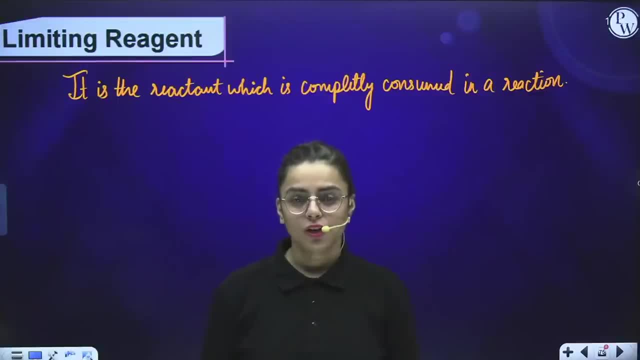 I said: what do you want to eat? He sent me: Let's have some burger, and all you know so. but but in the kitchen I observed: to make burger We need some buns and we need some buns or bread. 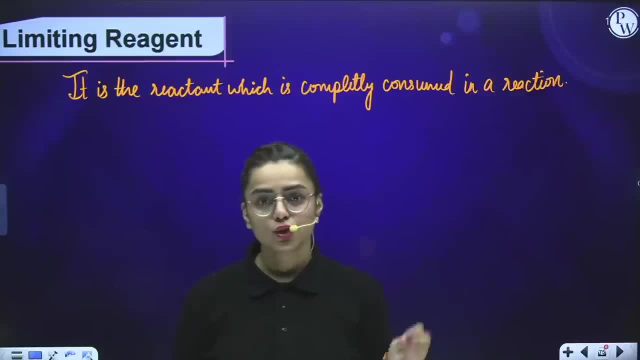 I would say: and along with that, we need some salad to put inside it, We need some cheese to put inside It. so what we did was: we need some buns and including other ingredients. We need these ingredients too. So to make burger, we had only and only two burger, two burger breads, right. 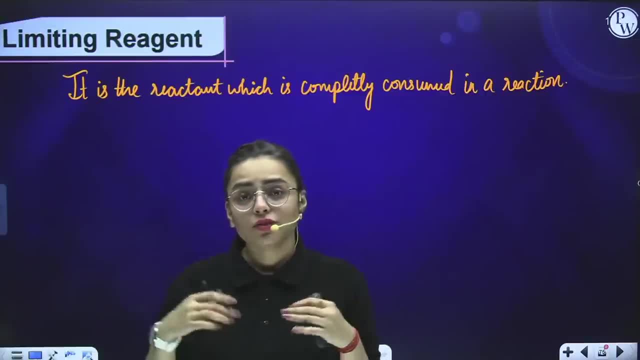 And we had ingredient in large quantity, but we were like we were only two of the persons, But but we were so hungry that we could eat four or five burgers, you know. so my brother said that I am very hungry, I want to eat more. 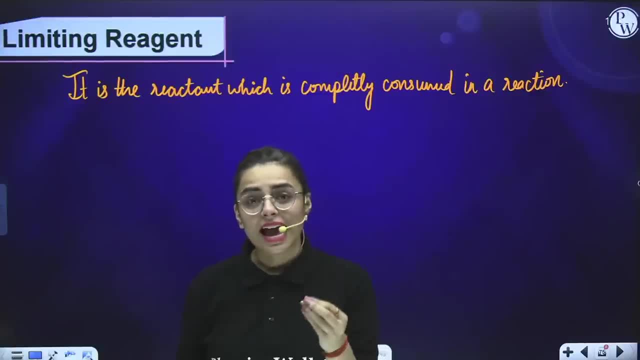 So what did this situations explain us? that? what is limiting reagent? in this case, Limiting reagent is the one which is present in less quantity and excess reagent is the one which is present in more quantity. So, according to this, I would say that limiting reagent is the reactant which is completely consumed in reaction. 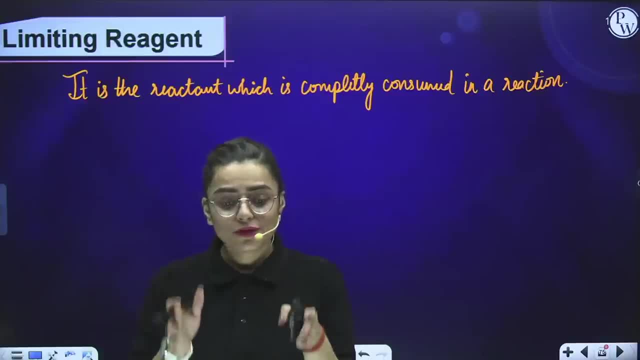 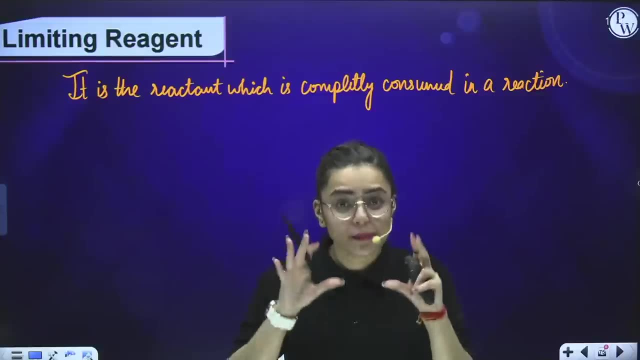 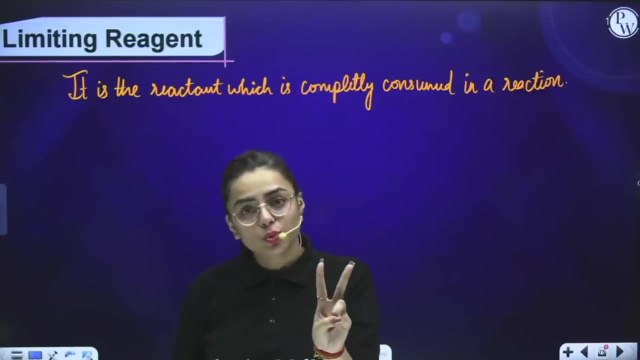 How I can explain you in the case of kitchen. See, if there are two breads, then only two burgers can be obtained, because bread is responsible, because it is As in limited quantity, it will make only two. if breads were more and ingredients were less, then we could have done something more and made something different. you know food ingredients with us, but the bread was only two. 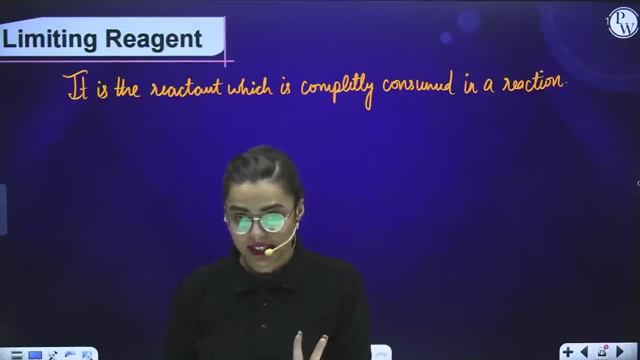 Then the burger produced will be only two, because it was the limiting reagent. That means limiting reagent. is that reagent which decides that how much the product will be formed? Okay, now see, it is the reactant Which is completely consumed in the reaction. 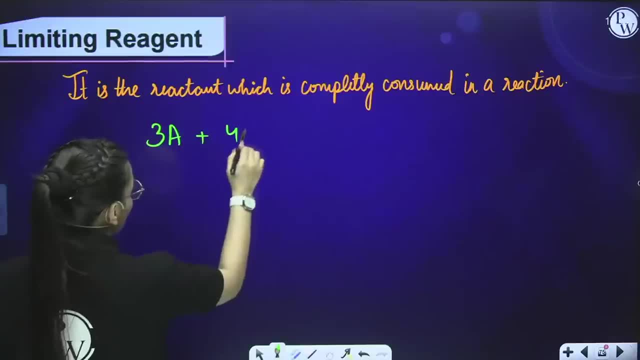 Let us take an example. For example, I have 3A plus 4B, gives 5C plus 60. Okay, and I am saying there are number of moles of A is 10, while number of moles of B is 20.. 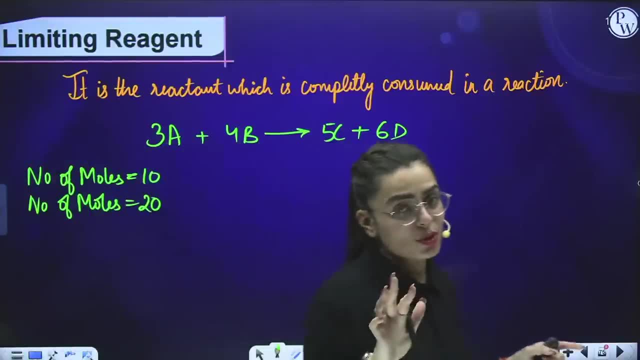 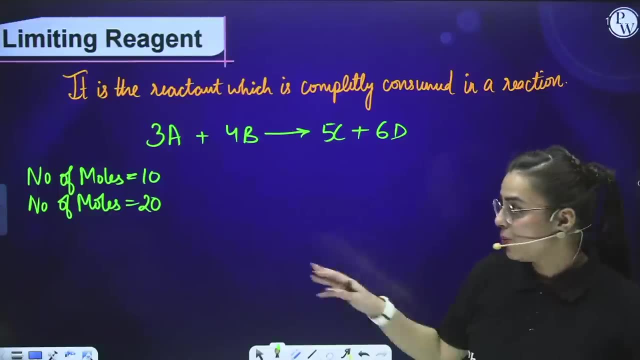 See, in the previous case only one situation was given. that was the 16 grams of CH4, and it was not given that What is the amount of O2? In it? now, in this case, both of the reactant number of moles are given. 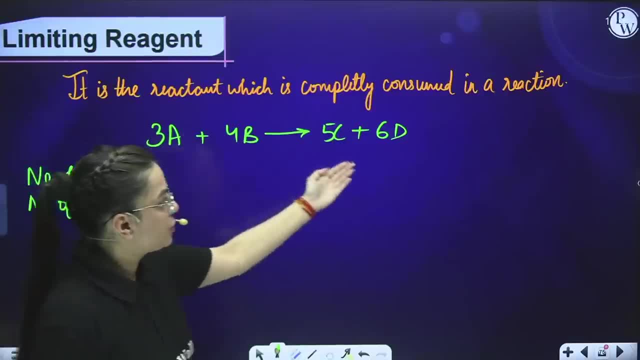 How do we identify that, with the help of which we can calculate C and D amount? Now we need to find out from both of these reactant which is a limiting reagent and which is excess reagent. The one which is limiting reagent will help us to calculate the amount of substances of the product right. 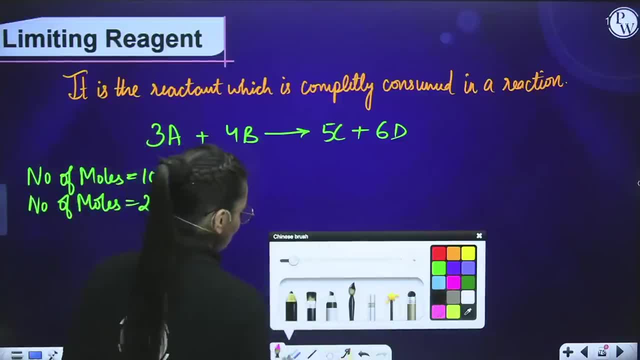 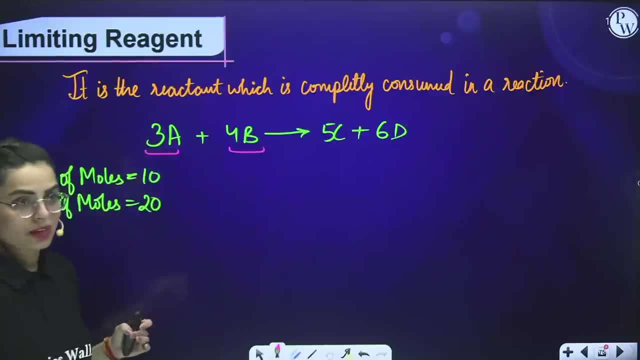 So see, what happens is: this is the balanced equation which is given to us. Now what we need to do is: we see that 3A here we see that 4B. we have reactant as 3A and we have another reactant as 4B. 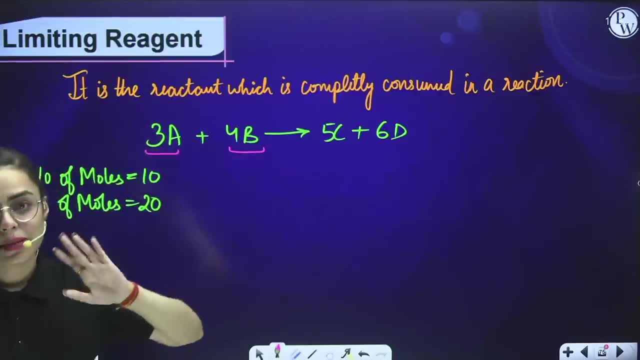 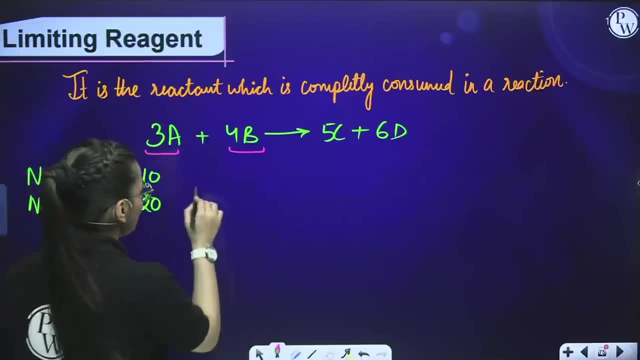 What is this? 3,, 4,, 5,, 6?? These are basically students. These are basically the stoichiometric coefficient. What we do is we calculate here number of moles by stoichiometry, and whose value is less is the limiting reagent. 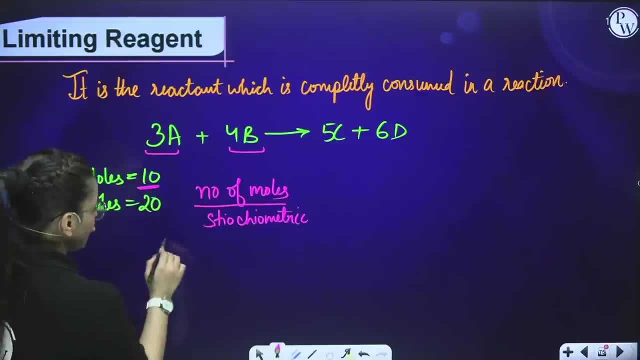 Now for 3A. number of moles of A is 10. divided by stoichiometry is the number in front of the reactant. It is 3. for B, The number of moles is 20 and the stoichiometry given here is 4.. 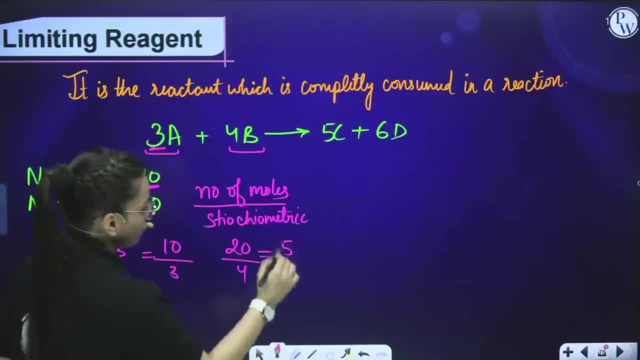 It is equal to 3.3, something, and it is equal to 5.. So which amount is less? obviously this amount is less. this amount is less. That means it is limiting reagent. It is our limiting reagent which will help us to calculate the values of the product. 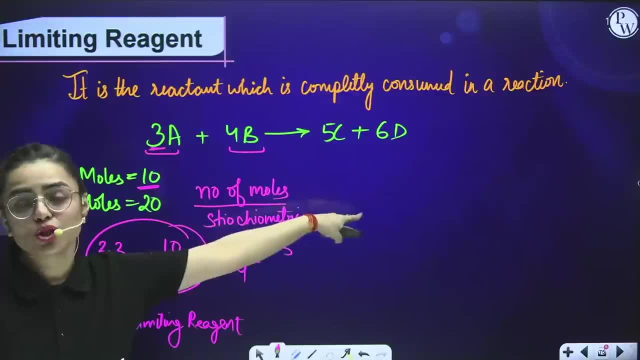 Now I ask you: what is the amount of substance, What are the number of moles obtained of the product C? How can you calculate? Will you take a? will you consider B? now, No, because B is present in excess and we will find question only through the limiting reagent. 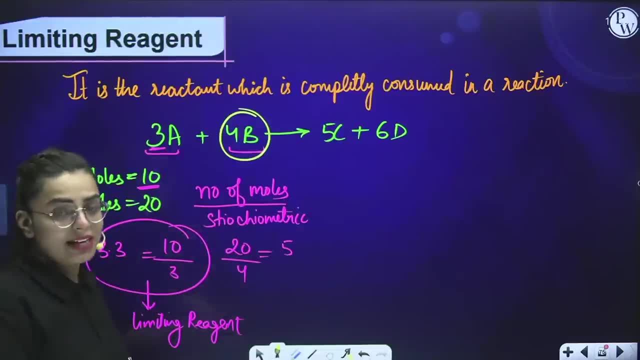 when two of the substances amounts are given to us. First we will find limiting reagent. How to find Divide number of moles by stoichiometry whose value is less? that is your limiting reagent. Now we have found this already. 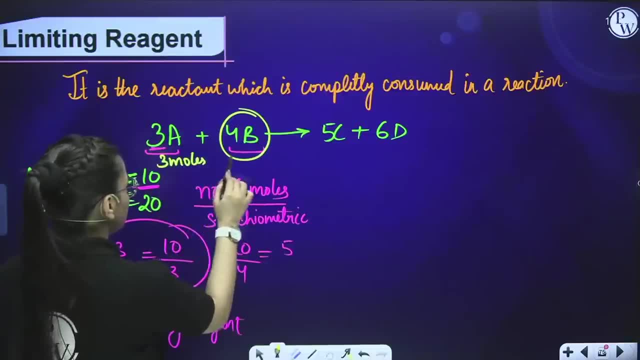 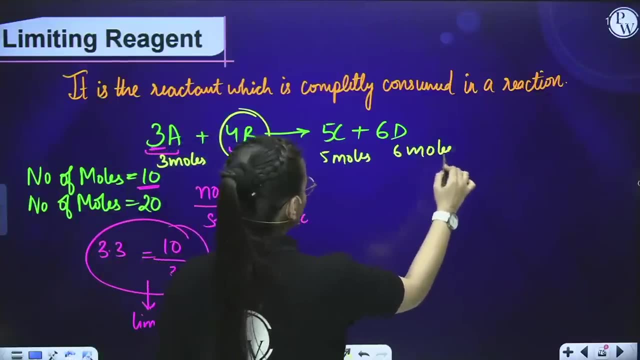 Now, as you know that this is 3 moles, This is 4 moles, This is 5 moles, This is 6 moles, as we have done in stoichiometry. Now, this will help us to find these right. 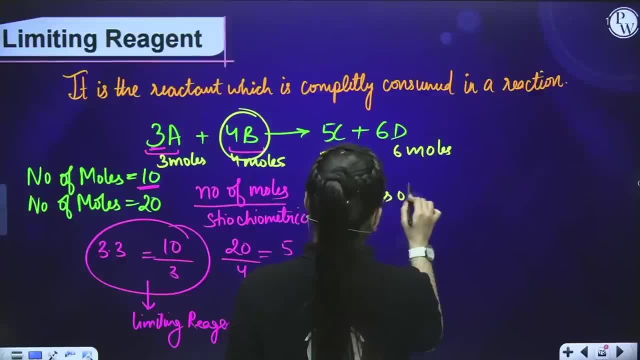 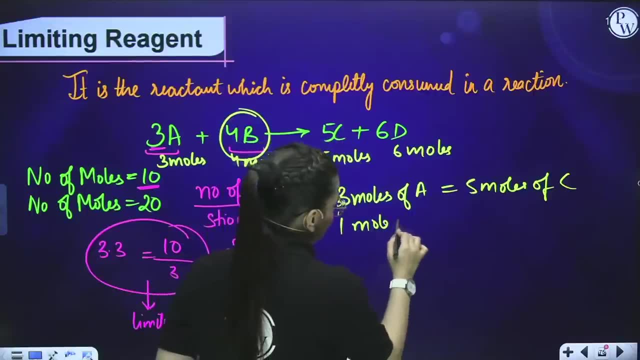 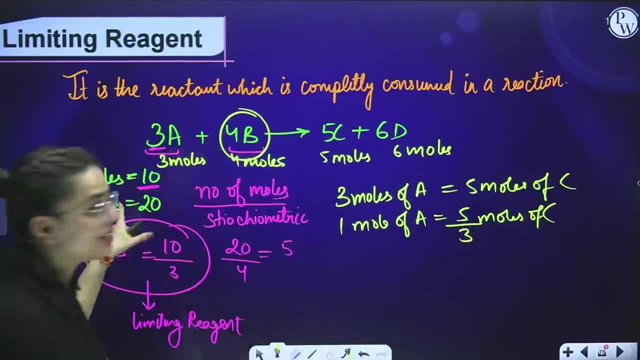 So I would say that 3 moles of A gives 5 moles of C right. 1 mole of A will give 5 by 3 moles of C right. So how many moles of A are given 10 moles right? 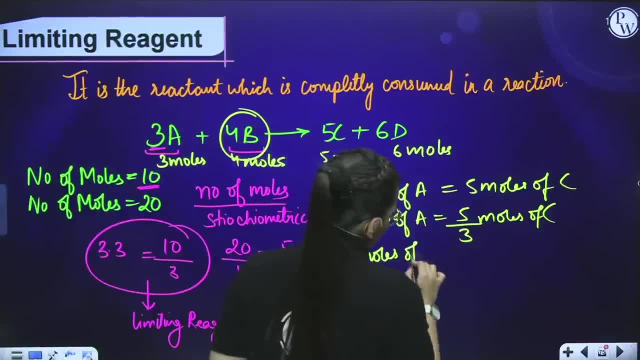 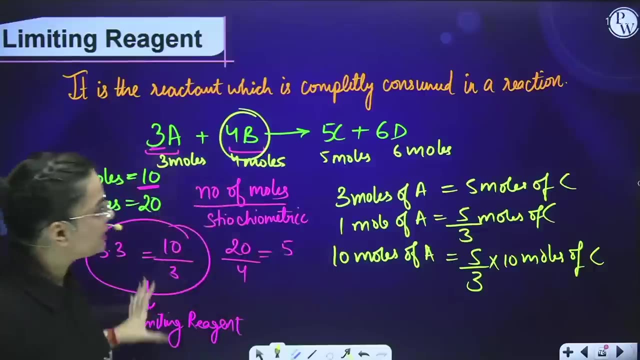 So 10 moles of A will give 5 by 3 into 10 moles of C, right. So by these we can find the number of moles. It comes out to be 16.66%, 66 value. So with the help of limiting reagent we can calculate any amount of the substance of the products. 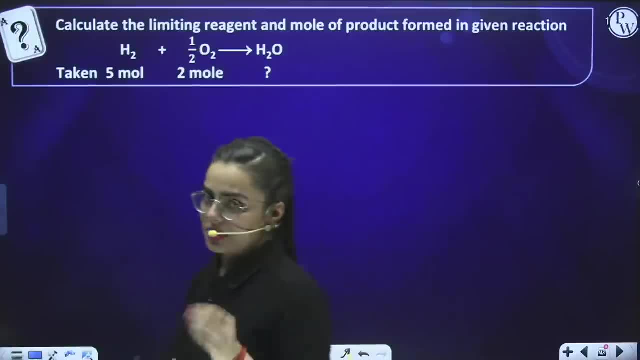 Clear students. now proceeding towards one of the questions, Let us see calculate the limiting reagent and the mole of product formed in the given reaction. We have H2 plus half O2 gives water. The first thing that we do is balance the equation. yet 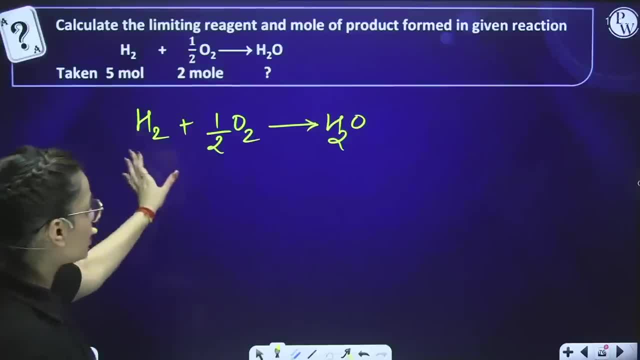 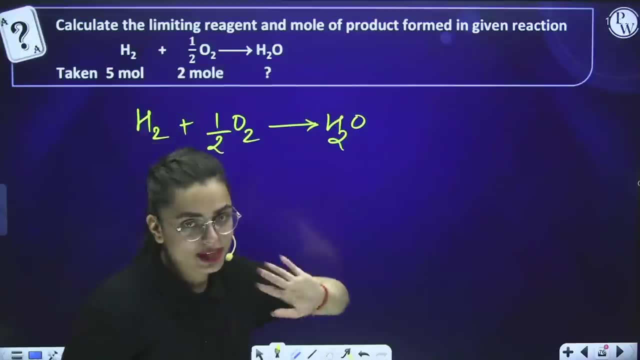 It is already balanced. here in the reactant side There are 2H, here It is 2H, here, O2 is, you know, 2 into 1 by 2 is 1 and here it is also 1.. It is already been balanced. 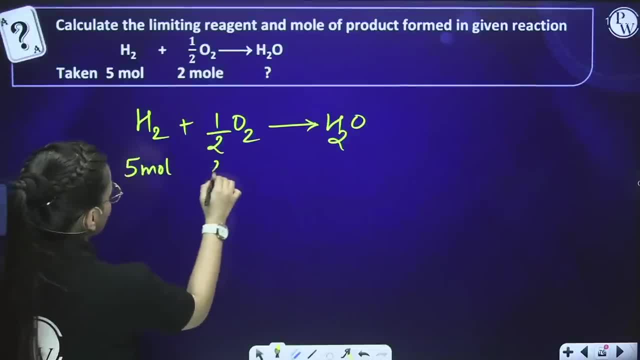 What we are given is: it is taken 5 moles and it is taken as 2 mole students. So what is the basic thing that we need to do is we need to divide number of moles by stoichiometry, number of moles by. 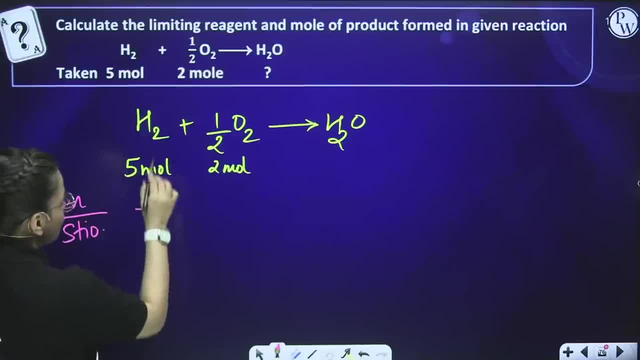 stoichiometry Coefficient. number of moles are 5 in this case. in stoichiometry, when nothing is given, It is considered at 1.. That means it is 5. now here: What is number of moles to what is stoichiometry half? 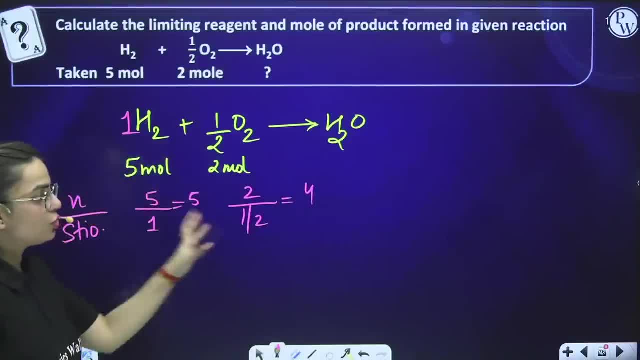 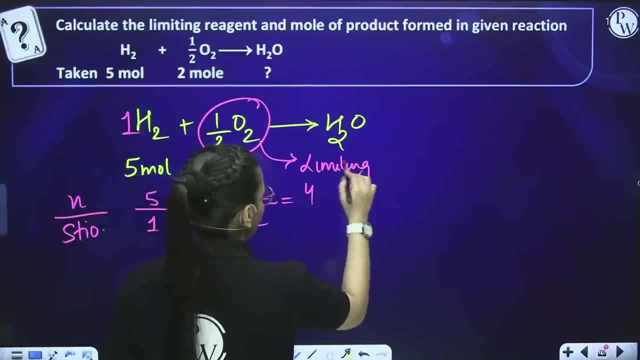 So it will go above and it will become 4 now from both of these, which is present in less amount. Obviously, this is present in less amount. That means it is referred to as limiting reagent. Now that means with the help of this we can calculate the mole of product formed in the given reaction. 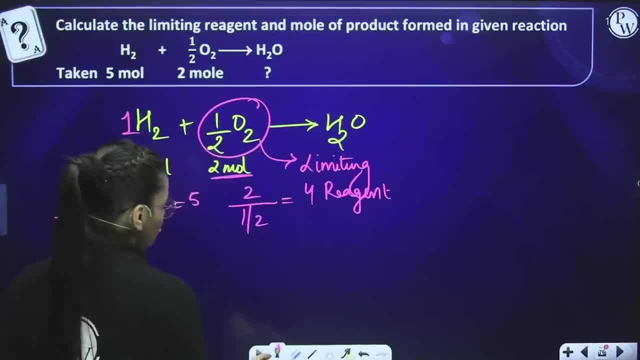 Now, if you see these are, these are already given to us as half moles and here it is 1 mole. the stoichiometry, So I would say half moles of O2, half moles of O2, gives 1 mole of water. 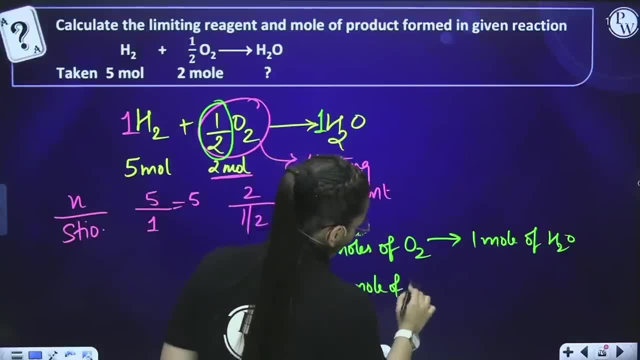 So 1 mole of O2 will give half mole of water Right And in other terms we need to calculate for 2 moles. So 2 moles of O2 will give half into 2 moles of water. That means how many moles of water are obtained. 1 mole of water is obtained. 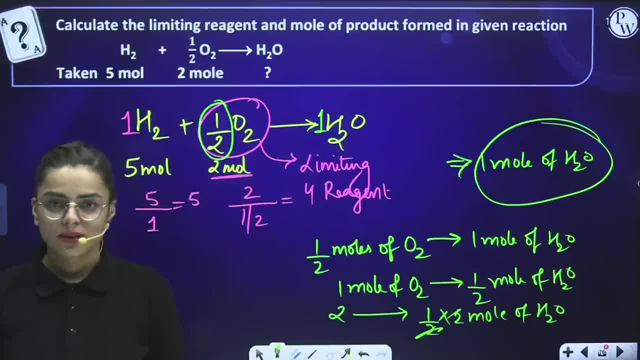 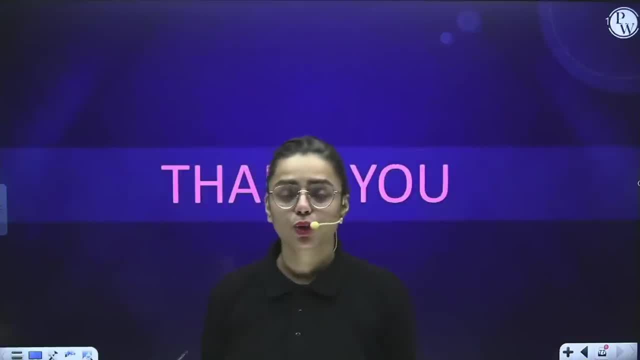 So by these you can calculate any of the questions. clear, students. So yes, my dear students, this chapter is finished here. Hopefully you liked the video, you like the chapter. Now the basic thing that you need to do is practice, practice a lot of questions on the topic wise, so that you can be perfect in every topic, in every aspect of some basic concepts of chemistry.